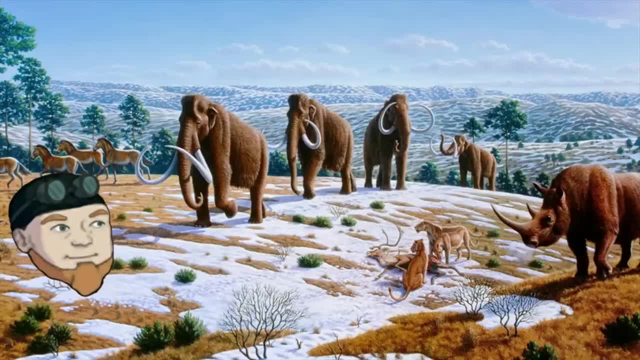 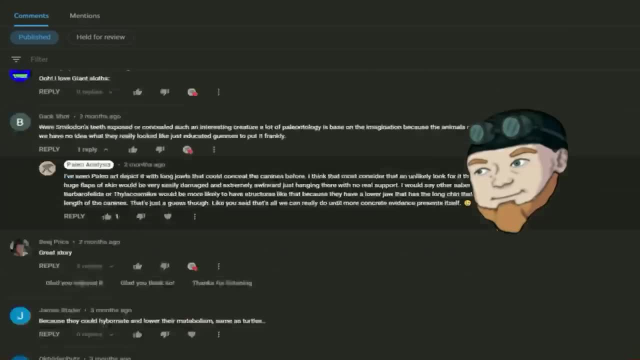 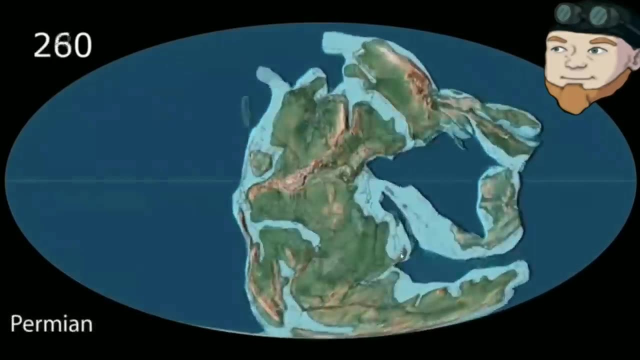 history. I got a lot of comments just saying: talk about the Pleistocene or talk about the Triassic, which I've already done quite a bit now- or talk about the Devonian. Okay, and all this kind of got me thinking What if I do all of it? What if I made a series of videos where I basically broadly 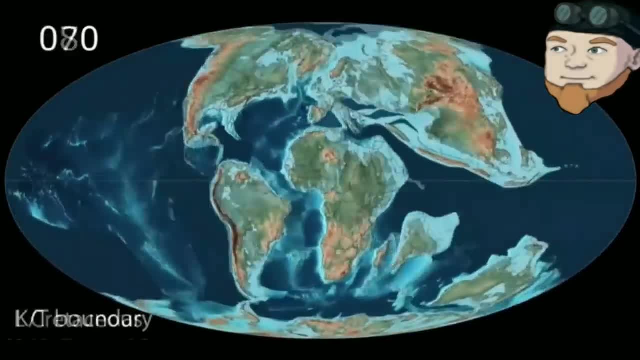 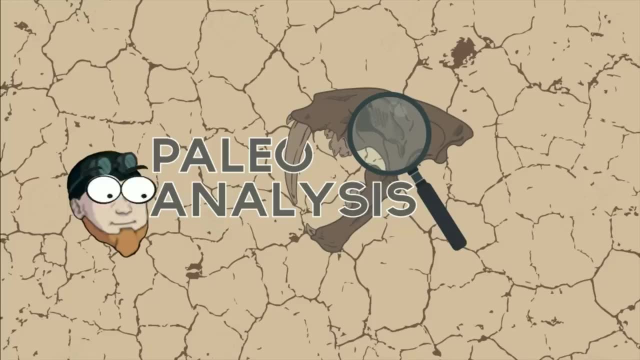 cover the lore of the Earth from the beginning all the way to the modern times. So that's what this video is going to be the start of, And I know that, starting at the very beginning, this video might not exactly rank in search, since it's probably going to feel more like an astronomy. 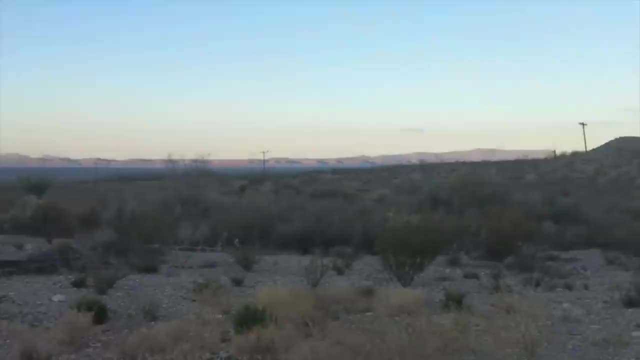 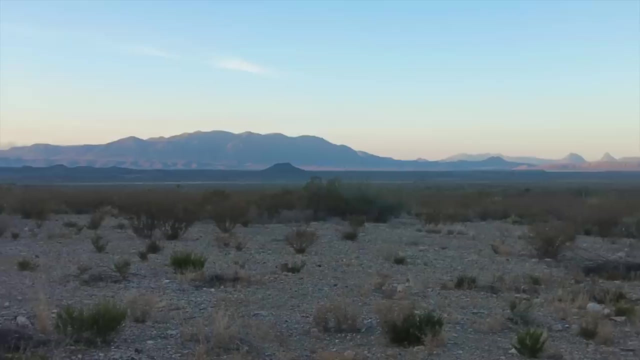 or geology video than a paleontology video. But eventually I'll be able to say that I've given a timeline to Earth's history that I can reference in future videos, And for this one I want to start with a little bit of context and then I'll be starting at the beginning, then going from there. 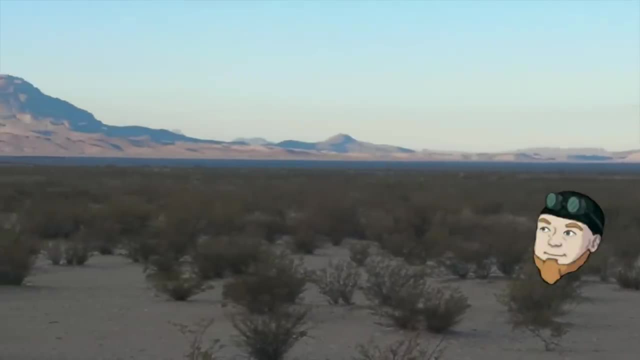 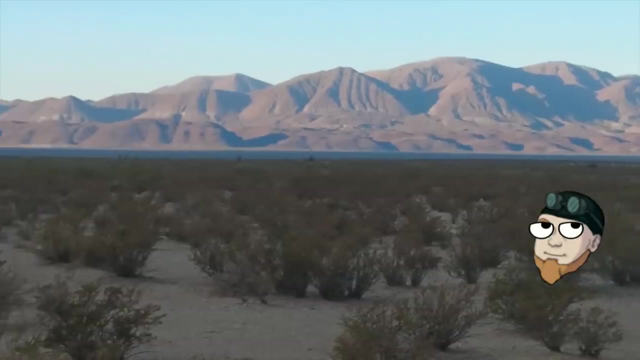 And this doesn't mean that this is what I'm going to be doing every single week, Just something that I'll be adding a video to every so often, Basically just whenever I either want to, or any time that I can't think of anything else to talk about. I'll plug one of these in, But with 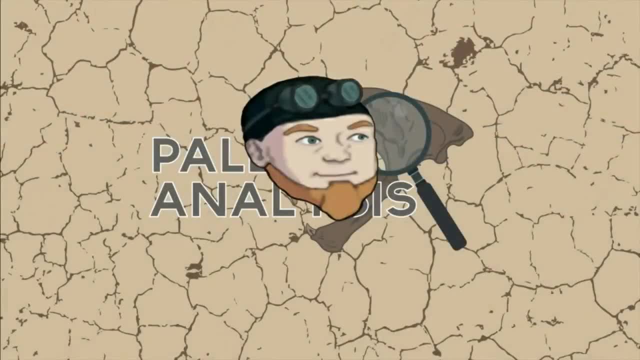 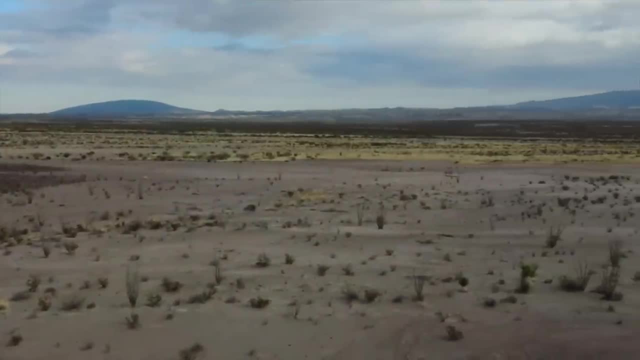 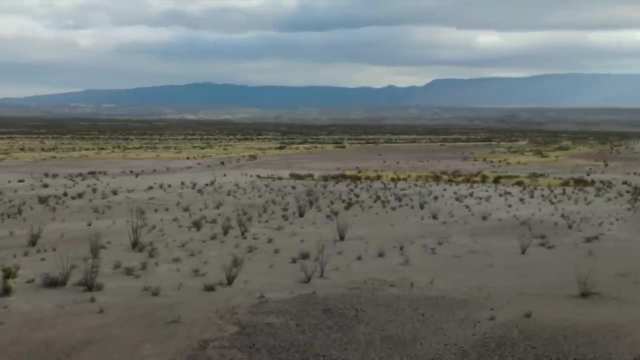 all that out of the way, let's get started with a little bit of context, A little something to lay out the chapters of this story. So before we really get into this, I think I should probably explain a few things. for those who don't already know how geologic time is measured, The history of the Earth spans roughly. 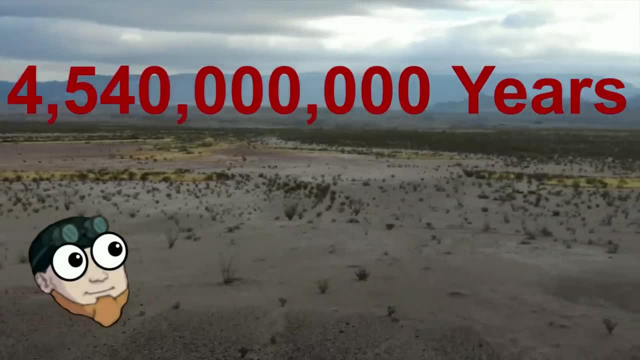 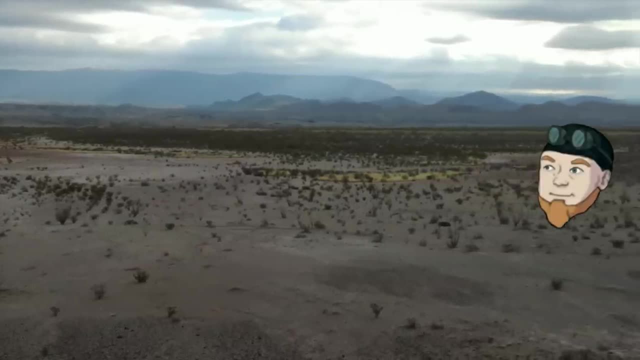 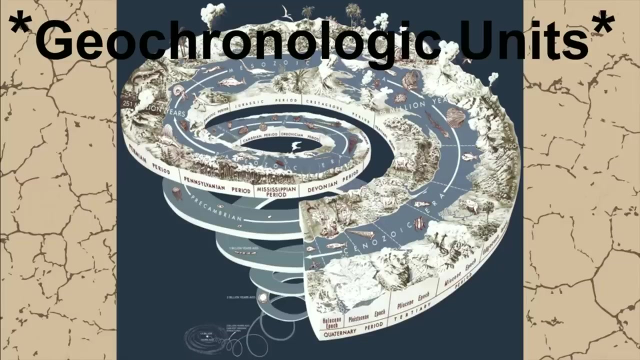 four billion five hundred and forty million years. This is an absolutely unfathomable amount of time. So to be able to help wrap our heads around something so vast, we've organized the history of time into several different chronological units, or geo chronological units, if you will. The smallest 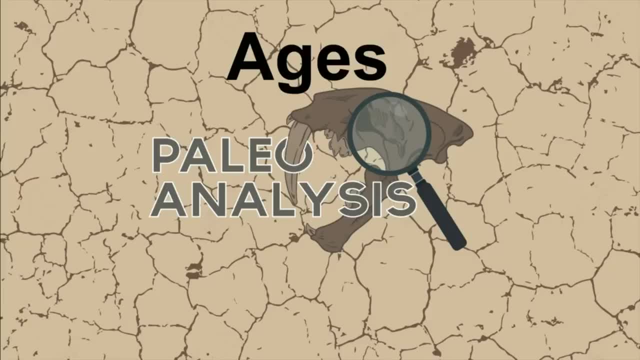 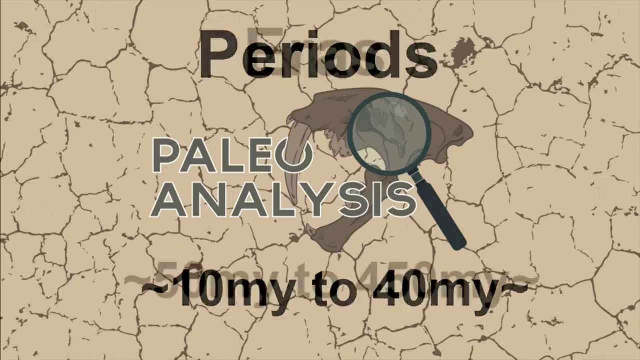 unit of measurement that we'll be using is ages, Although there isn't a hard and fast rule to this. ages are generally measured in up to millions of years. Epox are normally measured in several million years. Periods are normally measured in tens of millions of years. Eras are: 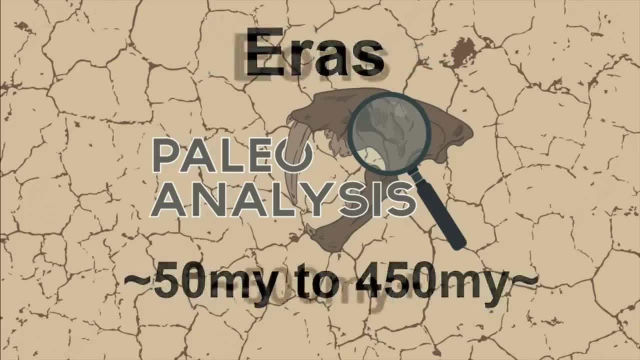 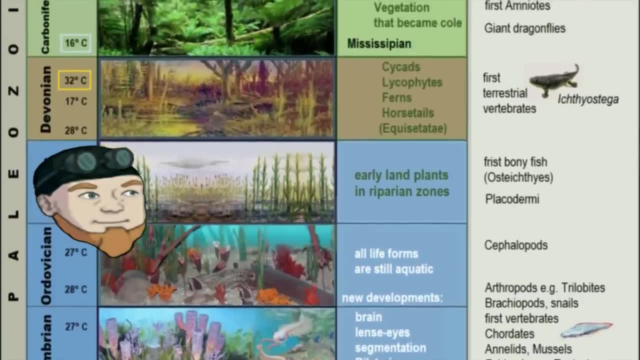 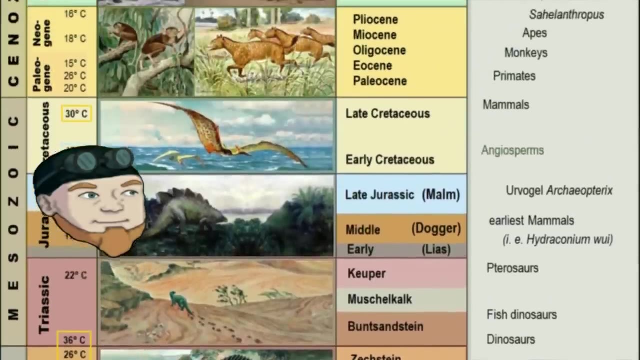 normally 50 to several hundred million years. And finally, Eons normally cover half a billion years or more. Now, as we move forward through time, you'll start to notice that I start covering smaller and smaller sections of the timeline. This is because the farther back in time you go, the less complete our geological record is. 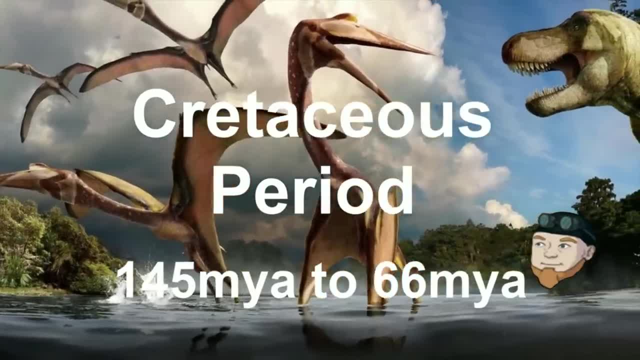 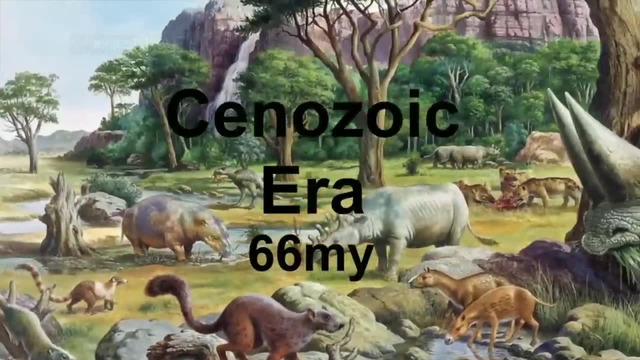 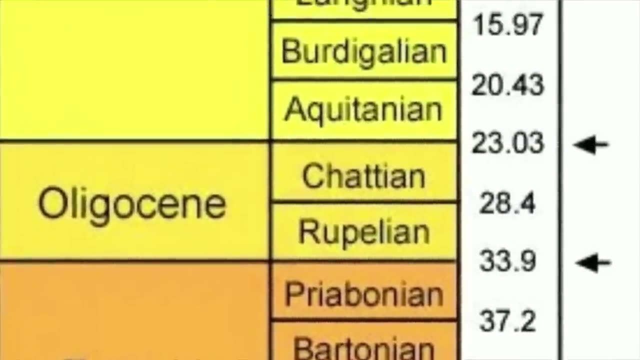 For example, the Cretaceous period lasted from 145 to 66 million years ago, so roughly 79 million years. This is a longer span of time than the entire Cenozoic era. This is because the Cenozoic is chopped up into smaller measurements, since we have so much more data to identify if a span of time is different enough to warrant a division. 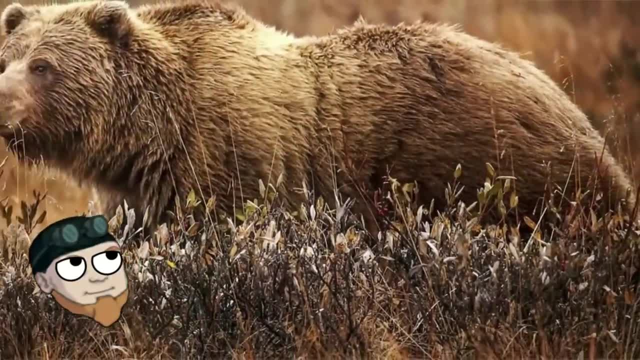 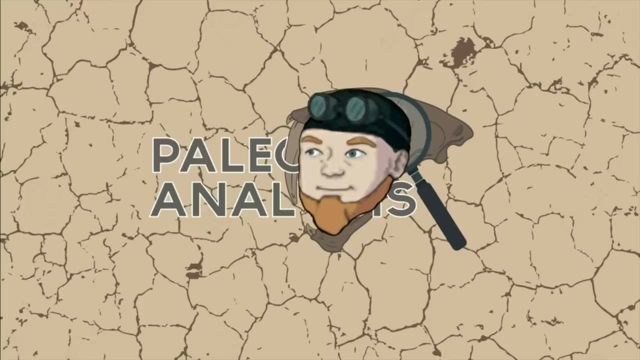 Well, that, and the fact that the Cenozoic is not actually over yet, But this is just something to keep in mind while I tell you all the story of where everything on Earth came from. And to start that story off, I'm going to have to go all the way back. 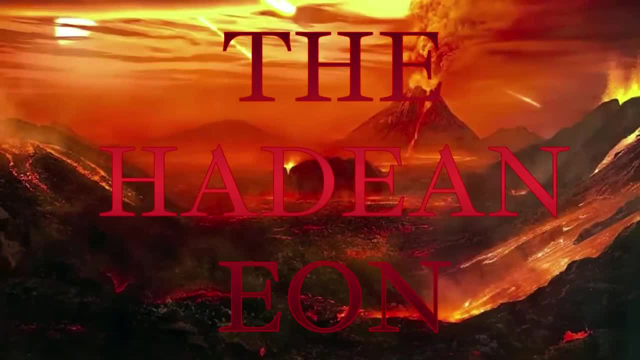 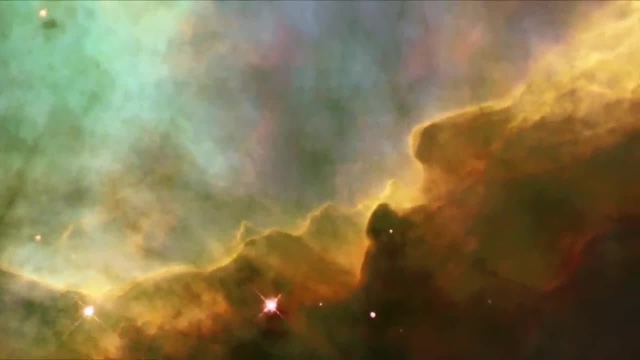 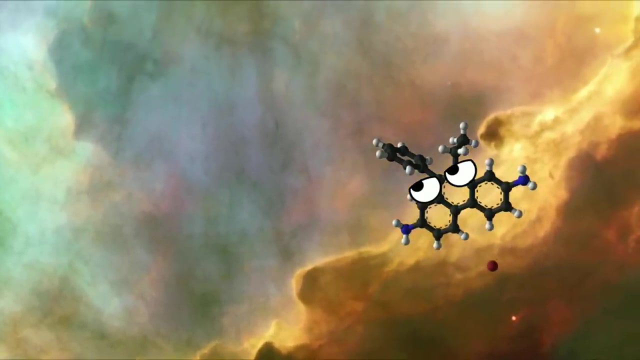 The story begins with a giant molecular cloud swirling around the Milky Way galaxy around 4.6 billion years ago. Yeah, I did say I was going all the way back, didn't I Wait? Oh God, I've gone so far back in time that I'm an ethidium bromide molecule. 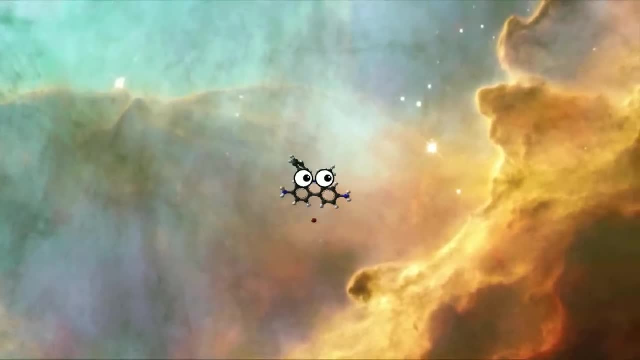 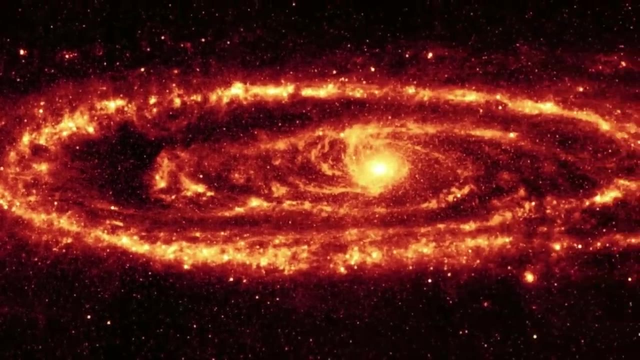 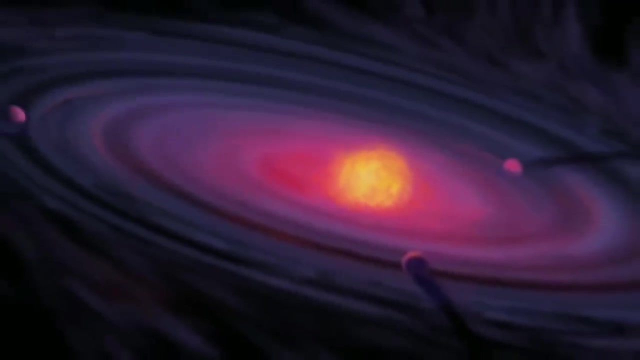 I'm literally a building block of life. Nooooooo, As the cloud spun, gravity started to make the heaviest materials gather in the center, while the rest started to form what's called a protoplanetary disk. And, as you might have guessed, eventually the mass of ultra-heavy material became our Sun. 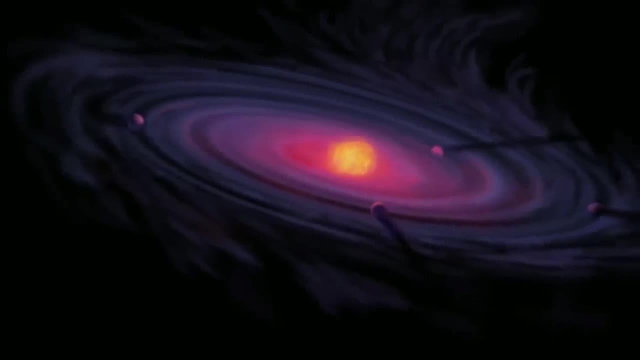 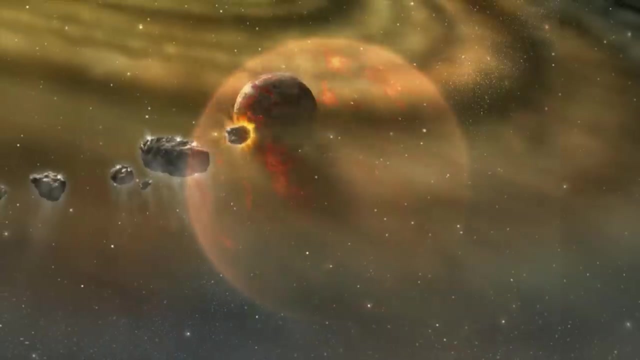 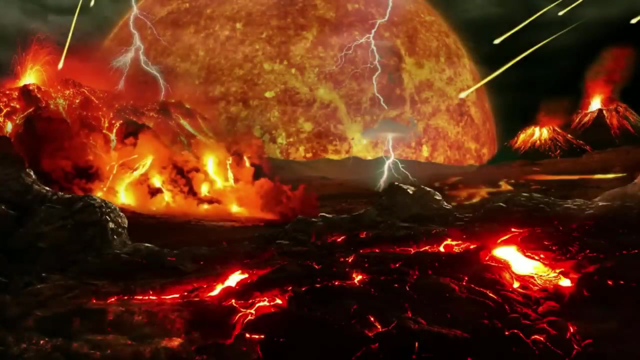 and the dust and particles that made up the disk started to form the newborn planets and other celestial bodies, And during this time our planet was born, Originally just another unassuming world floating around a new star, And currently Earth is about as far away from being recognizable as it ever will be. 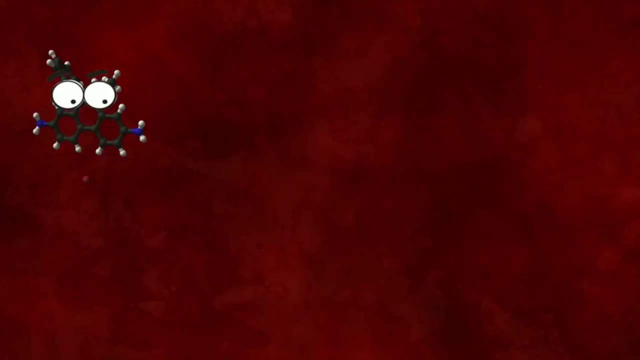 In fact, it probably looked more like Mustafar from Star Wars. So hellish was our future home that this entire aeon was given the name the Hadean. And yeah, it's actually named after the Greek god of the underworld, James Woods. 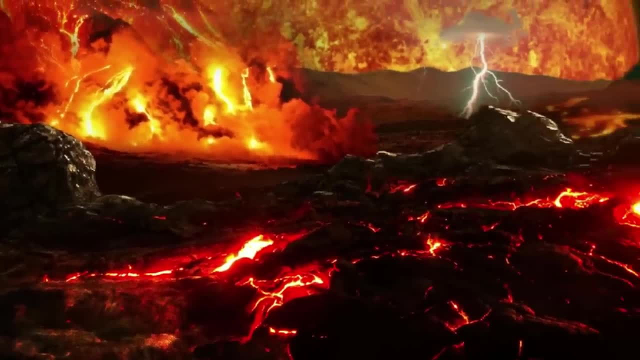 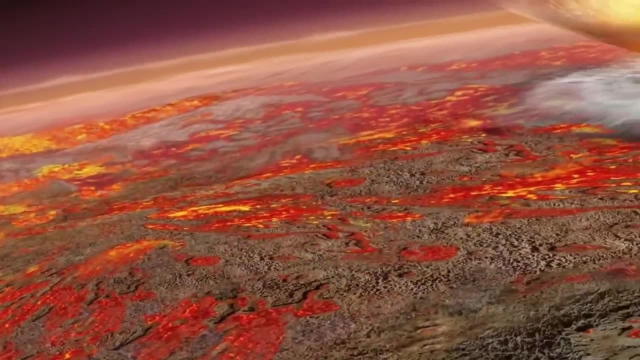 It was literally hell on Earth, in the most literal sense, for the majority of the first 600 million years. And to make things even worse, because there was so much other stuff out in the rest of the solar system forming, there was a lot more objects crossing paths in the form of impacts. 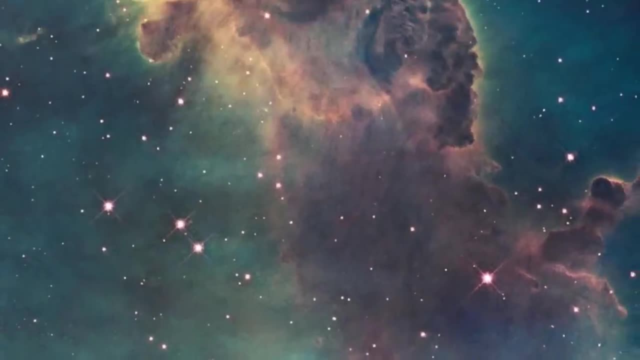 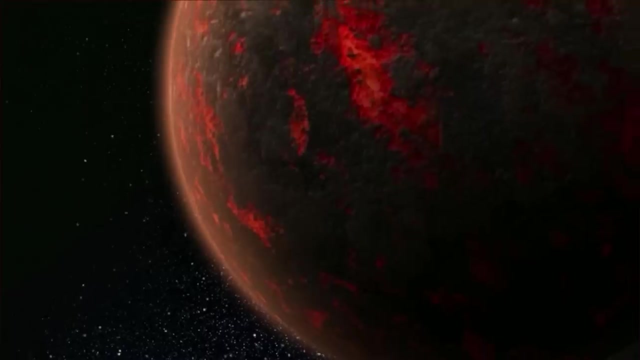 And sometime within the first 100 million years, the Earth is believed to have had an impact that would change the course of its future Around. this time, the Earth was starting to cool. However, it was still a hellacious ball of rock with very little chance of life ever forming. 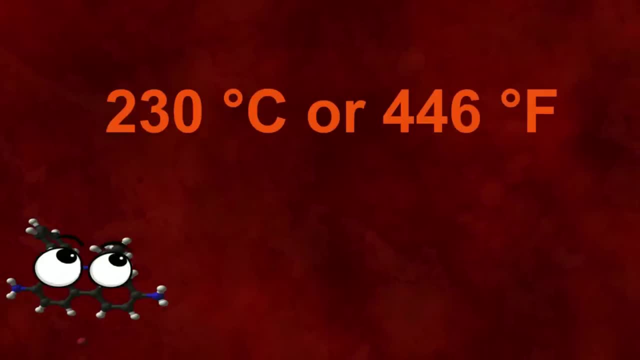 The average global temperature was around 230 degrees Celsius or 446 degrees Fahrenheit. However, many of the densities of the Earth's surface, including the Earth's surface surface, were completely destroyed. However, many of the densities of the Earth's surface, including the Earth's surface, were completely destroyed. 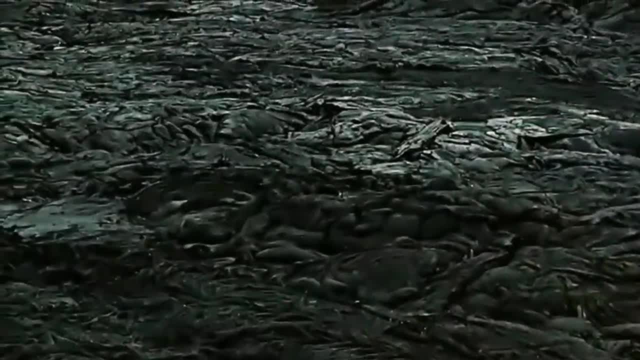 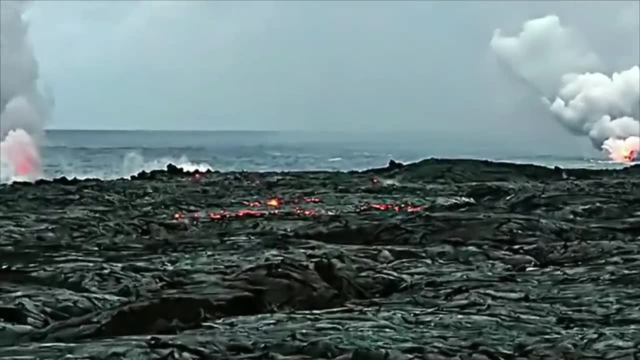 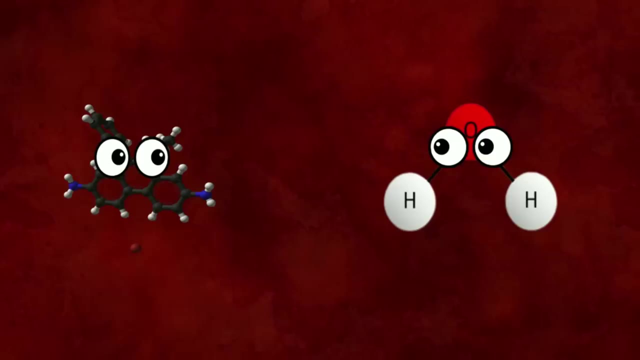 But even then the Denser materials were starting to solidify. However, there was one element that was only able to condense to liquid form because its temperature to form solid was down at 32 degrees Fahrenheit: A compound of Hydrogen and Oxygen. that would become the single most abundant ingredient in the recipe of life. 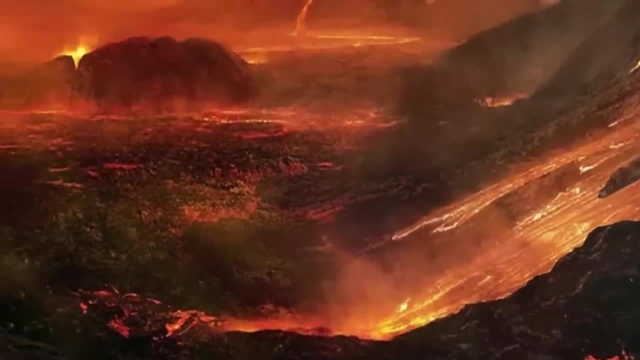 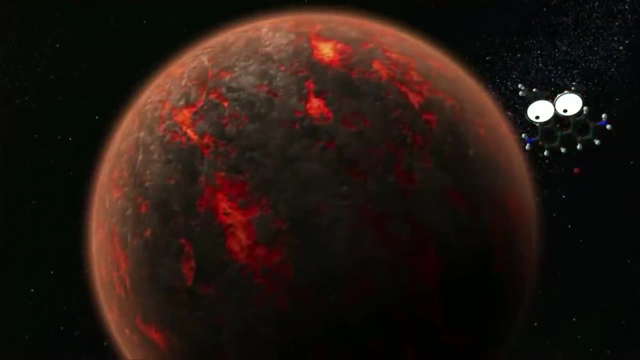 Water, And the only reason why it was even able to form a liquid is because the atmosphere was 27 times as dense as it is today. And it's very simple thing, huh. But how did it become a liquid And how did it become a wave? 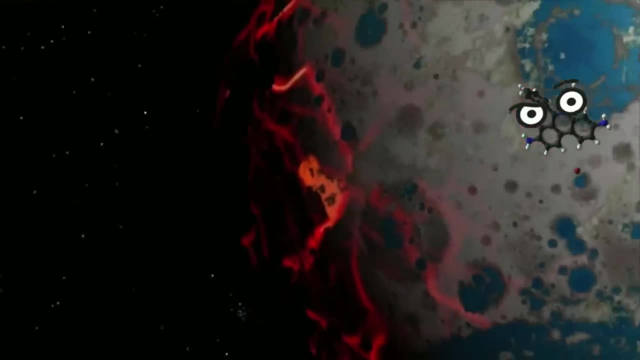 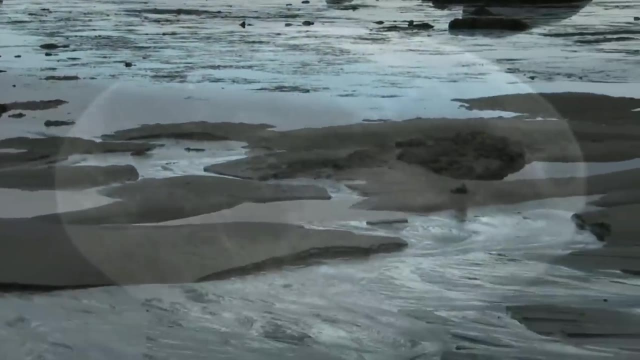 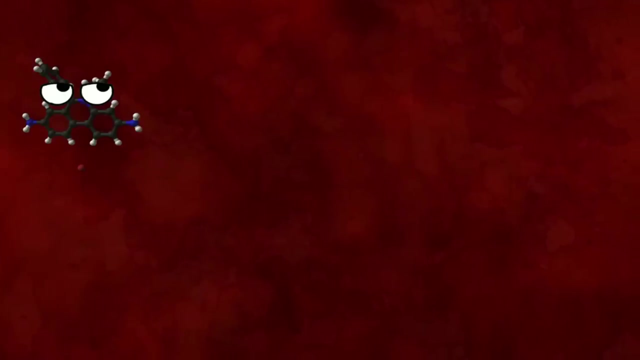 even get there? and, what's more, how do we even have the tides? there was no way for the tides to form because there was no object close by to create a gravitational pull needed for it. that is until a stray planet straight up t-boned us. yeah, i know, it sounds like some star trek grade stuff right now. 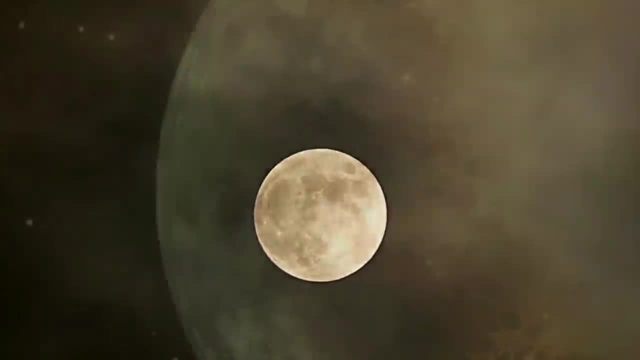 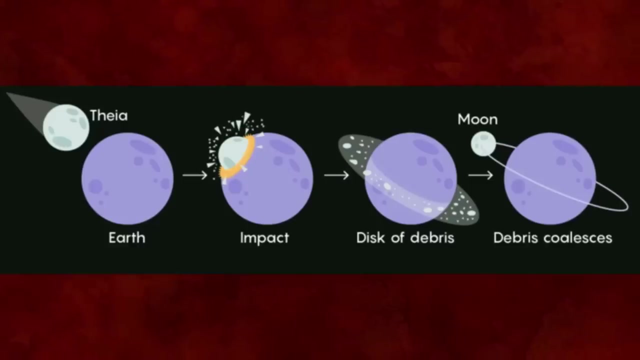 but the most plausible theory to the moon's origins is that it was formed from an impact between the earth and a planet that we now call thea. it's believed that part of thea remained in our orbit, as some of it was ripped away and added to the big ball of clay that we call home and the. 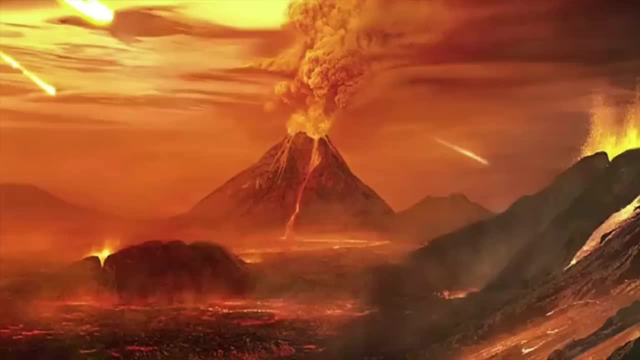 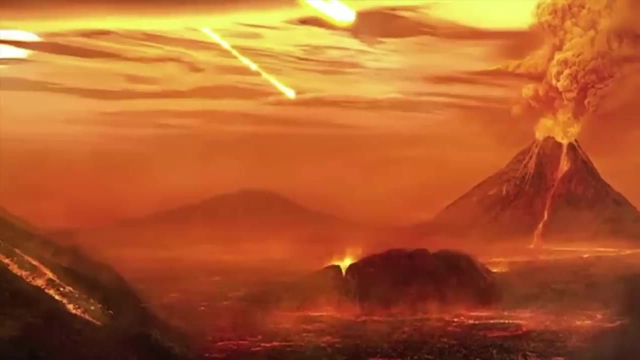 vaporized particles from this impact enveloped the globe. it was a combination of this with the helium and oxygen that had been slowly leaking away from the planet for the first hundred million years that we believe comprised our planet's earliest atmosphere, not one that we could currently breathe. 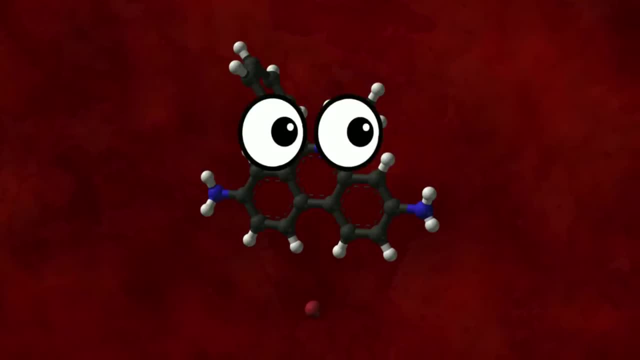 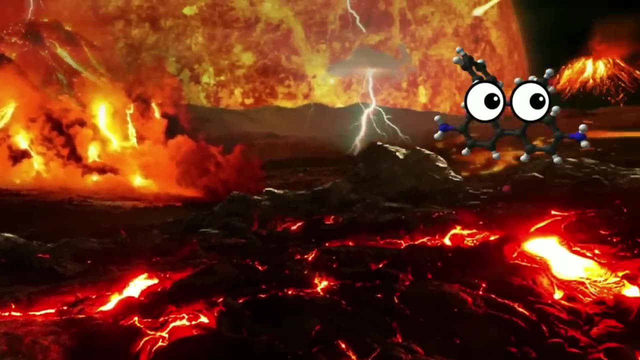 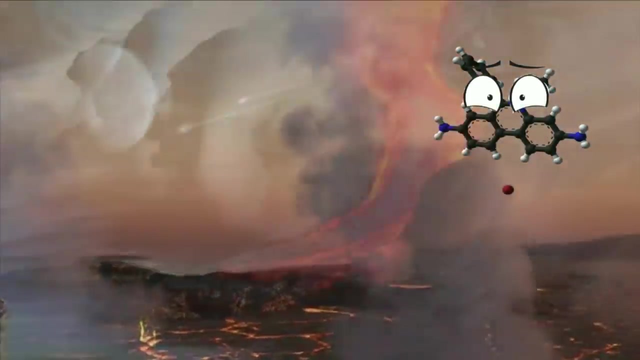 mind you you. this was the seed where everything really got started. so there we have it. just like that, the stage is set, even though the earth is still highly unstable geologically. there's a moon in the night sky, an atmosphere of mostly co2, sulfur and helium, and a tiny bit of liquid water in the lowest parts. 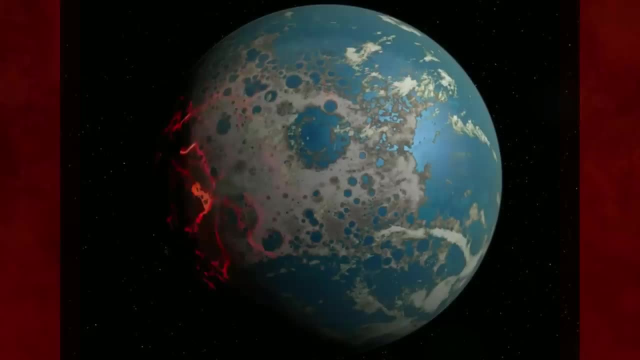 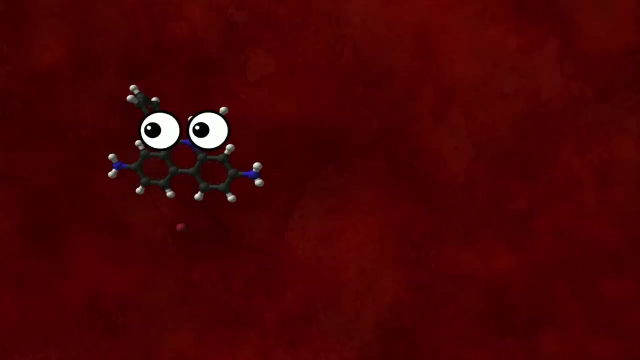 of our rocky world starting to really feel like home. but by the end of the hedian things were really starting to cool off a lot more, and this seems like a pretty good place to leave the story off because, honestly, there's still a ton we don't know about. this time there's only a very small. 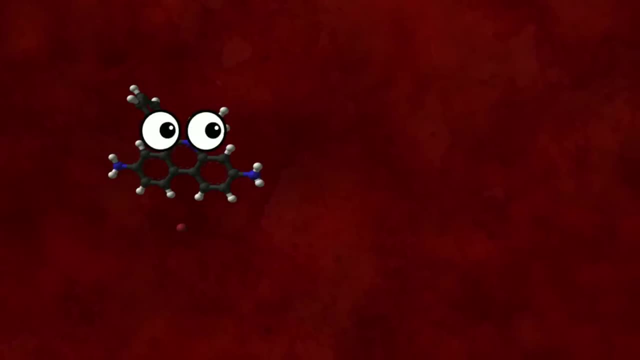 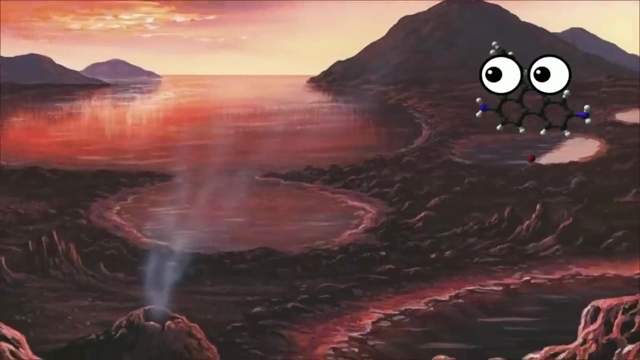 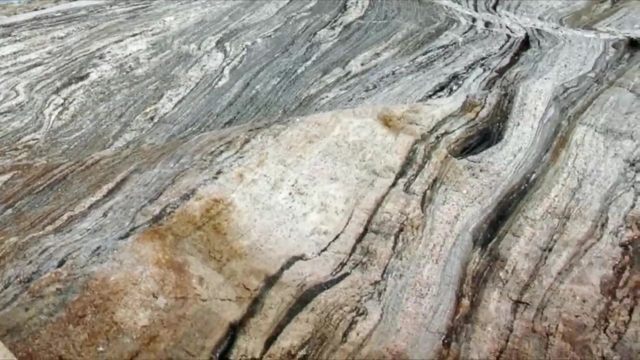 handful of locations where rocks that are this old even exists, because right where we're standing right now, at the end of the hedian, there's still 4 billion years that we still have to travel to get back to our time, and rocks just don't last that long on a geologically active world. so i 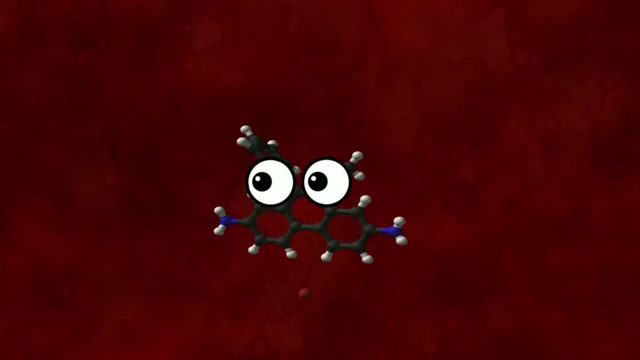 hope you enjoyed this first chapter in the history of our planet- if you did give this video a like, or. i'm really looking forward to continuing this story as well as continuing to make other videos about all different stuff, maybe in the next video i might actually get to cover something that's. 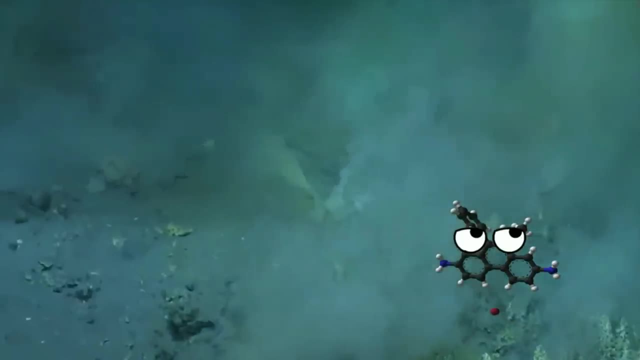 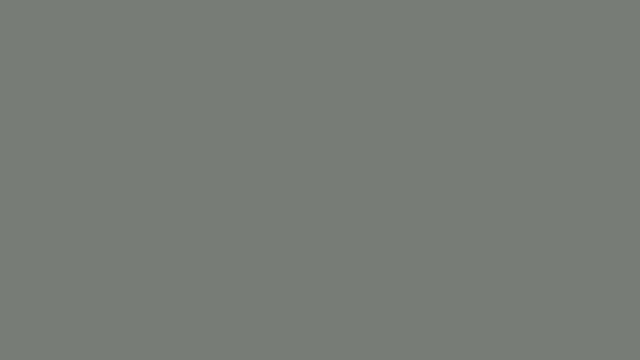 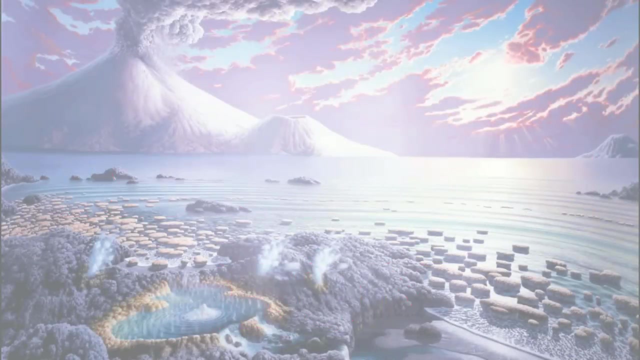 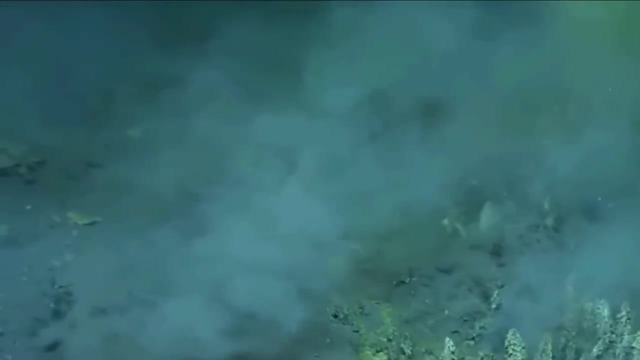 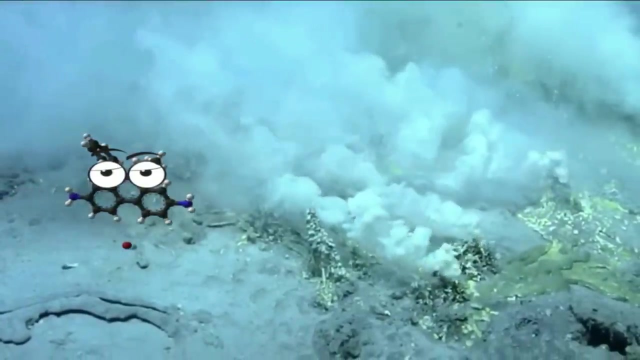 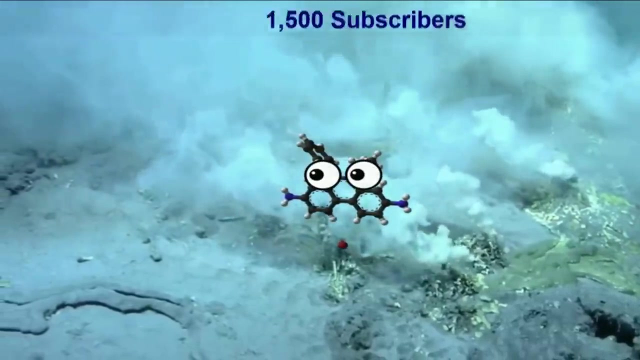 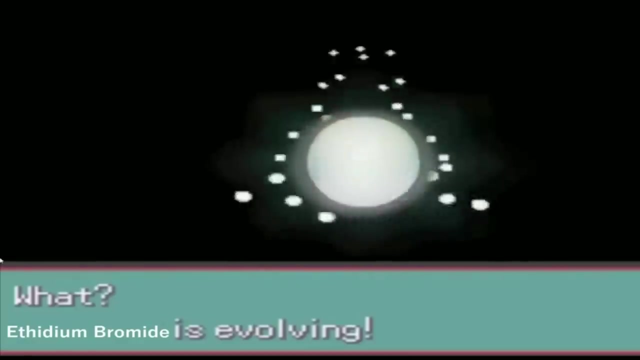 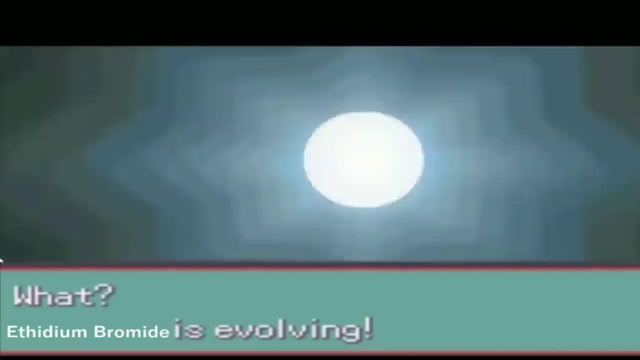 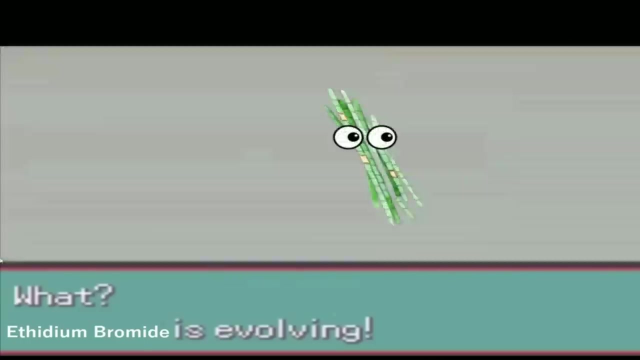 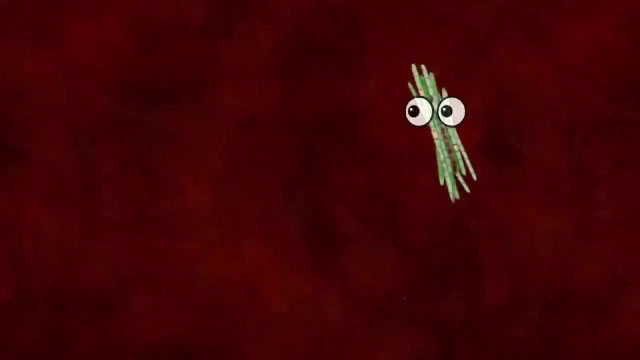 you know, alive. now, if you excuse me, i'm going to sit next to this hydrothermal vent and try to figure out how to turn back to normal. take care, everybody, and i'll see you guys in the next one. what the crap. oh so, in our last video we started our journey, exploring the complete history of life on earth. 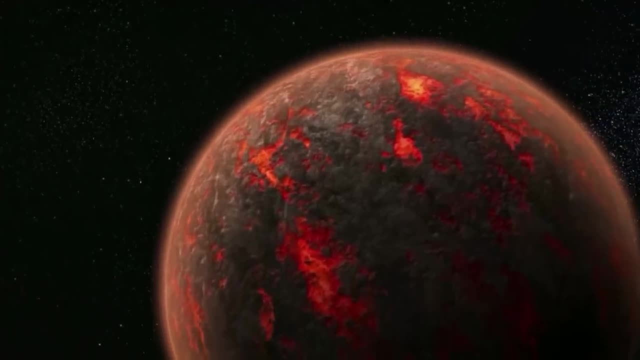 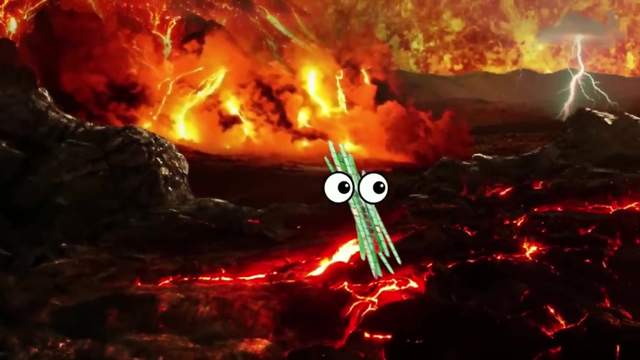 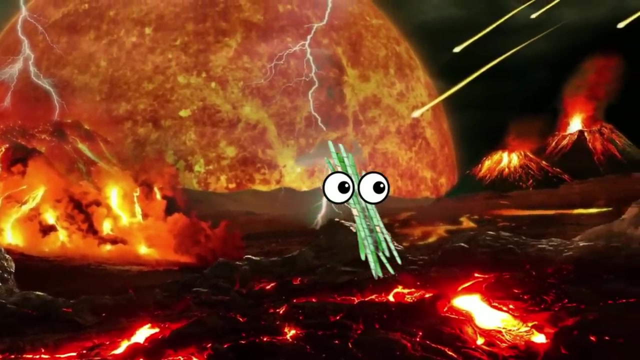 we talked about how our world was born, as well as what it was like for the first 600 million years of its development. in short, it wasn't pretty. lava, a toxic atmosphere and constant bombardment from other objects in the inner solar system were just part of daily life on earth during that time, but things were starting to. 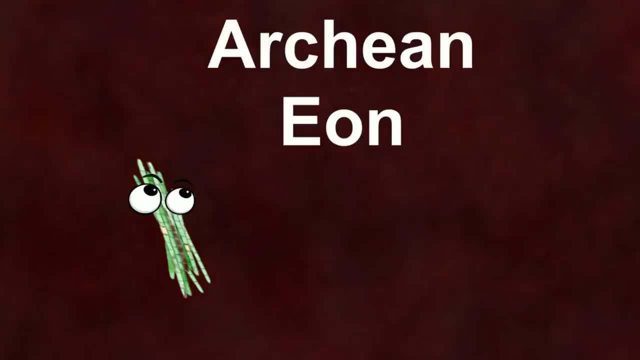 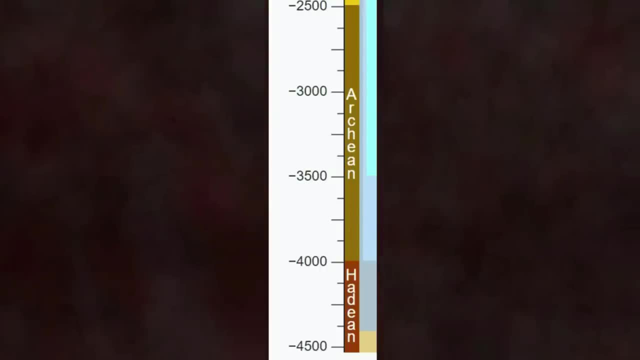 slowly improve on this little red marble as we enter the archaean eon, and this is a stretch of time that's three times longer than the stretch of time that we covered in the last one. by the time we get to the end of this video, we'll be about halfway through the complete history. 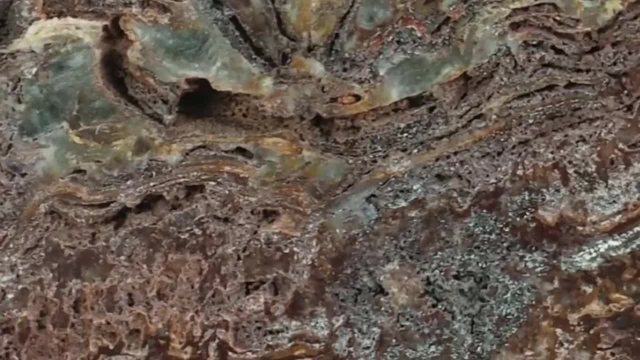 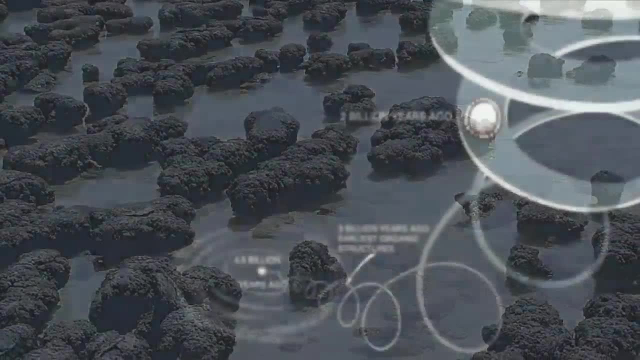 of the earth and luckily we have a little bit more information to go on than we did last time. but, as i said before, this will probably be the case with every video going forward, because the closer we get to the present day, the more complete our geological record is, and for the first time, we now 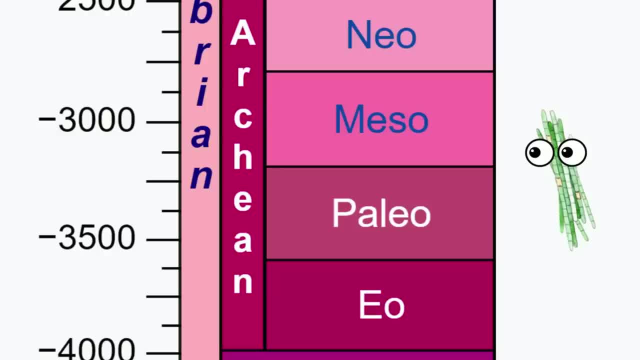 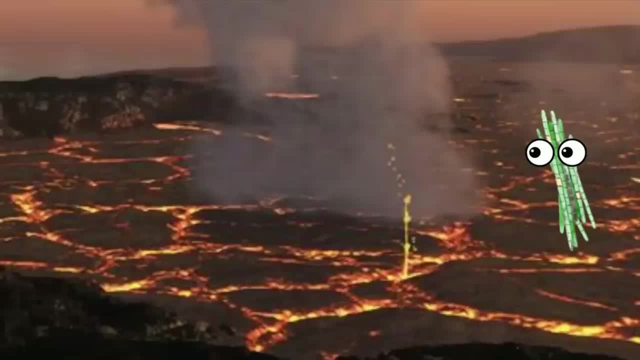 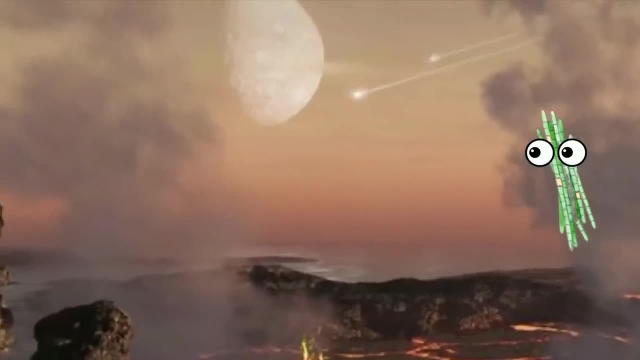 have enough data to actually divide this eon into eras. however, we still don't know enough about this time to merit giving each era its own individual video, but we'll get to that point soon enough. so now let's get into it, because we still have a long way to travel and before things get better. 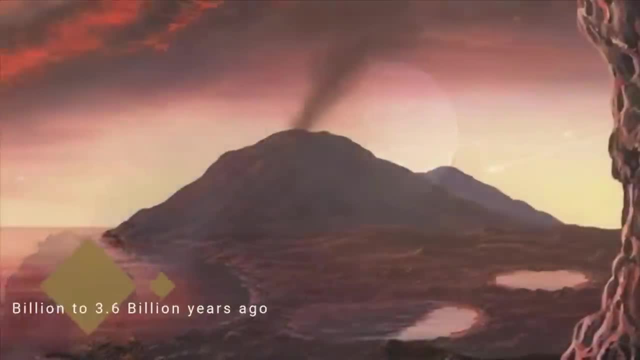 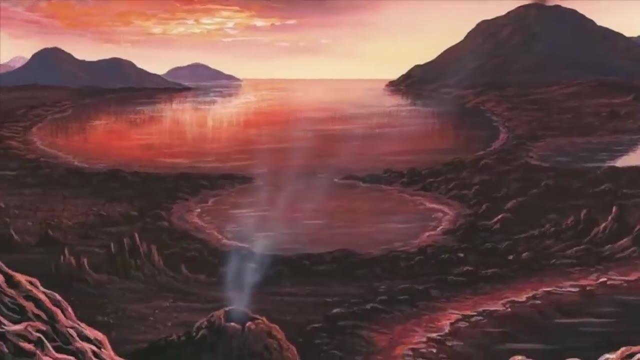 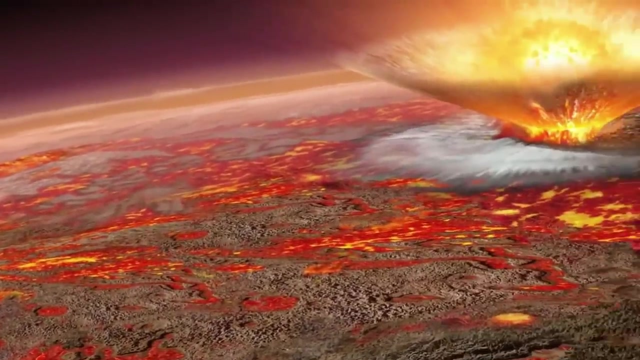 it looks like things are going to have to get a lot worse. the eo archaean began around 4 billion years ago, as the earth was in the throes of a major crisis. now we've already talked about how our planet has had to deal with constant barrages of impacts from 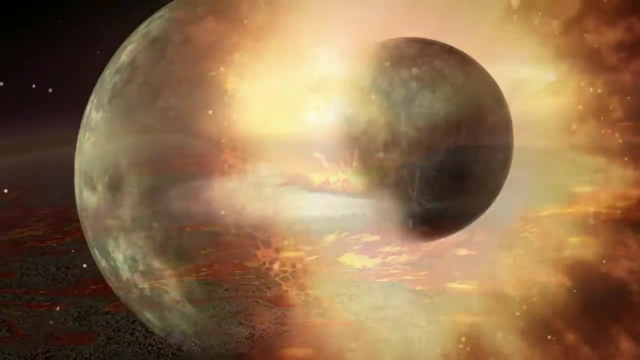 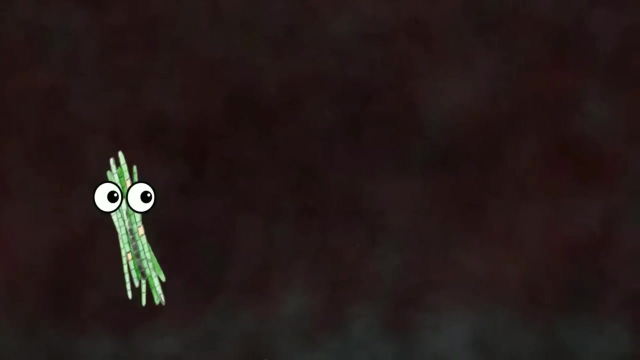 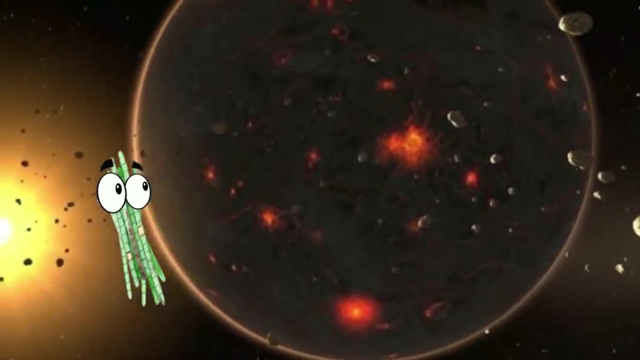 other objects in our solar system, including the major impact that would lead to the formation of the moon. but sometime before the end of the haitian, there would be a drastic increase in the frequency of impacts from asteroids and comets, so much so that, from 4.1 to 3.8 billion years ago, we 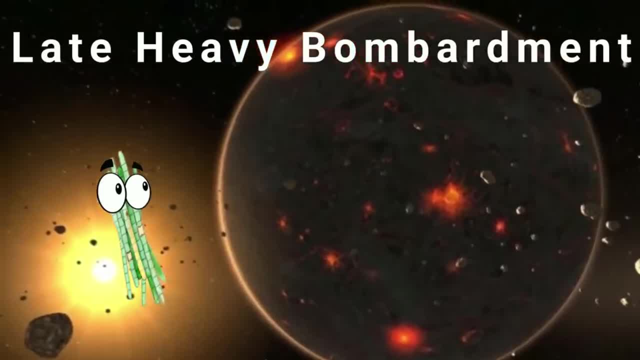 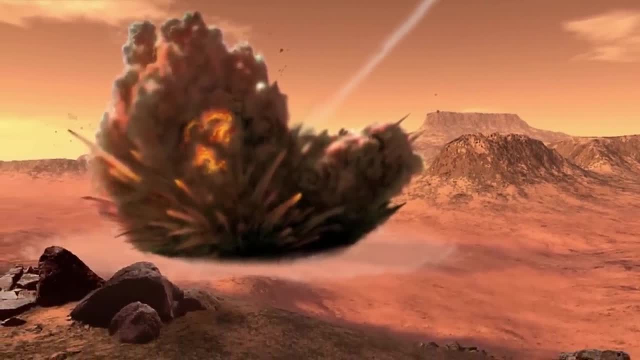 enter a time that has come to be referred to as the late heavy bombardment. some estimates calculate that there may have been as many as a few substantial impacts every millennium or so. this might sound like a bad thing, and it probably would be, had we actually been there to witness this. 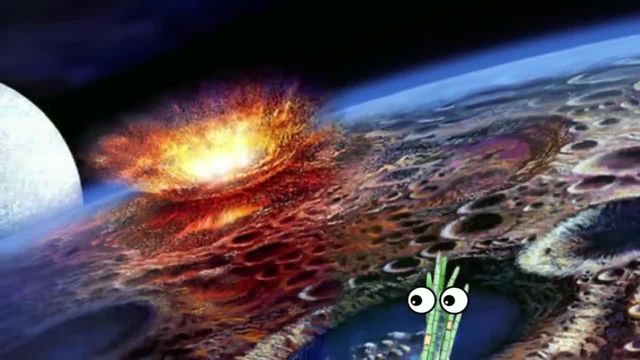 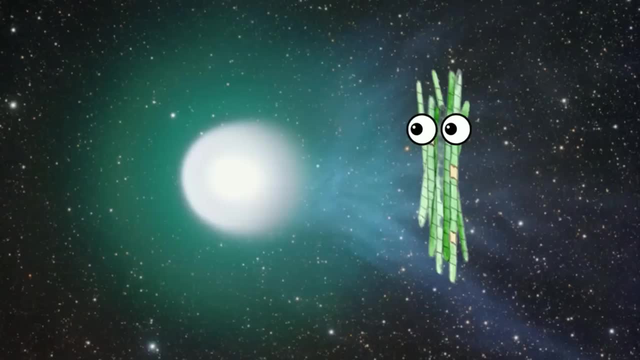 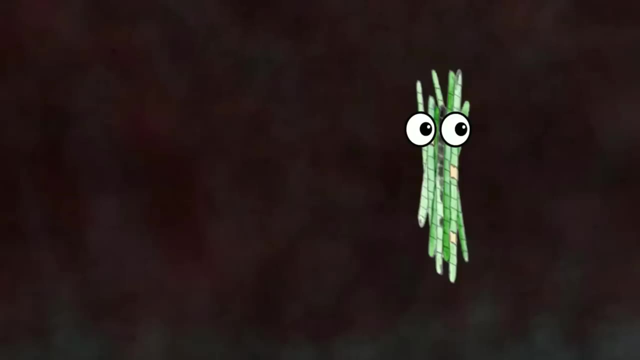 event taking place, but in all actuality, it may have had long-term effects that led to our world becoming one step closer to the earth we know today. you see, comets are not just solid chunks of rock, like asteroids. they're actually made up of mostly dust and ice and, as you may know, 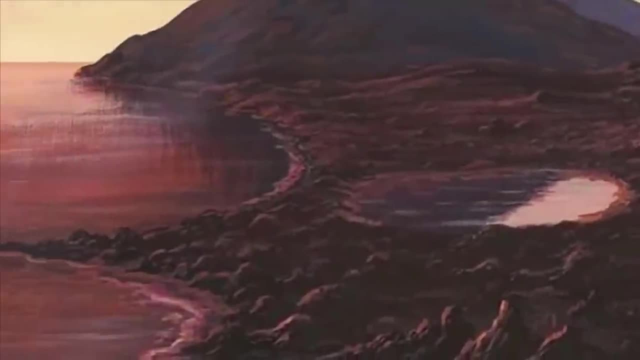 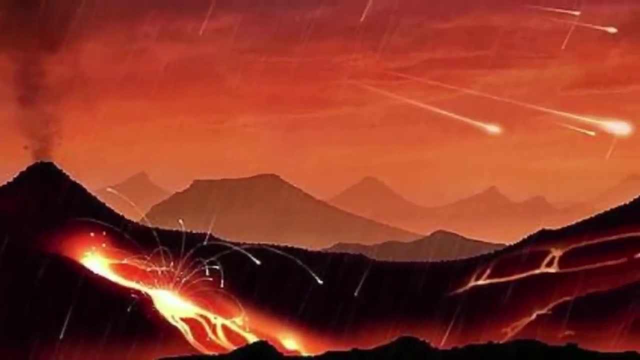 ice is frozen water, and although there was water on earth already, not nearly as much as a 70 that we have covering the planet today, it's believed that a large percentage of the water we have arrived in the form of cosmic snowballs being hucked at us every few centuries. now this is one. 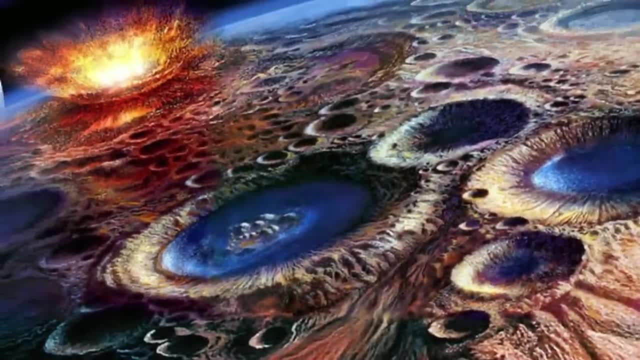 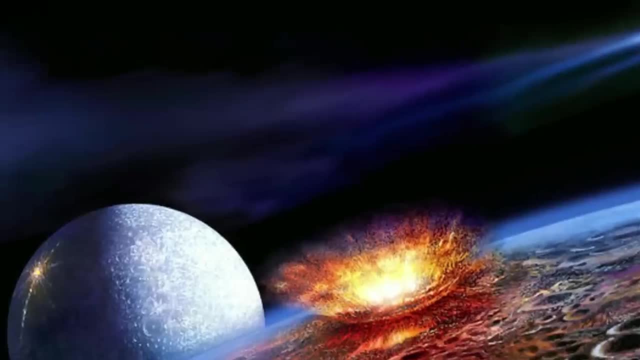 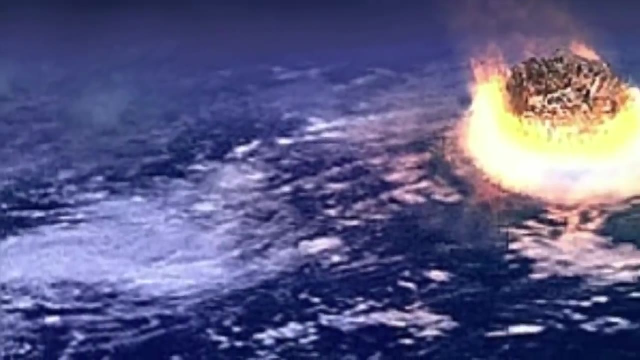 of the main things that scientists have come to define this era by, and even though this event would start to slow down by 3.8 billion years ago as the moon got further and further away from the earth, recent evidence has led many to believe that there may have been at least one impact around the 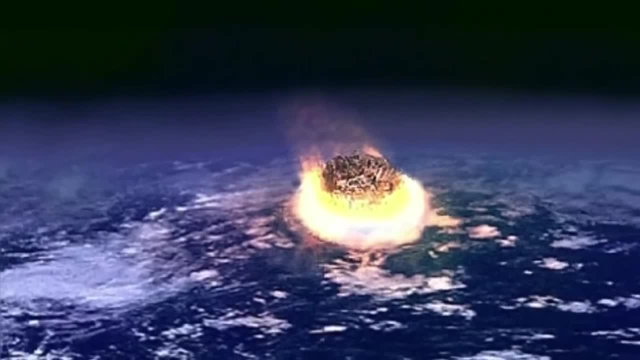 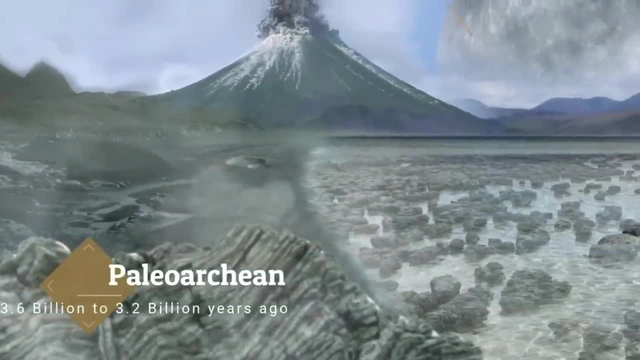 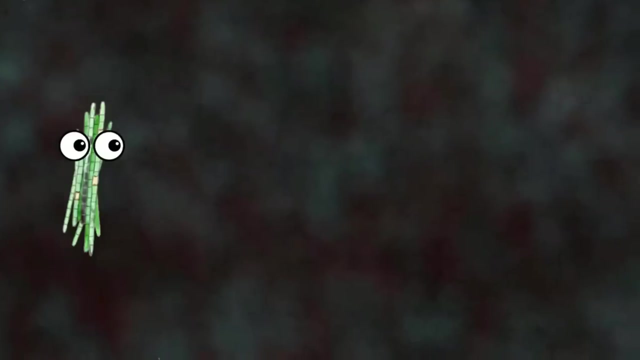 size of the one that wiped out the dinosaurs on average every 15 million years through the entire archean. starting at 3.6 billion years ago, we come to the paleoarchaean, an era lasting around 400 million years. this time has been defined by two major events that we know of so far. the first 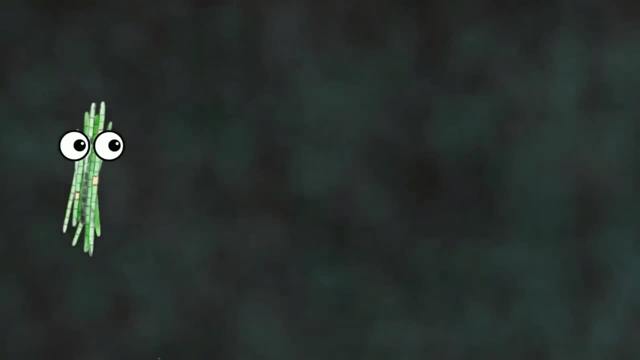 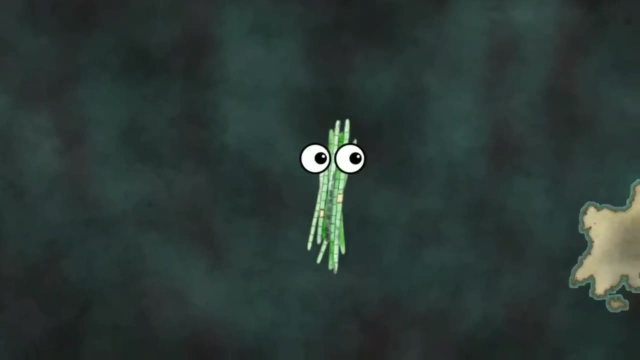 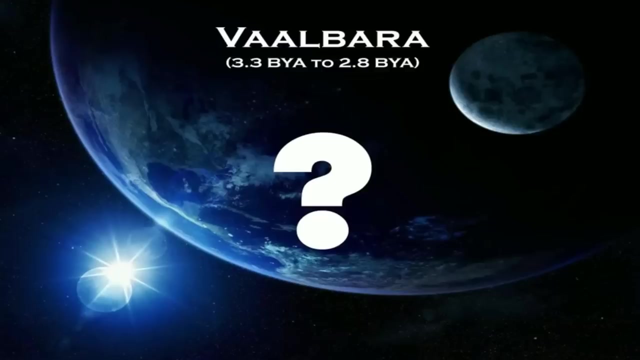 one being. as the sea level rose and the crust of the earth began to cool, the first large land mass would form. now, we can't know exactly what this land mass actually looked like, but we know that it was at least partly made up of western australia and south africa. it was given the name. 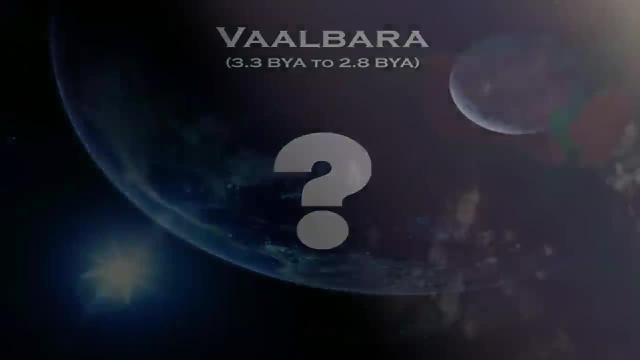 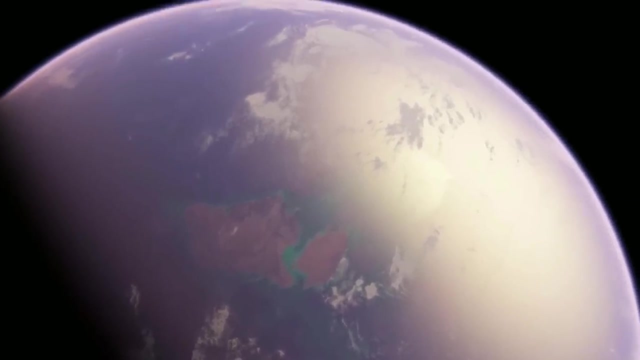 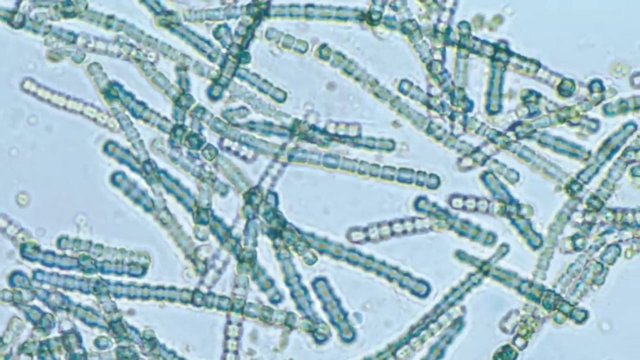 valberra and on its coasts would be the most important step in the history of our planet. yet we have at last arrived at the earliest evidence of life. now there's a very good chance that single-celled life had at least existed for millions of years before this, but this is the 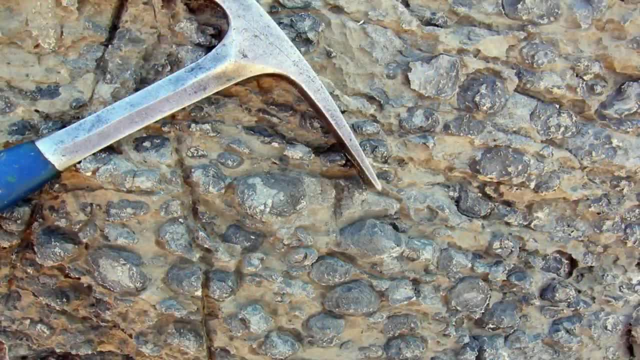 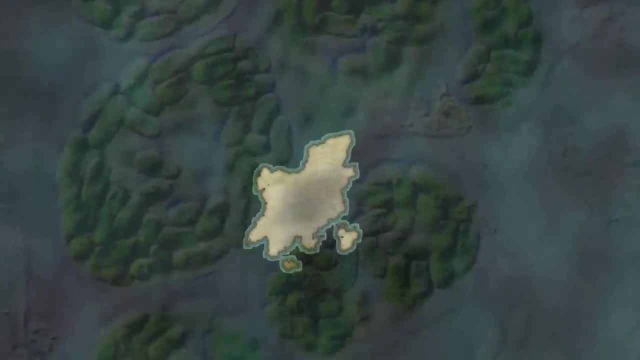 earliest evidence that has been found in the fossil record, and it might not seem like much, but it's believed that these little microbes called cyanobacteria would make a massive change to the entire world simply by doing what they do. for those of you who play spore, we've officially 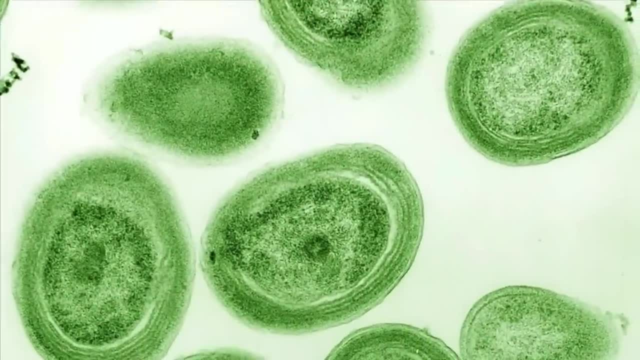 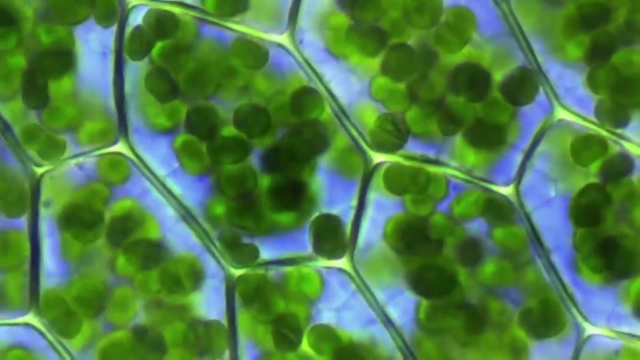 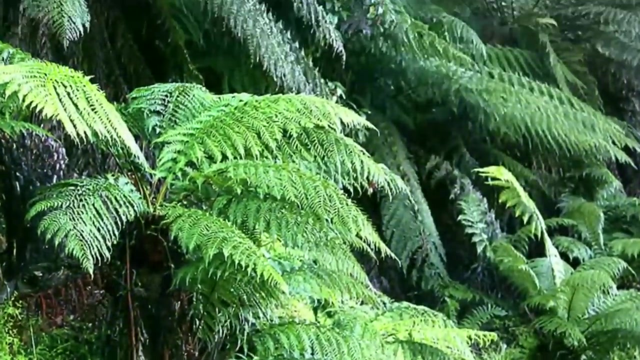 now entered the cell phase. these little guys lived in colonies and were constantly expanding along the coasts and eventually into the riverways of valberra. they created their own nutrients using photosynthesis, a process that works so well that it's been passed down to all living plants today. 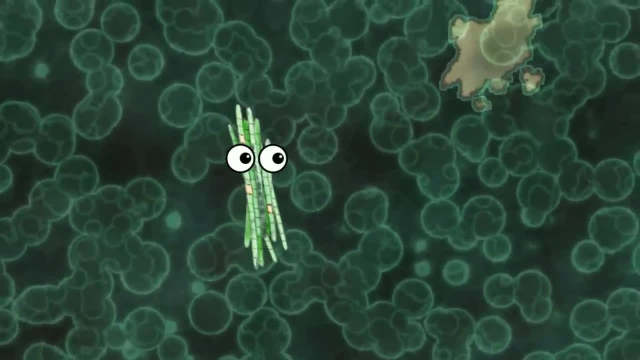 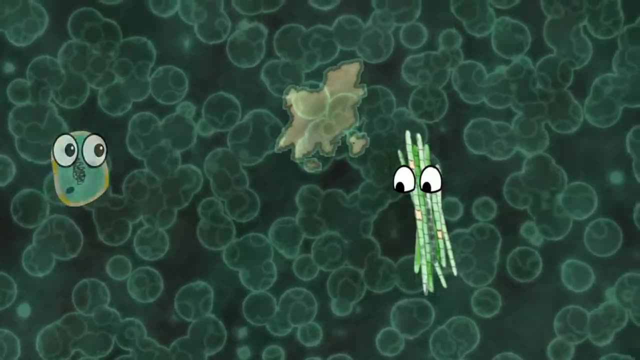 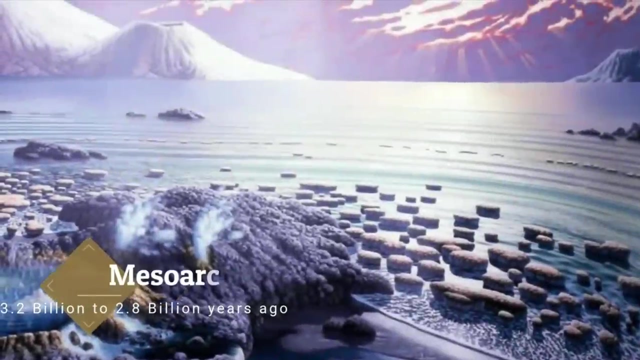 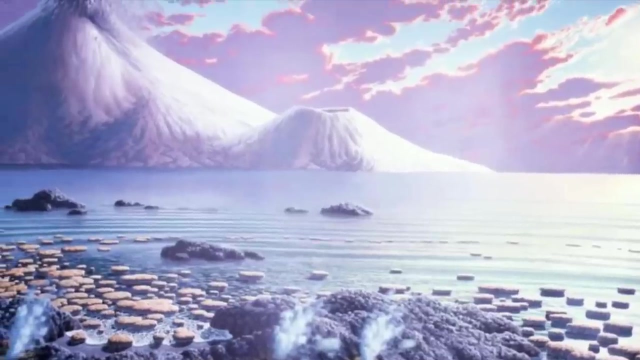 thriving in the carbon dioxide rich atmosphere. these first organisms would arguably become earth's very first rulers. you know, i suddenly feel proud to be a cyanobacteria. don't judge me. as we get into the mesoarchean, around 3.2 billion years ago, we start to see a new phenomenon. take 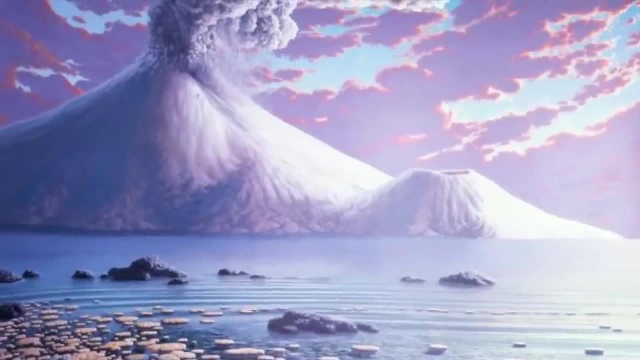 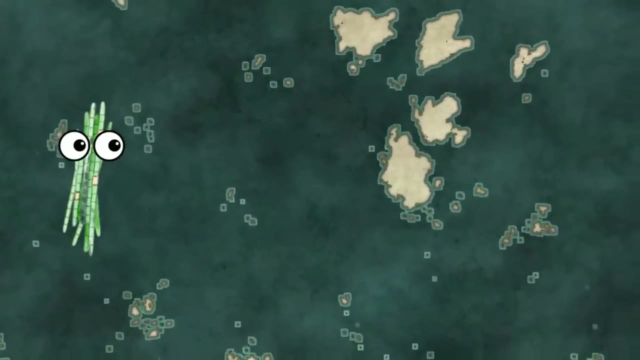 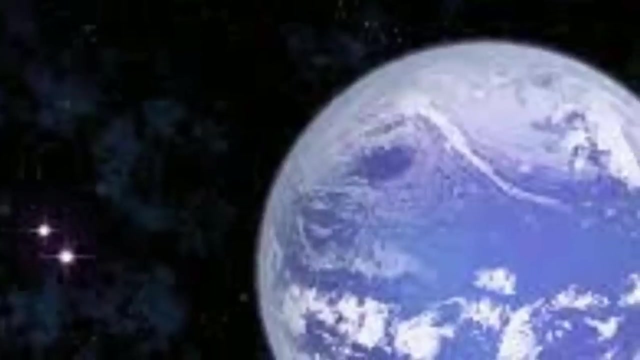 place. as a result of the cooler surface temperature of the ground, with the still coldest of temperatures and the most active volcanism underneath plate, tectonics begin to move the crust around the globe, causing continents to tear apart and form together to form supercontinents. by this point, the global temperature had already dropped considerably from. 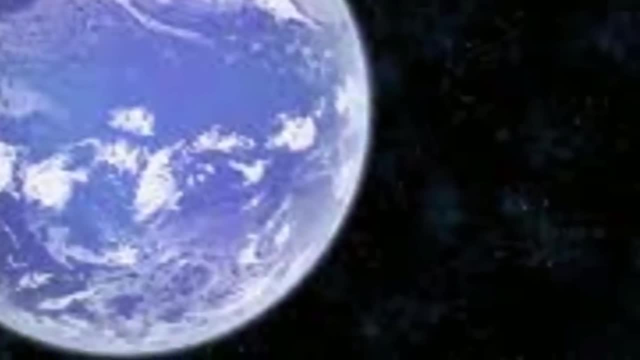 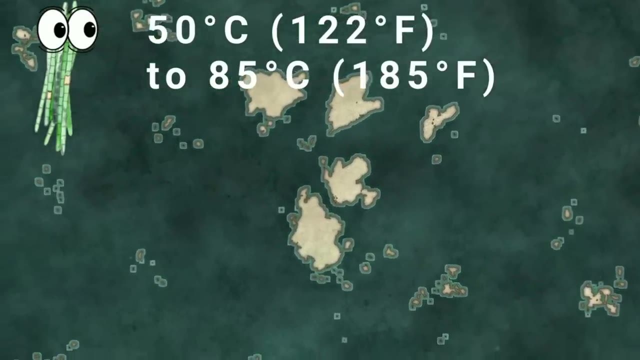 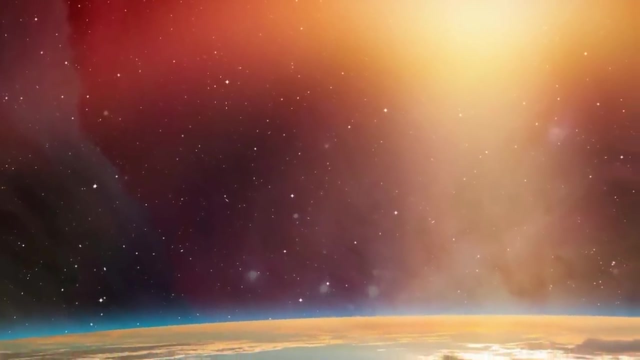 what it was back in the hadean, but it still isn't what we would call comfortable by today's standards. around 50 degrees celsius or 122 degrees fahrenheit, and 85 degrees celsius or 185 degrees fahrenheit was the average at this time. this was probably the case because the atmosphere was still 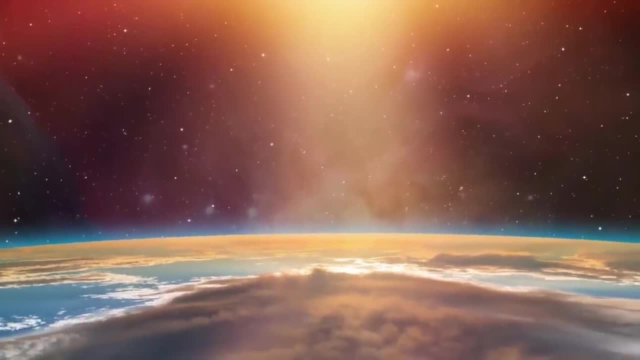 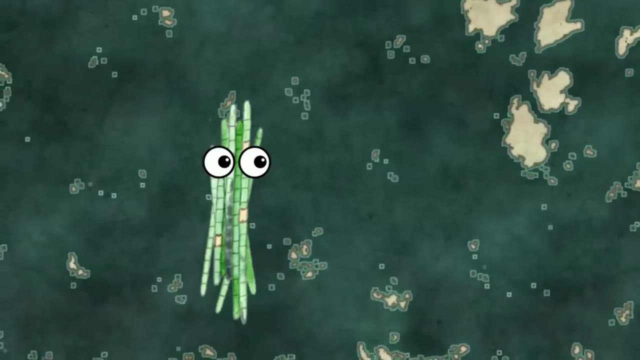 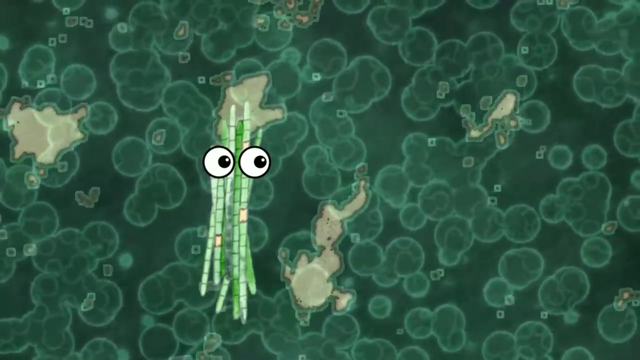 mostly comprised of greenhouse gases like methane and the previously mentioned carbon dioxide that was fueling the cyanobacteria empire, but this was something that would actually start to change as the current rulers of the archaean earth spread and diversified into different species and started to form complex microbial ecosystems. as the cyanobacteria took over, they would 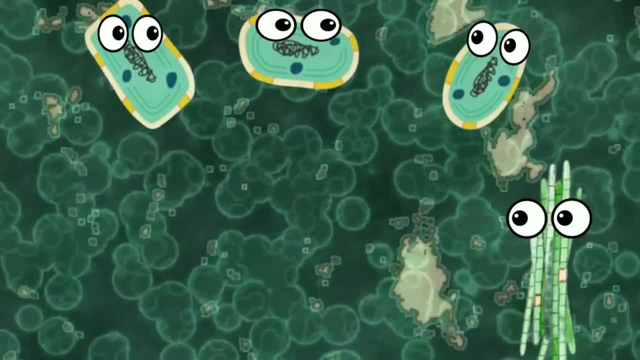 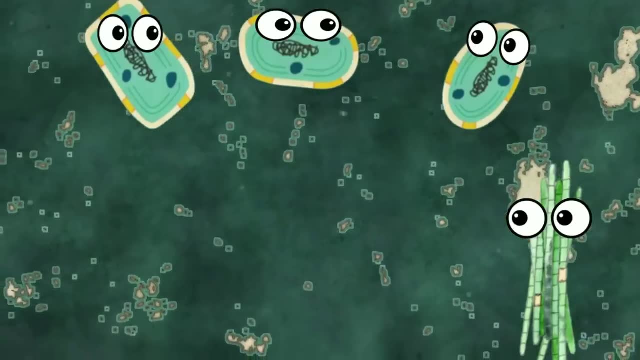 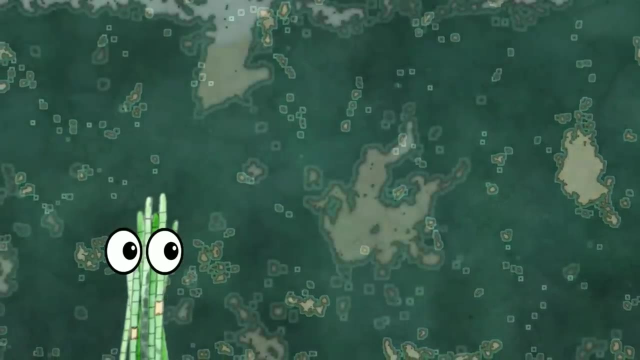 start to do something that we normally think of as only something that humans are capable of: drastic changes to the global climate. and they basically did this simply by existing. you see, as these microorganisms took in co2, they would produce oxygen as a byproduct. this would lead 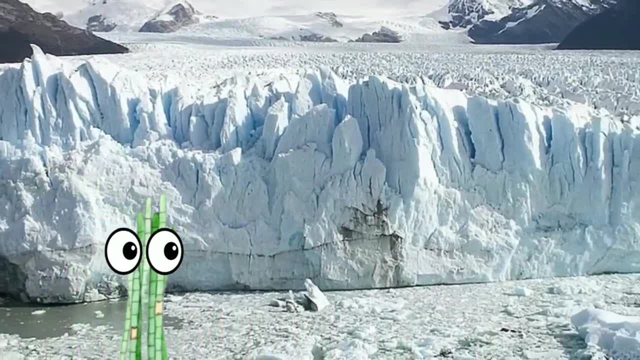 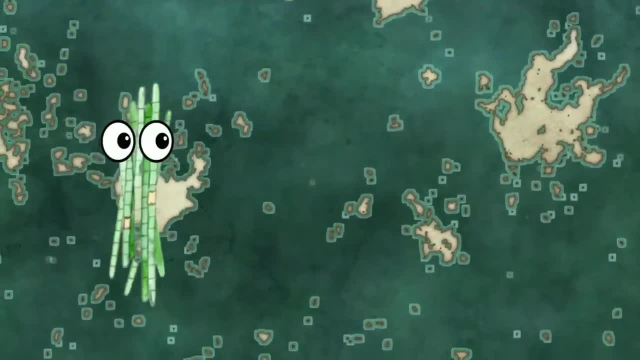 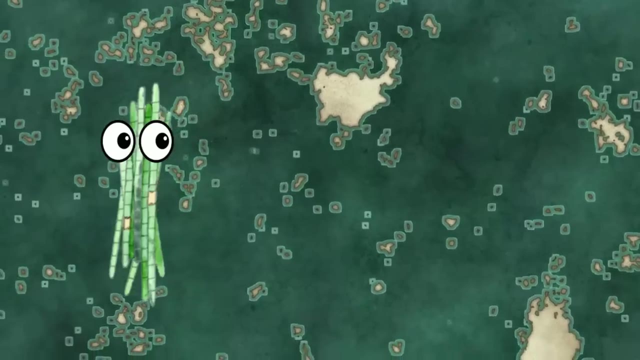 to a drop in temperatures until eventually by 2.9 billion years ago the earth would experience its very first glaciation at the poles. so in about half a billion years the cyanobacteria took over the world and made the hyper greenhouse climate cooler until earth. 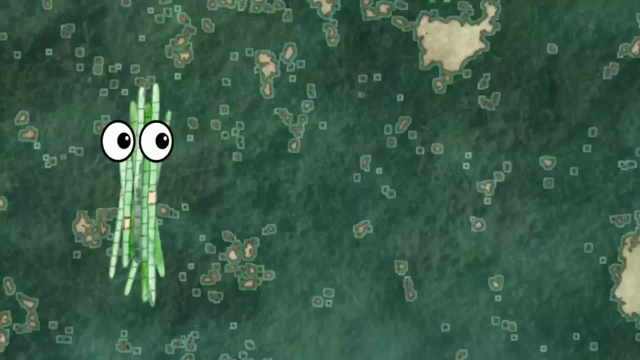 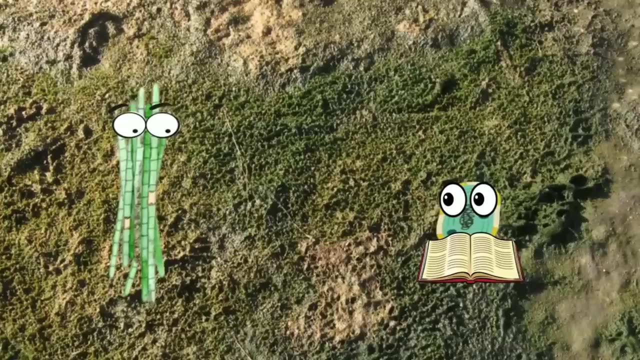 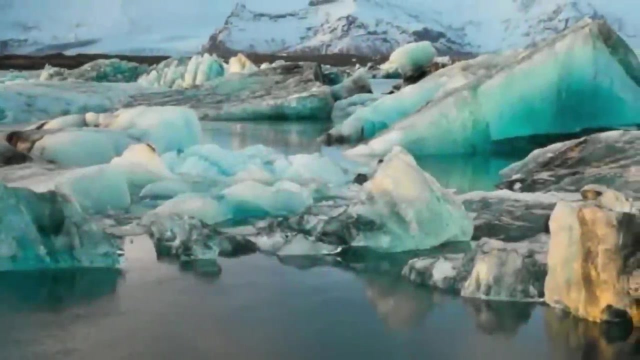 was basically experiencing its very first ice age. that's a lot of accomplishment for what is basically mats of green goo. excuse me, sir, have you learned of the glory of the green? the ice would not become a permanent fixture by 2.7 billion years ago. it had already completely receded. i say already. 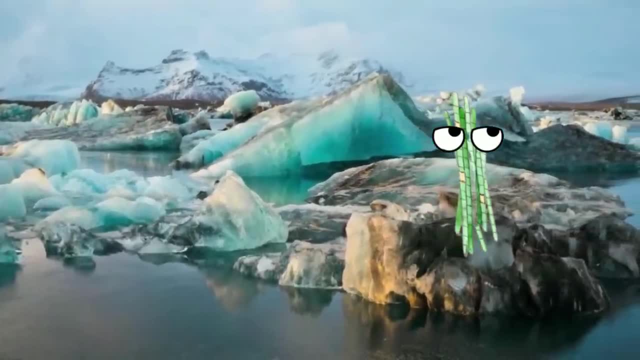 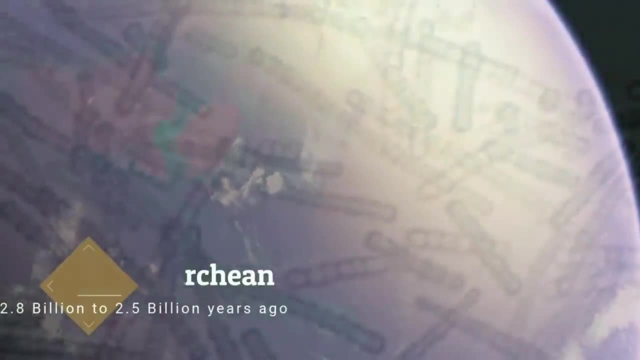 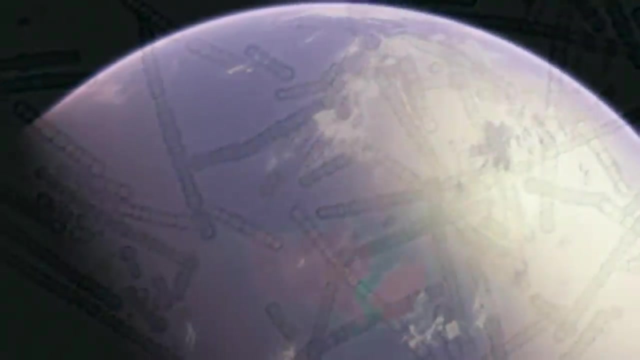 like we're not talking about 200 million years of cold. This marks the beginning of the fourth and final era of the Archean. the Neo-Archean And the cyanobacteria had made the world theirs, evolving into new niches and covering different environments all over the globe. 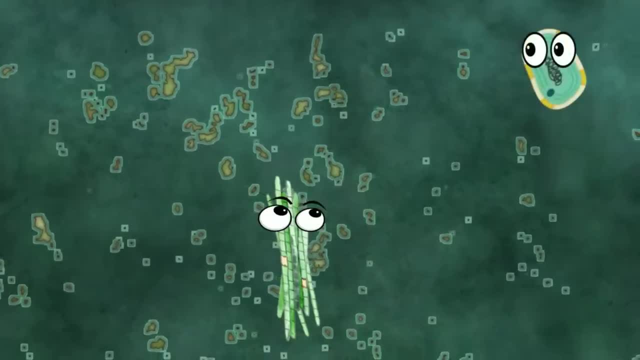 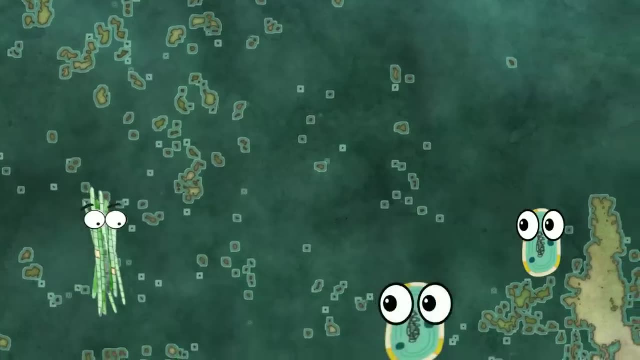 And let's not get it twisted. these guys were also the first organisms to adapt to dry land, as well As the microbial mats spread across the continents and islands. it's thought that the land would actually start to turn green for the first time. 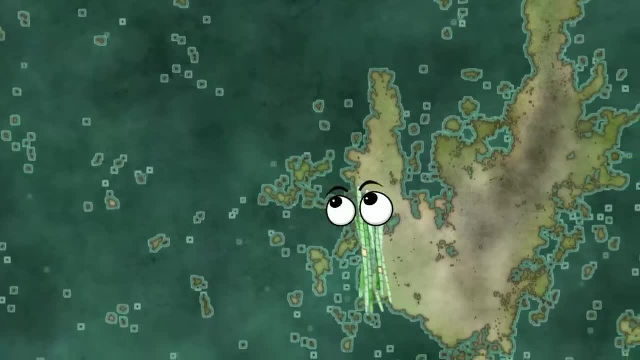 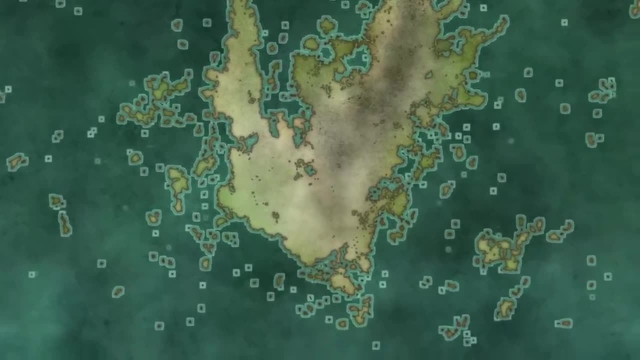 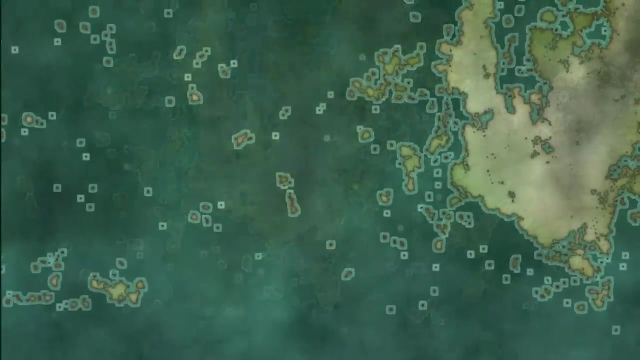 Not with true plants yet, but with microbial mats made up of trillions of tiny organisms who have managed to make the planet theirs, And over the millions of years that followed, the land masses would come together to form the first land that was large enough to be considered a supercontinent. 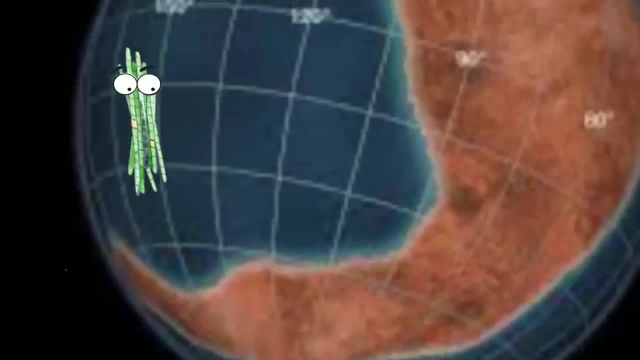 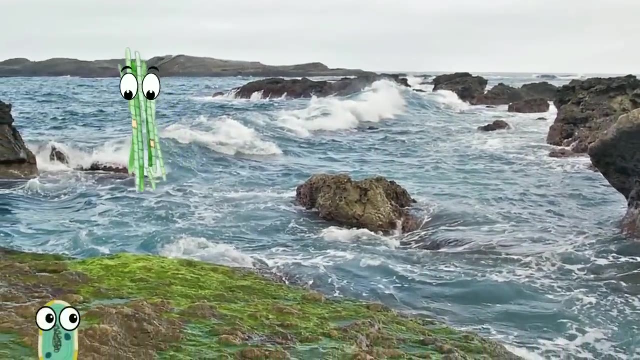 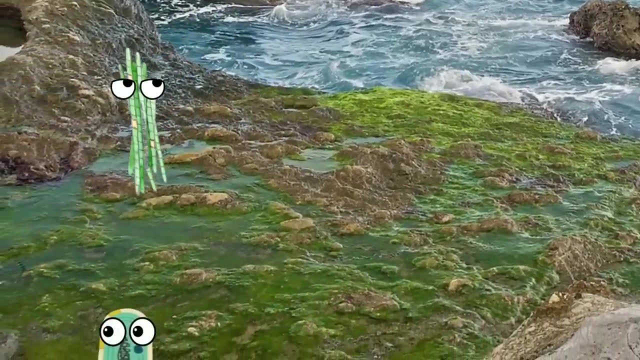 We now call this continent Kennerland, And it was well. it was largely empty, With, With the exception of the green goo slowly spreading across it, Almost like a moldy jelly just kinda slurkin' across there. Well, even though there actually wasn't mold yet, 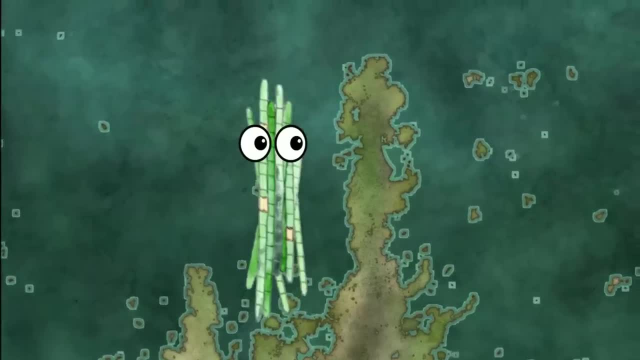 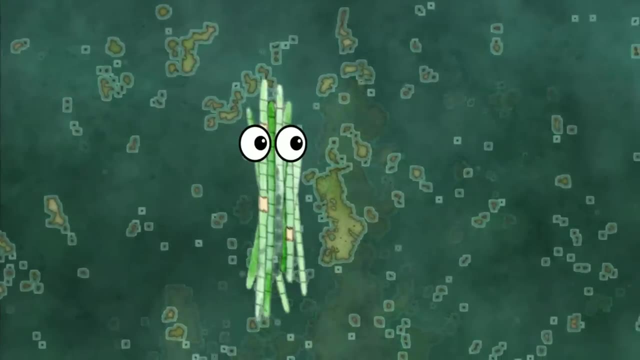 It's all quite beautiful, isn't it? It's amazing how sci-fi some of this stuff seems as I research these different times in Earth's past. It's really easy to seem like we're just glossing over everything And, to be honest, we are. 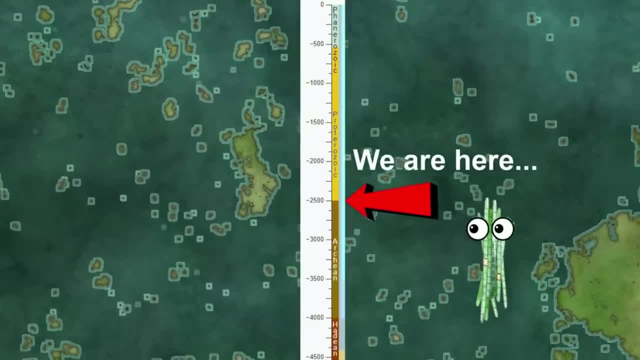 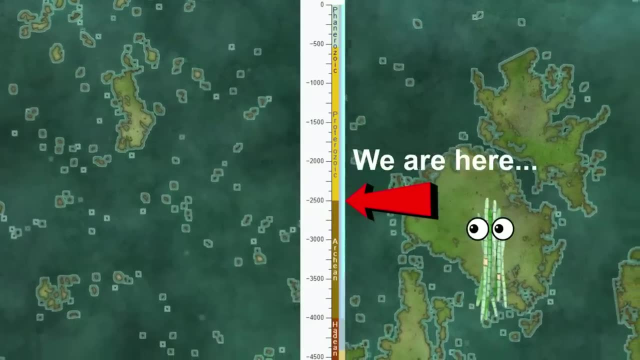 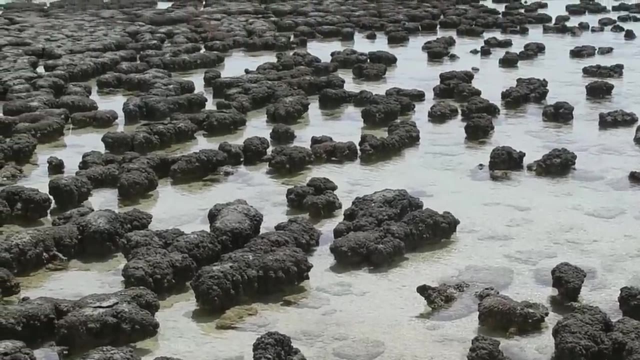 And this is because, now covering the first 50% of Earth's existence, we're still lacking a lot of the fossil record to be able to accurately know everything that was going on during this eon. The fossils from the once-proud cyanobacterian empire can now only be found in places like Shark Bay, Australia. 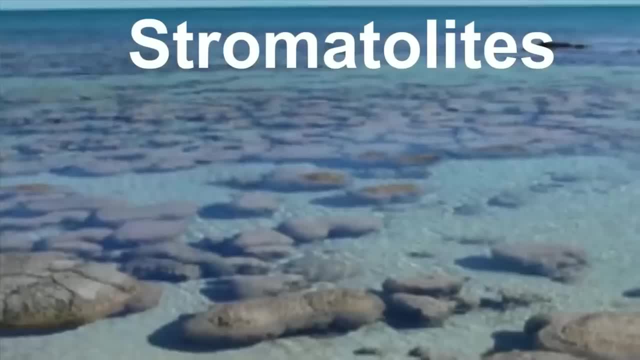 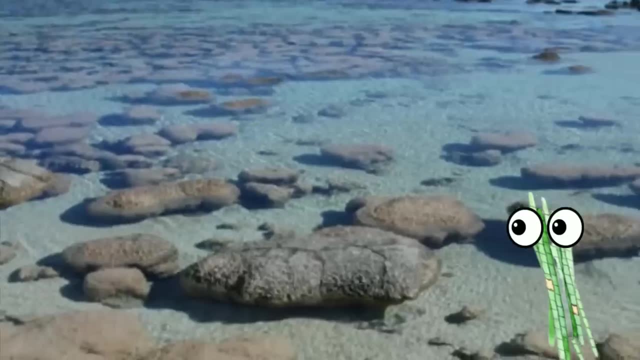 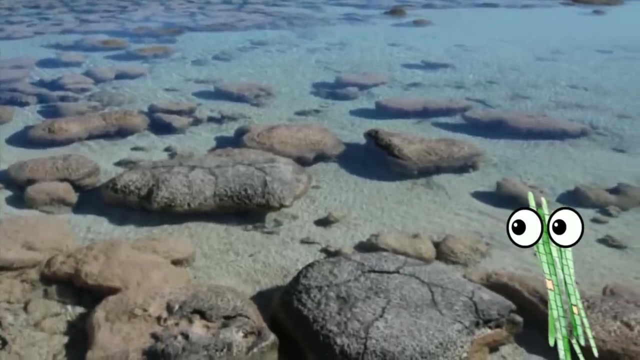 They're called stromatolites, and the top layers of these bulbs of rock are actually still alive. That's right. the cyanobacteria still continue to exist two and a half billion years after their reign as the microbial rock. That's right. the cyanobacteria still continue to exist two and a half billion years after their reign as the microbial rock. 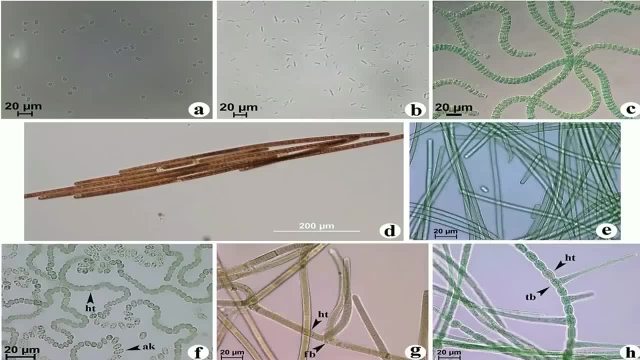 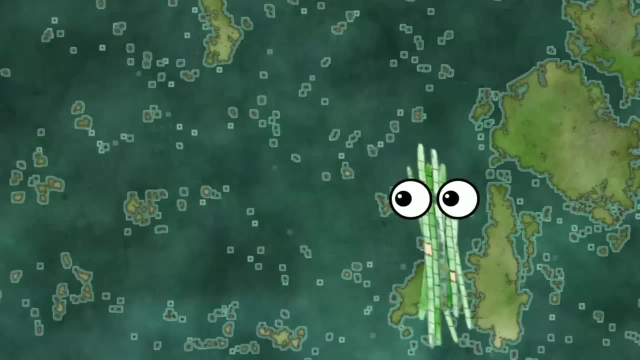 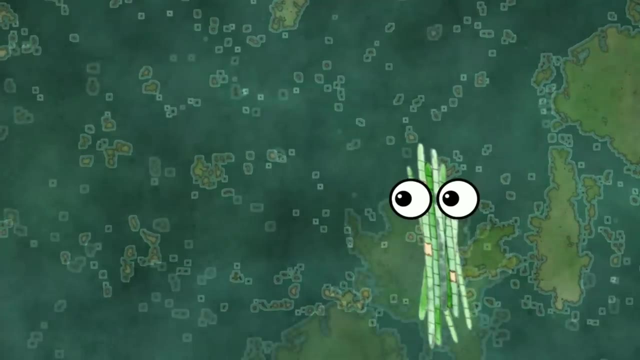 And cyanobacteria actually still exists today in a bunch of other niches, including commons, even living in our atmosphere, floating in the air today. And now we've come to the end of the Archean Eon. As I said, we are now already halfway home. 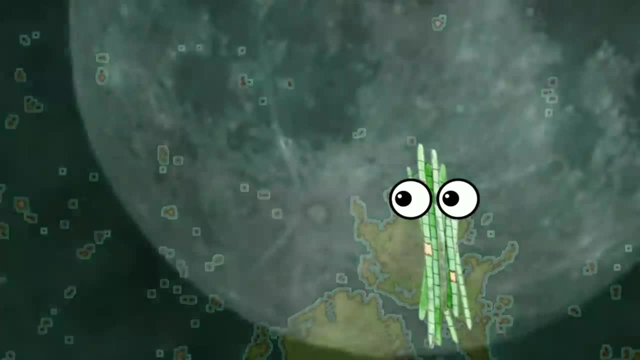 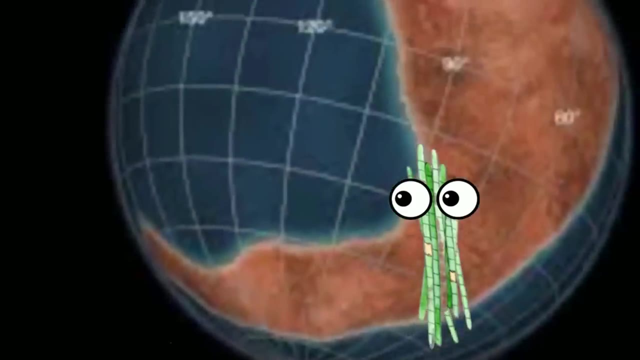 And from here things are going to start to get a little bit more complex. But to recap, our planet now has a moon, a solid crust with abundant water on its surface. two supercontinents have come together and been torn apart. we have a climate that's starting to. 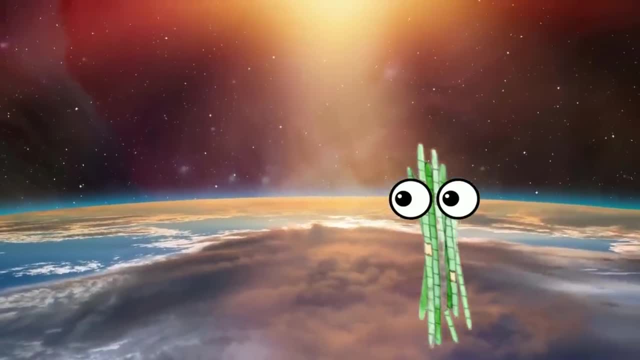 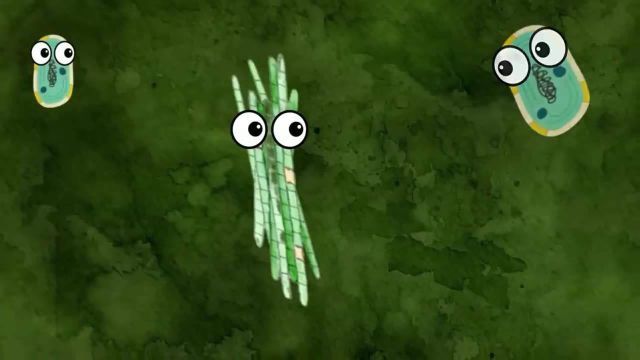 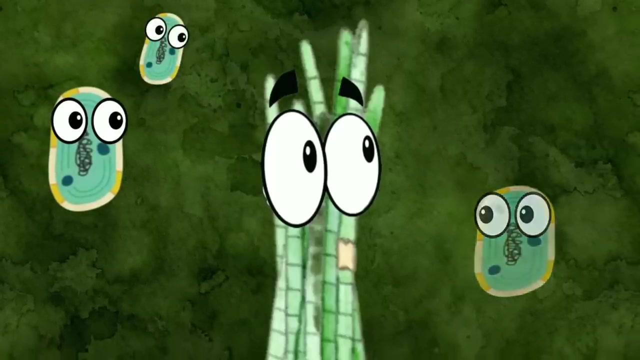 fluctuate and oxygen is becoming more and more abundant all the time, And much of this was thanks to the mighty cyanobacterian empire. You know, maybe I should just stay like this. Maybe I should just remain in the Archean and join a giant mass of goo For the glory of the empire. Wait what? 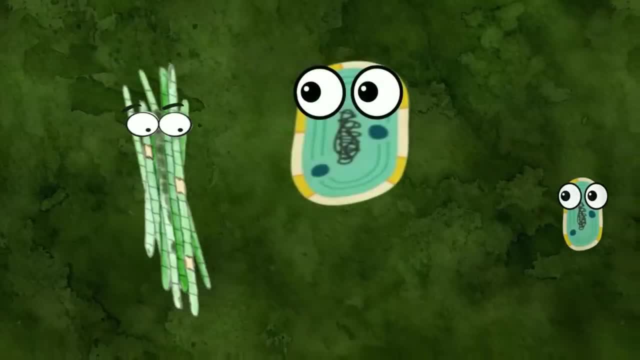 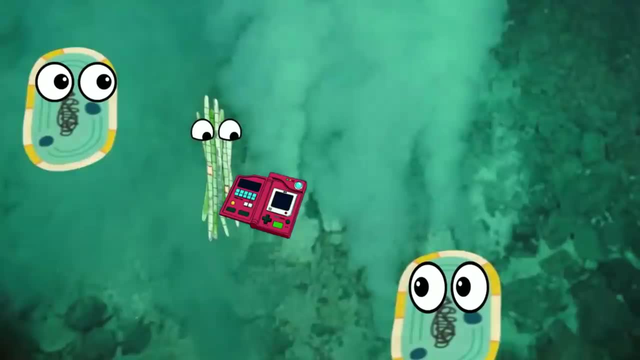 am I saying This sucks. I have to try to get back to becoming a human. I have to get back to my own time And, after consulting the Pokedex, I think I know how I evolved into this form by reaching 1,500 subscribers while being next to those hydrothermal vents at the end of the Hadean. 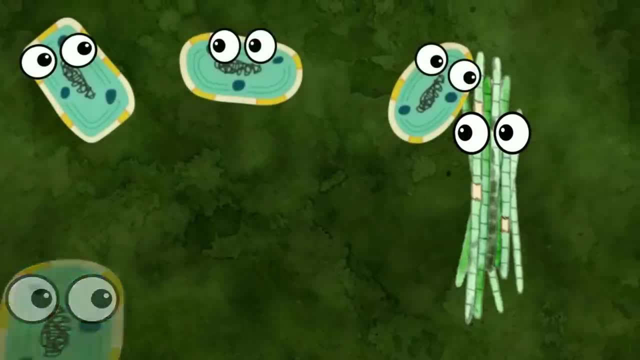 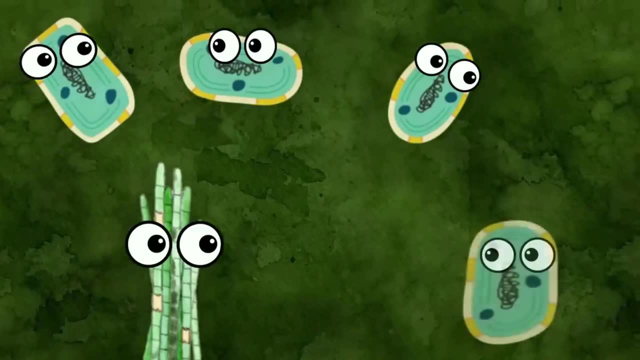 remember. So maybe that's the key. Maybe if I hit different milestones of subscribers while in the right location, I'll evolve to the next stage of my evolution and eventually become human again. Okay, so I know that this is something that I've been doing for a long time and I've been 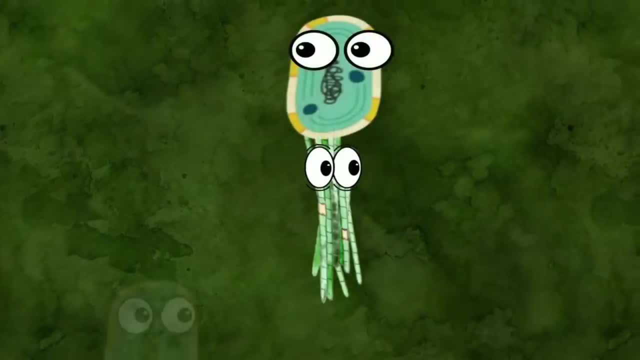 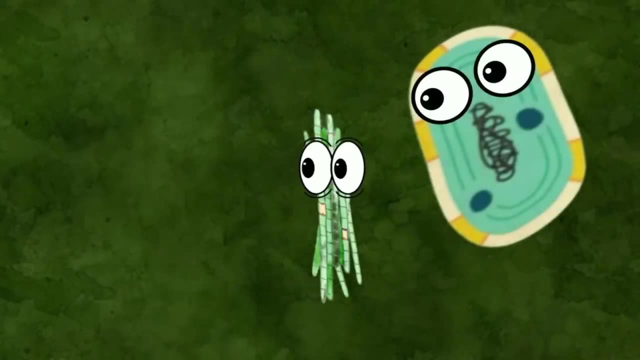 doing it for a long time and it's something that you're probably all used to hearing all the time, but this just became way more important. If you made it to this point in the video and you're not already, please, for the love of God, subscribe. And if you are subscribed already, 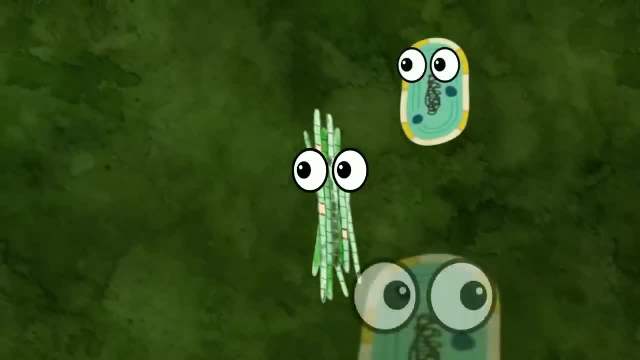 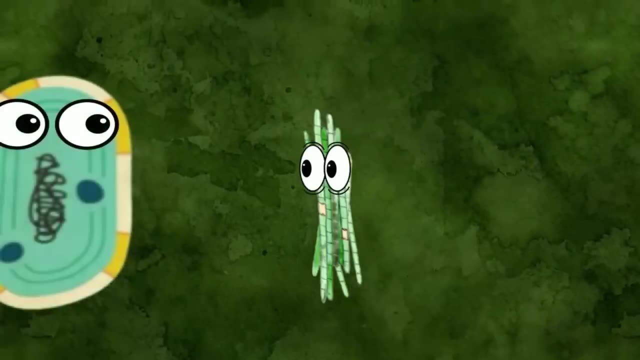 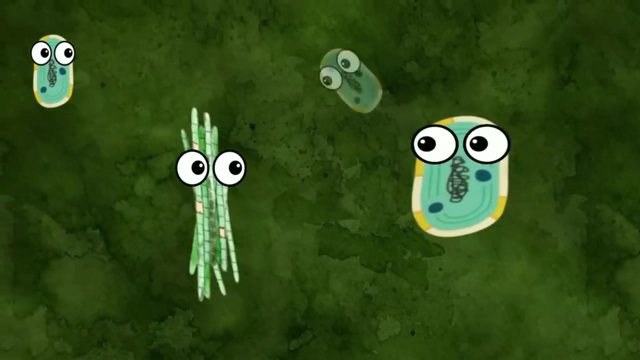 share this or any of my other videos to other people so they can subscribe. I need everyone's help to move forward through time and turn back into me again. Until I reach the next milestone, I have to go. Stay here with this colony, otherwise I'll dry out and die. 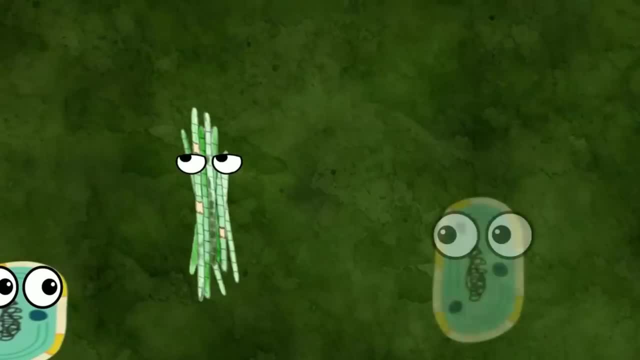 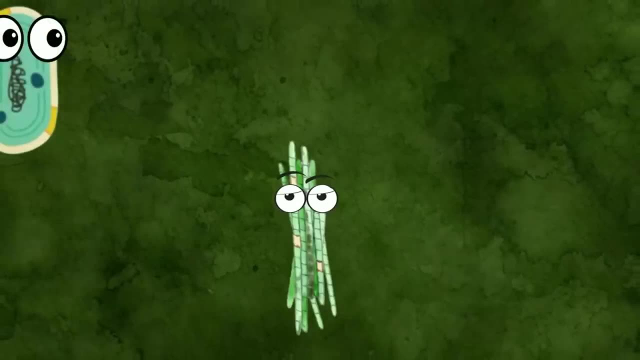 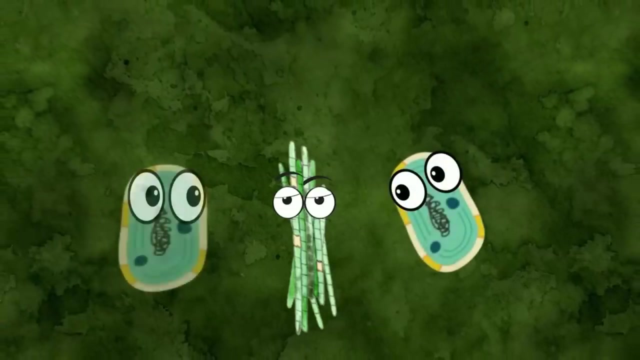 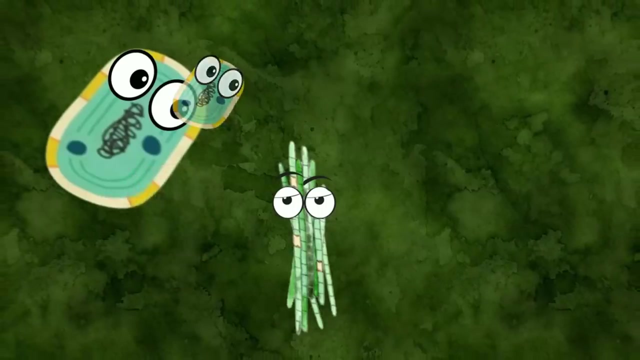 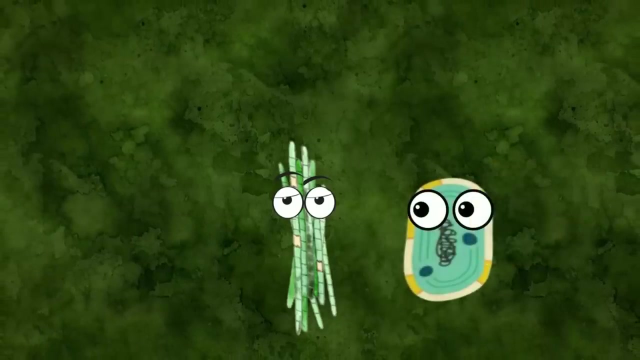 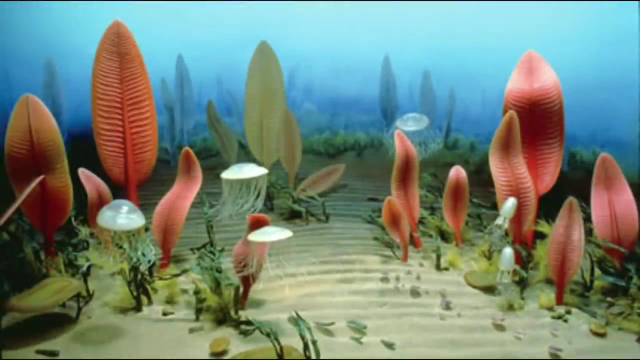 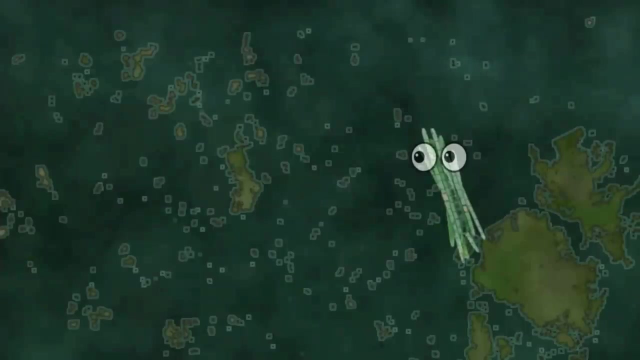 Please, seriously, these guys suck. All they do is talk about the glory of the goo. Until then, I'll just have to wait here. Take care everybody. Pray for me As we move through these ancient times in the past. 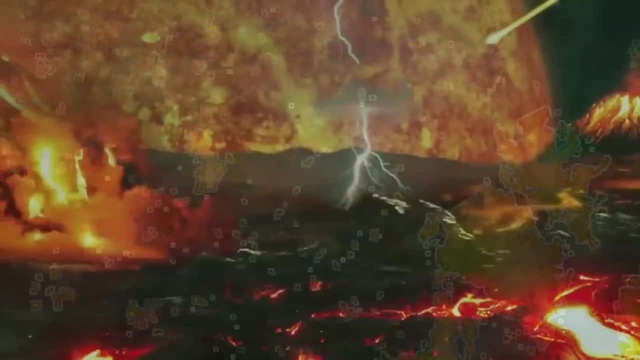 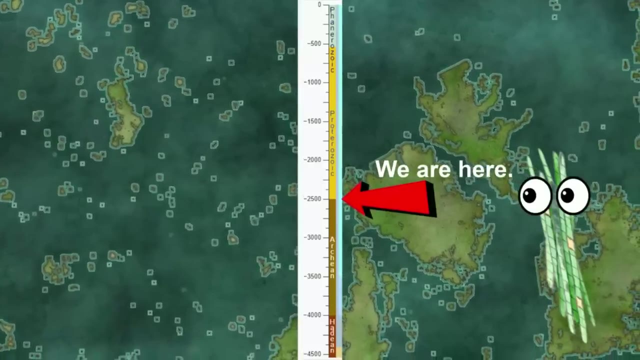 we've been making baby steps as the world's gone from a hellscape incapable of supporting life to something that shows some real potential, But it has been slow going. Over 3 billion years has already passed since the formation of the Earth and so far, the only things currently 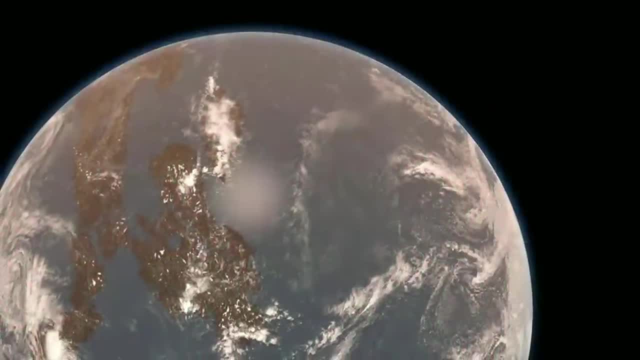 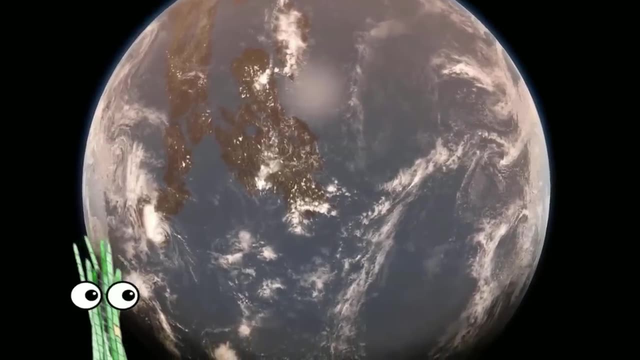 living look like this. But by the end of the Archean things were starting to at least slightly resemble our modern world, at least comparatively speaking, And with each step we move forward in time we're just a little bit closer to the world we know today. This will be. 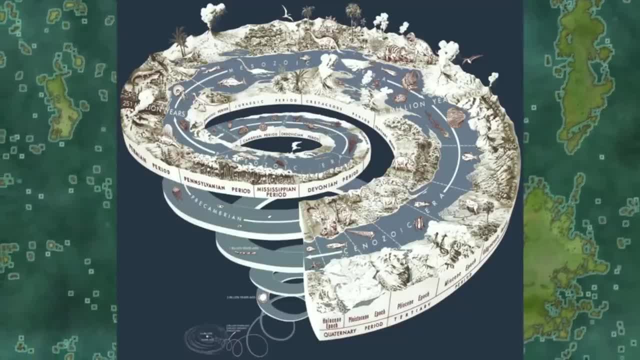 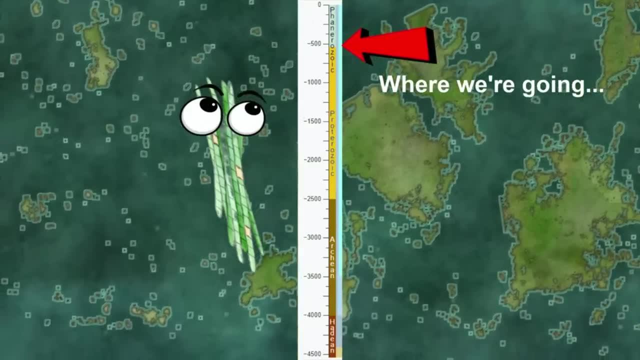 the last time that I cover anything that was made possible in the time that I had. I don't want to. I cover an entire aeon in a single episode in this series, because this video will take us all the way to just half a billion years ago, and that's when everything finally starts to get. 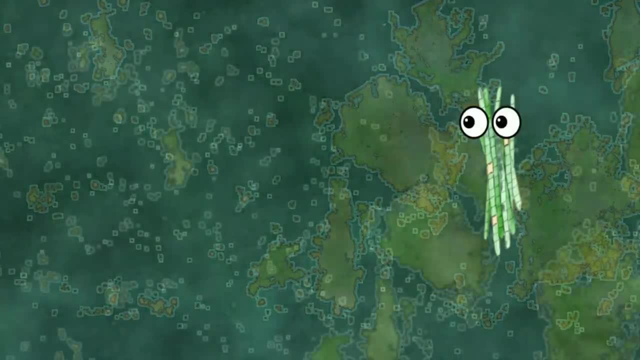 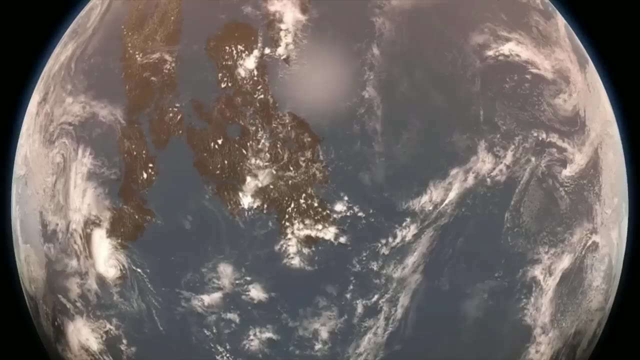 interesting. I feel like all this has just been the legwork to get us to the good stuff, and now, finally, we're at the last step of setting the stage. So now let's get into the Proterozoic Aeon and see what transformations the planet and the life on it go through over the next two billion. 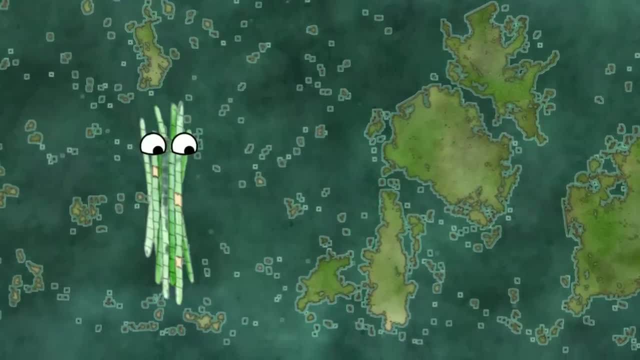 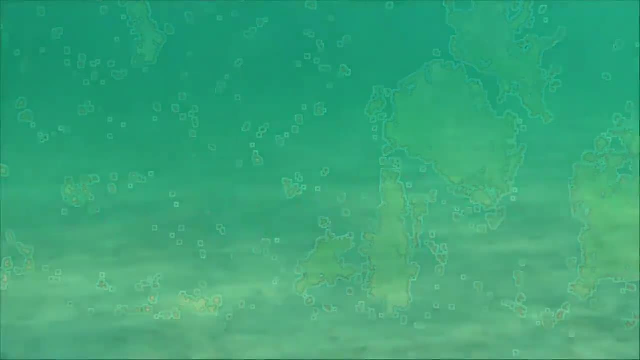 years, And this one actually turned out to be a little bit more interesting than I expected, because I actually didn't know a lot of the things that I ended up researching for this video. We start things off with the Paleoproterozoic. This is the longest of the three eras that make 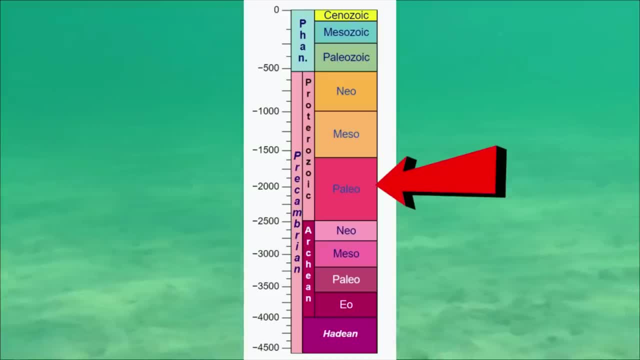 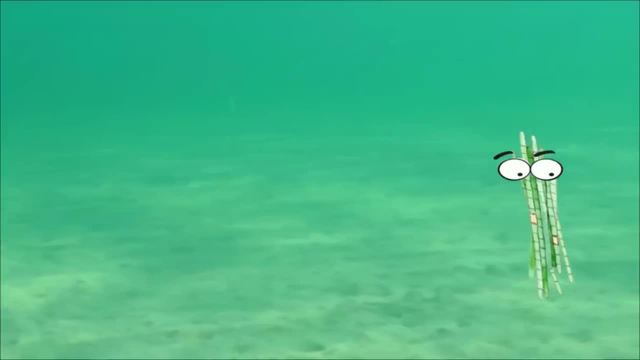 up this aeon, and in fact it's actually the longest era in geological history, covering from two and a half to 1.6 billion years ago. But I think, for several reasons, it would actually be easier if, Instead of covering each era like I did the last time, I just jumped from one major event to the 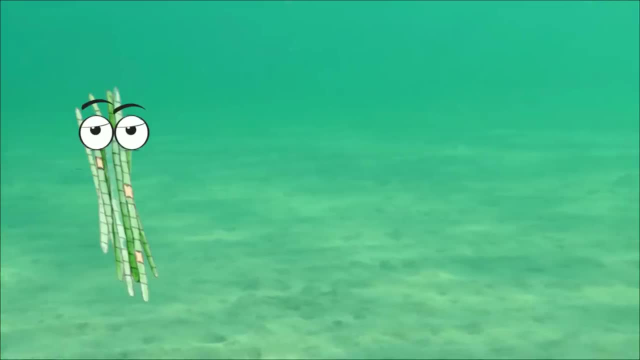 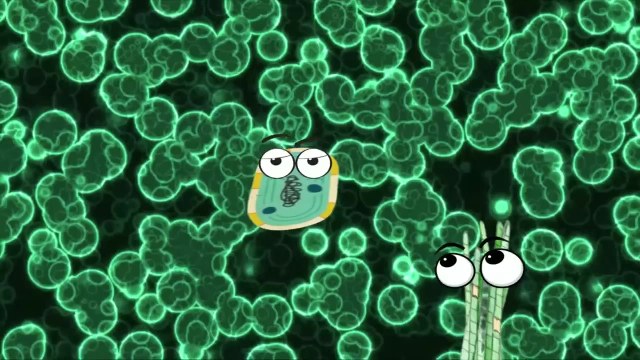 next and the reasons why will become clear as we move forward. And the first big thing that took place during this time is a direct result of events that took place in the Archean. You see, as the cyanobacteria spread and multiplied, they took in carbon dioxide and excreted oxygen At 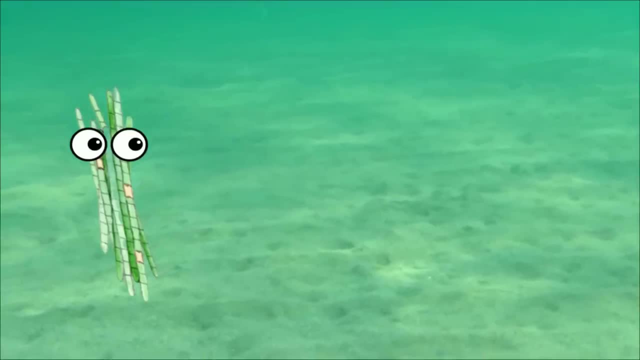 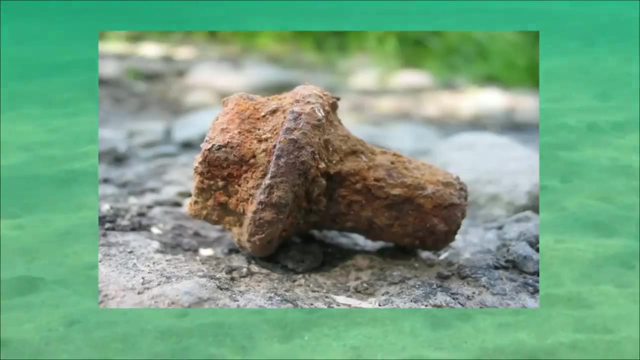 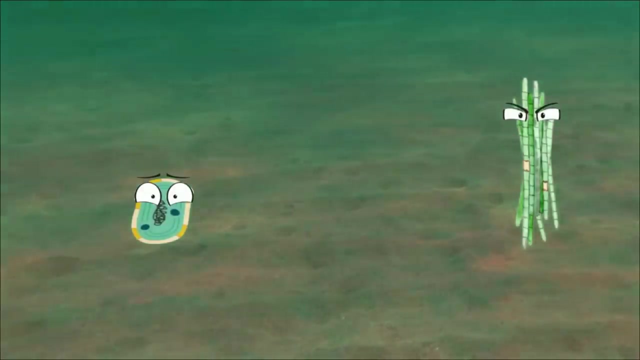 first, the increasing oxygen was kept in check by being absorbed by the increased iron that was in the oceans And as that happened, Oxygen did what oxygen does to iron and started to rust it, And it's believed that after several million years, the end result was the oceans turning from a turquoise color to a deep blood. 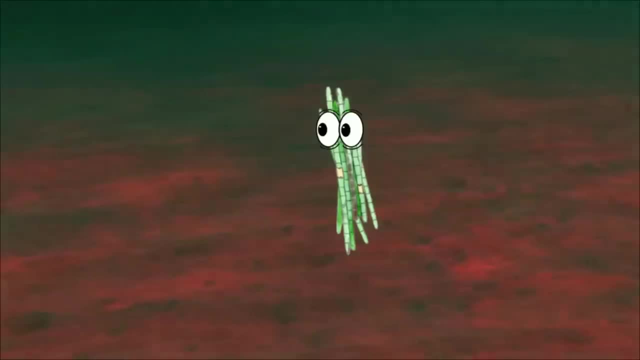 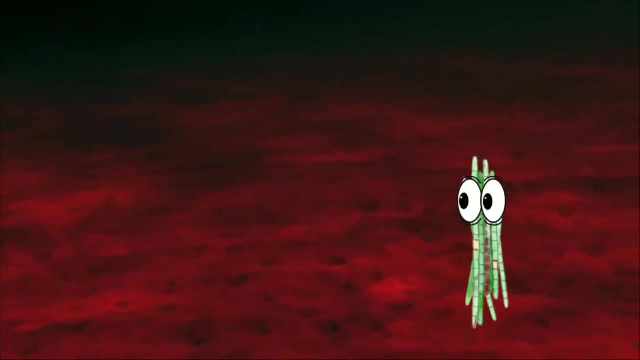 red. The rusted iron eventually drifted down to the seafloor and eventually made up the iron oxide that we see in these stunning formations. But there was a finite amount of iron in the oceans and as that dissipated, the oxygen would start to build up to levels that the earth had 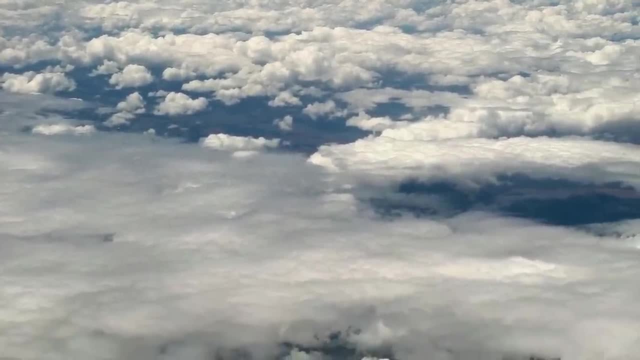 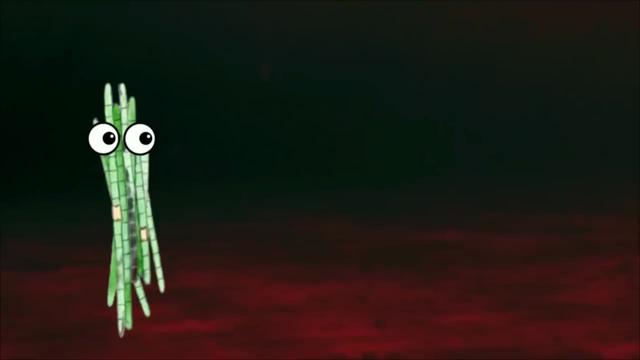 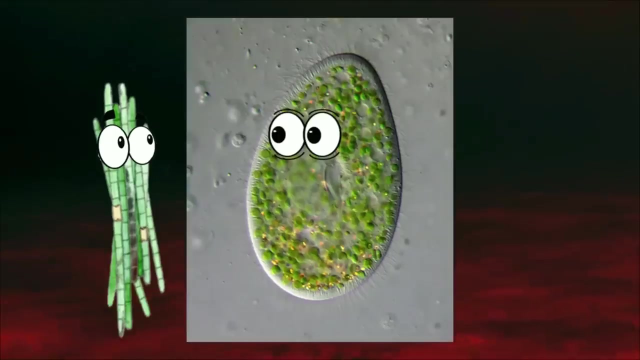 never seen before. This may sound like a good thing to us, but at that time, the oxygen was actually toxic to pretty much everything that was alive, And it makes sense if you think about it. The organisms that lived at that time lived on a world where carbon dioxide and methane were more abundant. 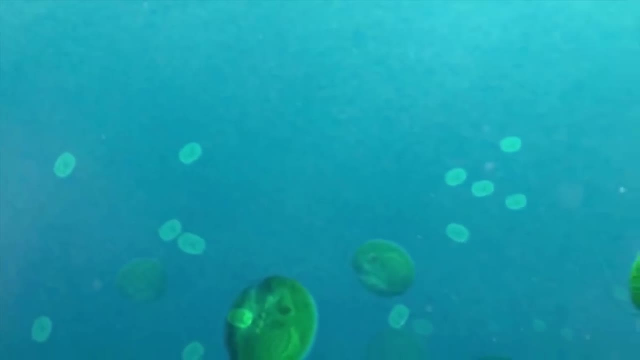 than oxygen. In fact, there was almost no oxygen at all until the cyanobacteria started farting it out all over the world. That's all the oxygen really was, to these guys, A waste And just like us when we exhale carbon dioxide, these guys were just like us when we exhale carbon dioxide. 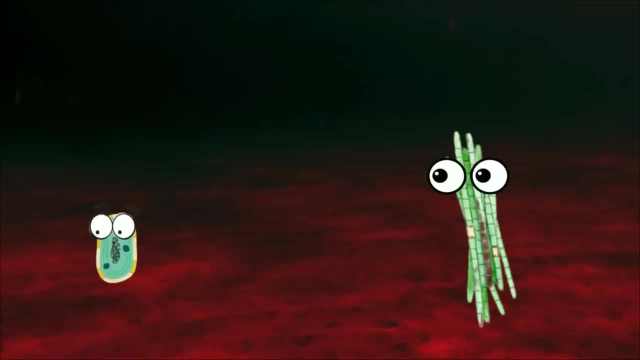 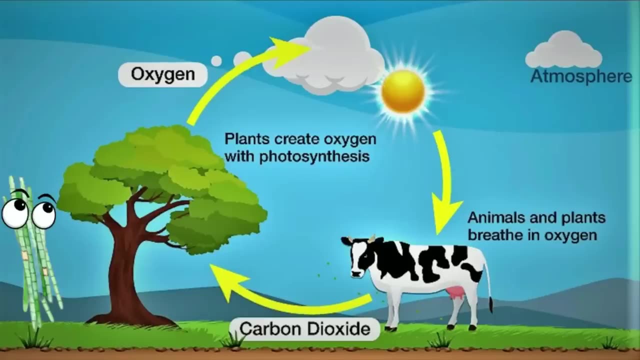 The amount of gases that these organisms give off is normally toxic in large quantities. In the modern world, there's checks and balances to this, because plants take in carbon dioxide and give off oxygen, and animals do the opposite. But during the early Proterozoic there was nothing on earth. 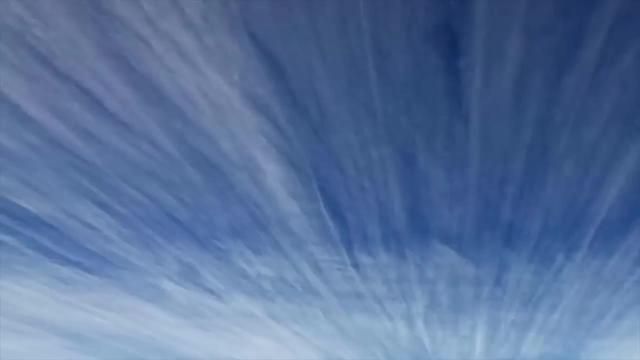 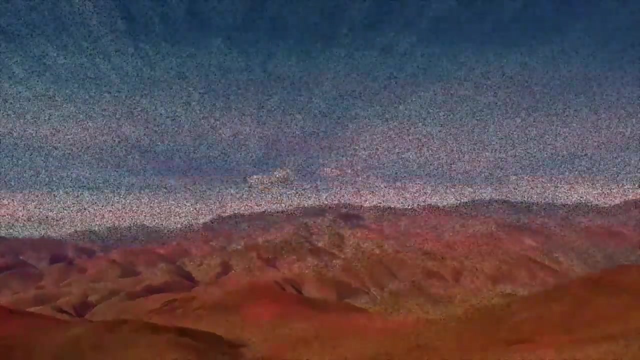 to take in oxygen and replace it with the new carbon dioxide. So the noxious, deadly cloud of oxygen kept building, And this would be the end of the line for the mighty cyanobacterian empire. That's right, Tim Tim. You and the rest of your kind are destined to slowly suffocate on your own farts. 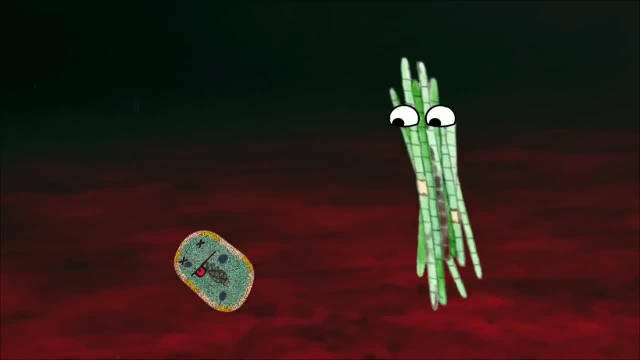 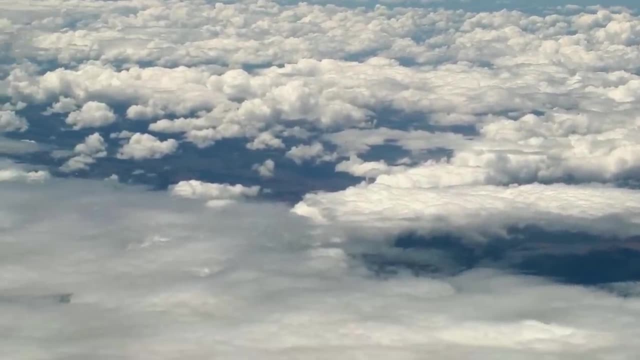 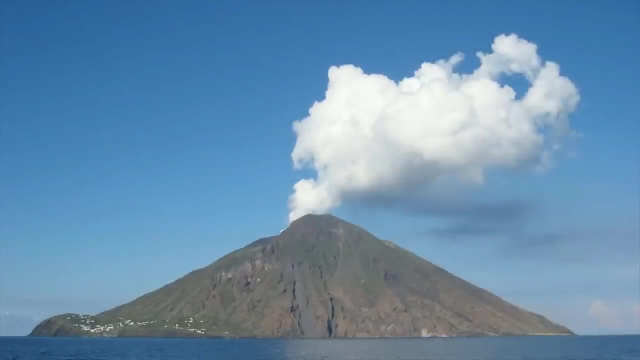 A fitting end, if you ask me. This would be the very first mass extinction that would ever happen on earth, Also known as the Great Oxidation Event or Great Oxidation Catastrophe. So the first great dying didn't start with a supervolcano or a meteor, but by the very air. we breathe today, And oxygen levels would continue to fluctuate throughout earth's history. This was just the first really massive jump that would ever take place, And the earth wasn't even done seemingly trying to cleanse itself of the goo infestation that it had contracted over the previous one and a half billion years, Because things were about. 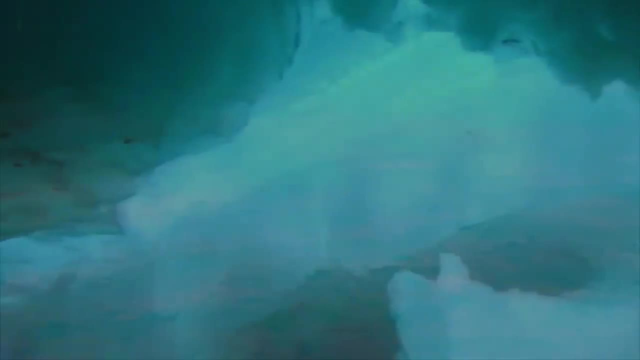 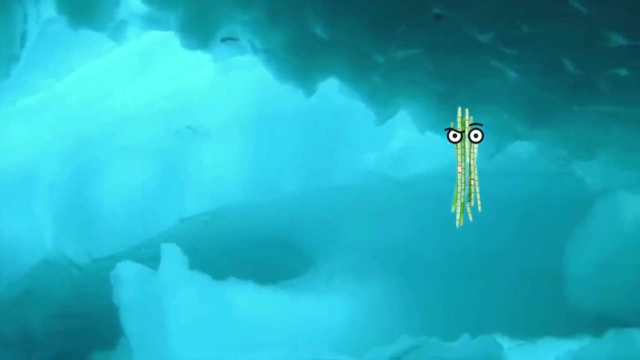 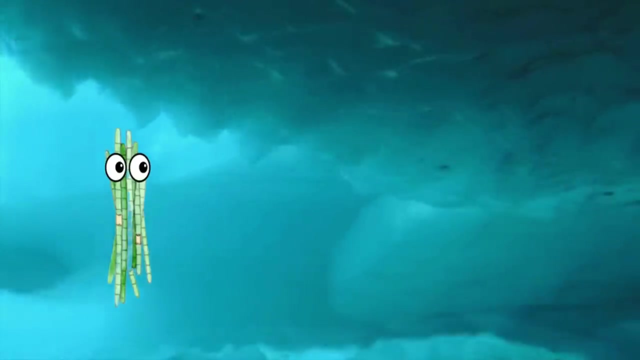 to go from bad to worse. Remember how, during the Archaea Neon, the increase in oxygen led to global cooling and inevitably resulted in the first glaciation. Well, you may have guessed this may foreshadowing for some things to come. The world was cooling at a 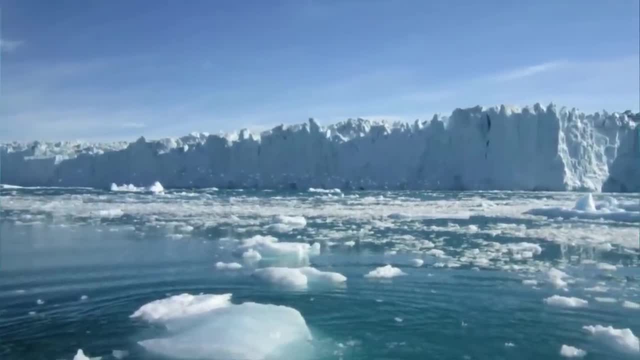 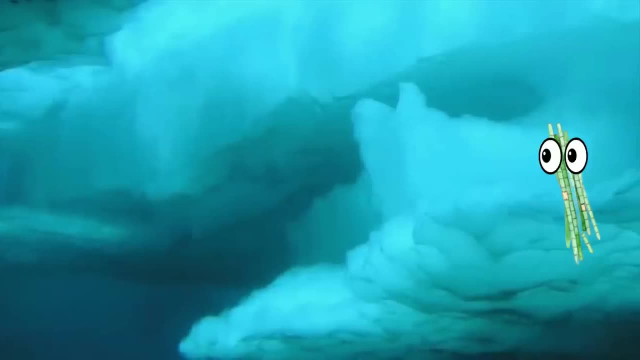 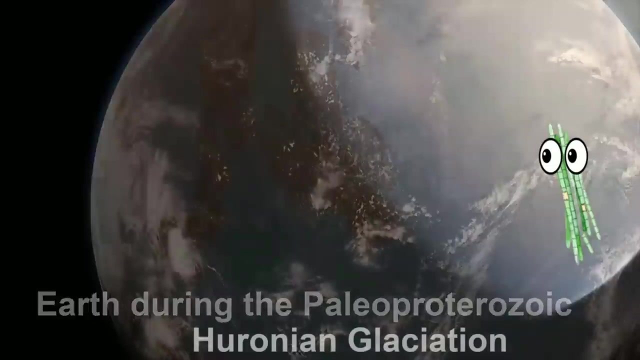 rapid rate as free oxygen built up in the atmosphere and there was nothing to counteract at this point. So eventually it resulted in a runaway glaciation that would go way beyond anything that Earth would see in the more recent past And for over 200 million years the earth 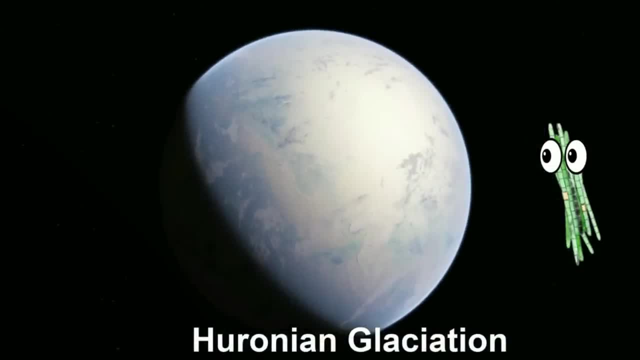 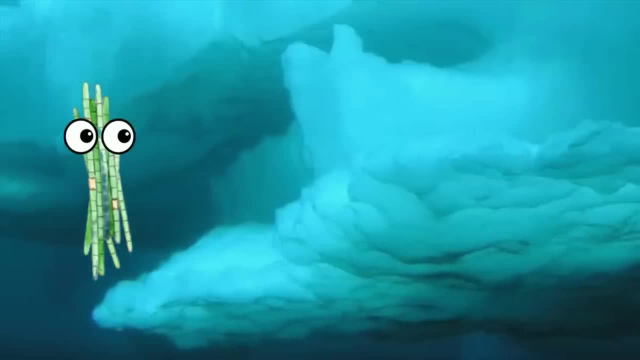 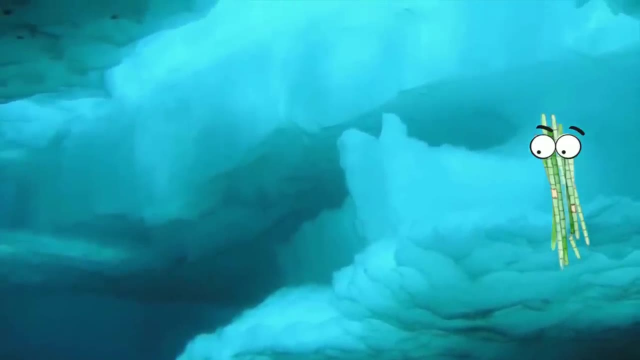 literally froze. This time has been called the Heronian Glaciation, or first snowball earth- Yeah, first. So at this point we've literally seen the earth transform from Mustafar to Hoth, and this could have been how the story of life on earth came to an end. 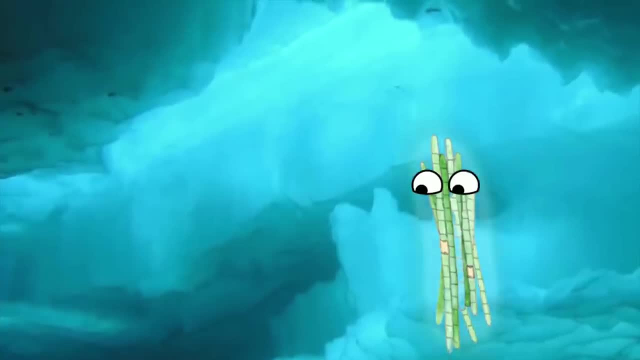 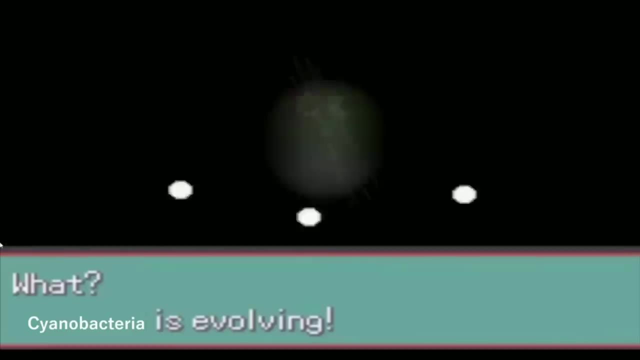 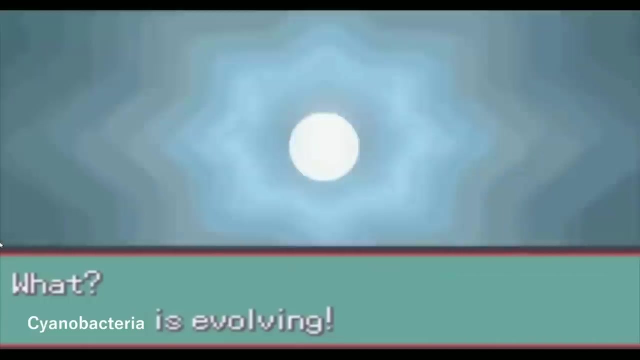 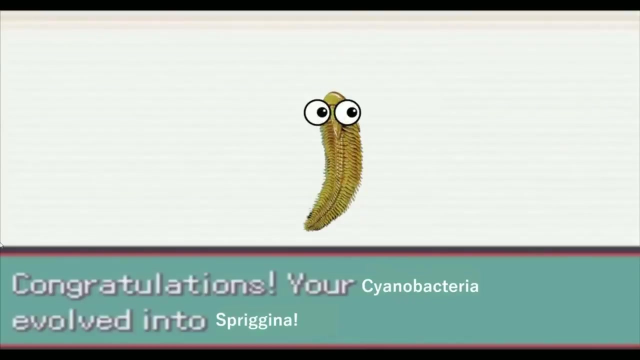 But sorry, I'm not going out like that because, thanks to all of you last week, it's time for an upgrade. Freedom, What No? And come to think of it, this actually brings me to the other big event that happened during. 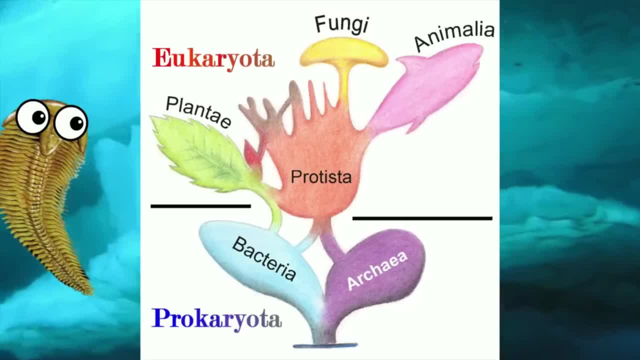 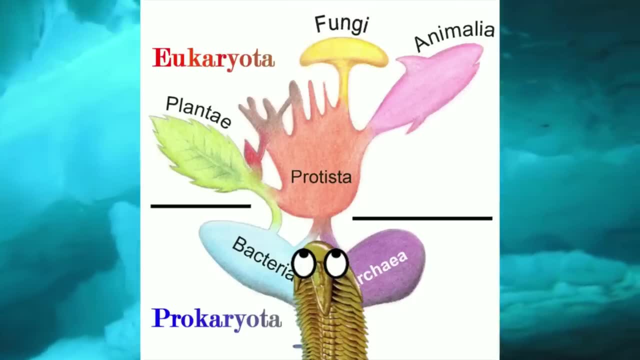 this era, The emergence of eukaryotes. Eukaryotes literally encompass every kingdom on earth that is multicellular, as well as some unicellular organisms like protists. Now there's some debate about what eukaryotes are, but I'm not going to go into that right now. I'm going to debate on whether or not they truly did evolve during the Paleoproterozoic, But to me, the fact that some of the cyanobacteria did manage to survive means it's likely that something had to start absorbing oxygen and releasing carbon dioxide at some point. 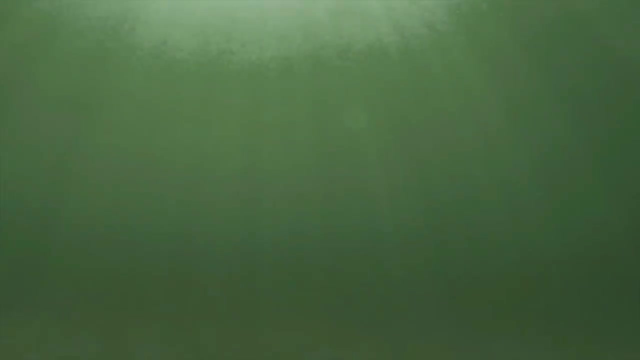 Following the Heronian glaciation, we come to a time that scientists have nicknamed the Boring Billion, And yeah, it's exactly what it sounds like. After the first mass extinction brought on by oxygen pollution and dramatic climate change, what was left when the world finally melted was a nutrient-poor world that was kind of stagnant for an actual billion years, Starting at 1.8 billion years ago. this time actually started to see a drop in oxygen once again, And this allowed the cyanobacteria to take control again. 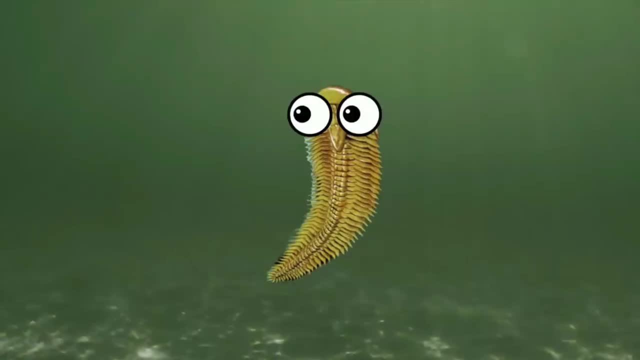 and this put us eukaryotes, in a bit of a tough spot, And this may be the first time that evolutionary pressure from another group of organisms started to affect the direction that evolution would go. You see, we eukaryotes seem to be a little bit more adaptive than the cyanobacteria. 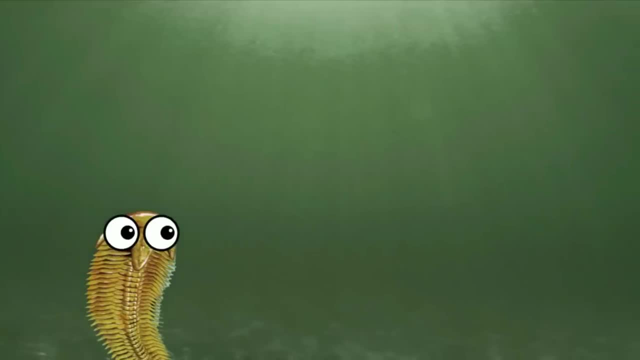 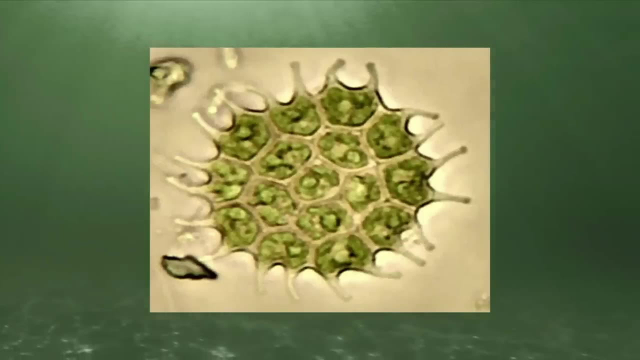 It's believed that, in the stale waters of the Boring Billion, our ancestors would branch off into three very different paths. The first would take a similar approach to the cyanobacteria and begin producing their own fuel from the sun, brought on by photosynthesis, Since sunlight was 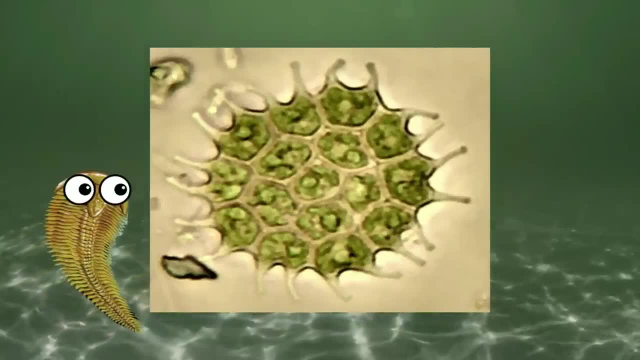 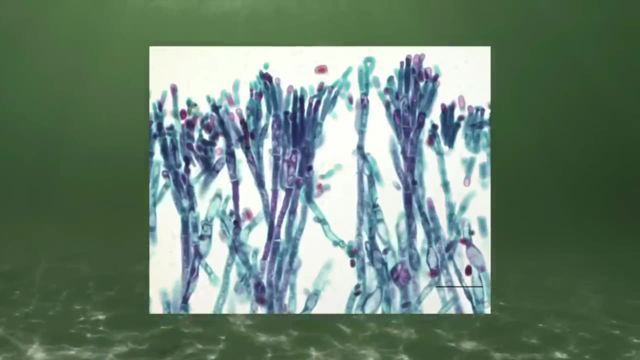 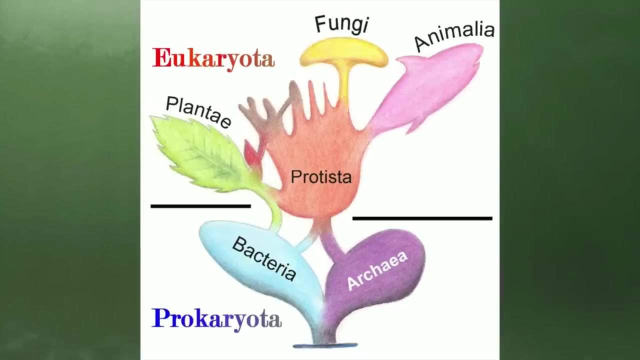 in plentiful supply and they didn't have to compete for it. Another would start breaking down the nutrients left inside the cells of dead organisms through decomposition. And finally, the last one, would start getting its energy from consuming other organisms. These are the most basic differences. between the three main kingdoms of multicellular eukaryotes. The producers using photosynthesis would eventually become the plants, the decomposers would become fungi and the consumers would become the insects. I should probably just mention real quick that there's way more than just three. 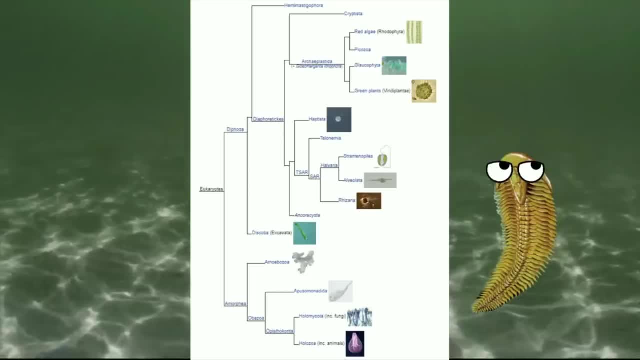 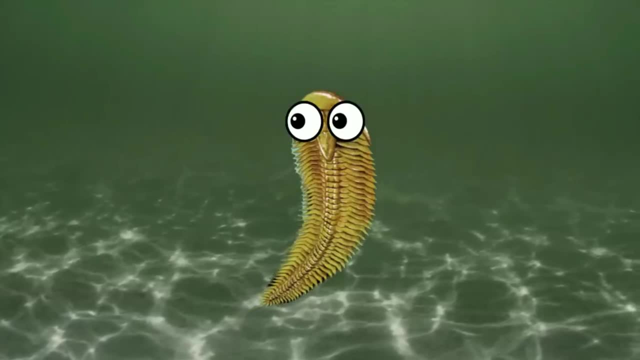 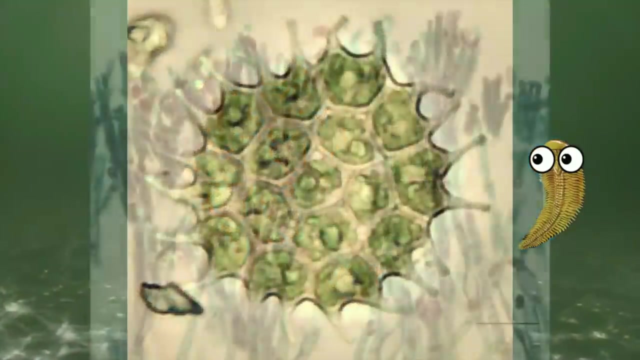 groups of eukaryotes, but for the premise of this story, those are the main three that we're going to be focusing on. So, in a way, the Boring Billion turned out to be very important because during this time, when the continents didn't even seem to be moving around a lot, the eukaryotes started to 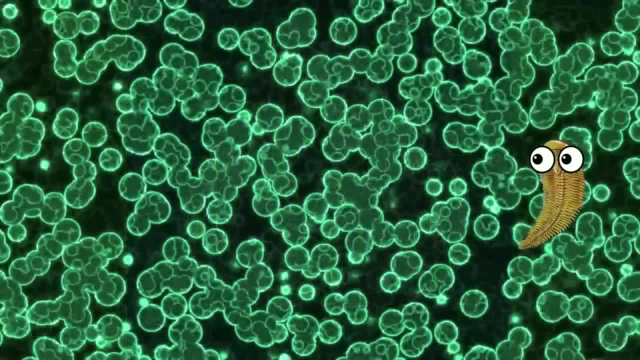 diversify. under the second cyanobacterian empire, Higher levels of methane given off by many, many or even a few organisms would be brought into the system, but for most of the time they didn't. For example, the eukaryote was the most plant-based plant that existed in the world and when it got 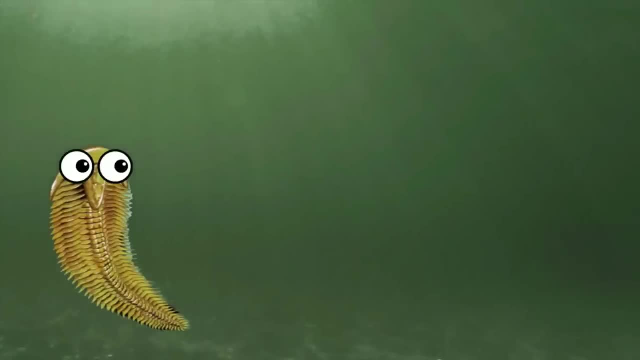 created, the eukaryotes would start to form a giant group of eukaryote, And that's why I would say that the Higher levels of methane given off by many of these microbes probably kept the water much warmer than during the Heronian glaciation. 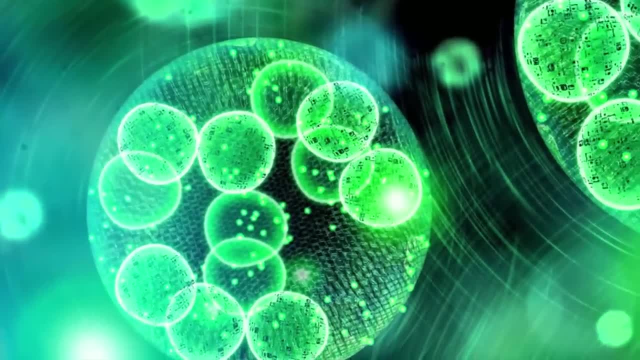 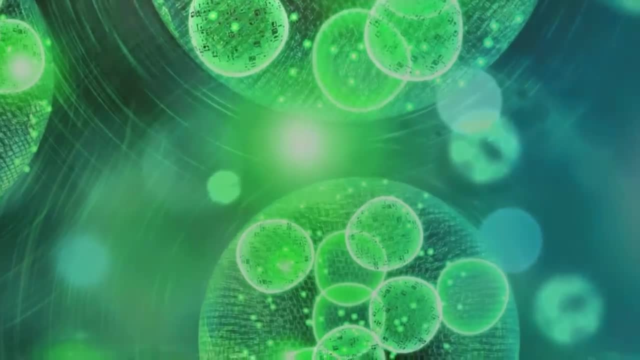 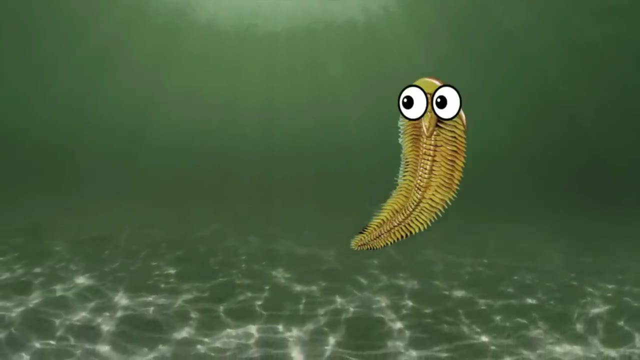 But as a result, the cyanobacteria continued to increase in population again, And inevitably they would have the same impact on the Earth a second time. And now, after all this time, we've arrived at something truly monumental Somewhere along the way during the Boring Billion. 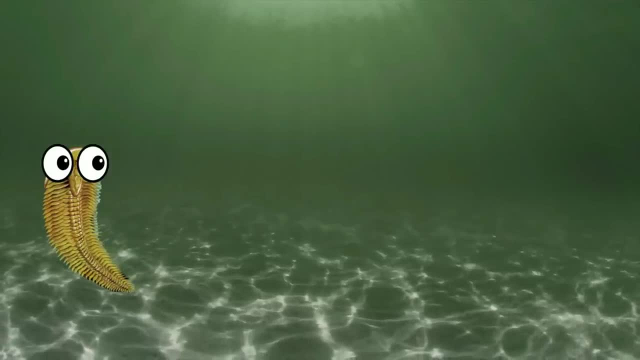 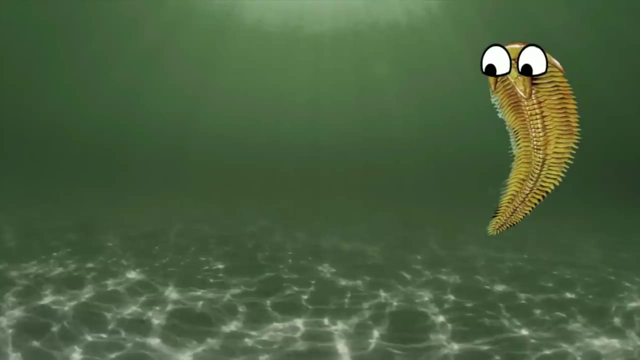 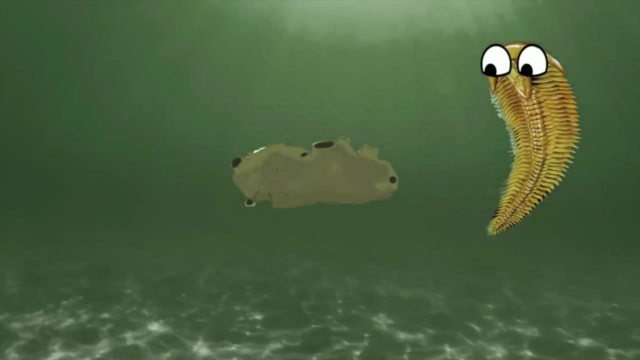 the different forms of life that evolved from the basal eukaryotes had become multicellular And around 760 million years ago, the very first animal with this new scale would appear in the fossil record, And it was a sponge. It was called Otavia. 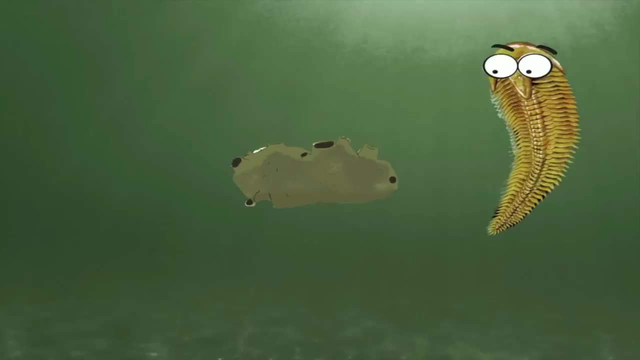 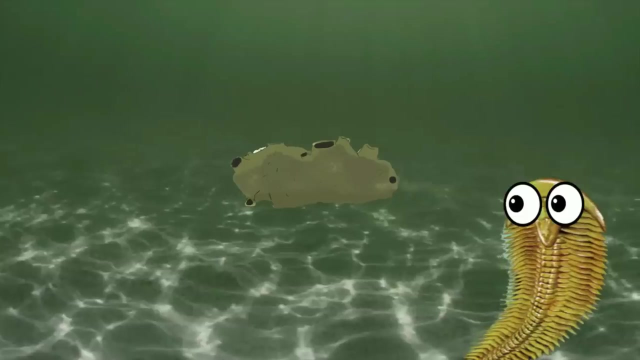 And although these creatures didn't have a nervous, digestive or circulatory system- and they still don't- they were still considered closer to invulnerable. They were closer to an animal than a fungi or a plant. They get their energy from filtering particles out of the water through their pores and 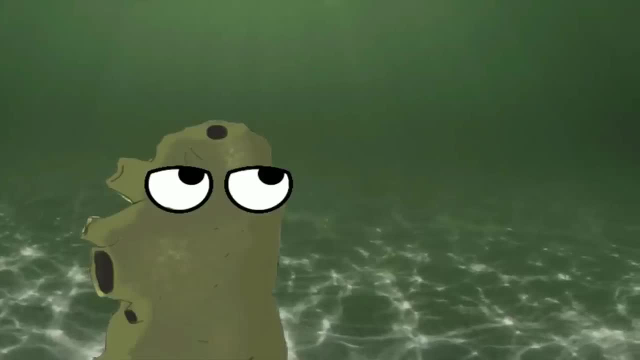 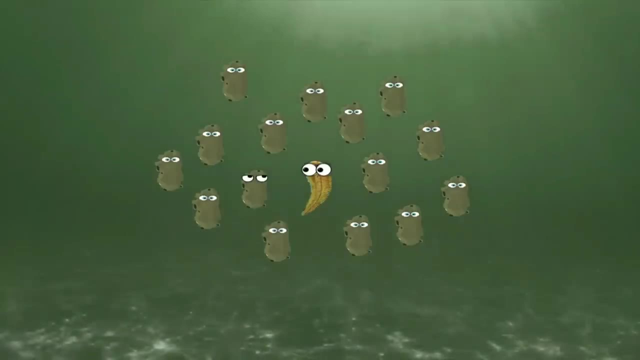 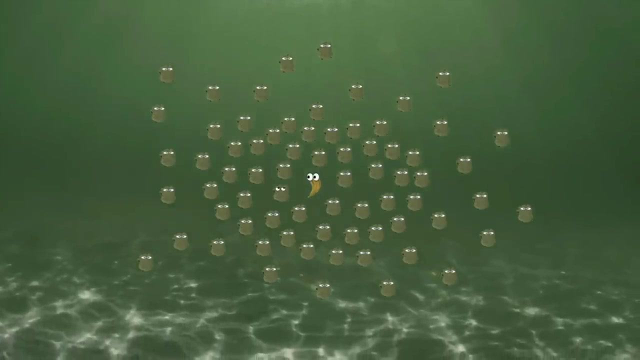 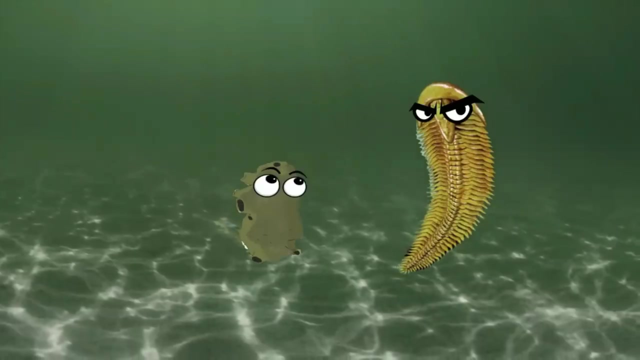 Wait, Wait a minute, Tim. Tim, That's right, I still live. Don't do that. I don't know how you managed to survive the oxidation catastrophe in Huronian Glaciation, But now we're about to get hit with a one-two punch of glaciations. 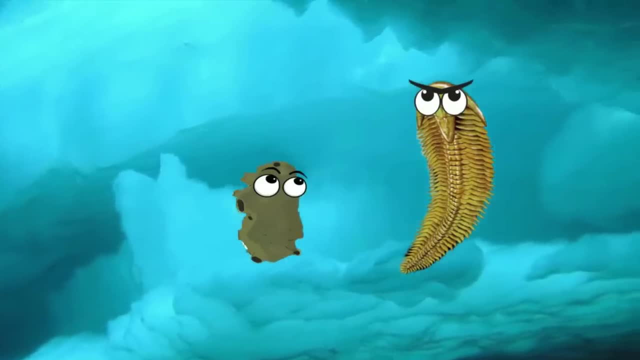 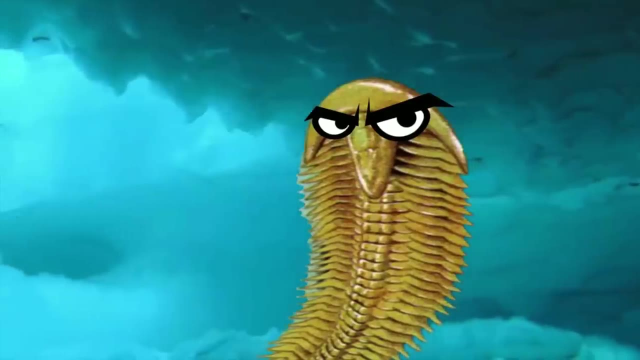 because your old friends won't stop multiplying and farting icehouse gases into the atmosphere. Yeah, okay, maybe some volcanoes might have had something to do with it too, But I'm still blaming you. But I'm not even a cyanobacteria anymore. 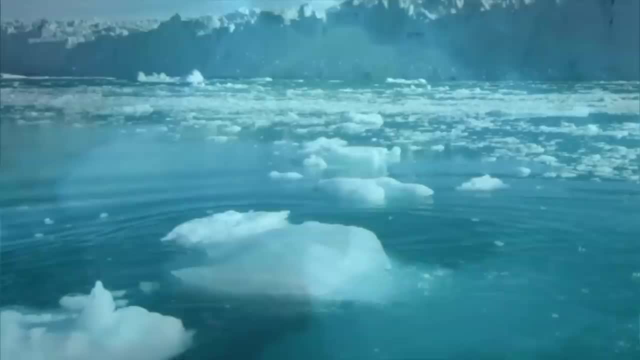 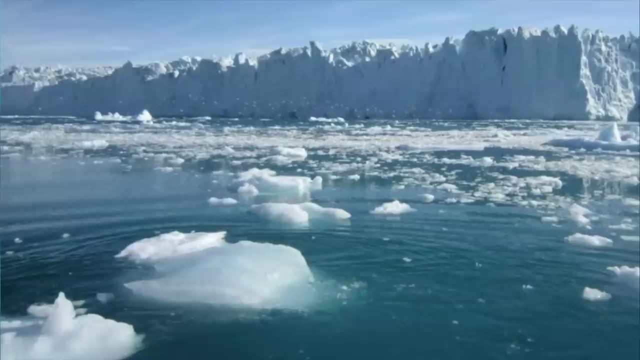 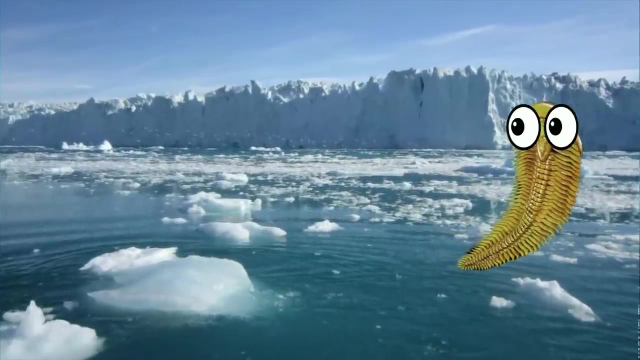 Shut up Tim. Tim The Cryogenian was a period in the Neocryonium Proterozoic that lasted from 720 to 635 million years ago. It was called this because the world, quite literally, was in a constant state of being cryogenically frozen and thawed During the 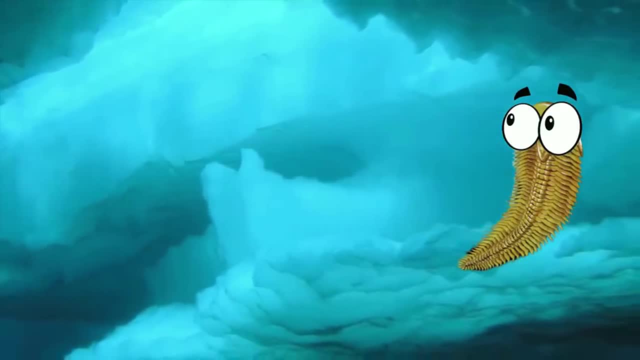 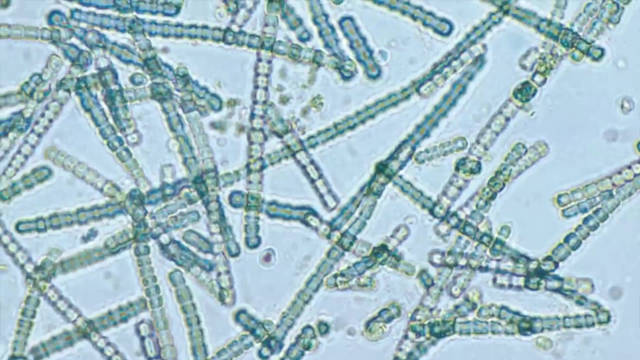 stretch of 85 million years, the planet likely became a giant ball of ice on two separate occasions. After all this, the world was in rough shape. The cyanobacteria were still around, but they were brought down from their status of rulers of the earth for sure As we enter the Ediacaran. 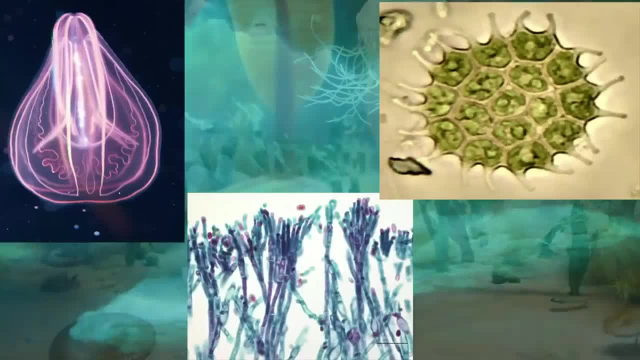 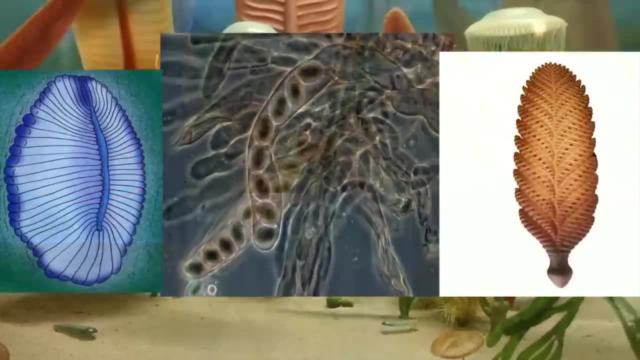 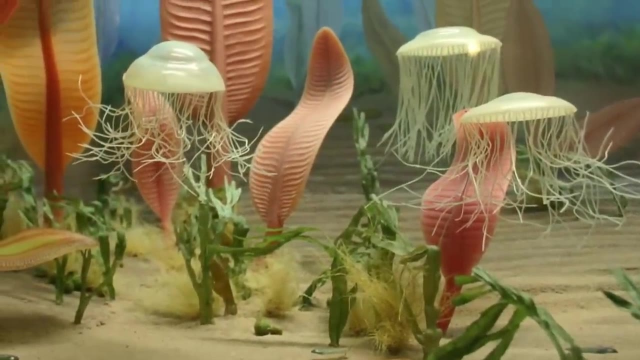 we see that a new group was ready to claim dominance. Somehow, all three groups of eukaryotes managed to survive the glacial roller coaster and come out of it ready to expand into new forms. It is here that we first start to see a seafloor that's populated with animals and plants. 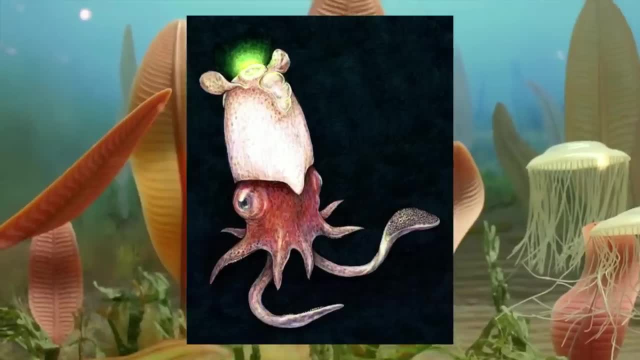 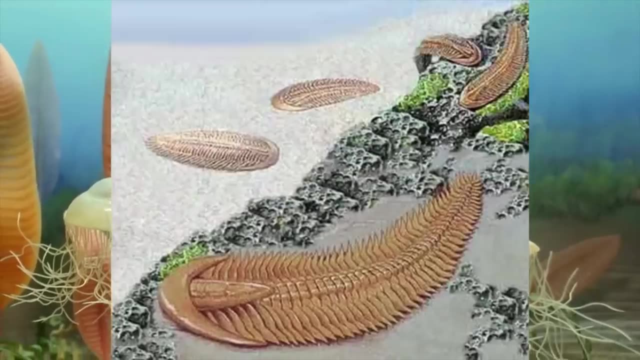 Jellies first started becoming abundant at this time, as well as possibly even the earliest basal settlements. The Eukaryotes were the first to survive the glacial roller coaster, and the cephalopods. That's still a debated topic, though It's also when we see my new form. 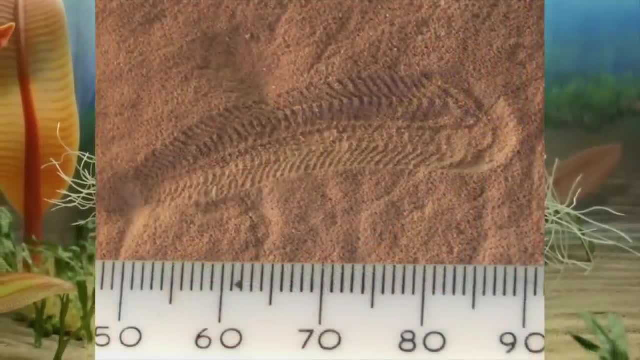 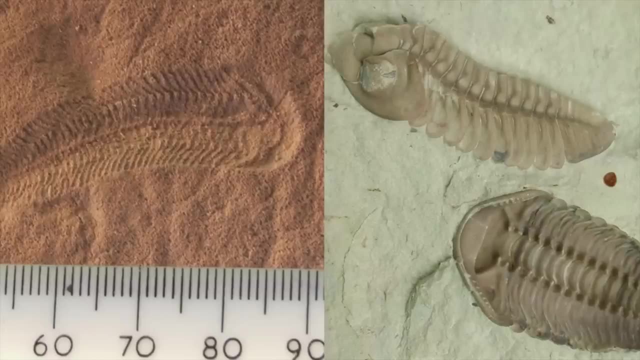 Spragina first appear in the fossil record in southwestern Australia, and you might notice that it bears a strong resemblance to a certain super widespread fossil that will appear in future episodes. One thing that we are sure of, though, is that, even though life was technically at its 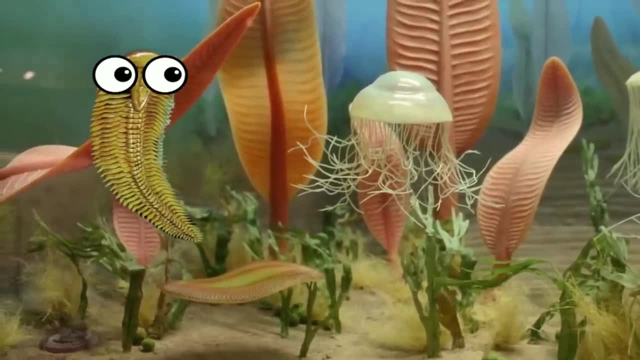 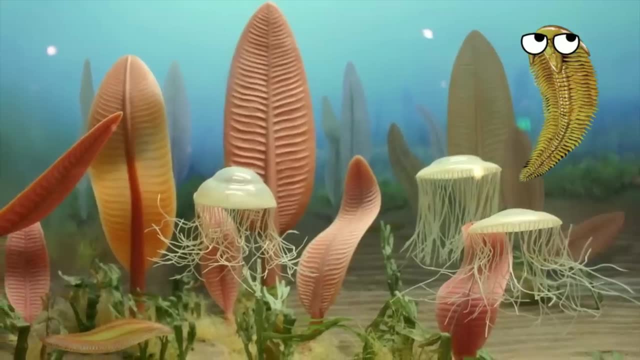 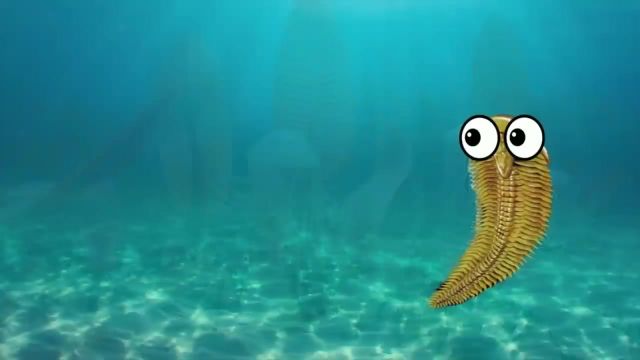 most complex as of yet. it was still pretty simple, Soft-bodied and most of them not even having brains. it's still a problem. It's still a pretty far cry from where we will eventually end up, but after being through every imaginable hellscape to get here, it's pretty beautiful, And now we've finally come to a big 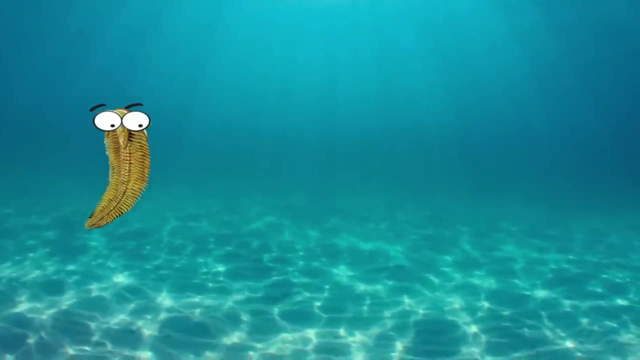 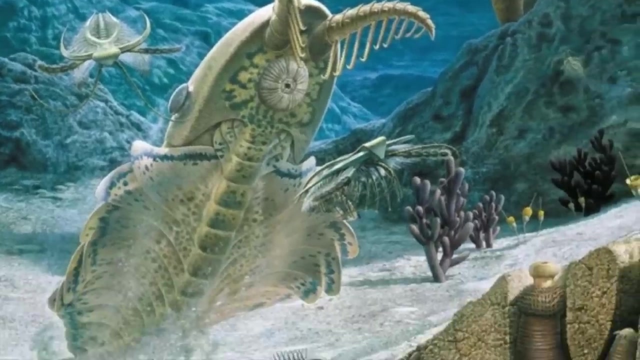 turning point. We've traveled through the first three eons- the Hadean, the Archean and the Proterozoic- and now we just have one left to go as we come to the dawn of the Phanerozoic Eon. 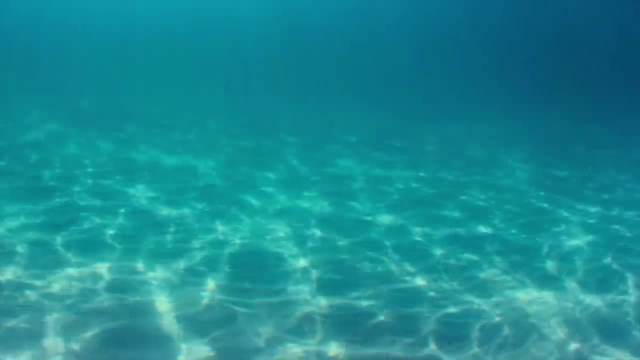 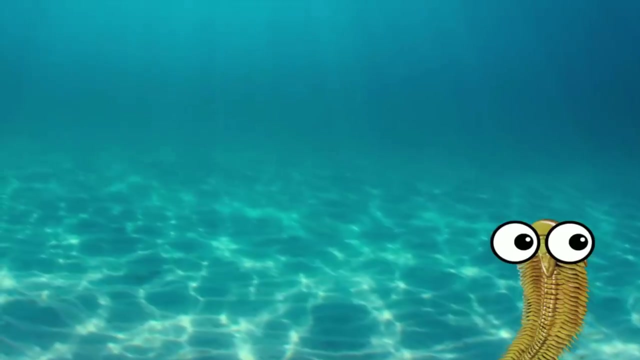 And here is where we'll need to slow down quite a bit, no longer flying through an entire eon in a single episode. Next time we'll start to get a lot more interesting, which is good, since I don't actually know how much longer I could stretch out the story of the Precambrian. 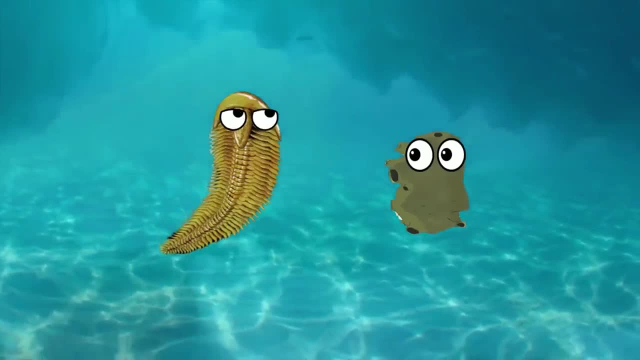 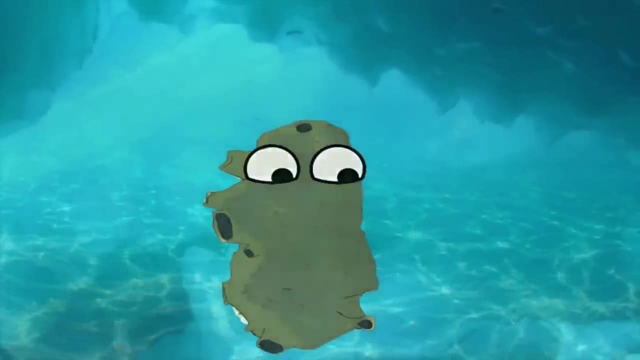 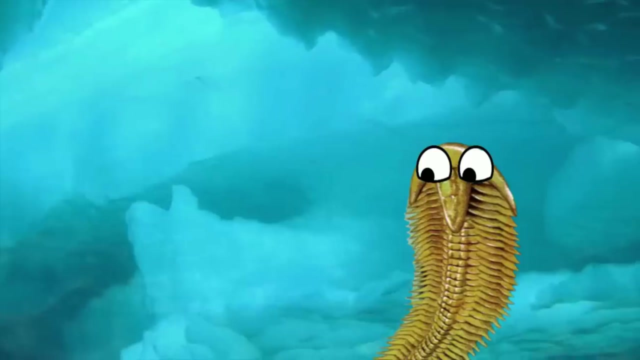 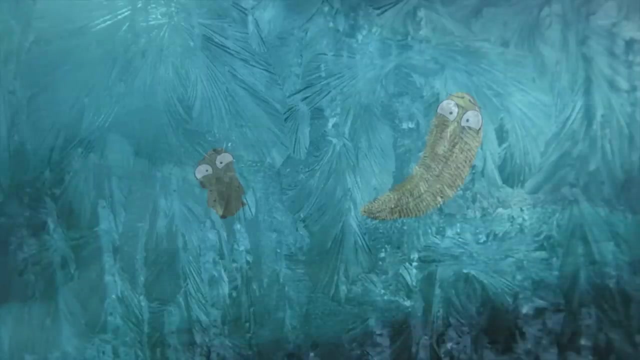 Alright, Tim, Tim, come on, I guess I'm stuck with you for now. I am the ultimate survivor. Yuck, Have a good one, everybody. Wait, did I miss something? Uh-oh, Help me, Help me. 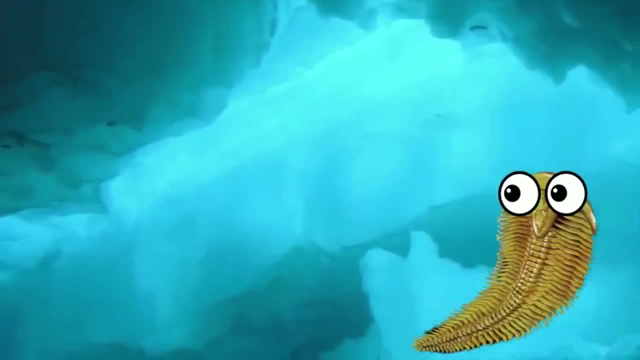 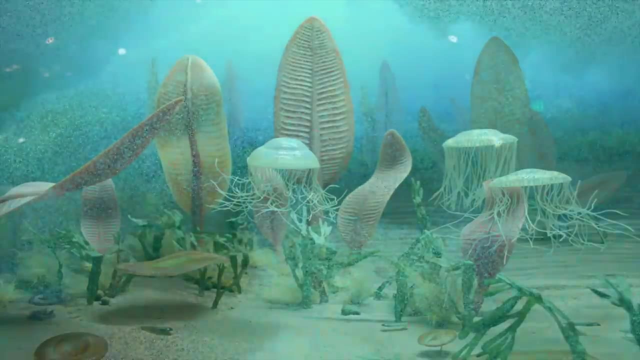 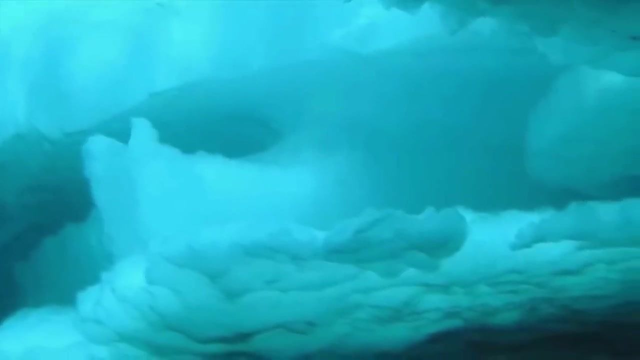 In the last episode, we discussed how, during the Proterozoic Eon, the Earth froze on its own. The Earth froze into a giant snowball three different times. These events may have caused mass extinctions each time, and the ones who survived would evolve into new species that would fill the niches left vacant by the ones who didn't make it. 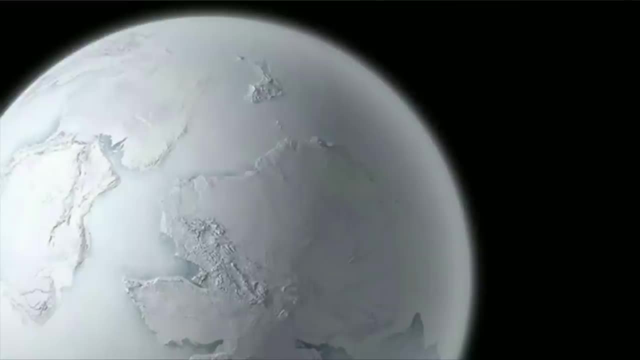 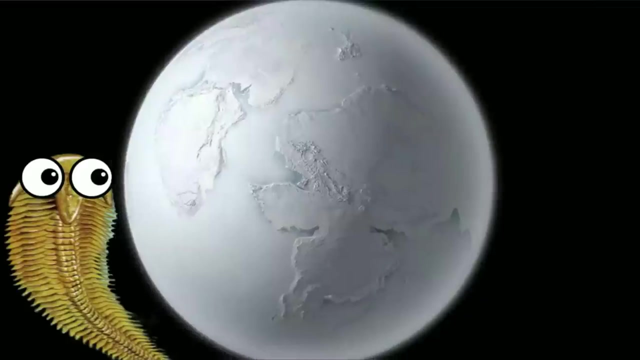 As you can see, I clearly missed one. There has been fossil evidence found that suggests that at the end of the Ediacaran there was a fourth major glaciation, And this would be the event that brought the entire eon to a close. 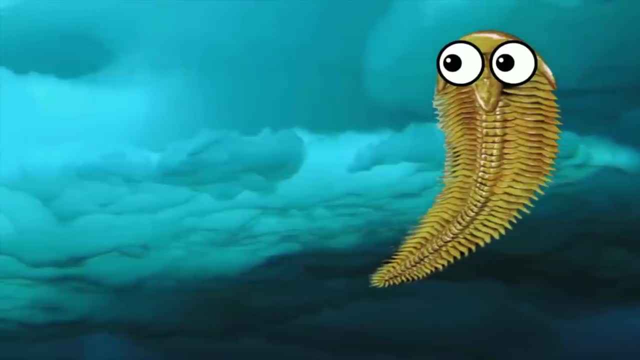 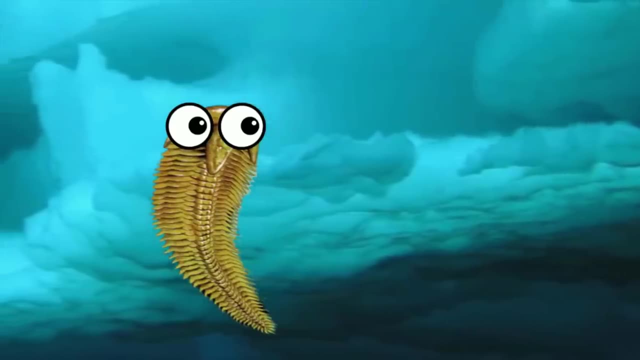 There's a lot that still isn't known about this glaciation. In fact, some scientists aren't even convinced that it happened, But if it did, it would help explain one of the most dramatic and mysterious events in all of Earth's history. 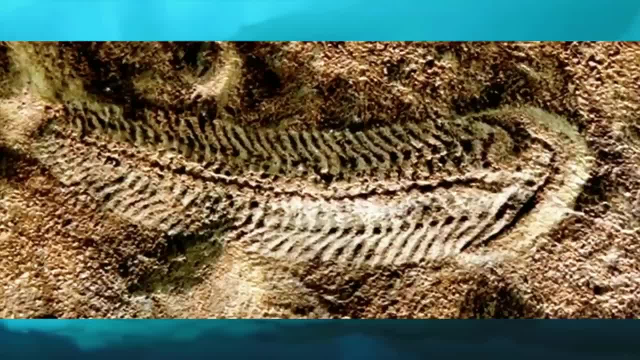 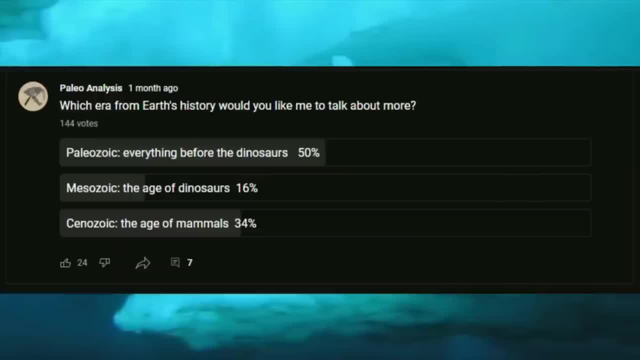 It's thought to have made life increasingly difficult for many of the squishy guys that were around at that time As we move into the beginning of the Paleozoic Era. Remember that poll I did a couple weeks ago where I asked what era you all wanted me to focus on the most? 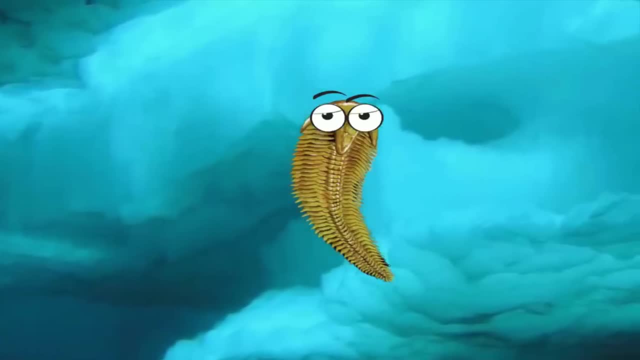 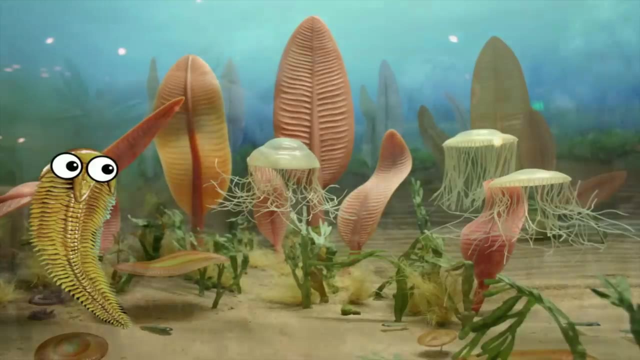 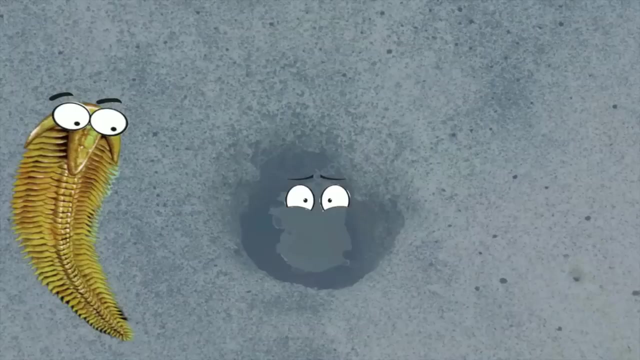 Well, here you go. We finally actually made it to a time period complex enough to actually be covered by most major documentaries. There's going to be a lot of changes moving forward from here, And it all started with Wait, Hey, Where'd Tim Tim go? 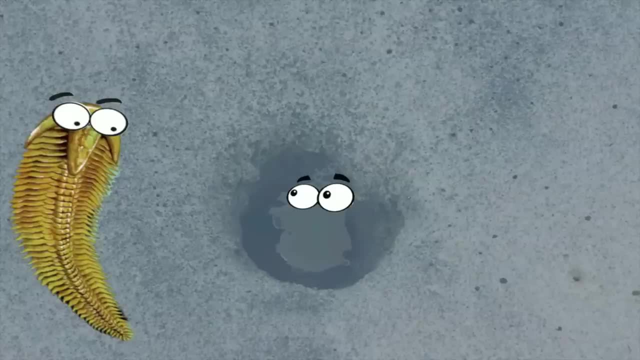 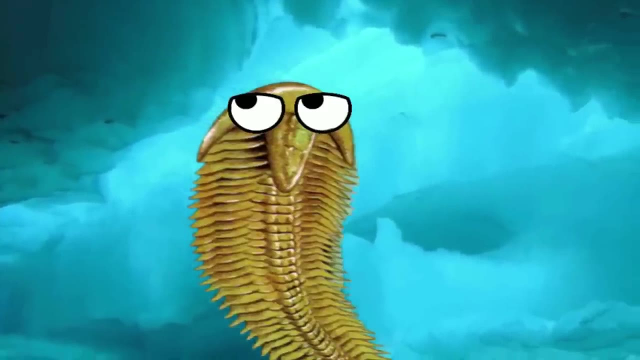 Tim Tim, What the crap are you doing? Some of us smarter squishies are trying to survive by hiding out in burrows. Alright, well, you gotta come out. People apparently like seeing you for some reason. Screw you, it's out. 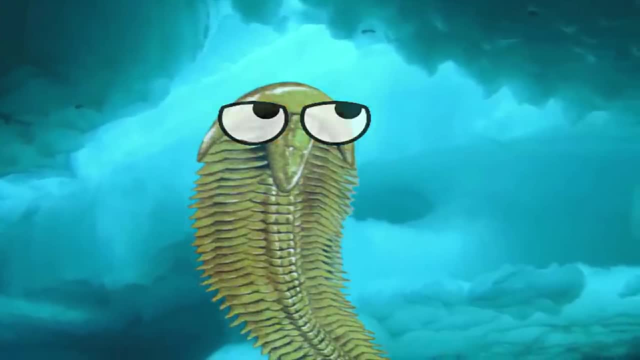 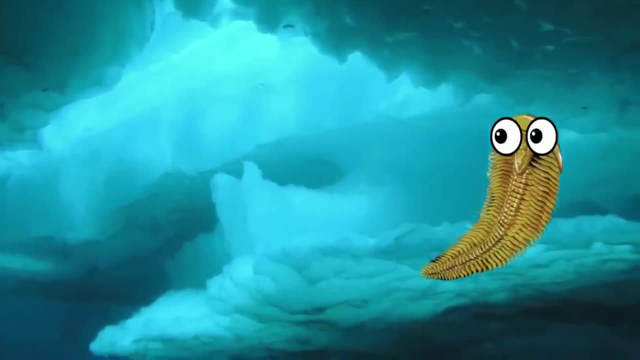 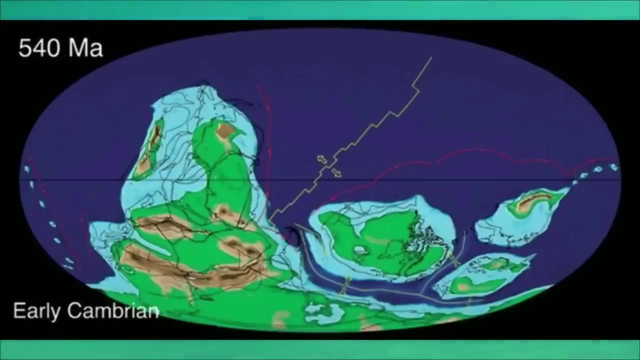 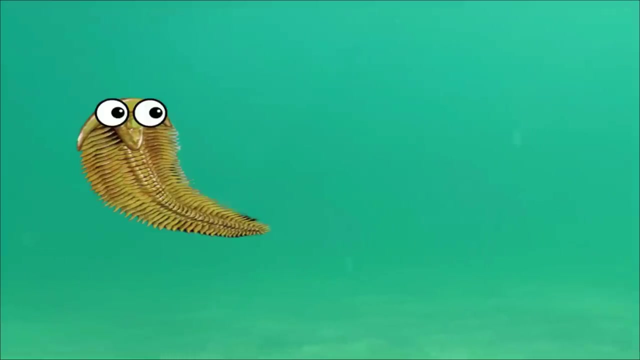 Whatever I'm going on without you. then, As the world recovered from this big freeze, the life that managed to eke out a living by being hardy enough or by taking refuge in burrows were about to go through an amazing transformation. Around 541 million years ago, as the oceans thawed out once again, there would be a ton of new niches left open, and the survivors would be ready to take advantage. 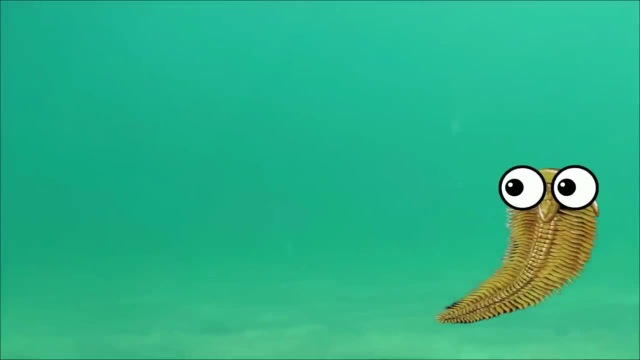 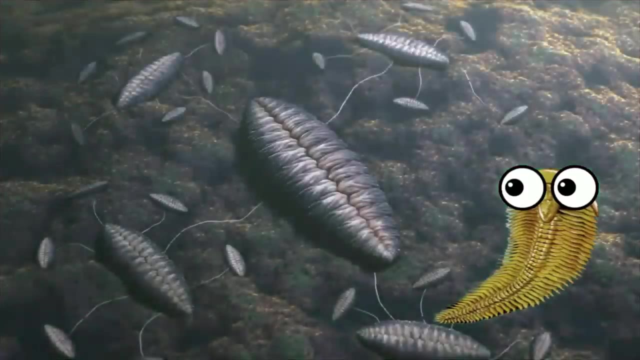 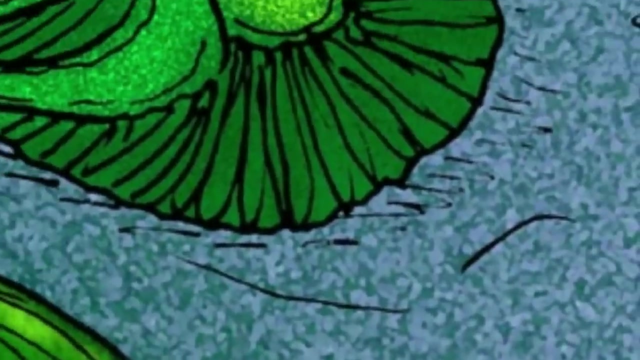 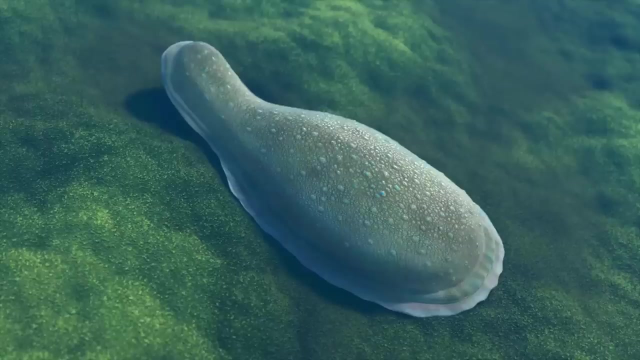 There was one thing missing from this puzzle of evolutionary forces, One thing that made this event stand out, more than just adaptive radiation, like we've discussed before, And that one thing would change everything from this time moving forward. You see, up until now, the animals that we have discussed only got their energy and nutrients by passively feeding on photosynthetic organisms through filter feeding or slurping goo out of the sand. 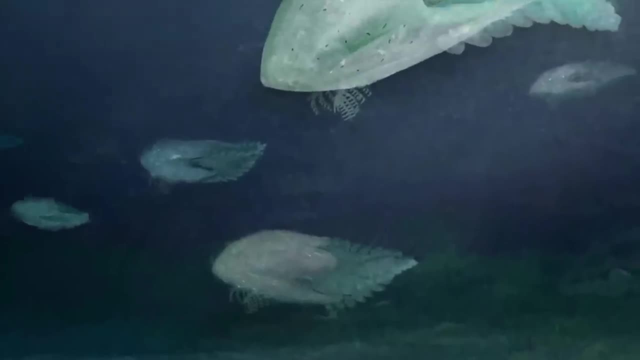 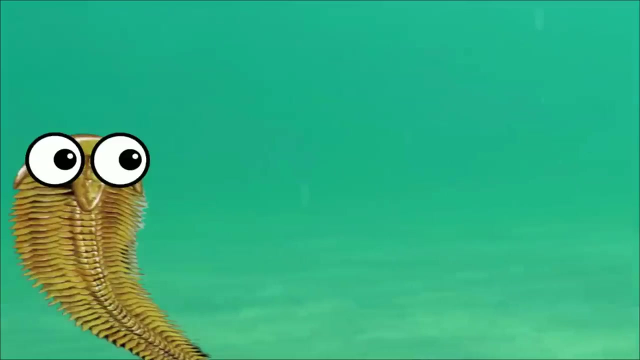 But now, for the very first time, we see animals actively hunting and eating other animals, And this would change the game forever. Suddenly, it wasn't enough to simply have the means of collecting food and a strategy to survive, whatever the Earth was throwing at us. 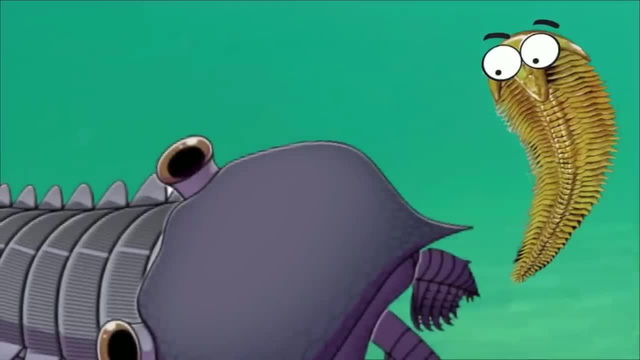 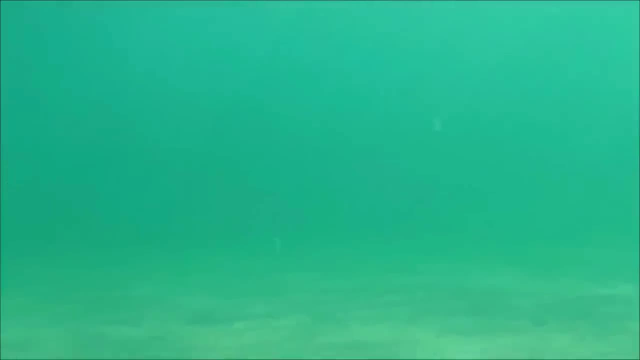 Now, all of a sudden, animals were out to get other animals, And the ones who didn't figure out a way to respond to this were easy prey. The first thing that every animal needed if they were going to survive in this competitive new ocean was a way to detect other animals around them. 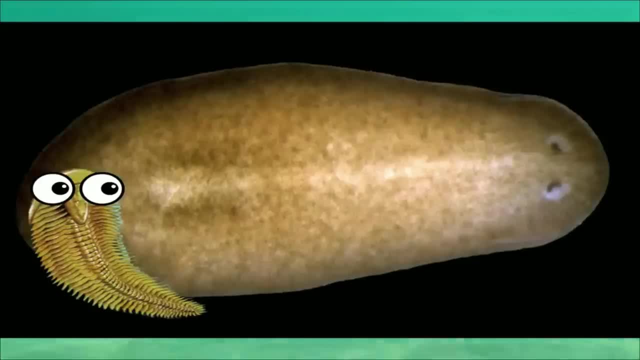 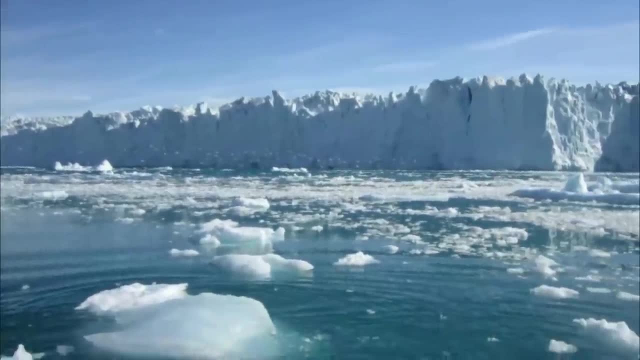 And luckily there was already many different creatures that were out there, Many different creatures that had basic light sensing organs on their heads. This may have first evolved during one of the glaciations to find areas where the ice was thin enough for light to shine through. 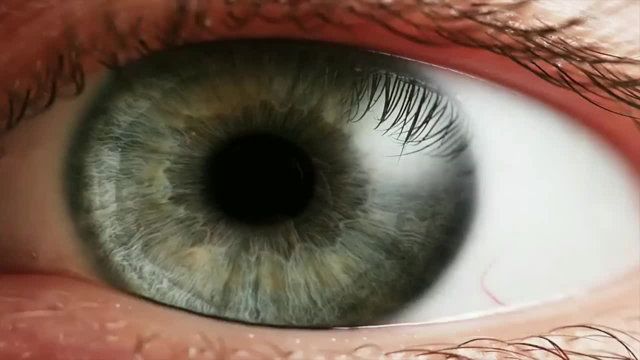 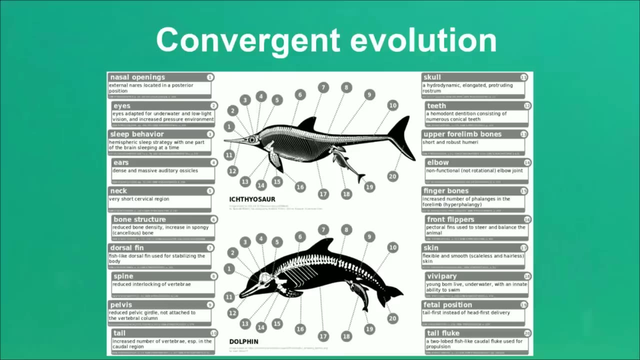 And now it'll become the basis for the very first eyes, And it seems that eyes may have actually evolved simultaneously in different, unrelated groups. This is a process called convergent evolution, A term that you should remember because it's going to come up a lot as we move forward through time. 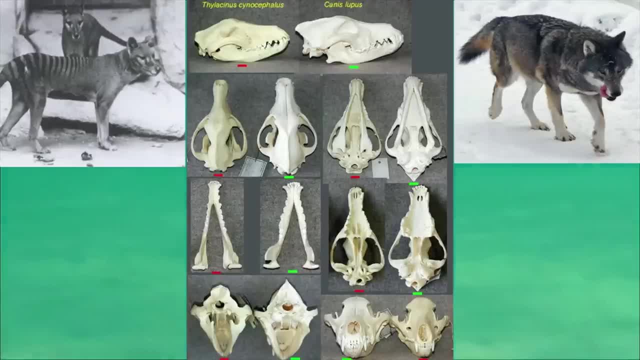 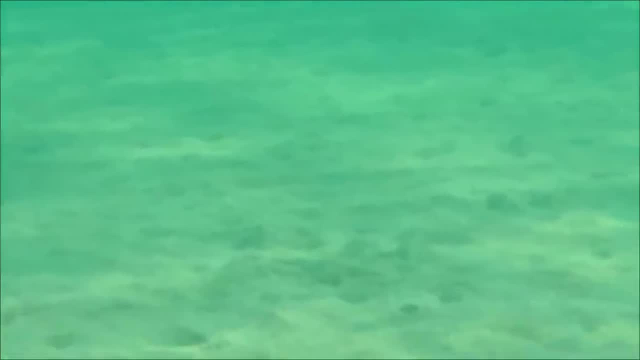 Basically, this is when two unrelated species evolve similar strategies or body types despite not being closely related. But now that animals could see one another, now they needed a way to deal with each other. There would be two major body plans that would really take off during this time. 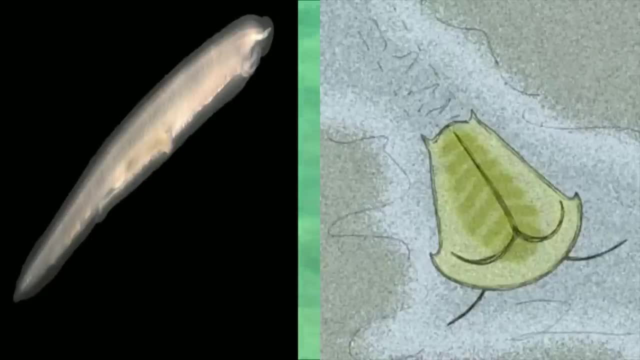 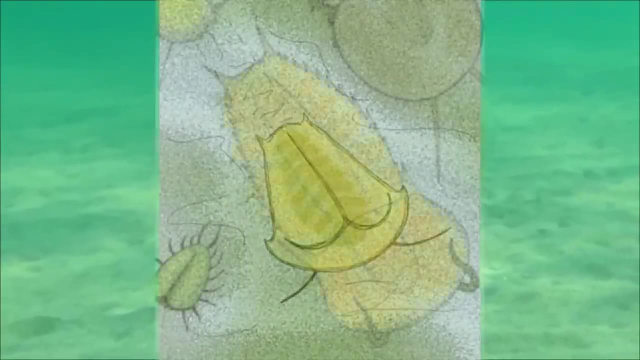 Or at least two major players that we're going to be focusing on moving forward. The first group would have a hard, bio-mineralized layer of armor around the outside of their body. This exoskeleton would protect them from attacks from carnivores. 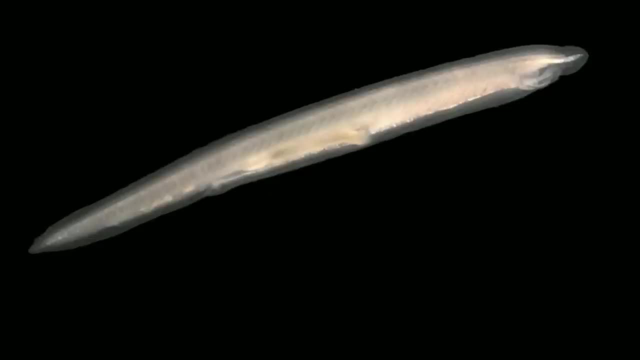 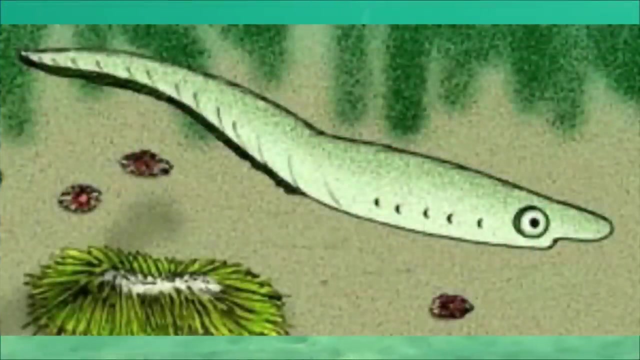 and become a staple feature among the arthropods. The other would develop a flexible dorsal cord that became the central point of the animal's nervous system, While also allowing for greater maneuverability and speed. This would become the template for every animal under the phylum Chordata. 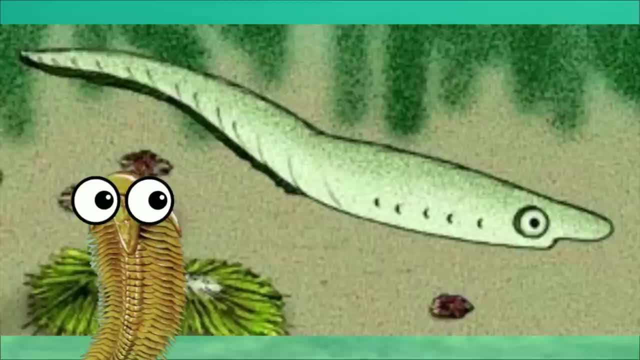 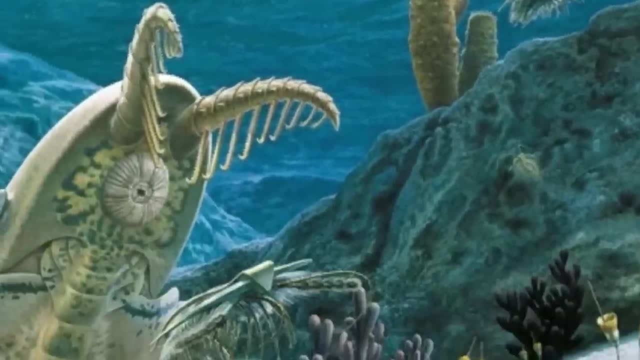 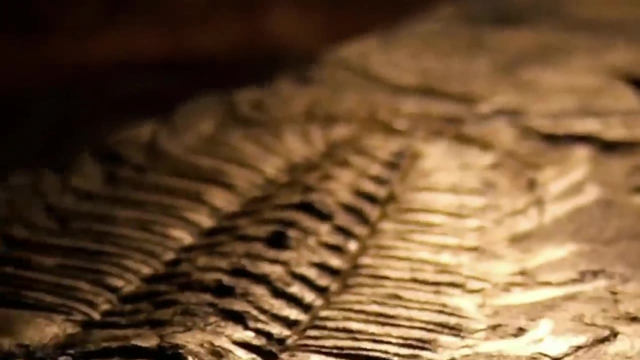 In other words the very first vertebrates, Thus making this one of our earliest ancestors. This evolutionary arms race between animals trying to basically one-up one another would become the driving force behind the Cambrian exception, The Cambrian Explosion, Where the combination of all these factors would culminate in adaptive radiation going into overdrive. 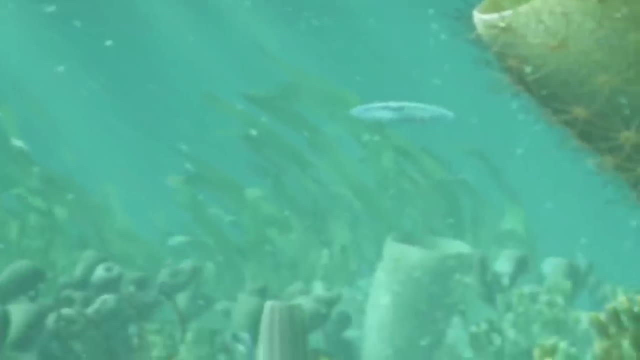 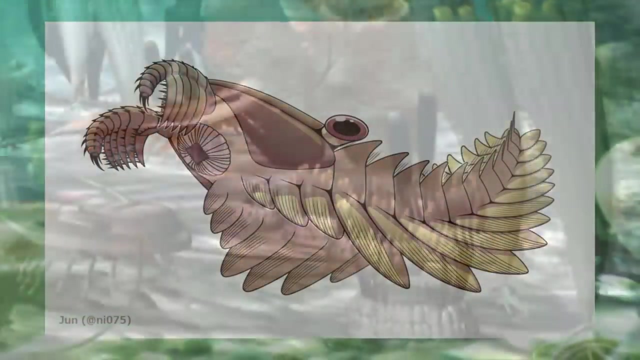 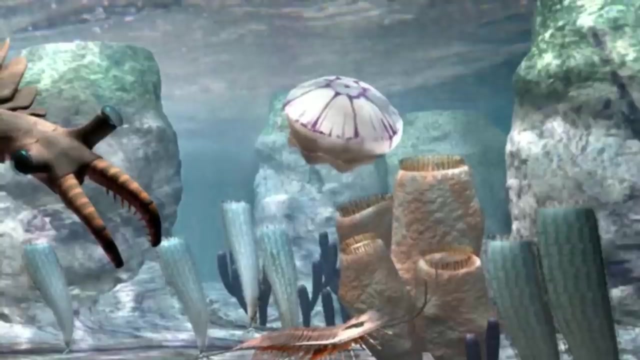 From 541 to 516 million years ago is the time that we call the Cambrian Explosion. Because of niches opening up and certain groups becoming predators, the oceans quickly filled with a menagerie of new, more complex forms of life than anything we've ever seen before. 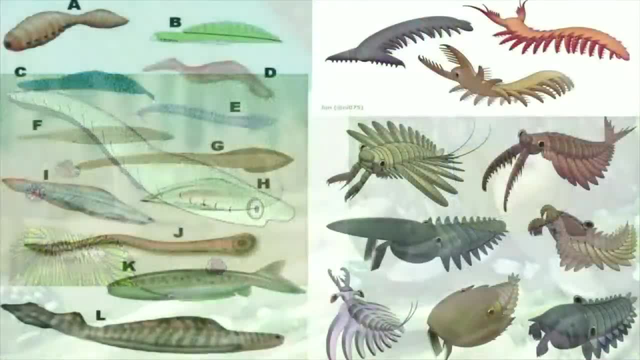 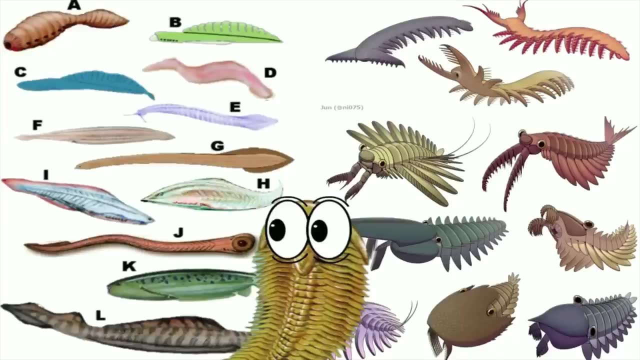 The basal, vertebrate and arthropod body plans had started reinventing themselves into every possible form nature could come up with, And it is impossible for me to be able to list off every new type of creature that we see in the fossils from this time. 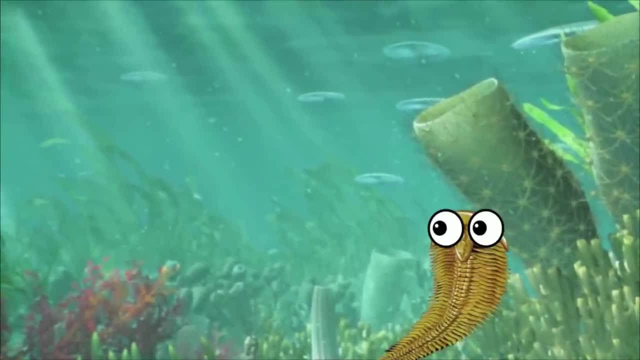 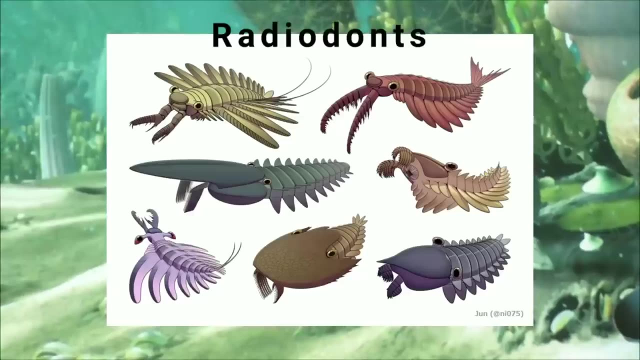 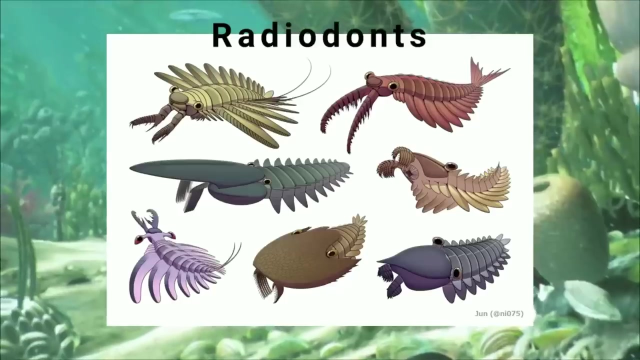 I feel like I could make several list videos talking about the different bizarre animals of this time, in the same vein as my Triassic Weirdo video. As this time started out, it seems that a group of arthropods called the Radiodonts started to become one of the most dominant groups. 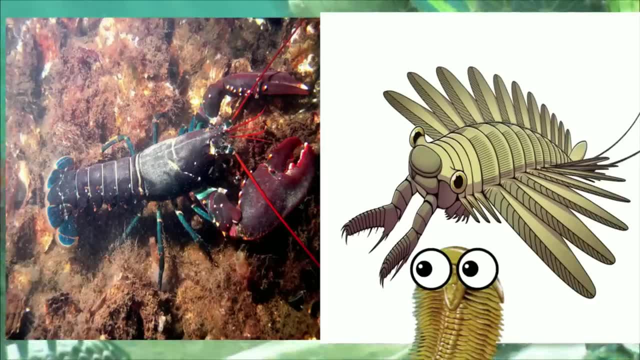 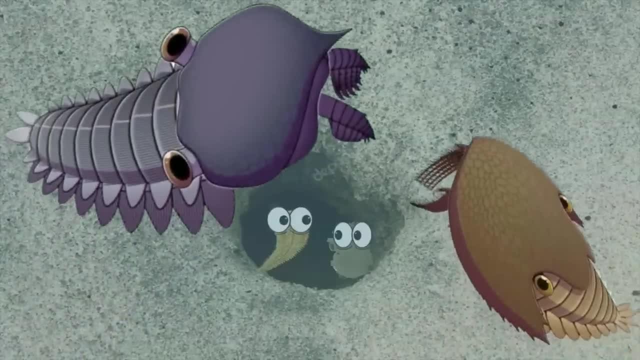 They in many ways share a lot of similarities with shrimp and lobsters, But maybe, if you cross those with the facehuggers from the Alien franchise, The rest of the animal kingdom had to come up with something, Because squishy worms and sponges were not going to be enough. 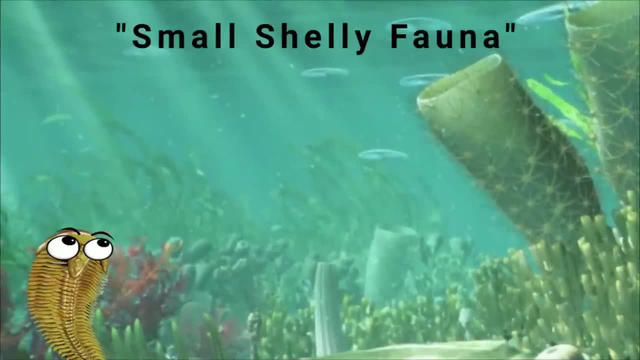 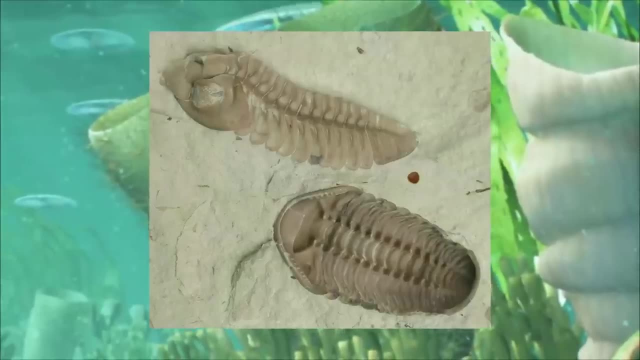 Some of the next things that we see evolve are what scientists call the Small Shelly Fauna. These were things like the first Gastropods, Brachiopods and Trilobites. Now it's impossible to say for sure if Trilobites are actually the direct descendants. 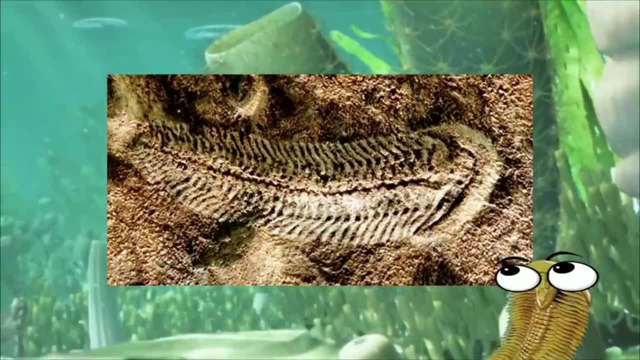 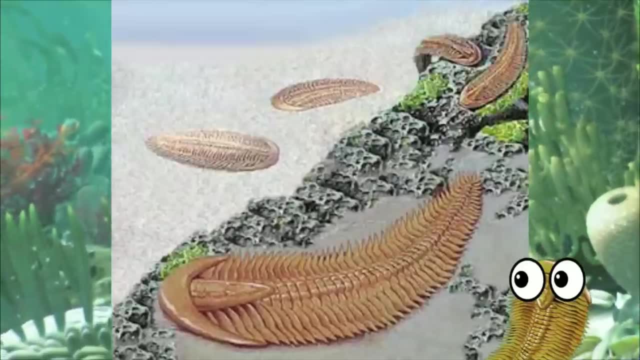 of Sprigina, like I said in the Ediacaran, But I personally feel like there's something of a family resemblance. But Sprigina was soft-bodied, more like a worm and definitely not like the pillbug-like critters of the Cambrian. 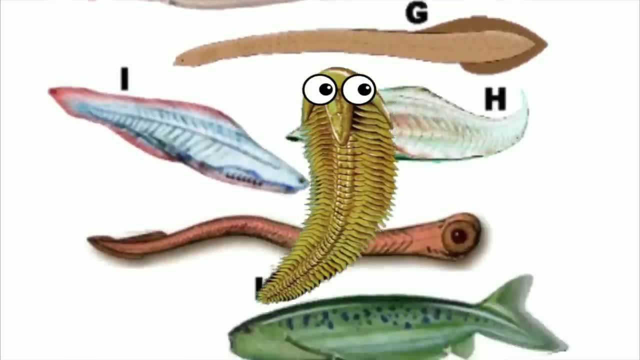 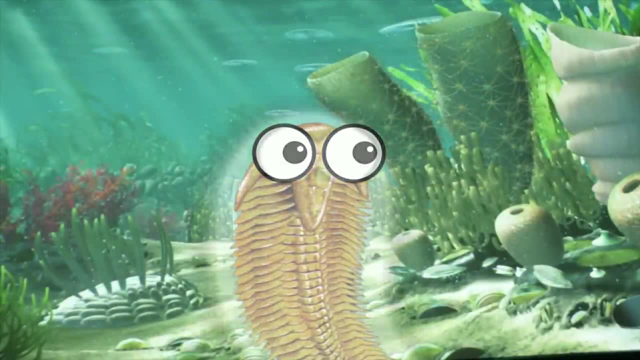 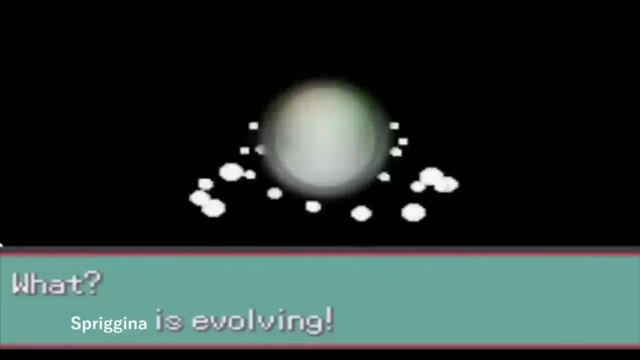 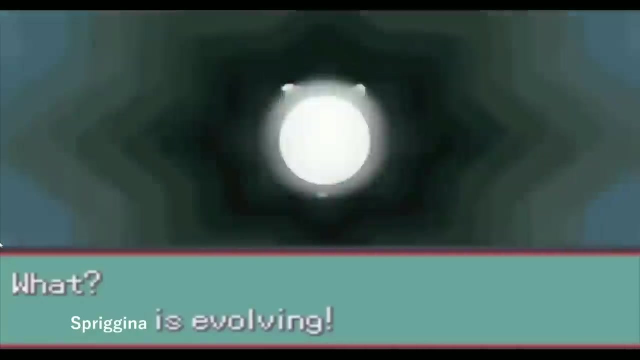 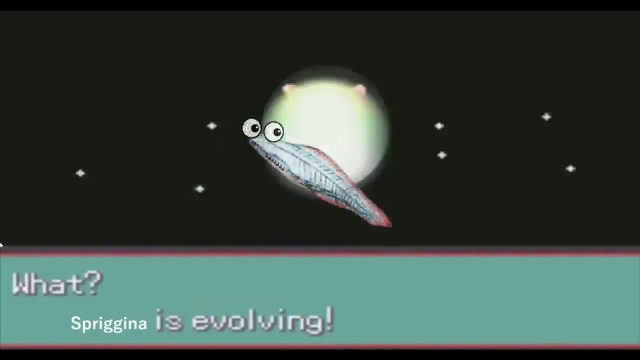 And it's also believed that the worm-like creatures branched out into those primitive chordates. And that's the path that I'm going to take this time, because that's the path that will inevitably lead to me becoming human again. Alright, Well, at least I have a spine. One of the earliest known chordates appeared around 535 million years ago, Named Hycoichthys. I think it shows characteristics of being the first ever fish And, even though that's probably a broad generalization, it's likely that it was at least very fish-like. 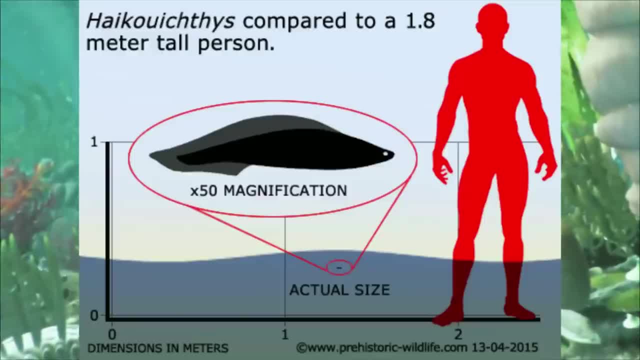 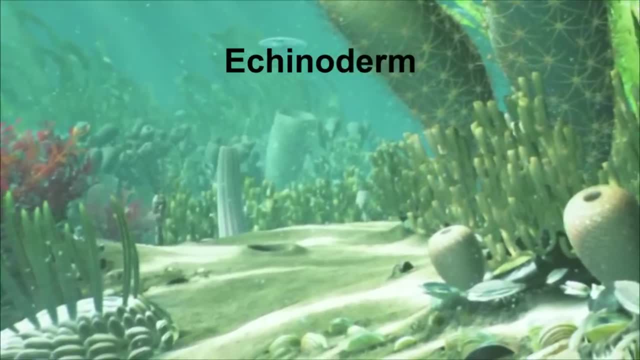 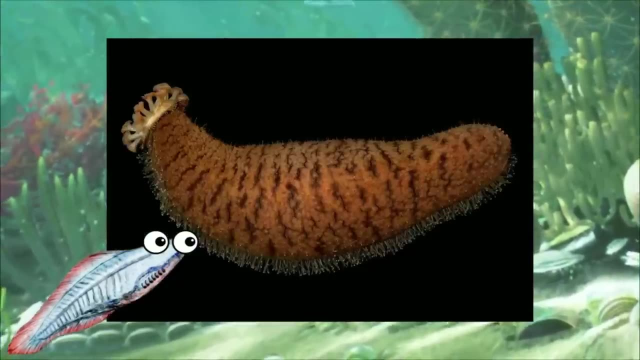 At only an inch long, with a flexible nerve cord on its back. this gave our ancestors a whole new strategy of avoiding arthropod predators. Echinoderms also evolved during the Cambrian as well, An expansive group that encompasses starfish, sea urchins, sand dollars and sea cucumbers. As well as a group called cranoids, or sea lilies, That look more like plants than animals at a surface level, Despite having a mineralized layer as well. these guys pretty much all used the strategy of avoiding the notice of other animals. 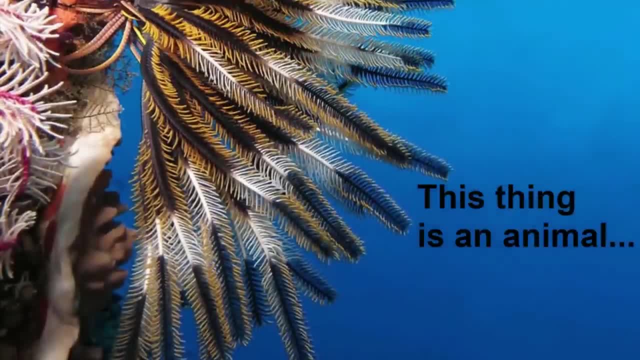 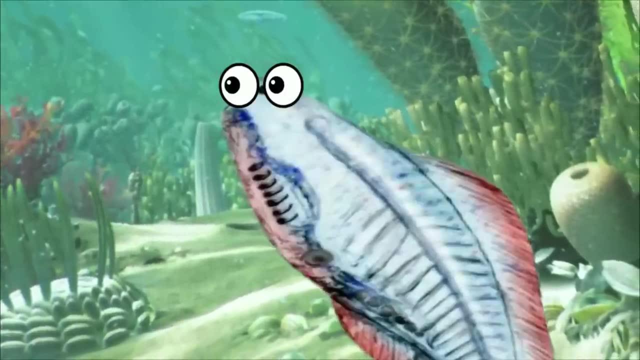 And in addition to all these groups that would give rise to many of the different groups of animals that we see today, there was also some really, really bizarre stuff. Stuff like the Cambrian freak show known as Hallucigenia- Now, with a name like that, you know this is going to be good. 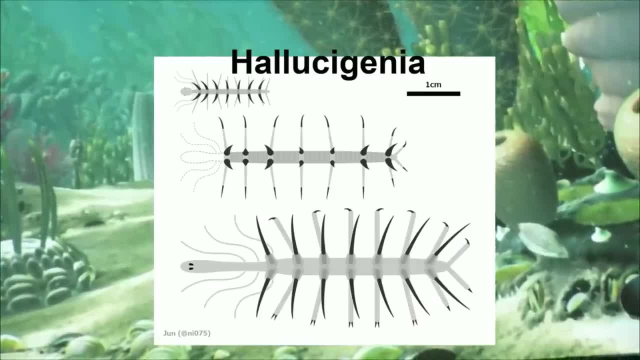 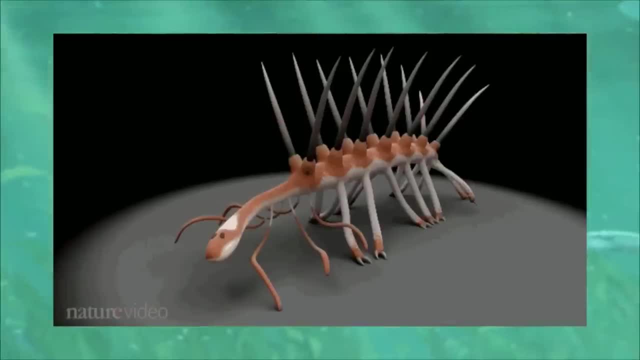 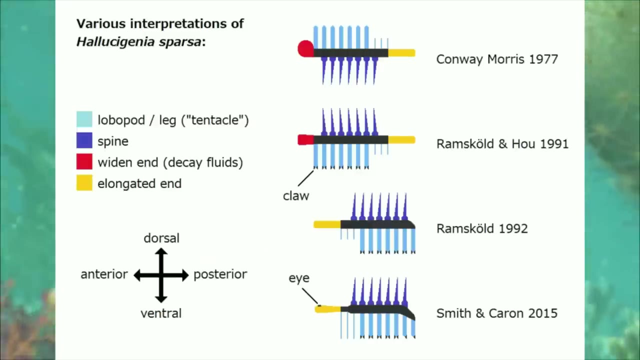 This biological erector set is supposed to be some sort of stem velvet worm And one of the most outlandish things to come out of our planet's deep past. It was originally believed that these tentacle spine things were legs. Some even thought that each one ended in a mouth that connected to a central stomach in the trunk. 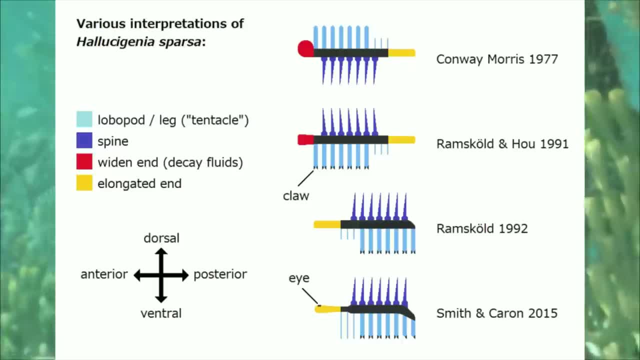 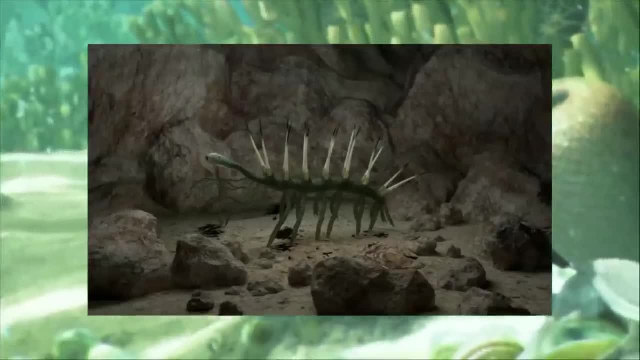 But then, in 1991,, it was discovered that scientists were actually looking at this thing upside down. Seriously, though, can you even blame them? It's now believed that these appendages serve the same purpose as every other major adaptation that we've talked about so far. 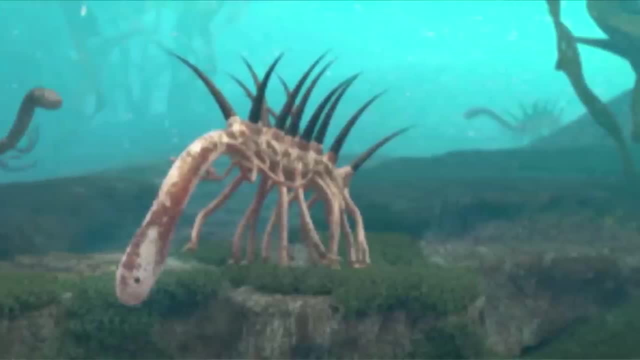 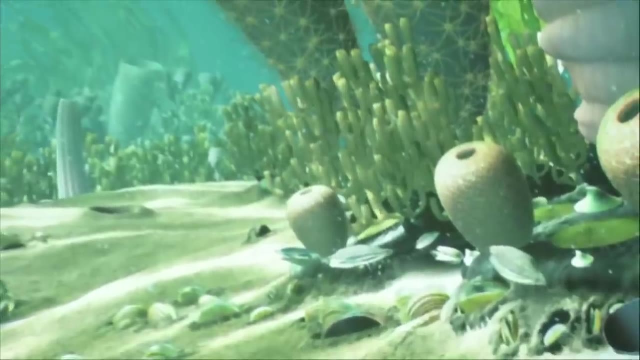 Being some type of defensive spines that these creatures evolved in response to the growing threat of predation in the shallow coastal seas of the Cambrian. This was an astounding amount of biodiversity within just a few million years, And we only have a small handful of snapshots to this time. 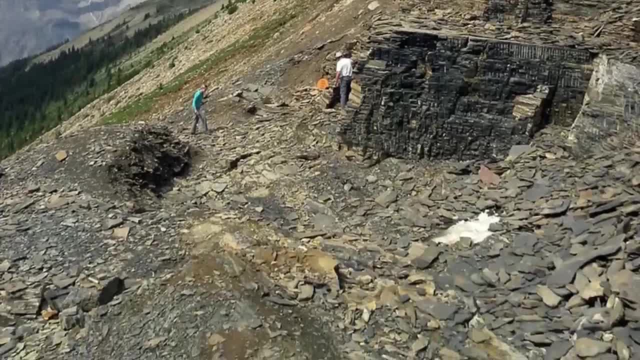 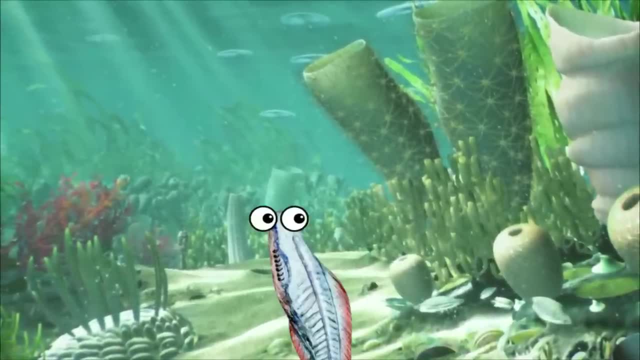 that allow us to learn about this pivotal part of our planet's past. So there's no doubt that there was profoundly more creatures inhabiting the Earth that we still haven't discovered, And in fact we may not, In fact we may never discover all of them. 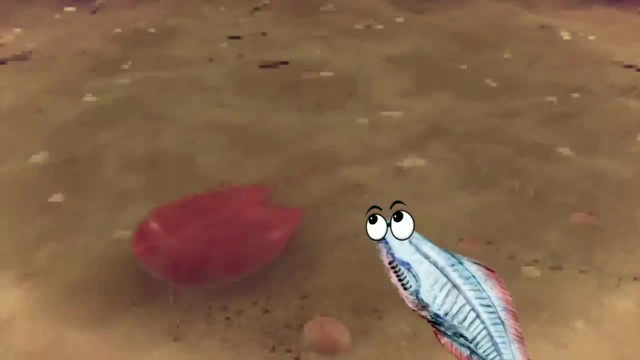 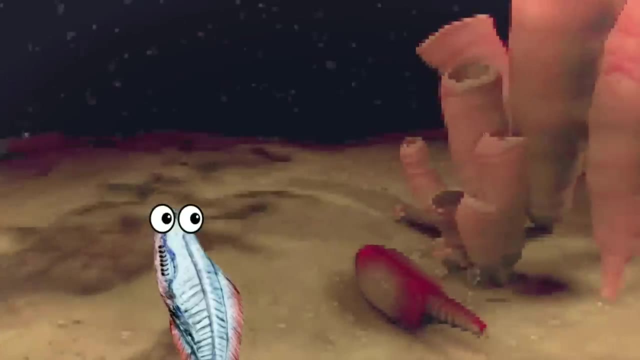 As we move into the middle Cambrian, the oceans become full of life and many of these different groups that got their start in the Cambrian explosion start to specialize. But life on Earth definitely looked very different than it does today. There may have been a few groups here and there that looked somewhat familiar. 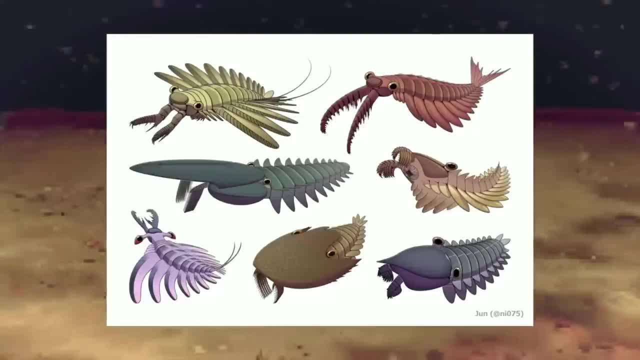 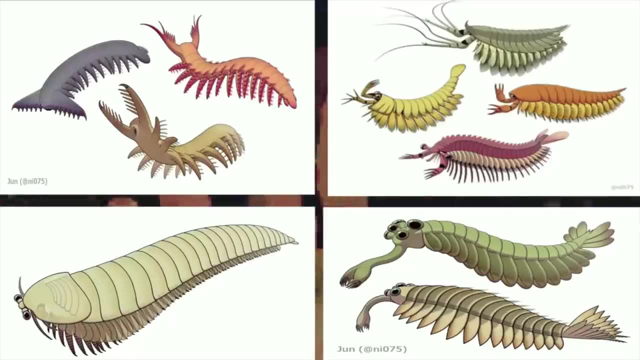 But for the most part, this was an alien world. The arthropods had further perfected their radiodont design by evolving into several other orders. They came in all different shapes and sizes, One of the most well-known families being a small, five-eyed monster. 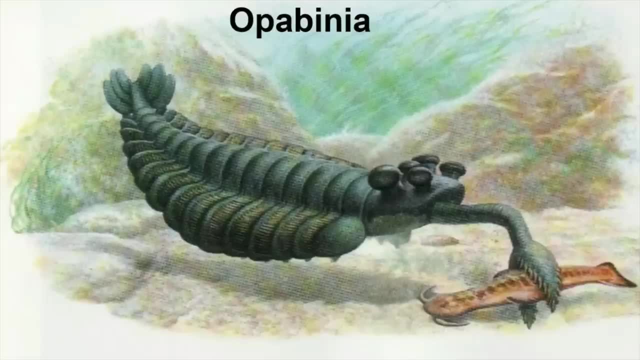 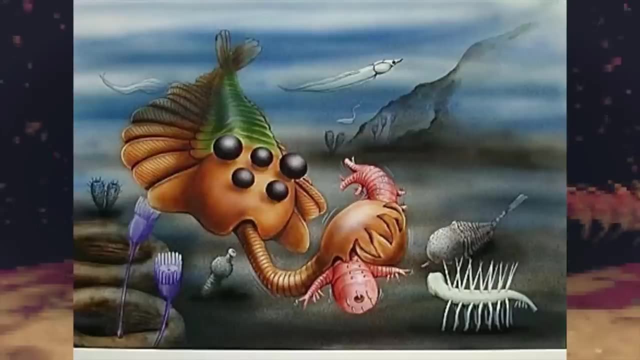 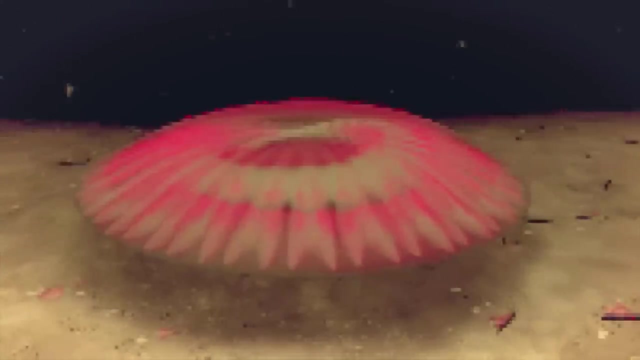 with a long trunk and a claw at the end of it for grabbing prey. It was called Opabinia And, at only seven centimeters long, it definitely wasn't the ruler of the seas, but it was a very specialized predator. You see, some creatures continued to use the strategy that had allowed them to survive the end of the Ediacaran. 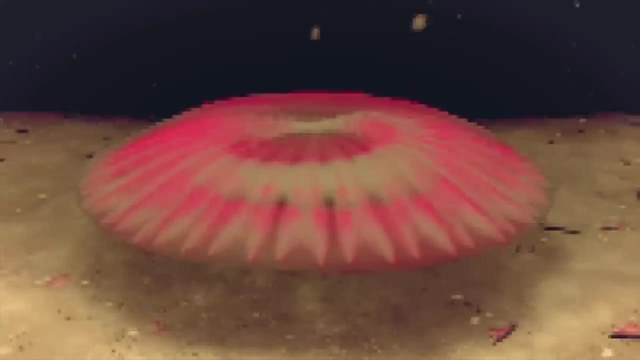 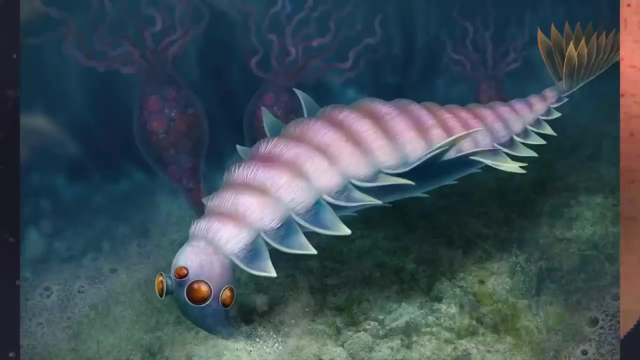 to avoid detection by predators, That being digging into the sand. But if there was a food source to exploit, you could bet that this group was ready to go for it. This is believed to have been the reason for Opabinia's weaponized proboscis. 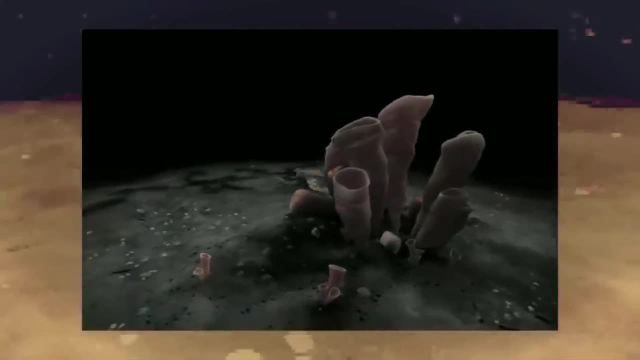 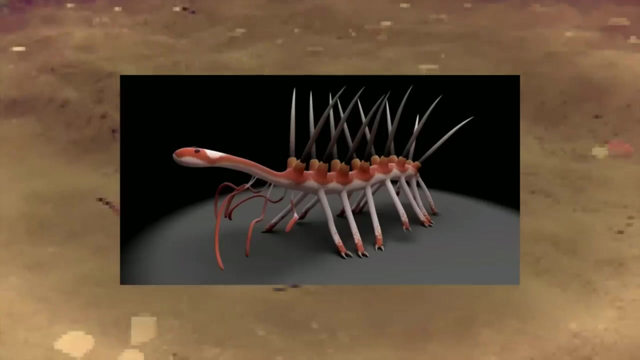 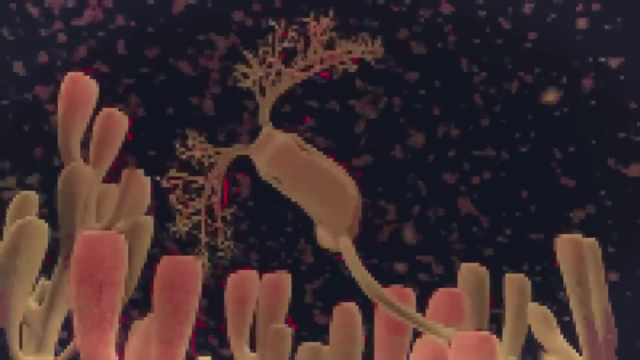 Swimming along the seafloor searching for signs of worms and things and then snatching them before they could escape. It's actually believed that predators like this were the main reason why Hallucigenia evolved the way that it did And the trilobites, mollusks, cranoids and sponges continued to expand, filling the warm seafloor with life. 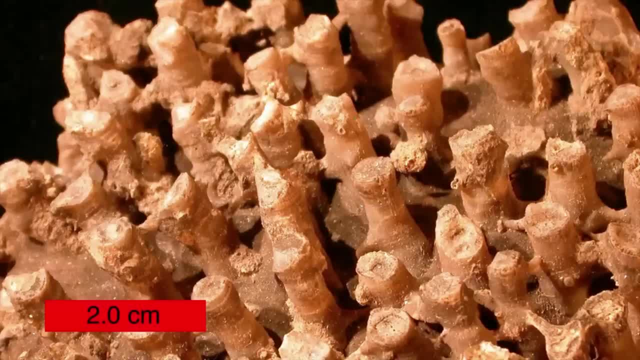 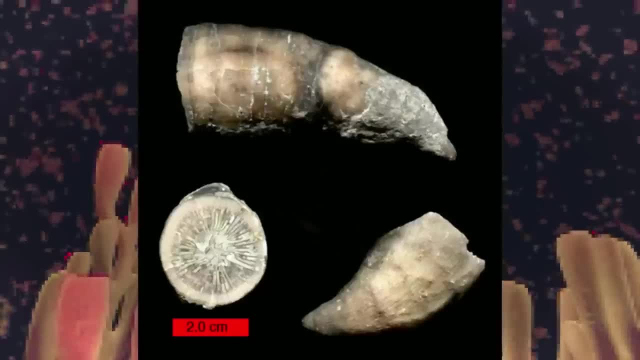 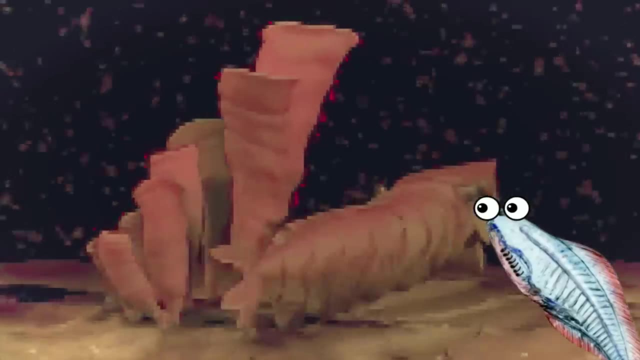 It was actually around this time that the first corals evolved as well. Although we don't think that they were nearly as widespread as they would be in later periods, we've still found evidence that they can trace their beginnings to this time. So what we are seeing now is a true complete biosphere form, with just one piece missing. The true apex predator And now leave it to the arthropods, because they were going to take a form that would change the game for everything living in the Cambrian oceans. And they did this by getting big, Like really big, by Cambrian animal standards. 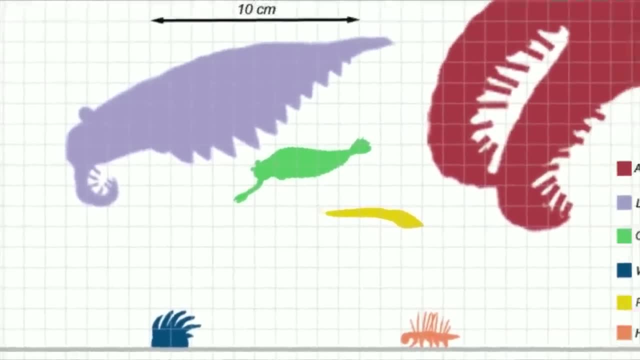 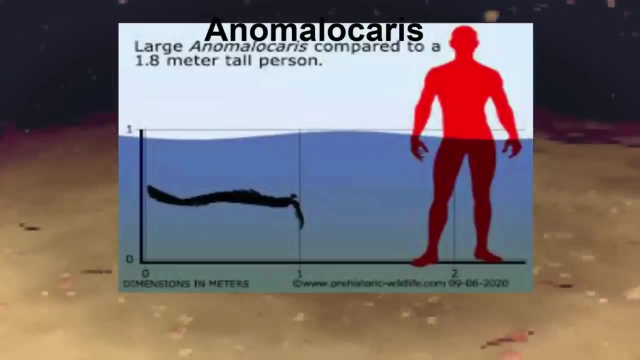 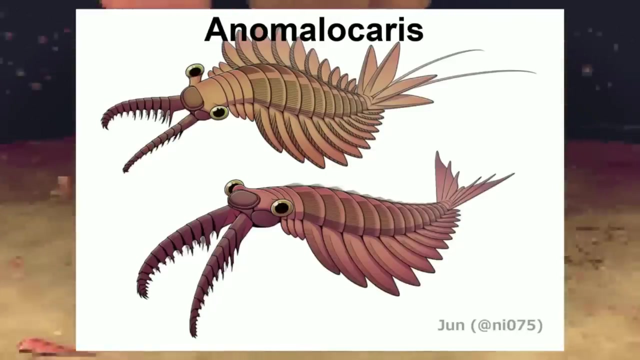 Up until now, everything that we've talked about was tiny, But by comparison, the massive Anomalocaris was a monster. It measured about a meter or three feet long and was undoubtedly filling the top predator role by taking a lot of the adaptations we've seen in earlier Radiodots. 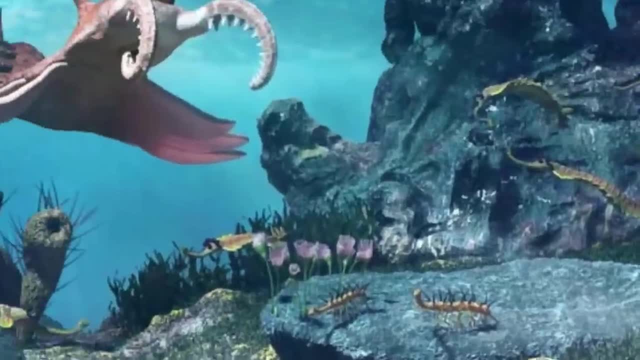 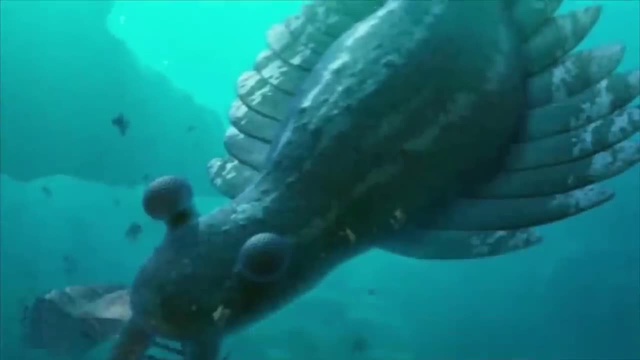 and fine-tuning them for the purposes of capturing and dispatching any prey it wanted, And it seems to have definitely worked. This animal is believed to have hunted and killed anything that its compound eyes could detect, And it probably had the keenest vision of any animal at this time. 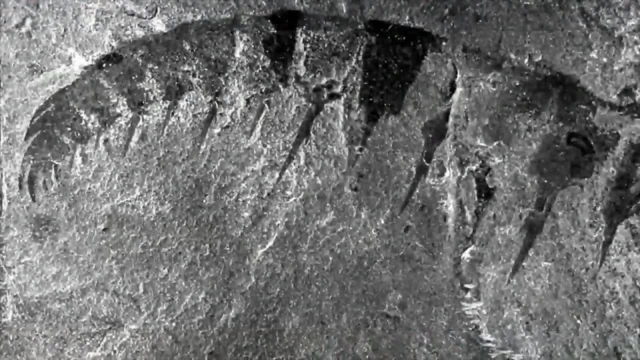 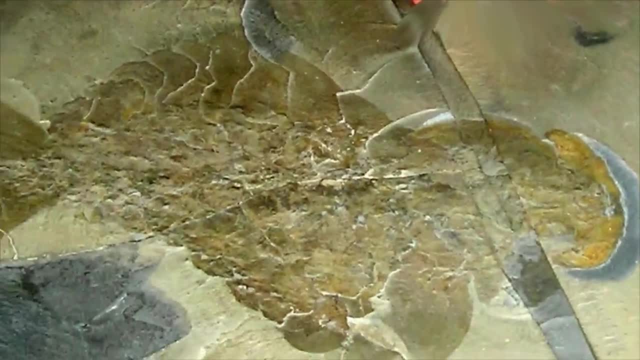 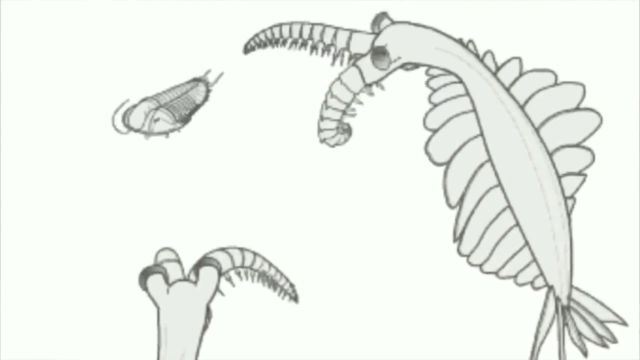 The long spiked appendages on its face were its main weapon as well as its way for manipulating its surroundings. The name Anomalocaris literally means strange shrimp, And it's actually one of the most well-known creatures. from this time It's kind of become right up there with the trilobite as the poster children of the Cambrian explosion. 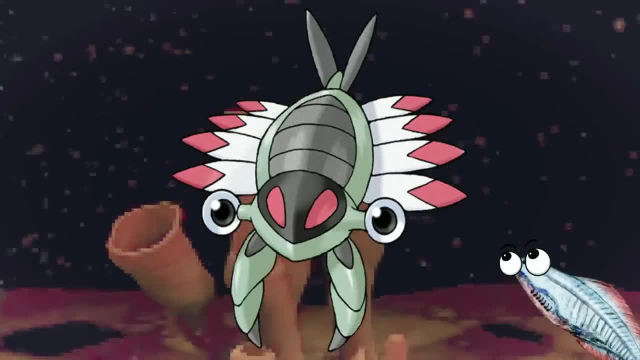 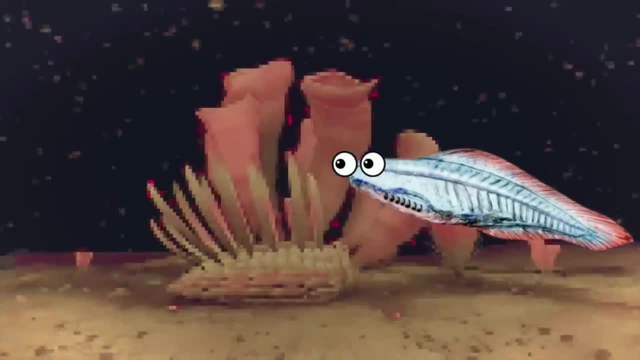 I guess having a Pokémon made in your image can even bring a half-billion-year-old giant shrimp monster into the limelight. And while all these new forms of invertebrate were evolving, we chordates weren't remaining stagnant either. We did, however, remain fairly small. With the arthropods and other weird creatures filling most of the macro roles in the shallow seas. it was probably a bit of a survival strategy. honestly, Remaining smaller meant that we could remain faster and more maneuverable to avoid monsters like Anomalocaris. 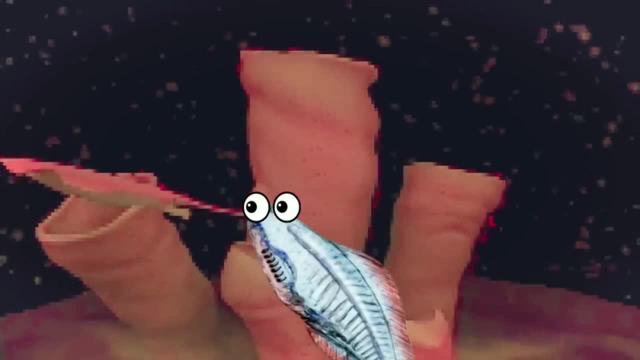 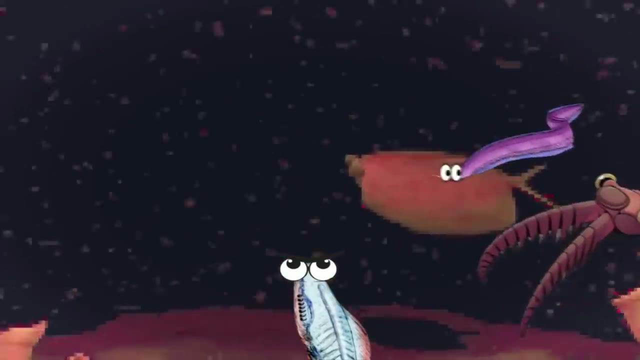 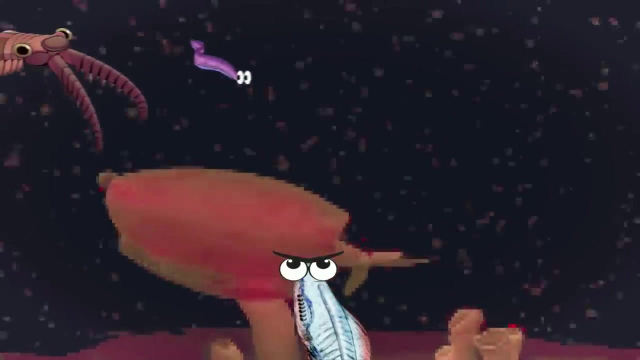 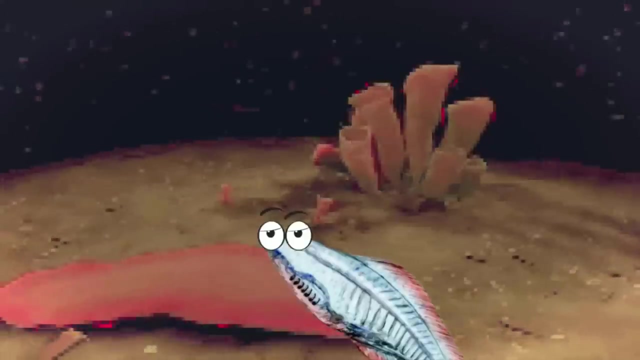 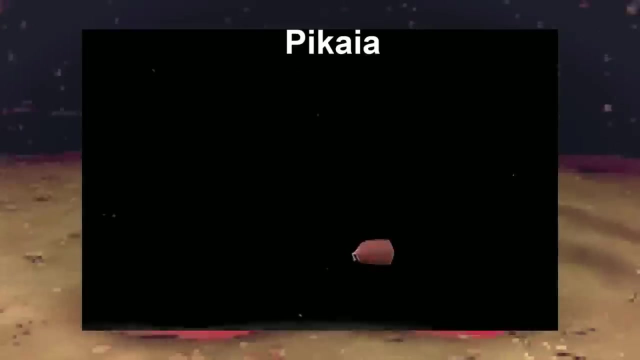 In the later Cambrian we would see another widespread chordate appear on the scene. Oh Tim-Tim, Good You survived. Tim-Tim is now a bit of a mystery creature called a pikaia. Although being pretty basal, it's believed that pikaia has most of the general characteristics of a basal chordate. 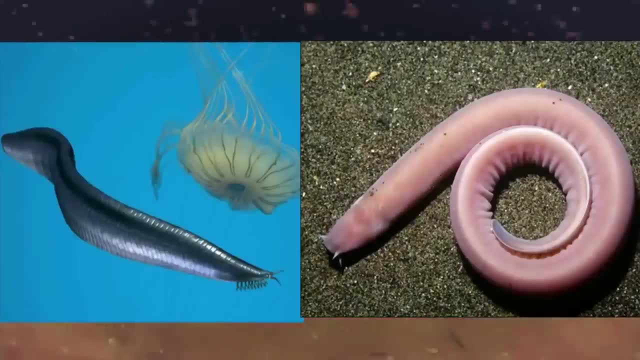 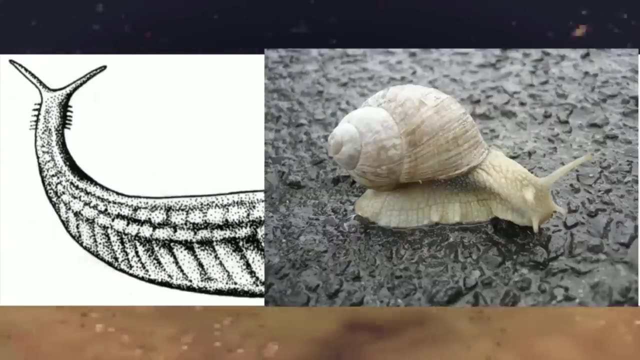 looking a little like a tiny hagfish or lamprey, with a flattened body and a distinct head. on the front end It also had a pair of antennae-like tentacles that made it look more like some sort of gastropod than any vertebrate we know of today. 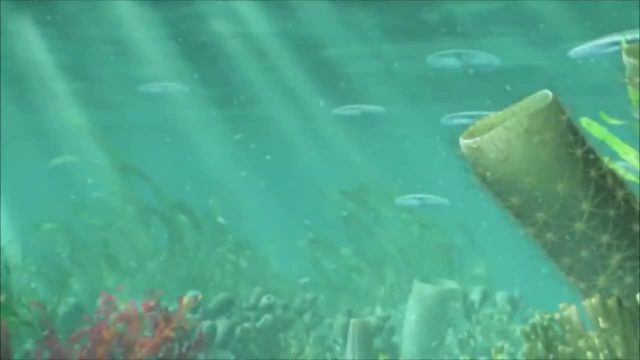 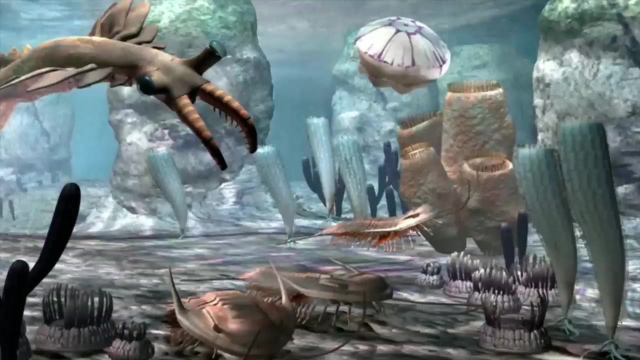 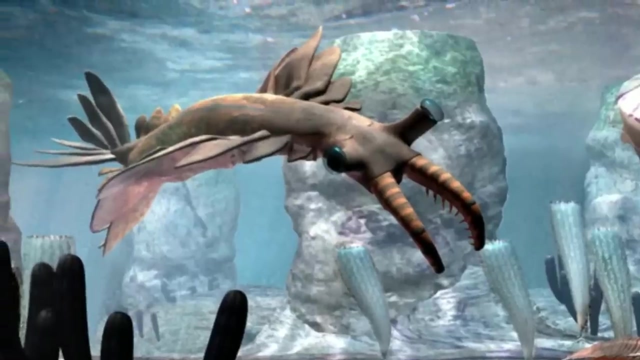 So who knows? really, The Cambrian is talked about as being the focal point of the evolution of life on this planet, And it really is. Every single group that exists today sees the beginnings of some direct origins in the bizarre alien creatures that existed here. 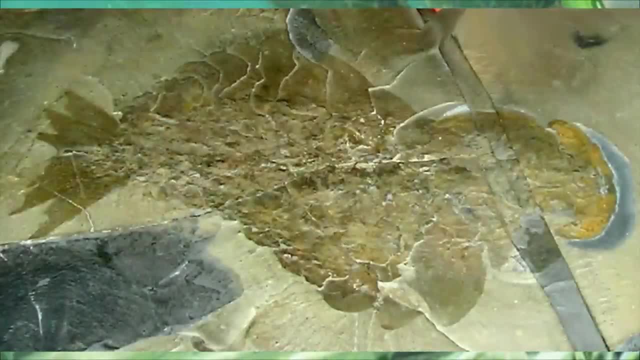 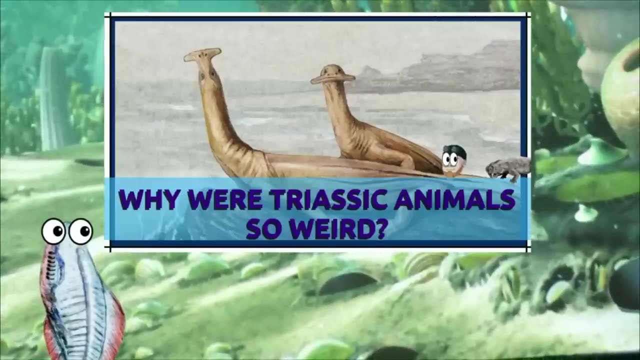 But there are countless others that for one reason or another, didn't make it. And, as I said in my video about the Triassic weirdos, these things appear weird to us today because of our perception. So much about our world has changed between now and then. 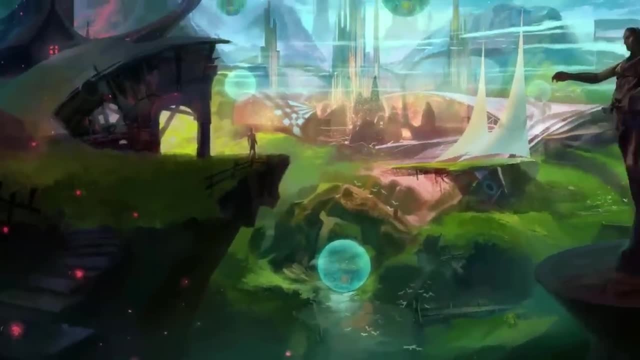 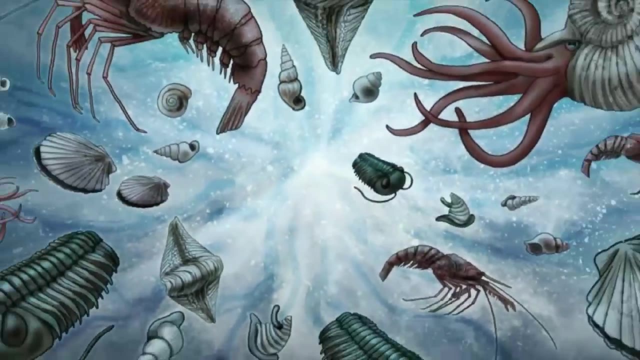 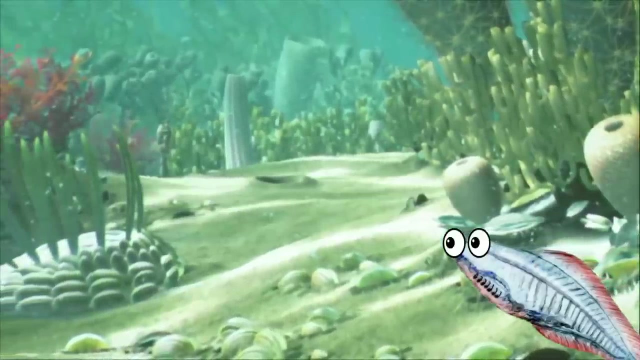 that if I told someone who didn't know any better that this was a concept for a sci-fi fantasy world, they would likely believe me. There are a ton of animals that I didn't get to discuss in this video And, as I said at the start, it would be impossible to give all these different groups their due credit. 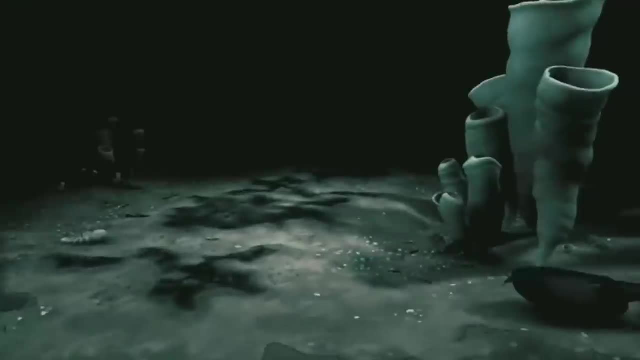 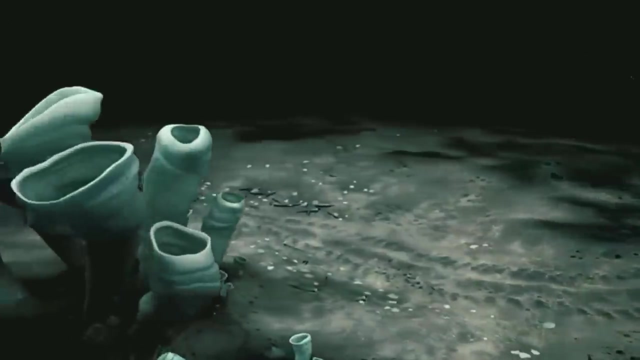 So I decided to talk about the most noteworthy ones that play the biggest part in future installments. But for many animals, their story ends here. This is because, as the Cambrian came to a close, the world would be wracked by a series of events that would cause several different drops in biodiversity. And there's a lot of theories and debates about what caused this. It could have been another round of glaciations, or fluctuation in oxygen yet again, Or it could have been a direct result to volcanic activity. It's really not known for sure. 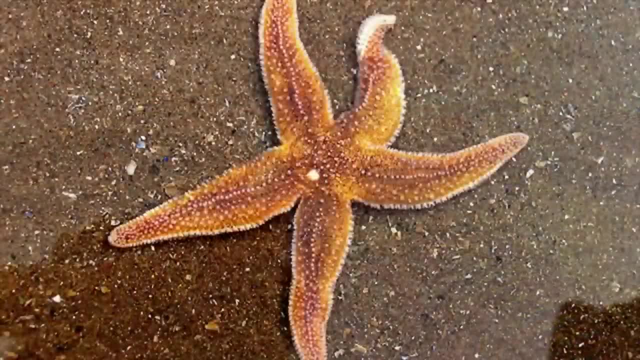 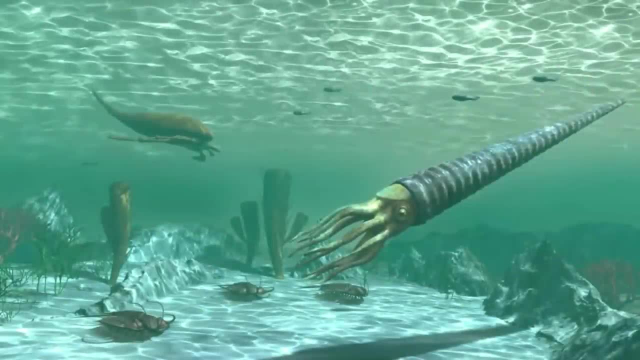 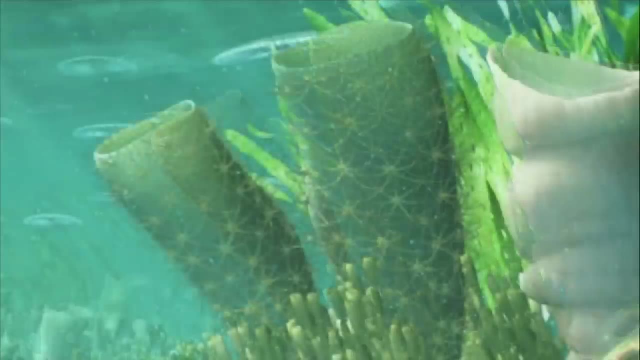 But for the animals that did survive, whatever took place at the end of the Cambrian, they would be setting the template for the remainder of the Paleozoic era. So let's talk about the Cambrian. Cambrian We left off 485 million years ago, with an extinction that brought the Cambrian to a close. 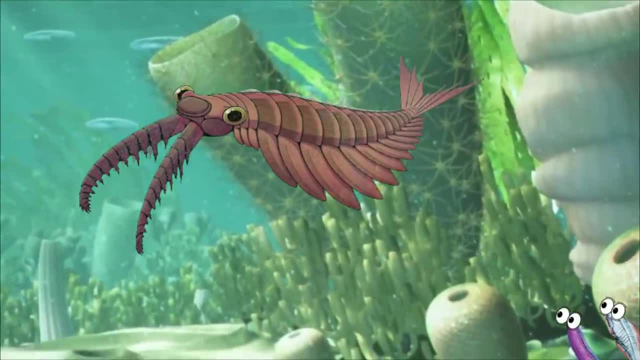 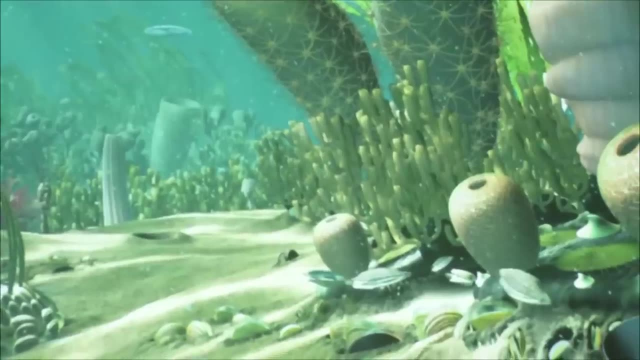 We lost a lot of the specialized Radiadon apex predators like Anomalocaris, But many groups, like the ever-enduring Trilobite, continued to press on And over the next 41 million years, life will flourish and the torch will be passed to new generations. 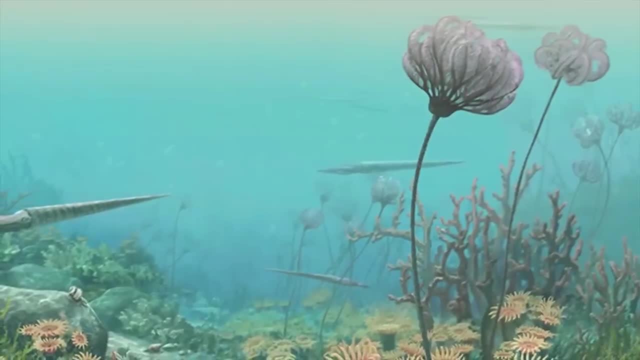 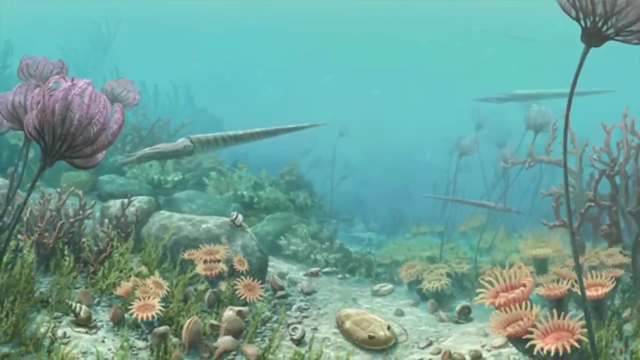 There will be new players on this stage of our planet as we get into the Ordovician period, And what better way to kick off this new period in Earth's history than with another round of adaptive radiation to fill the void left by all the species who died out at the end of the Cambrian. 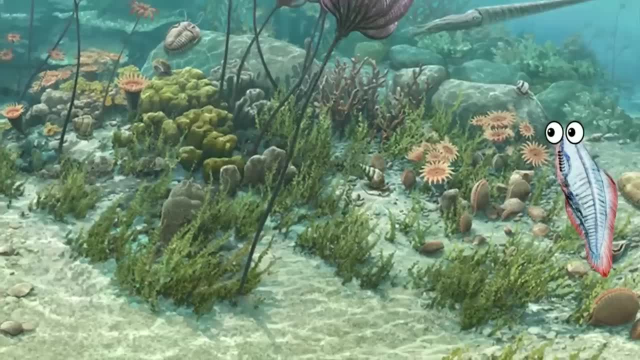 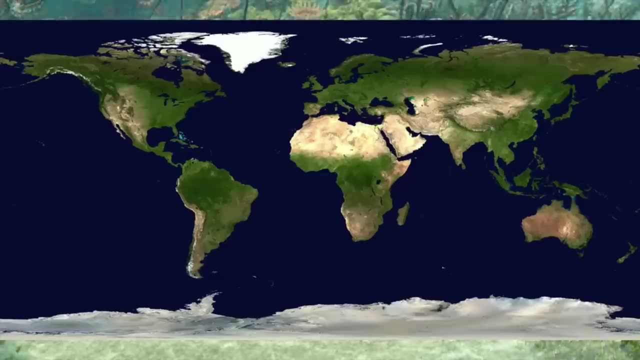 The interesting thing about looking at a map of what we think the continents looked like at this time is that it's literally the exact opposite of the world we know today. Today we see most of the joined land masses, primarily across the northern hemisphere. 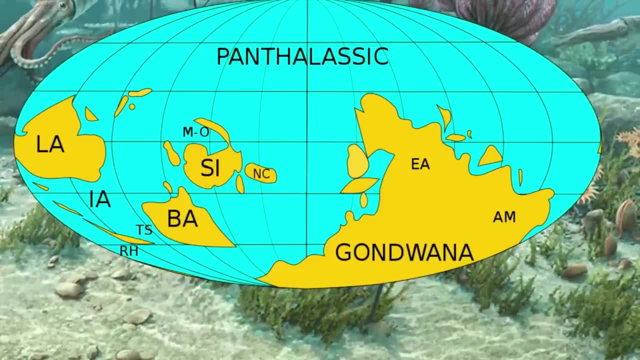 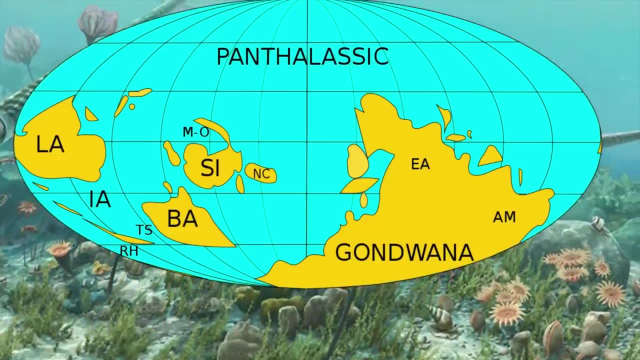 But during the Ordovician, the entire northern half of the planet was covered in a massive ocean called the Pantelassic Ocean. The southern hemisphere was dotted by islands and smaller continents and one massive land mass that extended from the south pole all the way to the equator. 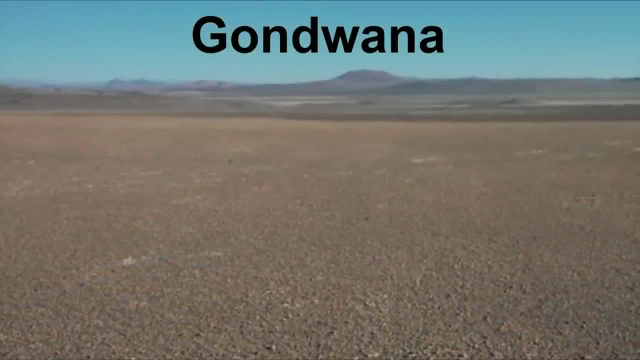 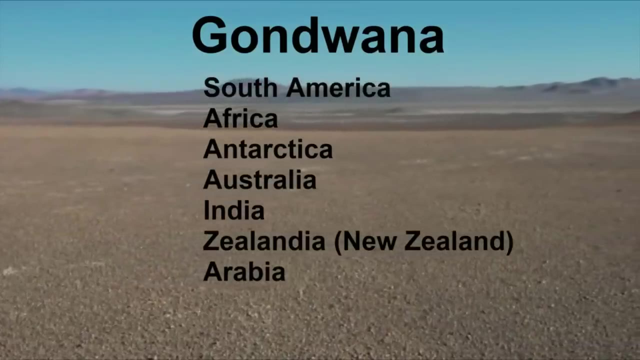 This supercontinent was called Gondwana, a massive slab of desert made up of what would eventually become South America, Africa, Antarctica, Australia, the Indian subcontinent, Zealandia and Arabia. These continents were as far as we could tell. 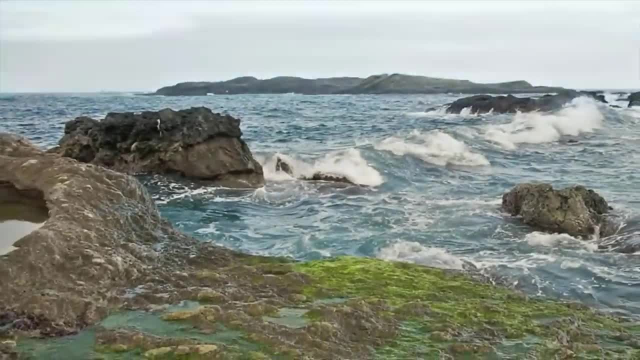 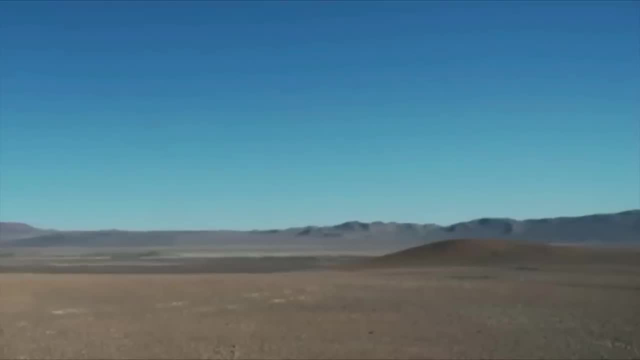 pretty much barren going into the Ordovician. There might have been colonies of cyanobacteria along the coast, but especially inland would have been entirely empty. But all that was about to change, because the very first forms of complex life were about to make the leap from the ocean onto dry land. 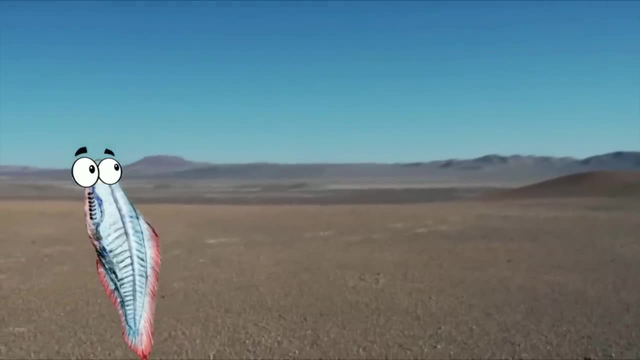 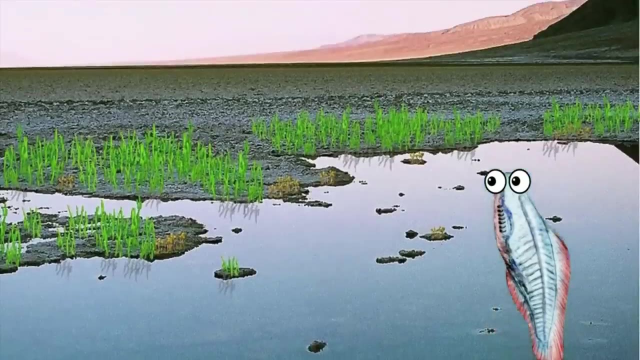 This might seem like a small change, but it is another major step in creating the world that we know today. It was around this time that the very first terrestrial plants evolved. Now we haven't checked back in with the plants since during the Proterozoic. 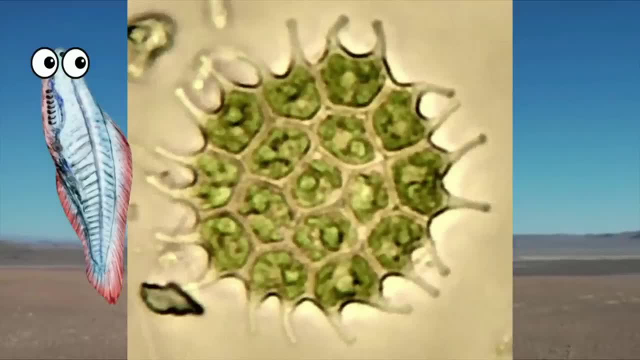 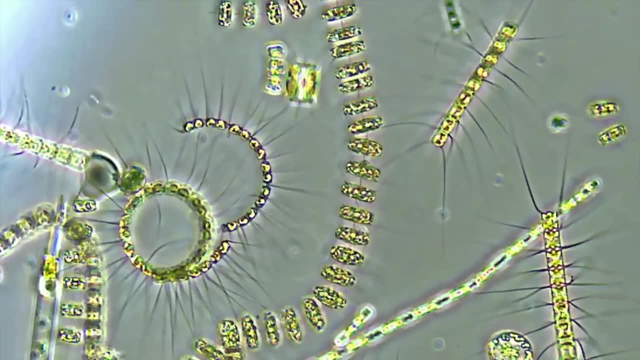 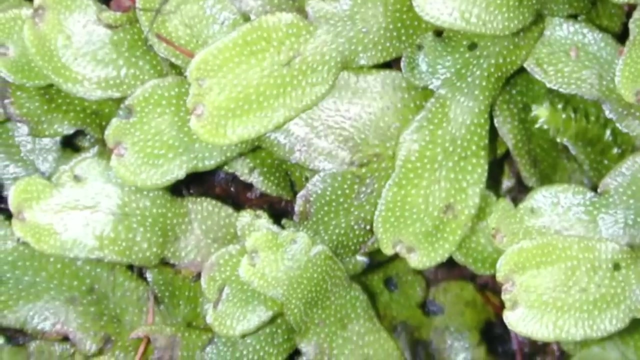 and that's because it seemed like they didn't really diversify much during the Cambrian, mostly staying microbial in the form of algae and surviving in the shadow of the cyanobacteria. But as they would start to move onto land, at first they would kind of resemble tiny non-vascular plants like liverworts. 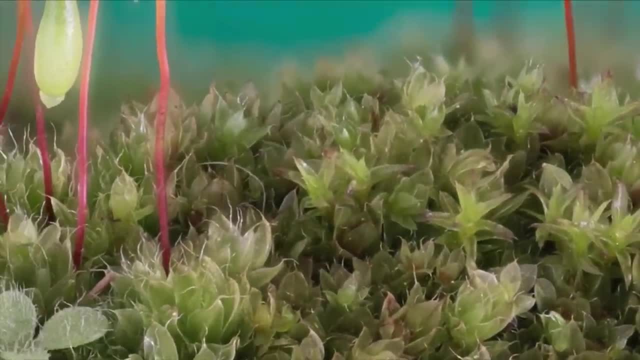 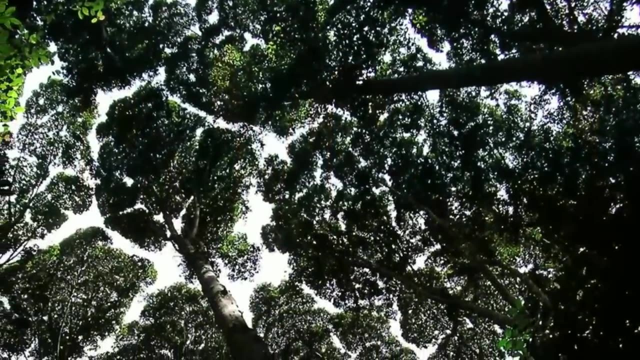 But as time went on and they adapted to life in the ocean, in the open air, they would evolve to be able to produce the very first spores. And it's from this very humble beginning that all complex plant life gets its start. And who knows if plants didn't make this journey first? 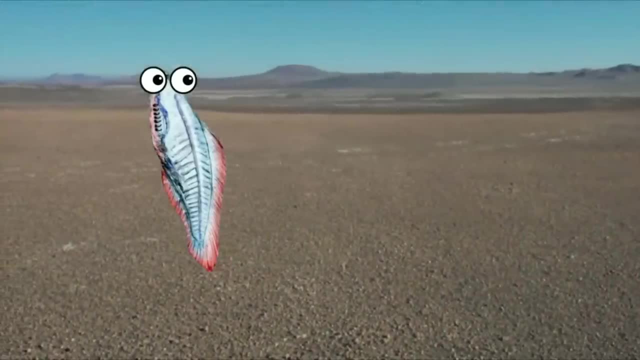 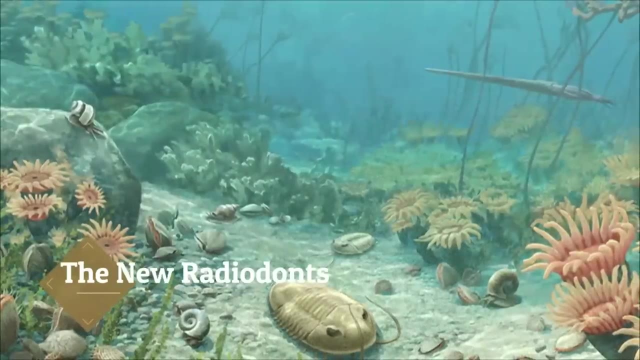 maybe animal life would have never crawled out of the sea in the first place, Because after all beforehand there really wasn't any reason to Over the course of the Ordovician, animal life started to bounce back from what happened at the end of the Cambrian. 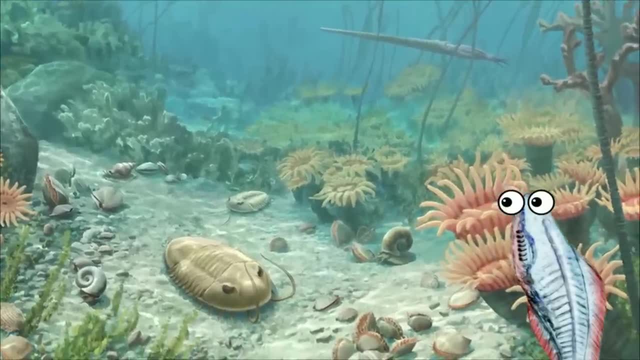 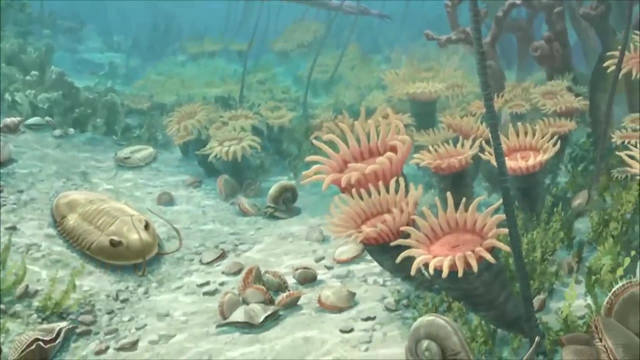 At some point, the diversity of life seemed to have been back on the upswing. Many of the bizarre life that had existed previously had faded into extinction, but several others did manage to hang on, And these were the ancestors of what was about to come next. 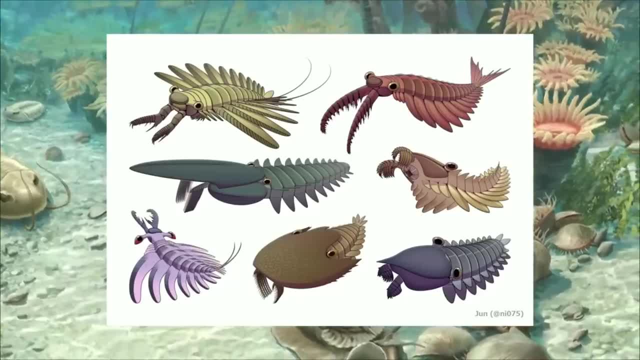 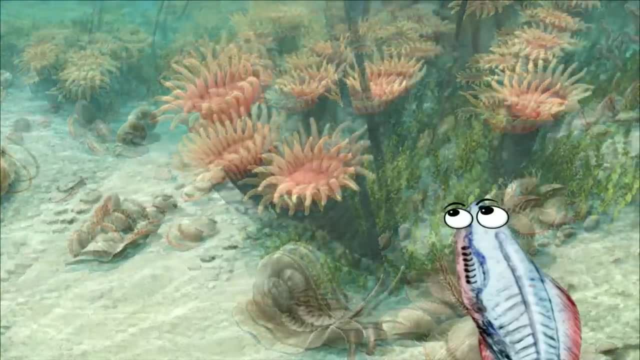 The Radiodonts will always be able to claim the title of the first super-predator, But by the Ordovician it seemed like those days were over. However, not all of them were completely wiped out. The ones that survived would be the ones that took on. 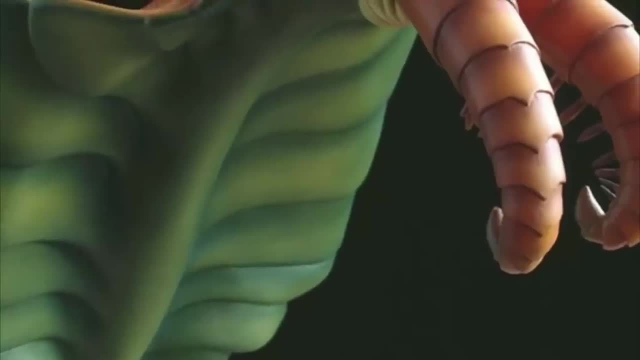 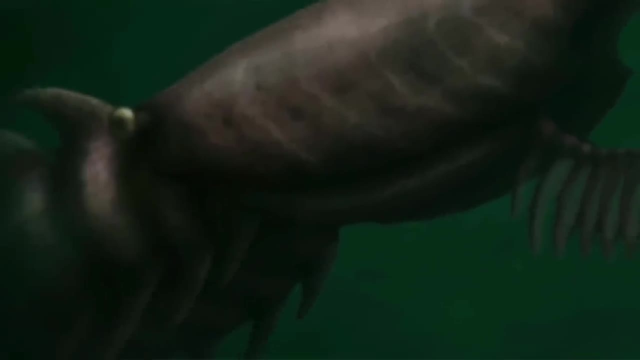 a bit of a different strategy to feeding than the hyper-carnivores we discussed in the last episode. They would become filter feeders and take advantage of the bounty of microscopic organisms that had been filling the ocean since all the way back in the Archean. 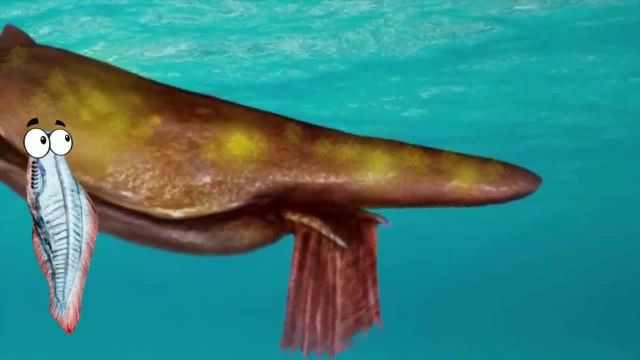 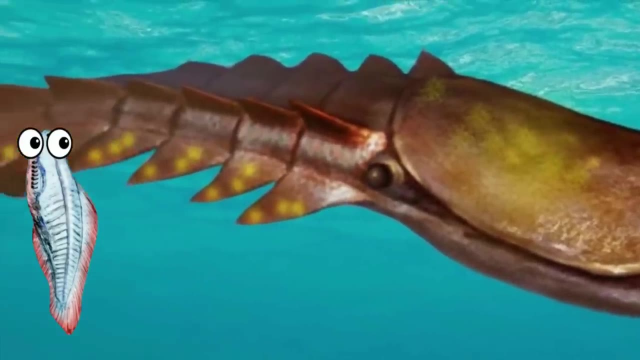 Maybe this became a more viable way to survive when many of the larger prey animals died out at the end of the Cambrian period, But this seems to have served them well because, as a result of this new lifestyle, the Radiodonts were one of the first large animal groups to recover. 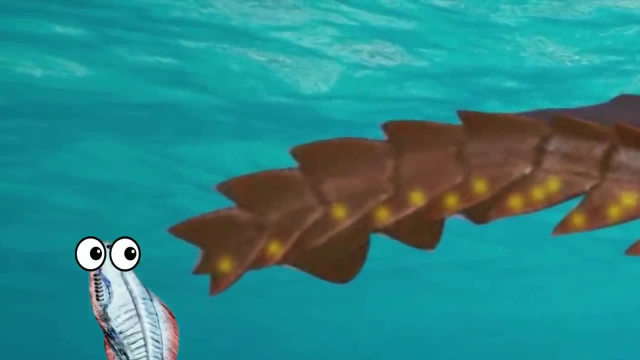 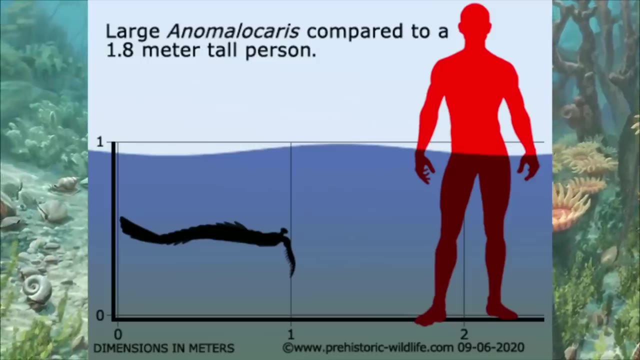 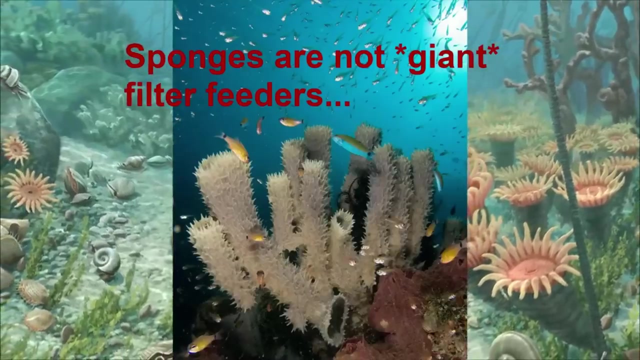 And beyond that, they actually got even bigger than they were before. Aegirocassus was among the largest, at two meters long and twice the size of Anomalocaris. This is the earliest known giant filter feeder, an evolutionary strategy that will be copied many times throughout Earth's history. including by the mammals, hundreds of millions of years later to create the largest member of that class of animals as well, By about 467 million years ago. the plant seemed to be back on track and was pretty well recovered from the Cambrian extinction. The trilobites were literally everywhere again. 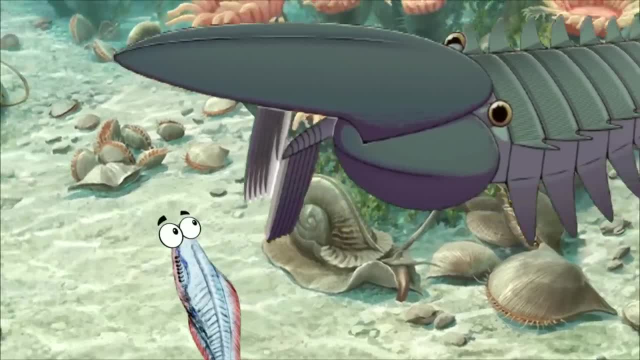 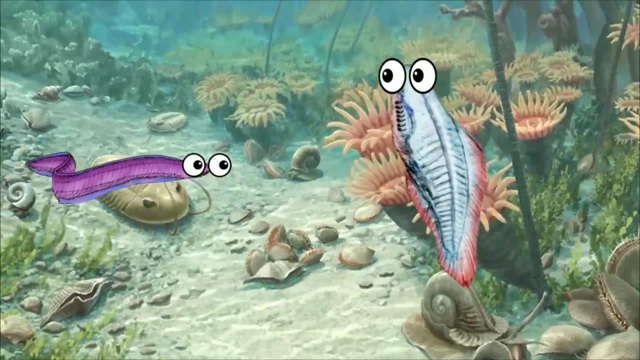 the Radiodonts had settled into their new role as gentle filter feeding crab monsters, and we vertebrates were hanging on, trying our best to get by in an arthropod world. Things were actually going pretty well, and it seems like things were only going to get better from here. 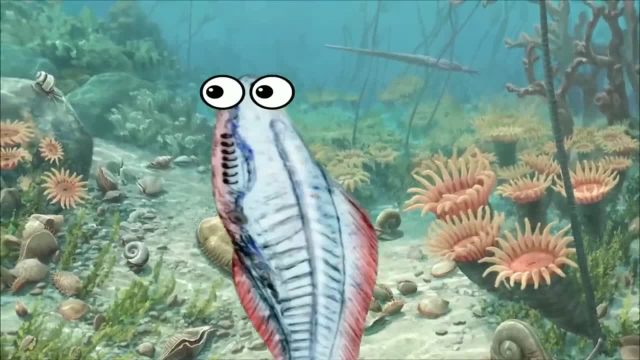 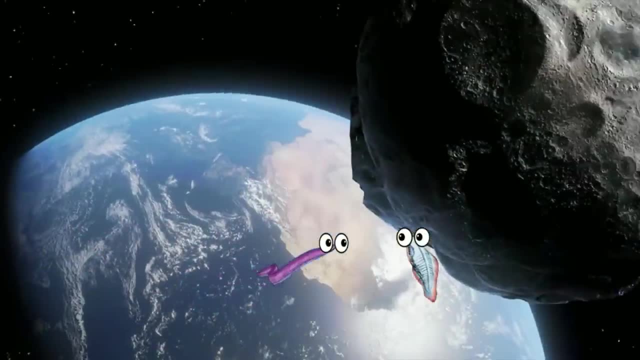 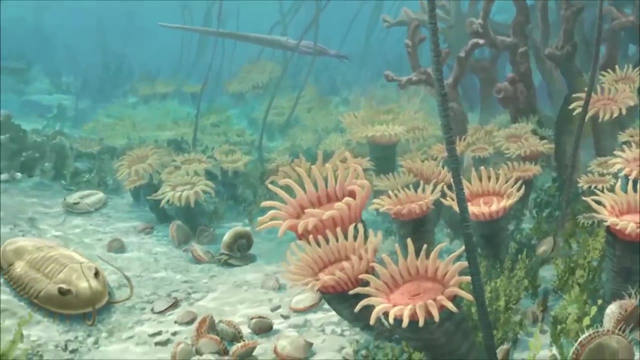 The oceans were once again flourishing with life. What, Tim Tim, What do you want? We have a situation. What situation? What situation? I was just saying how things were go- Oh Welp, so much for that. Things were going well until about the halfway point of the Ordovician. 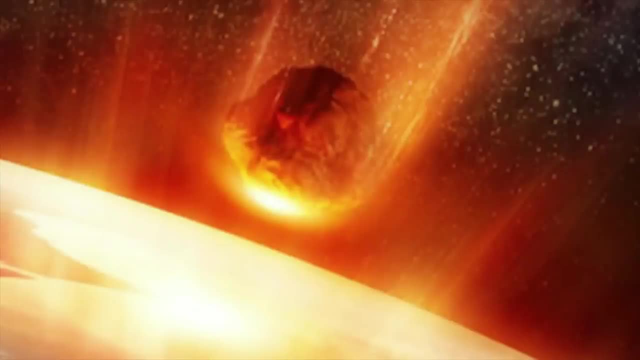 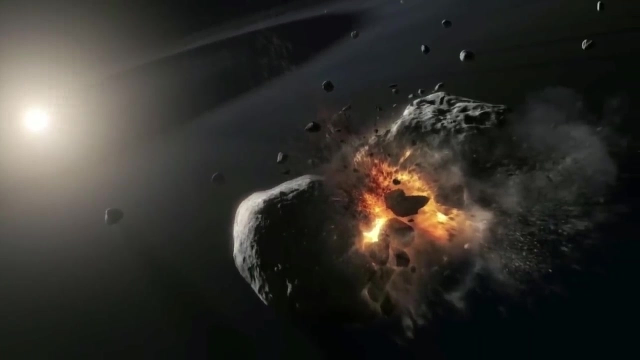 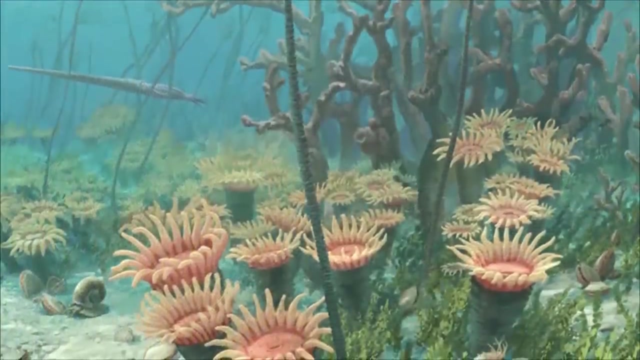 when there seems to have been a sudden, rapid increase in impacts from meteorites. This was a result of things continuing to break up in the inner solar system at this time, But what's really strange is, despite some estimates saying that the Earth was experiencing a hundred times as many impacts. 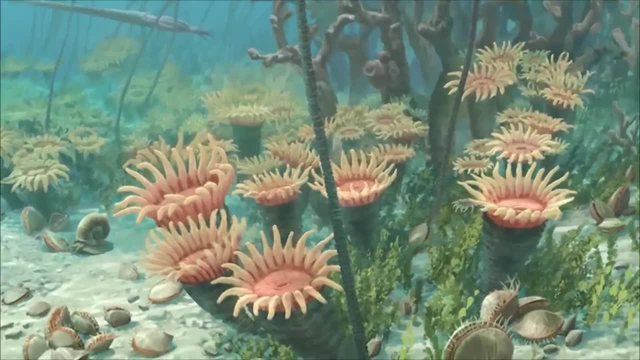 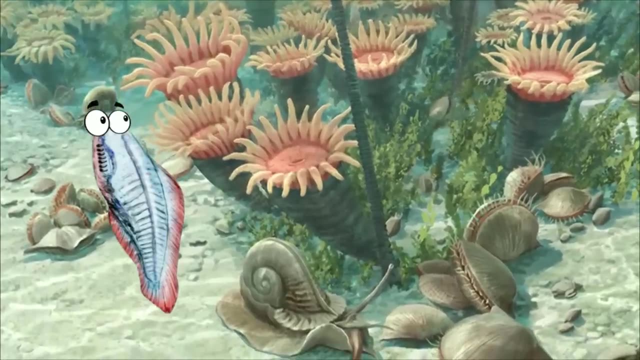 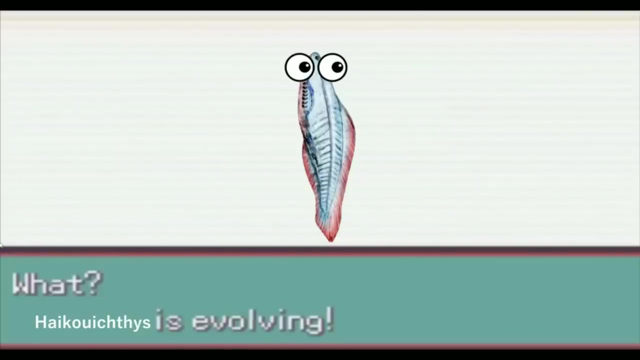 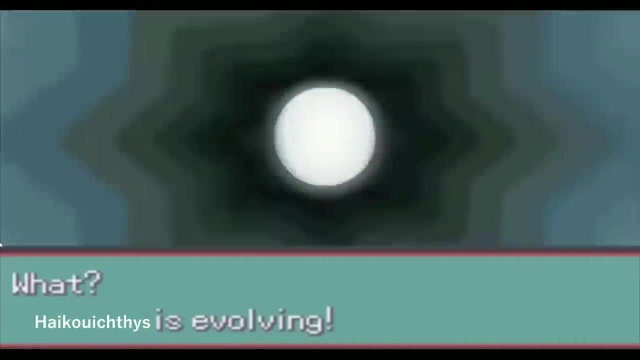 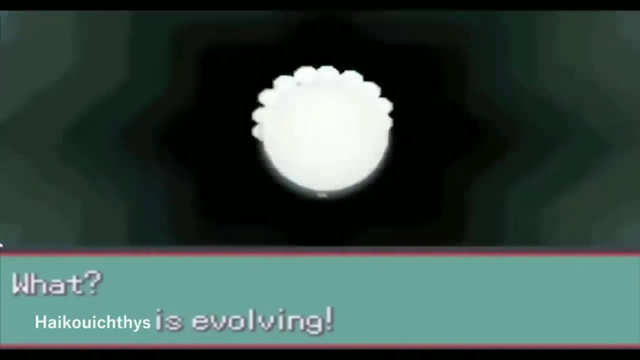 compared to what we have today. this doesn't seem directly connected to any mass extinctions. In fact, after this point, life just kept trucking along and became even more diverse. Wait, Woohoo, What now? All right then. 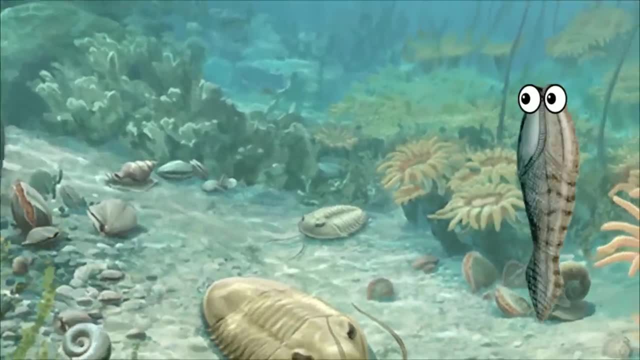 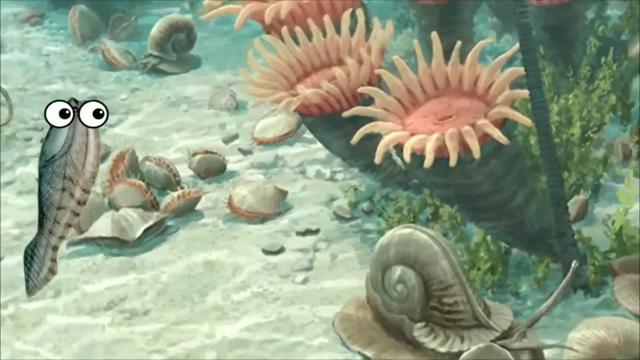 For millions of years. at this point there have been chordates, But we have lived in the shadow of the arthropod masters of the world. as well as other invertebrates And, for the most part, the very first chordates more resembled hagfish and lampreys. 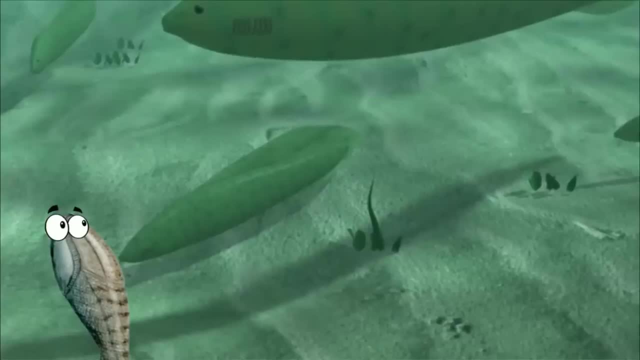 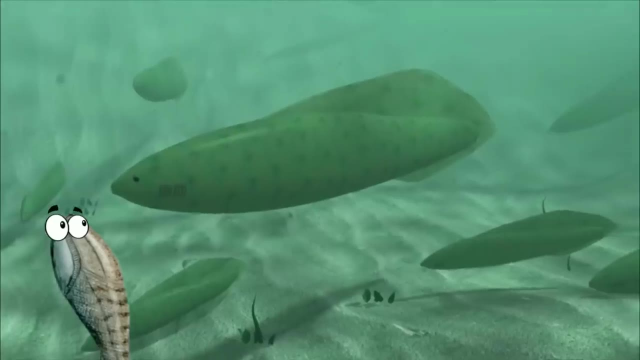 than any other true bony fish, And I use the term chordate rather than vertebrate because at that time our ancestors didn't even have a true backbone yet. But the next step in our evolution would take place here in the Ordovician. 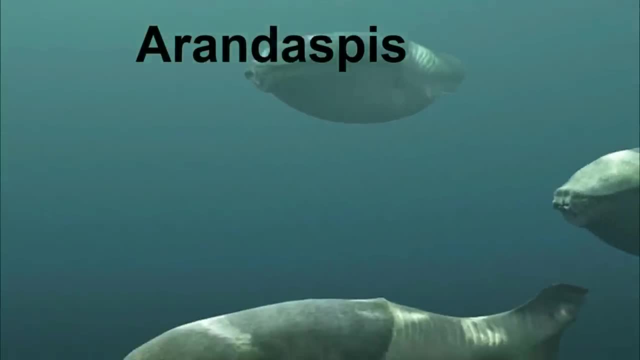 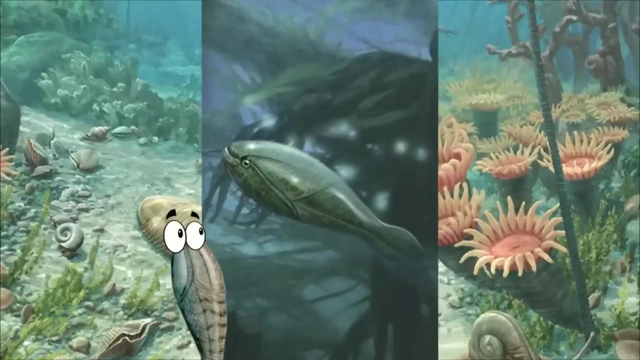 with the appearance of my next form, our Andaspis. Now, even though I wouldn't say that we're exactly ready to take over the world yet, at just 15 centimeters or 6 inches long, in terms of our evolutionary history, these guys are a pretty big deal. 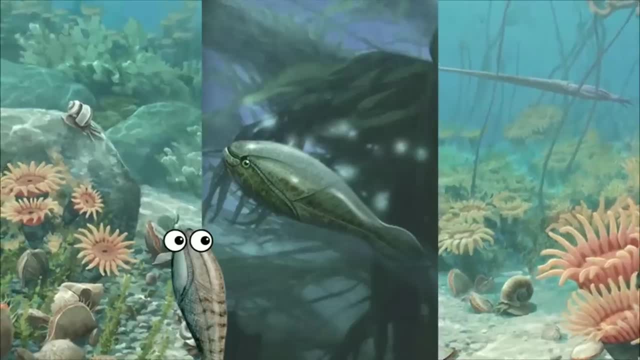 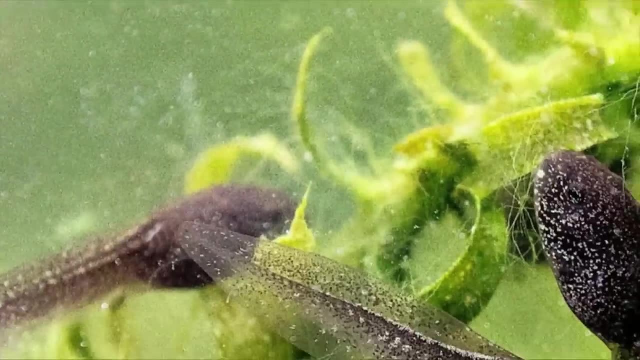 At this point, it's believed that Arendaspis was one of the first vertebrates, as well as one of the first true fish. Even though it didn't have any jaw or fins yet, it was probably able to get around using its tail, similarly to a modern tadpole. 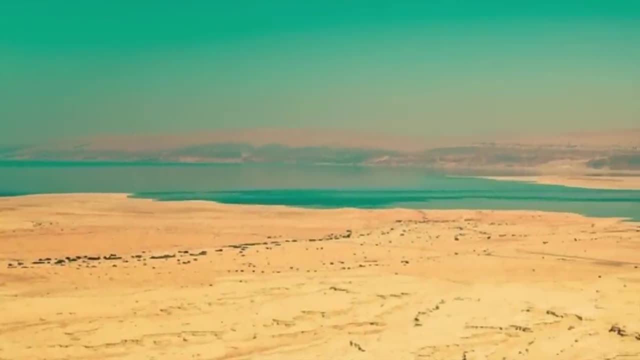 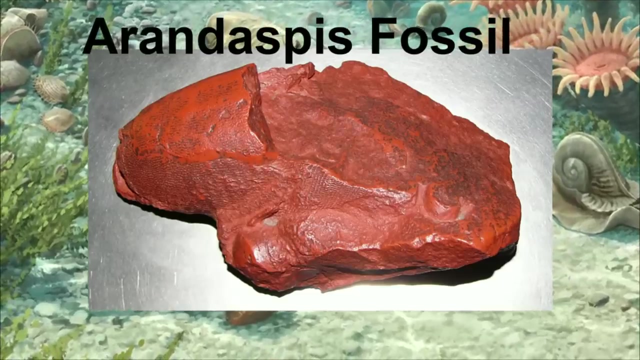 It was probably a filter feeder. They stuck to the shallow water coastlines of Gondwana and pretty much left the open oceans to the arthropods. And to help with protecting themselves from any possible confrontations that they might have, these early fish would develop protective armor on their heads. 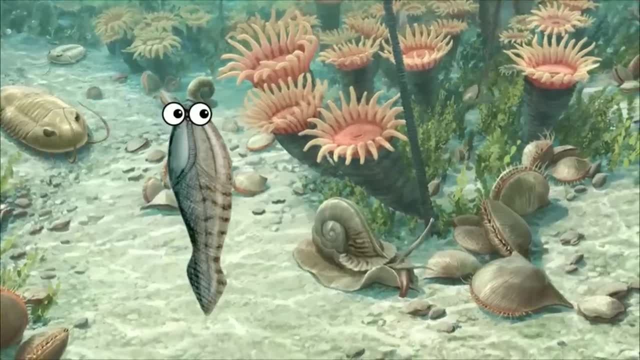 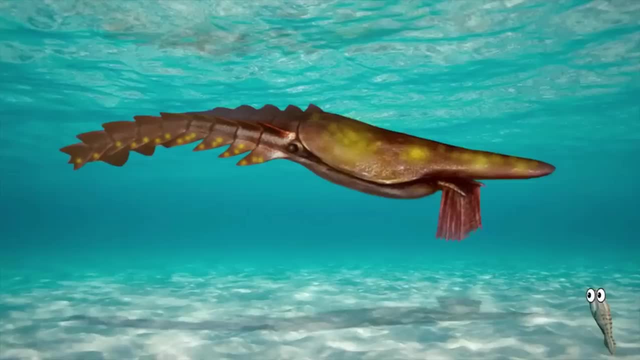 in the front of their bodies, A feature that might seem strange compared to fish today, but it would prove a trait that would one day give our ancestors a fighting chance in the race for life. And despite still being at something of a disadvantage, the first fish were obviously doing something right. 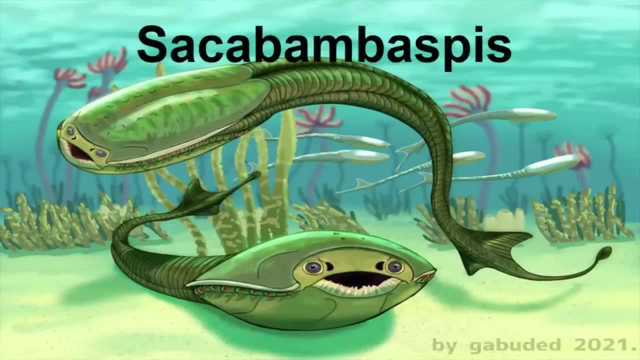 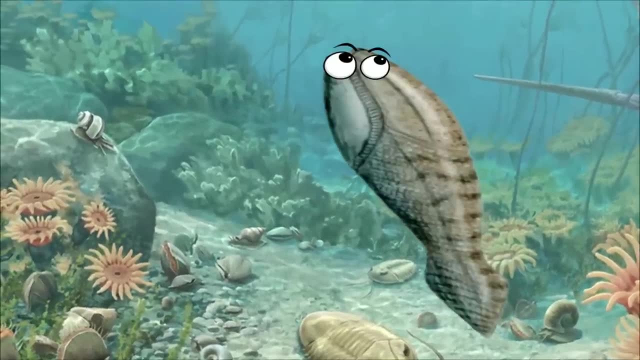 since they even started to diversify into other species like Saccabambaspis. Oh Hey, Tim Tim, How we doing? I think things are going pretty well. We're better protected than we've ever been, and the only radiodonts that are left are basically filter feeding crab whales. 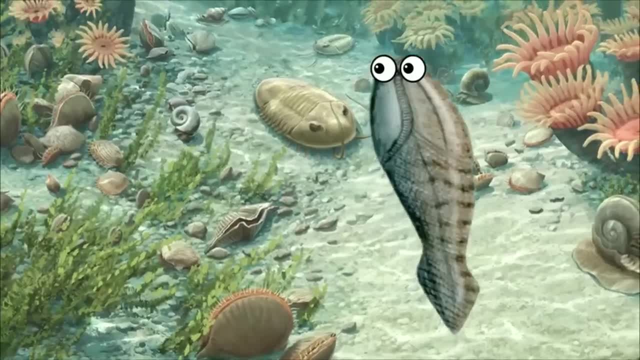 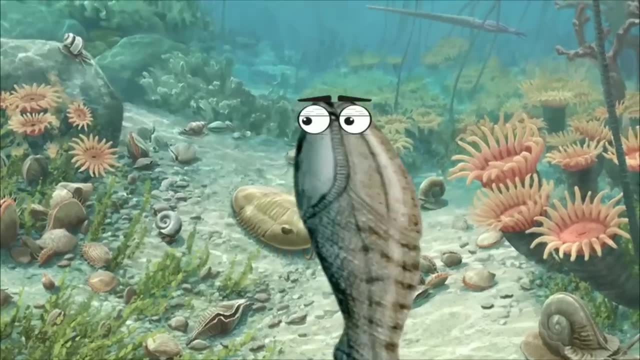 I feel like we might be forgetting something. What do you mean? Well, if the radiodonts are no longer a threat, something else has to be driving our evolution into these more defensive forms. I hate when you're right: Release the carrot krakens. 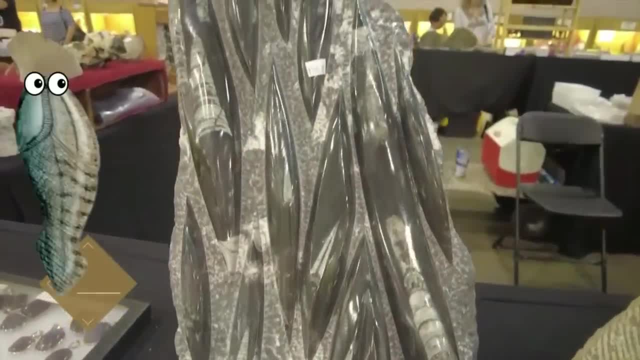 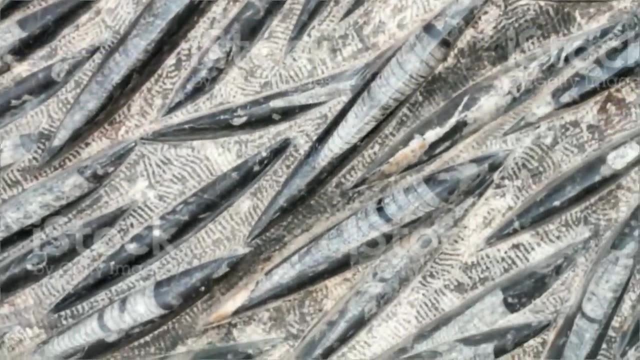 Have you ever seen fossils that look like this? Normally clusters of multiple cone-shaped cylinders that polish up really nice. They're one of the most common fossils that are collected, besides ammonites and trilobites, But a lot of people collect these without ever realizing what an important piece of the past they have. 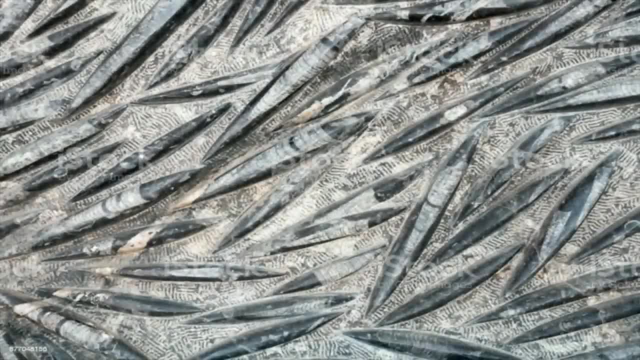 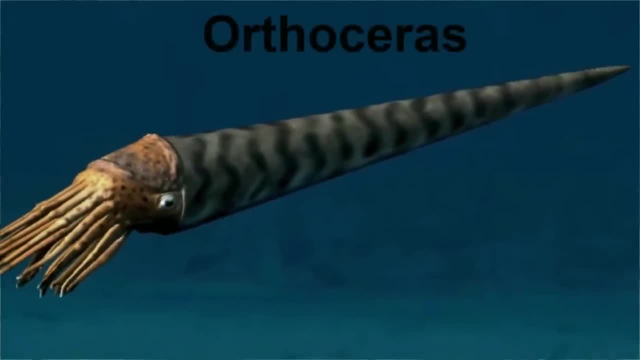 These are the remains of the shells from one of the most prolific predators the world has seen up until this point: an actively mobile carnivorous cephalopod called Orthoceras. Now we talked briefly about how cephalopods may have gotten their start all the way back in the Ediacaran. 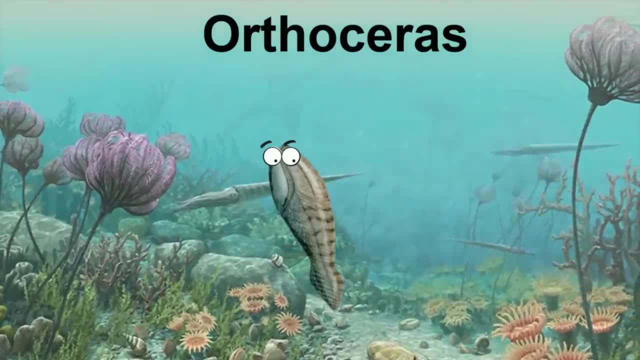 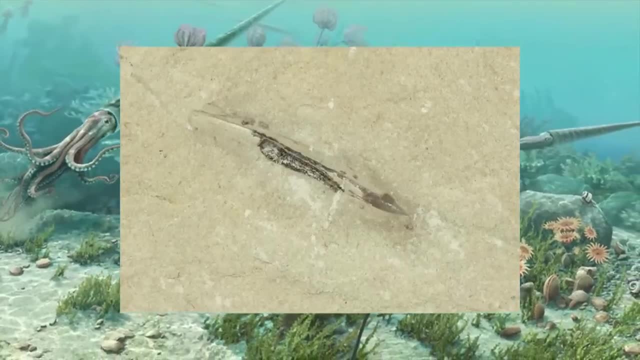 but it was kind of hard to say for sure, because most cephalopods don't fossilize very well, You know, since they don't have any bones. So there are a few trace imprint fossils that we think might be early members of this group. 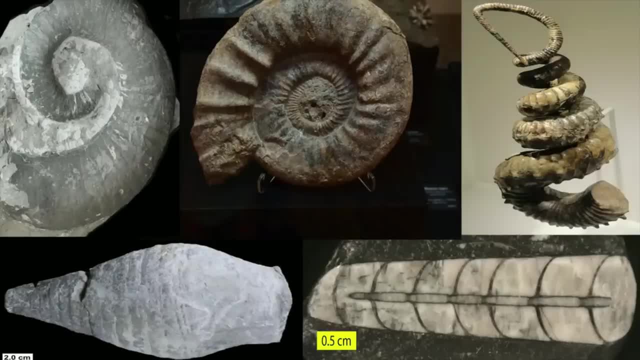 but we really can't say for sure. That would all change with the evolution of the subclass Nautiloidea, the group of cephalopods that have a hard shell, and includes everything from these guys to ammonites, all the way up to modern nautiluses today. 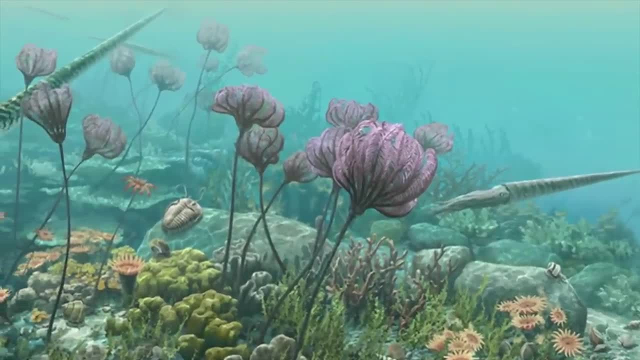 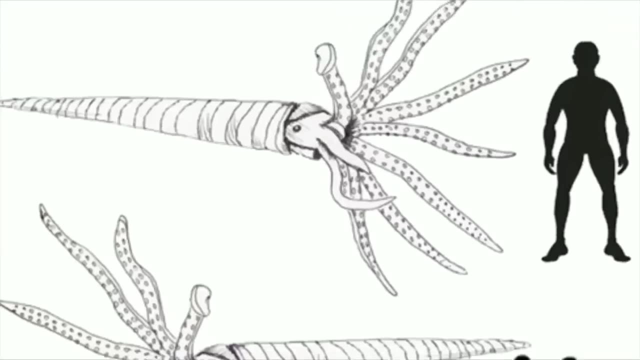 Orthoceras is actually a broad term that refers to several different species ranging in size from little guys the size of your finger all the way up to the 4.5-meter or 15-foot sea monster. that seemed like something from an old fisherman's tale. 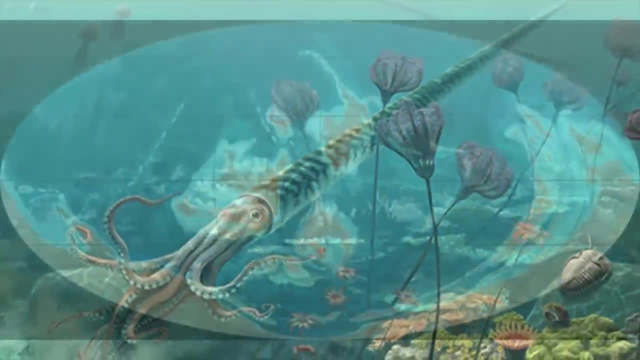 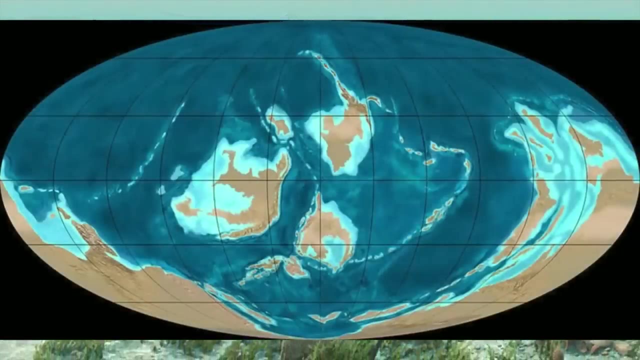 These guys were the rulers of the open ocean, taking over the position of apex predator in every corner of the globe. Their fossils have been found everywhere that there are marine deposits from this time period. And then on the ocean floor there was another new group of predators. 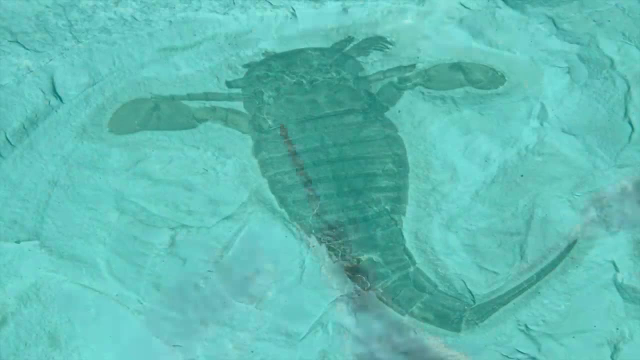 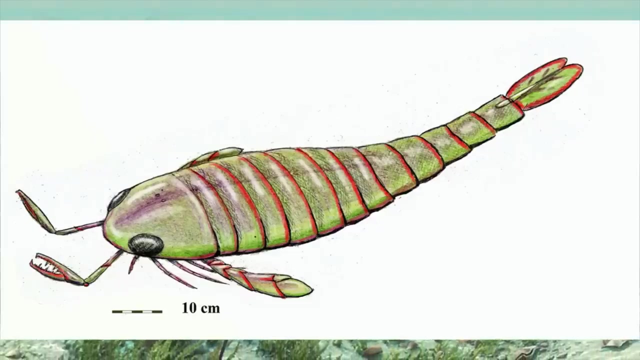 the very first Eurypterids, or sea scorpions. Despite the name, these marine arthropods are not true scorpions, But they're definitely closer to an arachnid than an insect in body plan, because their bodies have two segments: a head and an abdomen. 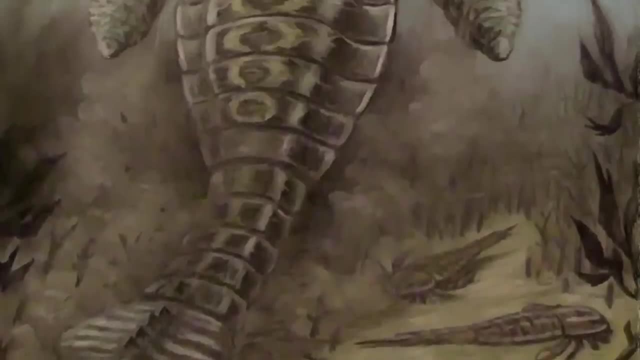 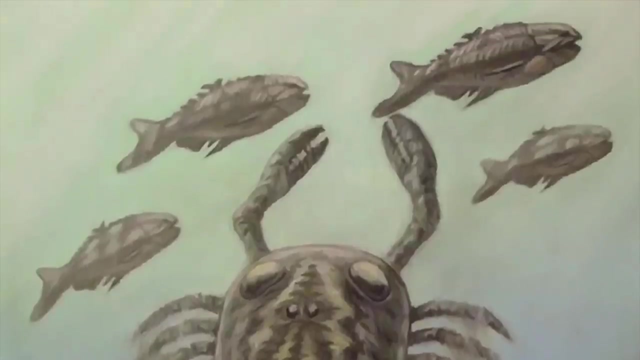 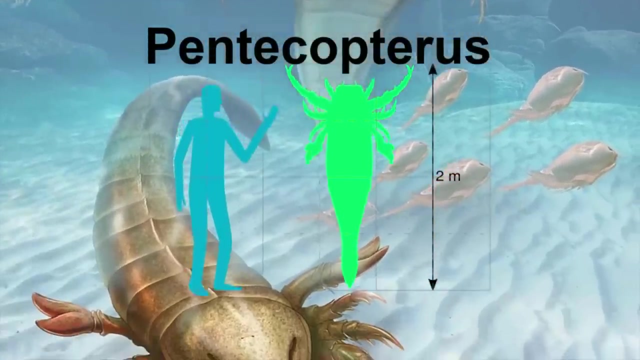 And I'll definitely be getting into them more as we go forward in time, But it's definitely worth mentioning that the earliest species of Eurypterid first appeared around the middle Ordovician 467 million years ago. Called Pentacopterus, it also was a considerable-sized carnivore. 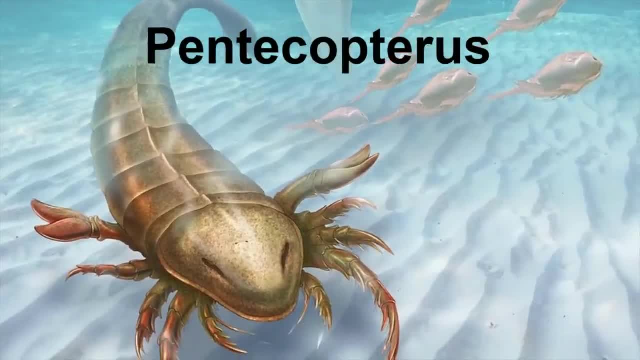 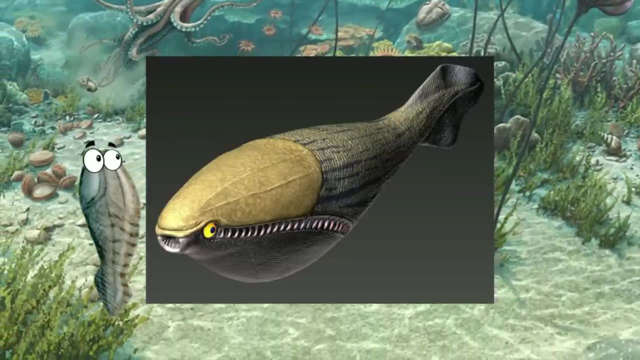 And it probably made the ocean floor every bit as dangerous as Orthoceras made the open ocean. And all these were probably the reasons why, even after evolving the defensive armor of our early ancestors, the first fish, were still confined to the shallow coasts. 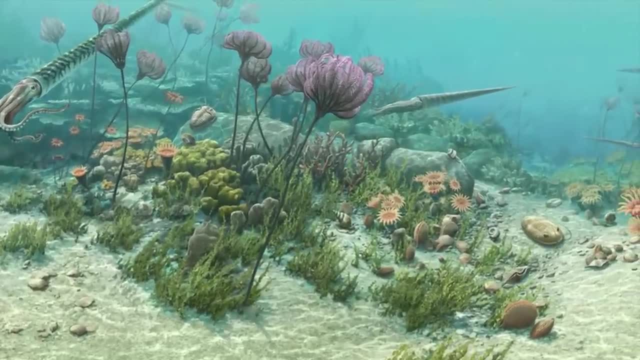 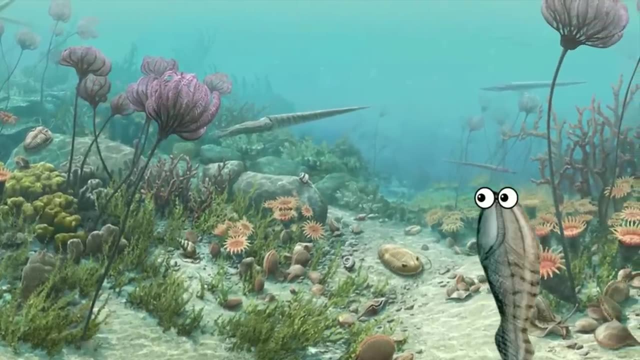 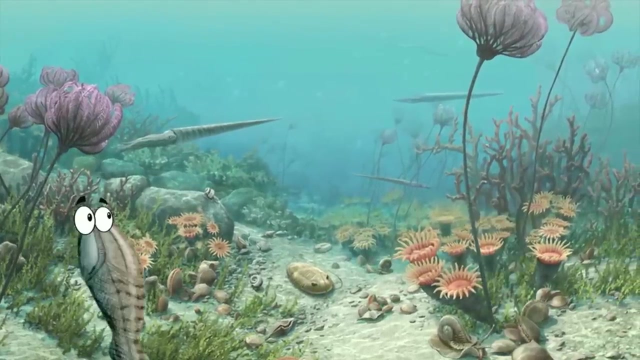 Most of the large animal roles were still being filled by invertebrates, leaving our ancestors confined to areas where we could better avoid them. However, as these giant cephalopods and arthropods became more and more specialized, it may have left them at something of a disadvantage for what happened next. 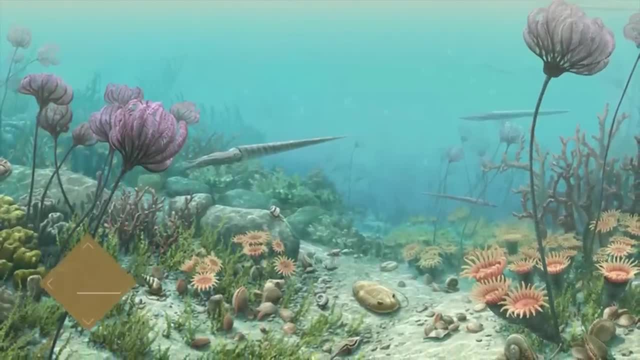 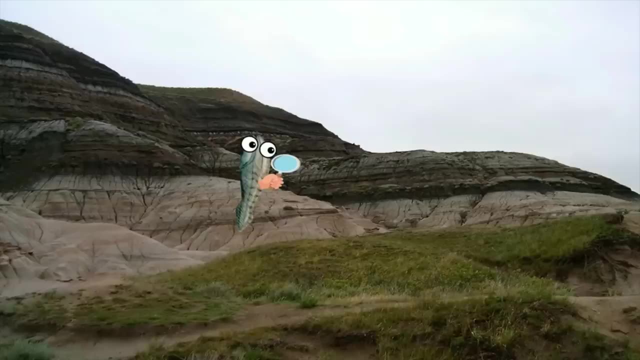 As we go forward in time, the periods of geological history are almost always concluded with a major drop or change in global biodiversity. It's the reason why scientists looking at the fossil record are able to say that this is a point in time when one geological period ends and another begins. 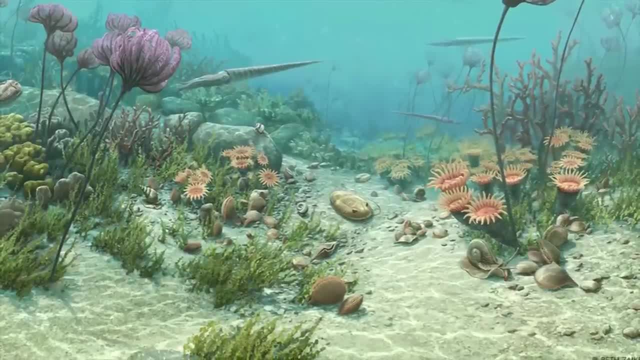 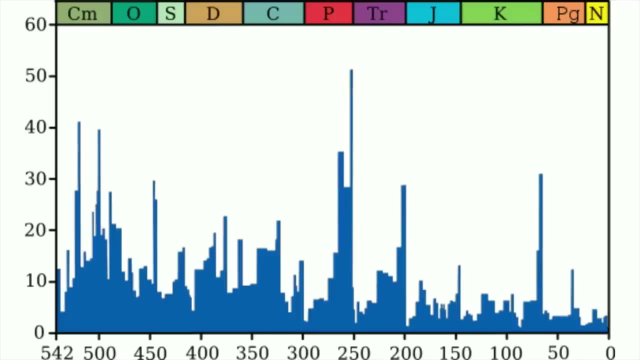 So this will become a reoccurring theme in the History of the Earth videos. That being said, however, there are only five events that have led to such a catastrophic loss of life that they are actually considered one of the true mass extinctions. 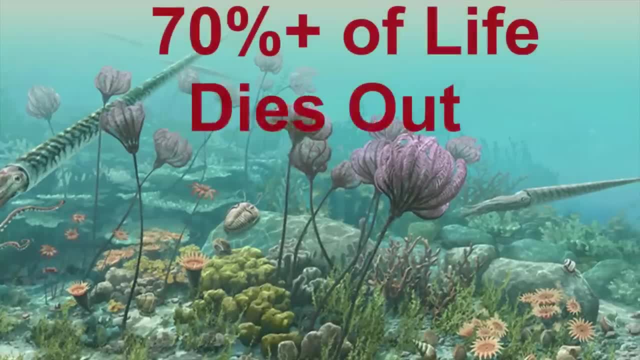 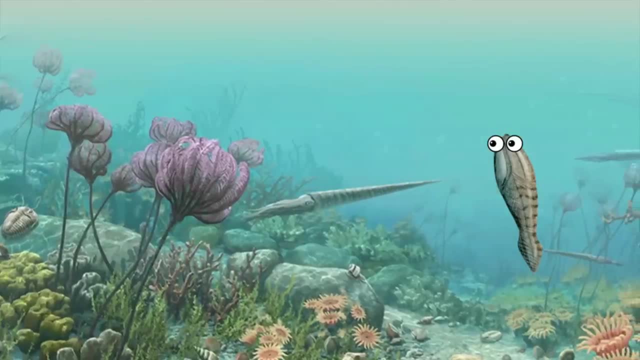 These are normally defined as an event where 70% or more of the species on Earth are wiped out. at that time, And as we get into the late Ordovician, from 445 to 440 million years ago, we come into the first of these great dyings. This happened over the course of 5 million years because of wild swings in the global climate. It started out with a glaciation that led to lower sea levels and cooler ocean temperatures. This likely destroyed the habitats that the early fish relied on for protection from the invertebrates. 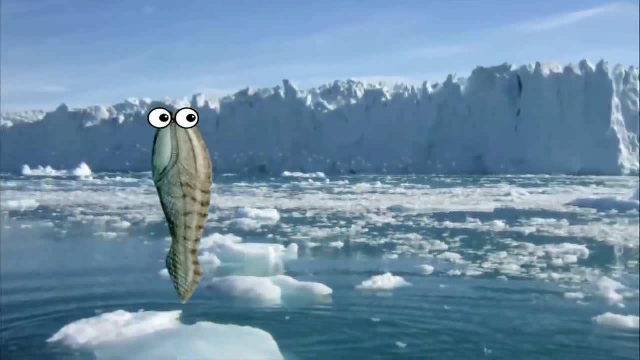 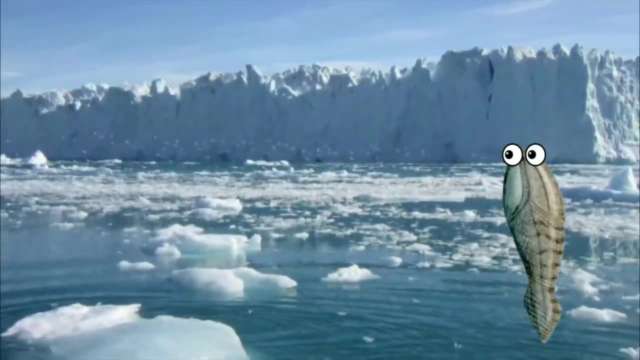 And had that been the end of it, life would have likely quickly recovered. But following the glaciation, the climate would do a complete 180 and switch from an ice house to a greenhouse, And this is when things would go to a critical point. 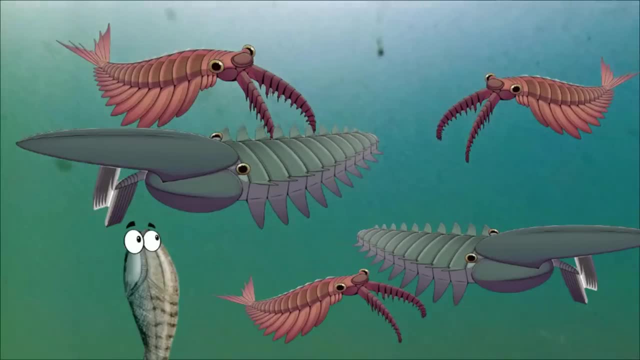 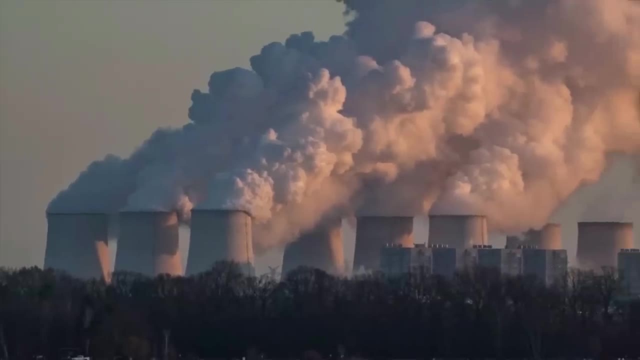 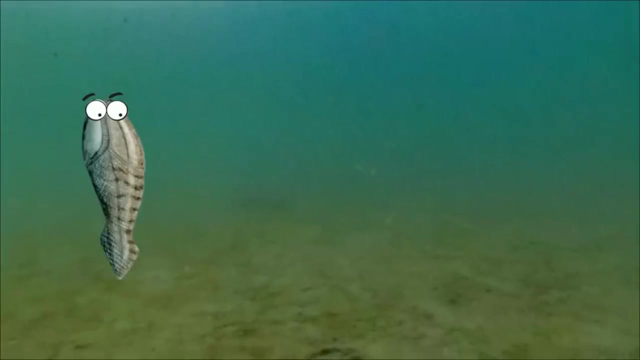 Climate change will always lead to extinctions of the most specialized species, But the more generalized ones will always manage to pull through. But rapid climate change from one extreme to another can push things to the absolute limit. And then things got even worse Because, as the oceans heated up, 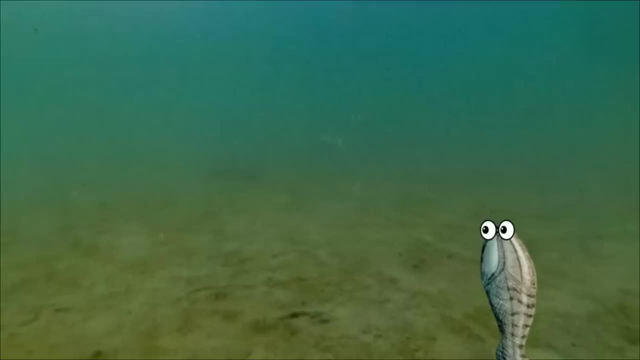 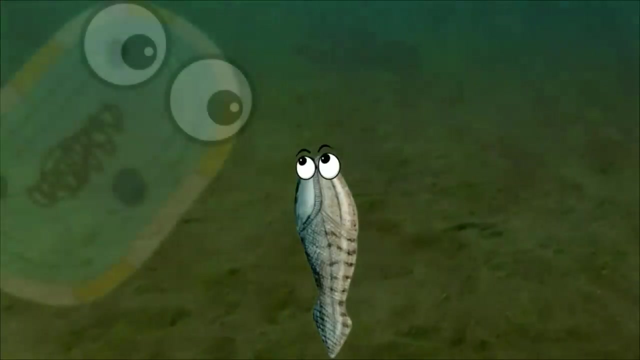 the amount of oxygen in the water would start to plummet, And that's never good for animal life, which at this point still lived exclusively in the water. But you know what it is good for: Cyanobacteria, That's right. 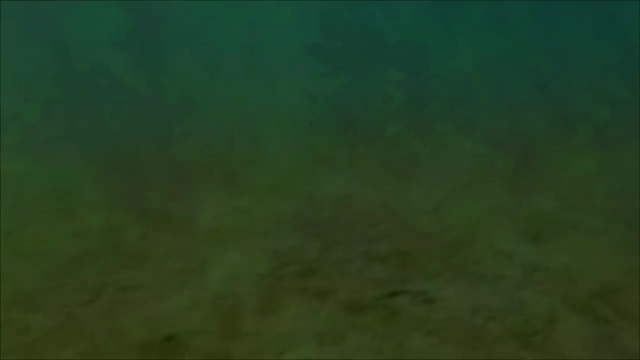 It's time for the return of the goo. As the cyanobacteria spread across the anoxic oceans of the late Ordovician, they literally choked every marine ecosystem And by the end of this rollercoaster of events, a staggering 85% of the species on Earth were wiped out. 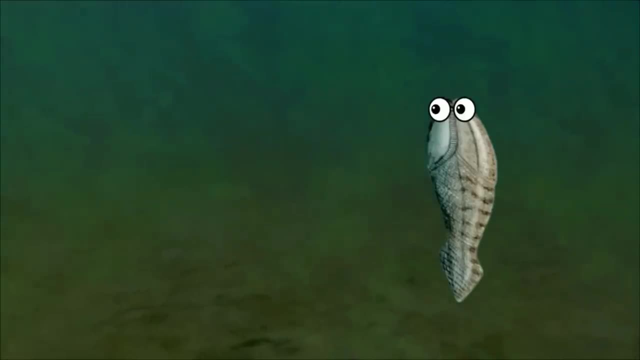 Making this extinction event well within the qualifications of one of the big five mass extinctions. In fact, despite this one being one of the least well-known, it's actually one of the worst. As the Ordovician comes to a close, we're left with a truly sick planet. 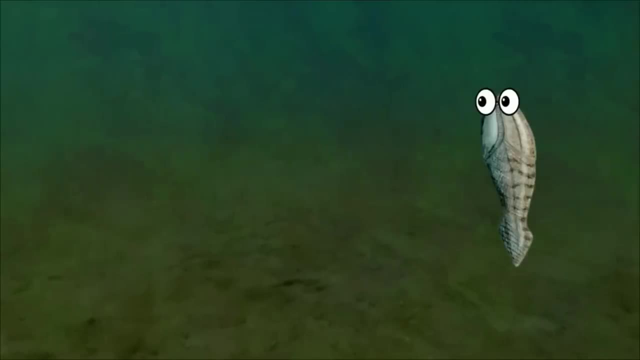 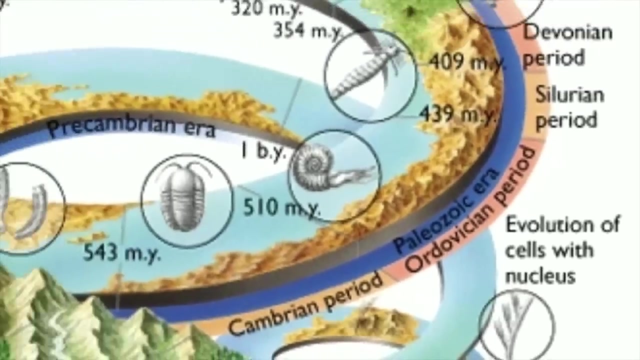 And there will be no swift explosive comeback that we've seen before. This level of cataclysm will take some time to recover from, But we still have about 444 million years to go to get back to the present, So life will inevitably find a way. 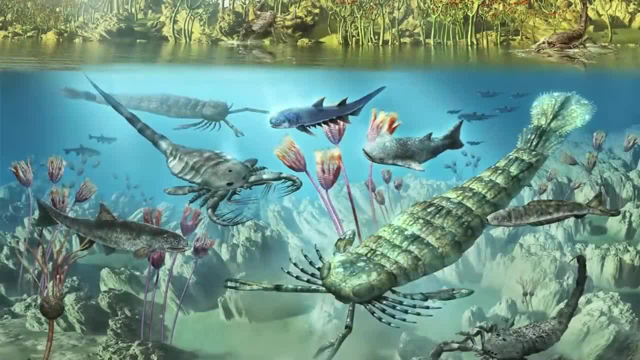 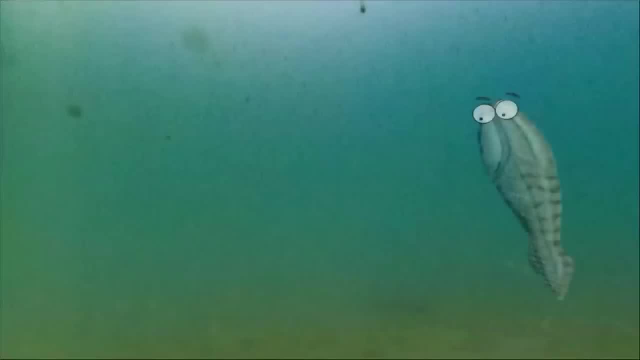 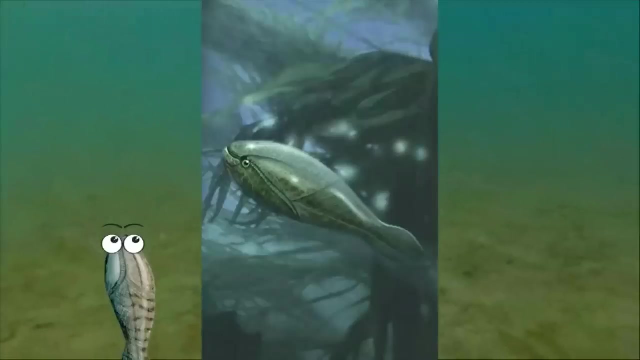 So the Ordovician ended on something of a depressing note. for sure, Complex life had been doing really well for millions of years, ever since the Cambrian explosion, And we were starting to see some really interesting ecosystems- At least the marine ones. Hell, by the end of the Ordovician. 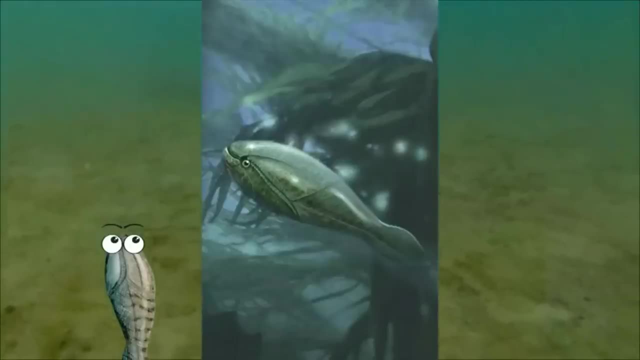 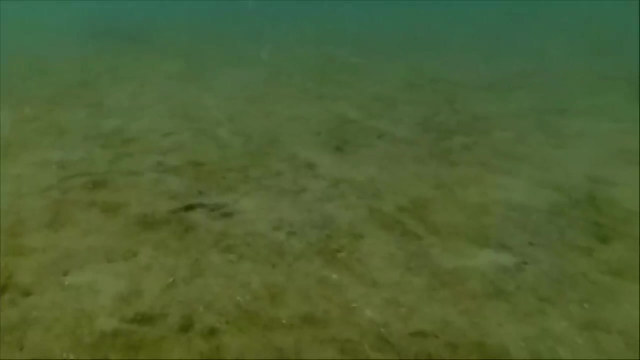 even the ancestral vertebrates were starting to be passable as true fish. But all that progress nearly came to a screeching halt when the planet went through a bit of a rollercoaster of climatic extremes. First it got cold, Not quite on the same level of another snowball Earth. 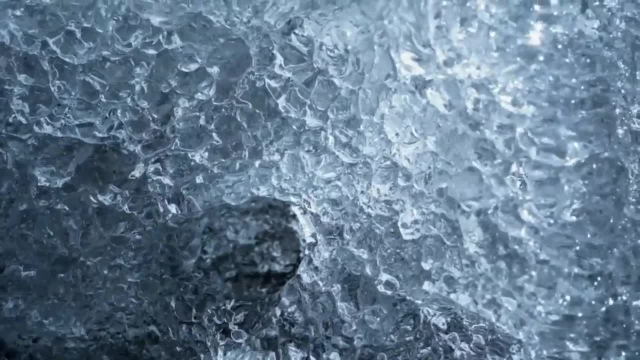 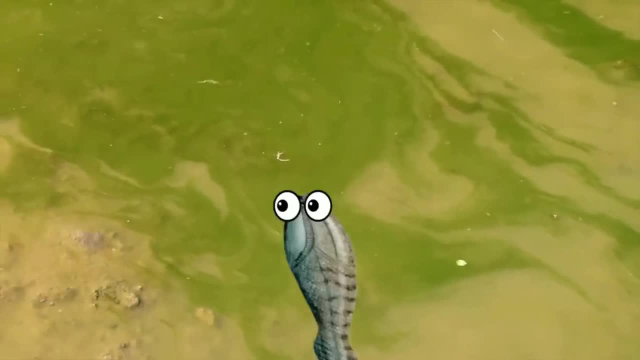 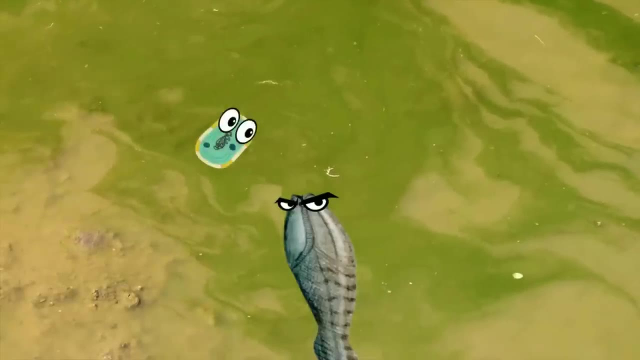 but still cold enough to be considered an ice age. Then it swung in the opposite direction and got warm and stagnant. Oxygen levels plummeted and the world's oceans were once again overwhelmed by cyanobacteria. Ugh, You were right. These guys are irritating. 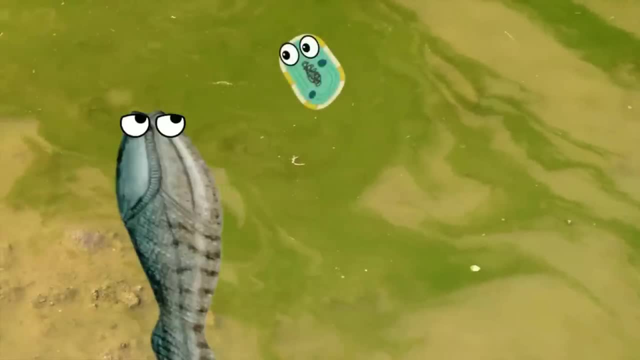 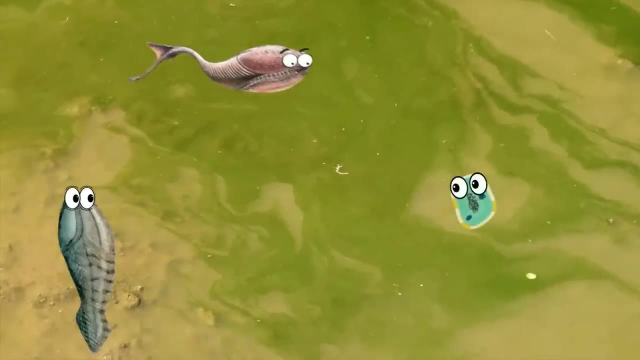 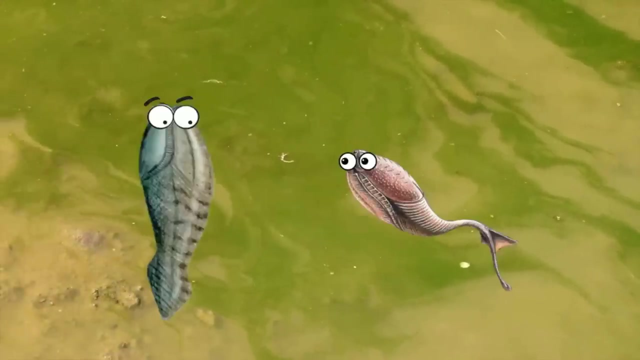 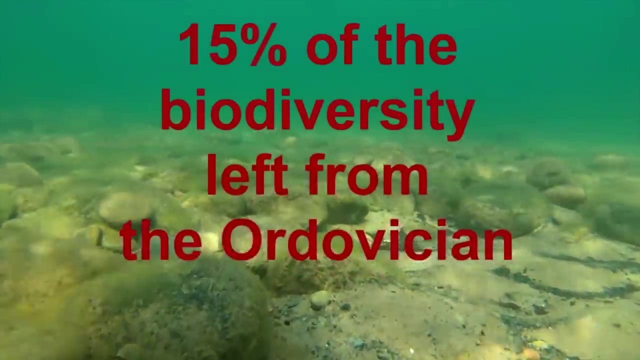 Yeah, tell me about it, But they're also tasty Alright. well, while you eat that, I think it's time that we move forward. As we leave the Ordovician behind, we're left with a world with only around 15% of its population. 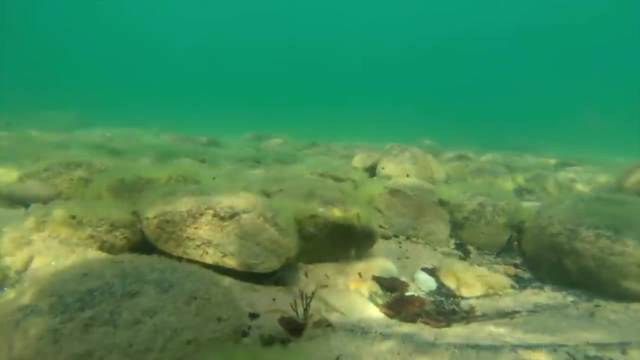 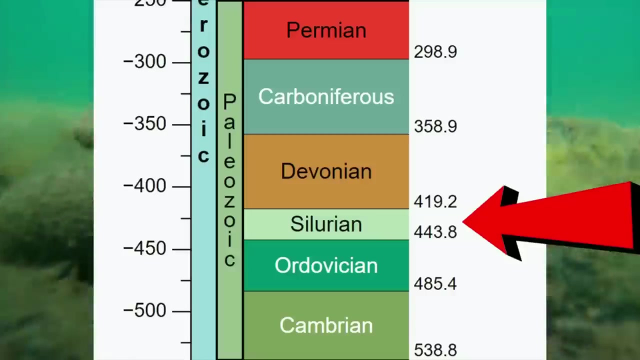 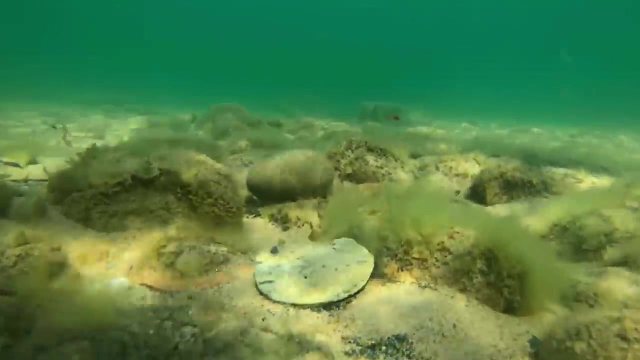 Life was going to have to take some time to recover from the first major bottleneck, since things became more complex than this, And that's what it seems like was happening during the roughly 25 million years that followed in the Silurian period, A comparatively short time in geologic terms. 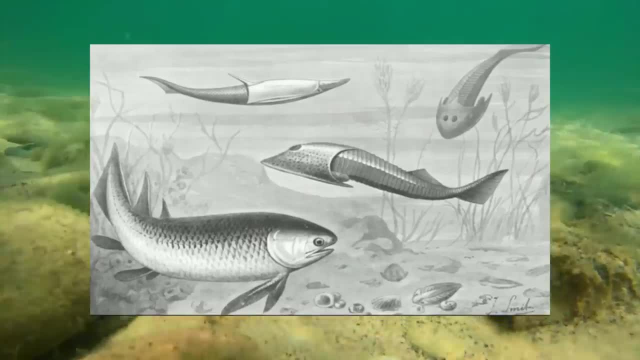 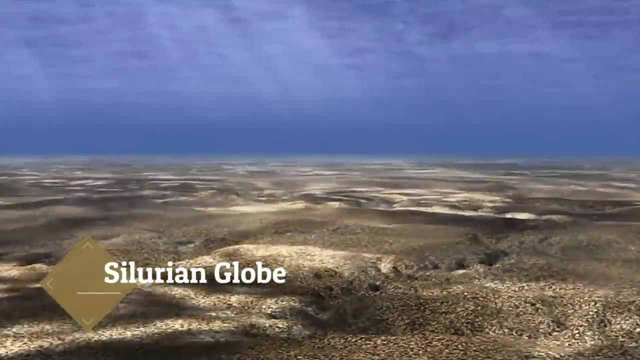 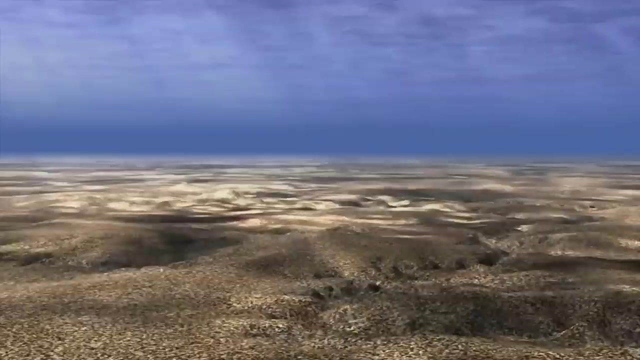 but definitely a very significant one, where the ancestors of everything alive today start to bounce back. In the wake of so much devastation, the warm climate that caused the glaciers to retreat to the south polar region of Gondwana continued to get even warmer. 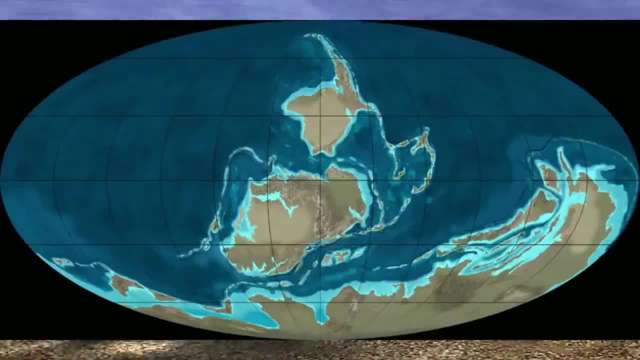 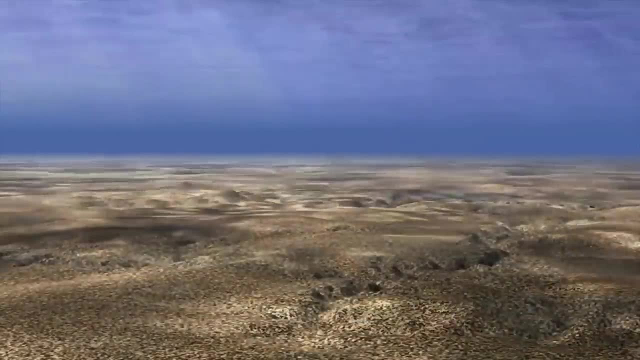 And this is how it would remain for the duration of this entire period. The thing that we tend to forget about climate change is that it's a constant factor in the story of life on Earth. Global warming, as well as global cooling, can have equally devastating effects. 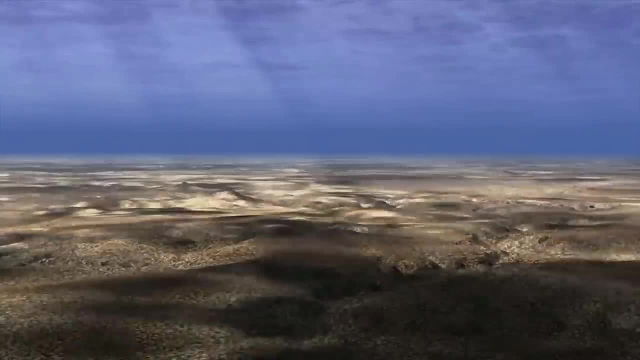 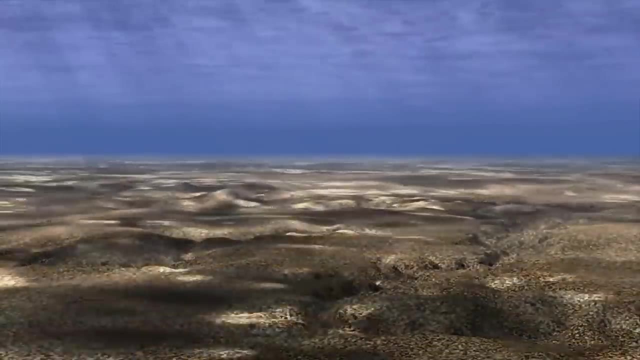 because it's a shift from what the current organisms living at the time are adapted to. Any time that you see long periods of time where the climate either remains the same or continues intensifying in the same direction, you will see animals adapt to be more and more. 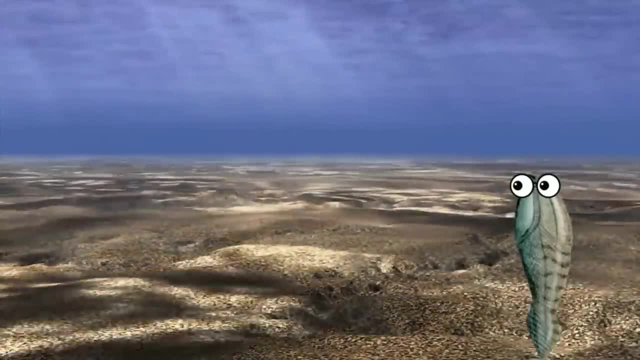 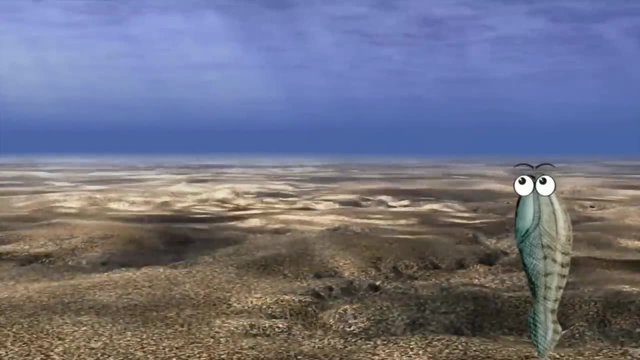 specialized to those conditions. So, despite the fact that the warming climate at the end of the Ordovician was one of the factors that led to a mass extinction, the animals that did survive did so because they were adaptable generalists who were able to make a living in the new 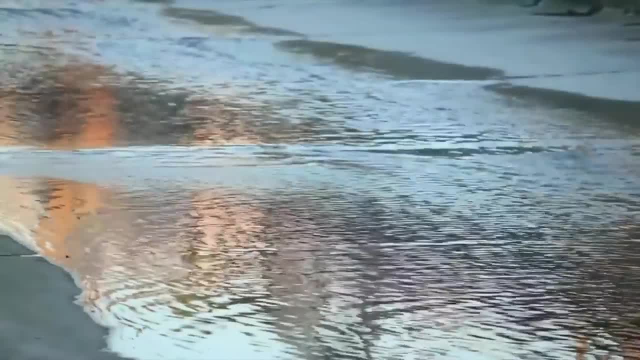 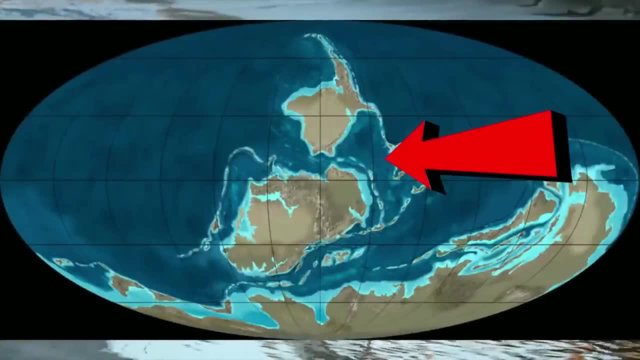 hot, lower oxygen world And, as sea levels began to rise, rivers and lakes would inundate them, the coastal areas of the supercontinent Gondwana, as well as the newly forming Euroamerica in the north, and this would become the perfect home. 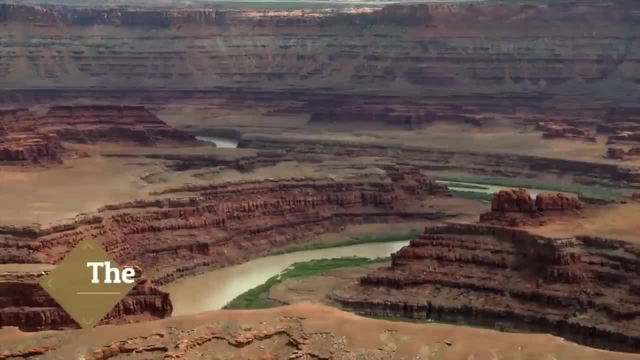 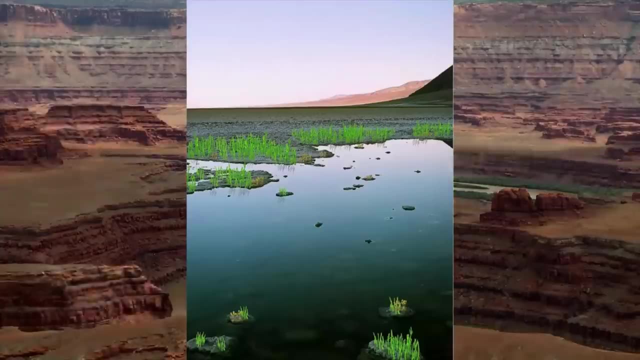 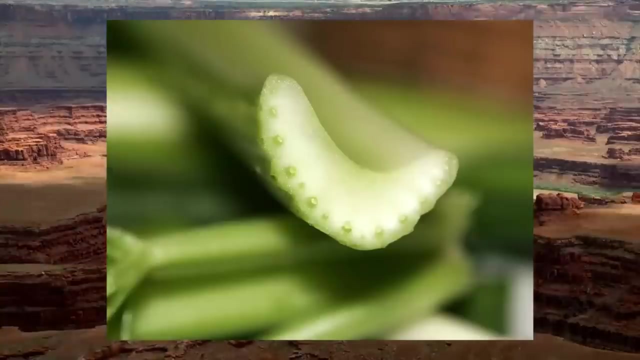 for some larger life forms. During the previous period, I spoke about how a few different species of plants were able to colonize the land, but they remained pretty small and simple. This would all change around 425 million years ago, when the plants finally gained vascular tissues. 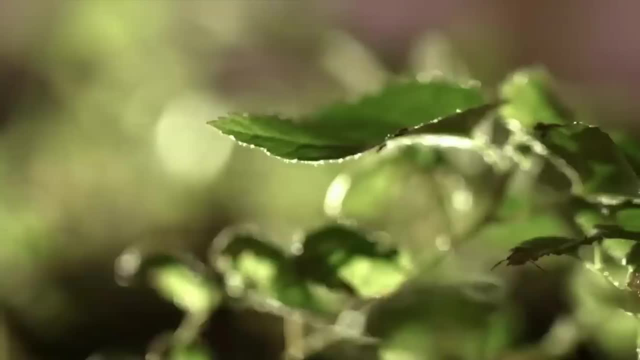 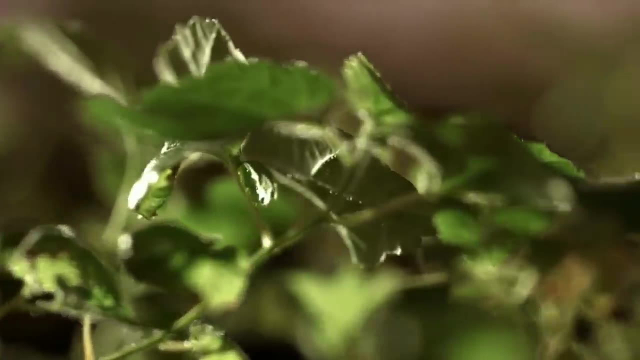 This was the first great leap forward in plant evolution. It allowed them to have a more stable structure and grow to greater sizes, as well as distribute water and nutrients throughout the plant. They were now capable of reaching up to the sky to access more of the sun's energy. 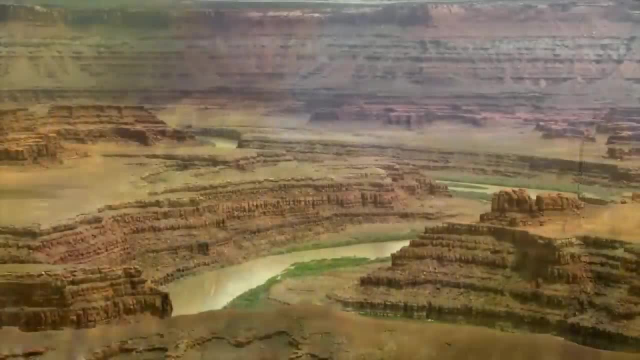 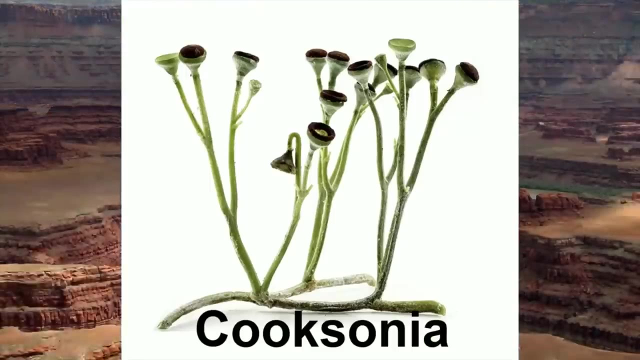 And along the streams and rivers of Silurian, Gondwana and Euroamerica. these early plants spread out even farther than their ancestors. Species like Cooksonia were some of the first to pioneer this new strategy, forming what could arguably be called. 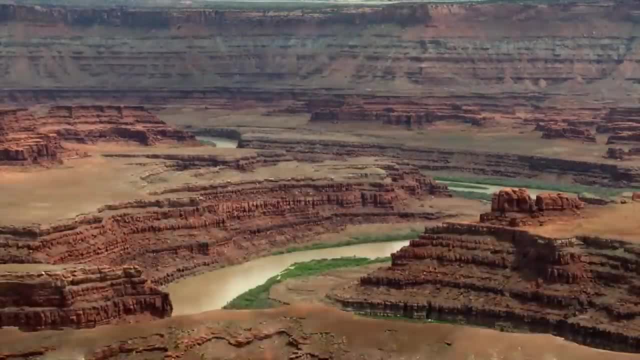 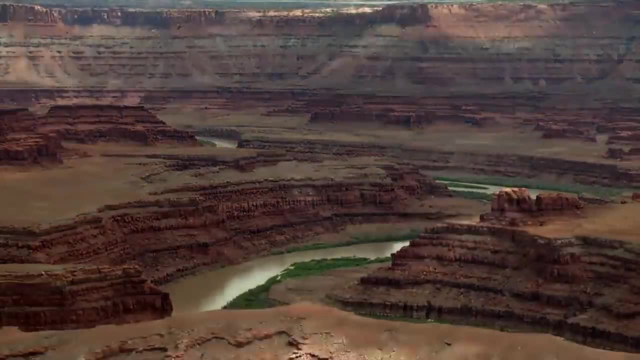 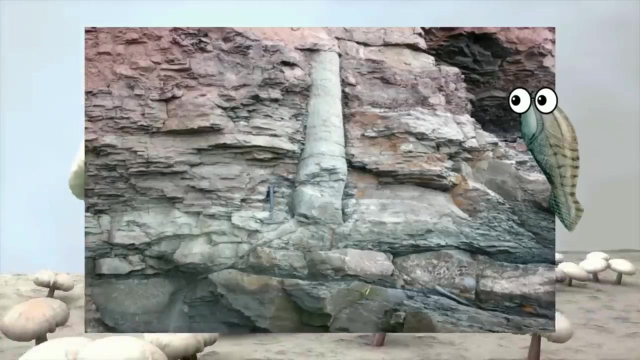 one of the first examples of a forest biome, But they wouldn't be the tallest organisms in these forests. That honor, instead, would go to an entirely different kingdom of organisms: Fungi. Yes, the very first forests on Earth were made up of giant tree-trunk-like fungus. 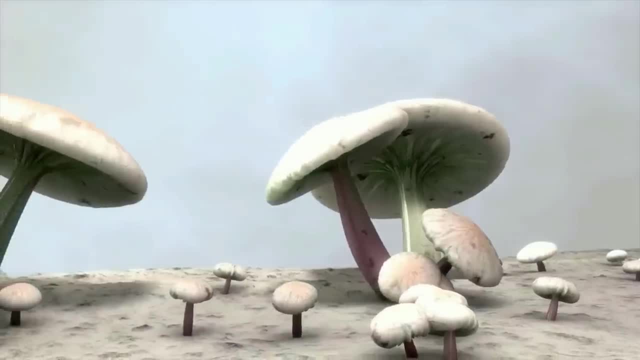 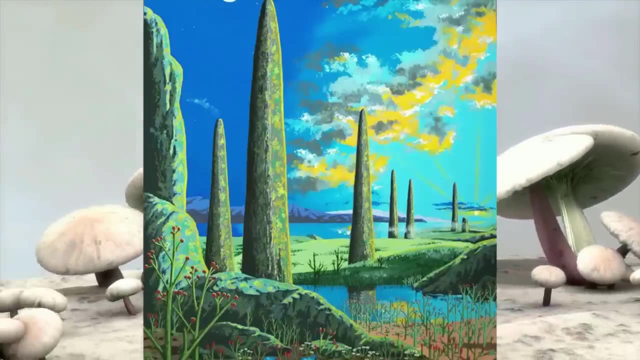 called Prototaxidides Now. technically, fungus had been expanding onto land ever since the Ordovician alongside the plants, But by about 420 million years ago they had become massive, eight-meter-tall trees, making them the largest organisms. 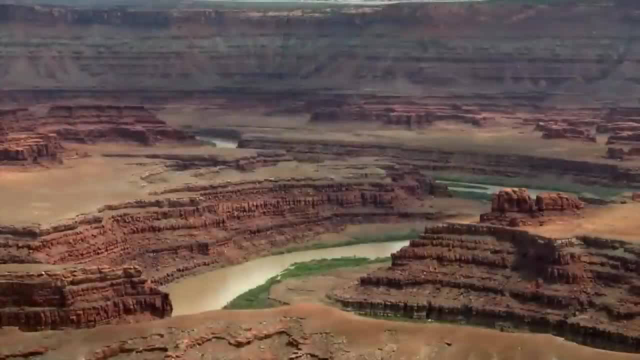 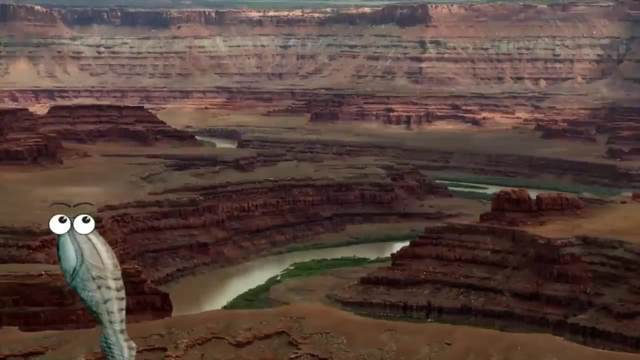 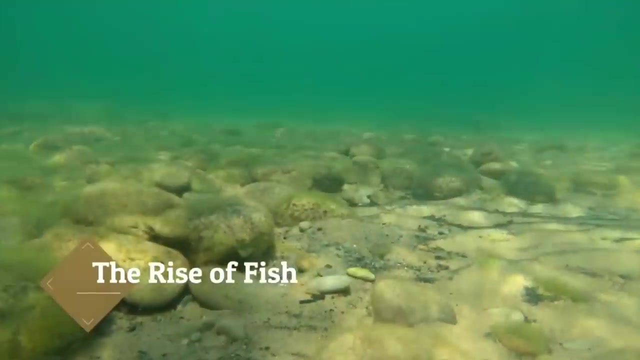 on Earth up to that point. This was the first time there was a really well-established terrestrial ecosystem fueled by the greenhouse climate and constant rain. There was just one thing missing, but that wouldn't be for long, As life on land was finally getting its proper start. in the towering fungal forests. life in the ocean was on the slow road to recovery. As far as we know, the large nautiloid predators like Orthoceras were some of the hardest hit by the Ordovician extinction. Some species of this group did survive. 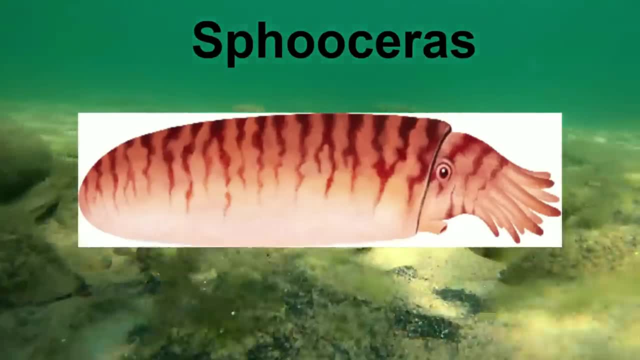 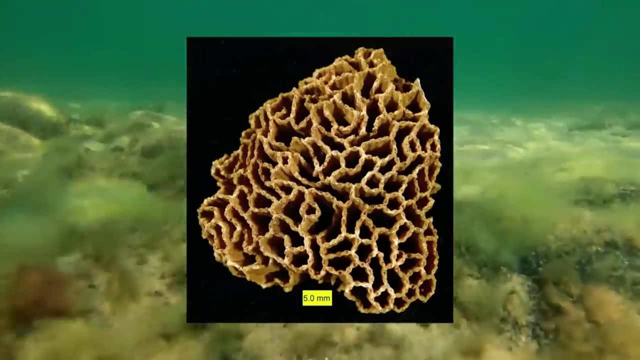 like Cephuseras, but they appear to have been less dominant going forward, And this left the niche of top predator open once again. And now, with the expansion of new types of corals and cranoids exploding in diversity, new marine ecosystems were beginning to open up. 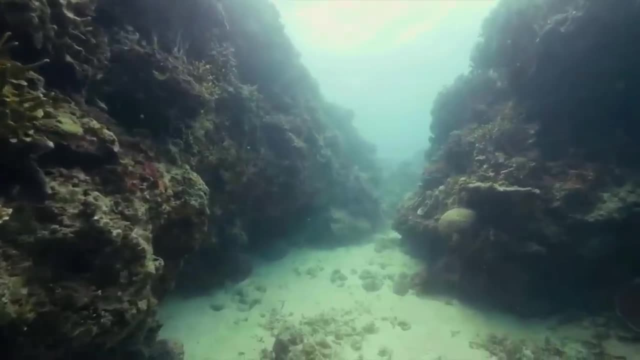 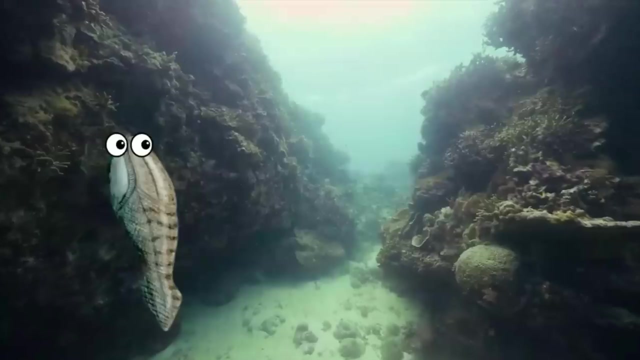 Something a little more similar to the corals reefs that we would know today, And, for the very first time, the chordates were finally ready to fight for the role of apex predator. The thing is, we needed something to be able, you know, eat something besides goo. 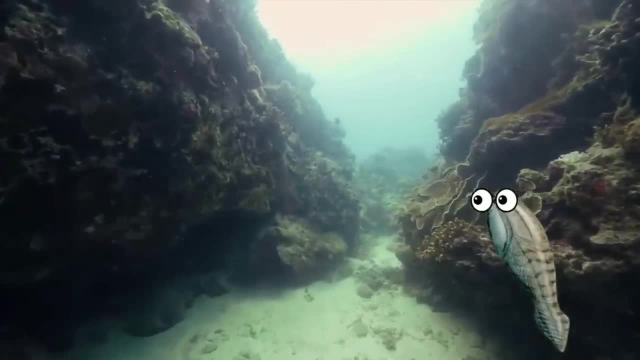 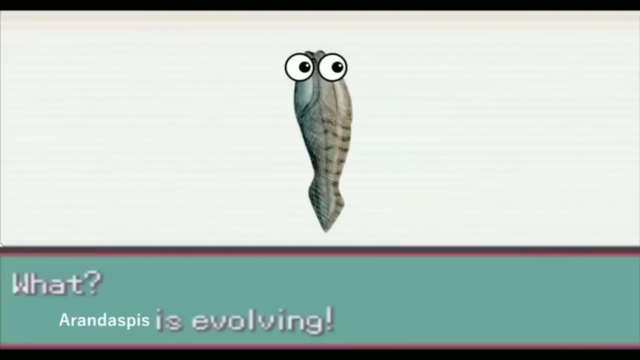 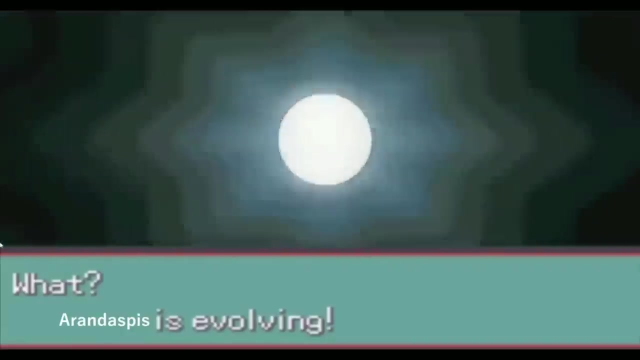 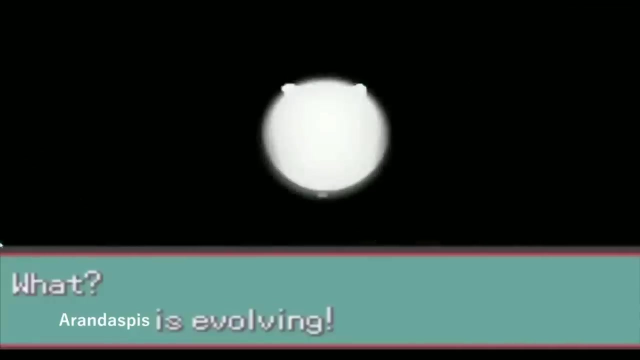 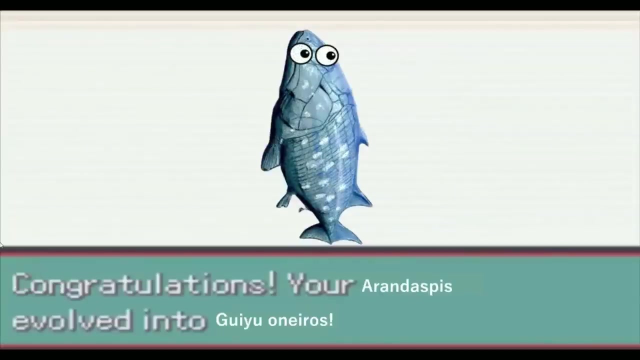 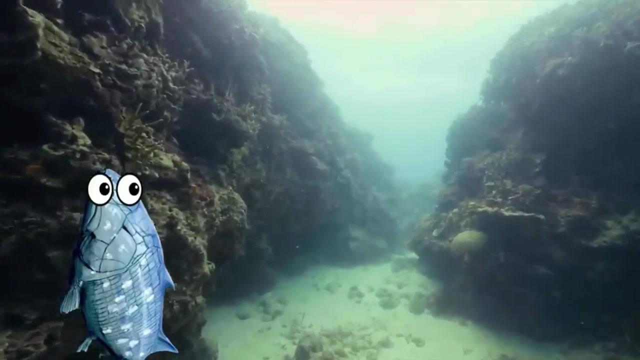 As well as a hard skeleton, The thing that would actually give us the name vertebrates, And you know what that means. This should be good Meep. It was around this time that these early true fish started to branch into several different forms. 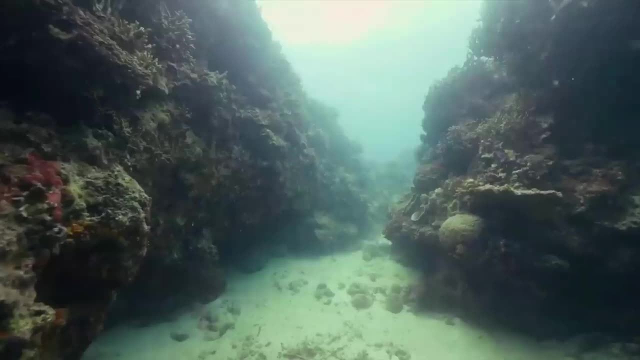 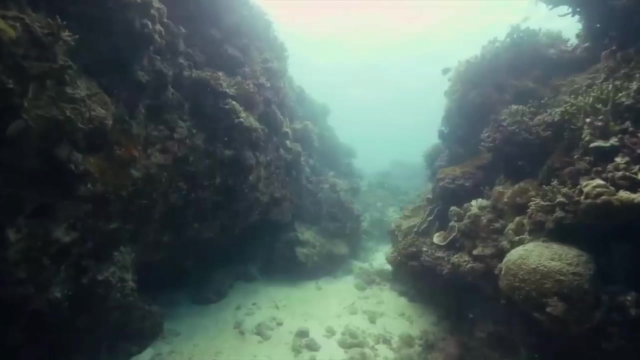 It all started with the evolution of movable jaws, And once that happened, vertebrates were finally able to move and take advantage of all the different food sources that had previously only been available to arthropods and cephalopods. The jawed fish split into three distinct groups. 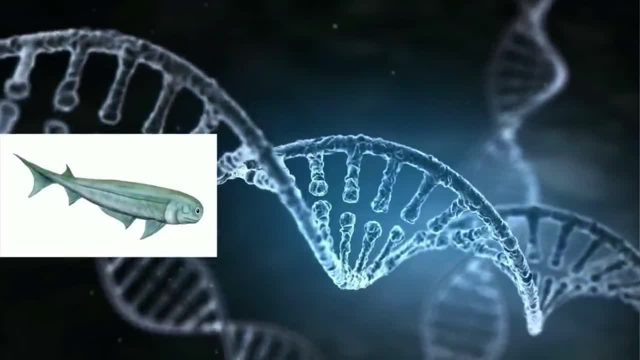 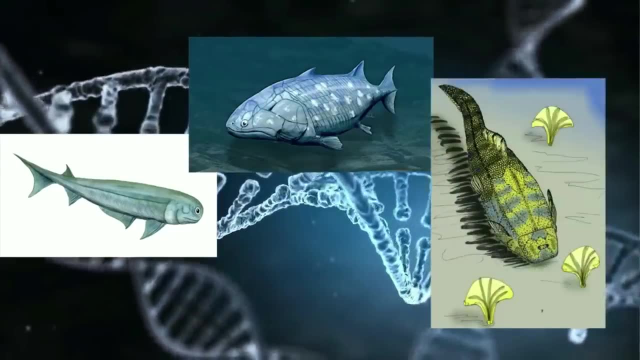 The cartilagelous fish, whose skeletons were made of a more flexible cartilage, The bony fish with the skeletons made of bone. And the armored fish, which took a strategy from the arthropods and had a partly external. 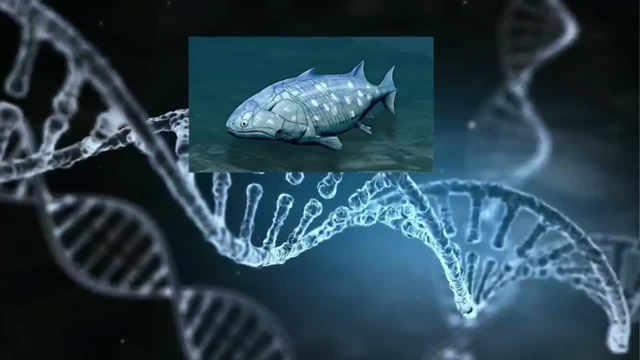 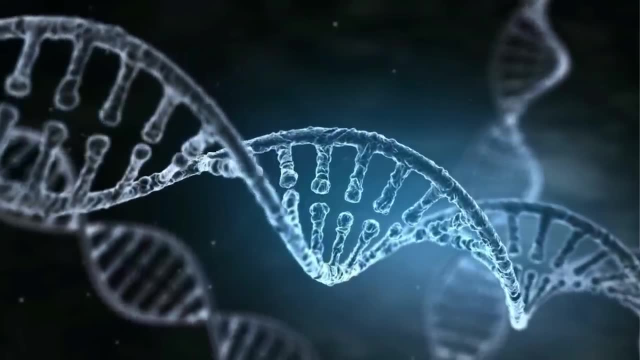 bony skeleton, which helped with defense, And then from there the bony fish would split into the ray-finned fish and the lobe-finned fish. It was really an age of fish diversification. And this is when my new form, Goyo oiranus. 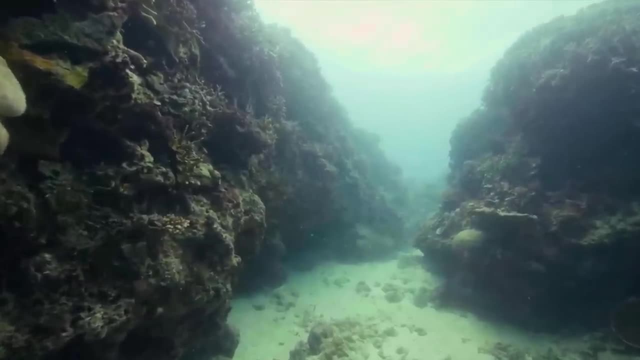 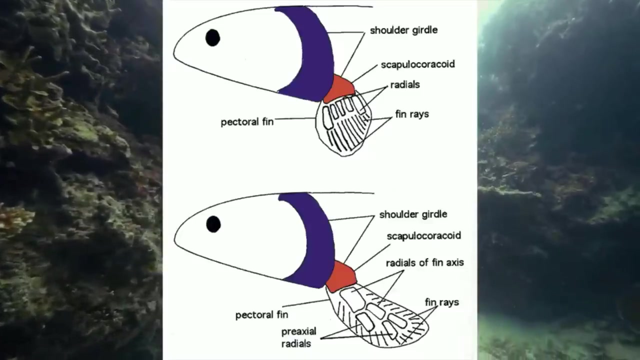 first appeared The earliest lobe-finned fish we currently know. What's special about these fish in particular is the fact that the fins are actually mounted to the pectoral and pelvic girdles. This allows for greater range of motion and possibly even the ability to bear weight on them. 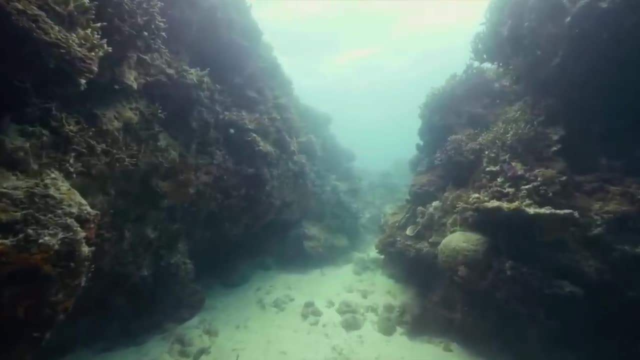 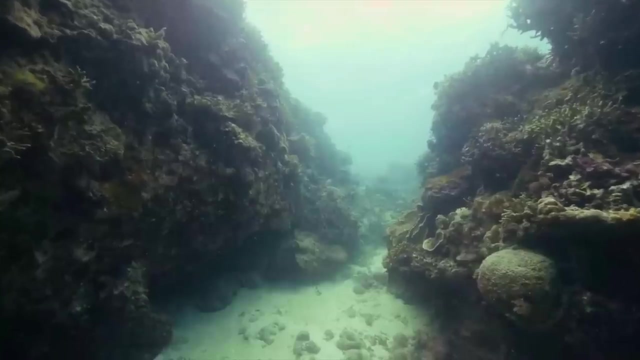 The seas were starting to fill with life once again, But the thing is, most of the fish still remained pretty small: Goyo just measuring around 30 centimeters long. But that was because, despite our explosive variety, that came in about 10 million years. 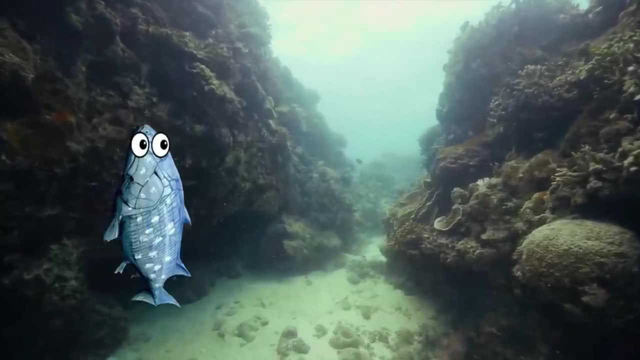 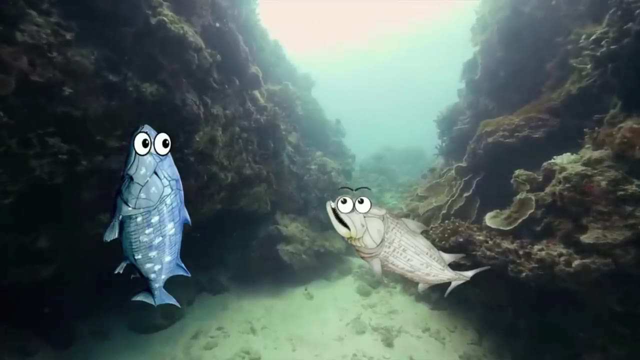 we were not alone. In fact, the fish were still far from the dominant group during the Silurian. Aw crap. Even with teeth like this, we still haven't taken over. Well, there was one, But it wasn't Andriolepis. 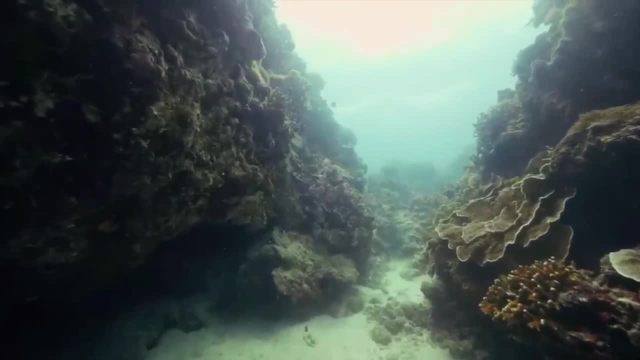 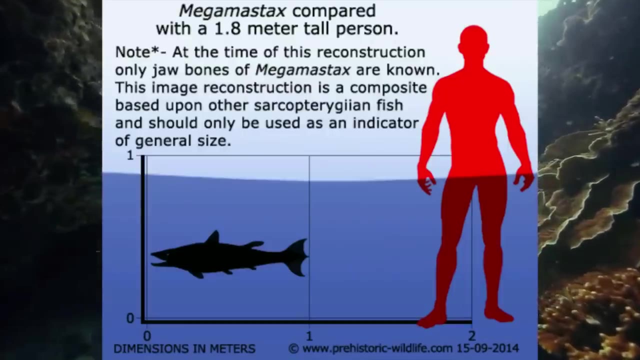 Sorry, The only one that even came close was the monster fish Megamastix, A lobe-finned fish that grew to a meter long, making it the largest vertebrate on Earth during this time. You're like a third of that size. 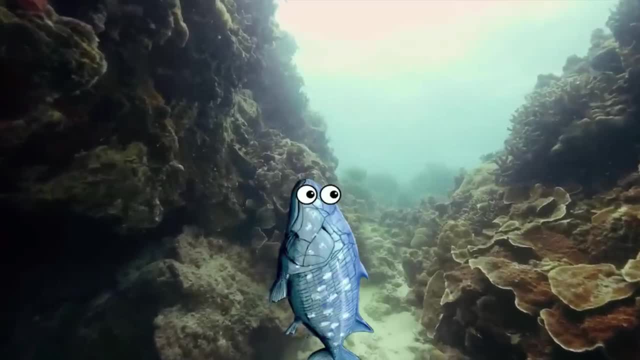 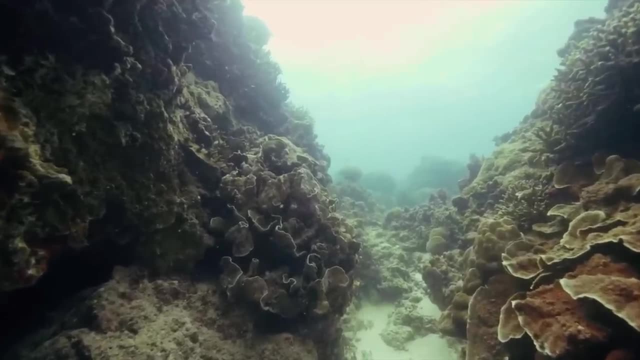 Plus, there's still another group of animals that I still need to cover from the Silurian, Another survivor from the Ordovician extinction that would become the ruler of these warm shallow seas. It's more big bugs, isn't it? 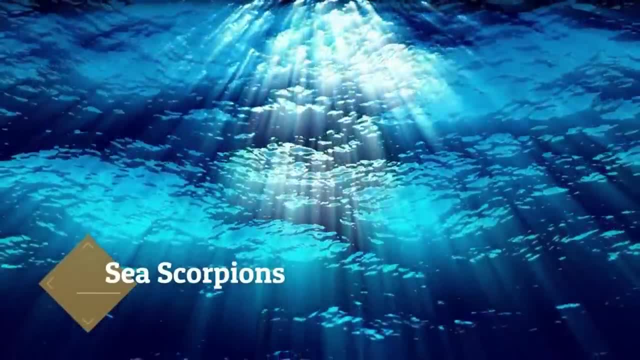 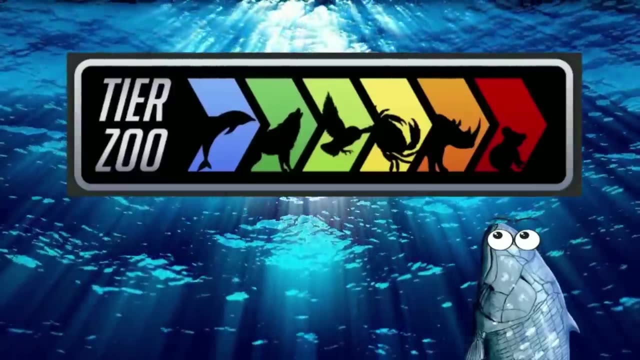 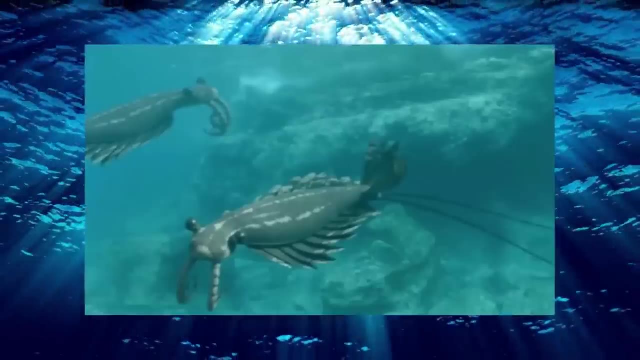 Oh yes. Ever since the Cambrian, the arthropods have been major competitors for dominance in the world's oceans. In TierZoo terms, they were top builds in the game. The first huge successes for them came in the form of trilobites and radiodonts. 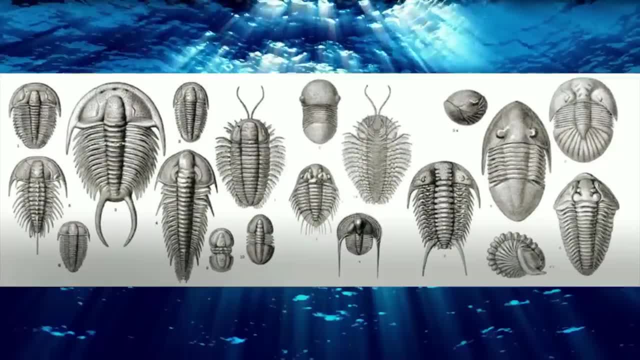 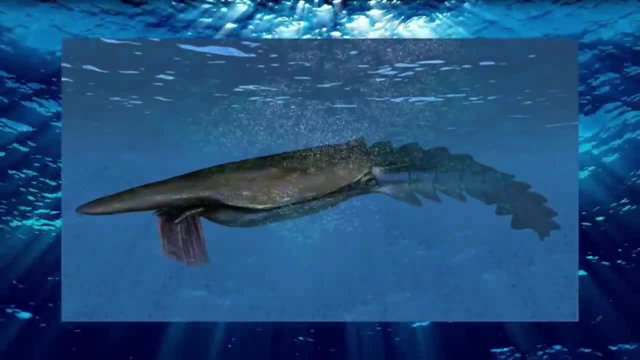 But there were many other groups that branched off along the way. The trilobites were still going strong and even bouncing back during the Silurian. However, the radiodonts were starting to run out of steam at this point, And as the Ordovician gave way to the Silurian, 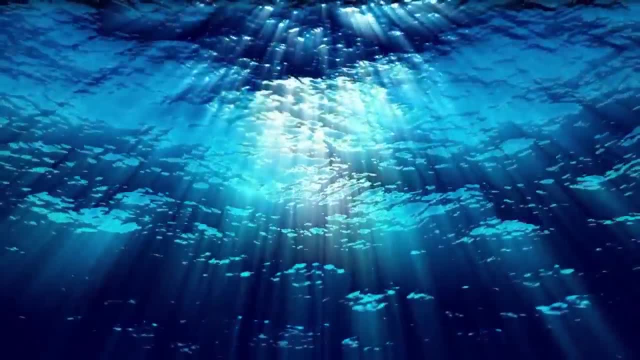 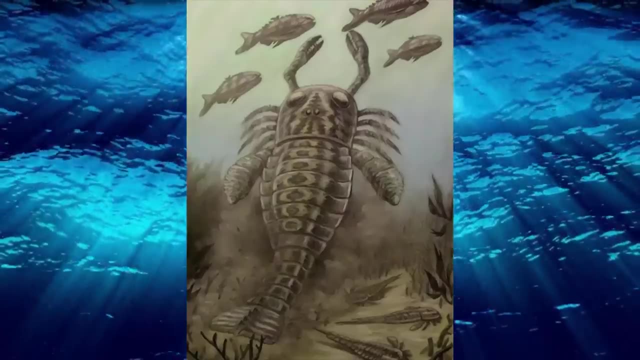 a new group of arthropods started to take that top predator role, The Eurypterids. We already talked about those first species, like Pentacopteris, and how they were a threat to the early vertebrates during the Ordovician. 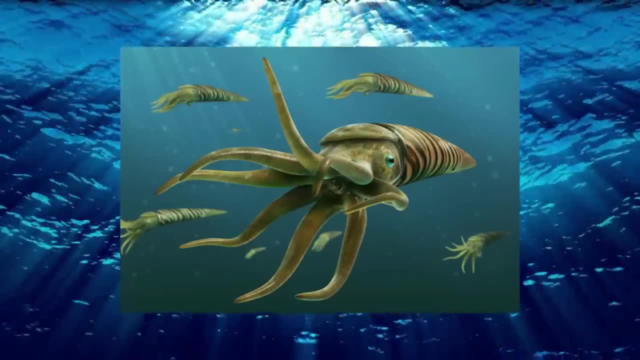 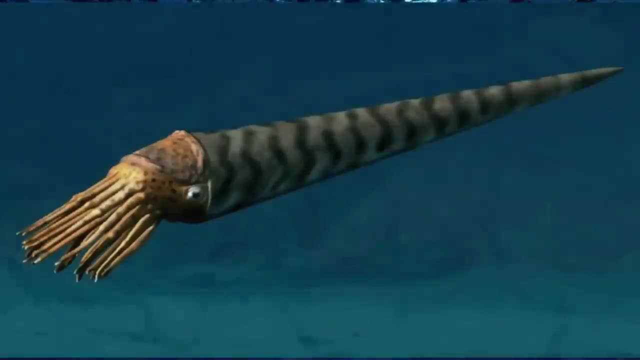 But the thing is they had a lot of competition from the large cephalopods, So they struggled to get out of the role of bottom feeders. And although the carrot krakens weren't entirely gone, they were definitely less abundant than they used to be. 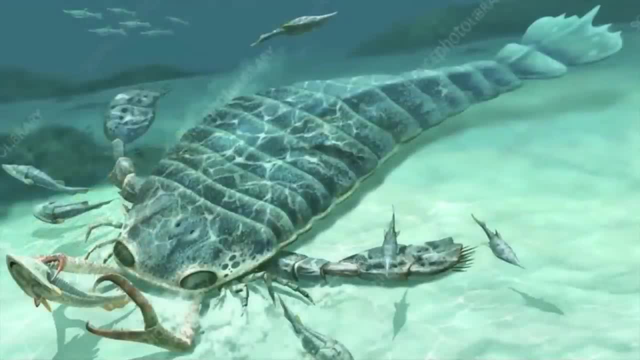 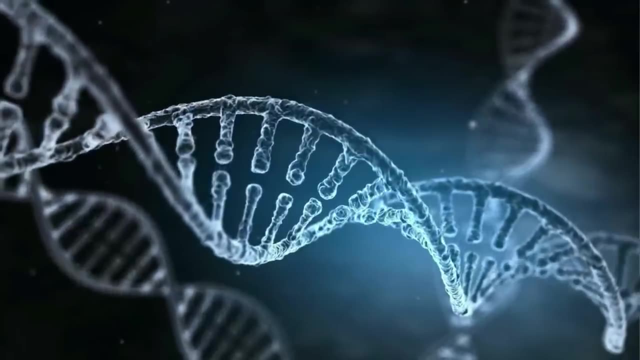 And just like we see time and again, there will always be something waiting to take advantage of open niches. It was finally the sea scorpions' time, And they would split into two different body plans and survival strategies. The Styloneuria-esque sea scorpions. 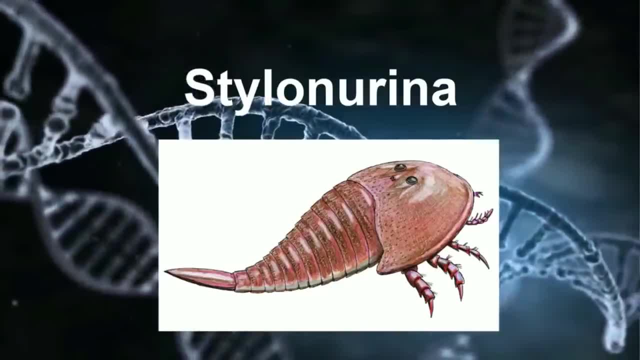 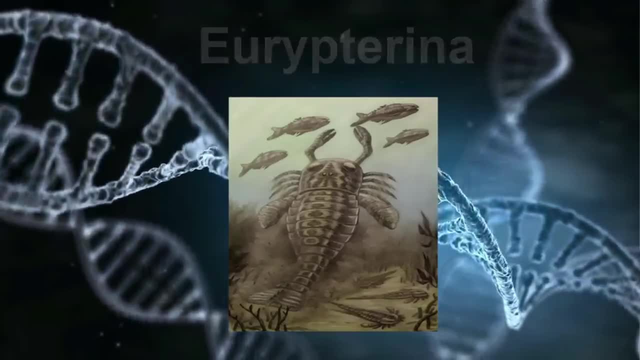 which remained smaller and kept to the ocean floor scavenging on whatever they could, And the Eurypterina sea scorpions, who took a more active hunting approach. They had paddle-like arms that allowed them to swim through open water. 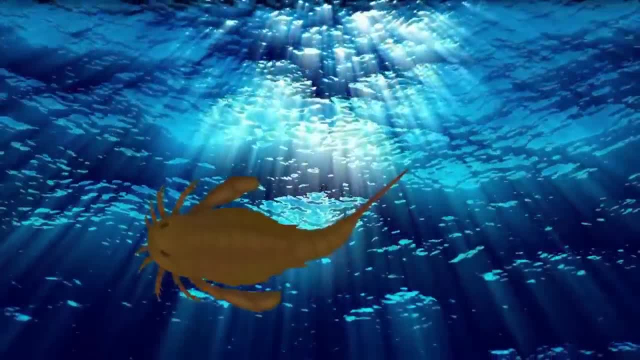 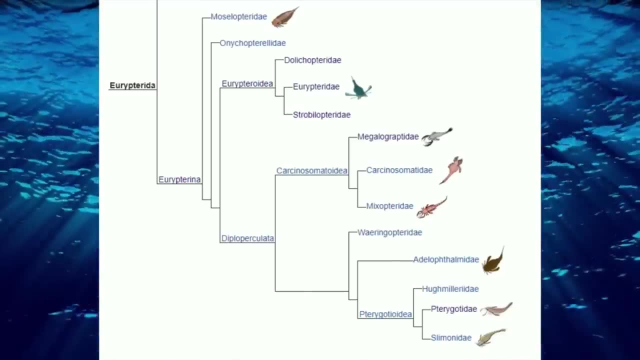 which gave them the edge they needed to become the kings of the panthelassic seas. This one group evolved into several different species, But by a wide margin. the most common was Eurypteris, which makes up up to 95% of the sea scorpion fossils. 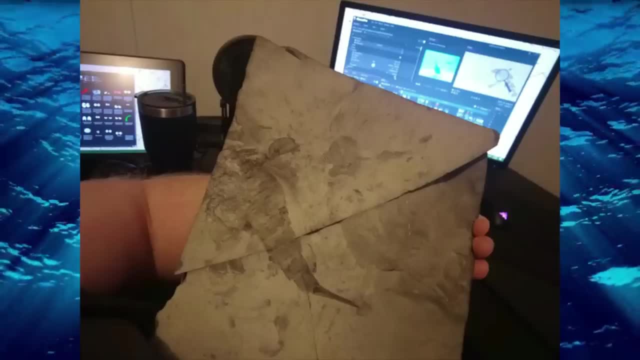 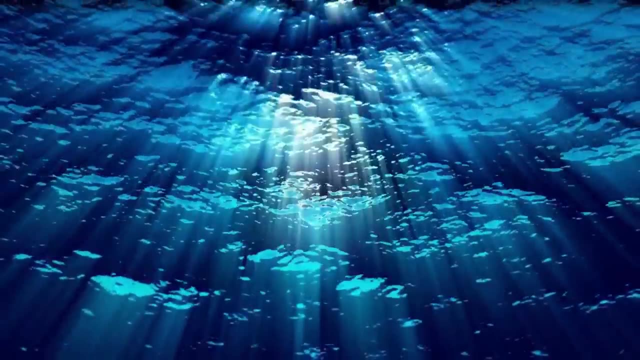 found from this time. I even own one Now. Eurypteris was a modestly sized little horror at between 13 and 60 centimeters long, But one genus of sea scorpions that stood out among the rest was the monstrous Pterygodus. 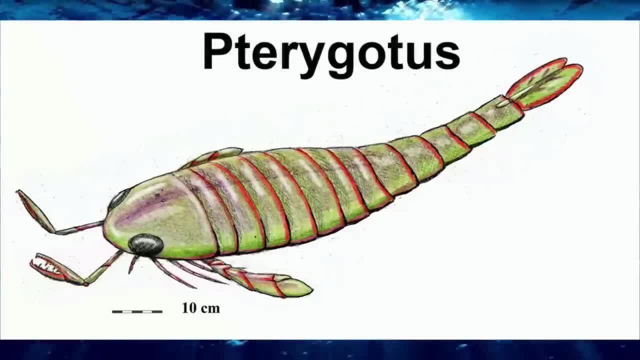 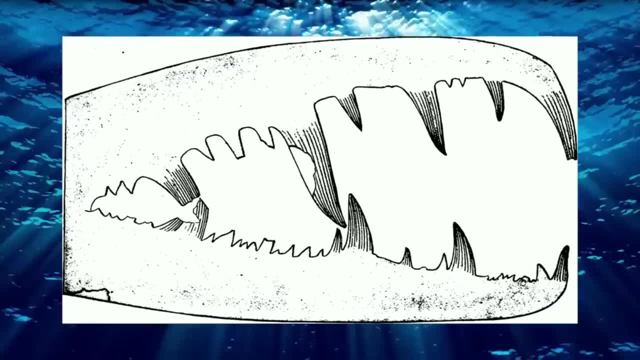 These guys were the apex predators of the Silurian. They grew to nearly 3 meters long and had grasping claws that actually make them look more like the true scorpions that they share their name with. It's actually believed that these arthropod predators 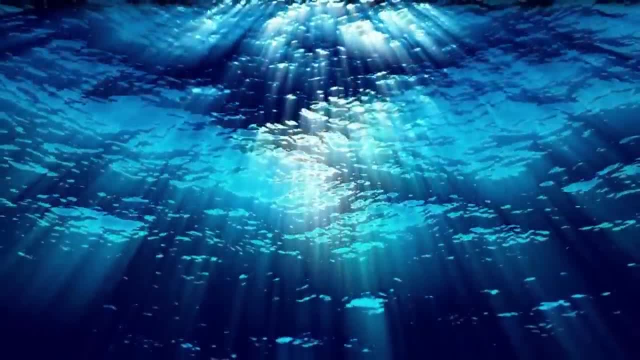 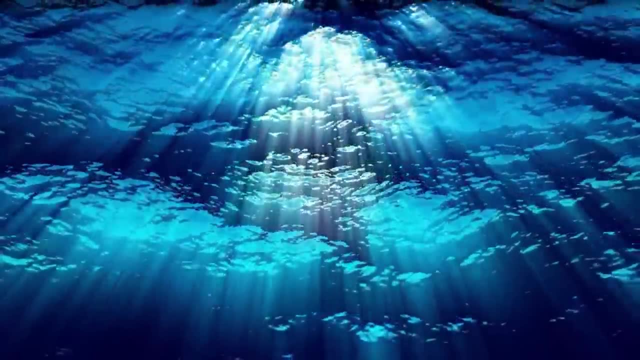 evolved in response to the explosion in fish diversity that was going on across the globe. It appeared to almost be an evolutionary art of an arms race between the two groups, And with things like Pterygodus, Megamastix and a handful of remaining squid around, 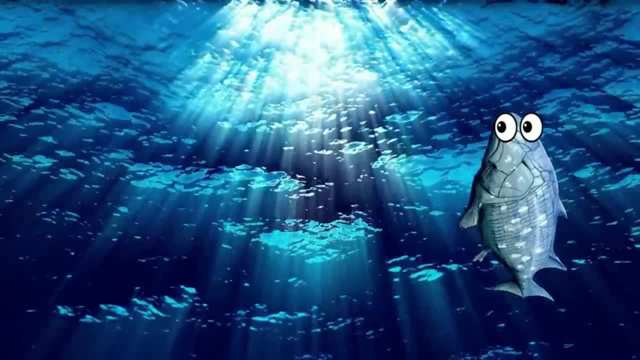 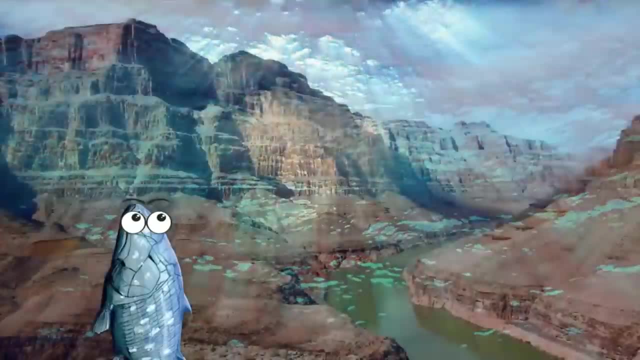 the oceans were getting pretty scary again. If you were small, it was beneficial for you to try to avoid these sea monsters, And the best way to do that would be to enter the New Frontier, a world where the only giant organisms was giant mushrooms. 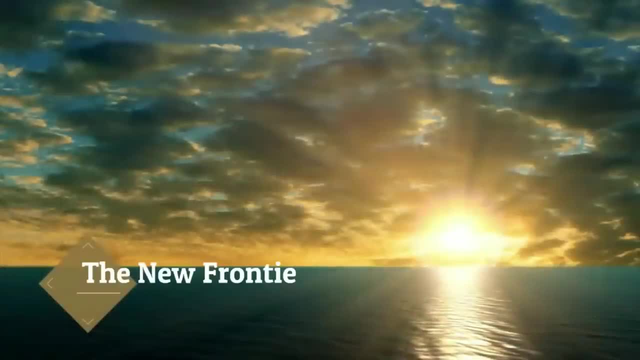 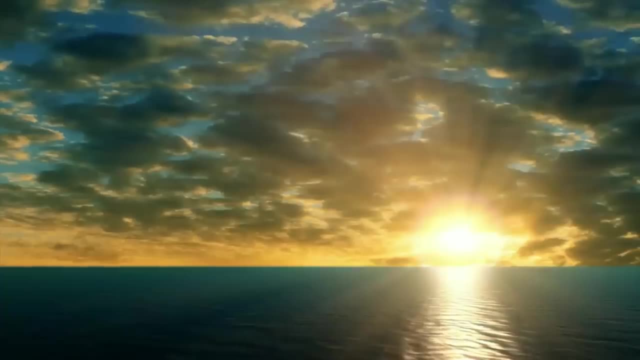 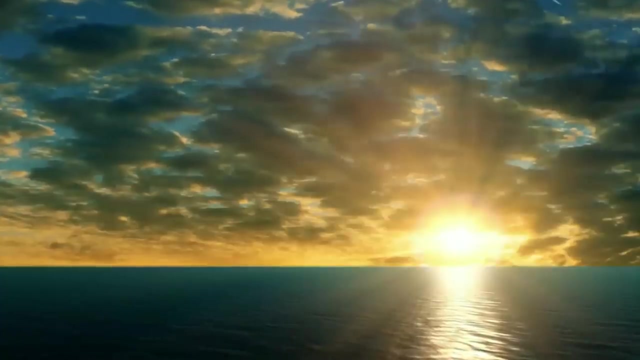 That's where the future is. The Silurian was not nearly as devastating as the end of most periods in Earth's history. There were a few notable things that happened, though. The climate that had held on for 25 million years was about to go from warm to hot. 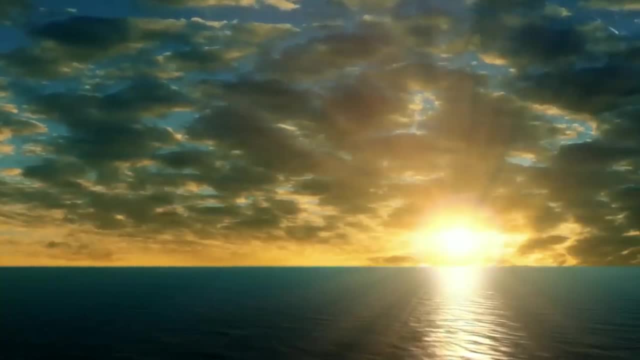 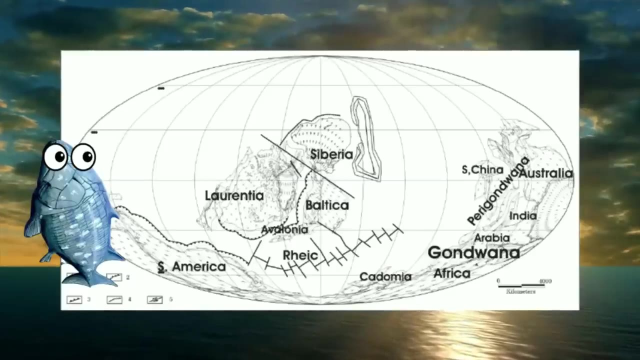 And, as a result, now there was no ice at all at the poles, And now tectonic activity was starting to ramp up. The last pieces of Euro-America were starting to come together as Siberia pushed into the North American plate, and this formed a new giant mountain range. 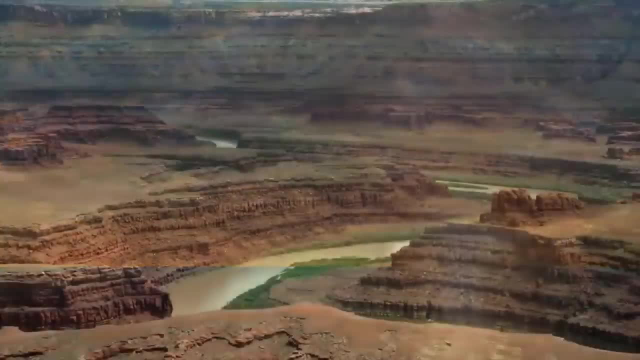 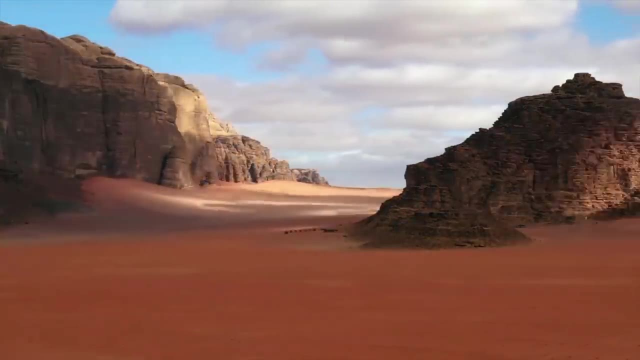 But currently there was nothing that could live there. All the plants and fungus that currently lived on land still had to stick close to the water, leaving the interior of both supercontinents a massive desert. But it's in this moment that our world is the most alive. 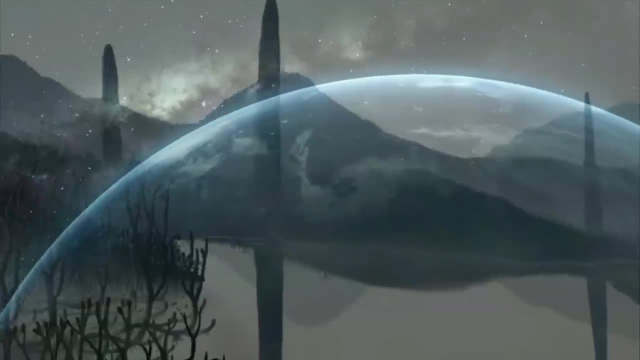 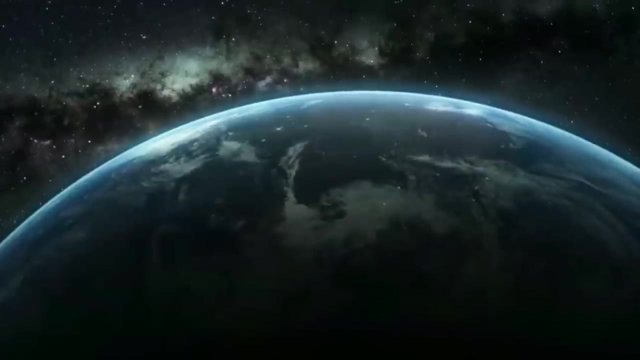 that it has been so far, And among the giant mushrooms and tiny plants, there is a chance that you might actually see movement for the very first time, Because, to survive the onslaught of the fish and sea scorpions competing beneath the waves, 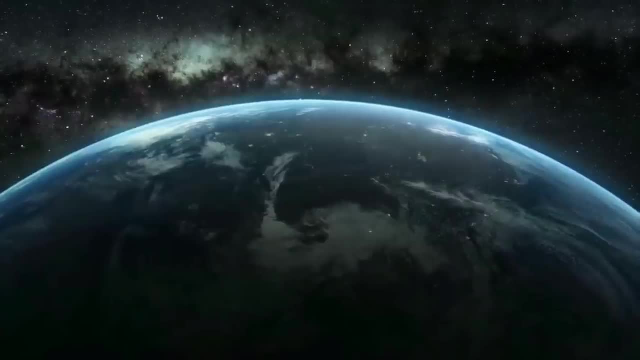 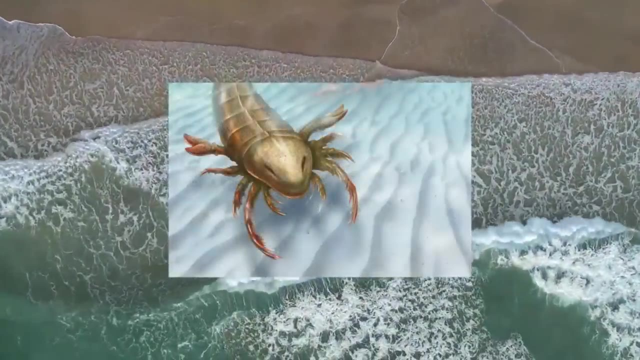 a few groups of small arthropods have managed to make the transition into living, at least part of the time, on land. It probably started small, with some different kinds of Eurypterids crawling up onto land to lay their eggs, far away from everything else. 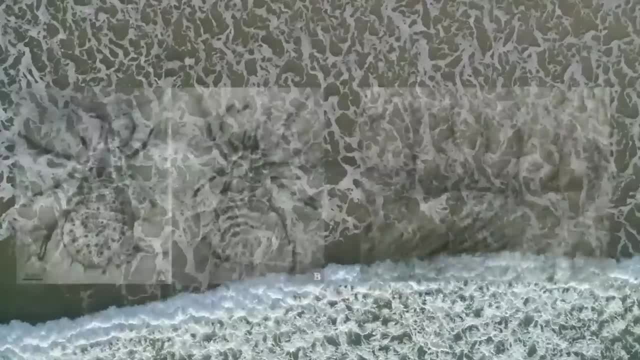 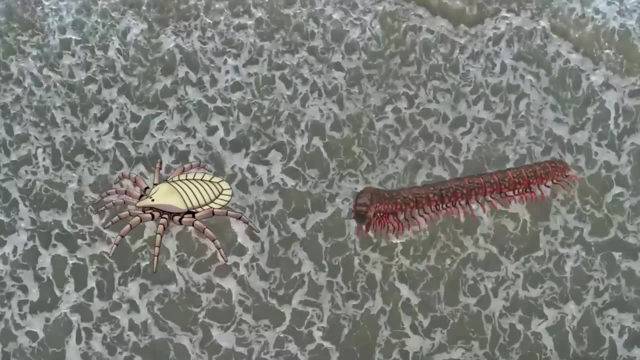 But by the time we get to the end of the Silurian, we see the first signs of fully terrestrial animals, The first pioneers being millipedes and possibly even the true arachnid cousins of the sea scorpions. For the moment at least, it was a bug's world. 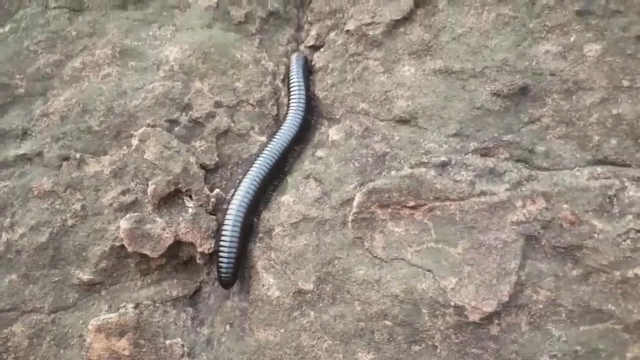 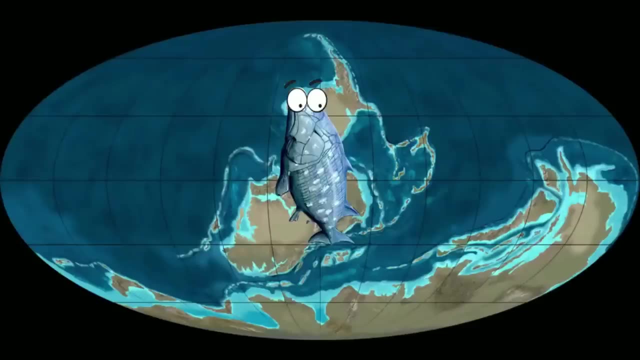 However, in the seas, the competition between vertebrates and arthropods was about to intensify. Going forward, things are going to get a lot more interesting, In my opinion at least, And actually the next three periods were some of the most requested times. 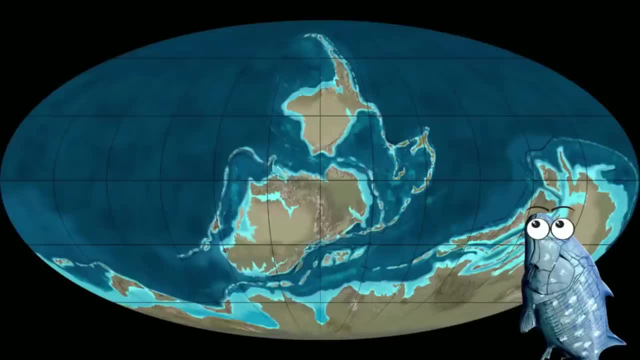 for me to cover. even before I started to do these deep dives into the history of the Earth, And considering how little publicity the Paleozoic gets and how interesting life gets during this time, I can see why. But for now I must leave you on this beautiful world. 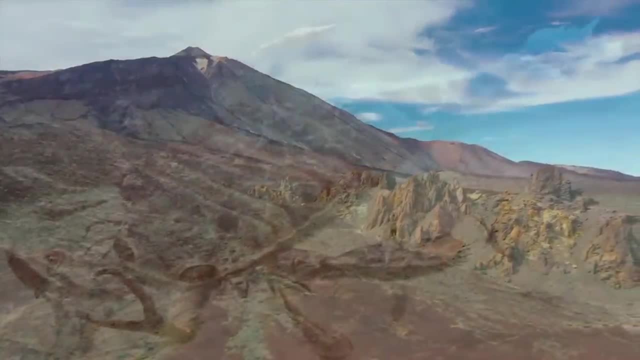 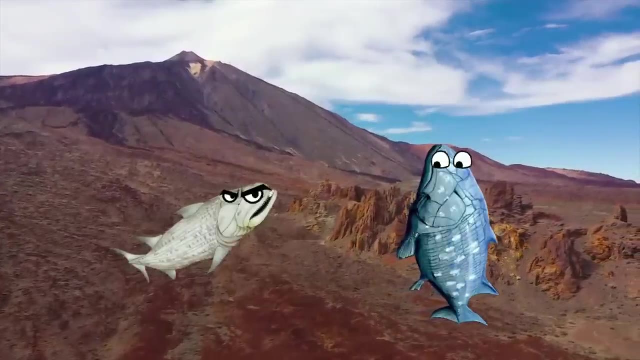 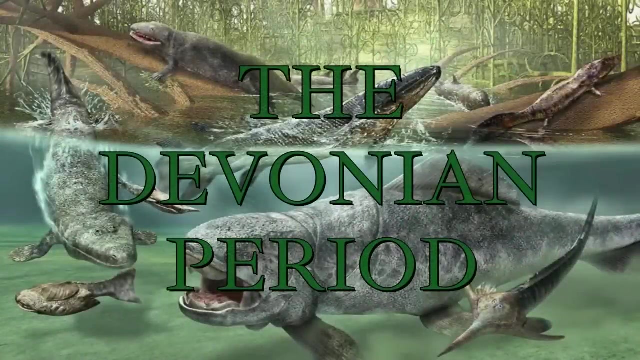 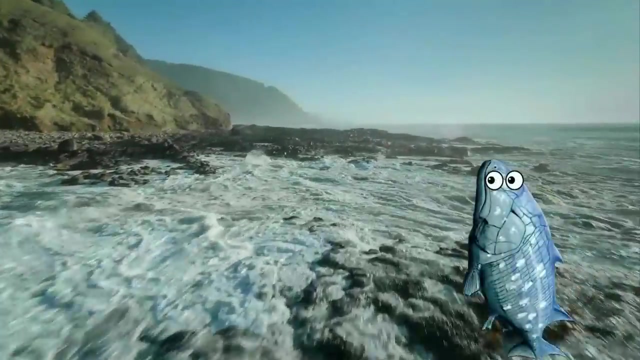 of giant mushroom trees, scorpions the size of crocodiles and Tim Tim looking like a creature cooked up by Jim Henson on cough syrup. Hey, Have a good one, everybody. Thanks for watching. Following the recovery from the Ordovician mass extinction. 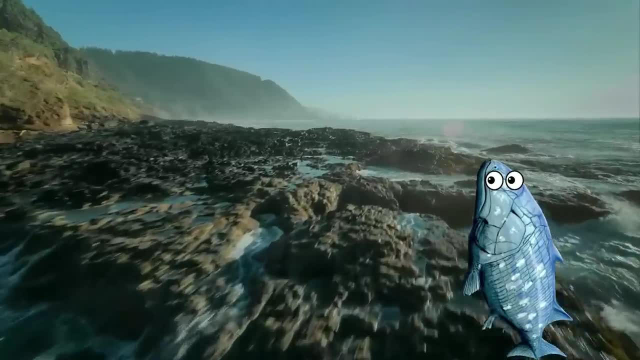 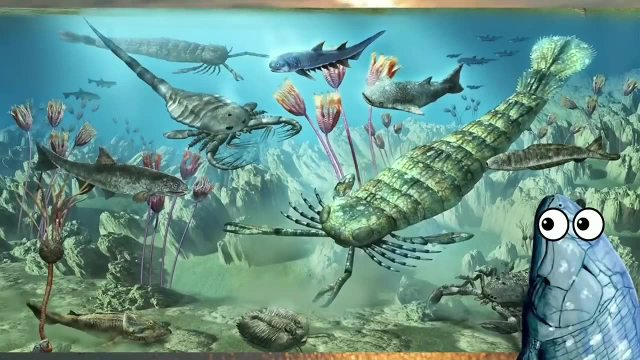 we started to see our world develop a lot of ecosystems that at least loosely resembled some of what we see today. In the seas, complex food webs of arthropods and fish were starting to thrive, And on land we were starting to see something akin to the very first forests. 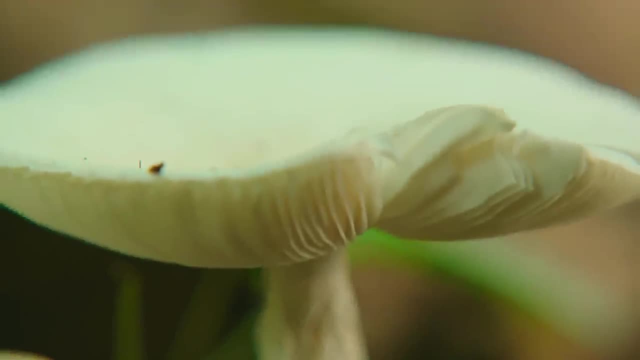 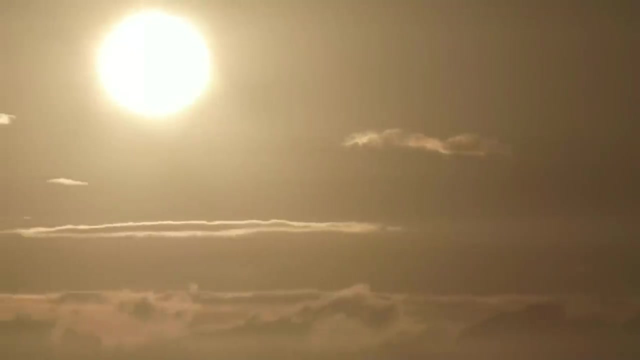 But instead of trees, the tallest organisms were strange forms of fungus that evolved into eight-meter-tall pillars and the true plants remaining closer to the forest floor. The relatively stable climate of the Silurian allowed life the chance to bounce back, But by the beginning of the Devonian 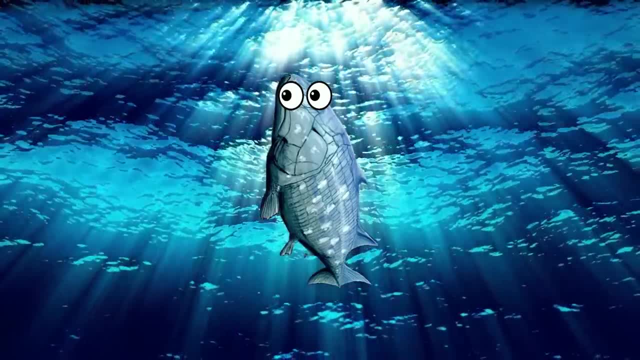 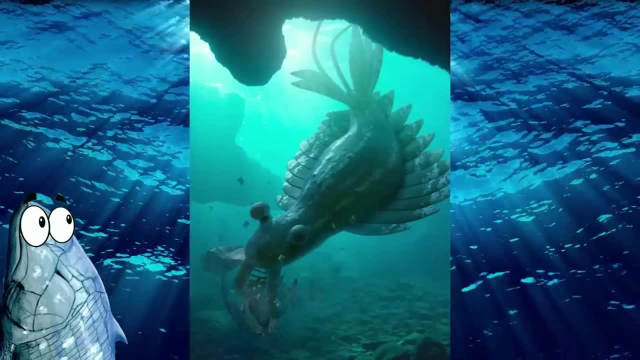 competition was about to pick up, all culminating into the first really big evolutionary arms race. On one side we had the arthropods, who had dominated most marine ecosystems since the Cambrian explosion, And on the other was the early vertebrates. 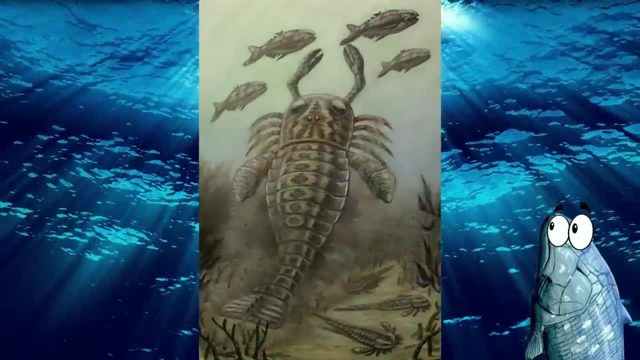 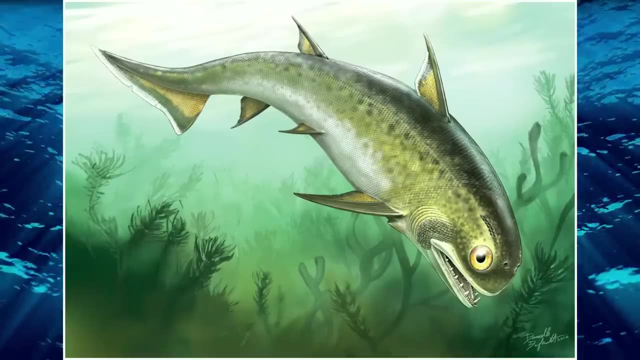 who had been at a bit of a disadvantage, without armored bodies that came in the form of exoskeletons. But ever since the evolution of Jaws, our ancestors were at least able to fight back. And around 419 million years ago, as the Silurian ended and the Devonian began, 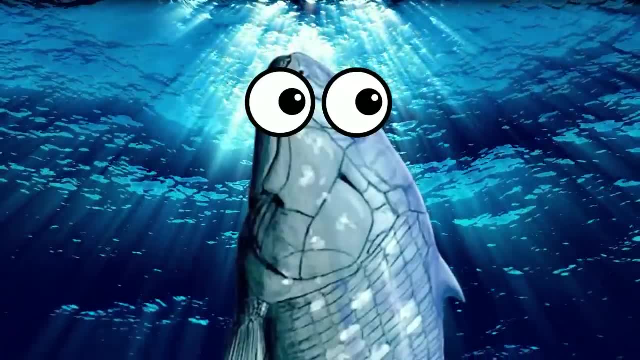 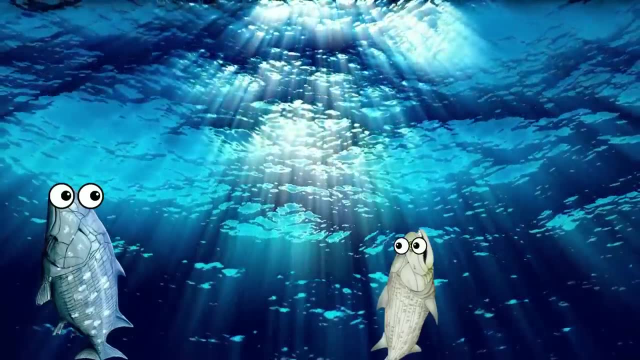 a surprising thing started to happen. We were about to start winning, Because at least one group of fish were starting to become every bit as defensive as the arthropods, And this would also give them the tools that they needed to become the apex predators in this increasingly bountiful world. 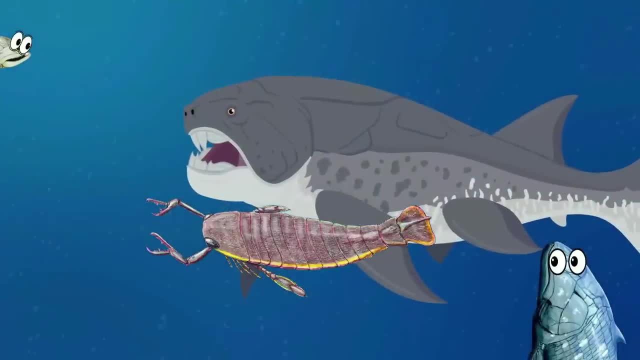 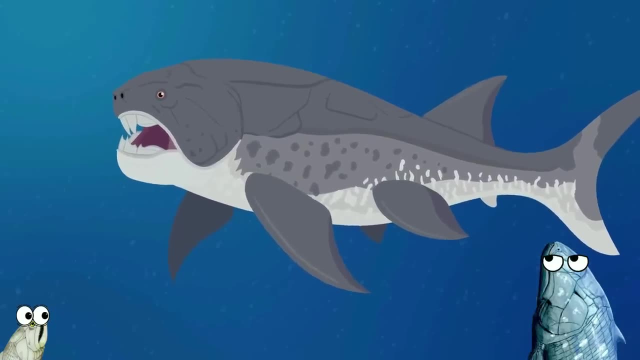 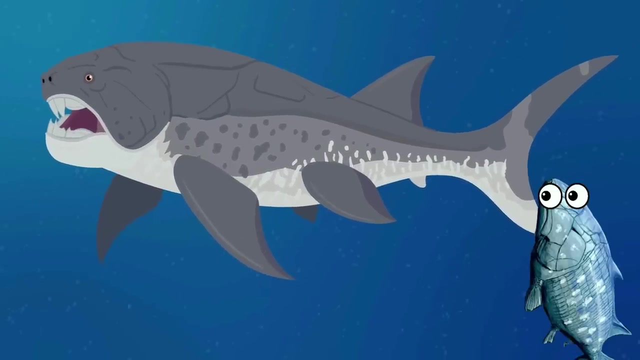 I cannot help you, but you know what can help you? A fish with a guillotine for a face? Huh, You may have a point. Maybe we should come up with a new strategy to get through this period, But we have a ton to get into before we even get into that. 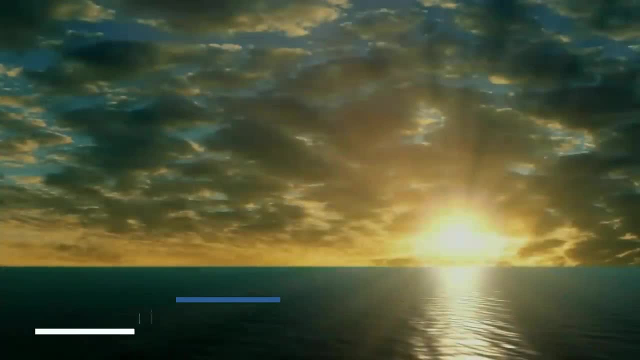 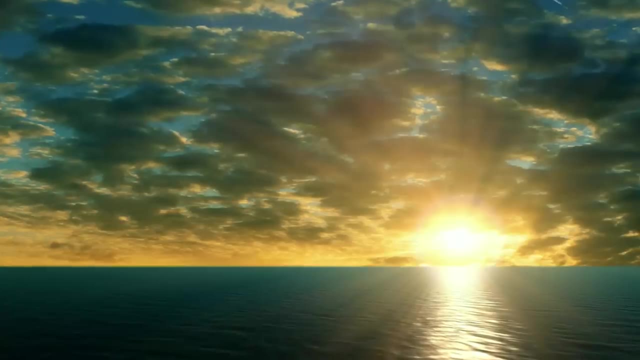 So let's dive into the Devonian. As I stated in the last episode, the Silurian was a pretty stable time in geologic and climactic terms. During the Devonian, Gondwana would remain as the largest landmass on the planet. 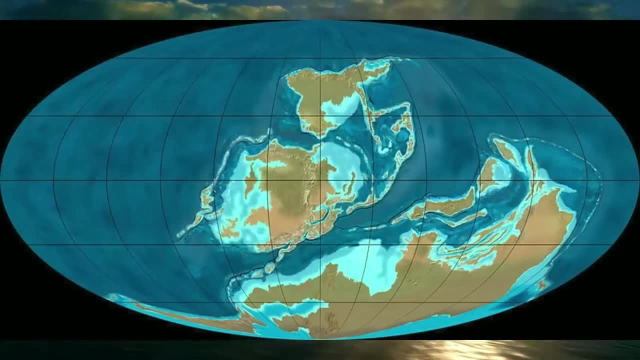 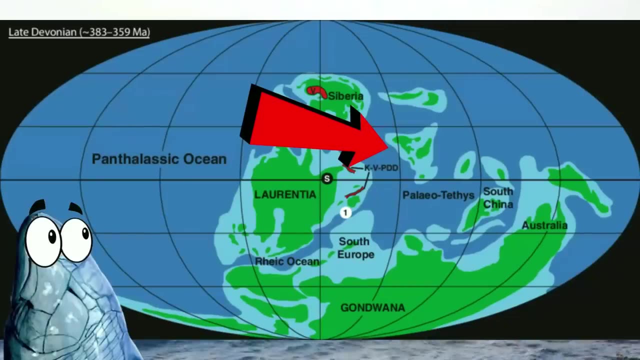 Over the 61 million years. it would start to move slightly northwestward, but still remaining entirely in the southern hemisphere. But several smaller landmasses had broken off of both Gondwana and Euramerica and kind of formed a closed-off seaway from the massive panthelassic ocean. 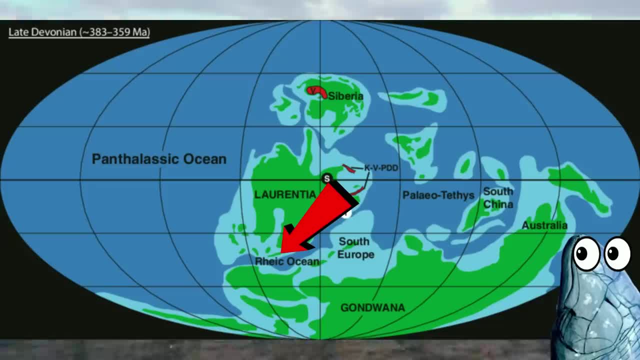 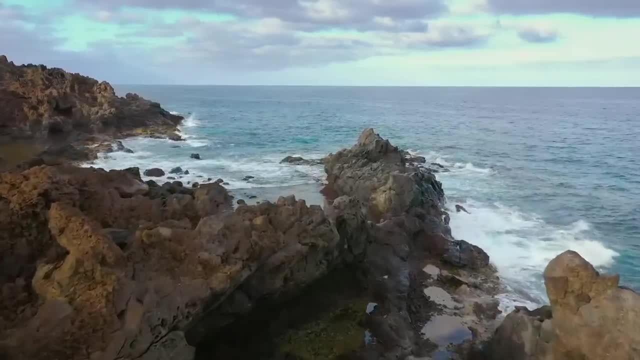 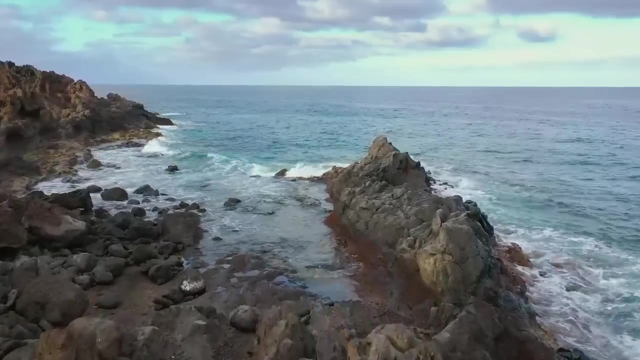 We call it the Paleotethis Sea, And it, along with a narrow seaway called the Raiake Ocean, would become the stage of a lot of noteworthy things that were about to start happening during this time. As far as the climate goes, the Devonian continued in a relatively warm trend. 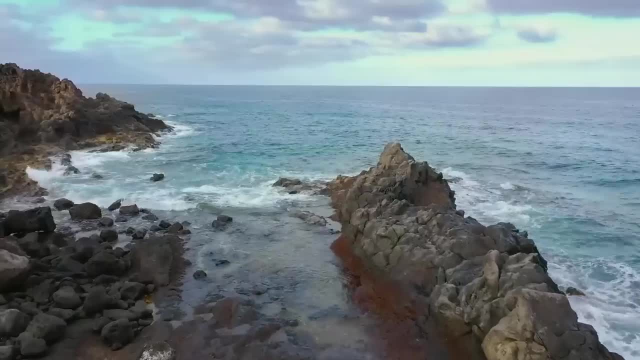 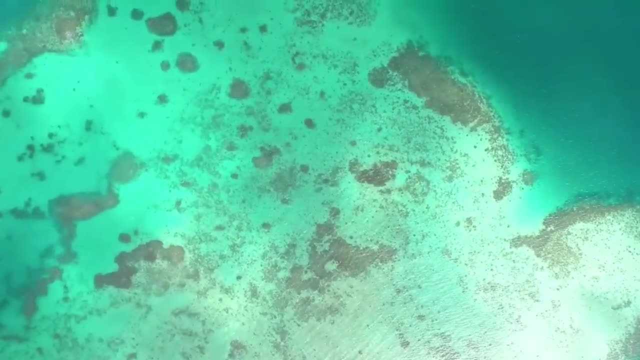 But there was a little more fluctuation than before. There probably was no ice at the poles, but because there was no ice, sea levels were very high, leading to an abundance of warm shallow marine habitats. This was something that had been slowly building up for a while. 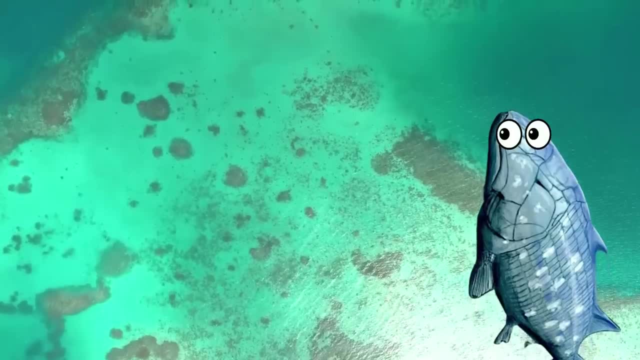 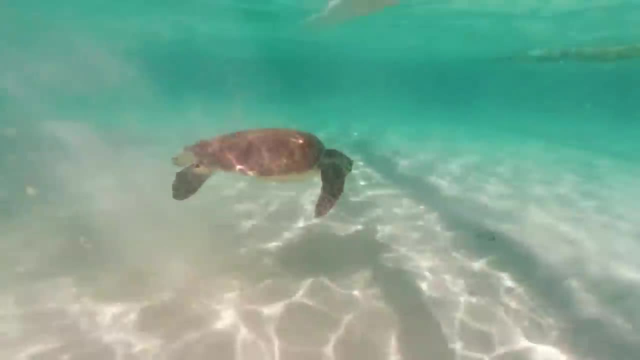 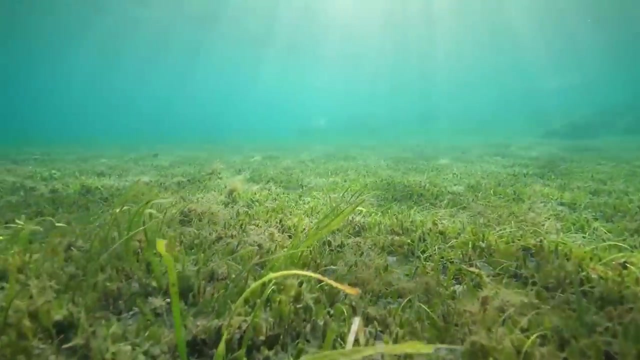 but with more and more shallow seas opening up, more different kinds of organisms can move in and adapt. In general, shallow seas are comparatively more productive than deep oceans because sunlight has an easier time penetrating shallow water. This allows photosynthetic organisms to spread. 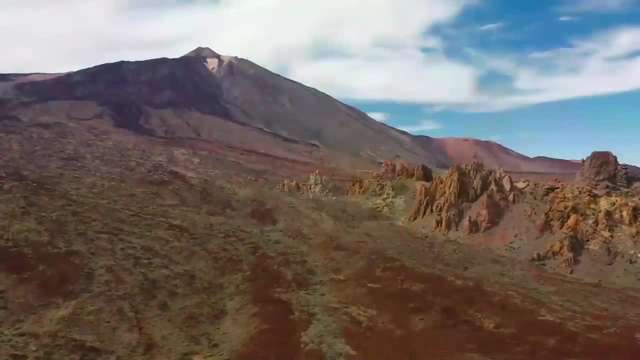 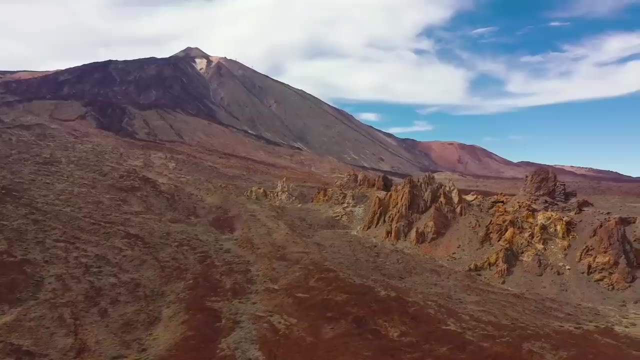 which makes up the base of any food web. We saw all that get started in the Silurian, but now, after so long with such stable conditions, many different groups were going to start struggling for dominance, And the ones that make the cut would be the ones that learned to take advantage. 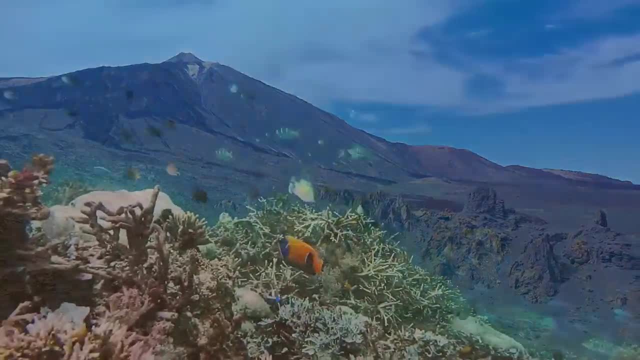 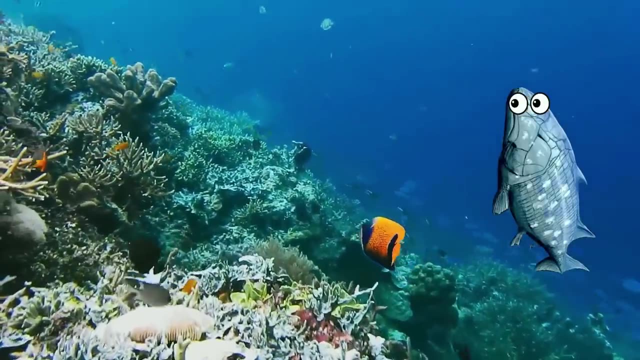 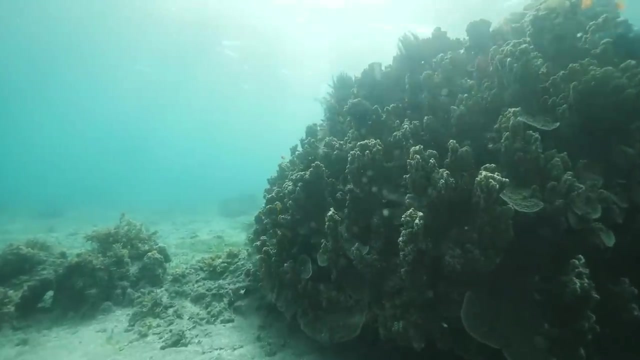 of the new biomes that were becoming available Today. coral reefs support countless different species of animals. They're basically the marine equivalent of tropical rainforests in terms of biodiversity, And corals have existed in some form ever since the Cambrian explosion. 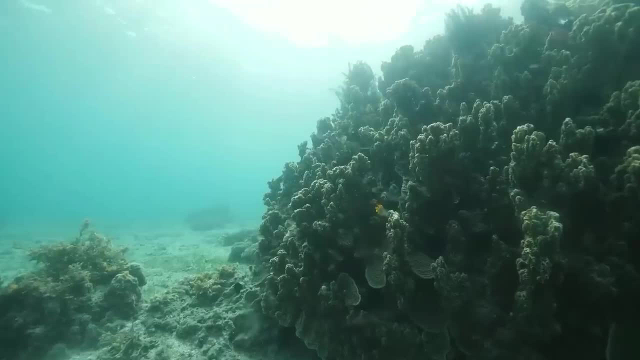 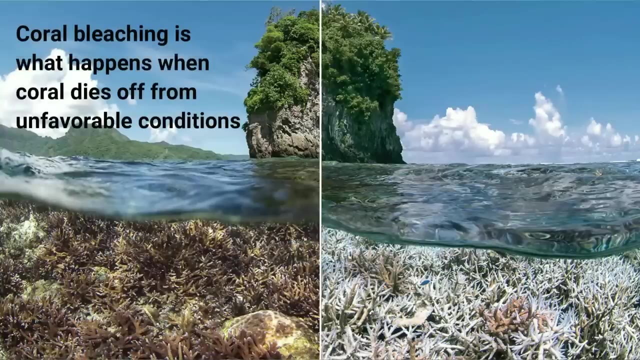 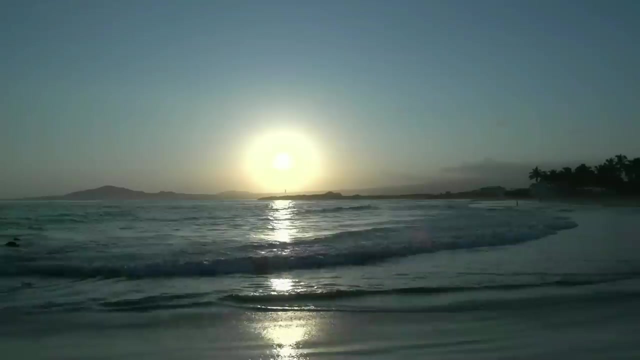 but they weren't building up the giant calcified structures that we would think of today, At least not yet. The thing about corals is they've always been really picky about things like ocean temperature and oxygen level and all that And throughout the Silurian and going into the Devonian. 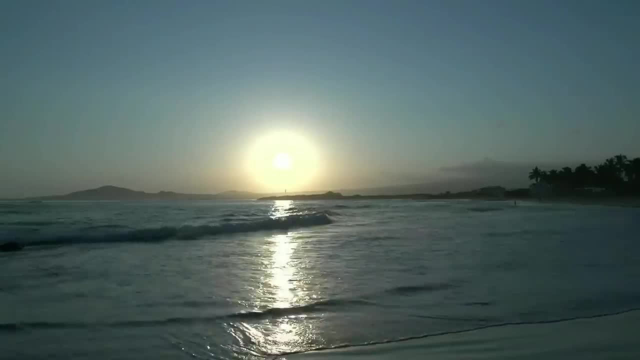 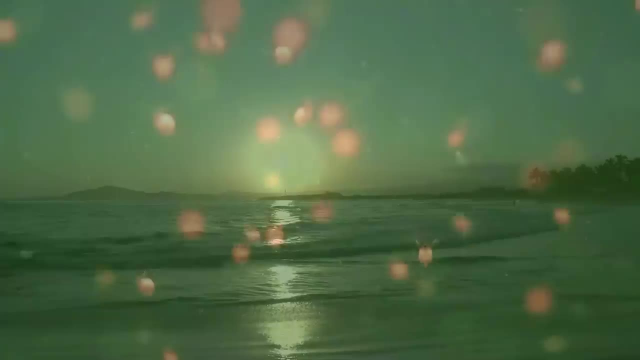 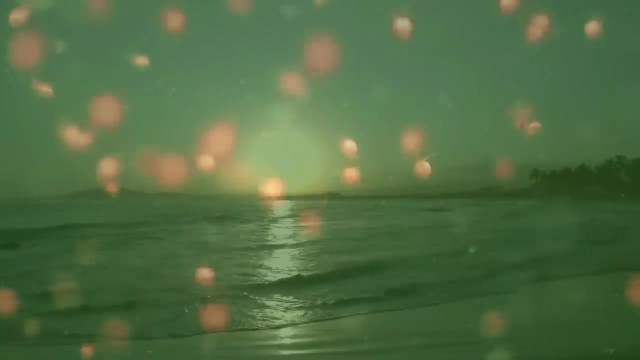 the water temperature was too warm for corals to spread into full-blown reefs, But there was another organism capable of forming reefs during this time. The very same things that have stuck around ever since the Archean: The cyanobacteria Ever since that now distant time. some species of goo had formed colonies and built up over time into structures called stromatolites. These would become the basis for some of the very first reefs and likely had been an ecosystem that benefited life for millions of years. But as we get into the Middle Devonian, the climate and ocean temperatures would drop slightly. Now it wasn't a lot, but it was enough to make a big difference for the rugose corals that were around at the time, Because, even though corals are picky once conditions are favorable. they spread much faster than the cyanobacteria can form stromatolites. So by the Middle Devonian we see a shift to the first large coral reefs that have been on Earth since they were largely wiped out by the Ordovician extinction. 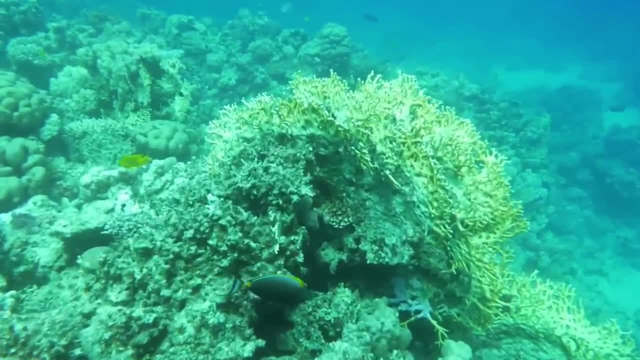 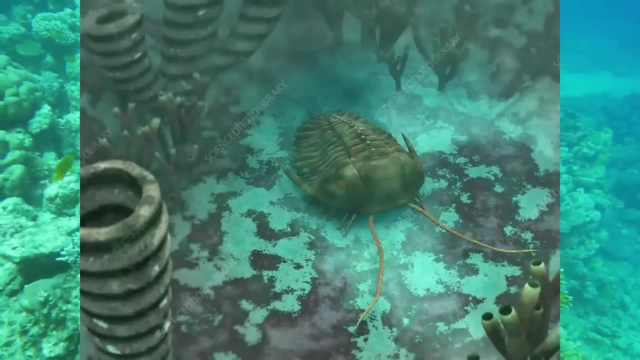 These reefs were populated by many creatures that we would consider familiar at this point in our journey, as well as a few new faces. The trilobites had fully recovered from their hit that they took at the end of the Ordovician as well. 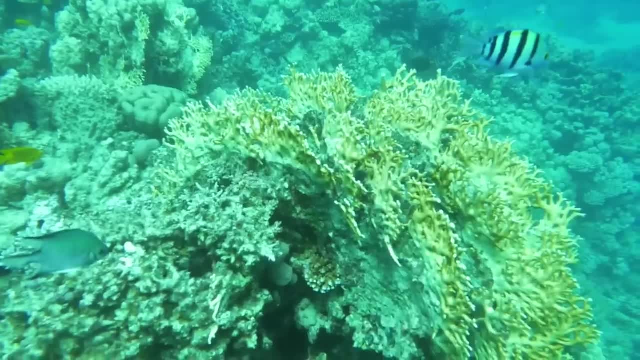 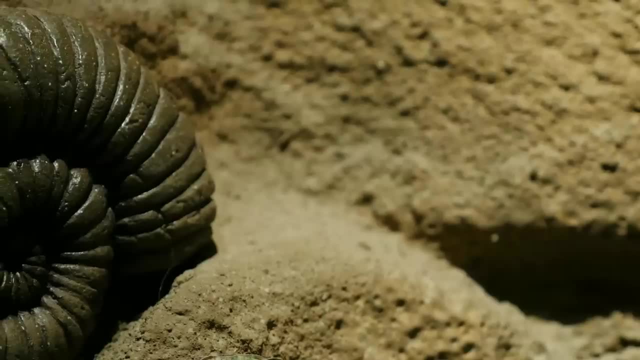 covering the sea floor like the invincible little troopers they are. But in the open water column a new group of animals was going to appear that was one day going to become an even more common piece of the fossil record than the indestructible pillbugs. 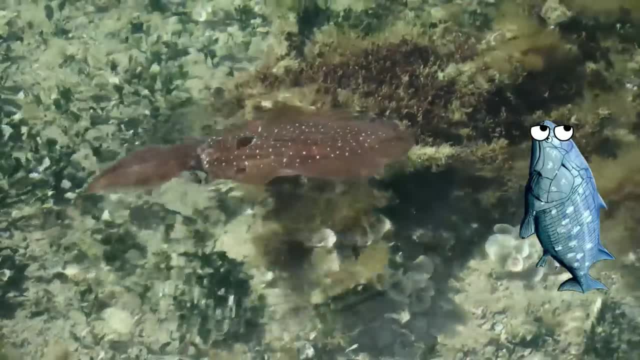 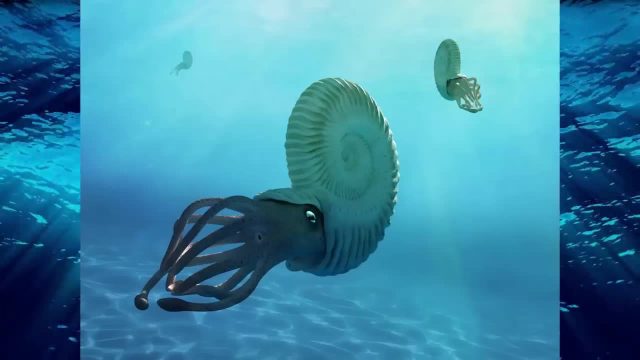 It would be coming from a group that famously doesn't fossilize very well. This is when the very first ammonites appeared. Ammonites are cephalopods, So these guys were distant descendants of the monstrous carrot krakens that ruled during the Ordovician. 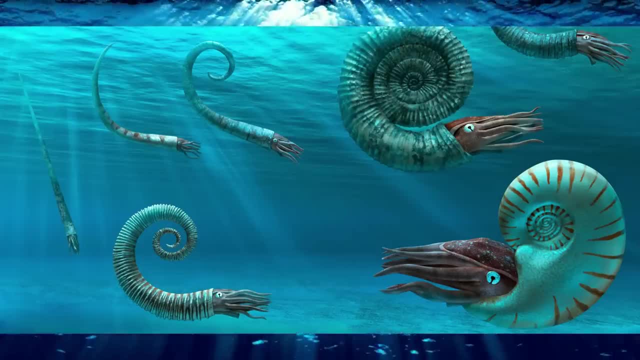 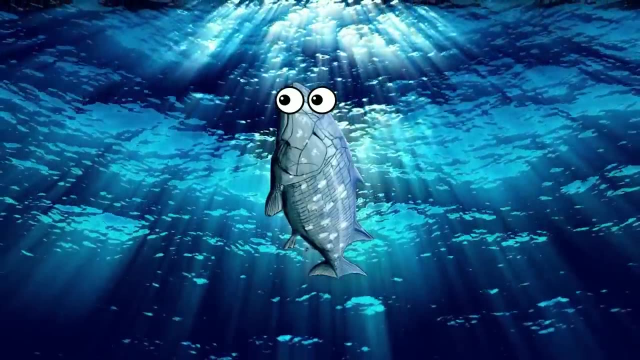 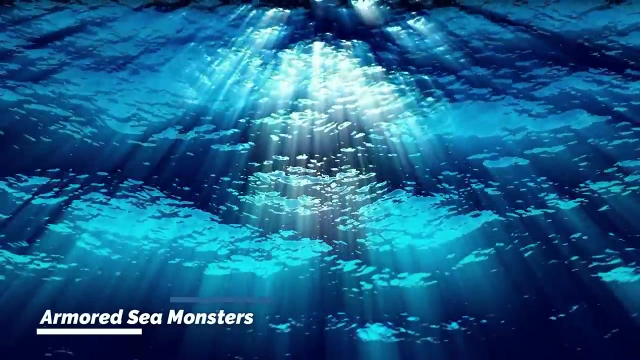 They were still carnivorous, like all other cephalopods, but it seems like the title of apex predator was not within their reach, Especially when you consider how much competition for that title was starting to ramp up Throughout the entire Silurian period. one group of animals was king. The eurypterids were still going strong by the beginning of the Devonian and environmentally there didn't seem to be very much to keep them down, But despite this we do see a steep drop off. 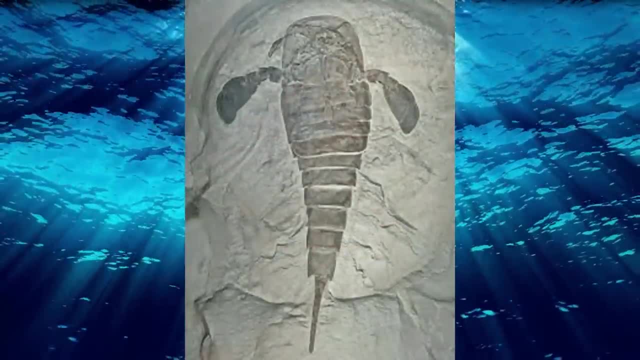 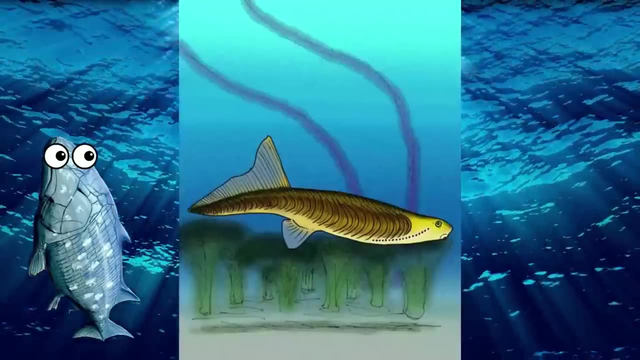 in the sea scorpion populations at this time. Scientists believe that this is because of new competition that would raise the stakes in the world's oceans. Up until now, jawless fish were the most common fish on Earth, But the vertebrates did manage to branch off. into a couple different variations, leading up to the Devonian, And that was all laying the groundwork for what was to come. It was now time for two groups to rise up and dethrone the arthropods. This is when the fish with skeletons. 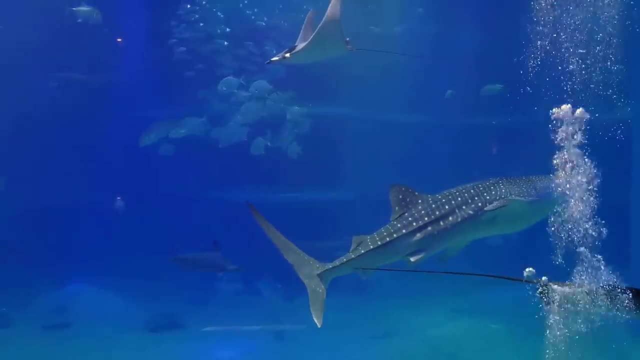 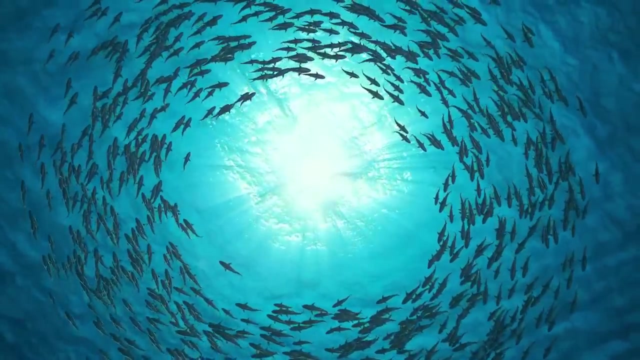 comprised of flexible cartilage, started to become more active predators, The very earliest sharks or cladodonts, And you would think that the first appearance of sharks would be a pretty big deal for marine ecosystems, But really they were kind of playing second fiddle. 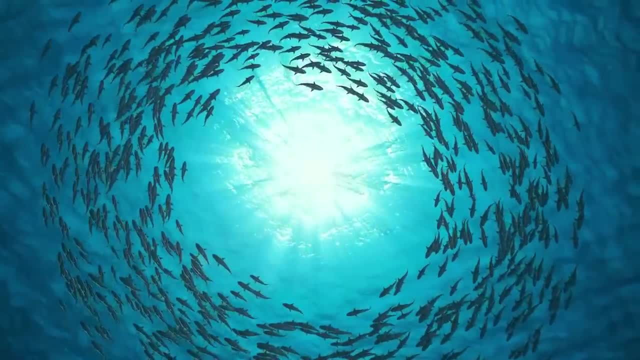 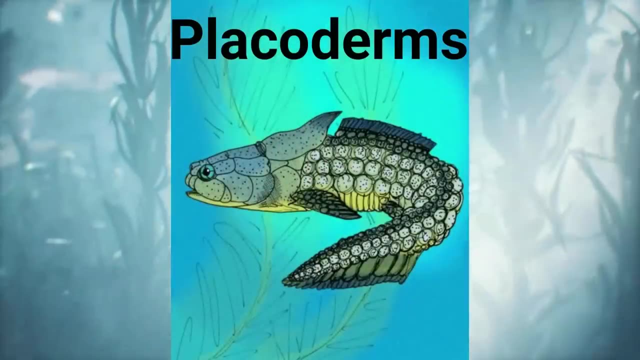 to the real monsters of this time, The second group of fish to rise up, the ones with bony armor on the outside. This group is called the placoderms and they are unlike any fish that we have today. They had jaws but technically no teeth. 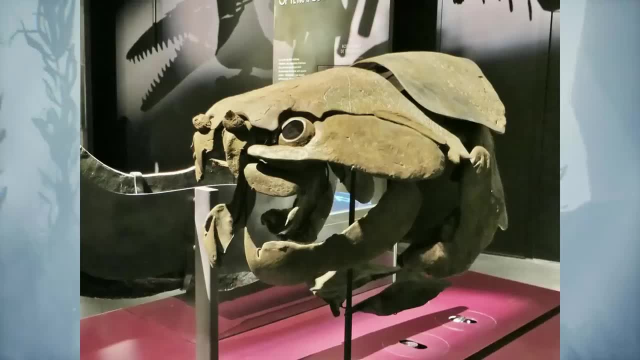 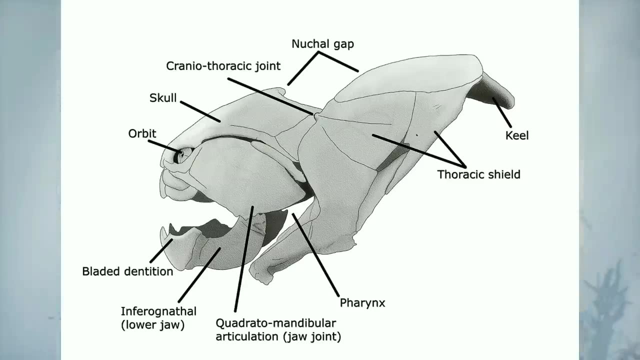 at least not in the same sense as you would think. Instead, the armored plates that made up the skulls formed a blade-like structure, sort of similar to a beak, And with these tools and defenses, this group of fish didn't just break out. as top predators, They started to explode into every possible niche they could. Even the smaller species were so defensive that the only things that could effectively feed on them were bigger placoderms. And that brings me to the thing that I know you all wanted me to talk about. 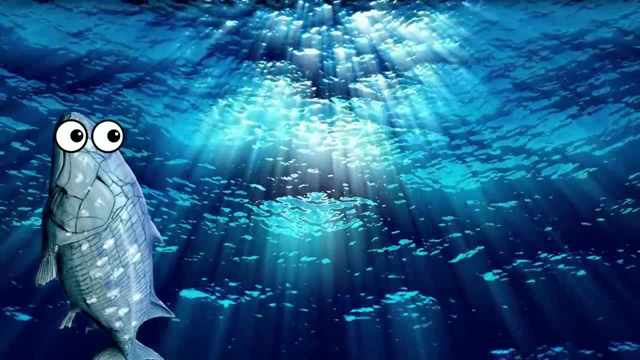 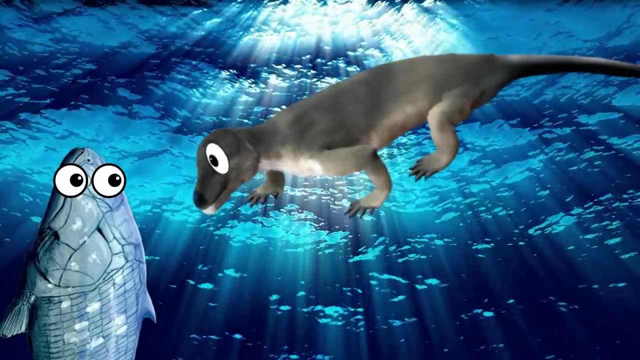 The biggest and baddest of the placoderms, Dunkleosteus, This nearly nine-meter, four-ton monster. Wait, Who are you? It's me, Tintin. Only I'm from the future and I came back to make a correction. 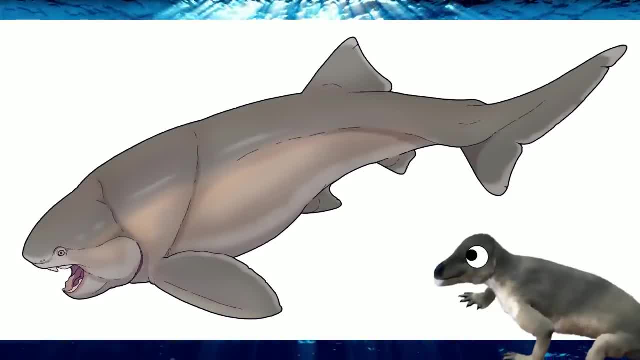 Because for years everyone has been depicting the guillotine-mouthed Dunkleosteus to look like this, with a kind of shark-like body measuring up to what'd you say nine meters. But the thing is, the only remains of this placoderm. 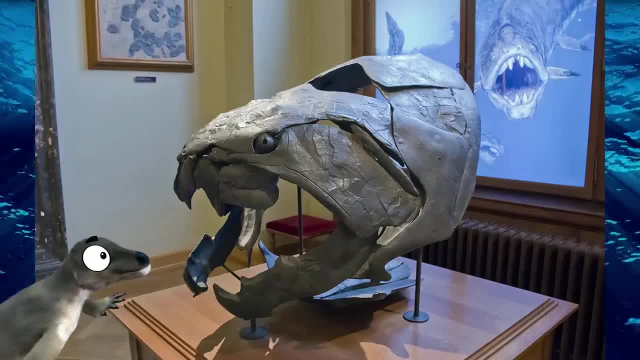 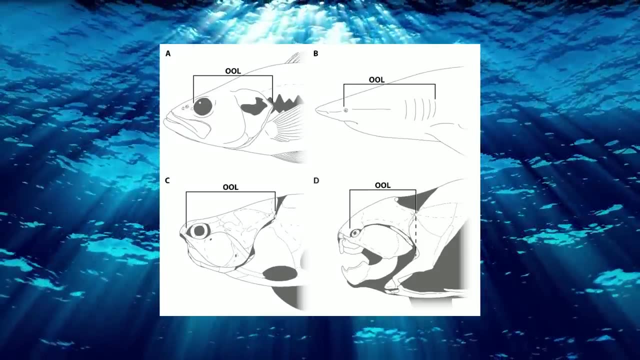 that have ever been found are just skulls and jaws, So for years this design was simply a guess, based on the body shapes that we knew of from more complete fish in this family, But recently new research has been done showing a direct correlation. 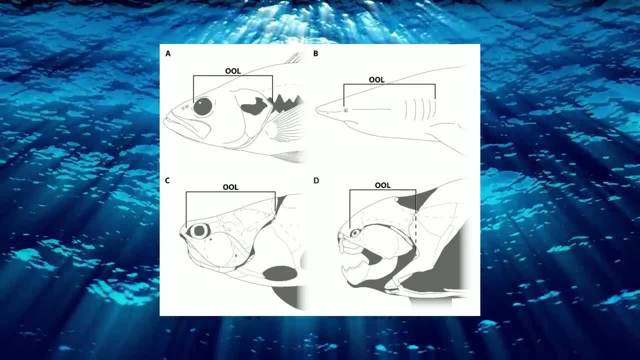 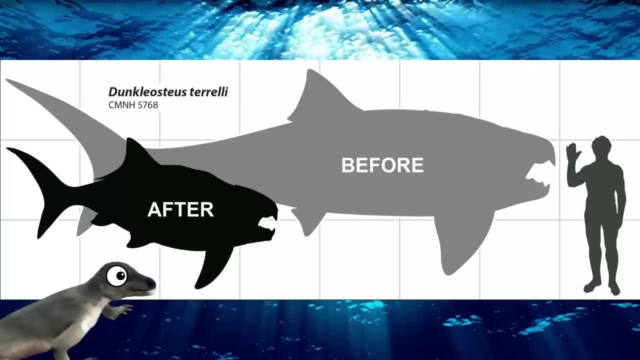 between the total body length and the measurement from the eye of the fish to the back of the gills. This metric has been tested and confirmed with every fish species that they've tried it on, living or extinct, And by this metric, Dunkleosteus probably measured. 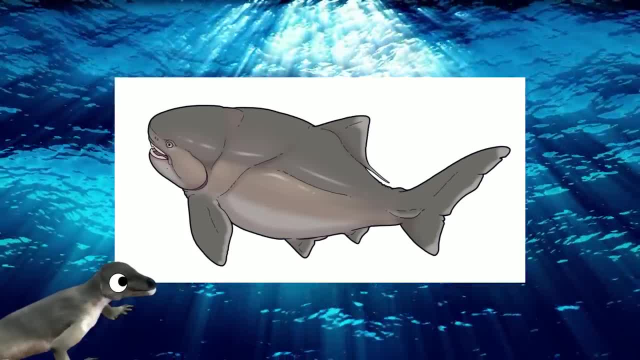 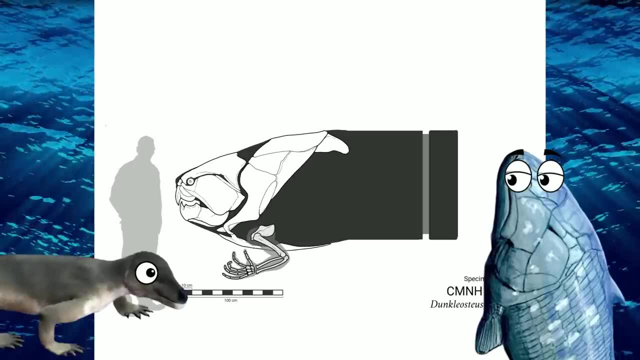 around half of what we previously thought. However, we still don't know exactly what its body looked like. It could have looked like this or like this, but personally, my vote is that it probably looked like this. Well, I see, Tim Tim's still an idiot in the future. 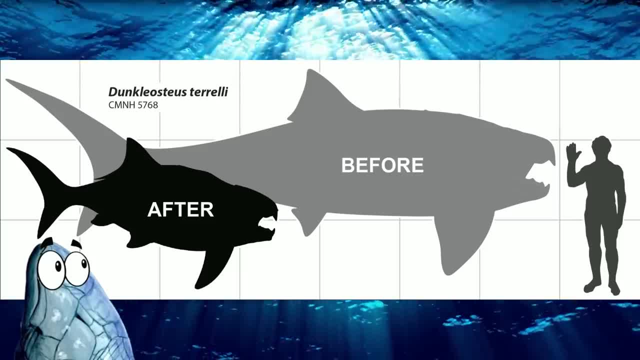 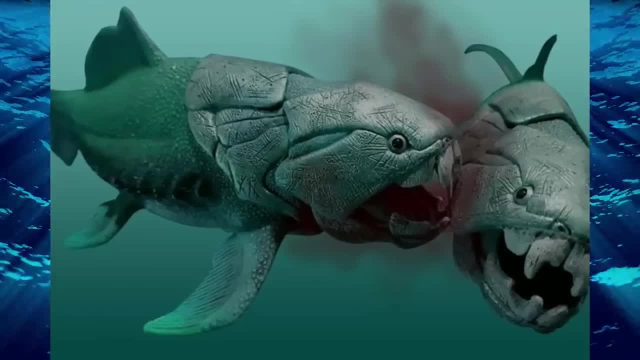 But either way, even at this reduced size, Dunkleosteus still would have been the top predator of the Devonian Seas. Its bite force was focused into the front of the fang tips and measured 80,000 PSI. I actually had to double check this. 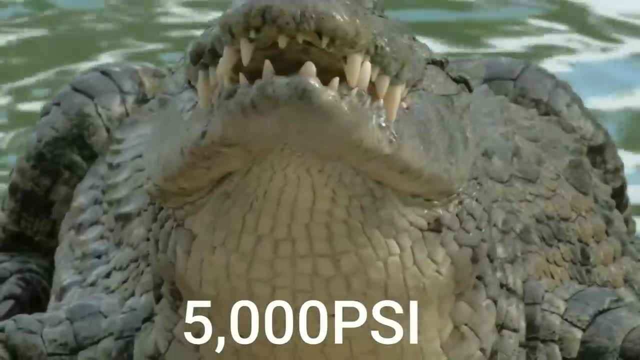 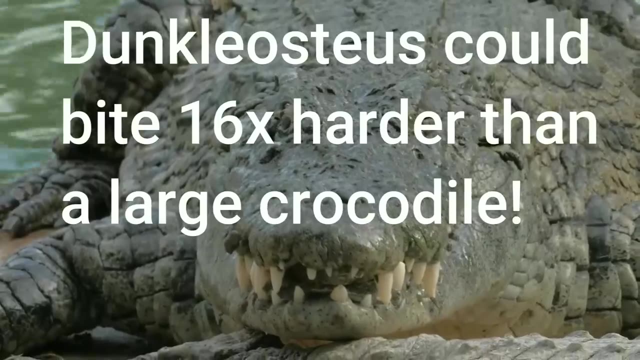 For context, the maximum estimated bite force of a Nile crocodile is around 5,000 PSI, So this thing could bite 16 times harder than a large crocodile, And it basically had a guillotine in its mouth With this thing at the top. 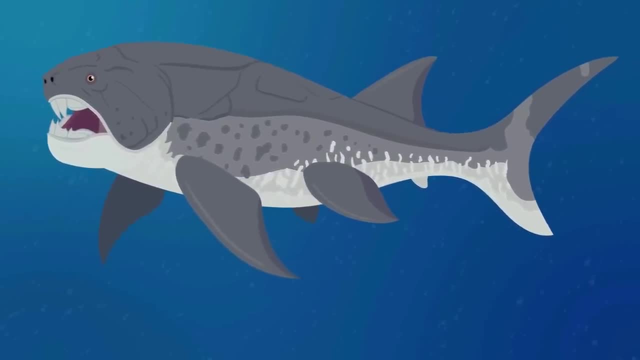 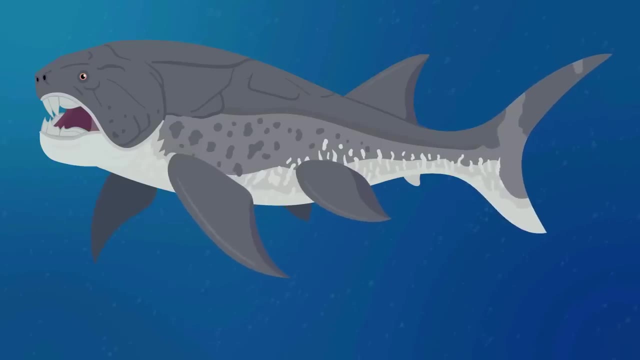 of the food chain. there really is no wonder why there was a sudden turn to more defensive forms. Arthropods were armored like the placoderms, but the way these new fish predators were armored in the front, with powerful muscled tails in the back and a flexible spine. 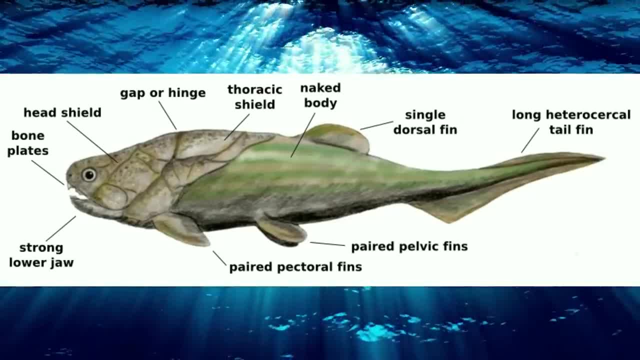 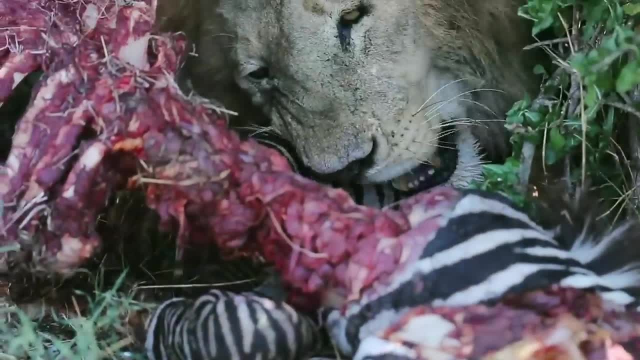 they were doing everything we had seen in other parts of the animal kingdom, only better. And since predators drive the evolution of prey by removing the individuals who don't cut it from the population, everything else on Earth was starting to evolve into the placoderms' world. 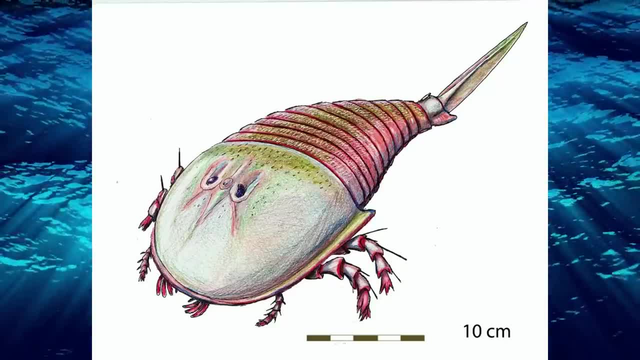 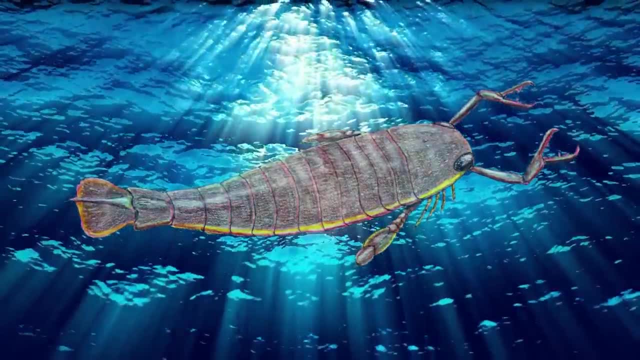 The Styloneuria sea scorpions would manage to hold on by not competing directly, But unfortunately the Erypterina sea scorpions were just going to fall victim to this power shift. It seems like if you couldn't keep up, 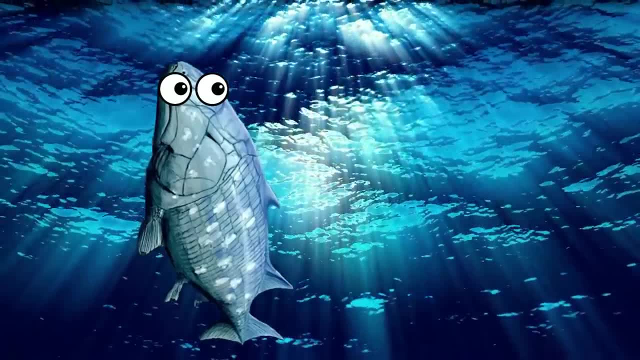 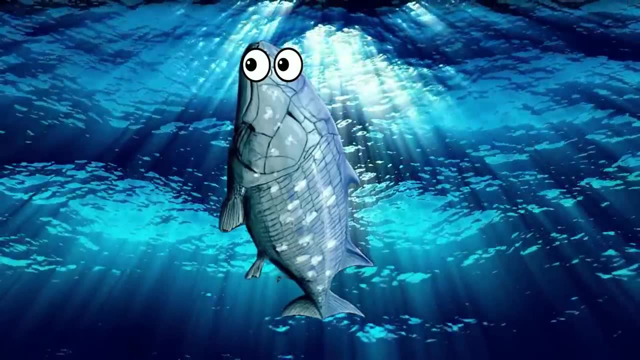 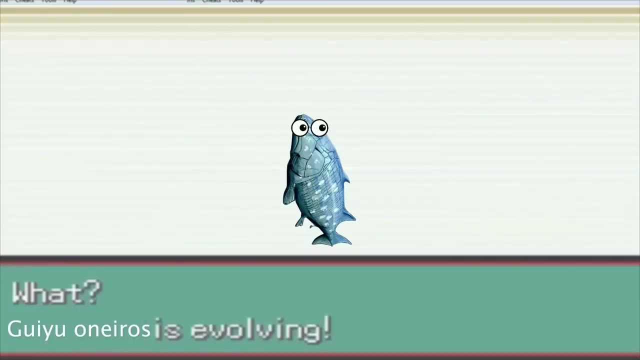 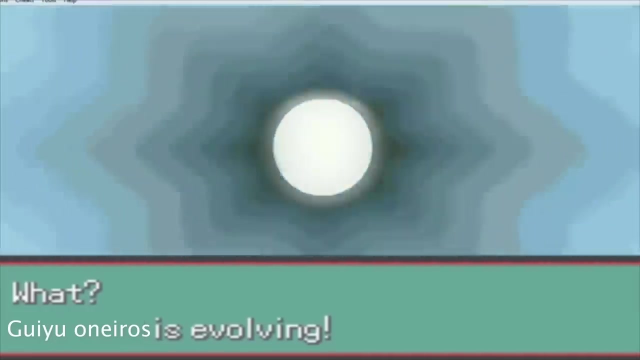 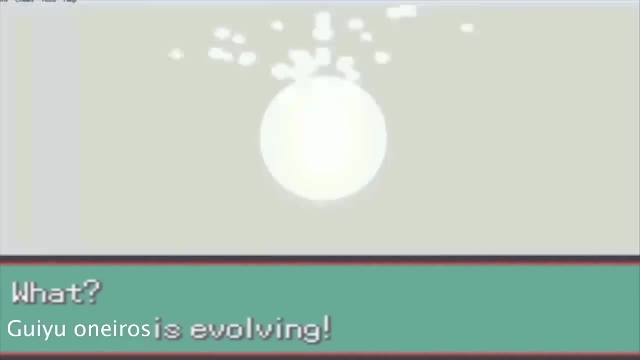 the best survival strategy was to get away and avoid the armored fish at all costs, And it would be this pressure that drives one of the most momentous events in the history of life on Earth. One small step for fish, One giant leap for vertebrate kind. 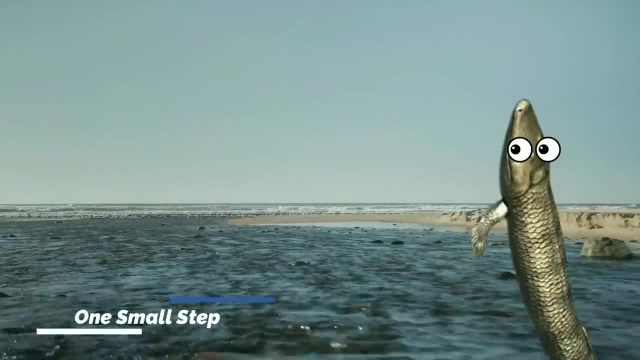 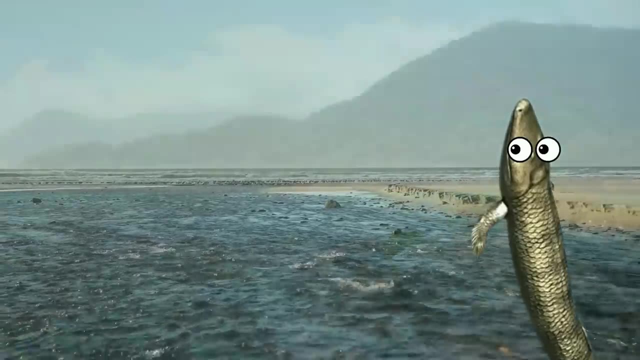 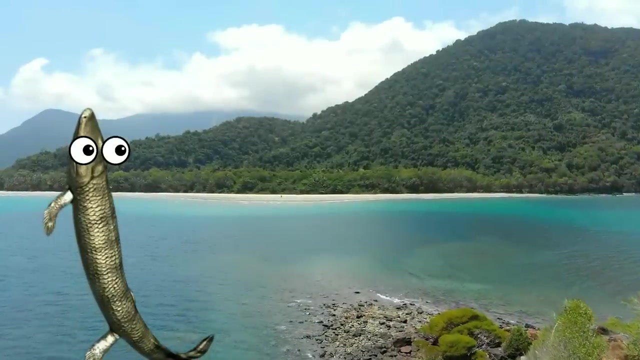 With life in the oceans becoming so dangerous, it's not surprising to think that if there was an alternative available, some organisms were going to go for it. And meanwhile, on land, as more complex rooted plants started to evolve, this allowed soils to stabilize. 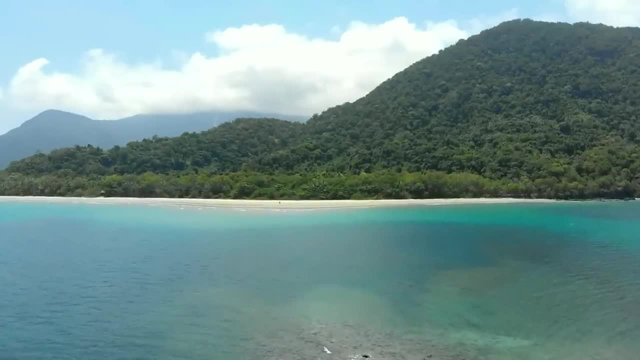 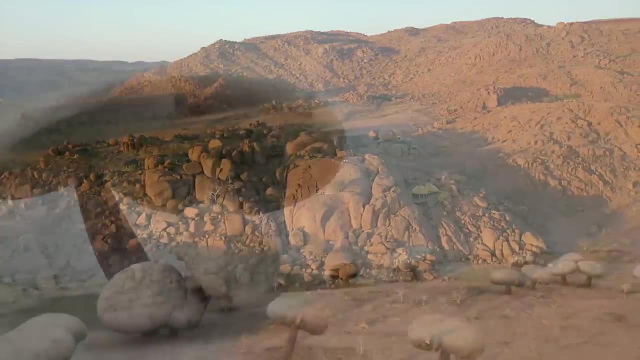 for the first time And the plants started to grow larger. This would change the dynamic of terrestrial ecosystems forever. Previously in the Silurian, the giant fungus like Prototaxidides were the largest things on land. But as the Devonian went on, they started to slowly get replaced by the very first large plants. It's unknown exactly why the fungal trees were failing while large plants were managing to survive, But one theory is that plants were better equipped to defend against being preyed on by arthropods. 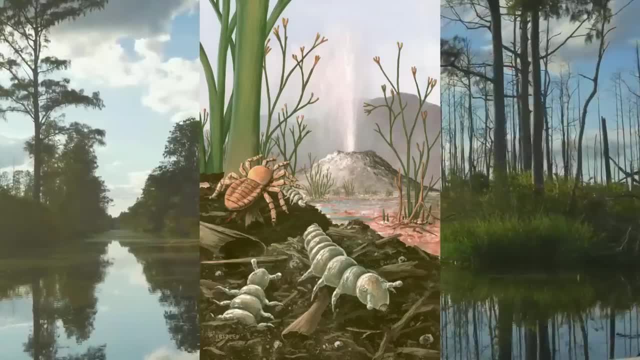 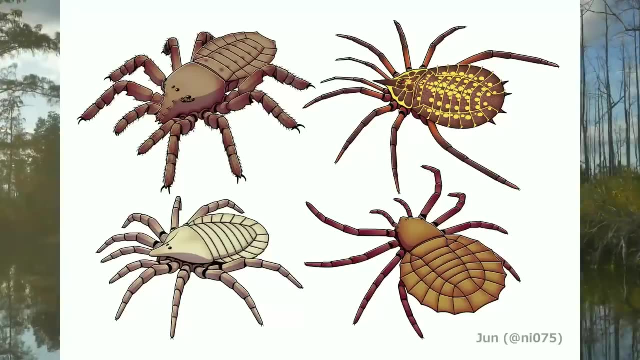 which there was starting to become a considerable variety. Things like centipedes and millipedes were common and the arachnids like true scorpions, mites and a strange group that looked like a cross between a tick or a mite. 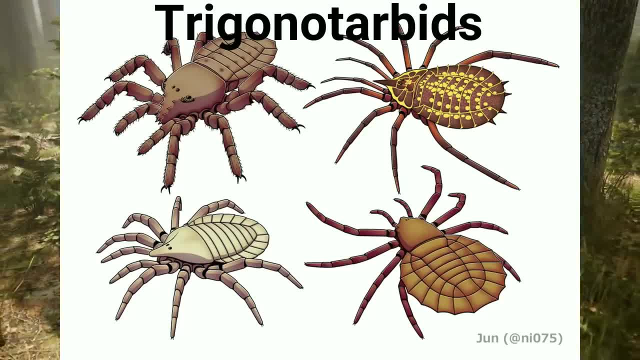 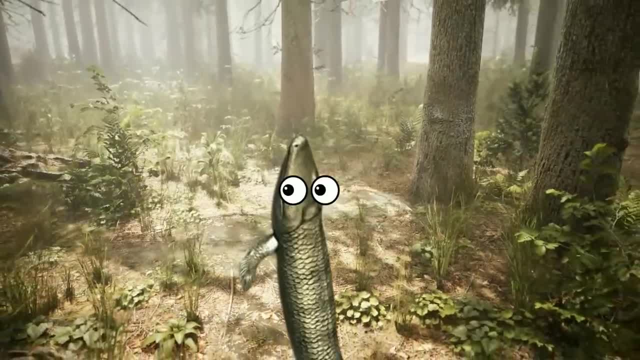 and a spider called the trigonotarbids had begun to diversify Throughout the Silurian. the invertebrates were left unchallenged on the land, But now it was time for that to change, As the plants spread across the land. 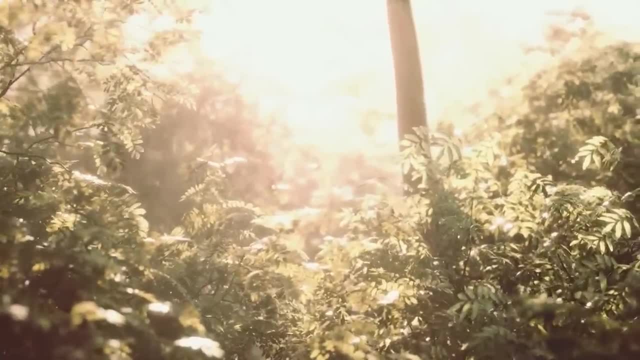 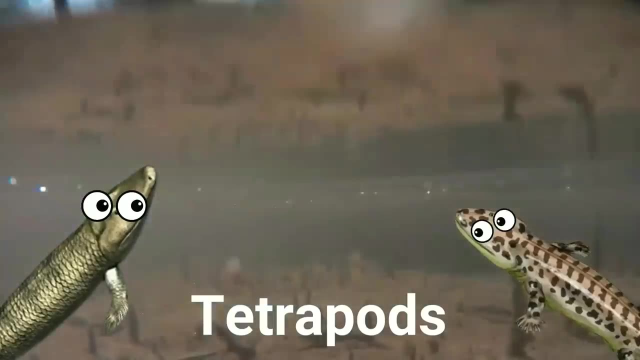 even far away from waterways along the coasts, you would find the very first vertebrates making the leap onto land, the tetrapods. I has feets. They evolved from the lobe-finned fish. that, to be honest. 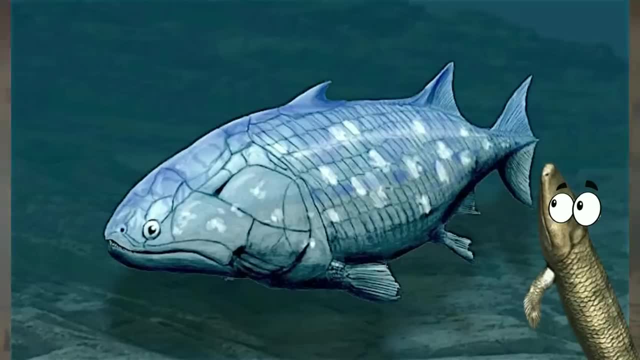 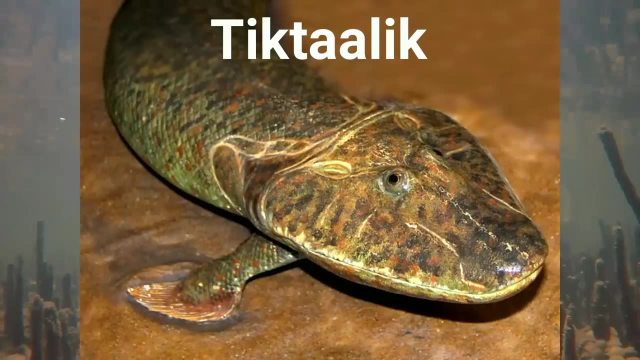 were struggling just as much to deal with the armored fish as well everything else, But this would give them the chance to survive. Now, this might seem like very humble beginnings, and well it is. These things were basically something between: 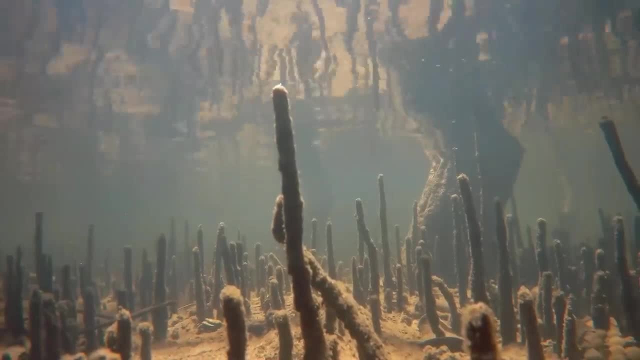 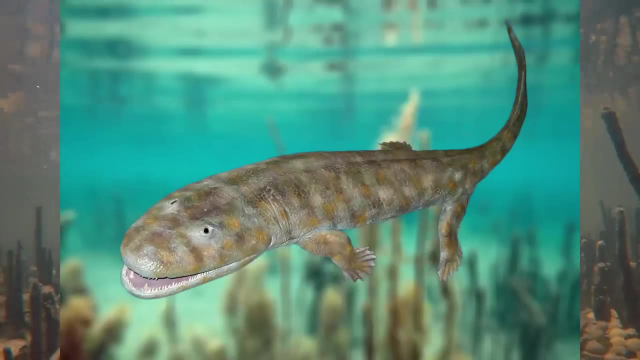 a salamander and a mudskipper, But their success is undeniable. Different species started popping up all over the Devonian world Using their limbs that were still something in between fins and feet, which in different species like Tiktaalik and Archaeostega. 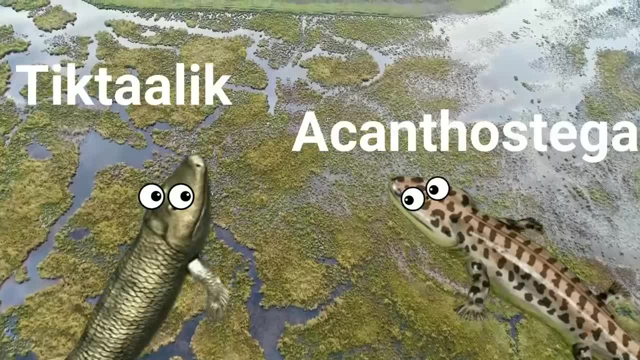 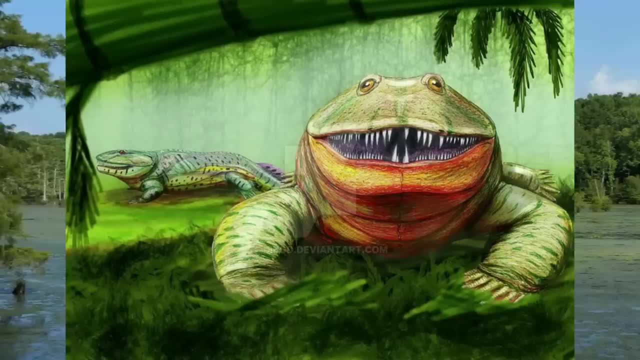 had eight digits on each, they were able to haul themselves up out of the reach of the placoderms, And in this new world they would likely become predators With eyes positioned on the top of their heads and sharp, needle-like teeth. 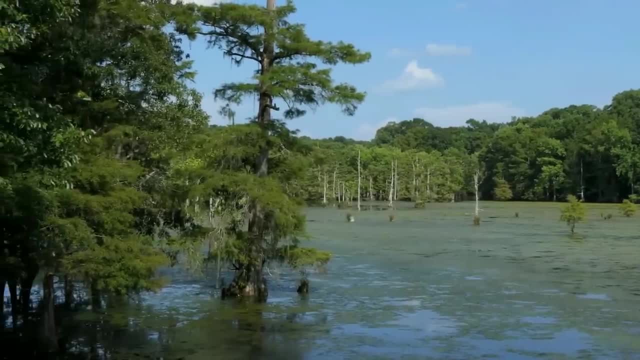 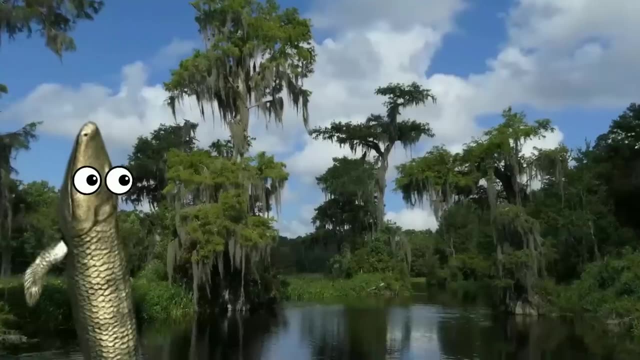 it's thought that they were the very first animals to make use of the ambush-hunting at the water's edge strategy that we would see many times in the future. These animals are a big deal to our understanding of life, because every single organism that lives today 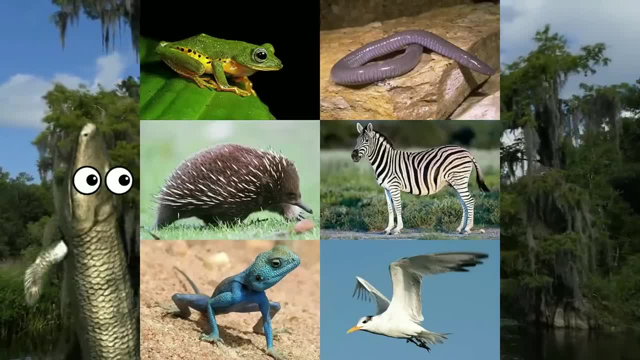 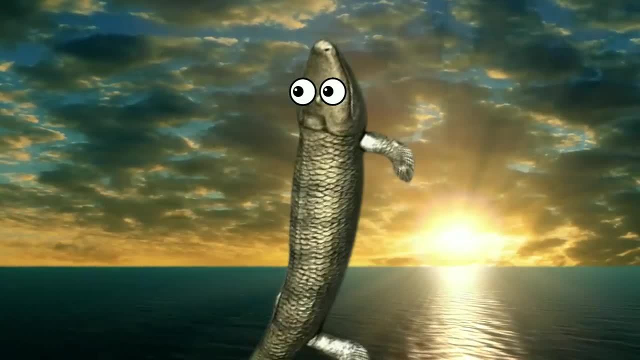 and has a backbone and lives on land, can trace their ancestry to the pioneering creatures of this time, Although they were still tied to the water, especially to reproduce. this was the blueprint of things to come, And it was lucky that we made this leap. 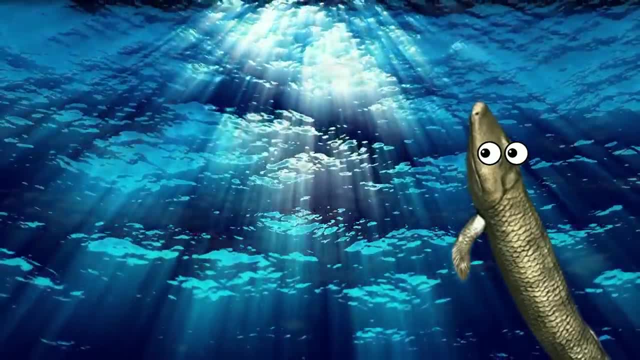 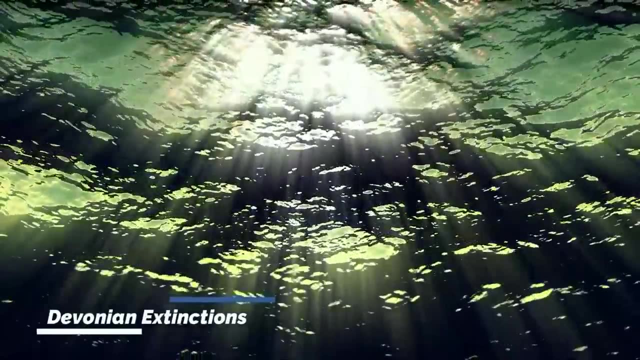 when we did, Because, as we come to the end of the Devonian, the world's oceans were about to hit hard times once again. The late Devonian extinction is not very well understood. A few things we can say, however, is one. 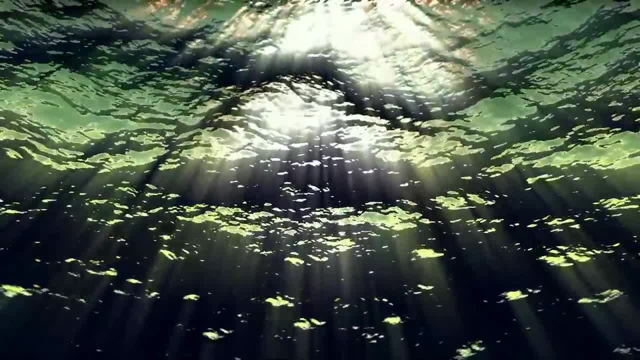 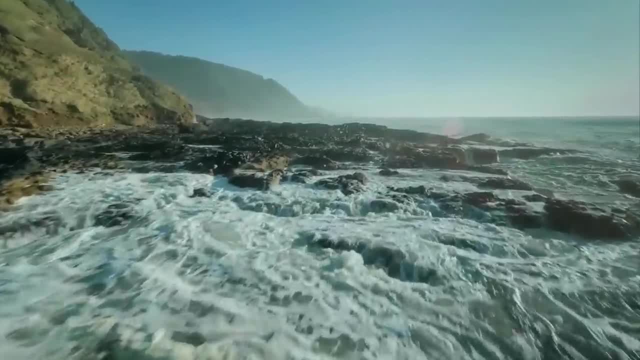 it doesn't appear to have been a single event, but rather multiple events that caused it. And two, the effects were much more severe in the oceans than on land or in freshwater ecosystems. One theory is that an asteroid impact may have been to blame. 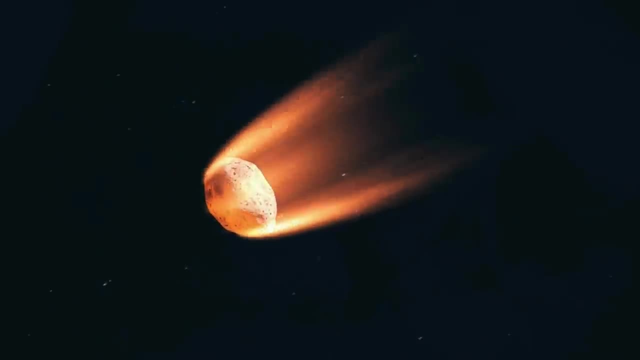 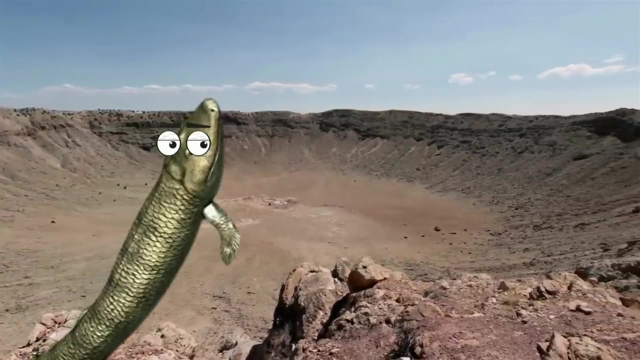 for part of it, but to many scientists this doesn't really check out. For one thing, so far there's been no impact site found, But that doesn't really matter because 350 million years has passed since then and there wouldn't be that much of a crater. 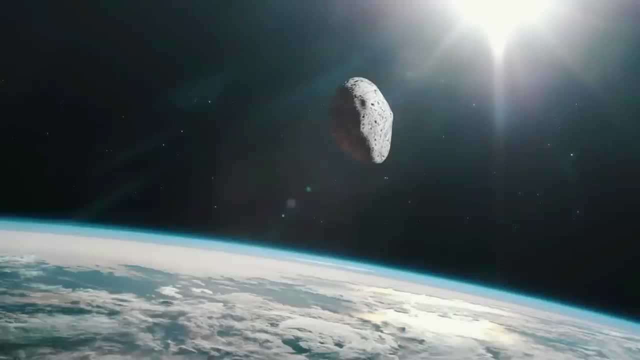 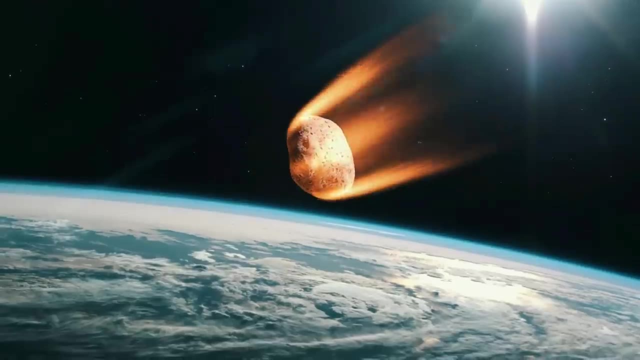 with that much time to erode. But the fact is that an asteroid impact would have equal effect on both land and sea, so most people think that it must have been an event that was specific to the oceans. The most popular theory is that something 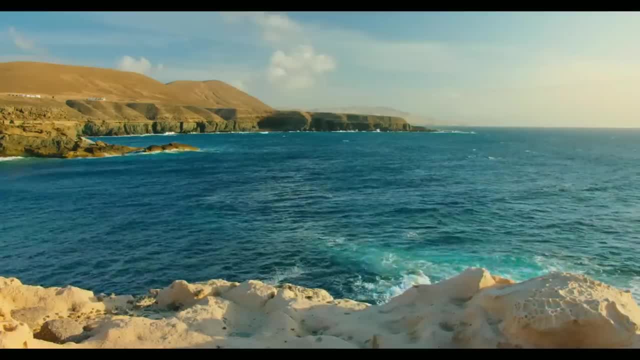 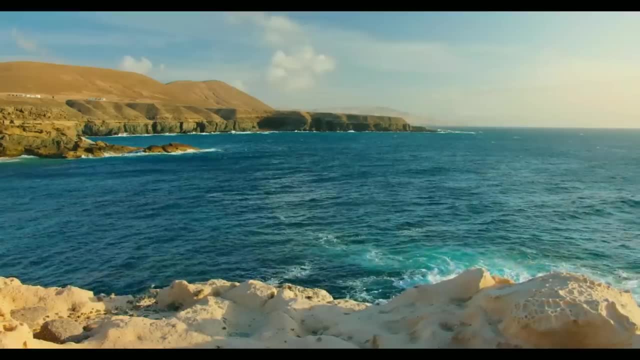 caused the oxygen levels in the oceans to plummet. This would have an adverse effect on many of the different groups that rose to dominance over this 61 million year period, But the fact is that there was no impact site to this 61 million year period. 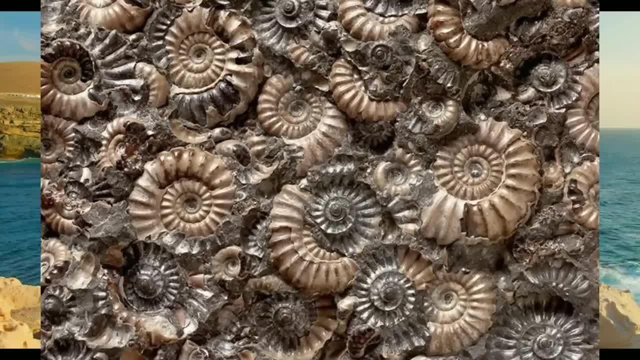 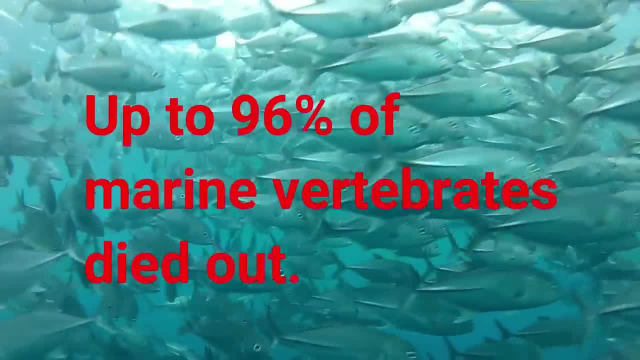 Brachiopods, trilobites and ammonites would all be hit hard by this, but they would pull through. But the worst effects were to the marine vertebrates. As much as 96% of them were wiped out in the last few million years. 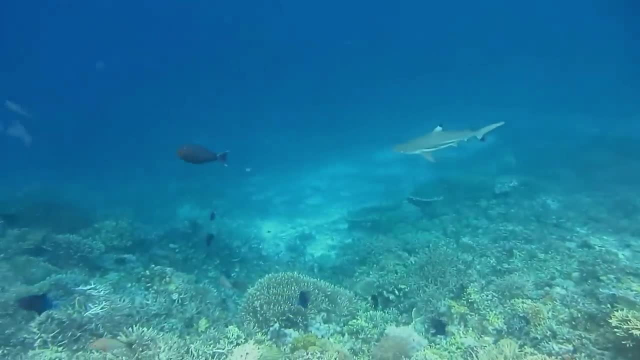 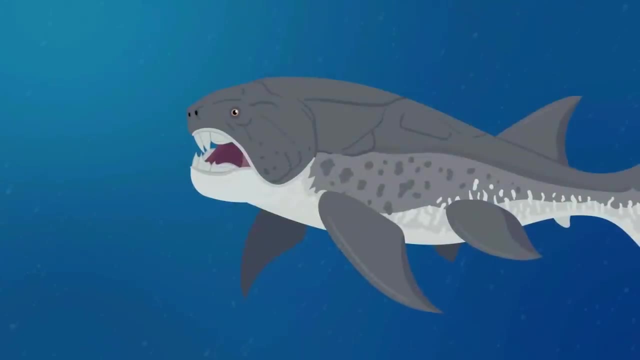 of the Devonian, The bony and cartilagelous fish managed to hang on, but unfortunately the armored placoderms were not so lucky. These animals were extremely well adapted to be the kings of the oceans And they were the first vertebrates. 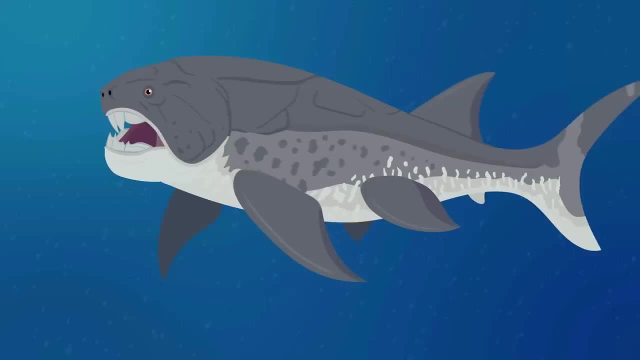 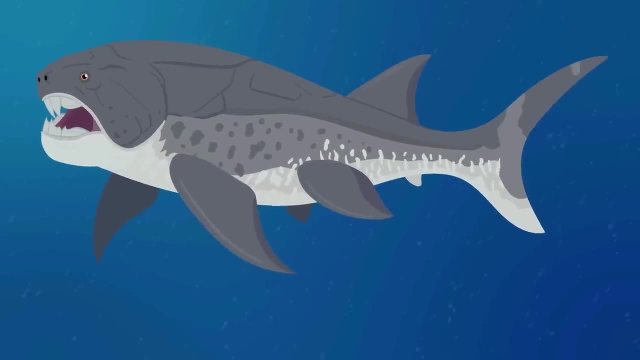 to take control away from the inverts And, although their rule was short, when you look at the total story of life on Earth, it showed for the first time that the body plan of an internal skeleton is not inherently inferior to an exoskeleton. 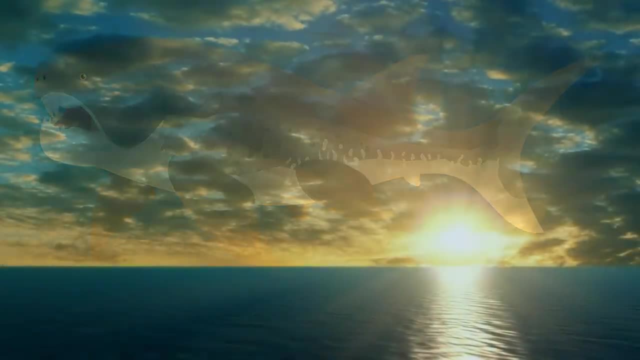 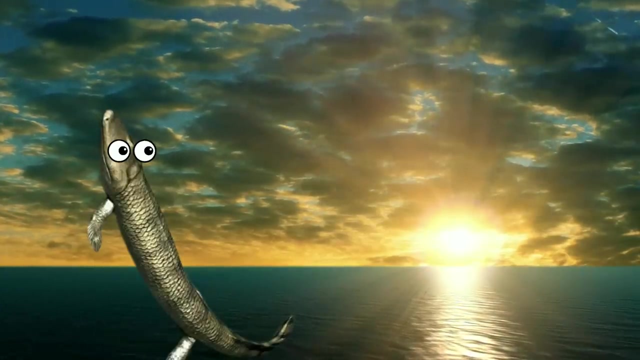 But once again it also shows that whenever a catastrophic change in the world takes place, it's the ones on top that have the most to lose. Whenever there's a major ecosystem collapse, the animals at the top of the food chain are normally the ones. 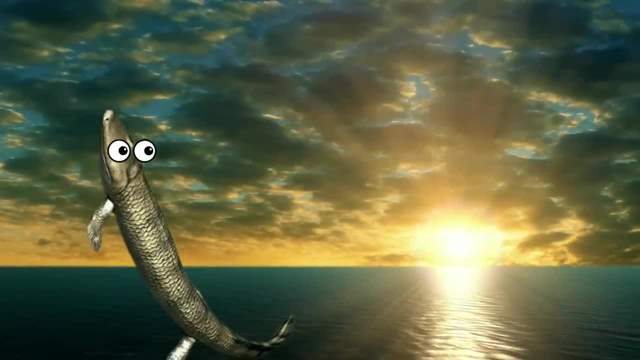 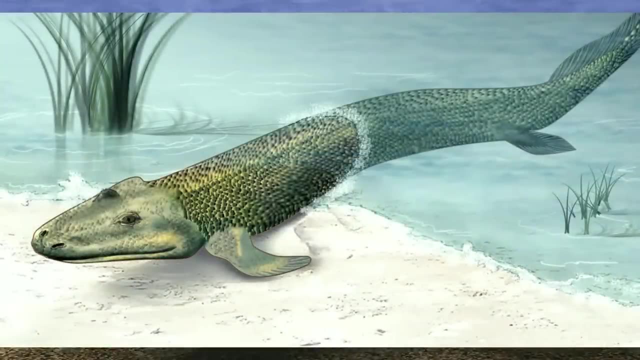 that are going to struggle the most to get what they need to survive. Whatever the cause of the die-off, at the end of the Devonian, our direct ancestors, like Tiktaalik, were relatively unaffected, In fact, as this period came to a close. 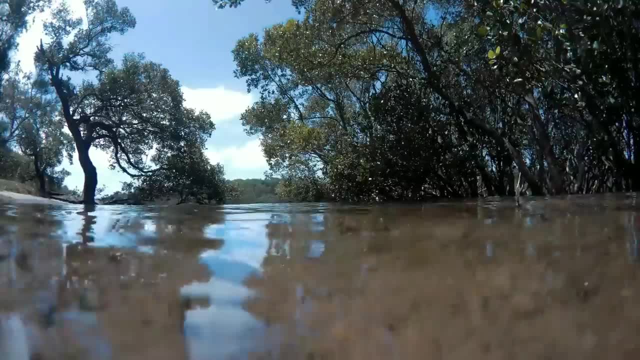 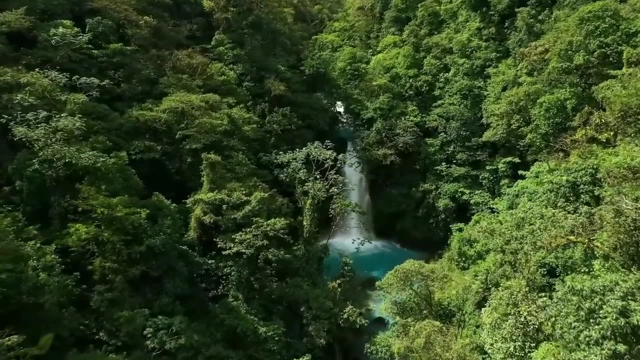 they were actually becoming more abundant than ever, And now the land was growing even more hospitable and trees started to spread across the globe and eventually, from pole to pole would be covered in an endless tropical forest, And that would be the stage for the next chapter. 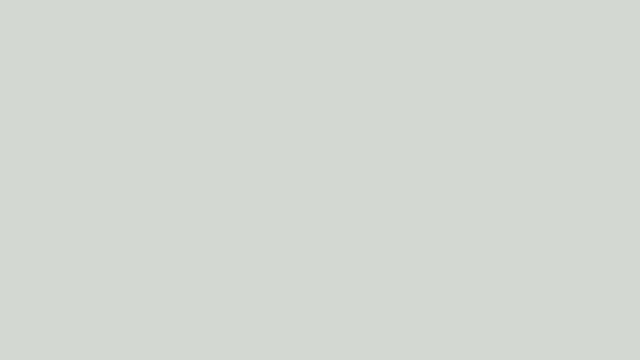 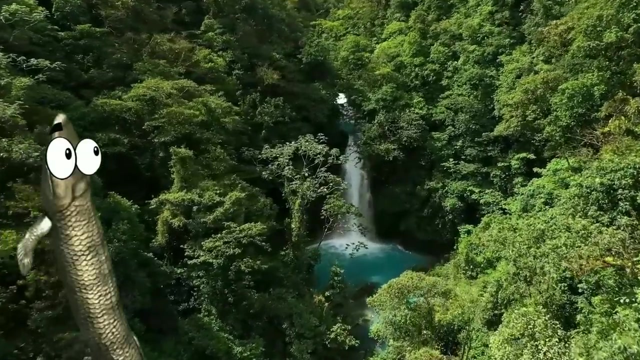 in the Odyssey of Life. So, getting back to our journey through time, the state of life at the end of the Devonian was very different depending on where you were standing. If you were one of the pioneers of the land, the world was pretty nice. 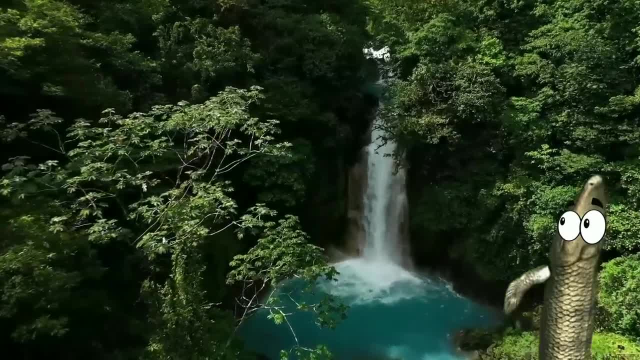 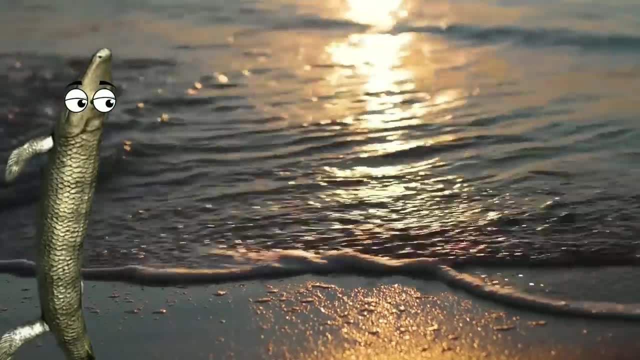 Forests were spreading out from the rivers and marshes, and there was getting to be more and more opportunity here all the time. But if you lived exclusively in the ocean, well, you're probably lucky to be alive. The world's oceans had been hit. 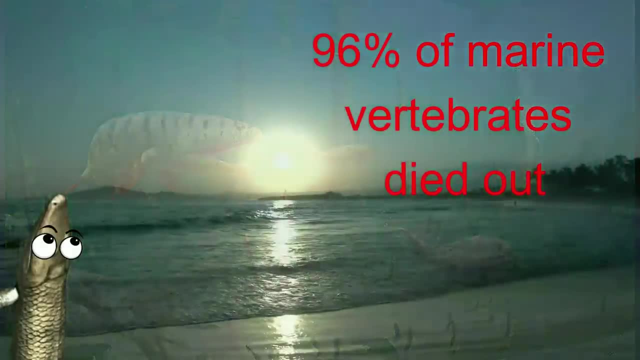 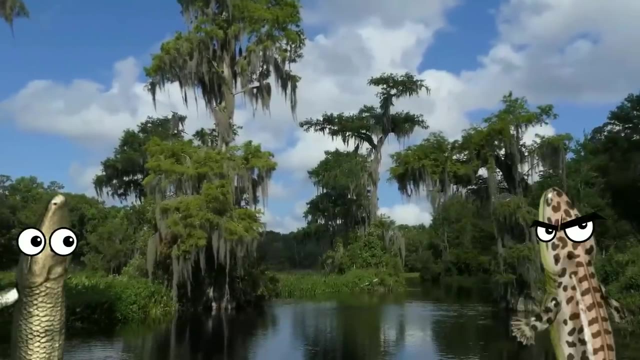 by a mass extinction that only left around 4% of the animals that were thriving previously. But the land didn't seem to be having these issues. I say good riddance. Well, that's rude. Everything keeps trying to eat me. 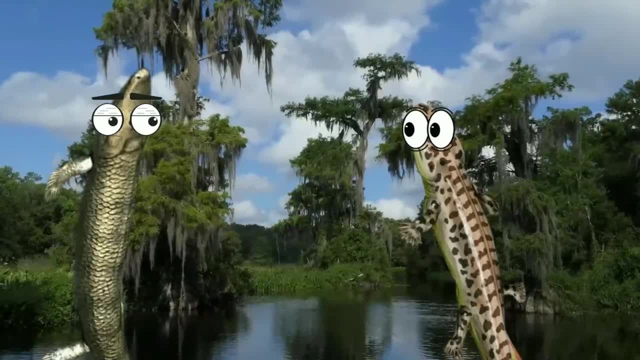 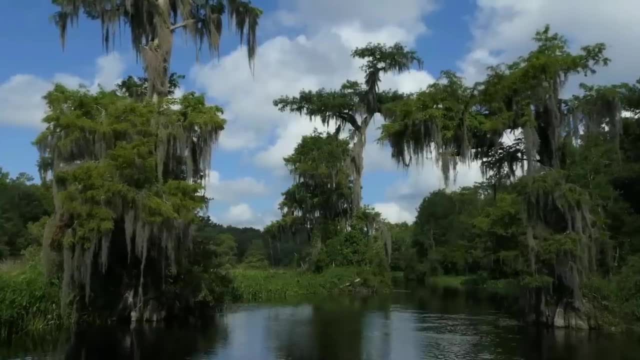 You think that's gonna stop just because we're on land? Uh, So, basically, as we go into the Carboniferous, there was once again a power vacuum in both the marine and terrestrial environments all over the world, for two totally different reasons. In the ocean, life was bouncing back from the death of the armored fish and many other dominant groups. And on land, the spread of the massive global forest would open up new opportunities for those who were able to adapt. This forest would become so all-encompassing. 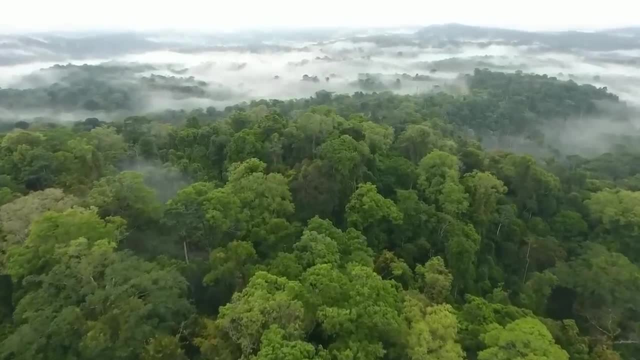 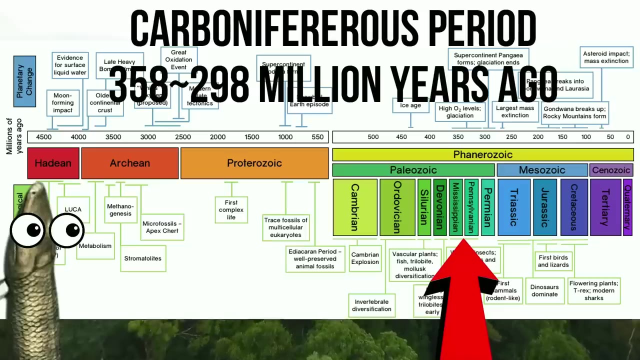 that not only would it have a very unique effect on our planet and its inhabitants at this time, but it would even affect our modern world in a critical way, Which is wild to think about, considering this period began 358 million years ago. I've been looking forward. 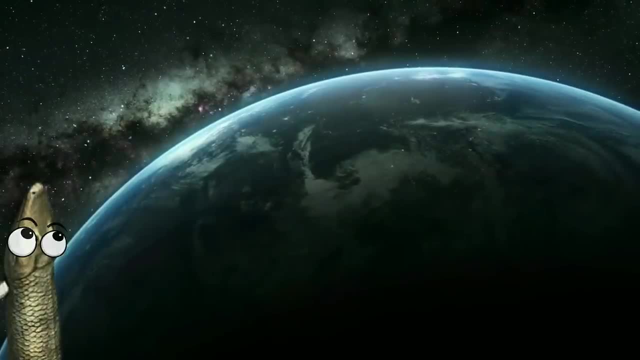 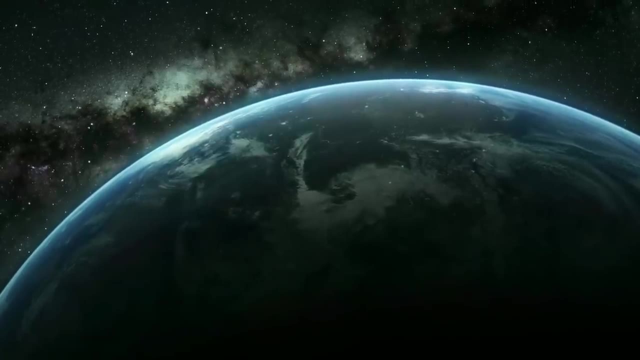 to this one. so let's dive into the Carboniferous jungles. During the Carboniferous, the world was undergoing more drastic changes than ever before. Gondwana was slowly drifting northwest on a collision course with Euramerica and Siberia. 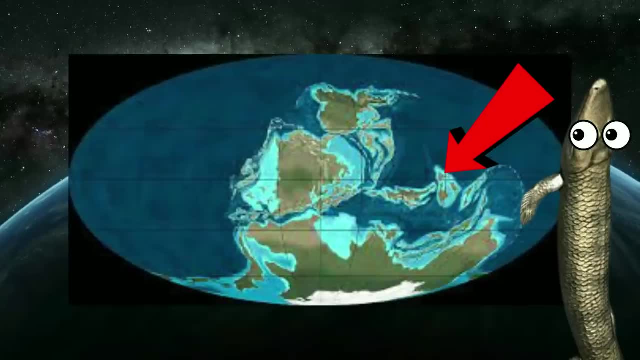 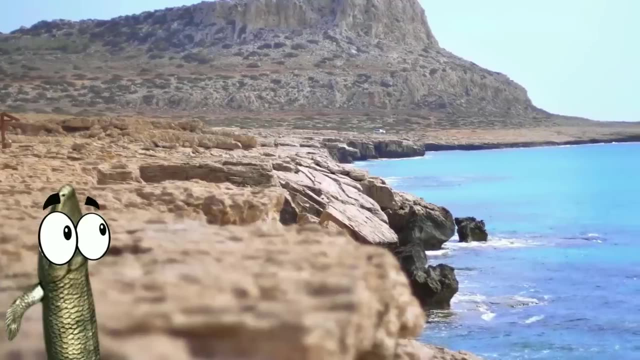 And the small chain of islands that started to form to the northeast of the supercontinent during the Devonian had grown into a small landmass in its own right. It's impossible to tell from looking at it, but this small island continent will one day make up. 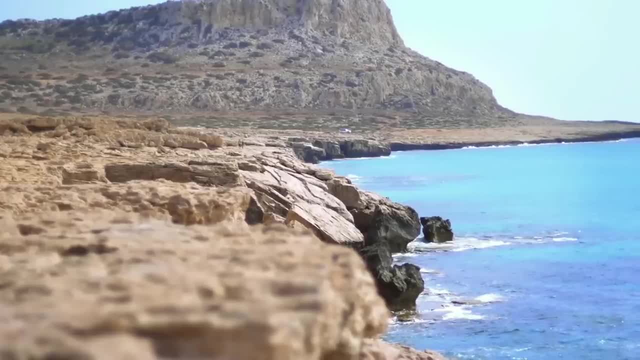 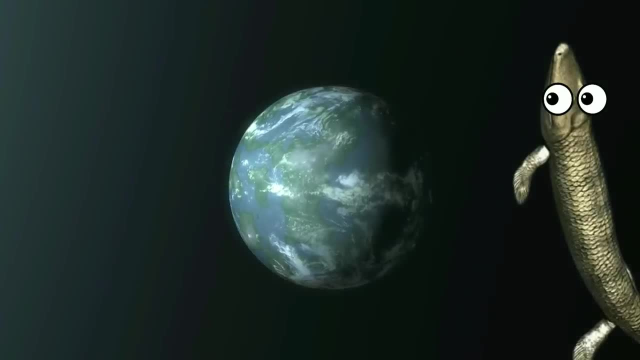 part of China. The formation of this landmass further isolated the panthelassic and paleotethis oceans from one another, But the real massive change was when this little blue and brown marble finally started to change into a blue and green marble. 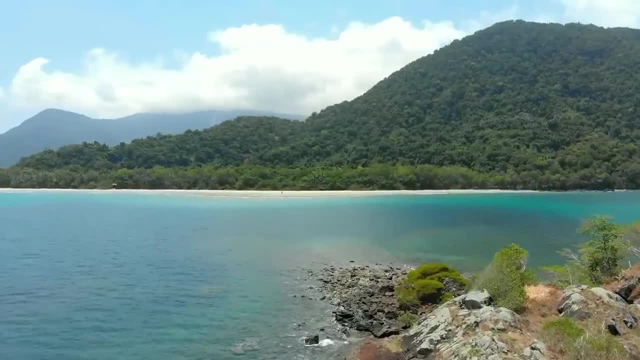 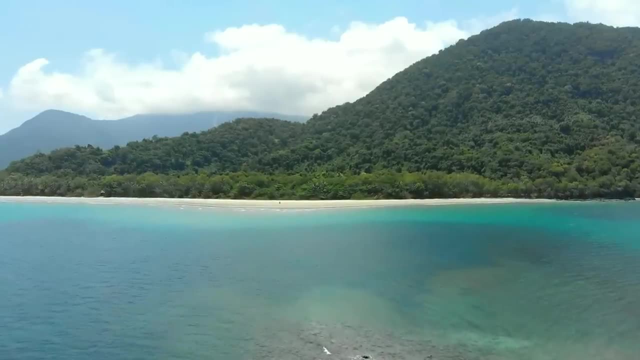 Plants, fungi, cyanobacteria and a few animals had been able to establish themselves on land in some capacity leading up to this time, But generally speaking, the first pioneers were restricted to staying close to the waterways, But this was all about to change. 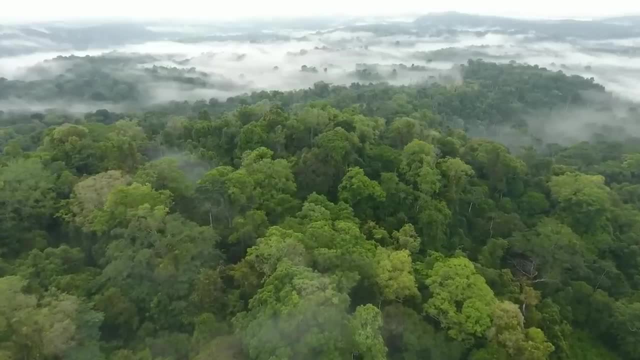 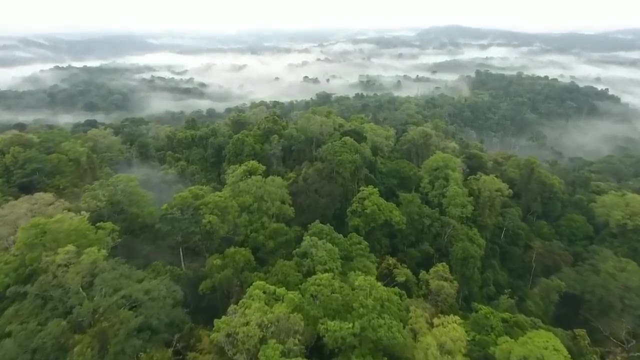 Because, in the hot, humid climate of the early Carboniferous, there was about to be an explosion of biodiversity every bit as impressive as the Cambrian or Ordovician explosions that we saw in the oceans of the past And the first organisms that we see this with. 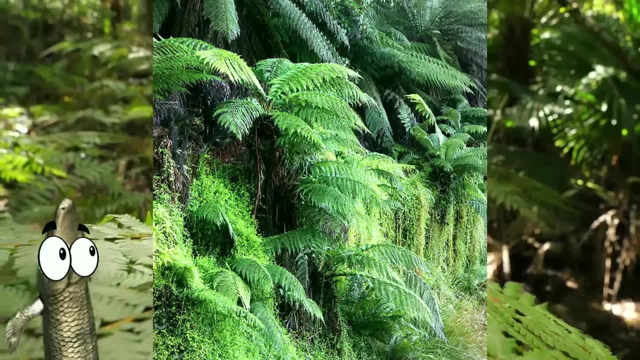 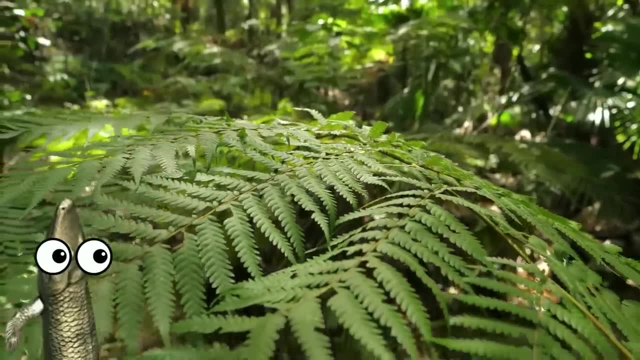 would be the plants. Horsetails, club mosses, ferns, primitive conifers and cycads all get their start here, And that's just the ones that we're familiar with today. This jungle would spread out from the rivers and ocean. 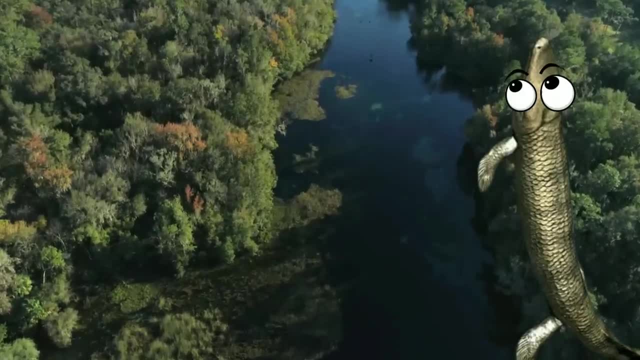 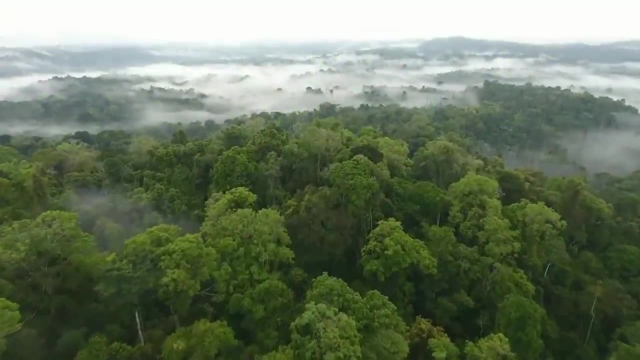 and cover the entire globe in an endless tree line, unlike anything we've seen up until now, And this would have a profound impact on the world in several ways. For one thing, plant life also meant a massive increase in oxygen, And any time that we see 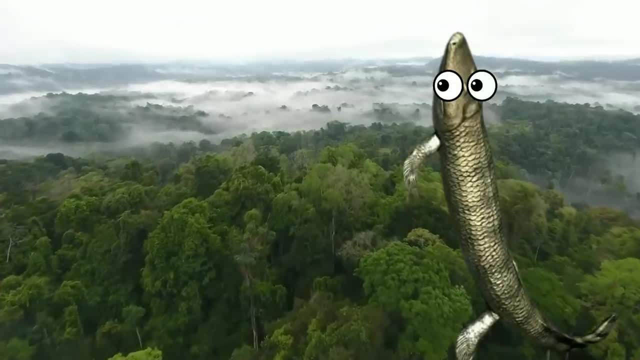 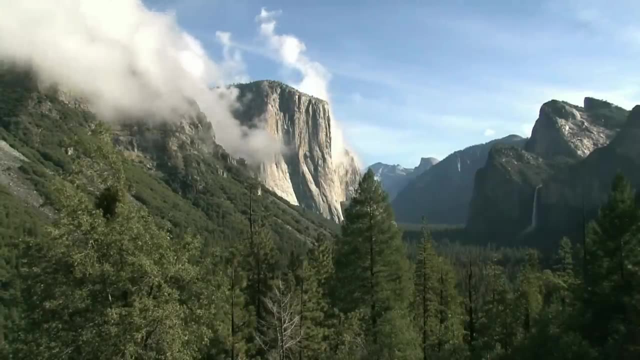 big changes in the air. usually that makes for big changes for everything else, as we've seen before. For one thing, it started to change the climate. We start to see a cooling trend by the middle Carboniferous that leads to an ice cap. 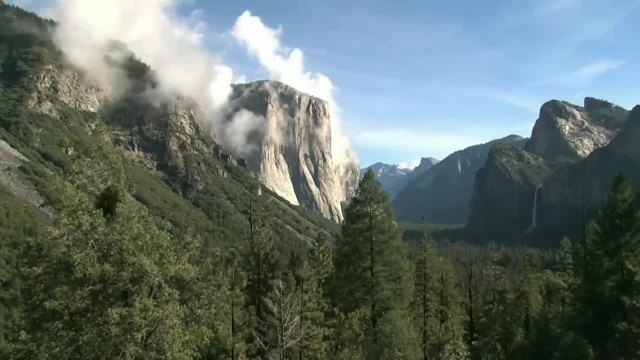 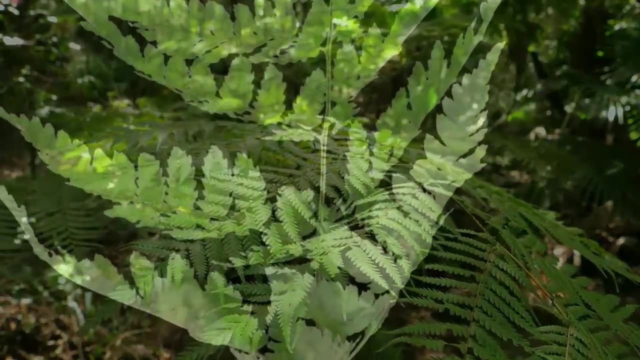 forming at the South Pole for the first time in millions of years, Probably the only part of the land that wasn't covered in vegetation. As this runaway effect continued on, generations of plants would come and go And old vegetation would fall to the forest floor. 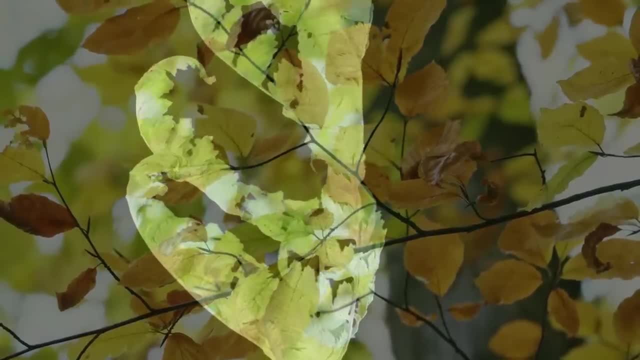 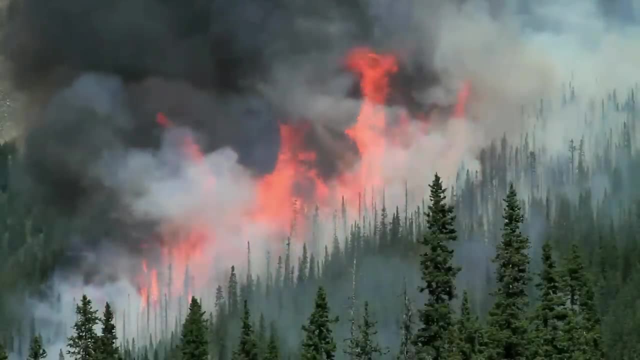 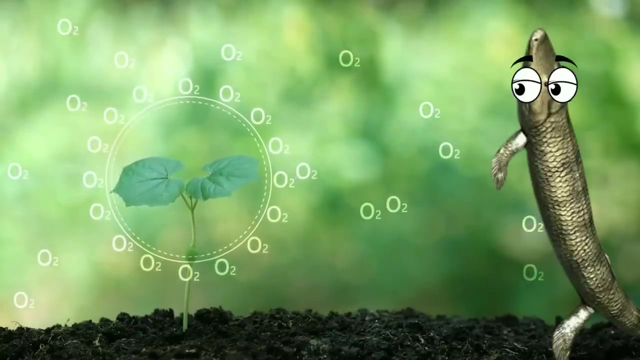 Either just through natural processes or, much more likely, forest fires. that would be taking place as an extra consequence of all the oxygen in the atmosphere, And these plants spent their entire lives taking in CO2 and expelling O2., Leaving the sea or carbon locked in their 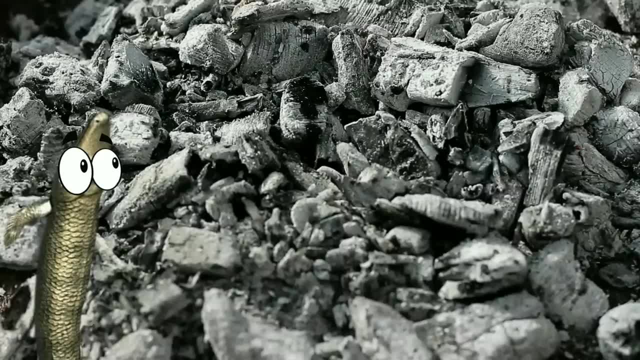 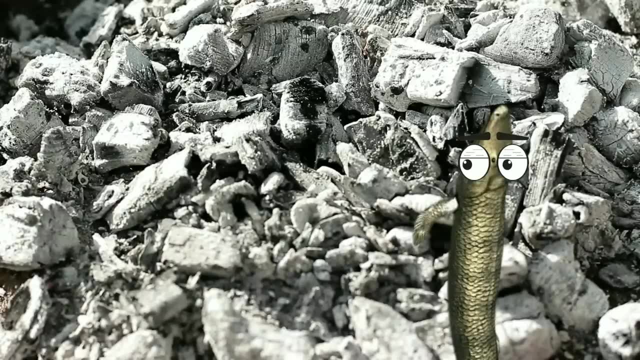 tissues And over the 60 million years of this period, this would be something that would be locked away in the Earth forever. So, slightly off topic, this is something that I hear from people all the time, People who say the use of fossil fuels. 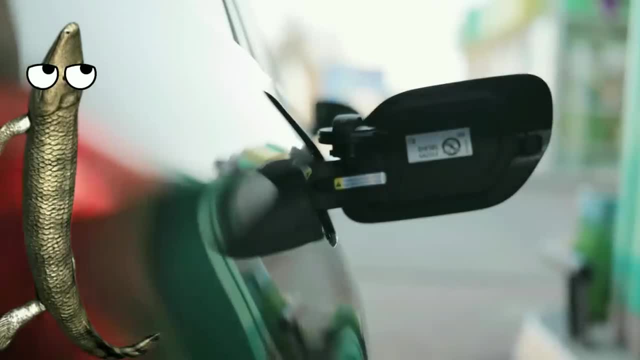 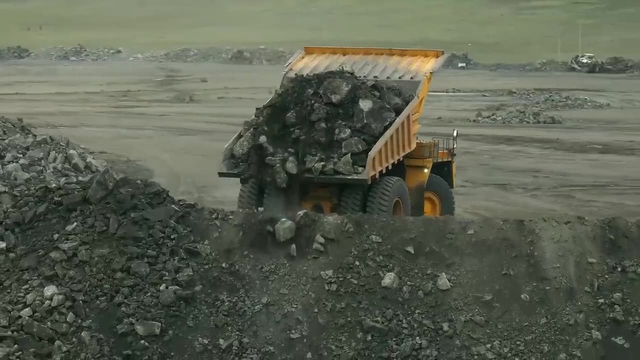 means that we're using the liquified fossil remains of dinosaurs are pretty much dead wrong. The overwhelming majority of the fossil fuels in use today originally are dated back to the coal beds of this time, 100 million years before the first dinosaur ever existed. 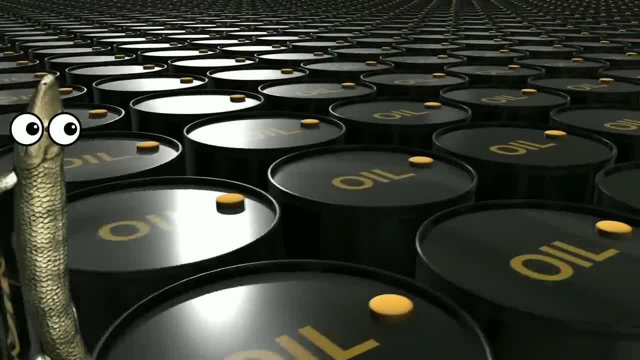 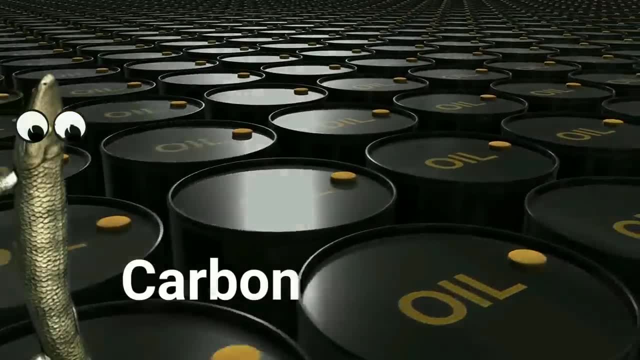 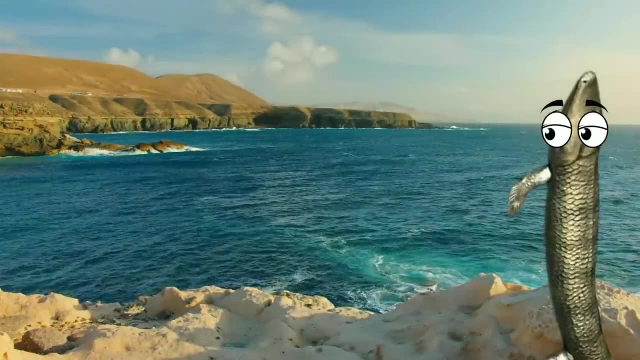 In fact, there's so much carbon in the deposits all over the world from this time that this is the inspiration behind the naming of this entire period: The Carboniferous Checking back in with the oceans. as I said before, the state that it was kind of. 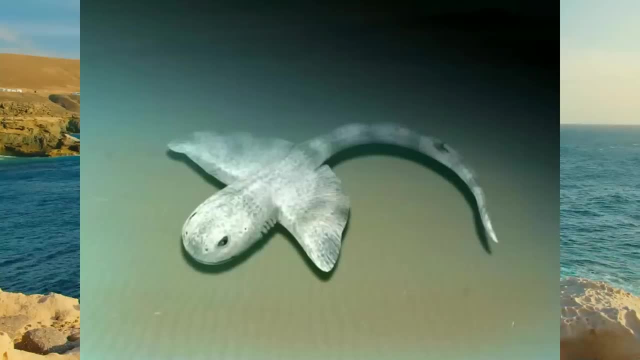 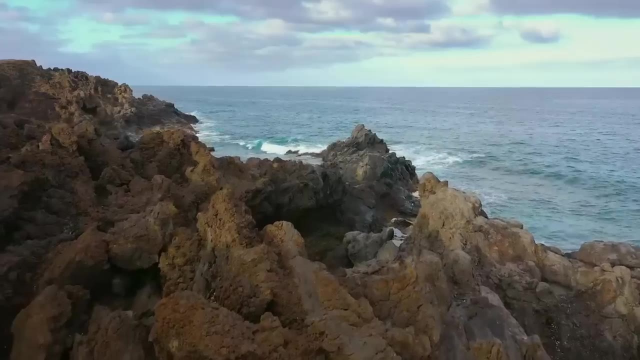 left in by the end of the Devonian was pretty sad, But of course, as always, extinctions leave opportunities open for the survivors to expand into new forms, And in the warm waters of the early Carboniferous there was about to be. 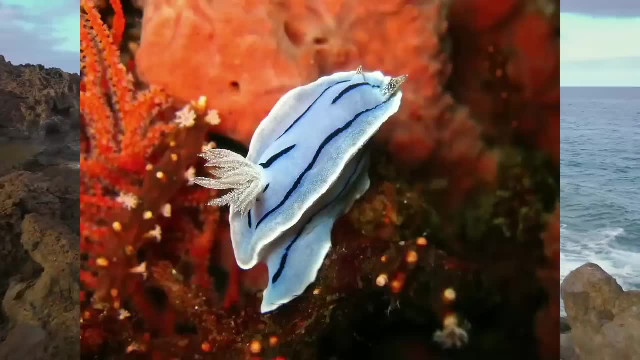 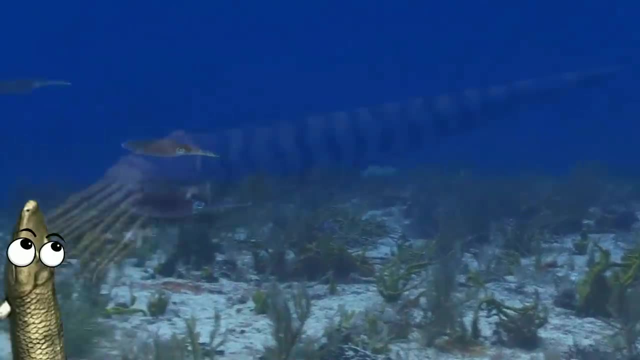 another mass extinction. Echinoderms, cranoids, gastropods and bivalves all managed to pull through, And the cephalopods were still hanging on as well. But by now the straight and curved-shelled varieties had died. out. What was left was the ammonites and the true nautiloids Which, despite animals like the modern nautilus bearing a resemblance to ammonites- this is how far back the two groups actually separated They may have been starting to get out-competed. by other forms of arthropods, like the true crustaceans. This seems to mark the end of the invertebrates reign as the rulers of the oceans, As the fish, despite losing 96% of their biodiversity by the end of the Devonian. 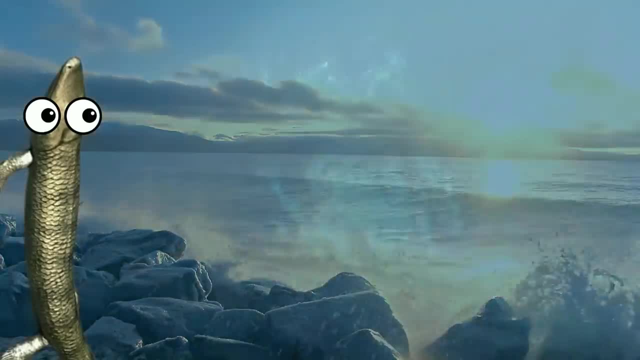 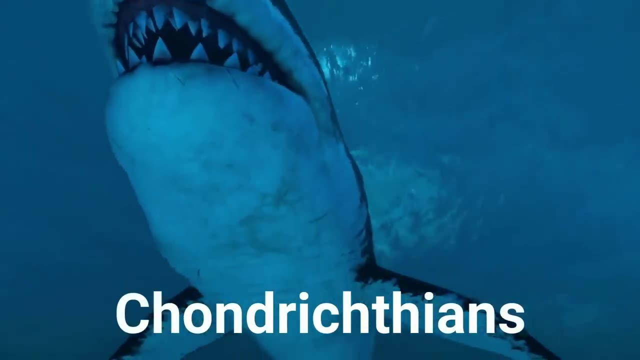 were about to take control for themselves, And this time it would be in a much more familiar form. This was the chondrichthian's time to rule The group of fish that, among other things, would lead to the shark. 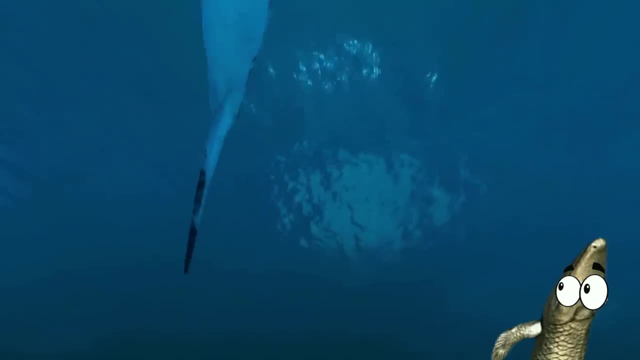 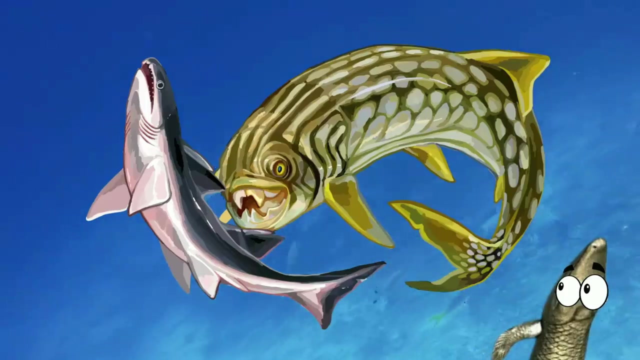 Now, this line of fish has been around since all the way back in the Silurian, but they had remained smaller and relied on their cartilage-based skeletons to allow them to be faster and evade the armored monsters that were filling the dominant roles. But now, 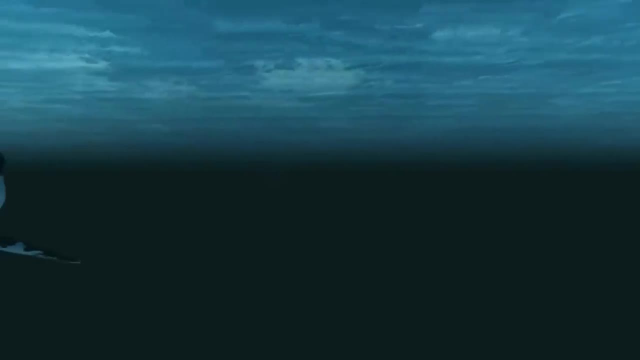 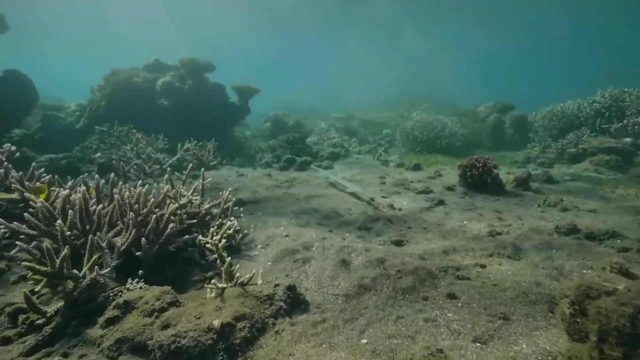 after the fall of the eurypterids and placoderms, it was the perfect moment for them to become the masters of the sea. The chondrichthians radiated into several different species of sharks and were successful, being a different group from the 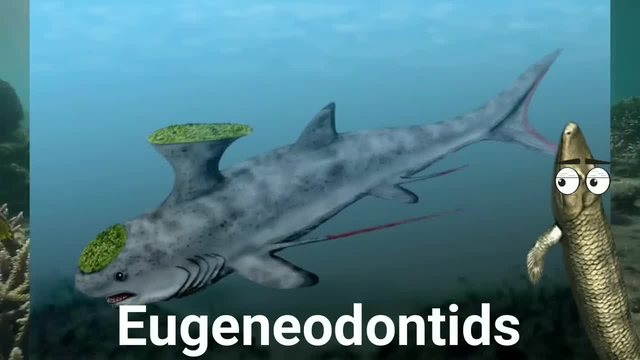 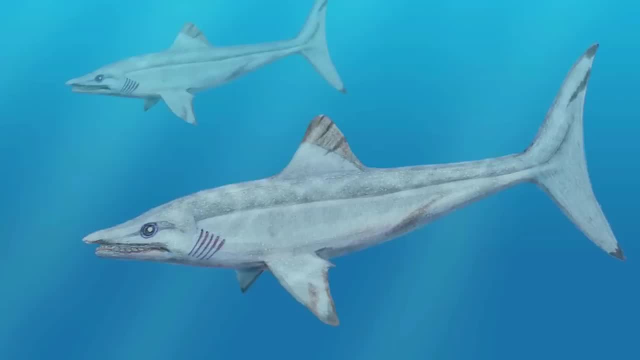 true sharks called eugeniodontids. These creatures had some very interesting face and head gear, But otherwise a lot of them were starting to be very similar to modern sharks. For example, there's the early species called cassiotis. This was one of the 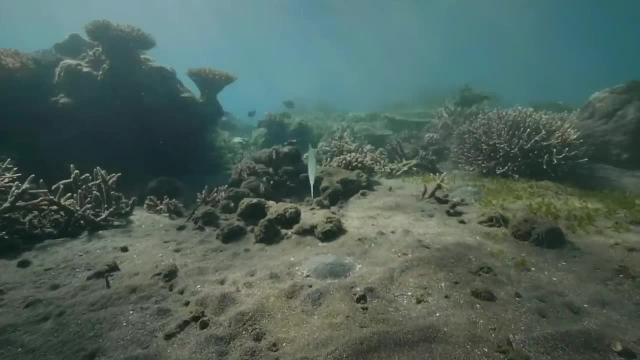 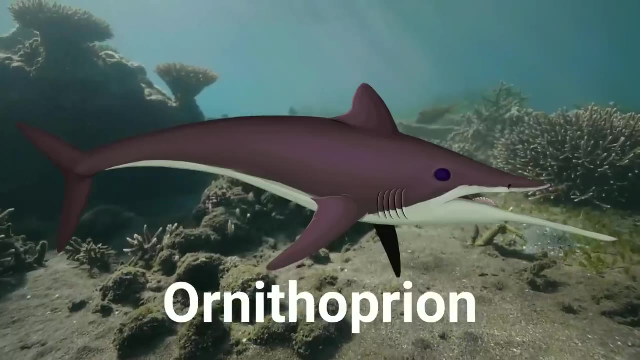 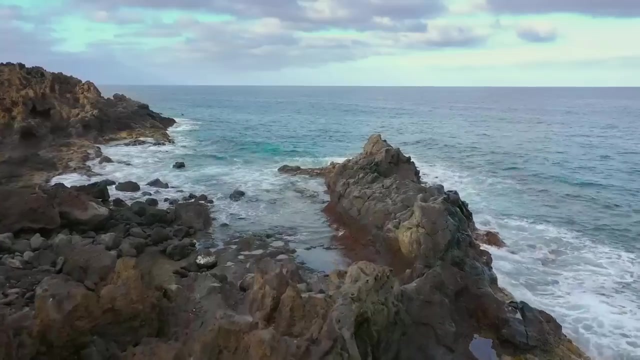 basial members of the group and although they would survive for quite a long time, it would also give rise to several other noteworthy creatures like the slightly different ones, which in itself would be the direct ancestor to probably the most well-known member of this. 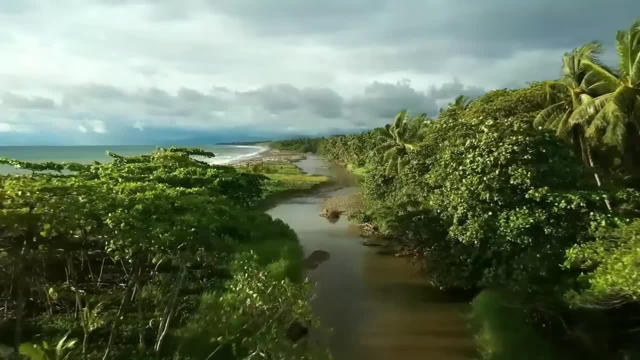 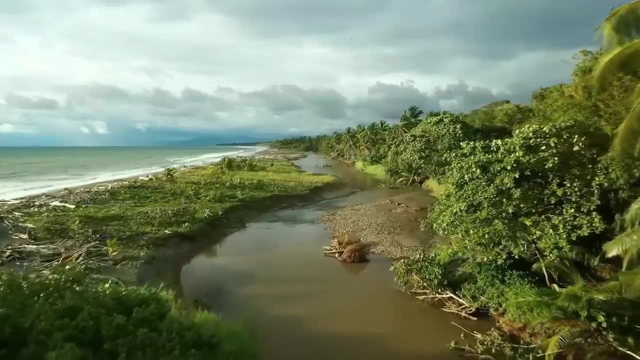 order in the future. The fish quickly bounced back as the Carboniferous went on, some groups even managing to spread into freshwater ecosystems, putting them in close proximity of the new world opening up in the air above In this world would be a world. 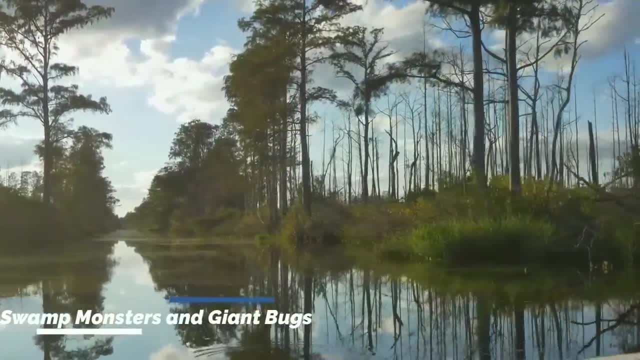 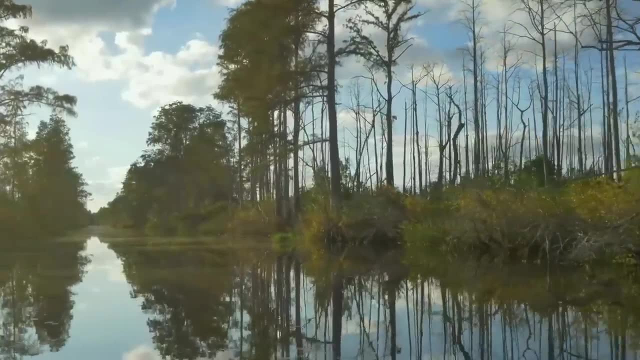 of swamp monsters and giant bugs. As oxygen levels skyrocketed and the land was covered in tropical forests and swamps, the vertebrates and arthropods were about to take their age-old evolutionary arms race to the new frontier. It was at this time that some of our tetrapod ancestors started to become true amphibians, finally developing the fins and fin-like legs into proper weight-bearing limbs. The earliest example of this was with a creature called Pederpes, a name which means Peter's foot. 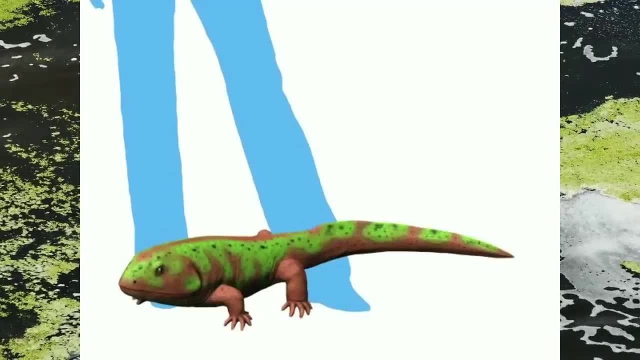 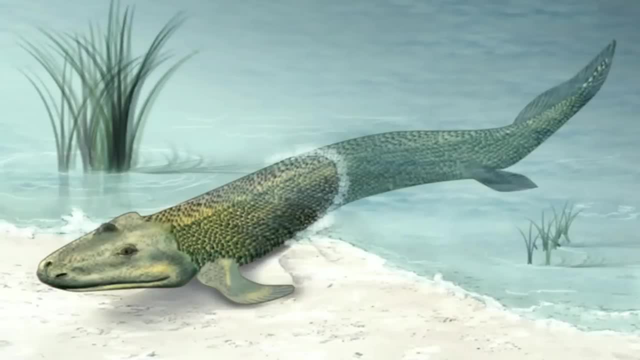 Who's Peter? This one-meter long creature is very important because it's currently thought to be the evolutionary link between the tetrapods that were more similar to lobe fin fish and the true amphibians, And also because fossils of land animals from the 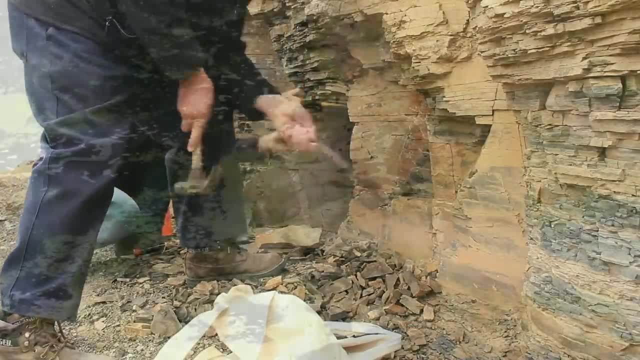 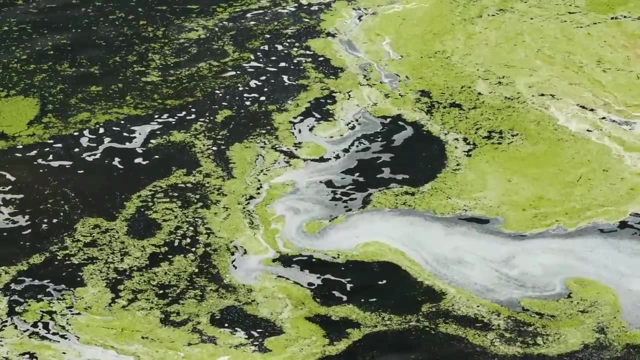 early Carboniferous are extremely rare. So for all we know, there might have been a ton of other animals like this crawling around, But as time goes on we do see a lot of other strange types of amphibian in the later stages. 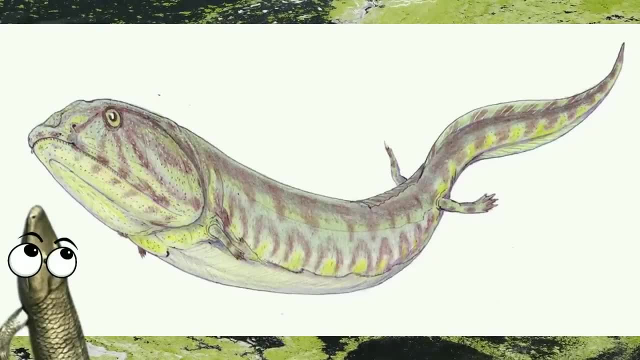 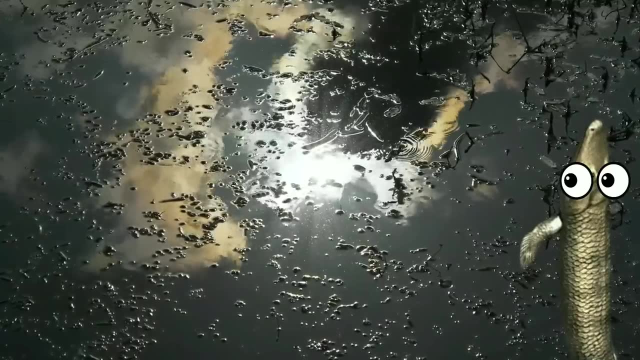 Some of them had their shiny new legs shrink and become more snake-like, like this thing called Coloradoerpeton, and then someone in the opposite direction and further developed their limbs for walking on land like Tuttytanus, And we even have 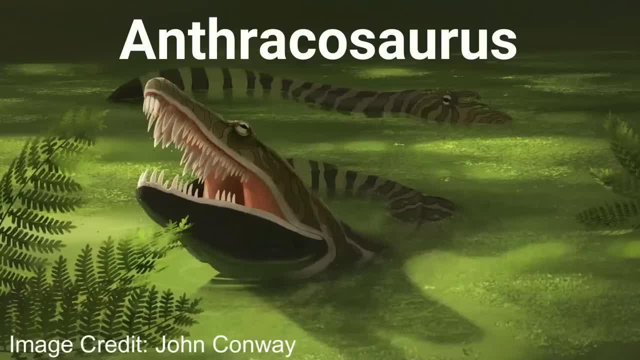 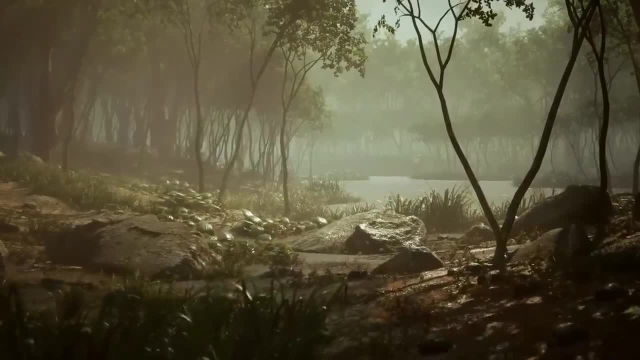 some major predators coming from this group, like Anthracosaurus, measuring up to three meters long and is also known as the reptile-like amphibians, But the most dominant of all was a group of ruling amphibians called Spondylus. 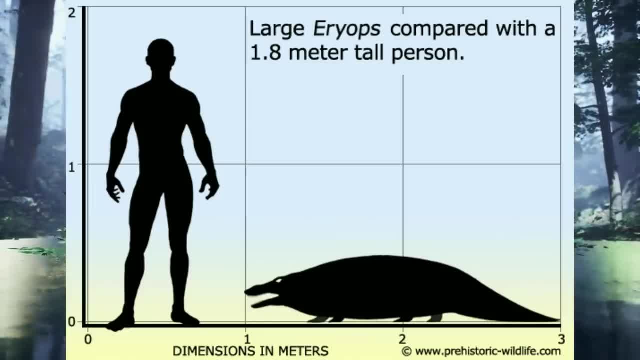 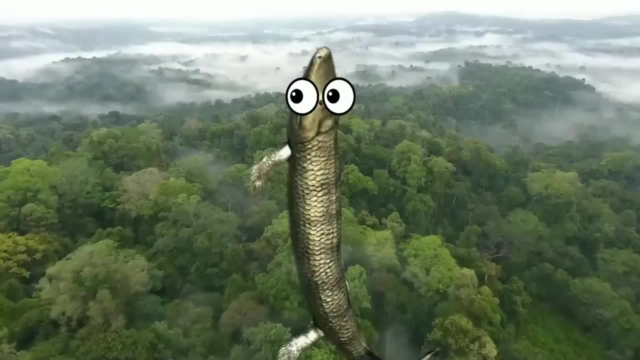 Large species like Eriops may have grown up to three meters long and two hundred kilograms, probably hunting, somewhat similar to, once again, crocodilians. These were some of the most powerful vertebrates on the land, But unfortunately, not only did our 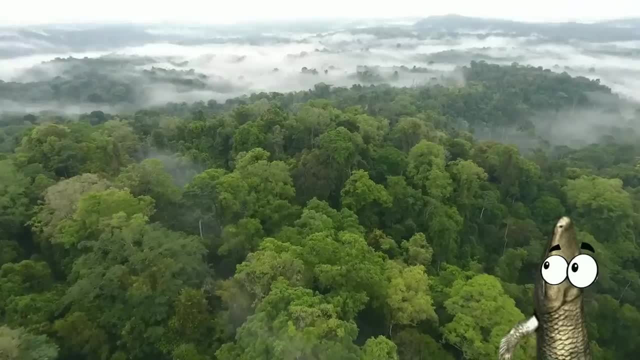 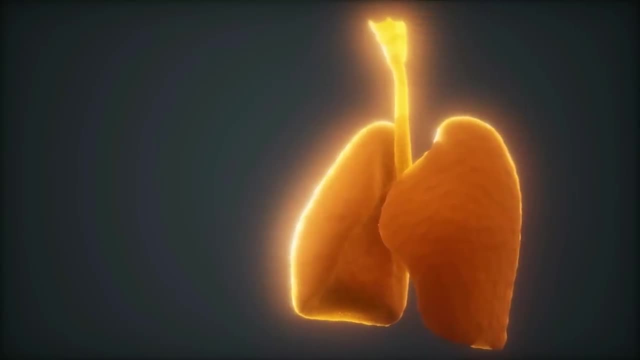 arthropod competitors have a head start colonizing the land, but the way that they were designed was going to give them an edge in this high-oxygen environment. You see, unlike terrestrial vertebrates, which have lungs and breathe through their nose and throat, terrestrial 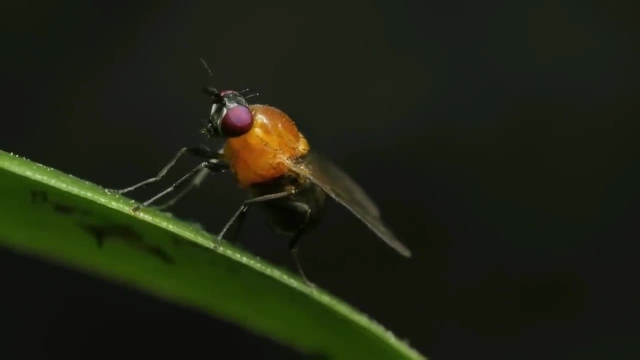 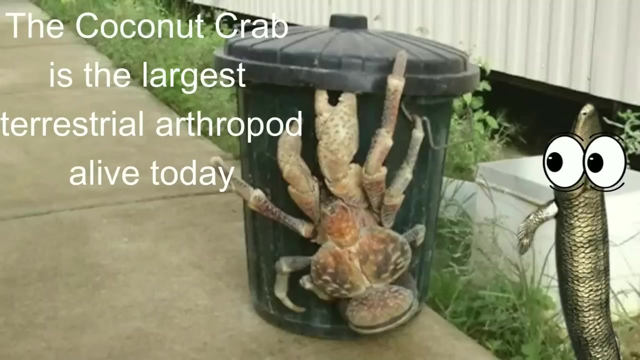 arthropods have openings across their bodies that connect to the tissues that need oxygen. That's why today there's an upper limit to the maximum size that arthropods can reach, Because in today's atmospheric oxygen level of 21%, bugs can't grow. 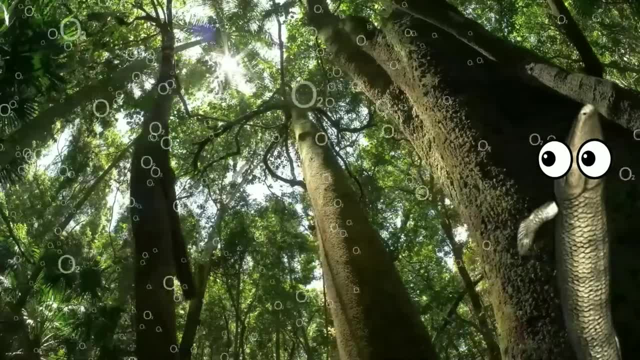 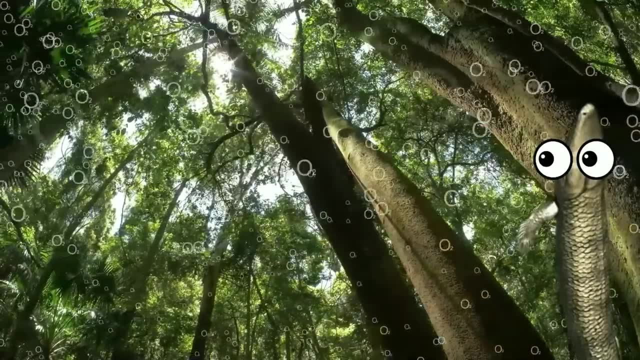 to three, four meters long. But if you crank the oxygen up to, say, 35%, as it was in the Carboniferous, suddenly the limit has been raised. In these jungles there were giant bugs Like the terrifying 70-centimeter-long. 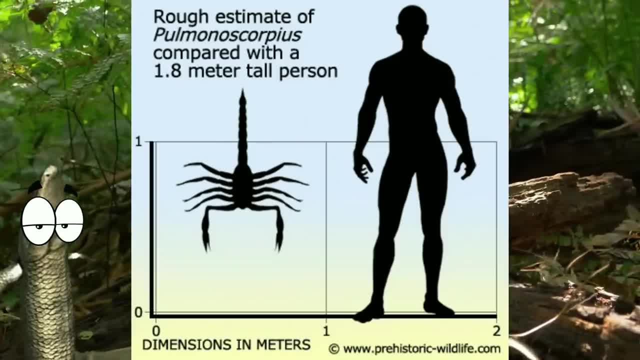 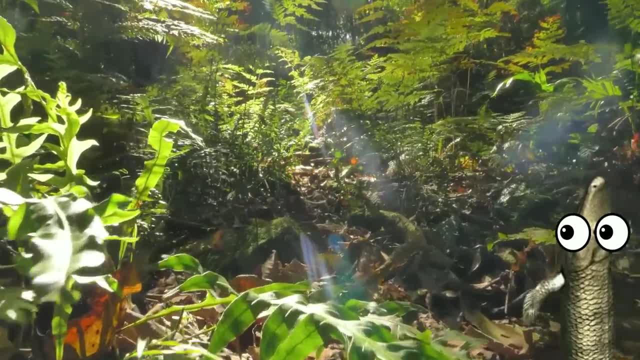 Pulmonoscorpius. Yes, this was a scorpion the length of a human arm, the largest any terrestrial arachnid would ever grow. And we also see the largest land invertebrate to ever exist, the herbivorous Arthroplura. 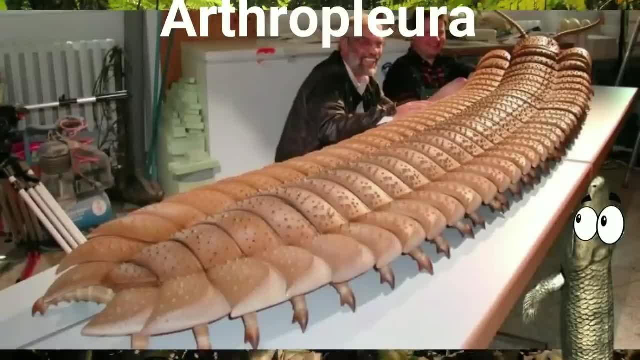 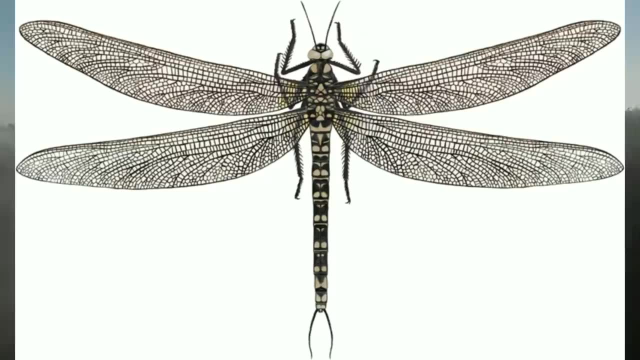 a millipede that could grow up to two and a half meters long, And the bugs would even take to the skies for the first time during this period, Most well known of which being the falcon-sized Meganura, a relative of modern dragonflies. 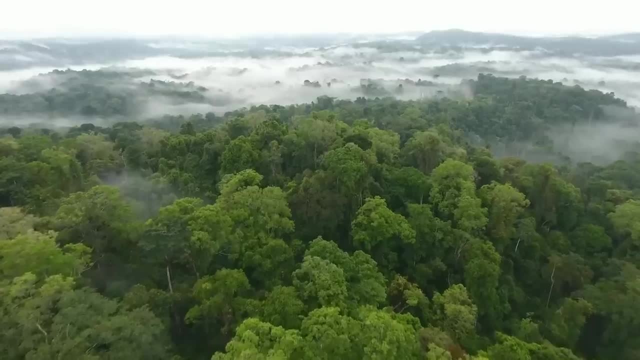 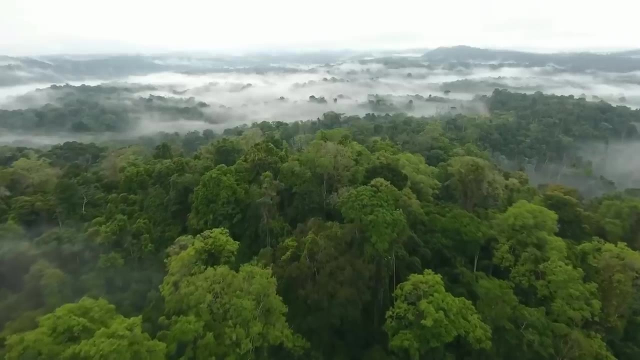 and damselflies. And among all these monsters, in the tropical landscape of the Carboniferous, there was even a relic of a bygone time, lurking in the swamps: The one and a half meter long Campyocephalus. the very last. 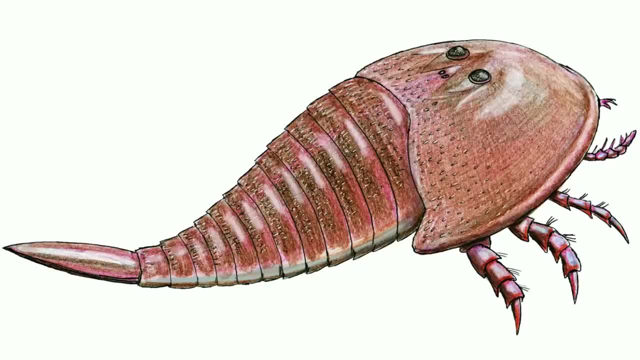 of the sea scorpions. Despite this guy's pedigree for predation, the Eurypterids' days were long past them at this point, Basically nothing more than an oversized horseshoe crab, probably using its shovel shaped body to push through the 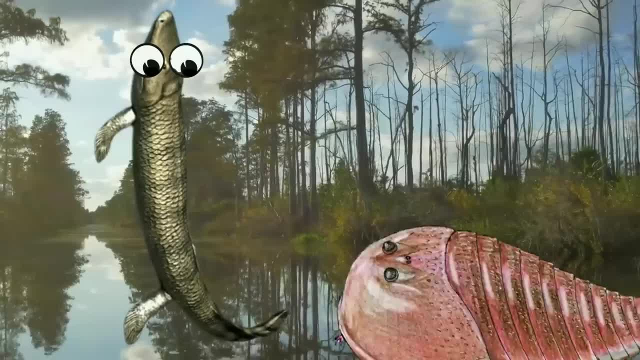 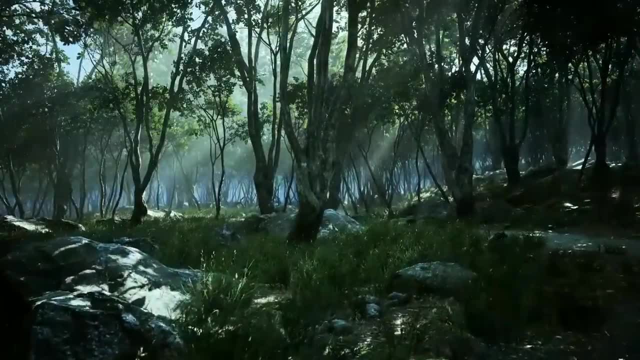 muck and scavenging on whatever it could. A humble end to what was once the top predator of the oceans, With all these strange creatures around the Carboniferous swamps, was likely a very dangerous place for many of the smaller vertebrates running. 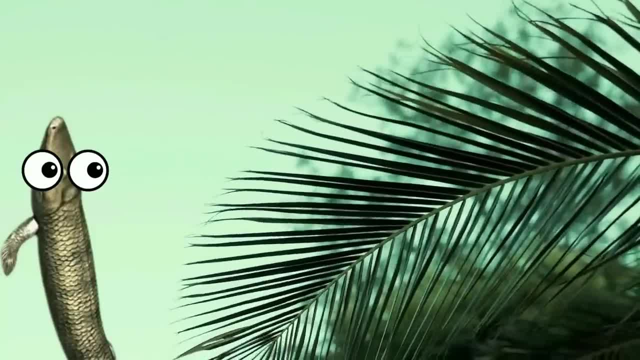 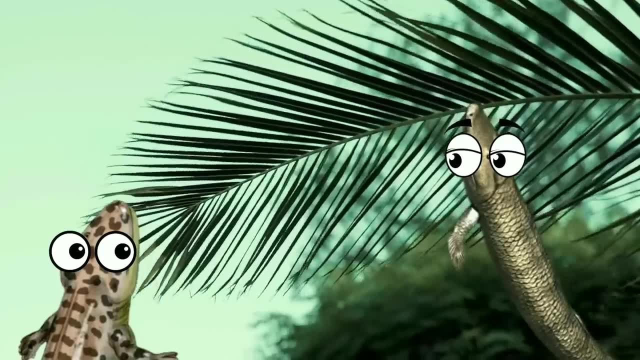 around Our direct tetrapod ancestors were constantly having to hide from giant carnivorous amphibians and bugs. They were also very dangerous to the Eurypterids. Setting aside all your shenanigans, I think we're going to need a new strategy. 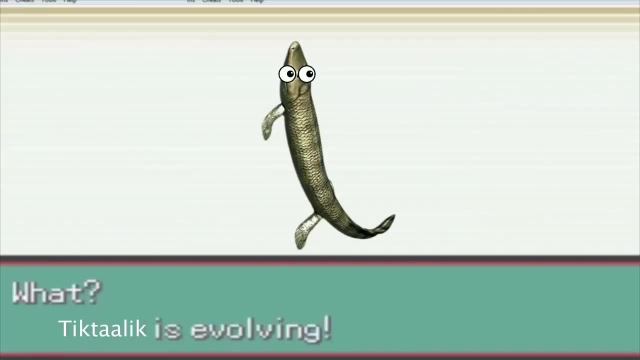 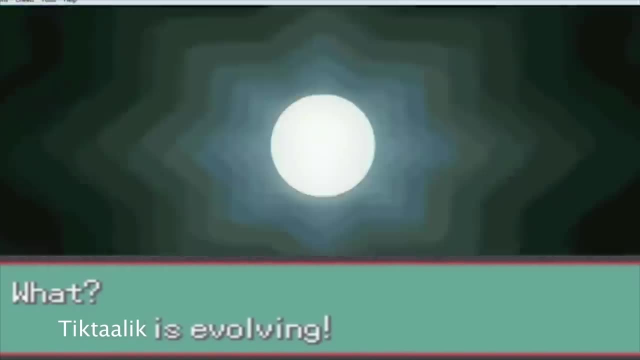 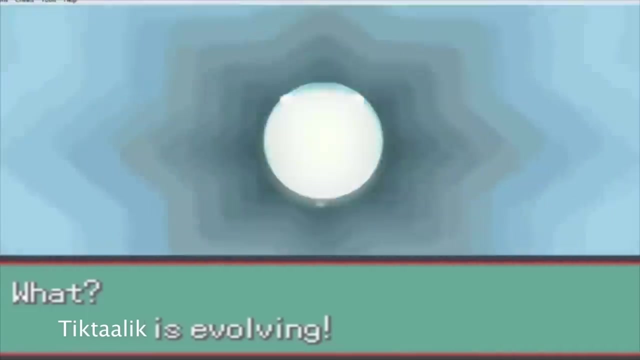 to survive this jungle. It's time for us to free ourselves from the swamp. Here we go again. The Eurypteridops are the most dangerous species in the world. They are the most dangerous species in the world. They are the most. 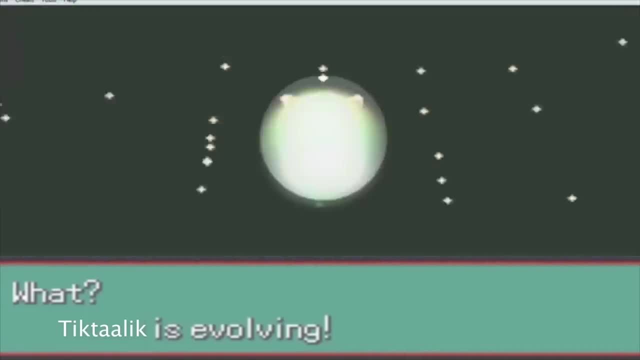 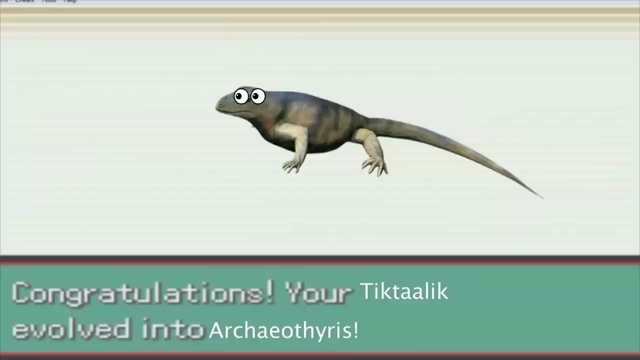 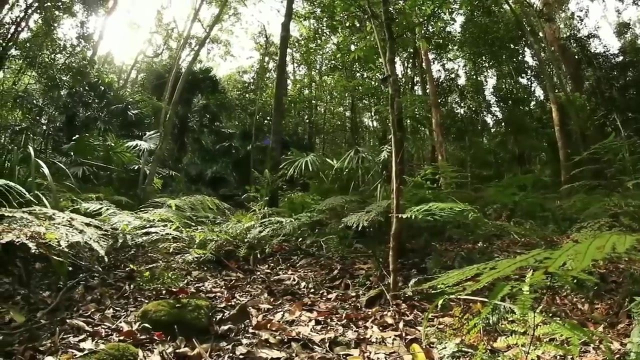 dangerous species in the world. Finally, a mammal adjacent, Going into the late Carboniferous. there was a major change on the horizon for our ancestors. You see, despite the fact that the forests were spreading far inland from the rivers and swamps. 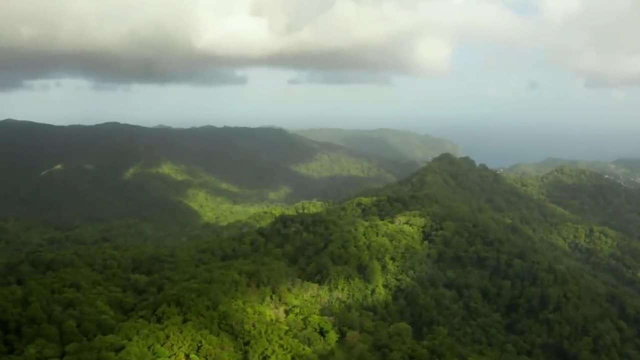 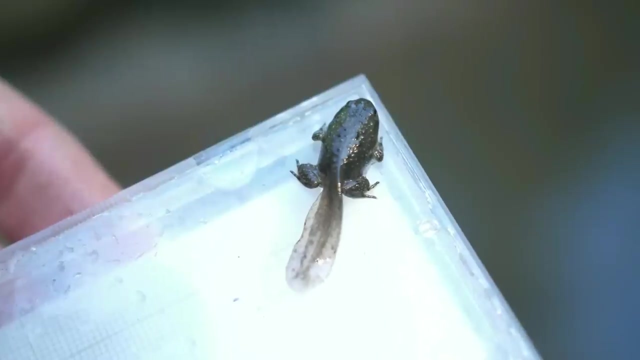 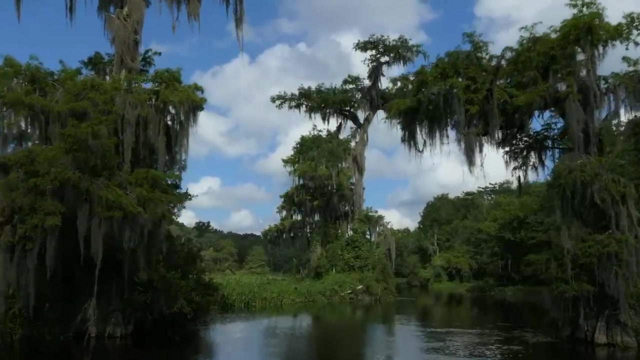 we were not able to do the same. This is because the early tetrapods were still dependent on the water. We could breathe air, but our skin was not capable of holding water. So if we spent too much time on dry land, we ran the risk. 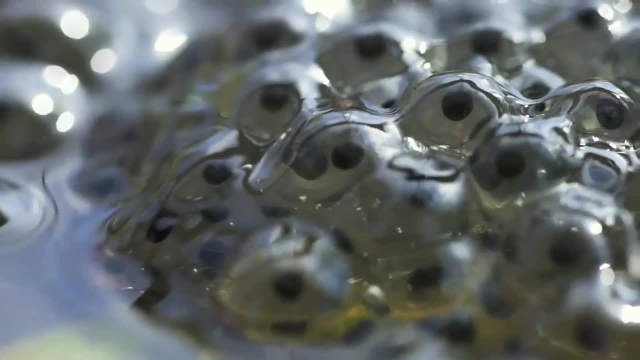 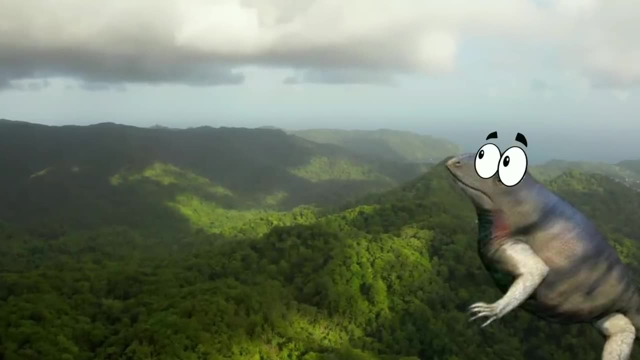 of drying out And our eggs were still completely dependent on the water. So for a while we were kind of stuck, But these were all issues that we were going to overcome. around 320 million years ago, As some of the amphibious tetrapods 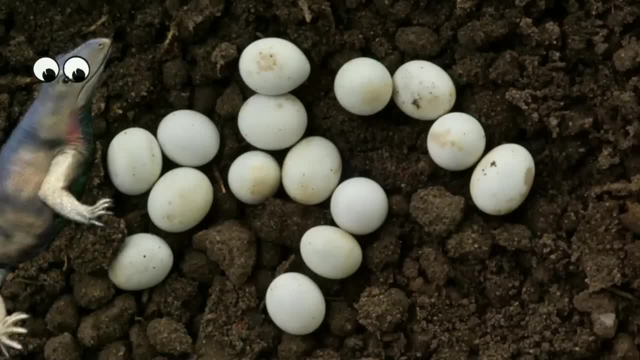 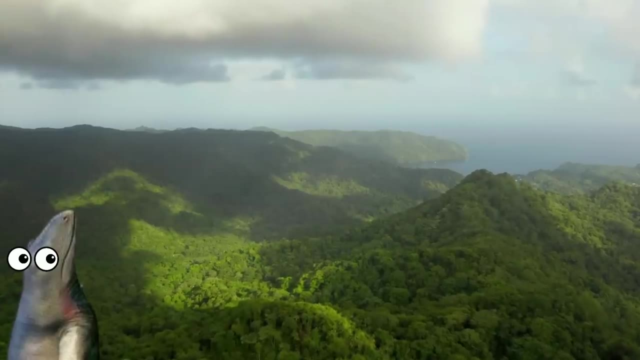 became the very first amniotes. Their thicker skin would make them less physically fragile, as well as allow them to be laid outside of the water. We were now truly all-terrain organisms And with these new adaptations, the amniotes spread across. 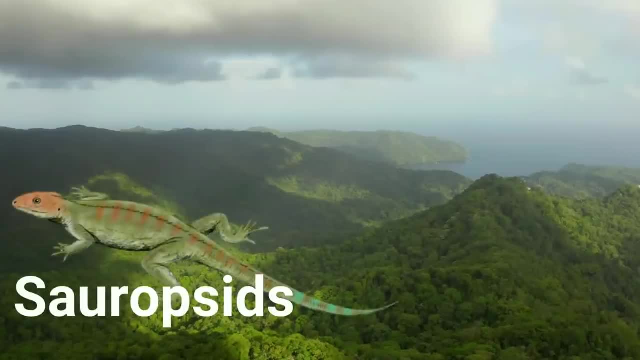 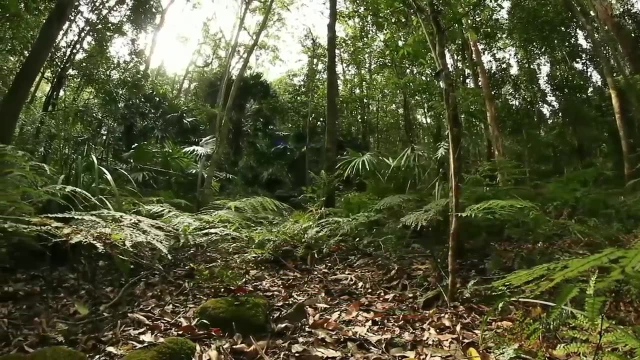 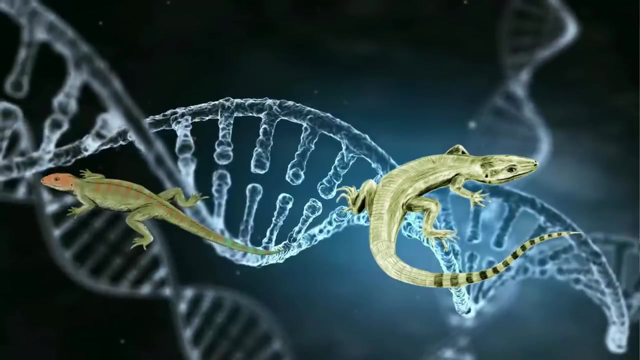 the world diversifying into two major clades, the sauropsids and the synapsids. Despite these early members of this order looking very similar to each other, inside there were differences that would be the defining features of the two clades. 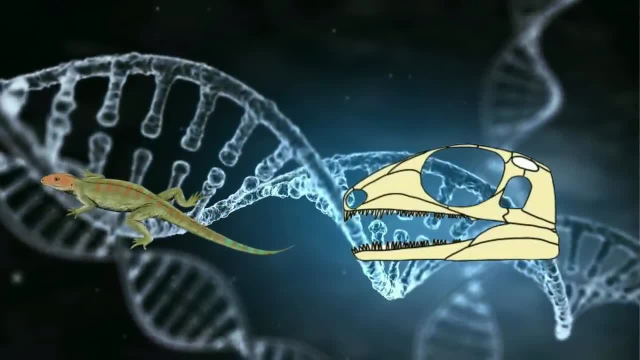 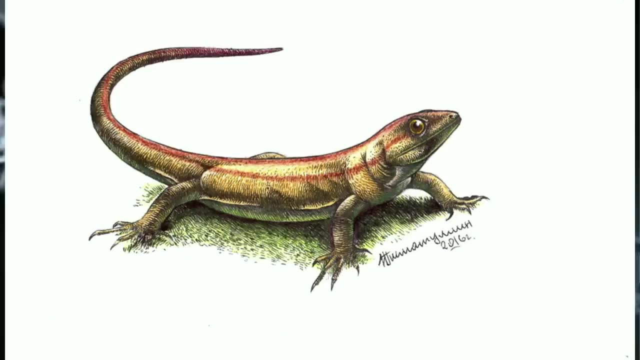 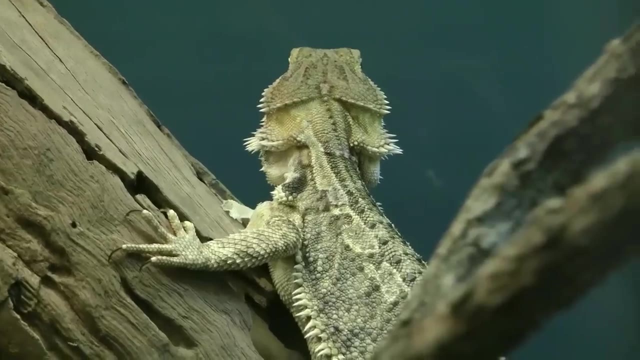 These can best be seen in the skulls and teeth. While the skulls of sauropsids had two openings besides the eye socket, synapsids only had one. The earliest known sauropsid was a tiny lizard-like animal called Cassinuria. This was the 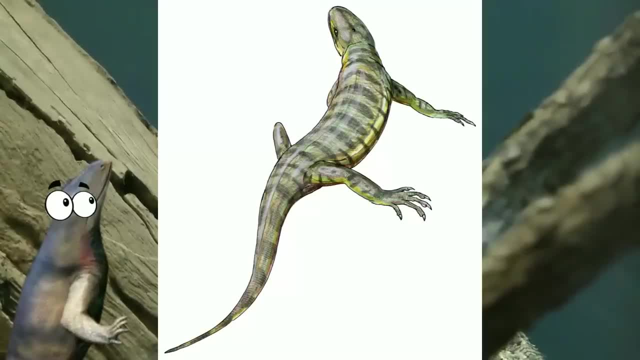 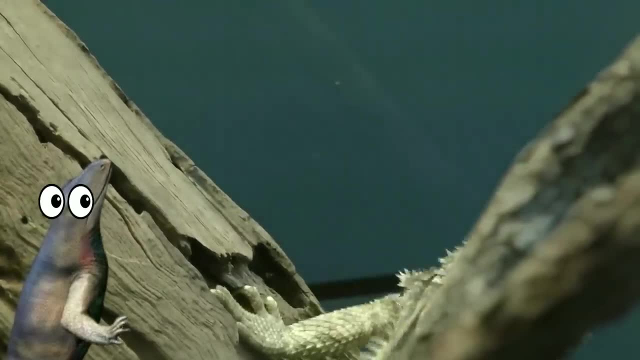 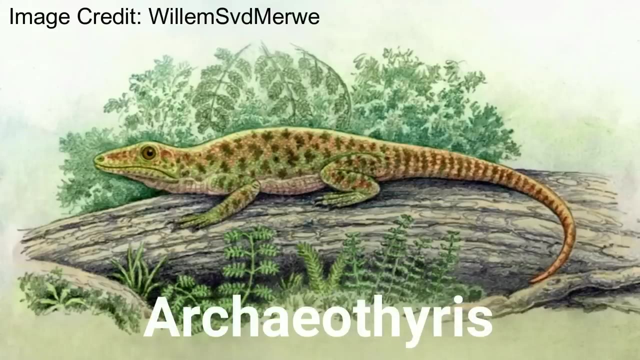 earliest animal to have claws on its fingers. Yet another adaptation that would be massively useful for future generations. The earliest of the sauropsids would be Archaeotherus, a tiny lizard, but was actually more advanced than the early sauropsids. It had stronger 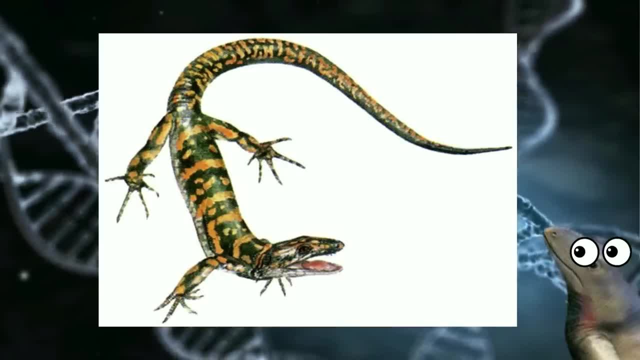 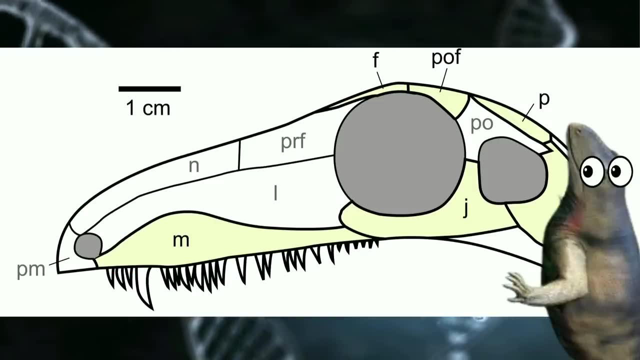 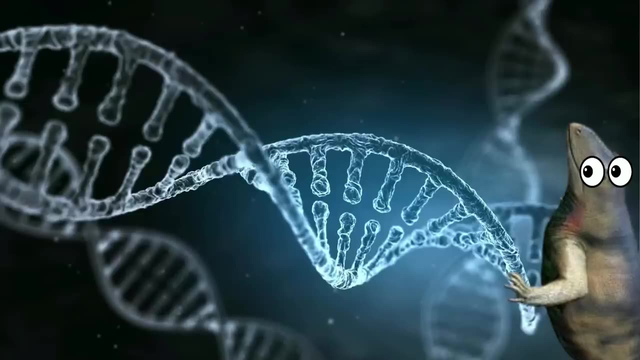 jaws than most animals at the time for this size and had a pronounced canine tooth. That was another thing that separated the sauropsids from the synapsids. The synapsids tended to have different teeth in their mouth, at least much more pronounced. 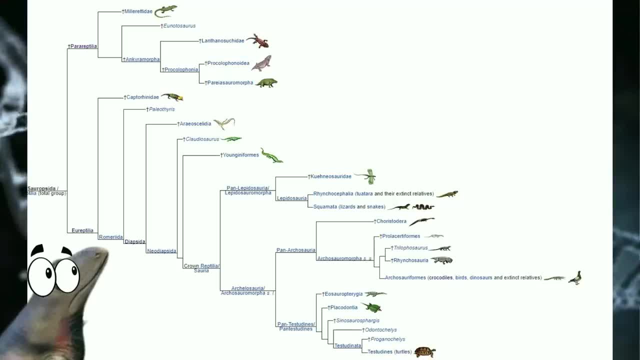 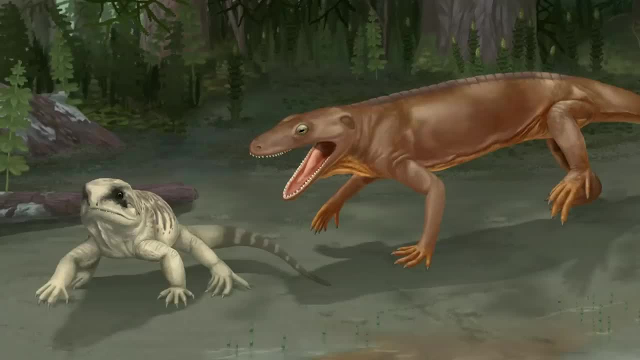 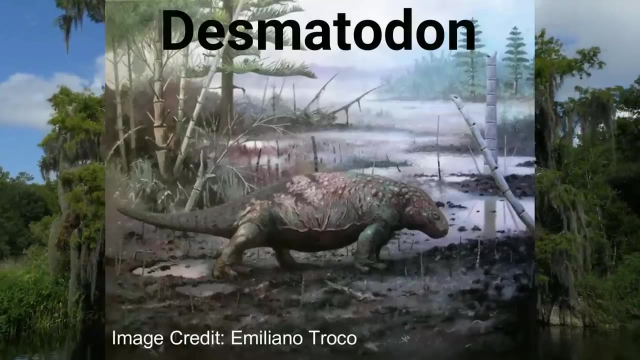 differences than what we saw in the sauropsids Now, despite all the amniotes looking pretty similar early on, they would explode over the next 20 million years and once again be able to fight back against the giant bugs and amphibians hiding in. 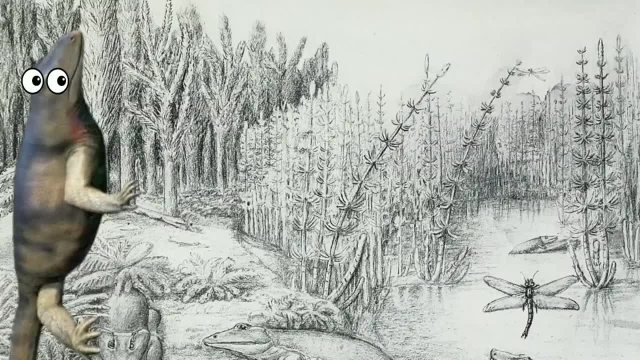 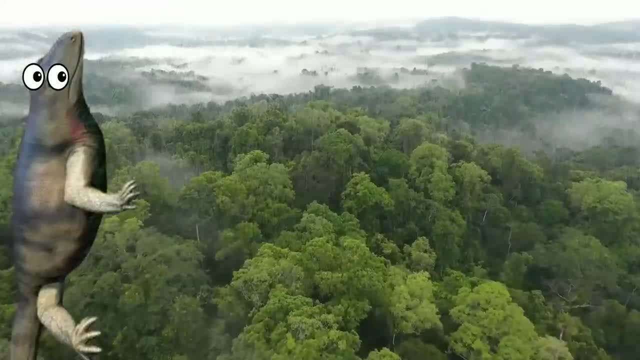 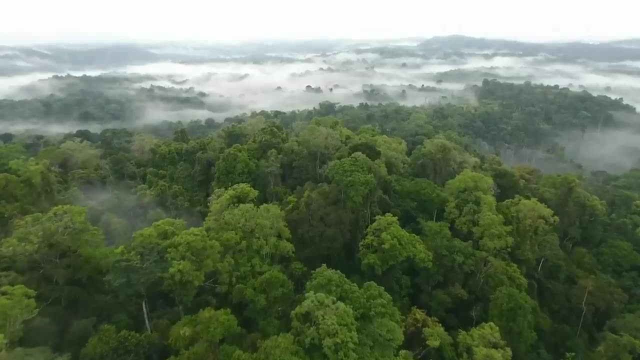 the swamp, And they would get larger too with herbivores, or the age of giant bugs, depending on which side you're on. I guess By the end of the period the amniotes were making a decent case for themselves, as they managed to. 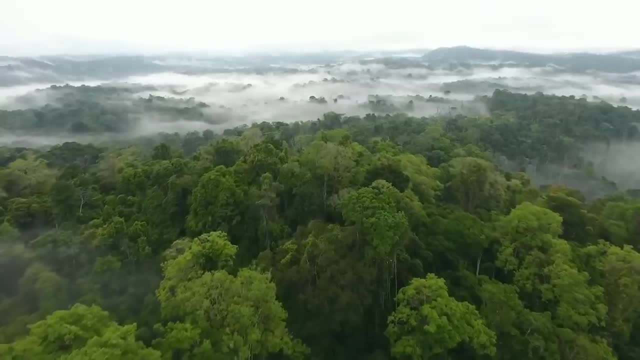 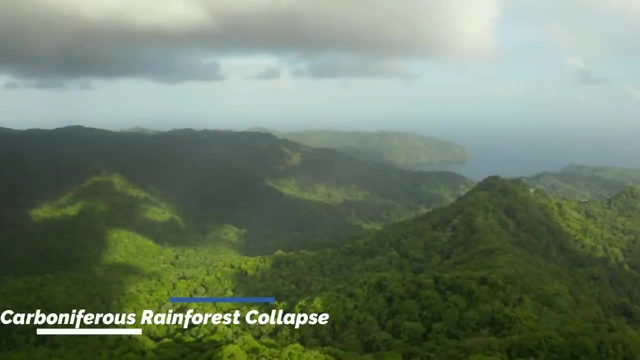 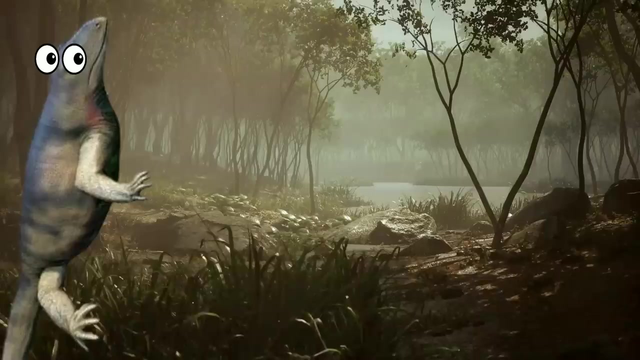 go anywhere that they wanted to, And it was a good thing that they did too, because as Gondwana and Euramerica came together, there was going to be a lot of changes that continued to have an effect on the climate as well. 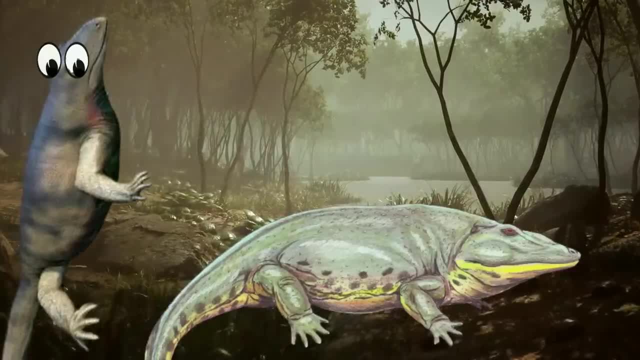 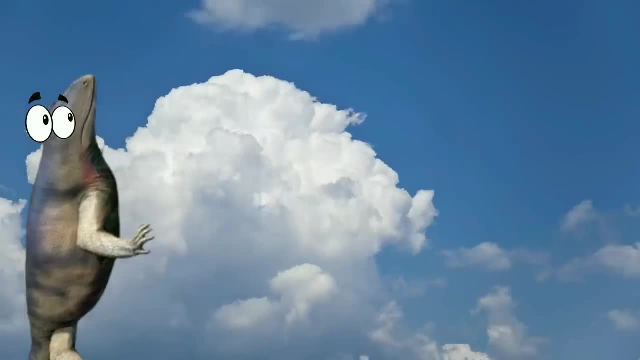 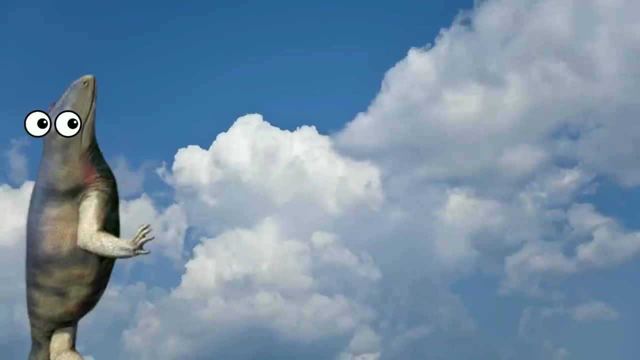 Through most of the Carboniferous. things remained pretty warm and humid, just the way the amphibians liked it, and the oxygen levels kept getting higher, just the way the giant bugs liked it. The problem was that this was creating a cycle that 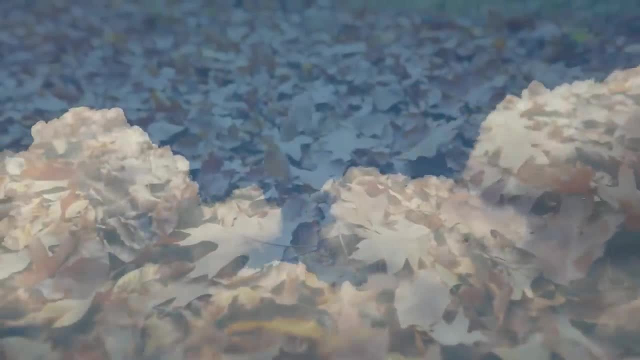 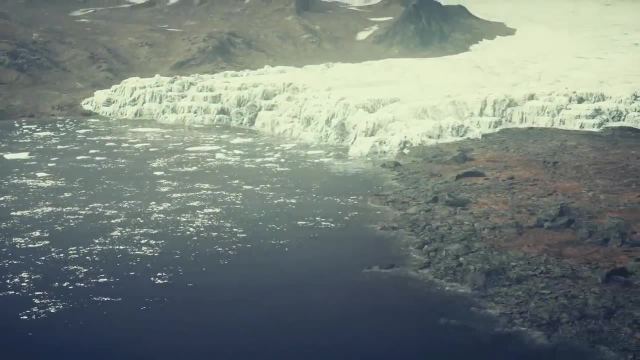 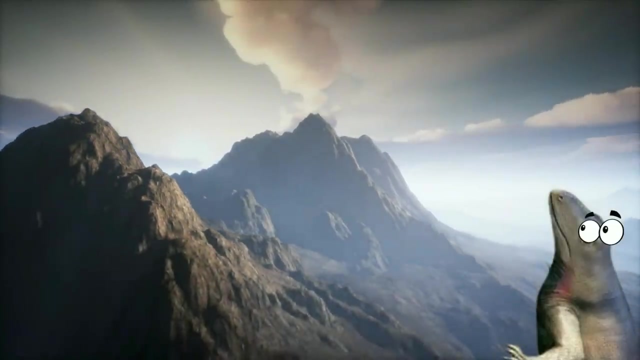 inevitably could not sustain itself because CO2 would start to get cooler. The glaciers over the South Pole started to expand. This dropped the sea level and made the climate drier, And then, as things were already starting to get dicey, Gondwana. 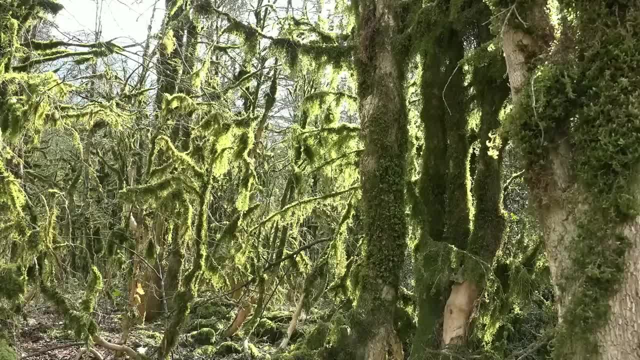 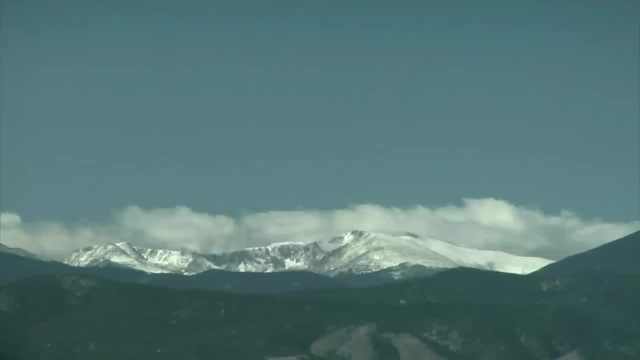 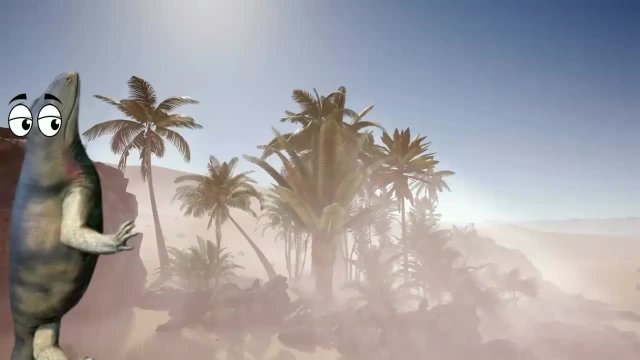 Siberia and Euramerica would finally come together to form the massive supercontinent known as Pangaea, And this led the ocean to the interior of the continent, And without rain, there can be no rainforests. This is known as the Carboniferous Rainforest Collapse, And this would be the event that brings this period to an end. As the southern region became locked in ice, the swamps and rainforests started to disappear. This would spell the end of the giant bugs. 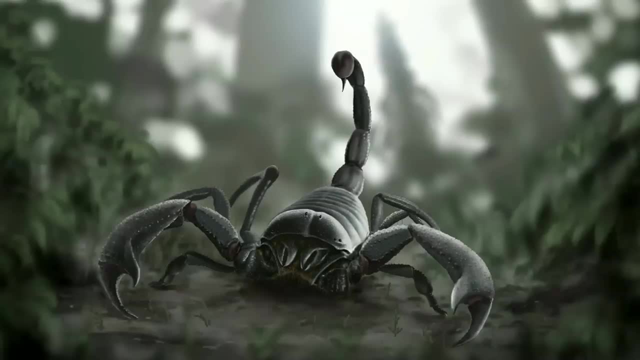 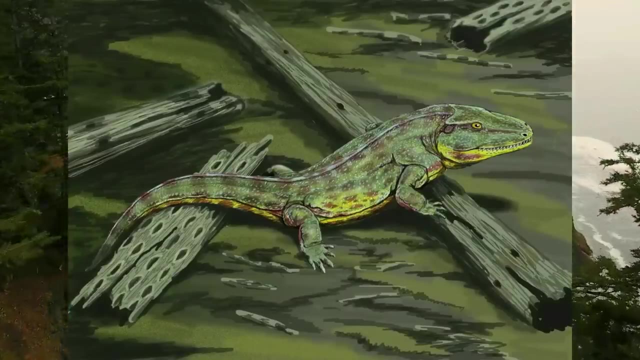 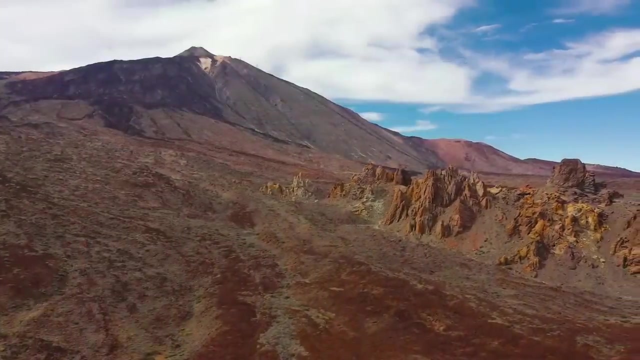 A few temdospondyls would manage to hang on in the coastal areas near the equator, But ironically, our ancestors were doing quite okay, And now, in this new dry world, the amniotes were going to take over. 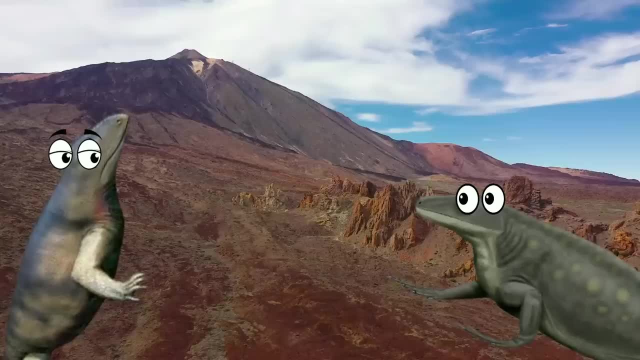 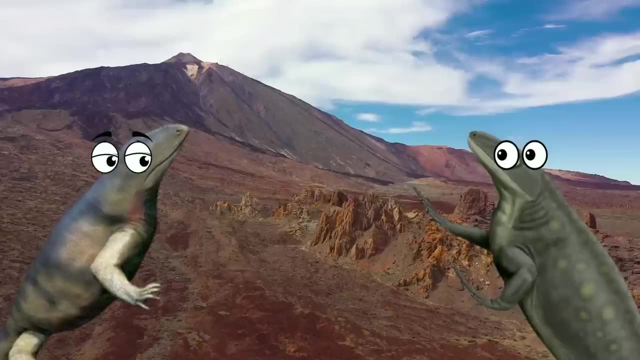 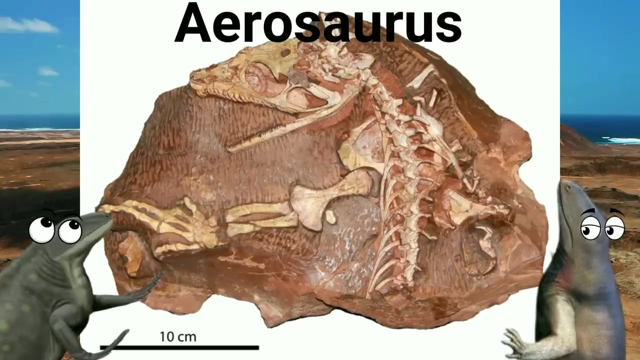 Especially the synapsids. Ah, Timtim, I see you as a stem mammal. Is the coast clear? Yep, Most of the bugs and swamp monsters are all dead. Timtim here has evolved into another synapsid called Aerosaurus. 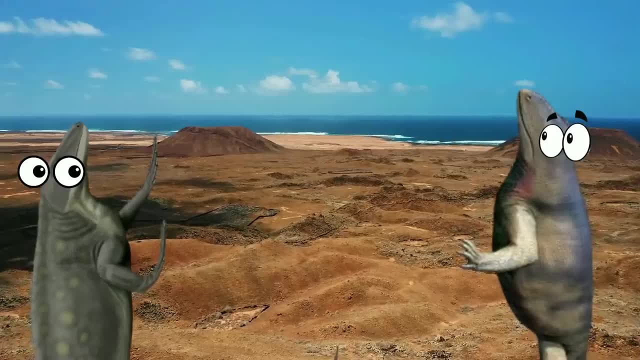 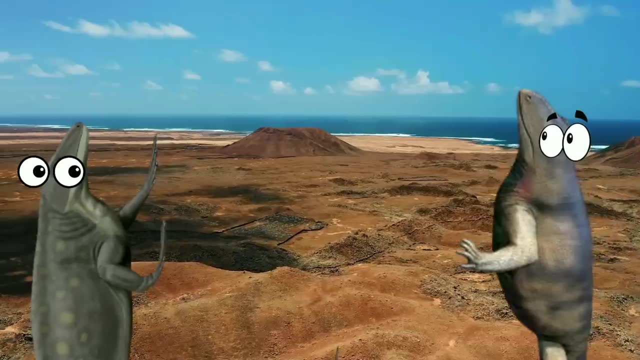 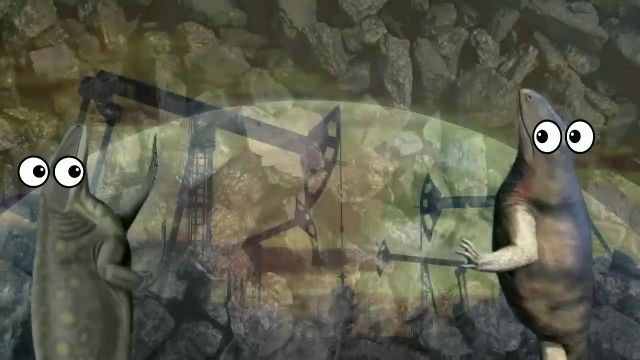 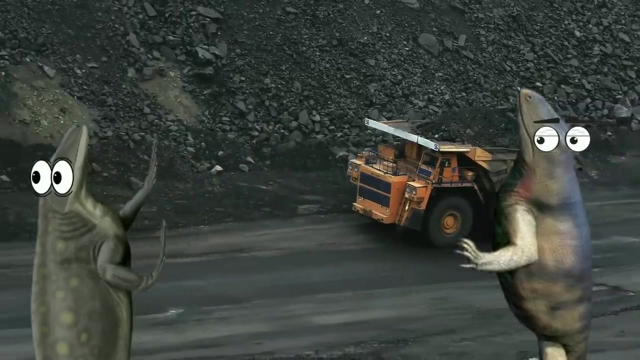 And I can't help but notice that you've picked a form that's particularly good at running. That's right, And I now have a little idea for the next episode. I'm excited to see what's going on in the next episode, But 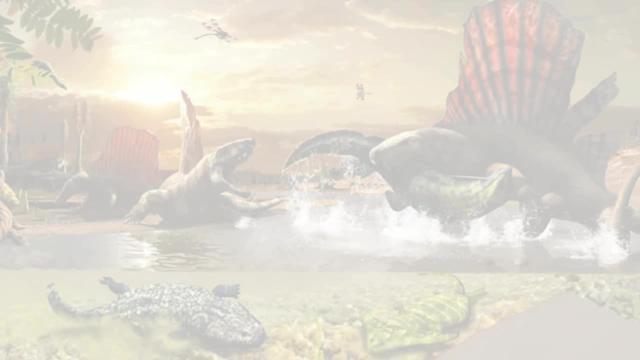 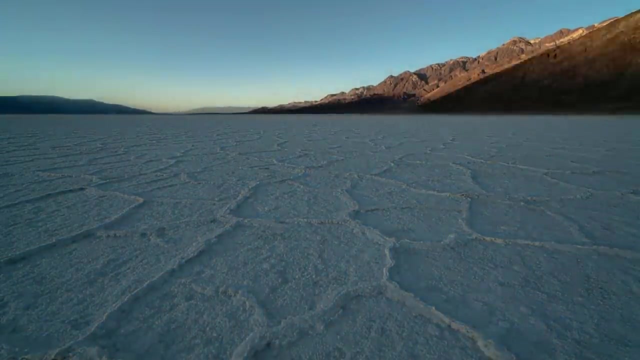 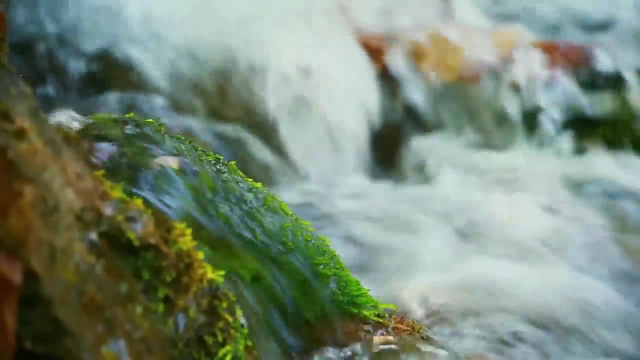 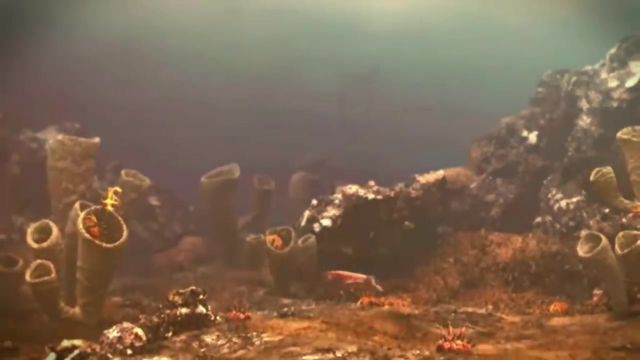 for now we come to the tail end of the Paleozoic Series. We've covered the rise of complex multicellular animals in the Ediacaran and the Cambrian Explosion, And ever since then it has seemed like the torch of world domination. 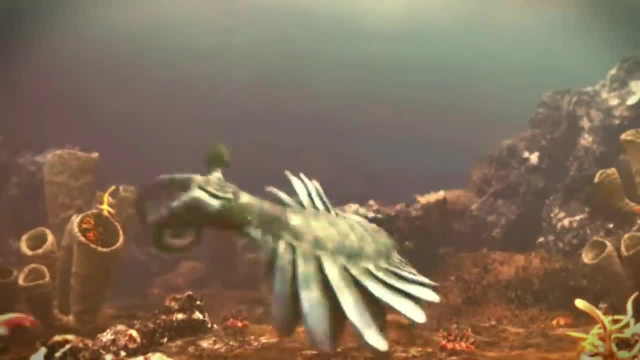 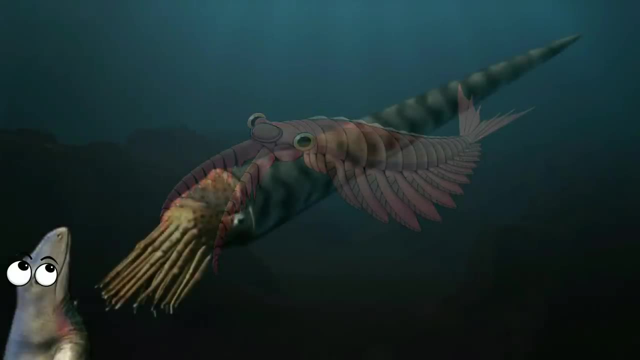 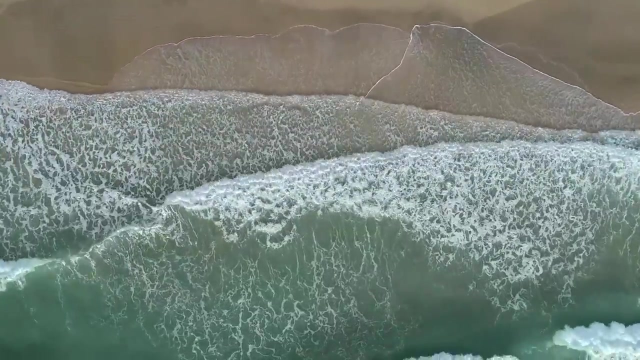 has been passed every couple of million years, Starting in the oceans with the Cephalopods, the Eurypterids and the Placoderms, And all this conflict beneath the waves had led to different groups slowly colonizing the land. 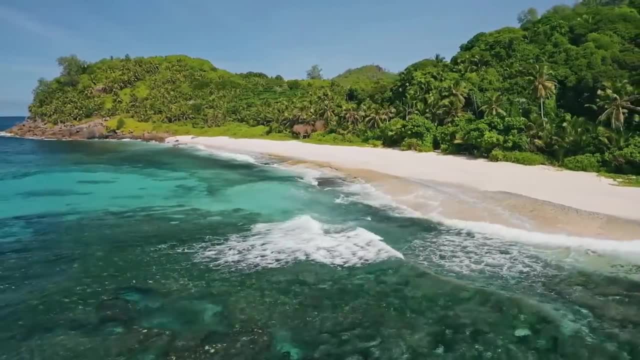 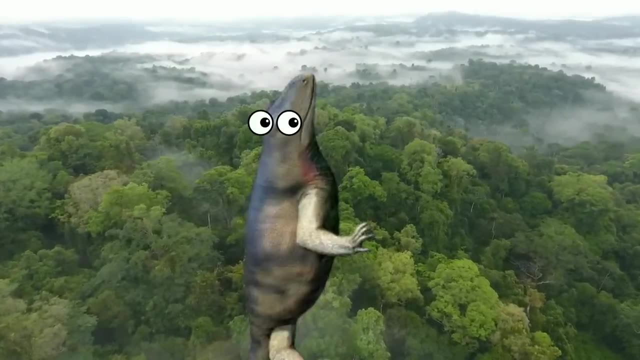 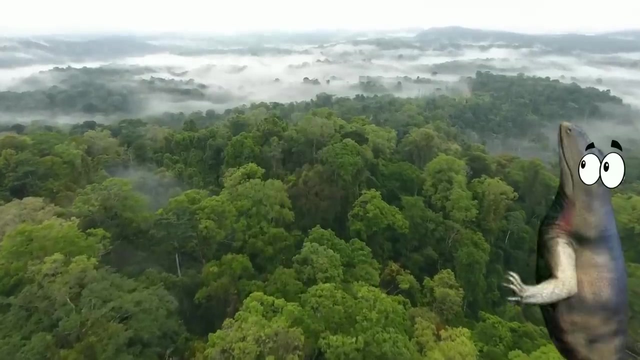 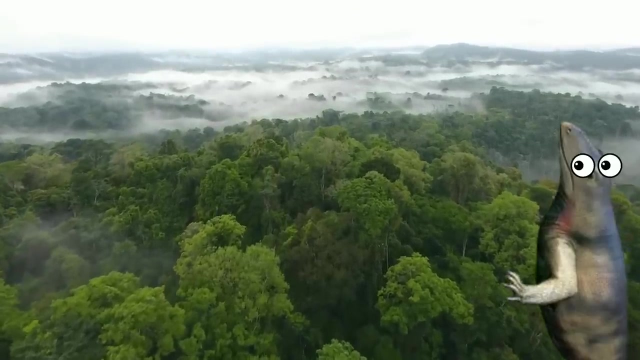 And by the time we get to the Carboniferous, we see our very first thriving terrestrial global ecosystem in the form of a rainforest in the middle of the ocean. The climate, the atmosphere or the continents moving around has always seemed to shuffle. 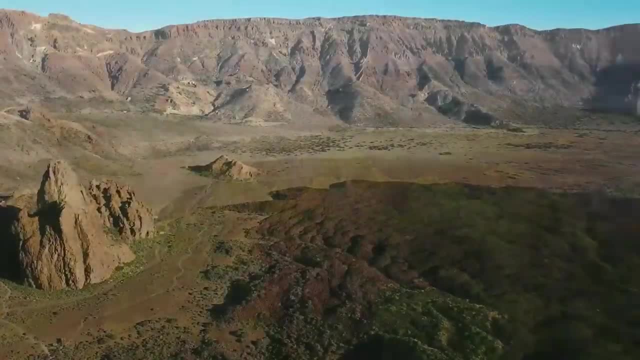 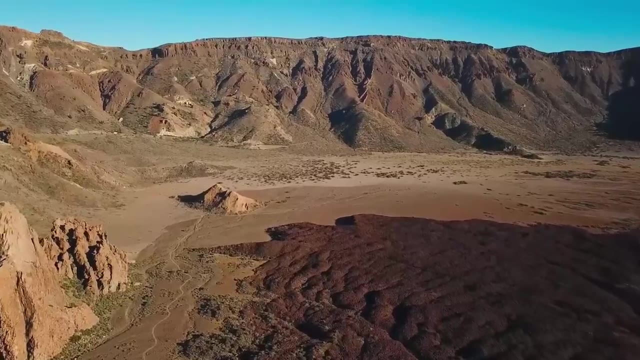 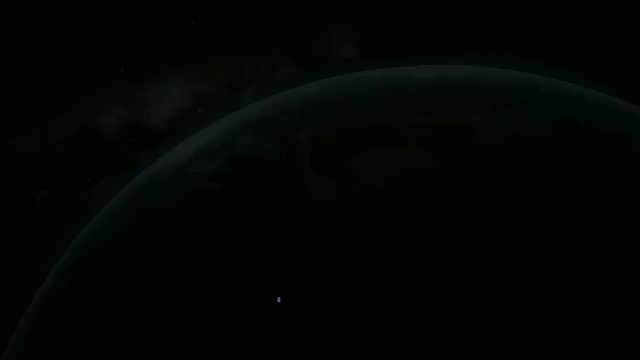 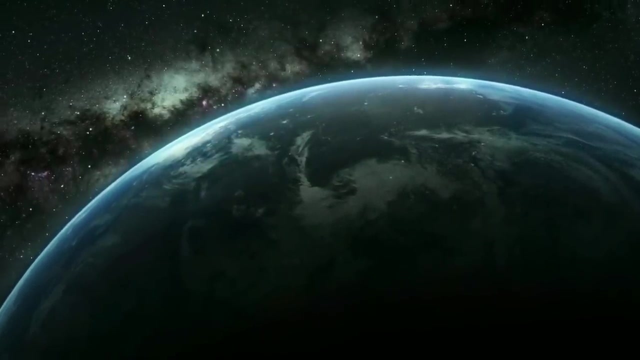 the cards, and every time new animals would end up on top, And most recently, it seemed like our ancestors were finally being dealt a good hand. So let's continue our journey through the Permian, Going into the Permian. the continents were continuing. 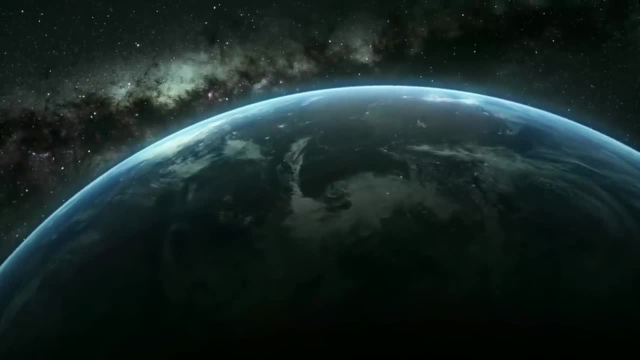 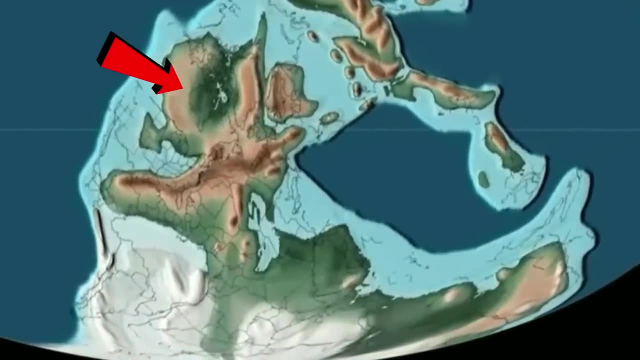 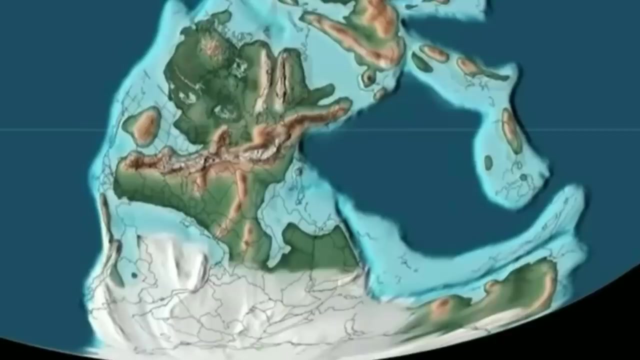 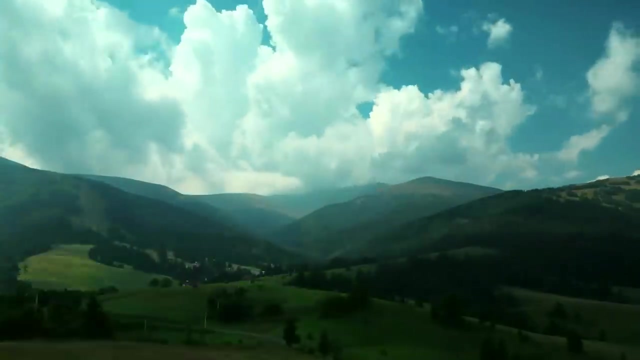 on the same path they had started on millions of years before, And this would lead to several changes to both the climate and the landscape. For one thing, the landmasses of Gondwana are a very powerful scene on Earth since the Hadean. 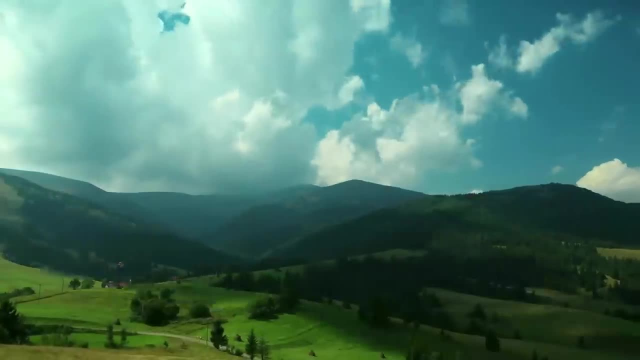 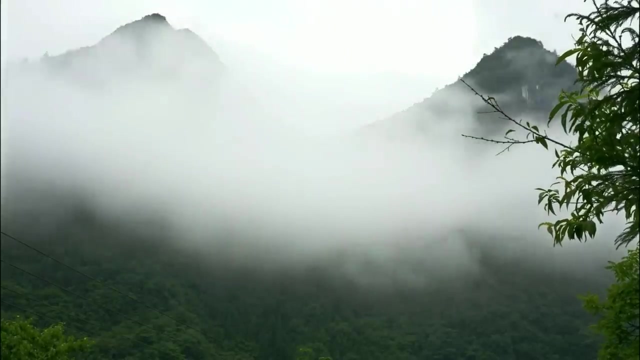 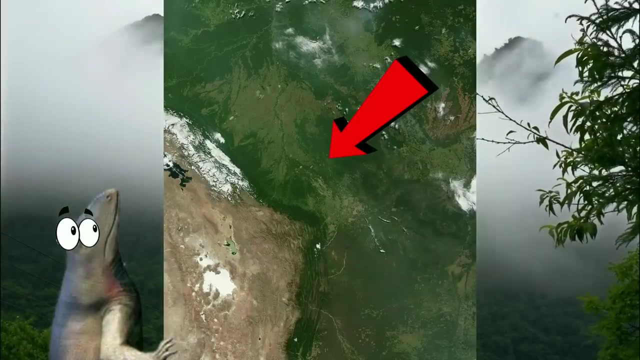 and Archean eons. Now, one thing about large mountain ranges is that they can have a very drastic effect on the regional climate, Because if a mountain range becomes tall enough, it can literally block moisture from getting past it. That's why, when you look, 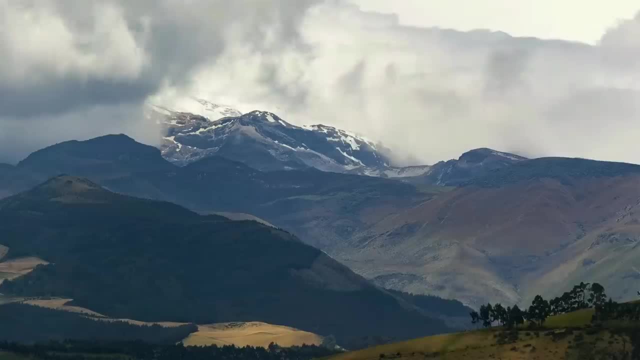 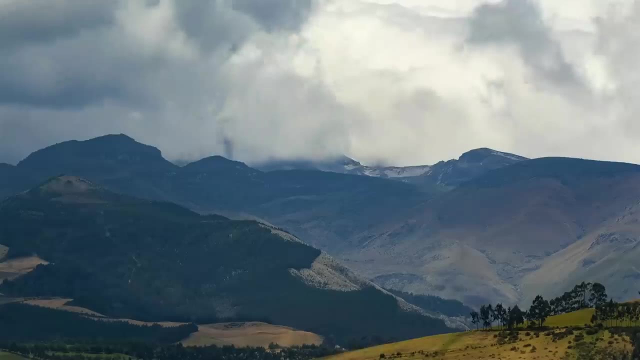 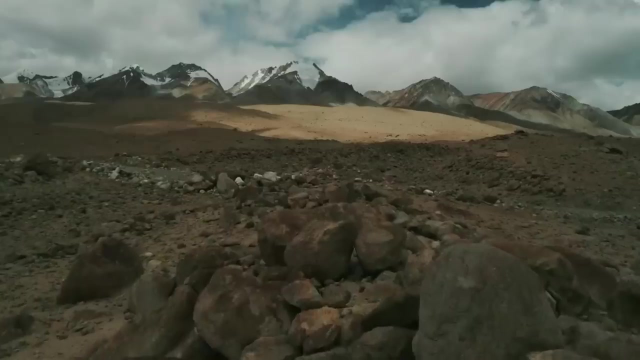 at a map. this is called the rain shadow effect, And in a situation where there was already a limited amount of water making it to the interior of the continent to begin with, this would create a situation where there would be two drastically different environments. 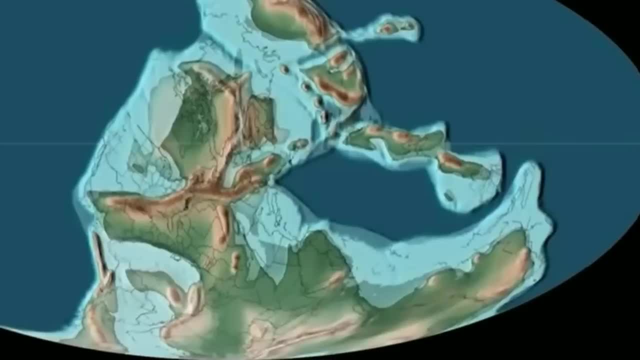 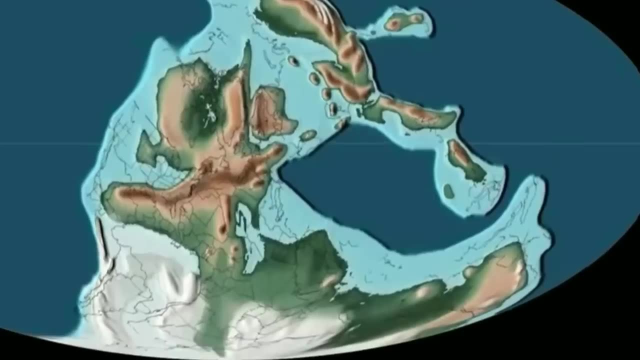 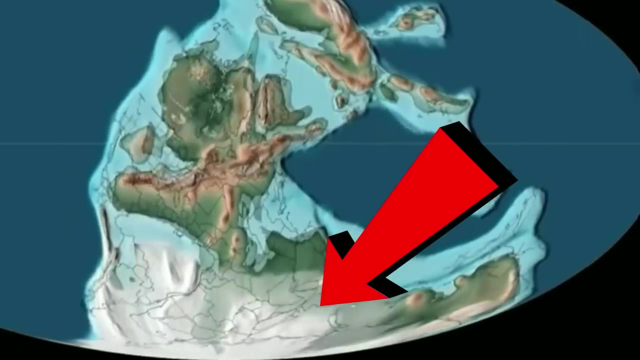 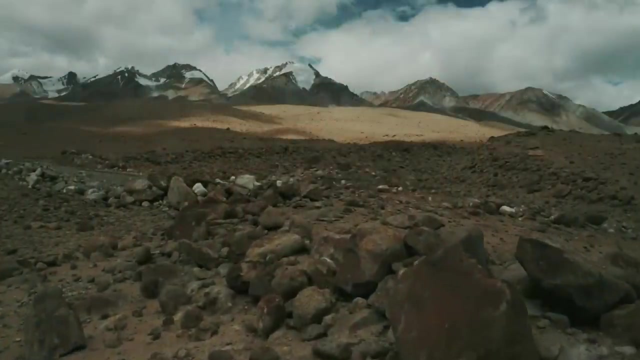 The lush coastal tropical forests and the massive desert in the late Carboniferous had now led to a full blown ice age in the early Permian, known as the Late Paleozoic Ice Age. This one spread glaciers across the southern continent of Gondwana. 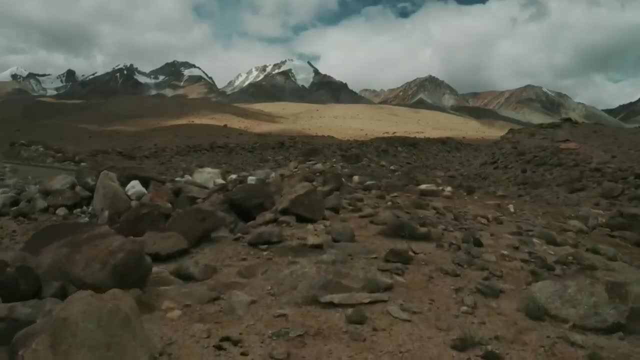 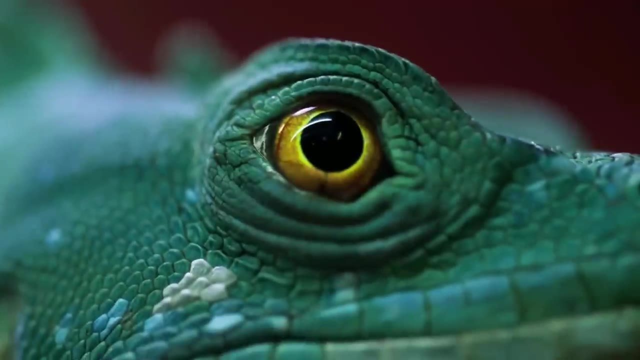 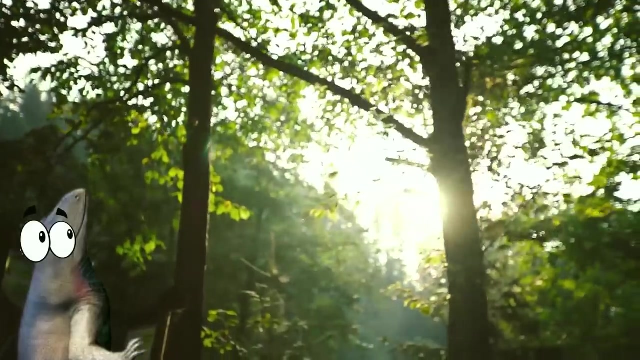 So this actually led to even more climatic extremes, with so many different environments around them. But there was an issue: Up until this point, everything alive on Earth was exothermic or cold blooded, Meaning that they needed to warm their bodies. 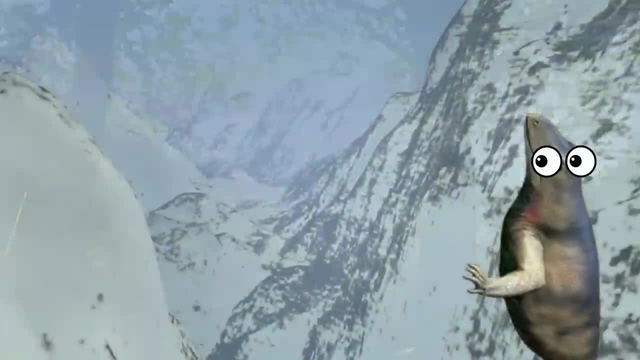 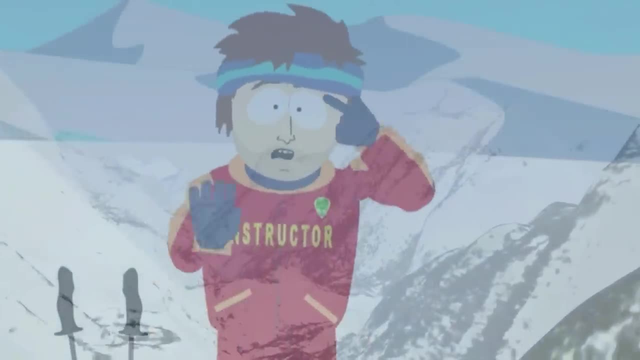 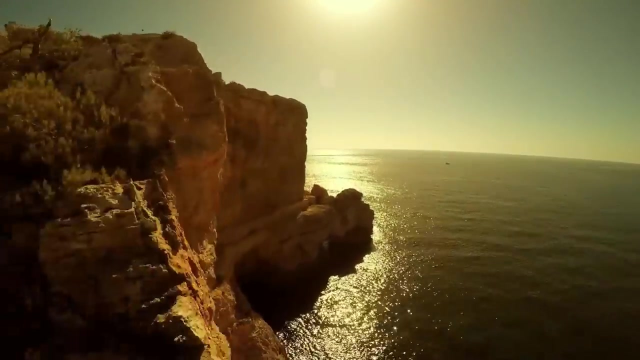 with the heat of the sun to be able to process their food and fuel themselves. Fortunately, if you're exothermic and you live on a world that is in the grip of an ice age, you'll be able to do much more than that. 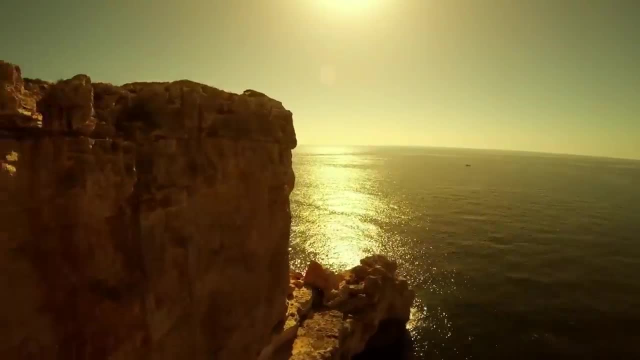 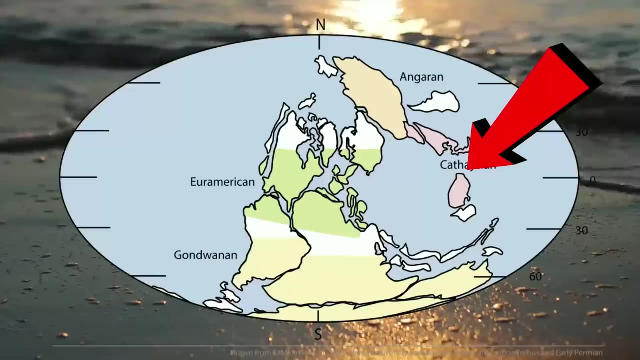 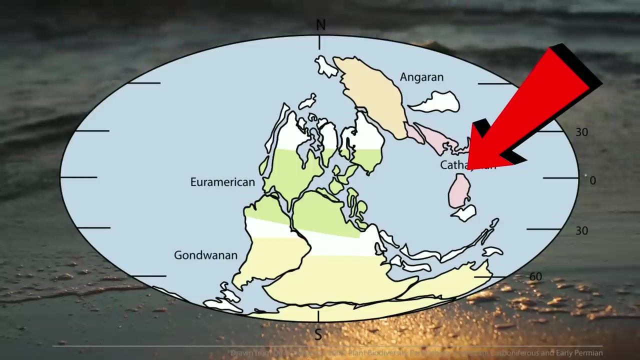 But before we get into that, let's check back in with life in the oceans. With the growing glaciers at the South Pole dropping the sea level, this caused the island land masses, like what would one day become China and Southeast Asia- to grow to land masses. 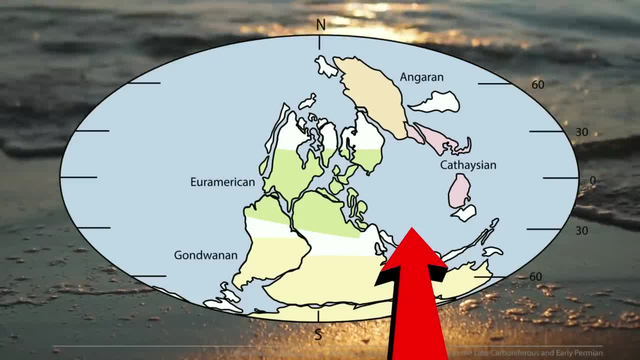 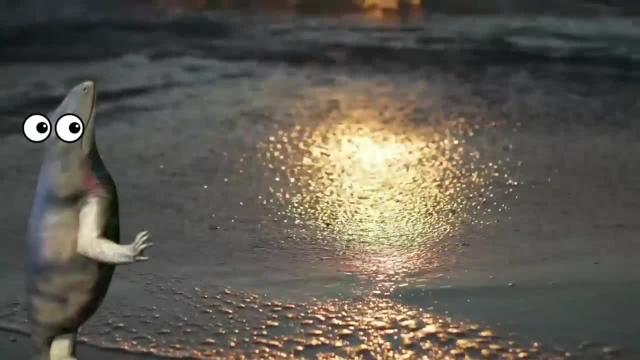 nearly the size of Australia. This isolated the Paleotethis and this likely led to a division in the evolutionary paths from the animals living in each. And I say likely because it's hard to say 100% for sure, because we don't actually 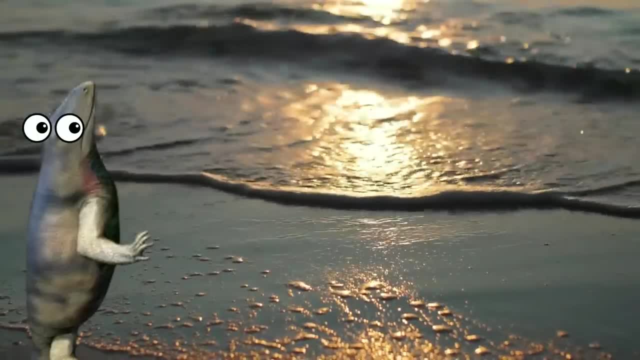 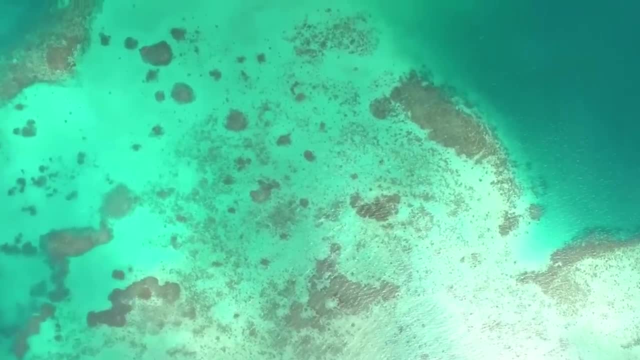 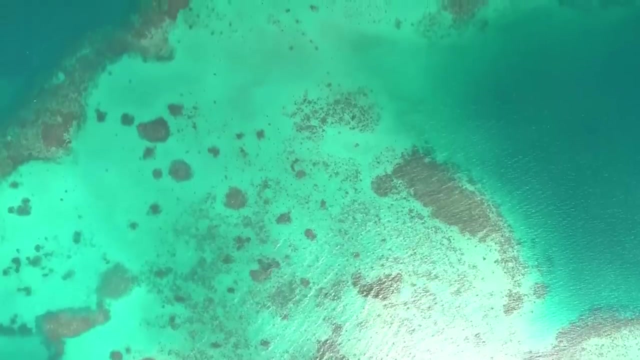 have a ton of fossils from the panthelassic ocean, during this time at least, of large animals. Almost all of what we know is from the more shallow Paleotethis, And here we see that some forms of life had managed to bounce back. 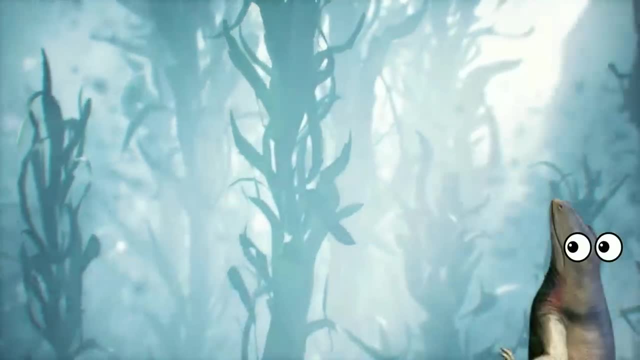 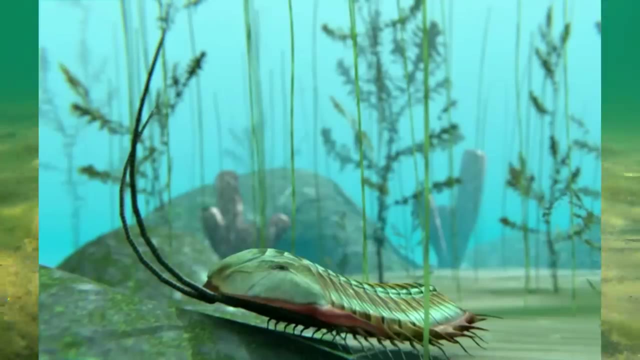 after all this time, One that still managed to hang on were the ever persistent trilobites who, despite becoming exceedingly rare on a sea floor covered in mollusks, echinoderms and brachiopods, were able to eke. out a living in a handful of different species. They just won't die. They're like sea cockroaches Pretty much. No matter how many times they've been killed, they're still alive. The only species that survived this time was a particular 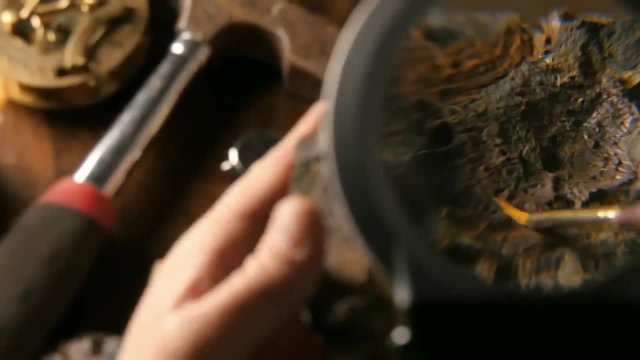 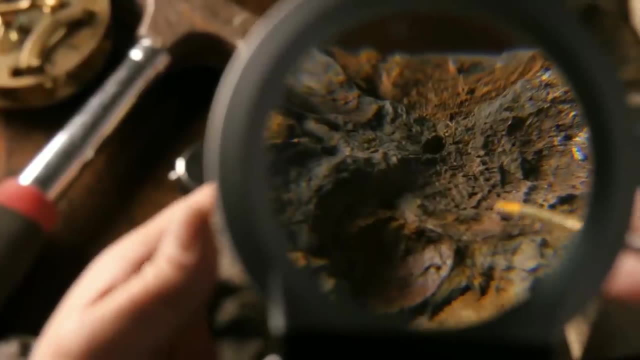 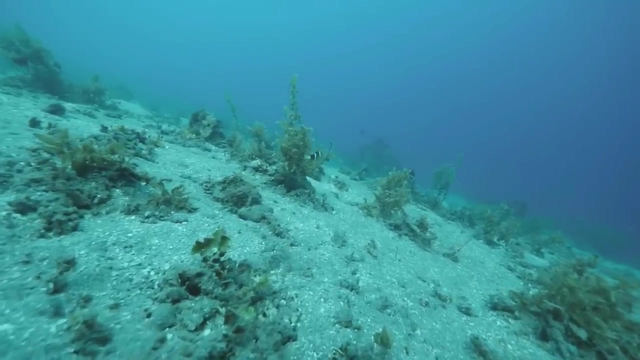 kind of ammonite called goniatites. Now, this was an older order of ammonite, but it was definitely their golden age. They're so common in early Permian marine fossil layers that paleontologists actually used them as an index fossil to identify. 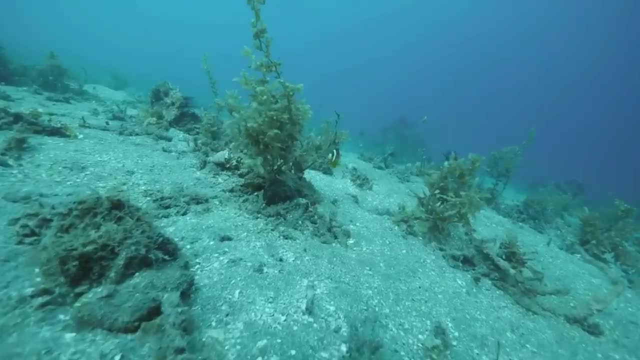 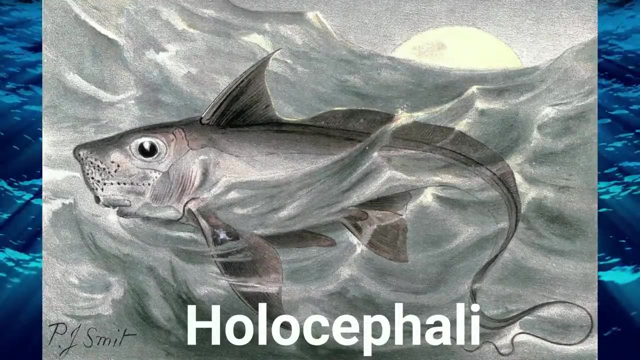 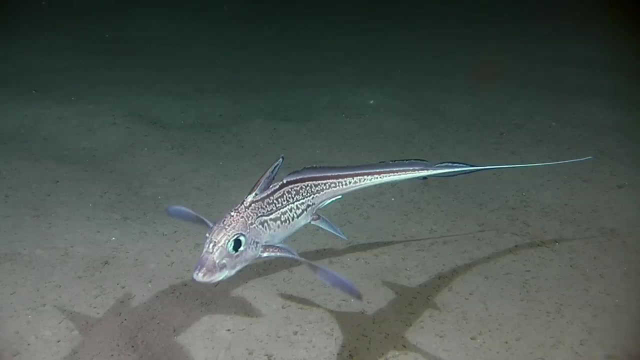 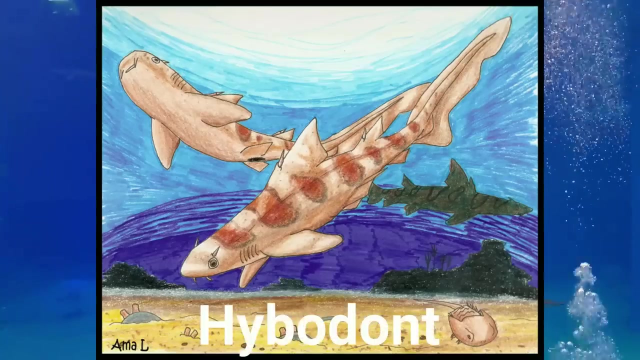 other species that were living in the ocean. In the early 1st century, the Chondrichthians were taking over and diversifying, Especially a clade known as holocephaly, which is a clade that is not very well represented. 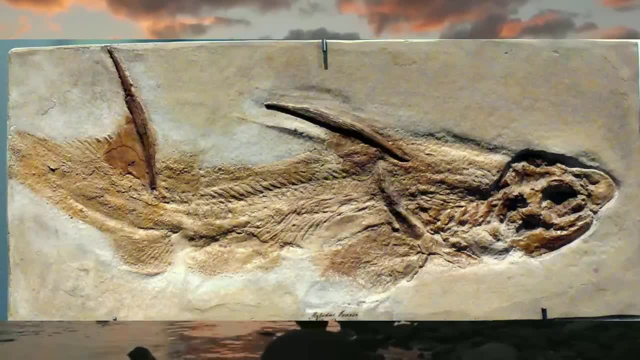 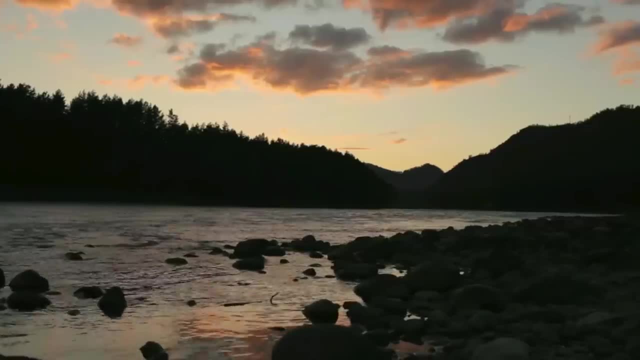 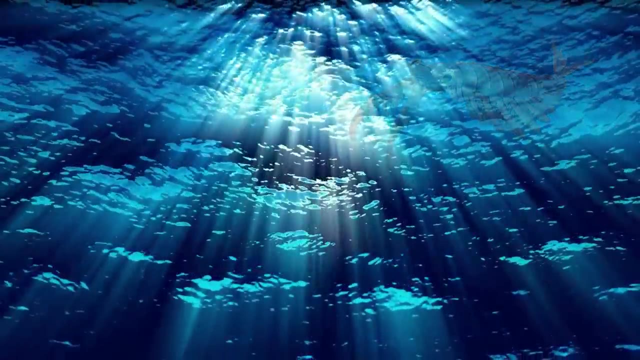 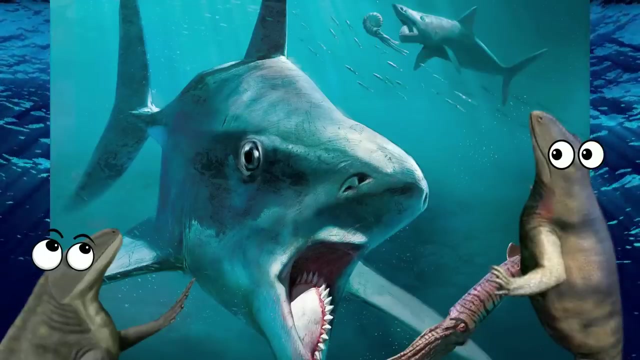 today, but does contain a few of the most common marine fossils in the world. The Chondrichthians were known for taking refuge in freshwater environments from the true top predators of the ocean, the Eugeniodontids. And, if you thought, 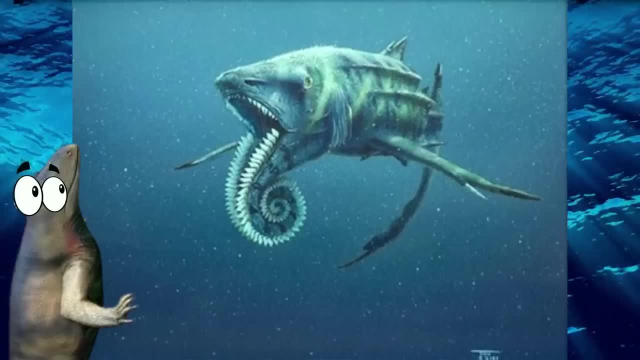 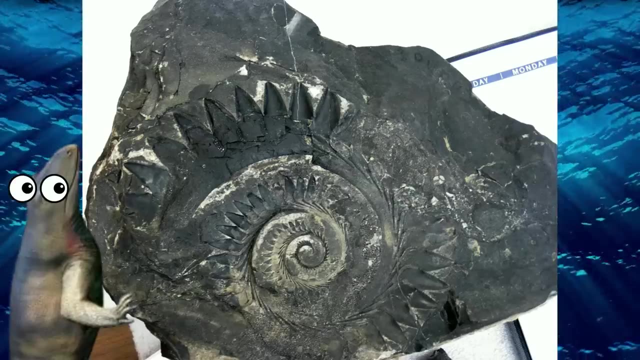 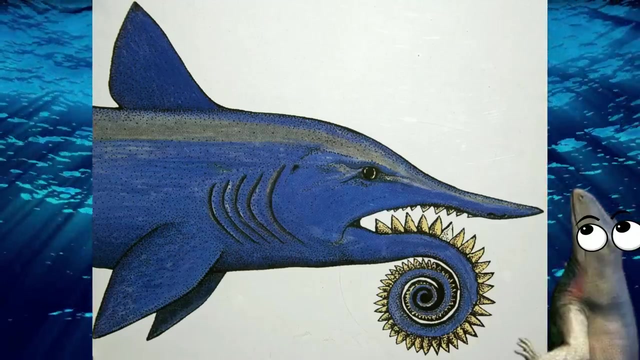 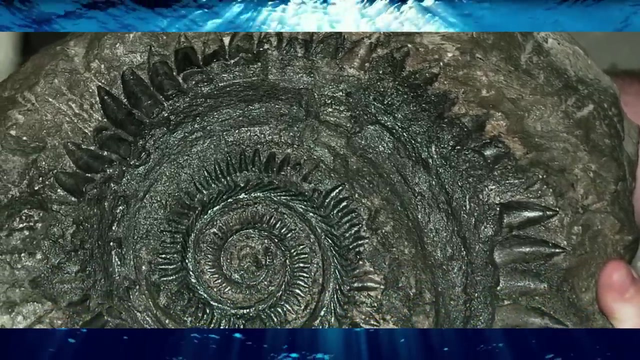 that armored fish, sea scorpions, carrot snails or sea snails were found in the ocean, then you are wrong. The Chondrichthians were known for taking over and diversifying in the ocean. The Chondrichthians- 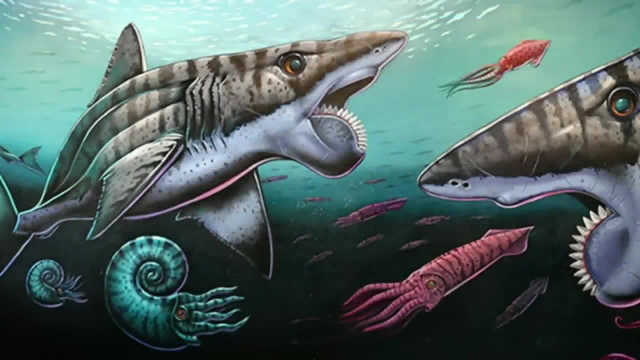 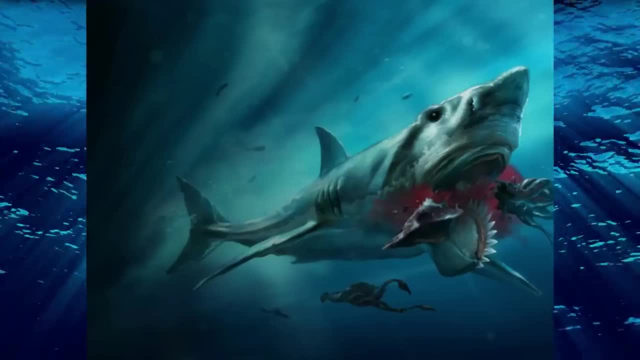 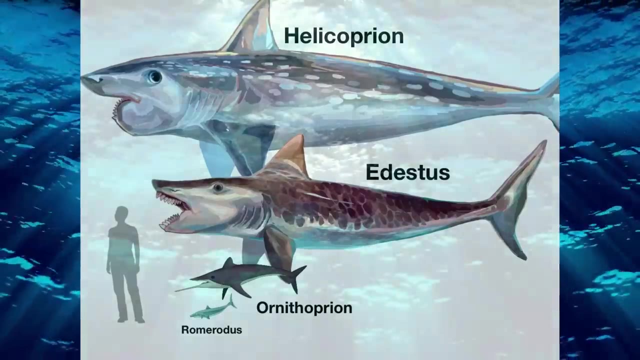 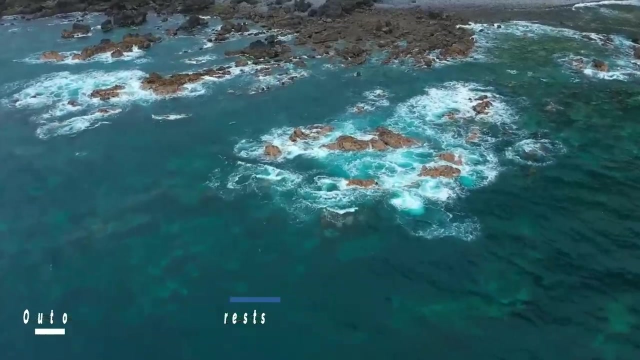 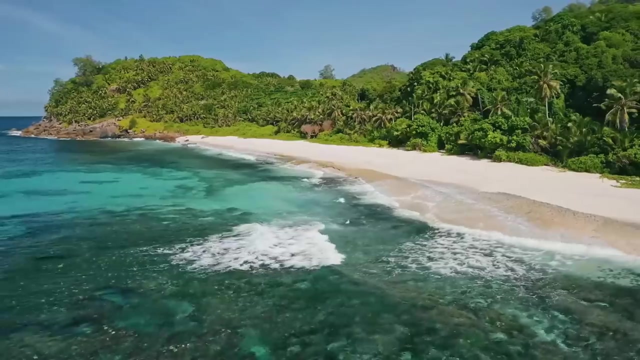 were known for hunting the most common prey available, the guniatite ammonites, But at up to 8 meters long, this animal was very likely the unchallenged king of the early Permian seas, As we saw in the last episode. 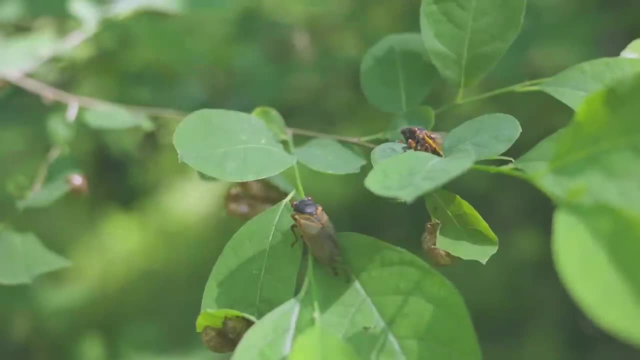 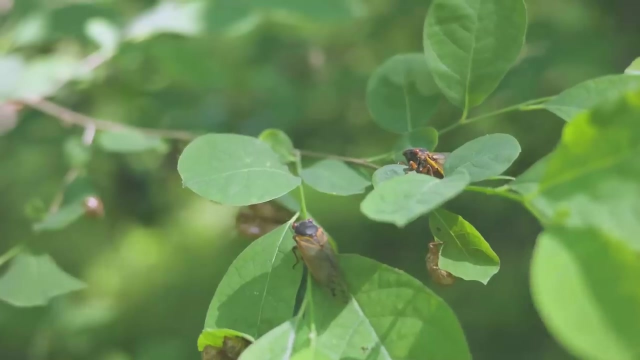 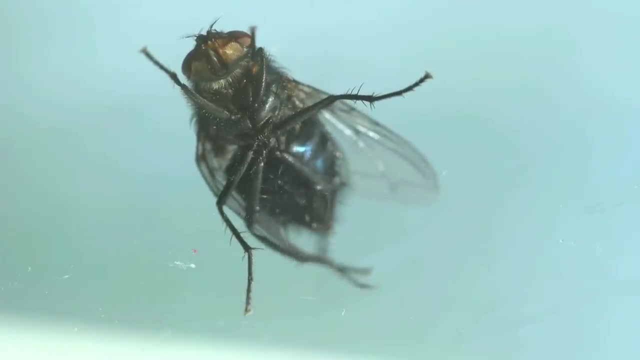 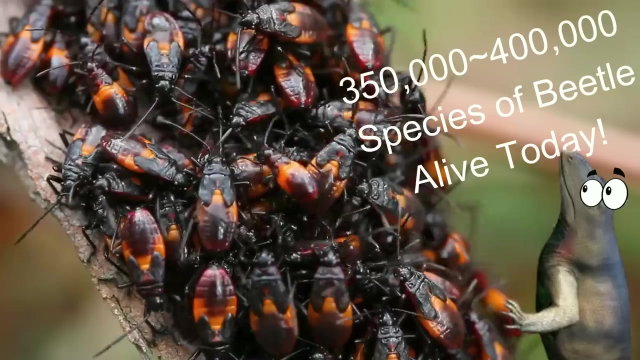 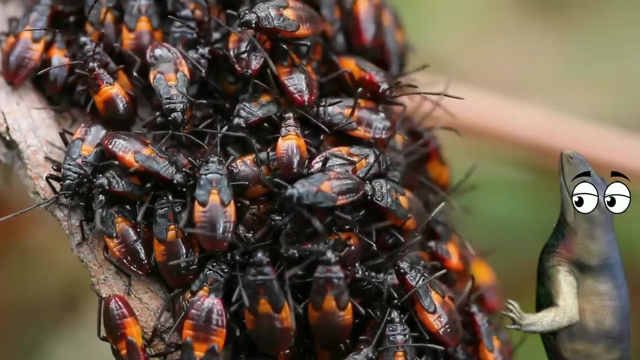 the Chondrichthians were known as the giant arthropods, but this was definitely a very different world Because there was less oxygen. the age of the Chondrichthians was very low. The Chondrichthians were known. 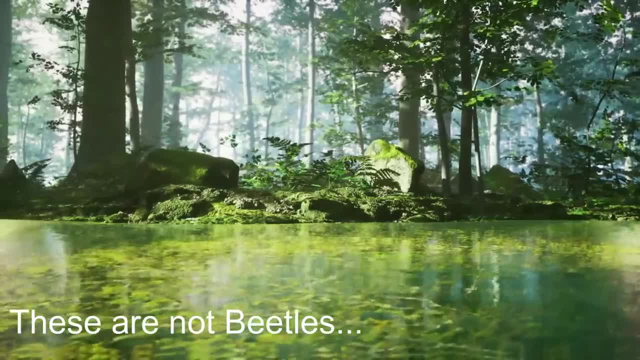 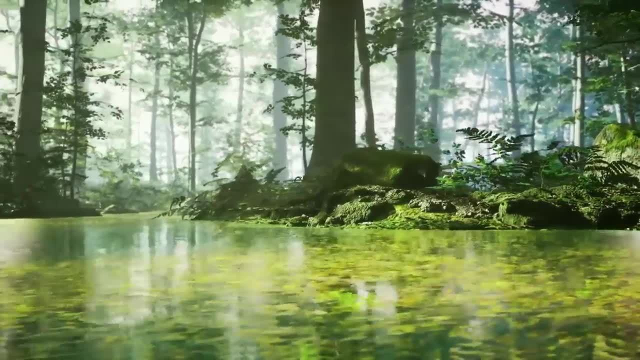 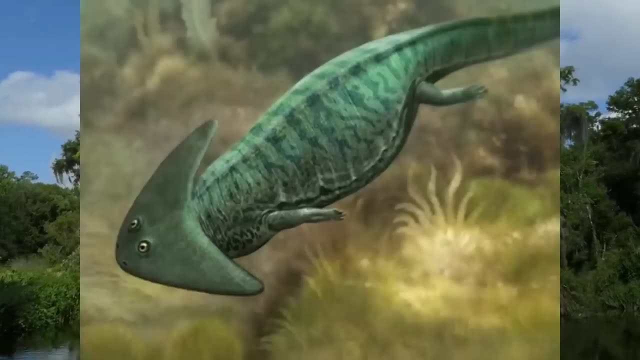 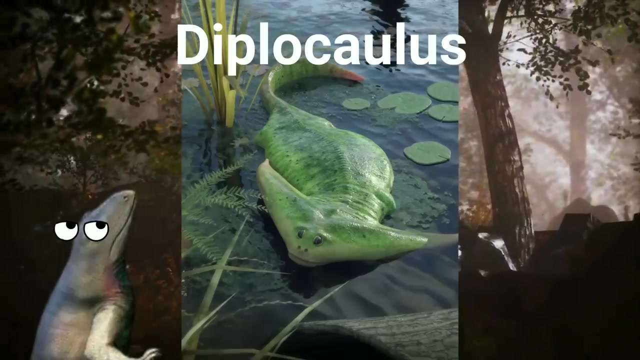 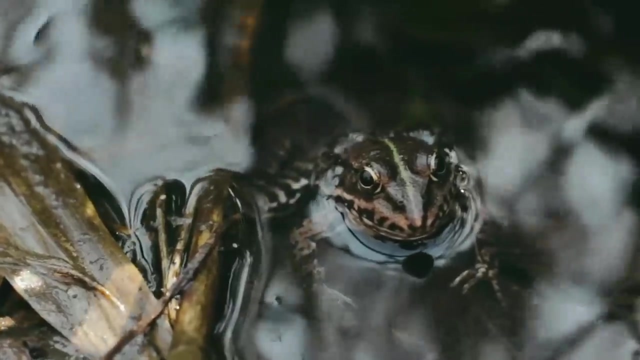 as the most powerful species of the Chondrichthians. They were known as the most powerful species of the Chondrichthians. The Chondrichthians were known as the most popular species of the Chondrichthians. The. 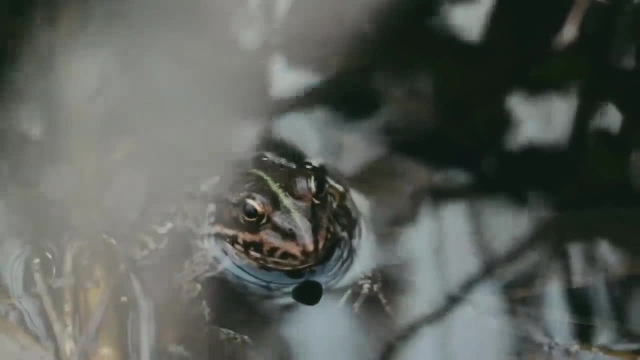 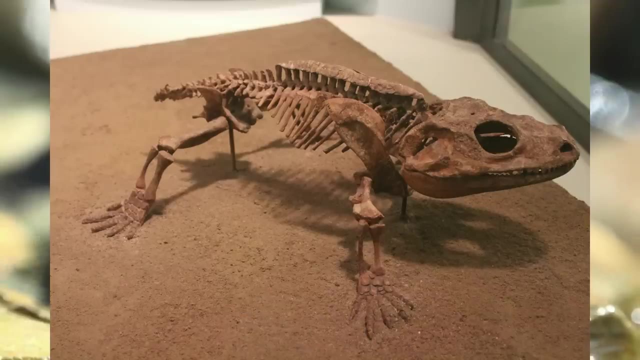 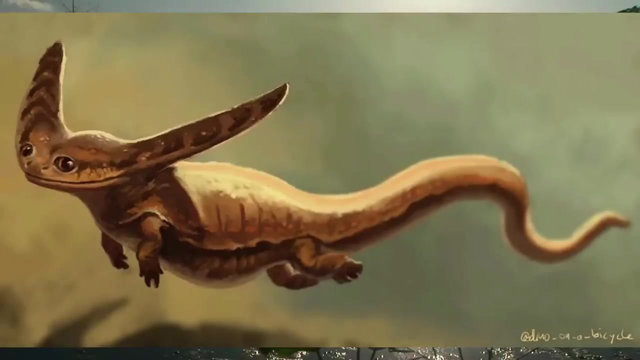 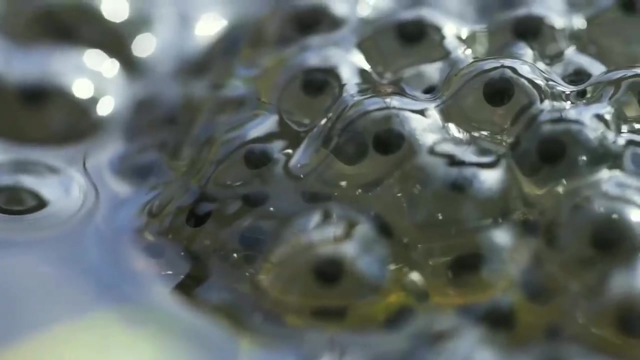 Chondrichthians were known as the most powerful species of the Chondrichthians. The Chondrichthians were known as the well. the fact is that they could not spread to an overwhelming majority of the land because they were still tied to the water and they would also struggle. 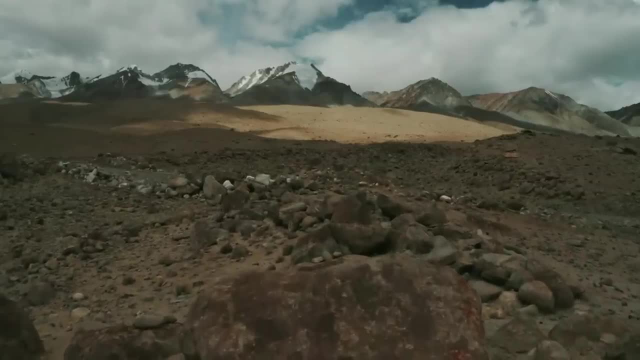 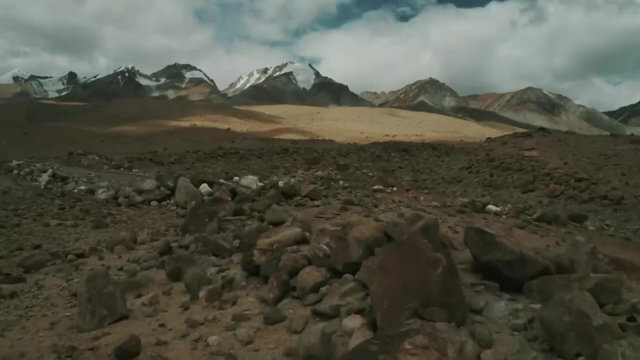 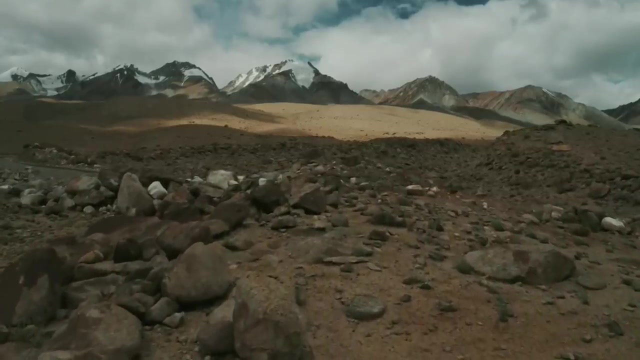 to adapt to colder regions, which at first was actually something that everything on earth was struggling with. But perhaps the fact that the world was in the grip of an ice age was actually the thing that pushed some animals to make a change. That is one of the theories behind a standout feature that 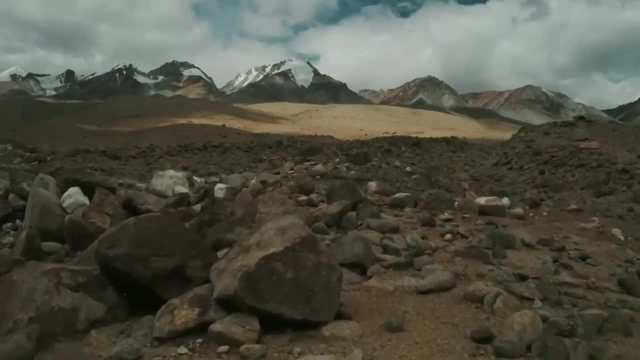 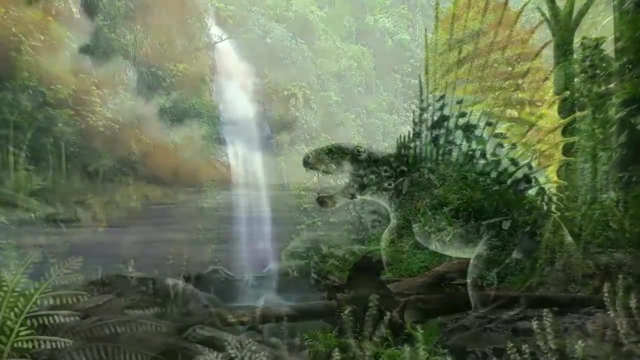 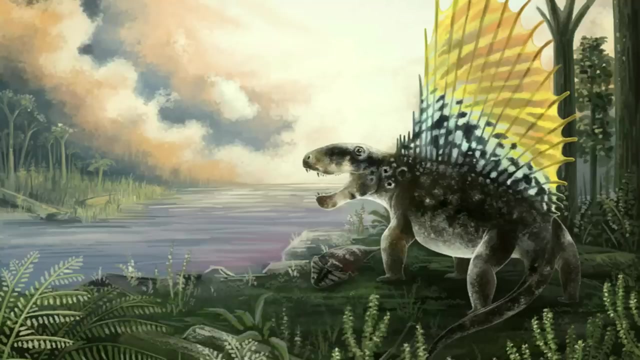 first evolved during this time period with some of the most famous Permian animals, especially one of the top predators of the early Permian, the Cephenacodontid Dimetrodon. This was one of the various different families of synapsid who were diversifying during this time, and although this species was 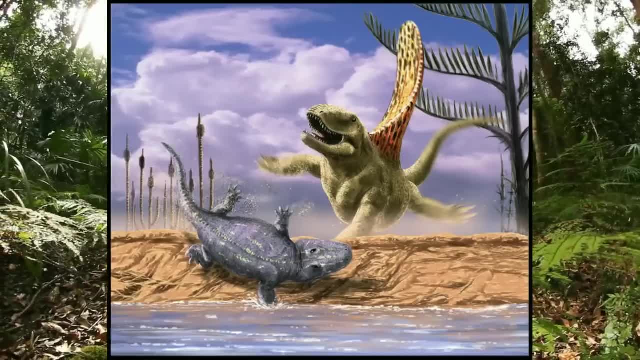 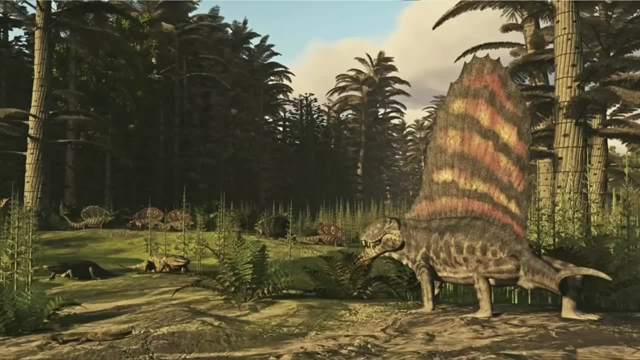 primarily a hunter of amphibians in the swamps, where it probably mostly lived. it is thought that their ability to regulate their body temperature more than the average person would have been able to do so. The fact that they evolved more effectively than any other group of tetrapods at the time is what gave them the edge in the wildly different 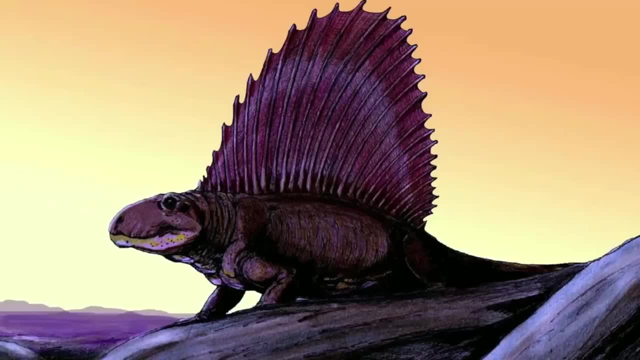 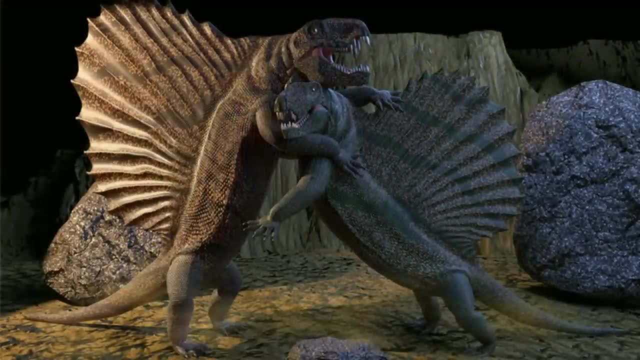 climates of the late Paleozoic Ice Age. We're not sure if Dimetrodon's sail was an adaptation for thermoregulation or maybe just used as a sexual display, but what we do see is that there were several different animals, especially. 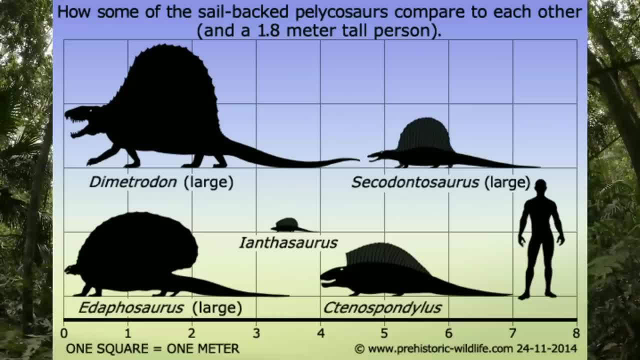 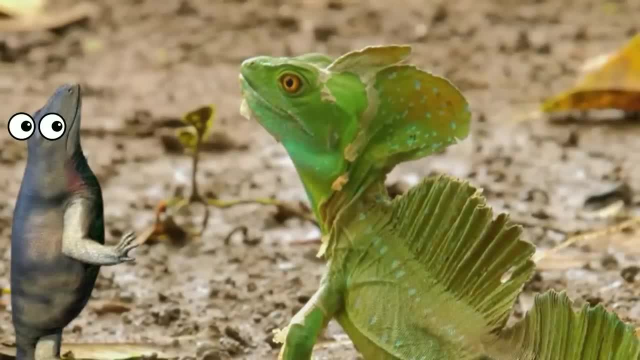 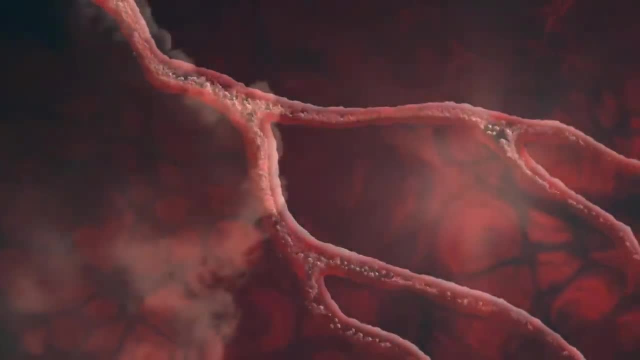 among the early synapsids that evolved this feature independently. I mean, if I'm being honest, it could have been better. After all, we see lots of reptiles today using sails as a sexual display. but we also know that the sail would have been packed with blood vessels. so when blood moved through the thin membrane of 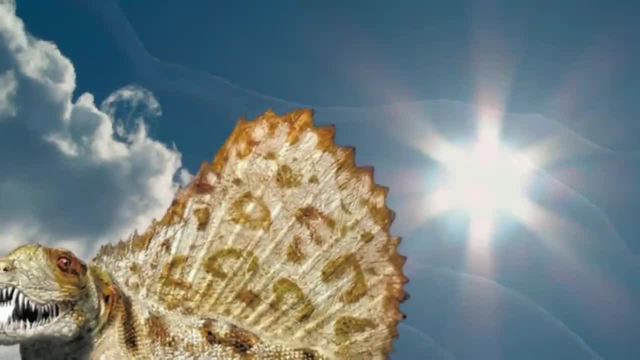 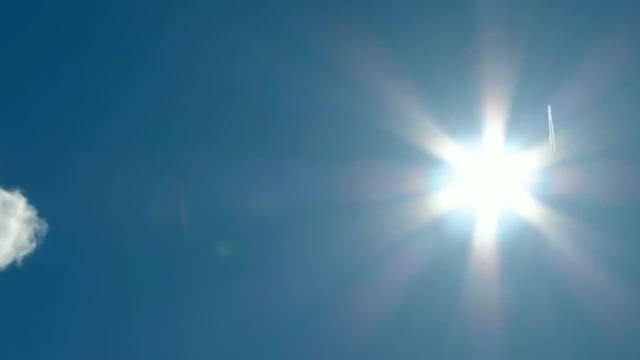 the sail and the animal was sunning itself, the blood would start to warm, So this could have been the first steps toward the very first group of animals becoming endothermic or warm-blooded, and this would be the thing that allows these animals to take over the world, as well as the 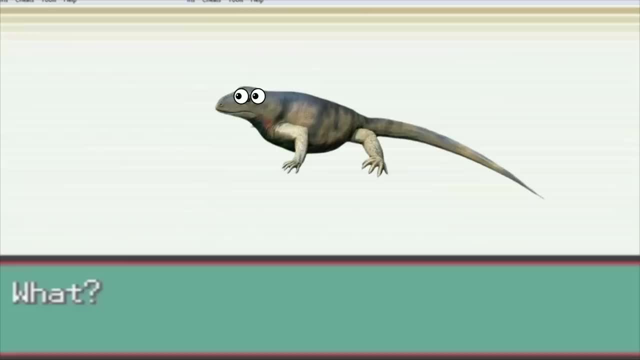 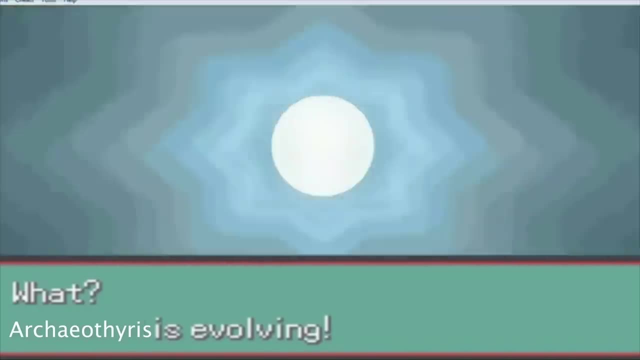 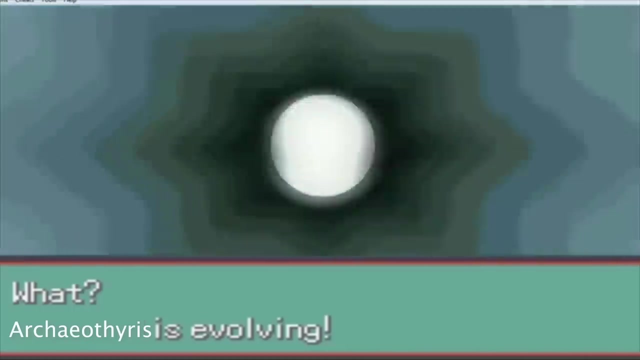 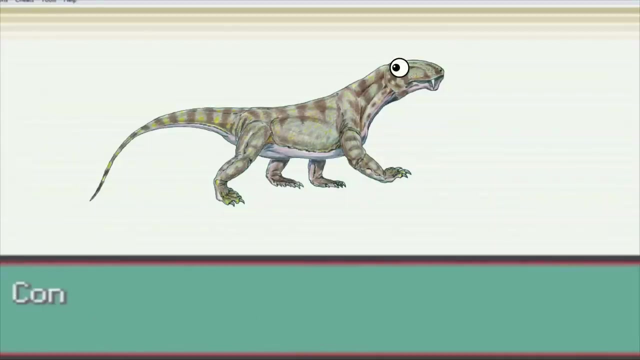 thing that allows me to be able to live in the world I want to be able to live in the world I want to live in. Why do you all care if my character stands upright? Alright, now at least I don't have flounder eyes. 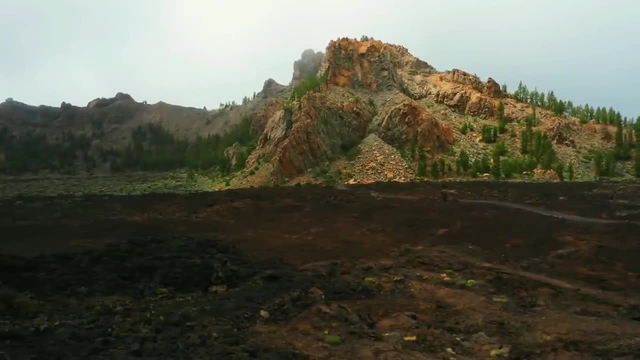 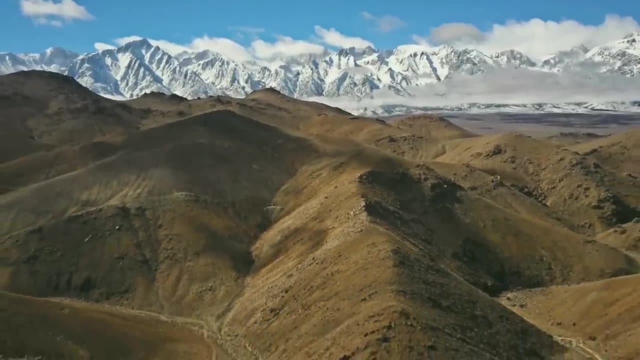 Across the warmer, arid regions of Pangea. the diapsids and synapsids were on the rise, and they were starting to get larger as well. This would be most evident in the first group of large herbivores to lumber across the land, the diadestids like Desmododon that have been 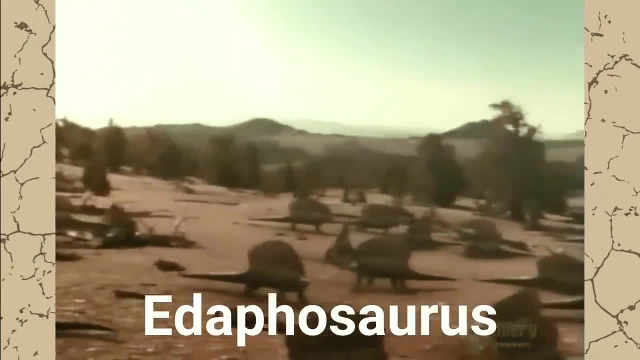 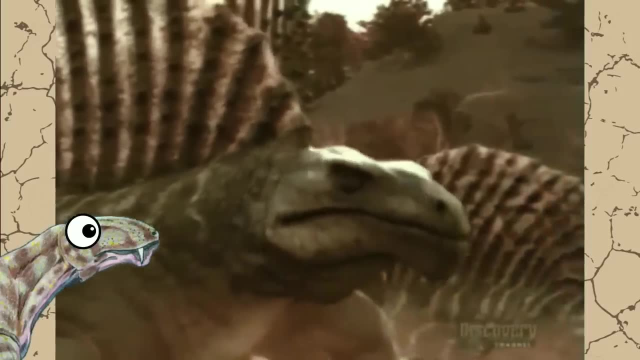 around since the Carboniferous, along with the sail-backed herbivore Adaphosaurus, which, despite the resemblance, is actually only a distant relative of Dimetrodon. Of these groups, the ones that lived in the swamps and forests were likely prey for the 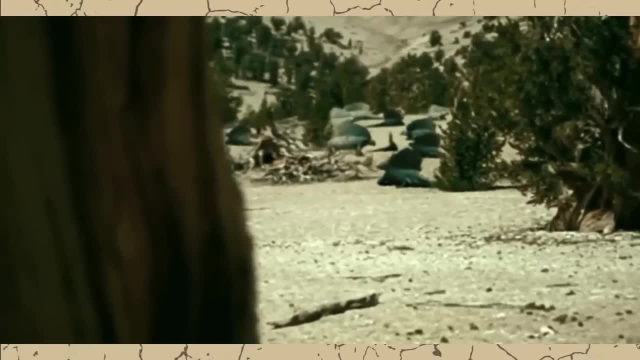 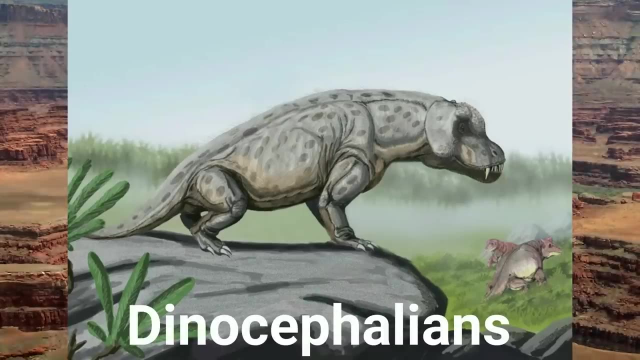 sail-backed carnivore, but for the ones that expanded out into the desert, they would be facing a very different threat. Another group of carnivorous synapsids called the Dinocephalians. This was one of the first groups to rise up during the beginning of the Permian. 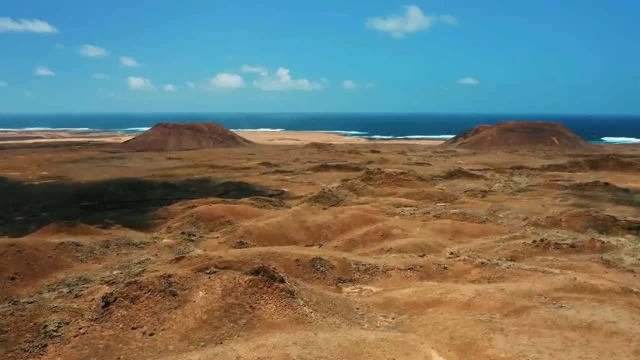 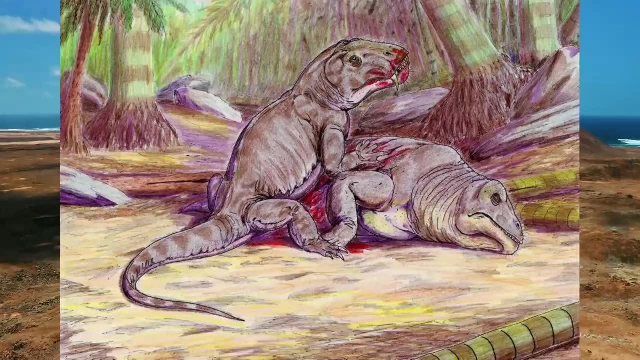 and they started to diversify into many different forms. There were herbivores like the dome-headed Tapinocephalus, which grew to the size of a tree, and the Dinocephalus, which grew to the size of a black rhino, and the largest carnivore of the period, Titanophonius, which was bigger than a. 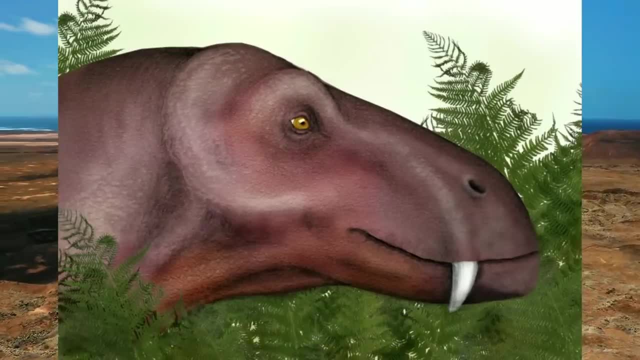 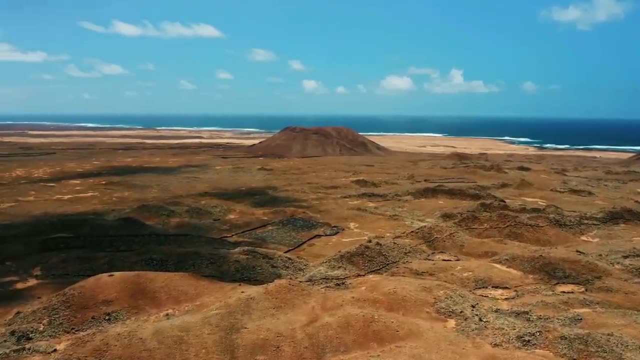 tiger and had a pair of pronounced canine teeth that it would use to dispatch its prey, And there were even some species of omnivores eating up mix of both plants and animals, like Titanosuchus. There were even some that did spread into the coastal forest and become semi-aquatic. 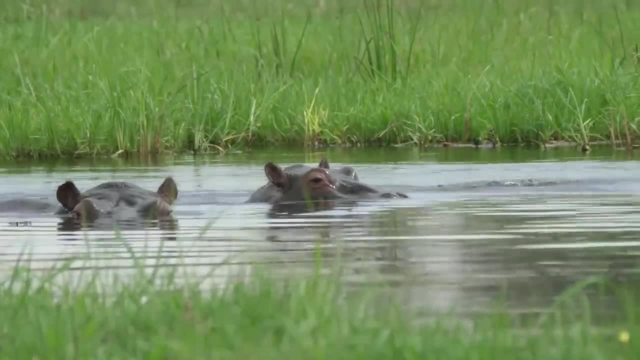 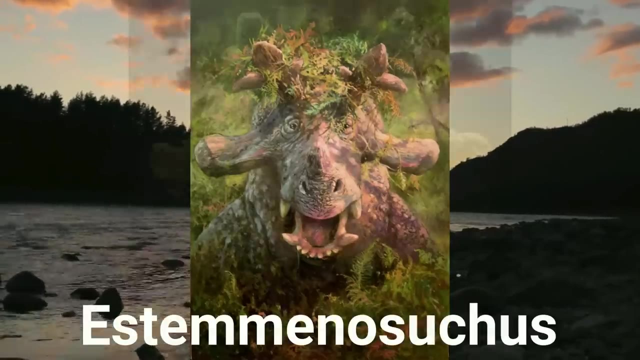 returning to the water and living similarly to crocodiles and hippos in this regard, And these would by far be the most common species of omnivores in the world. But there were also some that were the most bizarre, Like look at this thing, It's called Asteminosuchus and, as you can see, 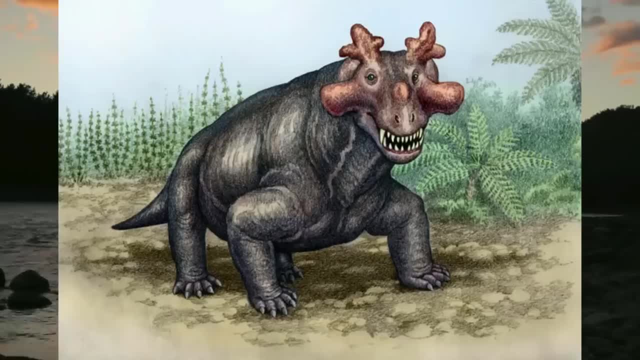 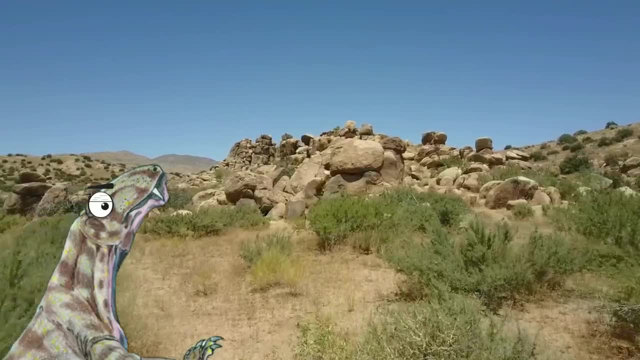 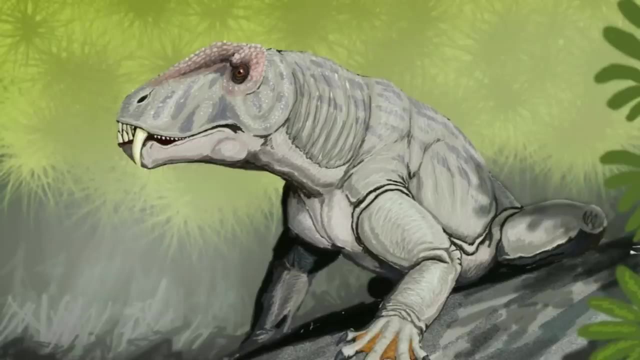 it quite literally wears the crown for the most bizarre Permian synapsid. But to find a close runner-up we have to look at a different member of the synapsids from the Dinocephalians altogether, the tiny-headed herbivore Cotylohricus. As you can see through the Permian. 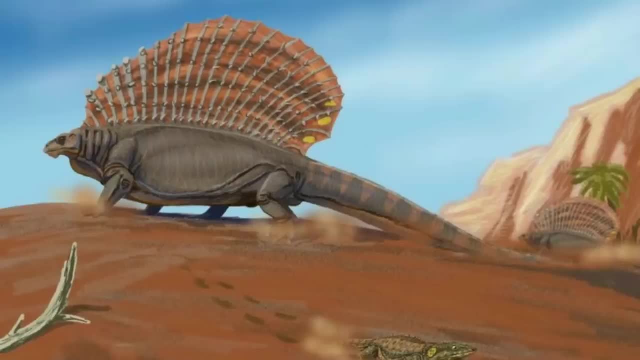 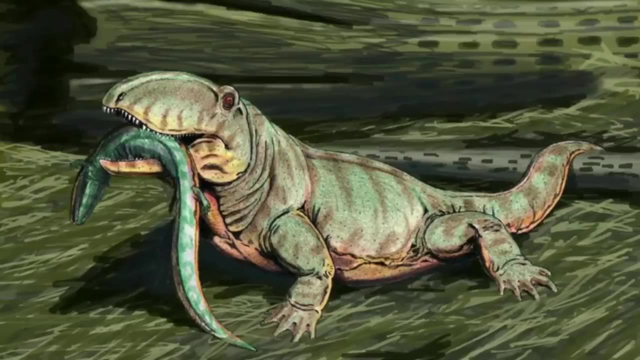 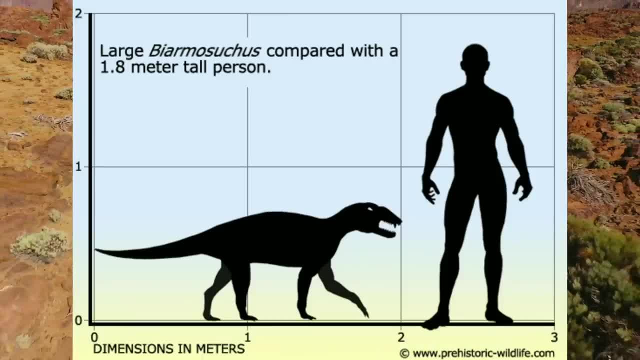 Cotylohricus Cotylohricus Cotylohricus Cotylohricus Cotylohricus Cotylohricus Cotylohricus. This animal was a dog-sized hunter who likely couldn't stand up to monsters. like Titanophonius or Dimetrodon, but was able to make a living hunting smaller prey. The larger-than-average eyes I've happened to find means that we may have been able to make a living hunting at night, when many of the larger synapsids were asleep. 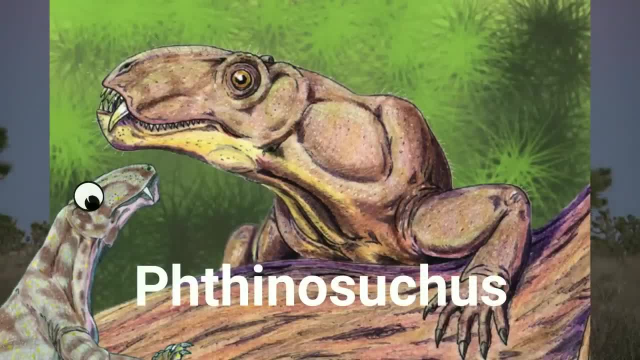 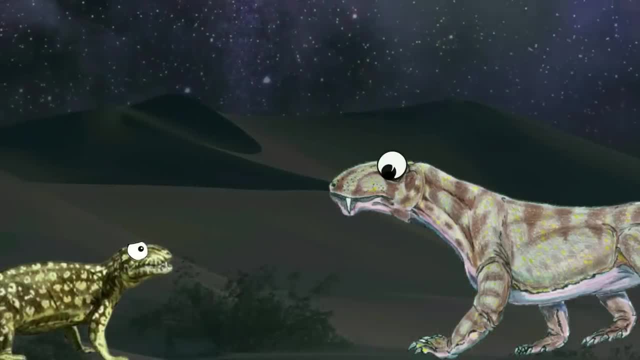 And the same goes for Phythenosuchus Fe-fe-fe-fe-feta-fre-fu-fi-fi-fi- F traffic licence, The 15th engine right Tim-Tim. Why do we keep finding ourselves in the underdog positions? 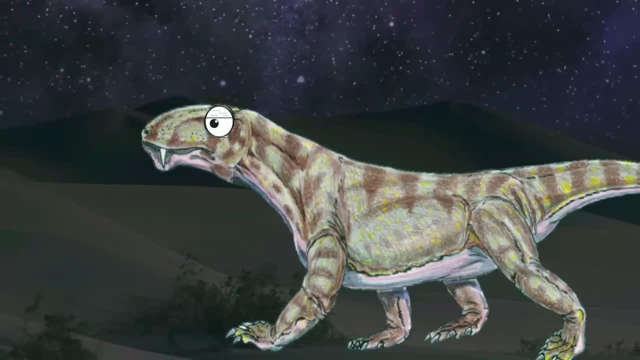 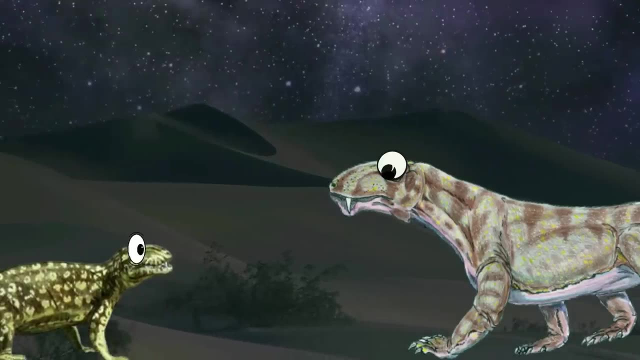 I mean, we've definitely been in worse spots. At least we can have a good strategy for avoiding all the stuff that wants to kill us. And plus, I happen to know that better days are coming. What was that What? What was what? 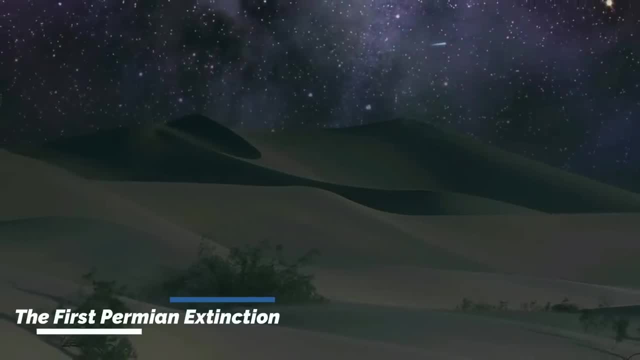 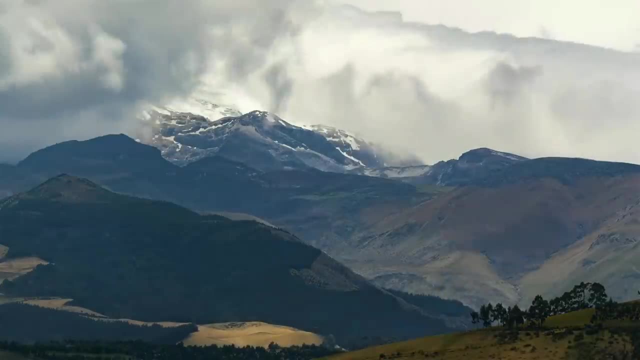 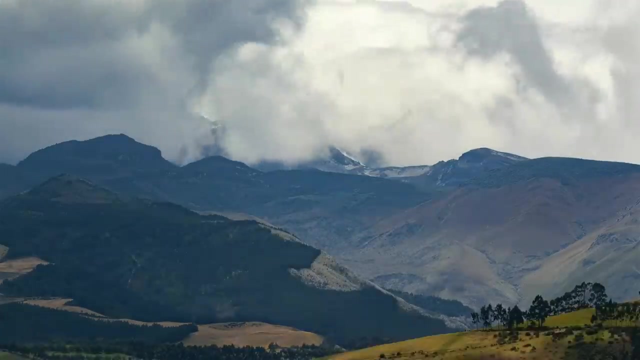 as we come around to 273 million years ago. there would then be a shift in the climate. we have seen a world populated by cold-blooded animals adapt and thrive in a world in the grip of an ice age, but it was gradually getting warmer again, and as much as the animals did an excellent 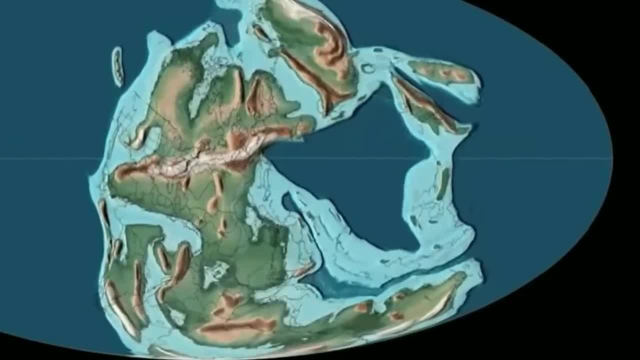 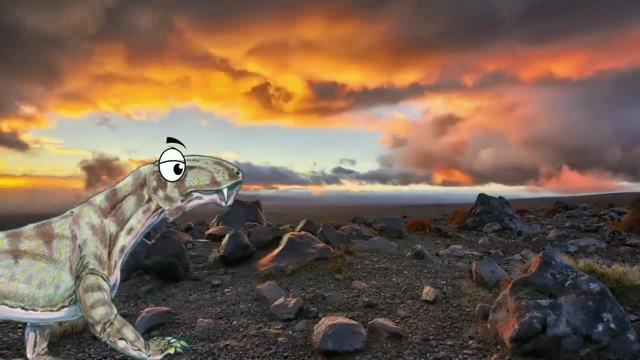 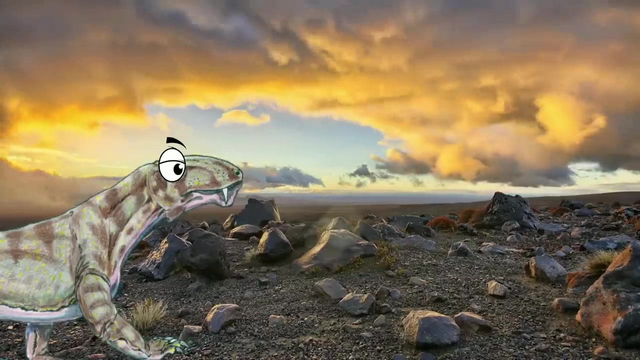 job, expanding into every possible niche over the past 25 million years now. those animals were specialized to the world as it was at the time, and things were not going to go as you might expect either. one would think that the melting glaciers would lead to rising sea levels and, in turn, more. 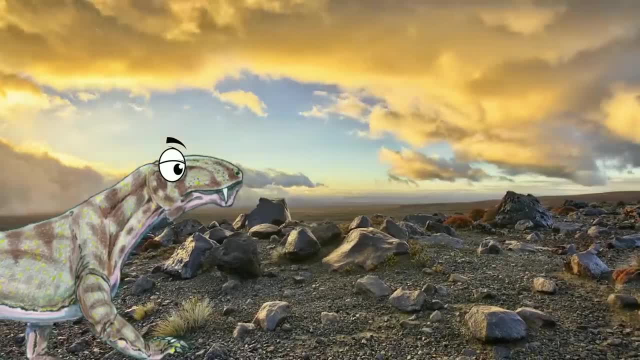 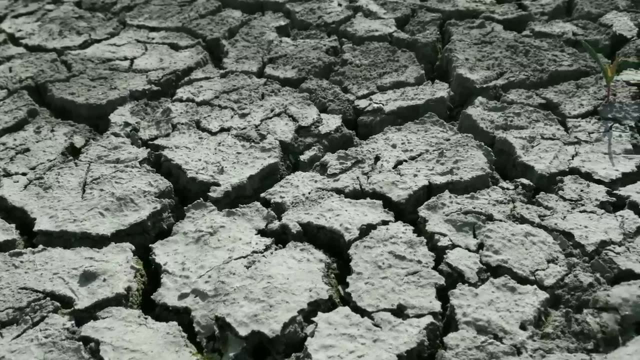 water to spread rainfall to the interior of pangea. so, yeah, it would get hotter, but at least there would be more liquid water to go around. but unfortunately the way it played out was not that simple sea levels did rise, but the presence of the mountains that were in the middle of the. 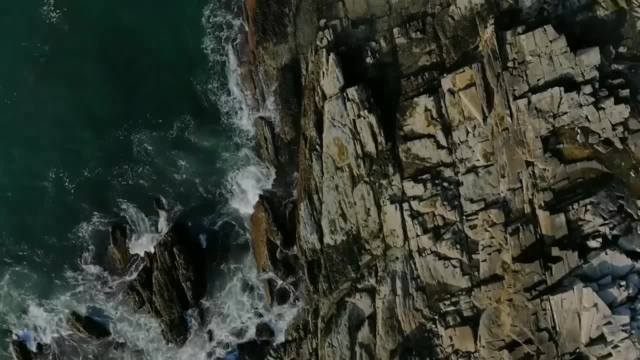 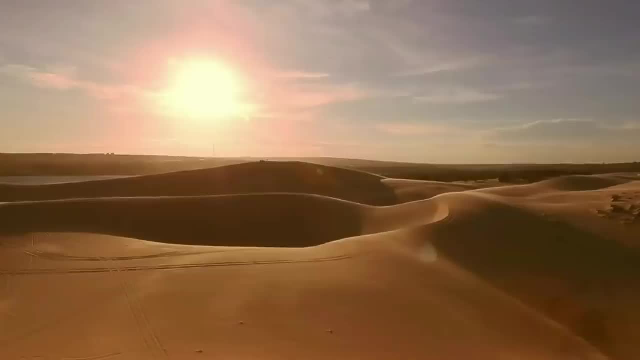 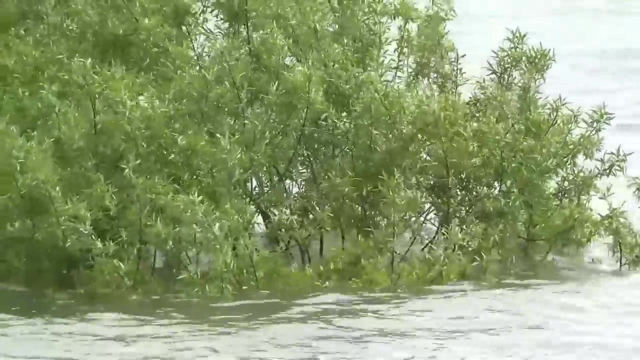 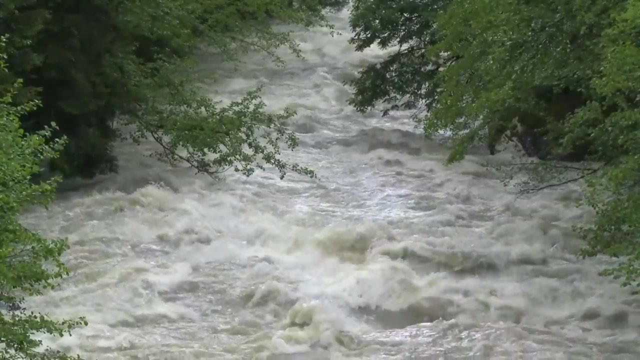 mountains were still blocked off by the mountains, so it got hotter, but, if anything, it also got even drier. the only places that could get more rain were the places that really didn't need it. this probably caused widespread flooding throughout the coastal swamps and forests and the runaway. 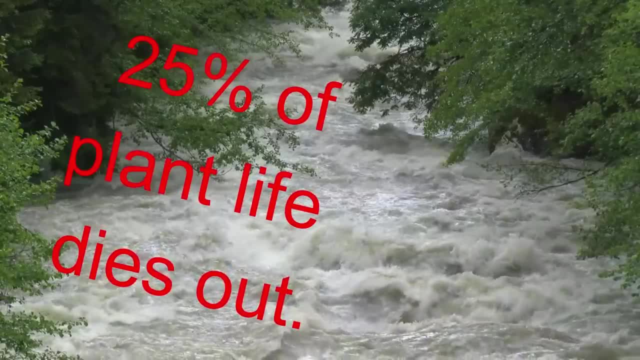 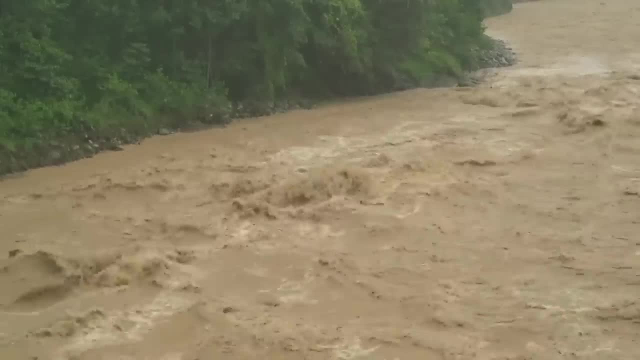 effects of this would cause around twenty five percent of the plant species to die out, and that's never good for a food web. this would once again lead to the demise of many of the animals at the top of the food chain. around this time, Helicoprion disappears from the world's. 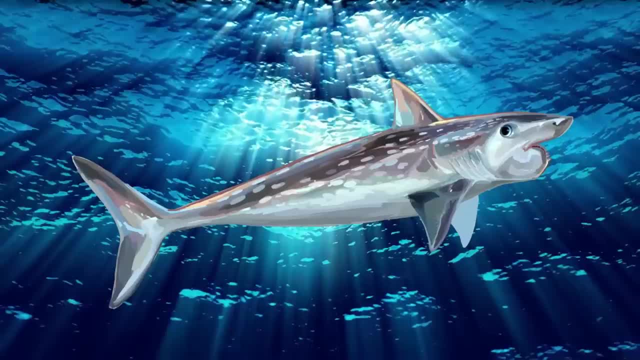 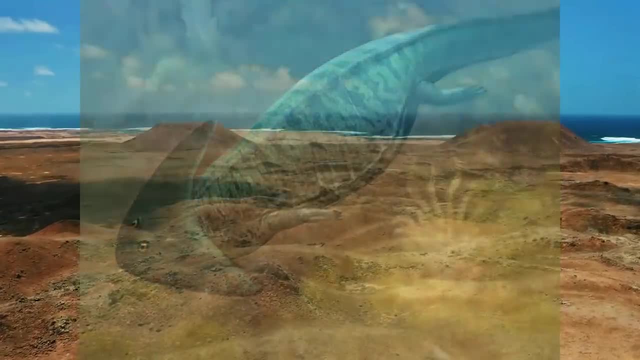 oceans, as many of its different favored ammonite prey were becoming too rare for the giant to sustain itself, and on land, many of the temnospondyls were falling on hard times, and so would many of the first synapsids that had previously been dominant. 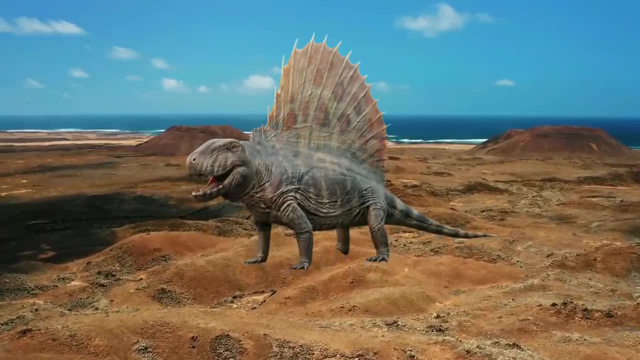 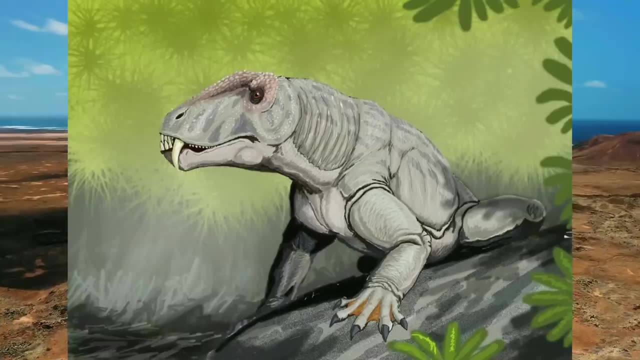 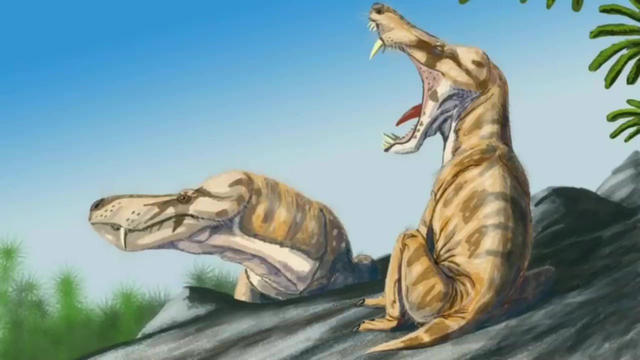 and this is when Dimetrodon, the most famous stem mammal of all, ran out of steam inland. many of the groups that came to dominate did survive, but so many species would be taken out that this was no longer the Dinocephalian's world and there were other synapsids that were more generalized and 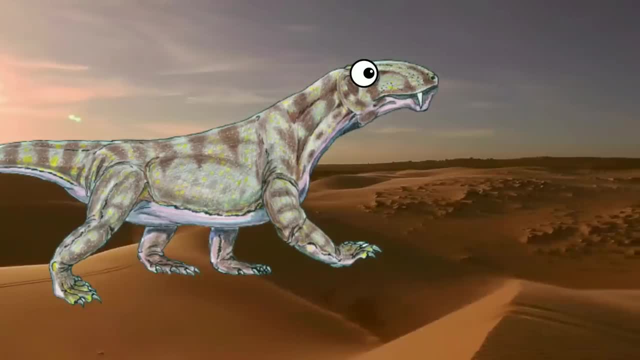 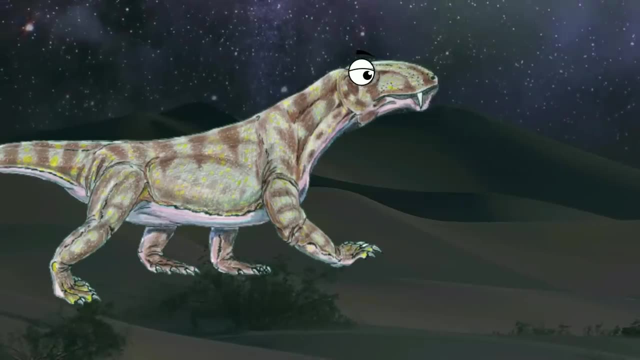 ready to take advantage of this new hot Earth. so you're probably wondering why I chose to divide the Permian in half, and if it's not already clear, it will definitely be the case that the Dinocephalian would become more clear in the next episode of the series. basically, the animals of the early and 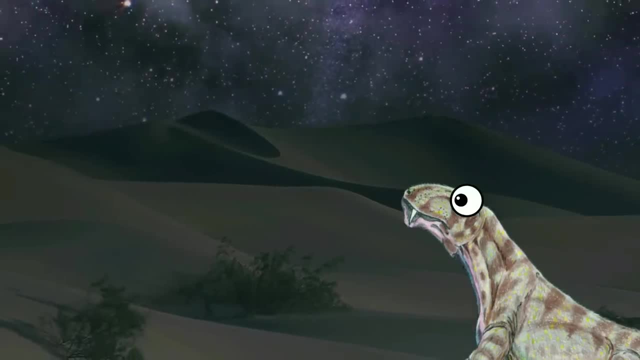 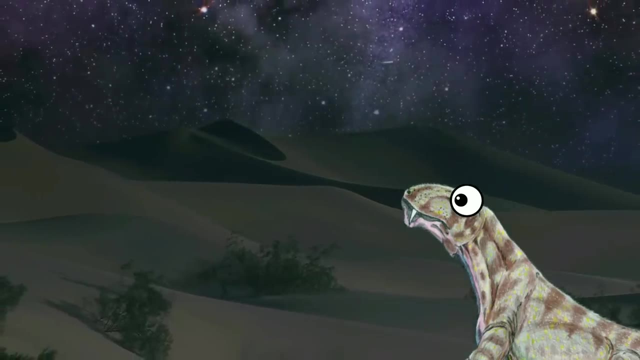 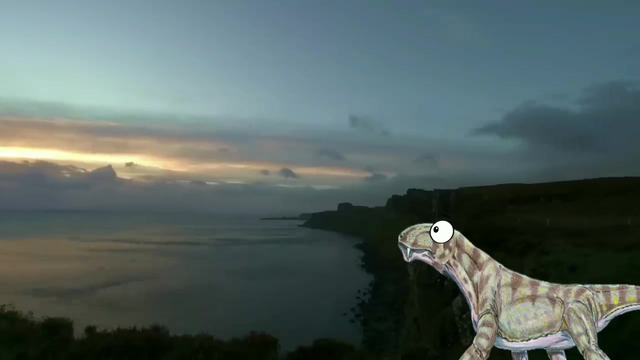 late Permian are so radically different from each other because of the extinction that took place right in the middle that it would be very hard to tell the story properly in just one episode. plus, this script is already over 3 000 words long and I need to get started on Paleo rewind so, as we 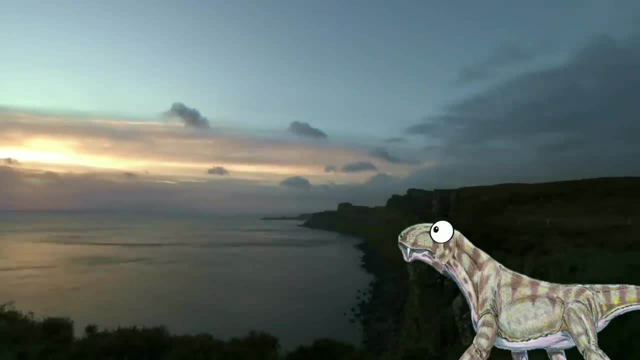 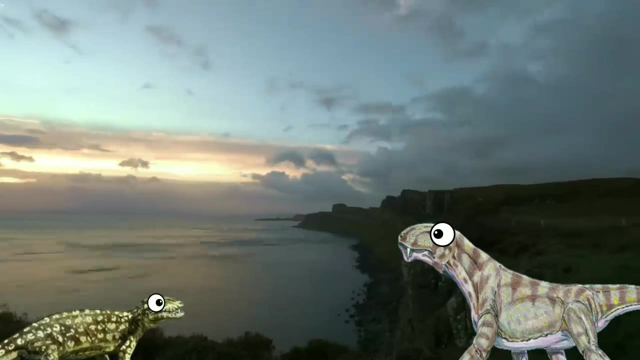 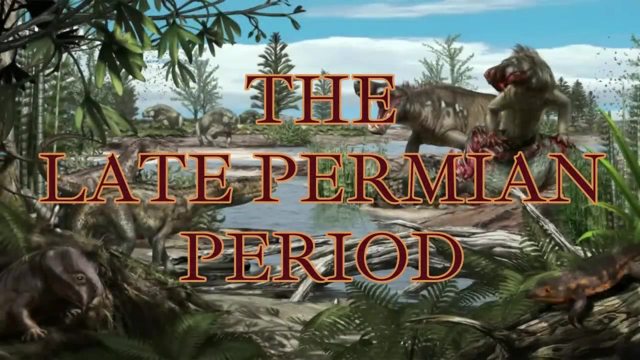 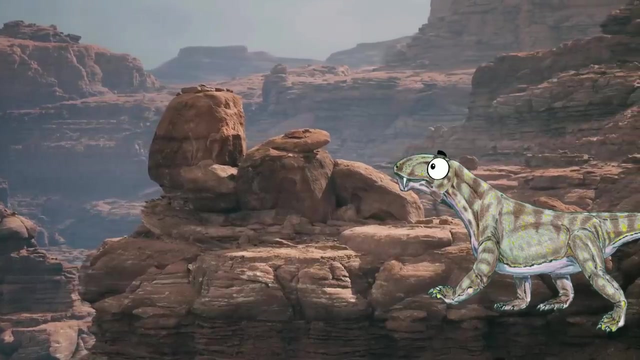 go forward. we will see what synapsids manage to pull through and how they will adapt to living on a continent that is continuing to slam together. is the ground shaking? no, have a good one everybody. well, at long last we have come to the end of the Permian period. our world has already gone through. 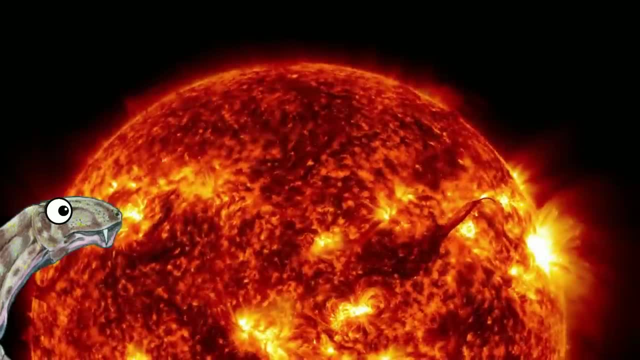 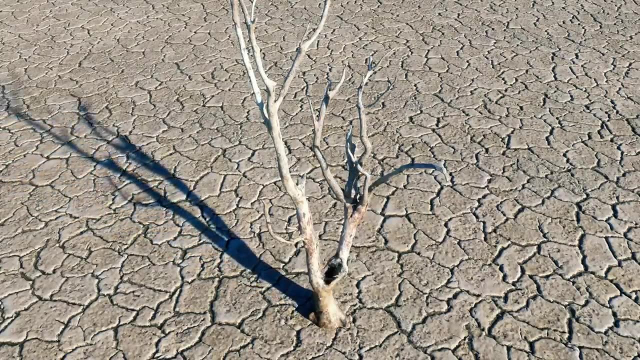 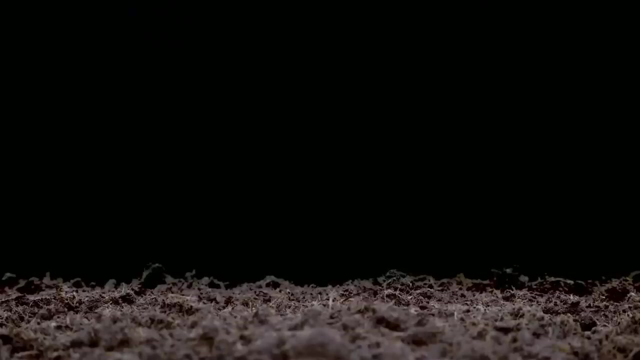 so many changes since we started, with the fiery ball floating through the infant solar system, despite the fact that we had just seen yet another die-off of several different species, leaving only around one-third of the terrestrial animals alive, we would see life continue to press on, and something 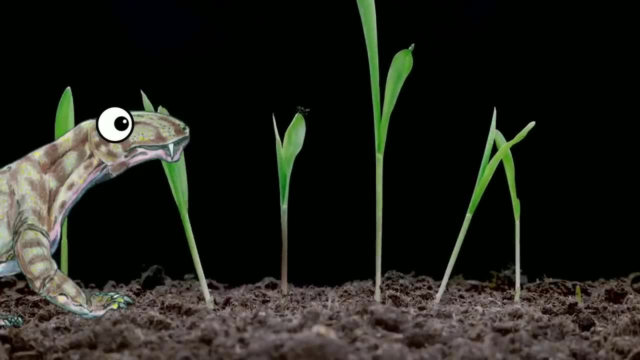 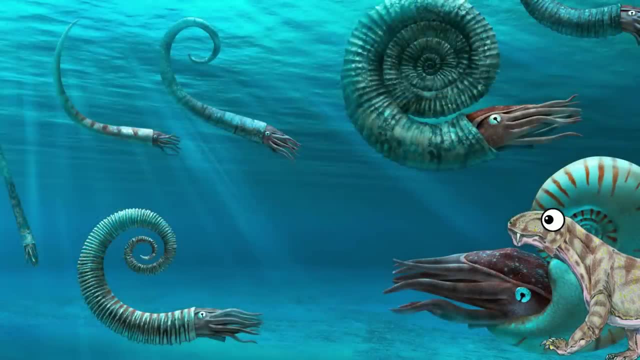 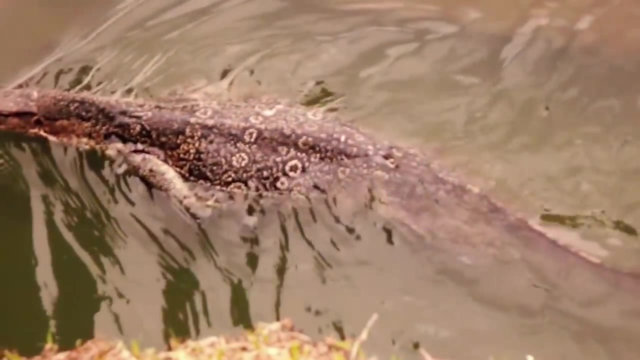 that you may have noticed, with each event that has resulted in a drop in biodiversity, every time it seems like the animals that make it through are just a little bit tougher for it- not necessarily stronger, but better adapted to the changing world. but unfortunately, regardless of how enduring the plants and animals on this planet become, 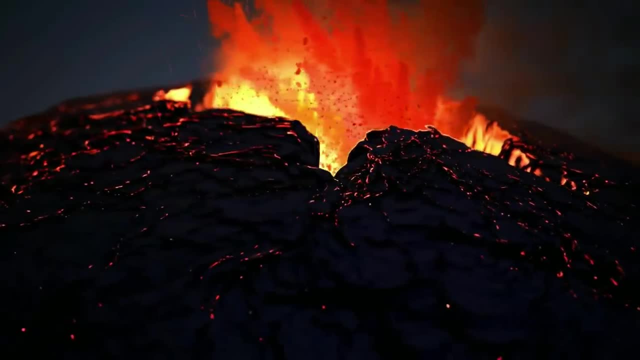 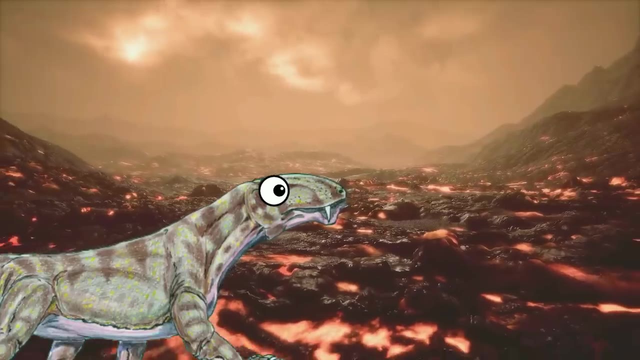 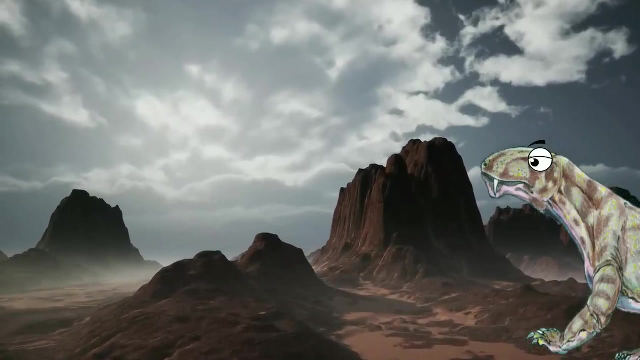 the Earth will always have the final say in who lives or dies. and as the Continental plates continue to push into each other, tectonic forces were building to a tipping point that could have ramifications for every living being on Earth, but for the moment we synapsids were still on top, even. 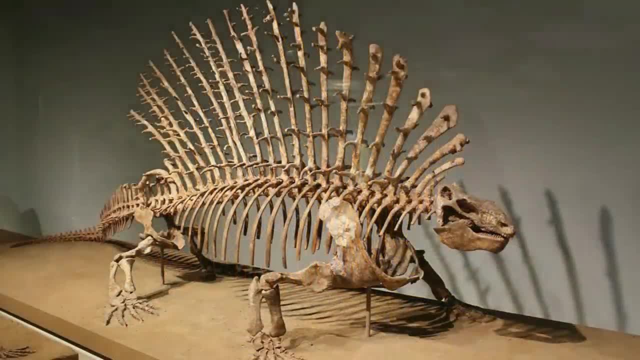 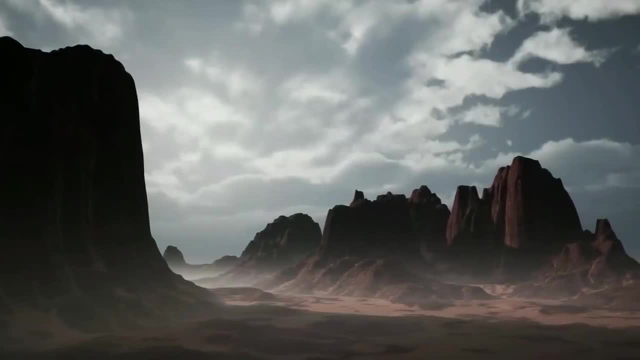 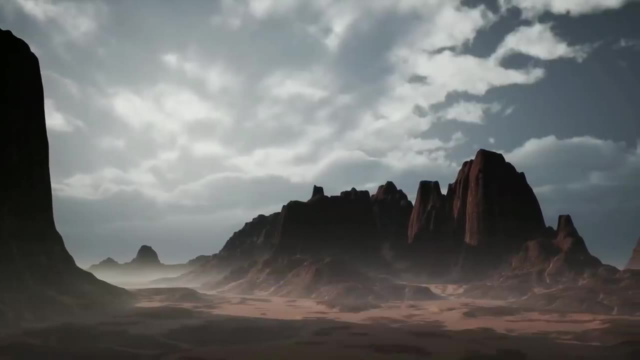 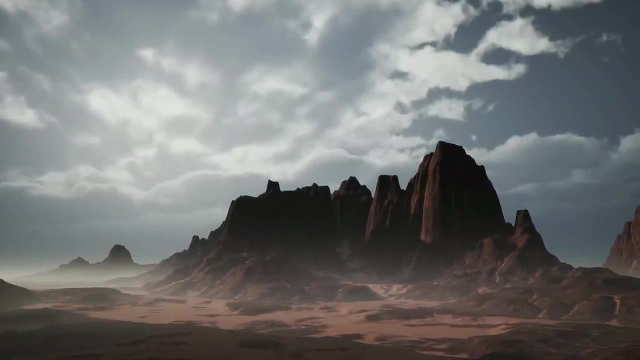 though many general like Dimetrodon and Adaphosaurus were gone, several others pushed on, and that's where we pick up in the second half of the Permian period. I have a bad feeling about this picking up where things left off. tectonic activity was beginning to get more volatile. a string of microcontinents called chimeria sheared away from the southern Gondola and Dwan and half of Pangea, and started drifting north towards what would one day become Eurasia. this caused the paleotethis Sea to start to close and the neotethis Sea on the other side to start. to expand. this also pushed the chain of Chinese island continents northward on the same collision course. as this happened, the Continental forces that had at this point been building, since the two main continents had come together at the end of the Carboniferous, would result in Mountain. 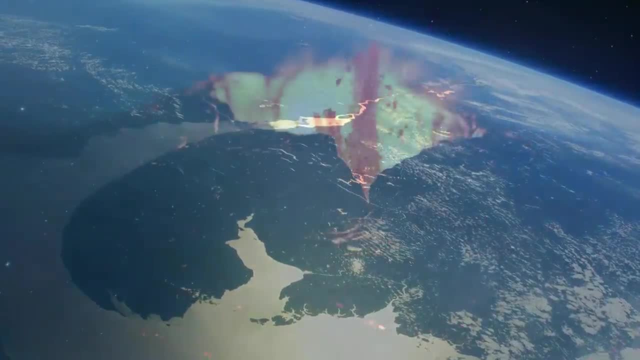 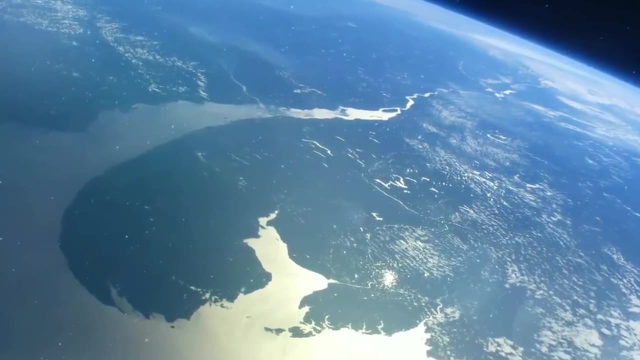 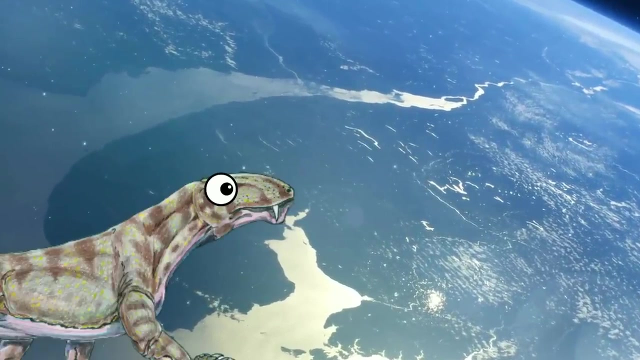 ranges and volcanoes being pushed up all throughout the massive continent. despite this all being one landmass, this was still made up of several Continental plates, all of which were pushing together, which was the driving force behind all this activity. one place where this would happen is at the far western edge of your America, pushing up mountains at the coast. 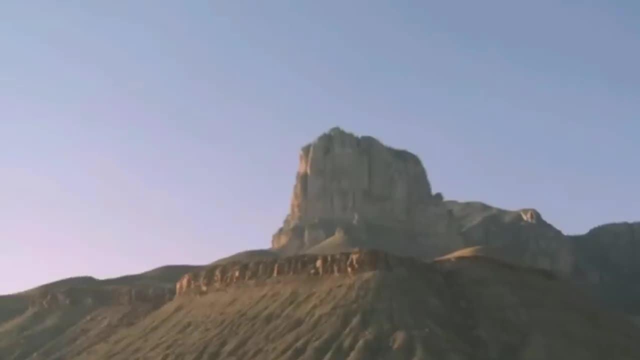 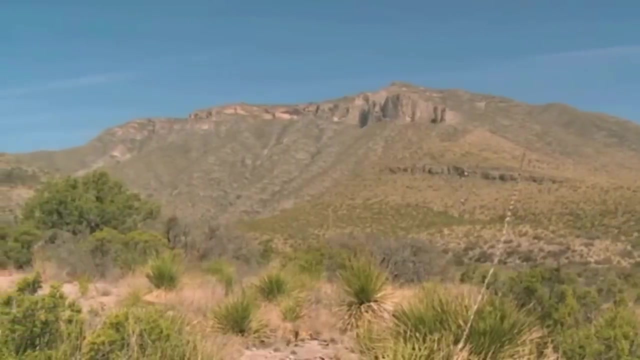 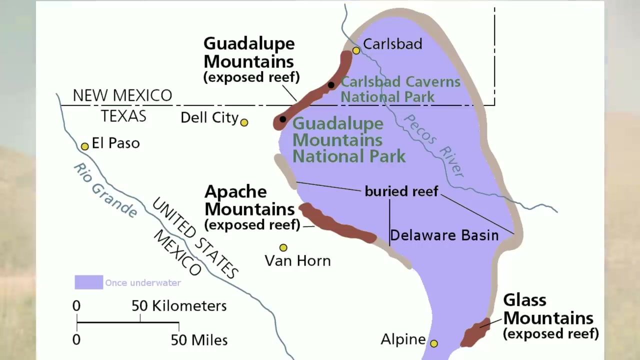 that in 260 million years, would be known as the Guadalupe Mountains. today, In the 21st century, this is a very small, 105 kilometer or 65 mile long mountain range that is only around 2600 meters tall at the Texas-New Mexico border. 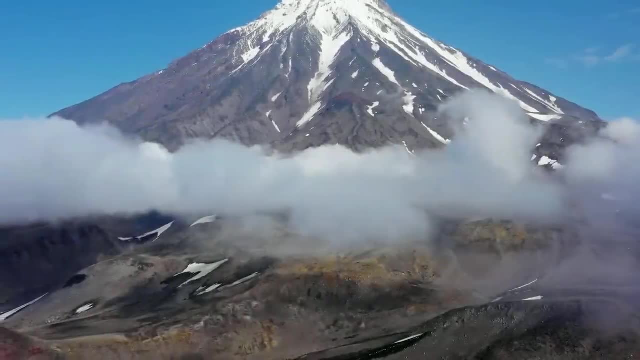 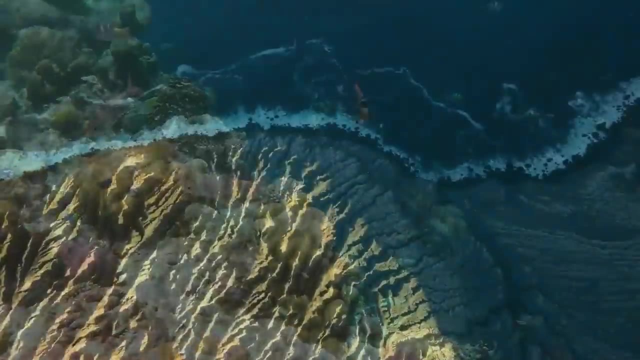 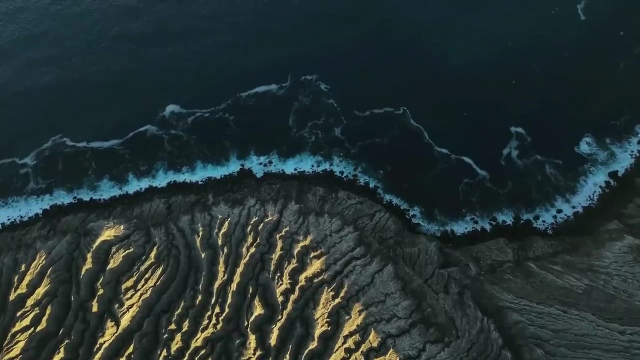 But during the Permian this was a substantial mountain range pushing up what was previously a part of an inland sea covered in a reef. This spelled doom for any of the marine animals that lived here at the time, But this would also preserve an excellent snapshot for paleontologists to find hundreds 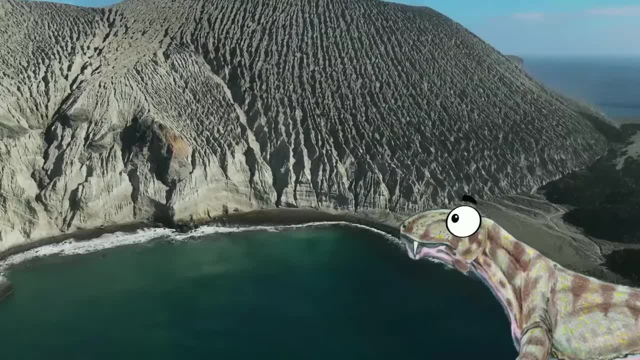 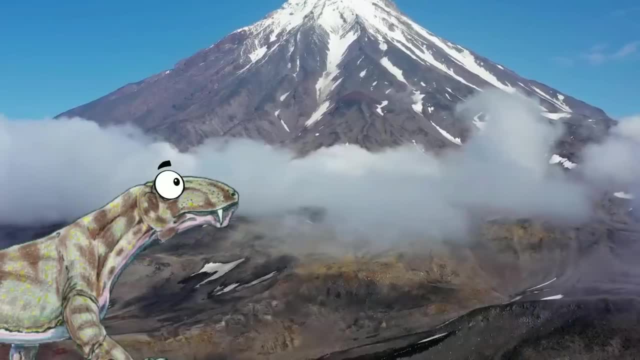 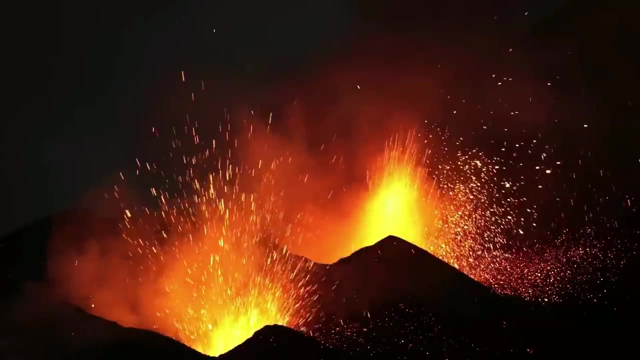 of millions of years later in the modern day- And this was just one example. This would become a reoccurring theme throughout the remainder of this period. The planet itself was becoming the most violent that it has been since the Archean, And every time that the Earth would roar to life. 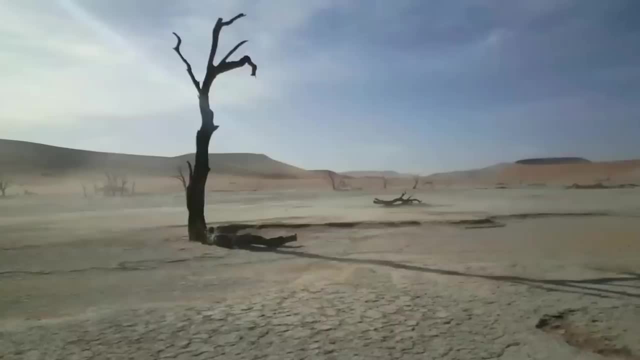 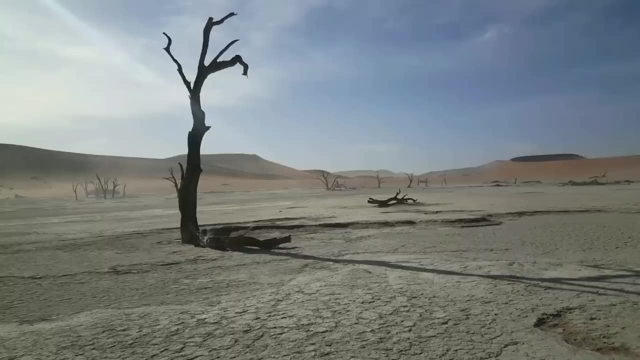 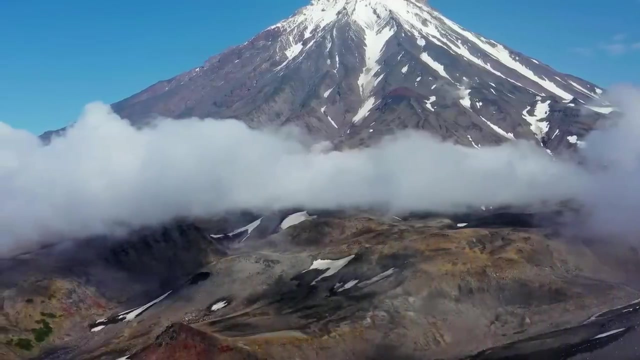 the local inhabitants wouldn't stand a chance. The other side effect of this was the interior of Pangea was becoming increasingly arid, For all the same reasons that we mentioned in the last video. When you put more mountains out there, it's going to block more rain from getting to more. 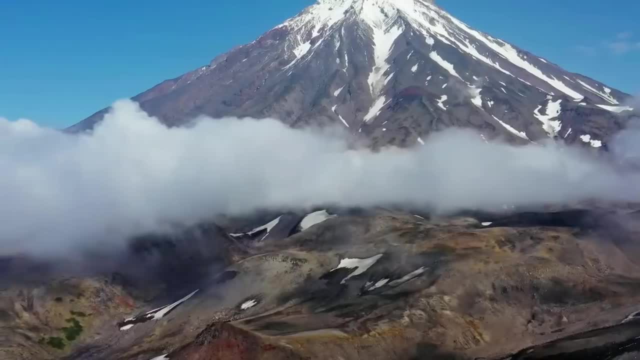 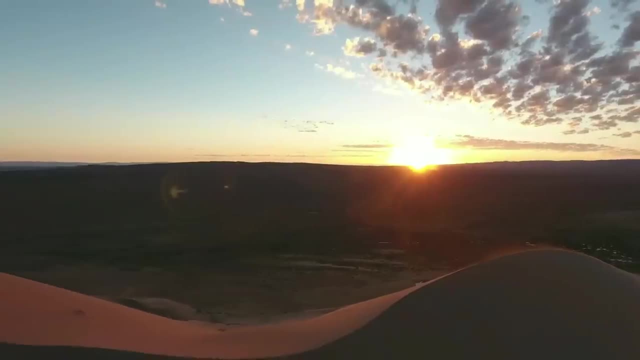 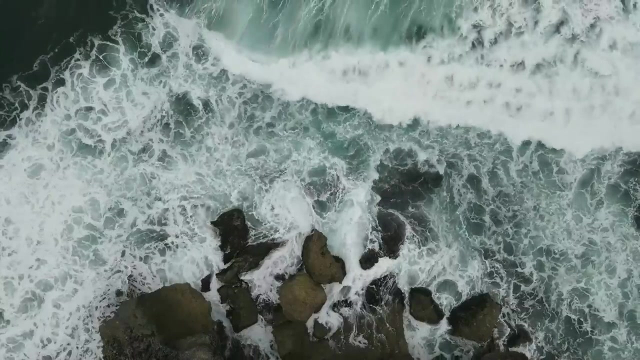 areas. It wasn't always hot all across Pangea. Many areas had similar conditions to Central Asia today, Kind of something like the Gobi Desert. So as the last of the glaciers at the poles melted away, the sea levels would also continue. 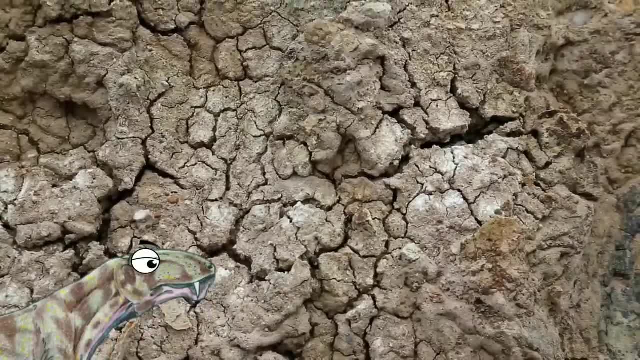 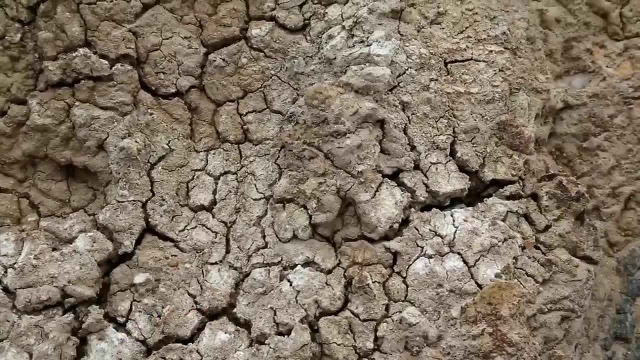 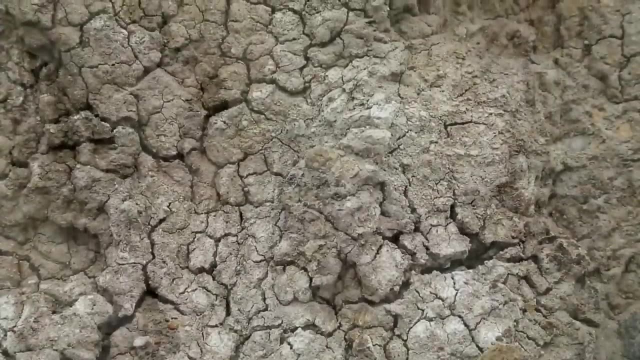 to rise. The world was definitely in crisis And, as a result, life was struggling to bounce back from the most recent extinction. Those that were going to pull through and see their descendants inherit the world were going to have to be the toughest that they've ever been. 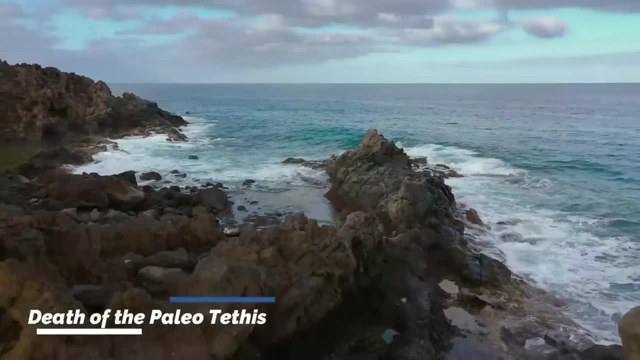 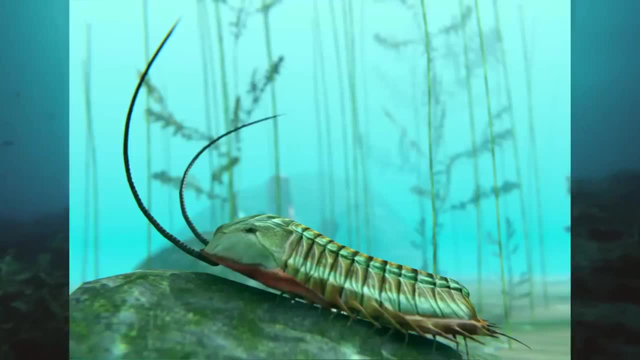 As the continents above were experiencing severe droughts, they were also struggling to survive. They were experiencing such great unrest. Beneath the waves life was chugging along. The trilobites that had been hanging on for so long had been withered down to only a 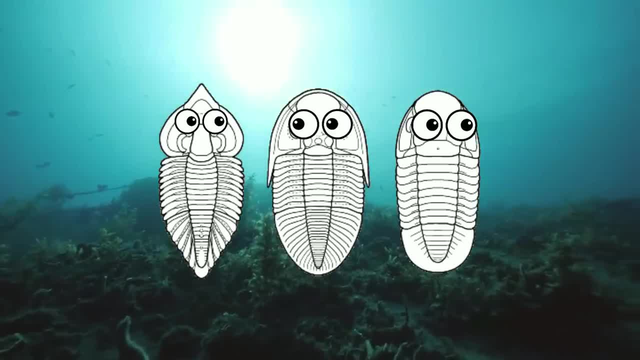 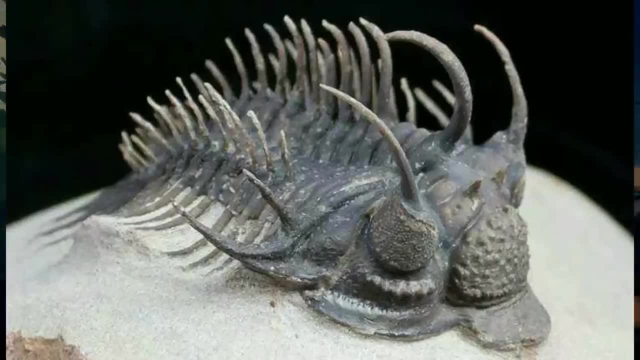 couple of different families, But they were about to be thrown a lifeline In reaction to some of the creatures being wiped out in the previous extinction. the trilobites were about to explode in diversity for the first time since the Silurian. 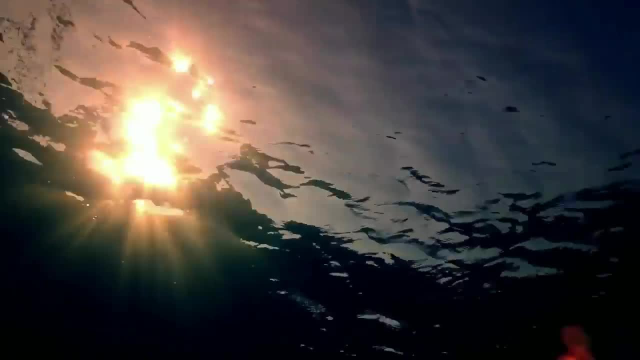 It finally seems like things were starting to look up. The other major niche of the trilobites was the Pangea. The other major niche of the trilobites was the Pangea. The only niche that was left open from the mid-Permian extinction was the spot as an apex. 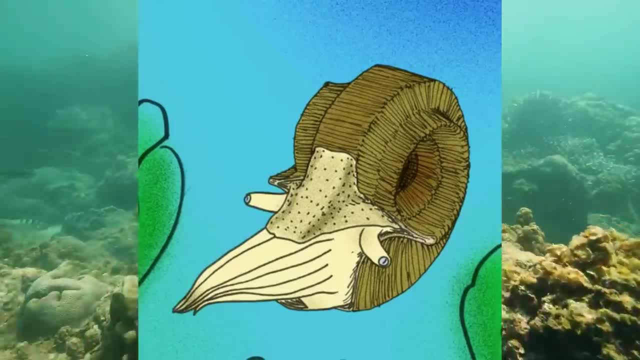 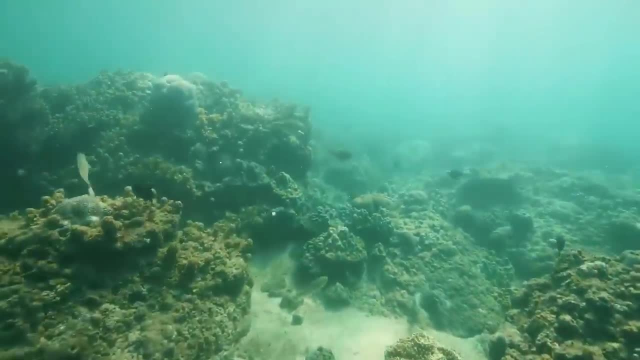 predator, And with the ammonites recovering and returning to their role along with the bony fish, it was only a matter of time before some new sea monster came on the scene. At first, the lack of large macro-predators would be filled by, of all things, a relic. 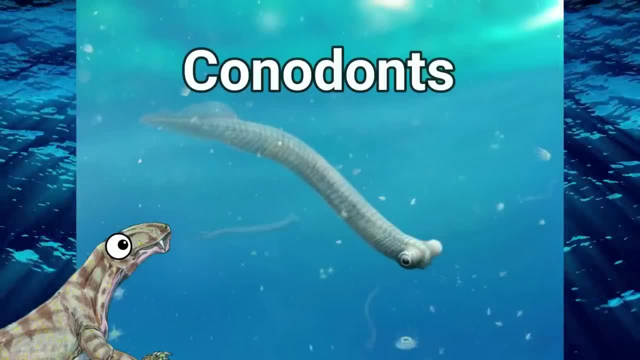 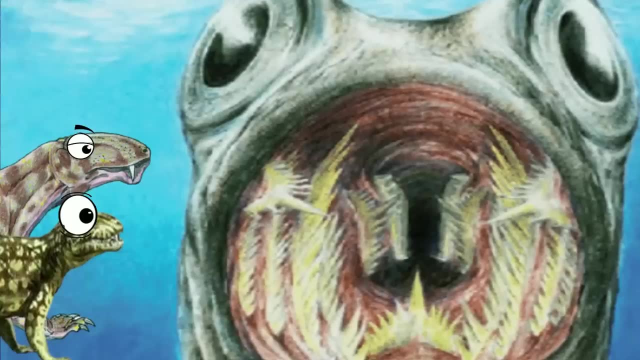 family of jawless vertebrates called the Cannodonts. The top predators were jawless HAH. What Are you serious? This is rich. Remember when we had to flee the oceans because of all the Ah? What the crap is that? 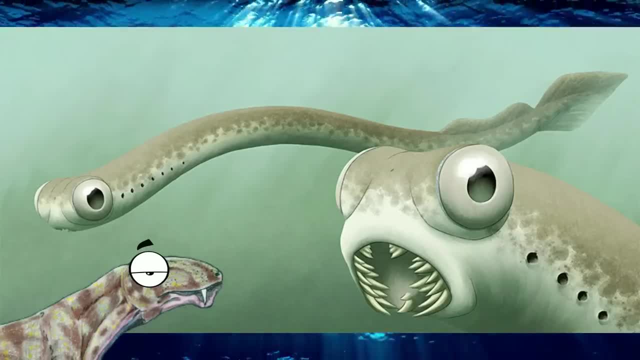 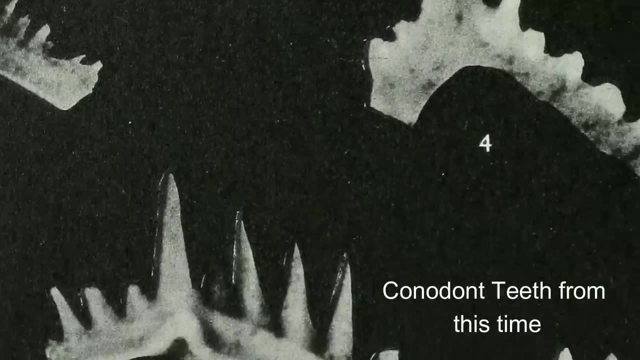 That would be the disturbing set of teeth that these lamprey-like creatures had in their sucker-shaped mouths. Although these animals have been around since the Cambrian, this time did see them expand and diversify, But I still wouldn't quite call them apex predators. That role would actually go to a much more familiar face. With the eugeniodontids gone, it was finally time for the hybodonts to spread back into the open ocean and become top predators. This is not exactly the same branch of the chondrichthyans as modern sharks we know today. 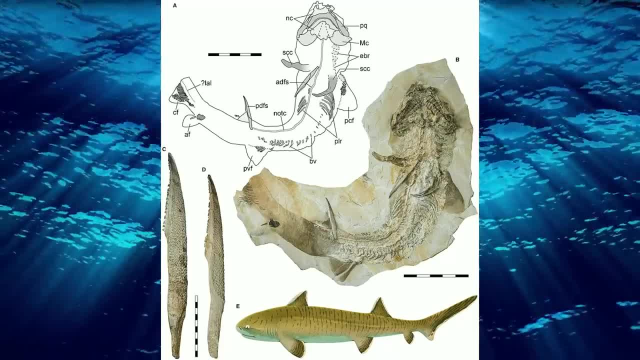 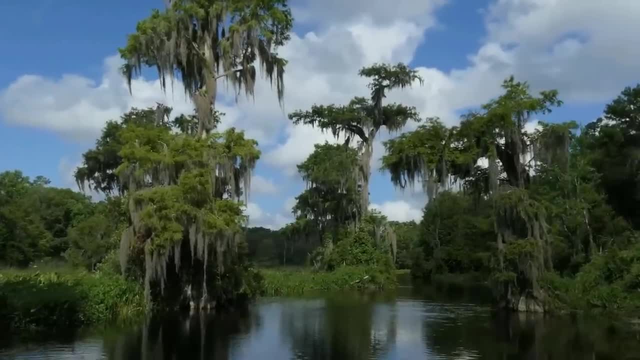 but they were a close cousin and likely filled a similar role. As some returned to the open water, others remained in the freshwater rivers to dominate there, And with that it's time for us to come ashore again and see what's going on. 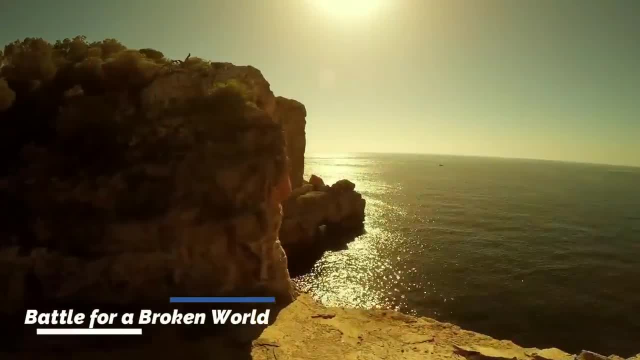 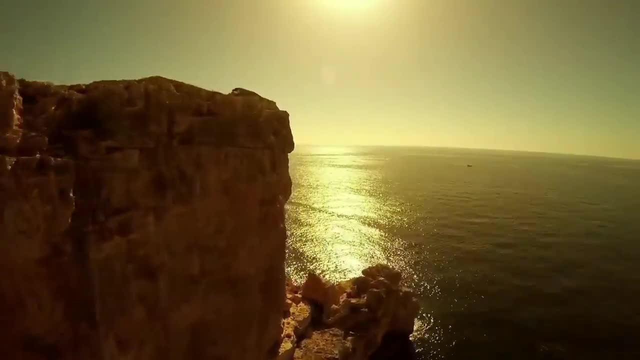 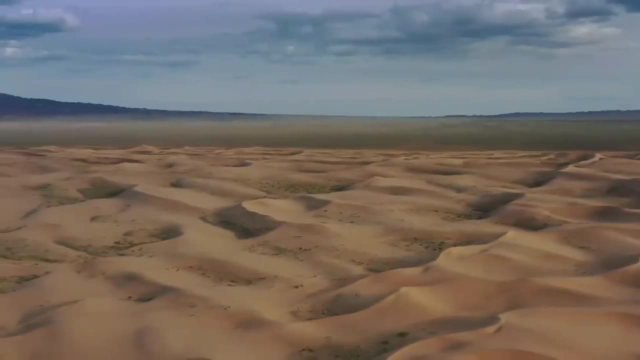 What's going on throughout Pangea? Normally, following a mass extinction, we see a dramatic rise in new organisms stepping up to fill the roles that were previously held by the ones that disappeared. Then new plants and animals become specialized to the current environment. 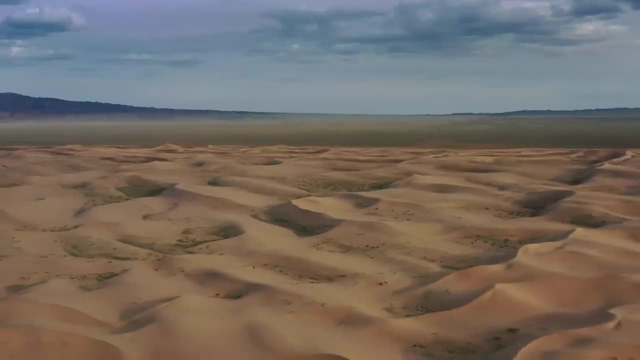 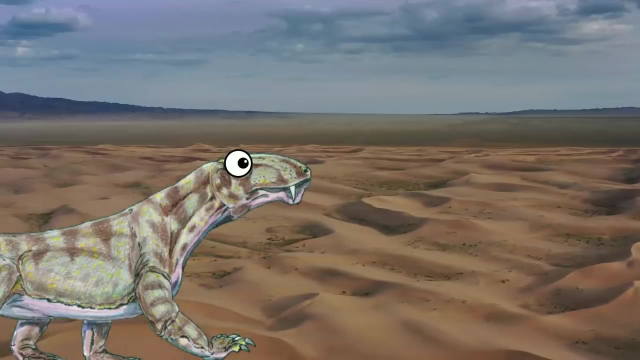 And those would rule for as long as the new environmental conditions remained the same. The problem is, because of all this geologic upheaval, a lot of the conditions that caused the extinction, a lot of the conditions that caused the extinction at the middle of the Permian- 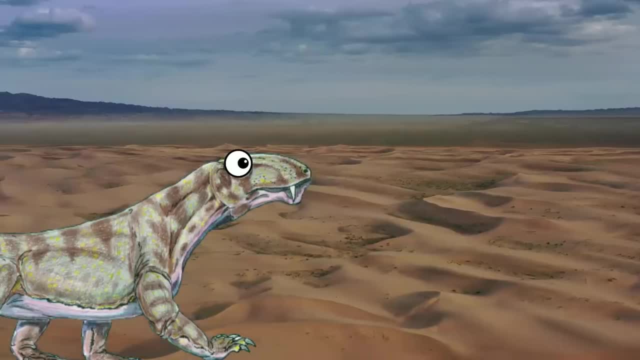 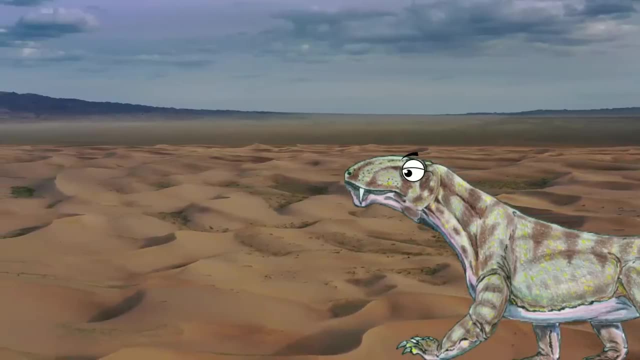 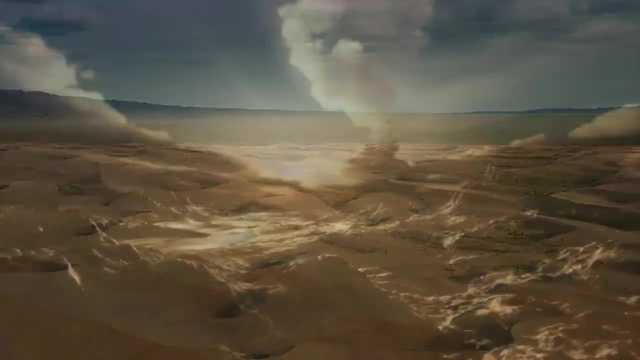 were still continuing for several million years after, And these conditions were not very hospitable for macro life in general. So for about 10 million years following that event, biodiversity across the globe remained fairly low, But as I said in the last episode, 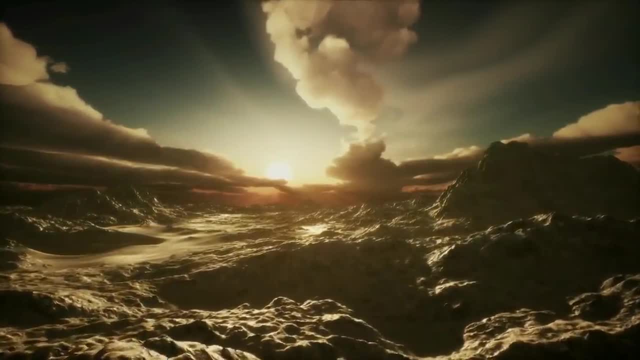 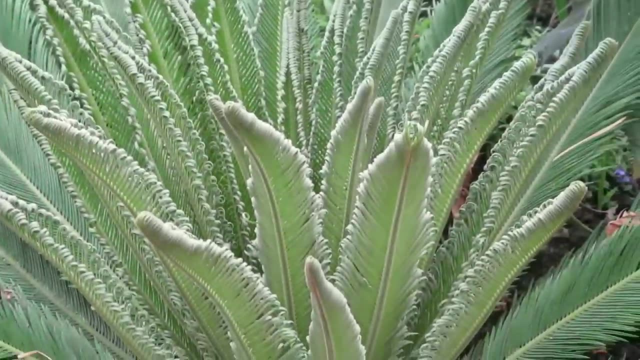 there were still some groups managing to hang on. One group of plants that got their start in the early Permian and would eke by on the arid global continent would be the cycads, And this would be enough to give some animals a chance. 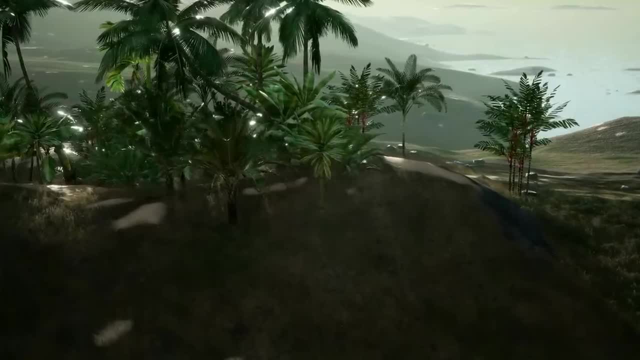 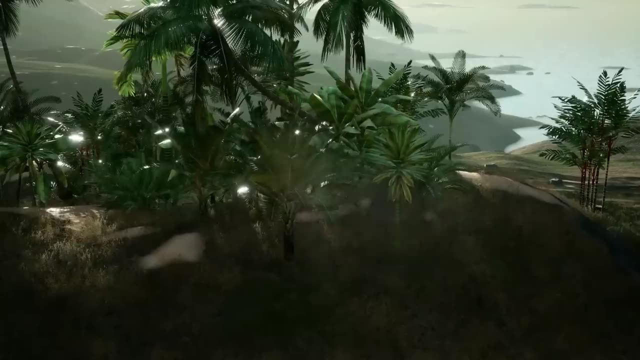 Despite early cycads being nutritionally poor, some herbivores were able to sustain themselves on this new type of plant. These would be the synapsids and diapsids that would survive in the late Permian deserts and coastal forests. Life, however, was a struggle. 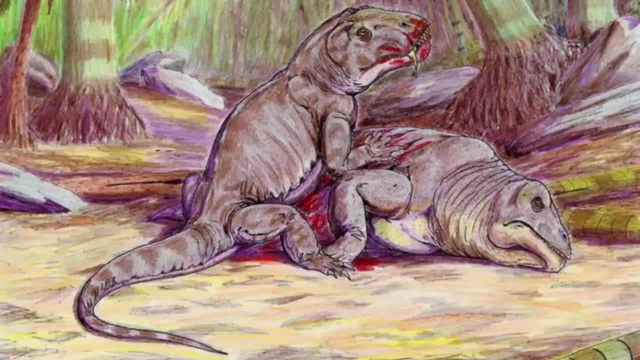 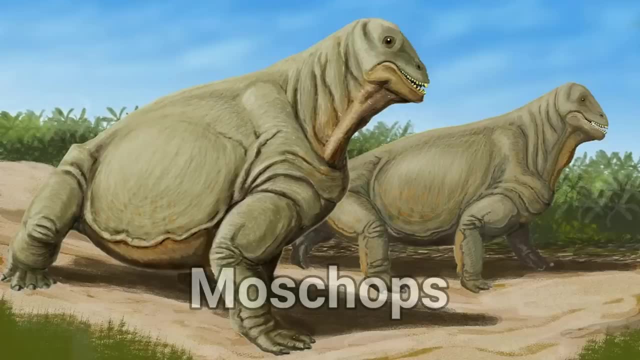 And the last of the Dinocephalians were still able to claim their title of dominance for the moment, But their grip was slipping. One species that did well for a while was Moschops, a species of Tapinosophallus whose 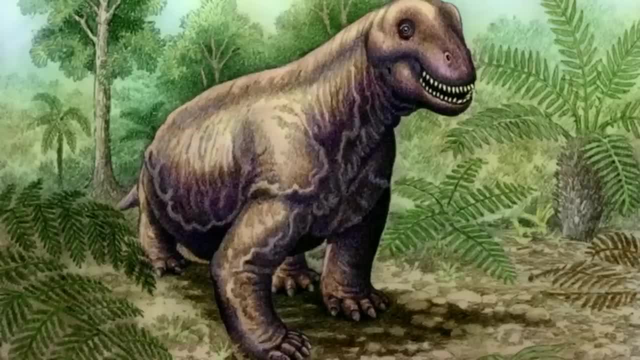 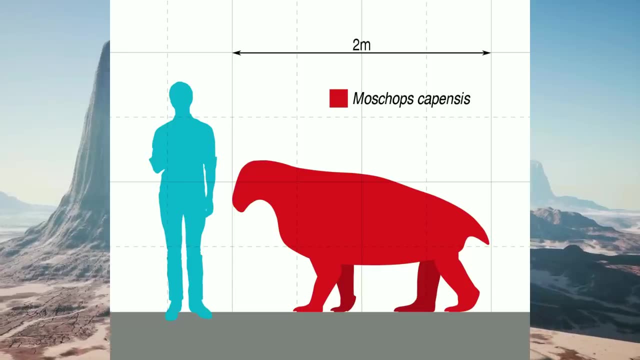 rise appears to be linked to the rise of the first cycads. In response to this being the most readily food available, Moschops became well adapted for consuming tough, hard to digest vegetation, So kind of think of it as like the camel of its day. 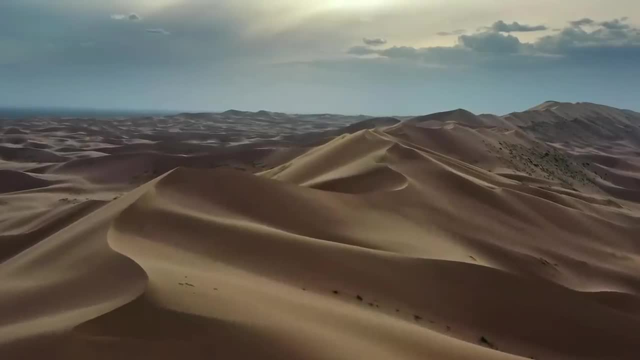 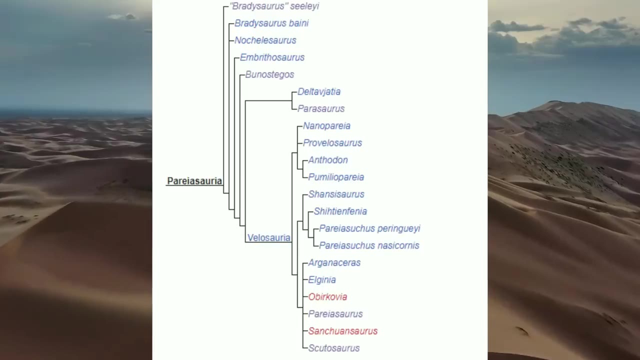 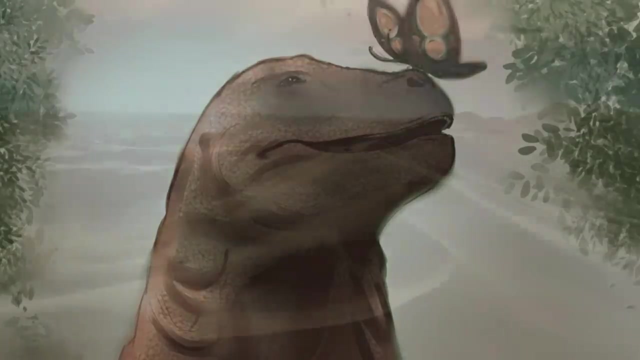 But it would start to see some competition from equally hardy creatures Like the diapsid Parasaur Bradysaurus. The Parasaurs as a whole quickly spread across Pangea and became the dominant group of large herbivores, eventually pushing the Tapinosophallids to the brink of extinction. 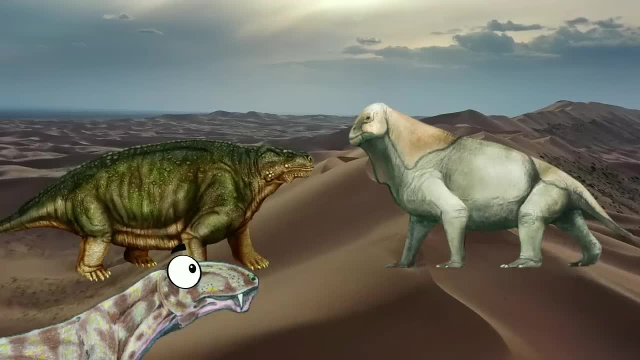 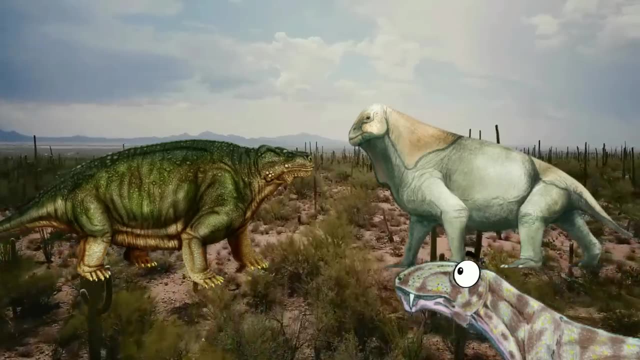 And it's actually pretty interesting when you look at these creatures, how similar these two very distinct families were. I guess, no matter what clade they were a part of being a squat, barrel-bodied animal with a short muzzle and peglite-like body, they were still a part of the group. 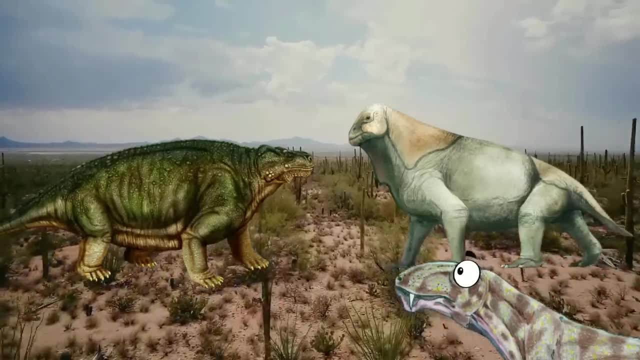 I guess, no matter what clade they were a part of, being a squat, barrel-bodied animal with a short muzzle and peglite-like body, they were still a part of the group In the latter half of the Permian. they were on their way and, as these herbivores competed, 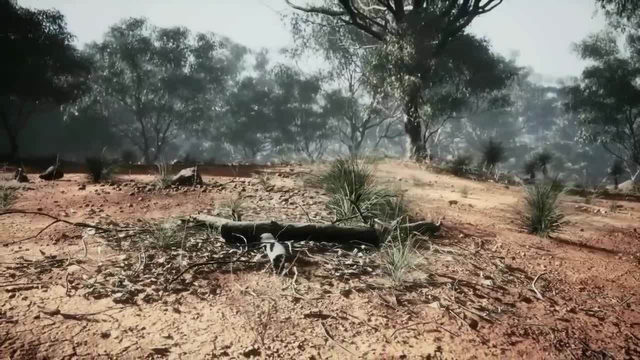 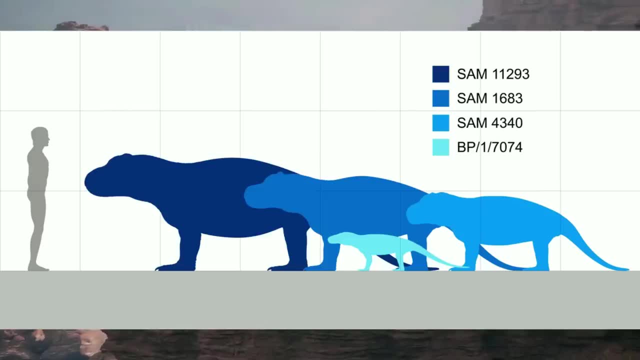 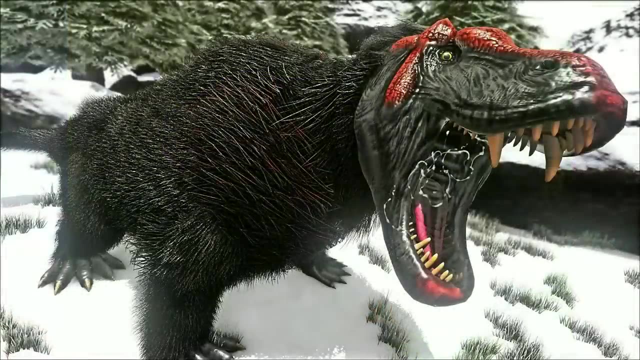 amongst each other. of course, new carnivores would follow suit with another Dinosophallian Atenosaurus. This was the monster of its time. If Titanophonius in the last episode was comparable to a tiger, then this thing was comparable. 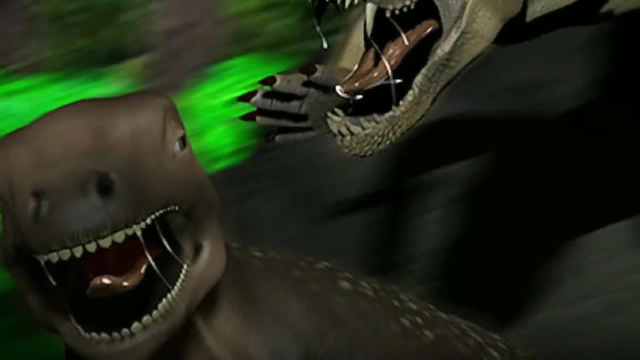 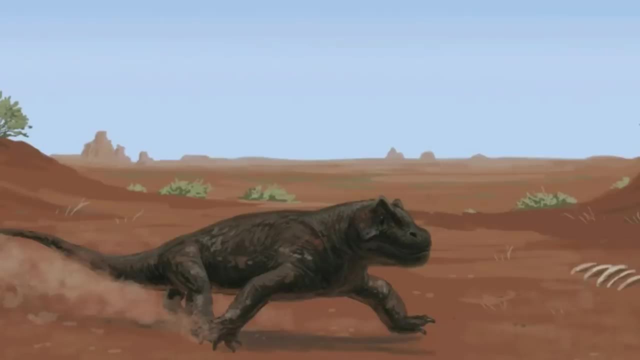 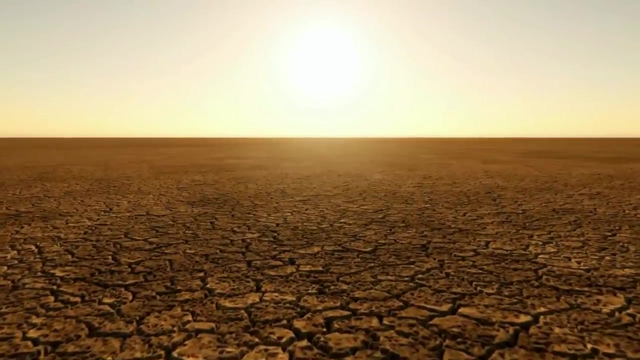 to a bear And it was the terror of any Moshchops or Bradysaurus that it encountered. But even though it was the king of the desert, even it had some competition from other therapsids And considering how shaky the hold these animals had on their environment was, it would be. 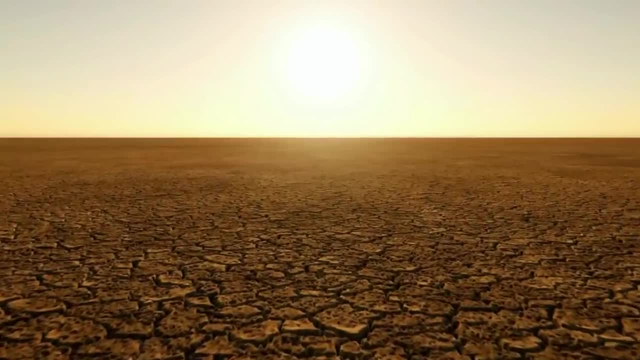 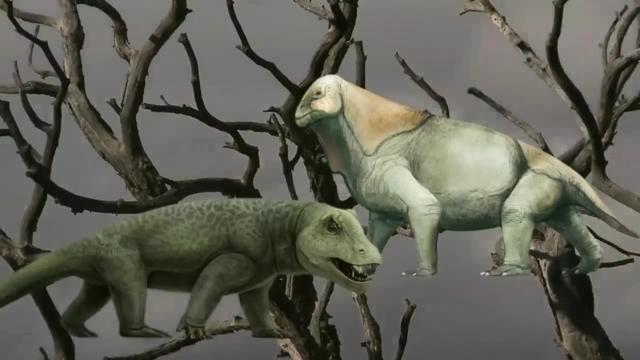 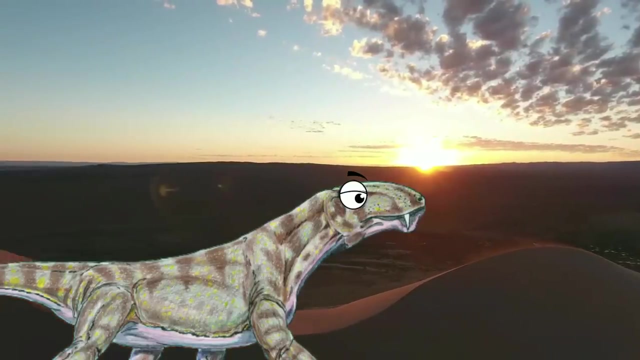 all too easy for the balance of power to tip once again. As we get into the Late Permian, around 260 million years ago, we see the last of many of the previously mentioned groups finally die off. The fact is that the Middle Permian was just a really rough time to be alive, and many 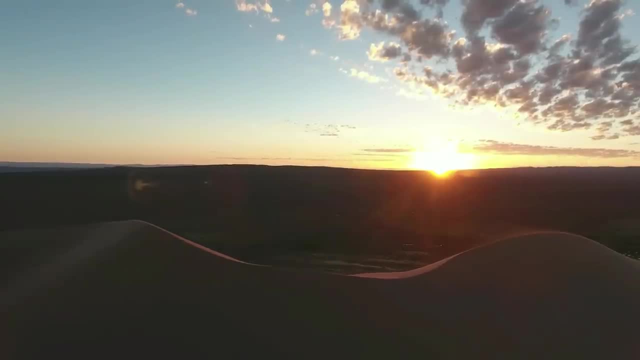 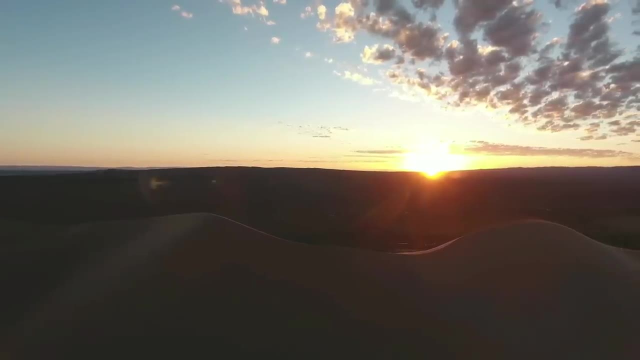 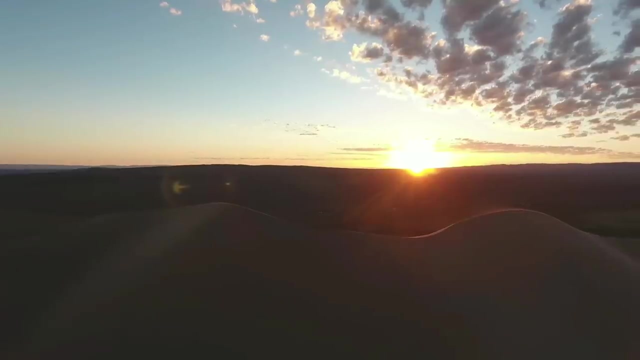 of the animals were barely making it as is With such limited resources. the last thing that these animals needed was new competition. But new therapsids were adapting to this hellish world And if there wasn't a place for them, they were going to push other creatures out of. 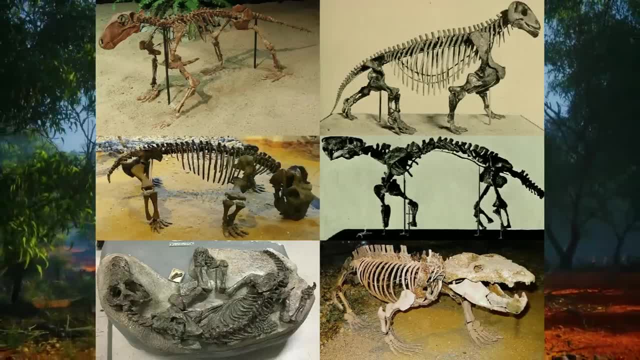 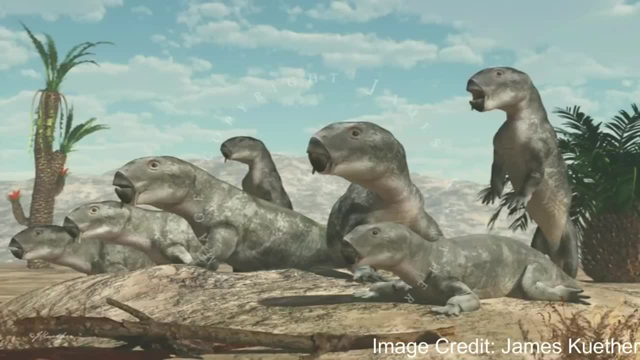 the way. They took all the qualities that made the therapsids unique and built on them, For instance Their specialized teeth. But ironically, one group of herbivorous therapsids called the Dicynodonts traded in their teeth for a beak. that made them even better at eating through tough plants and roots than the Tapiocephalids. 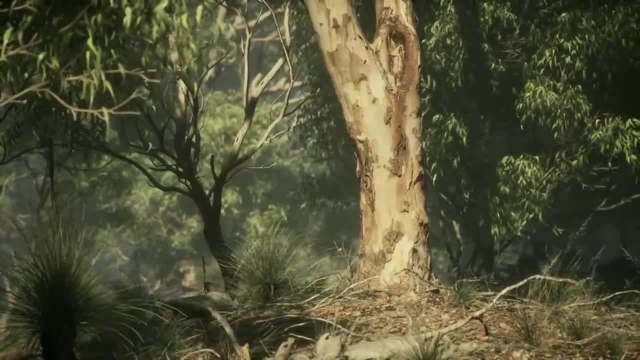 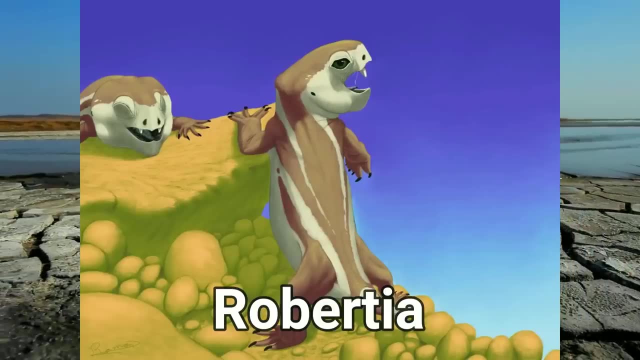 And this would be the key to their truly explosive success story. They started out small, with animals like Robertia, who still actually maintained two teeth. A set of tusks, theorized to be a case of sexual dimorphisms, were found in the middle. 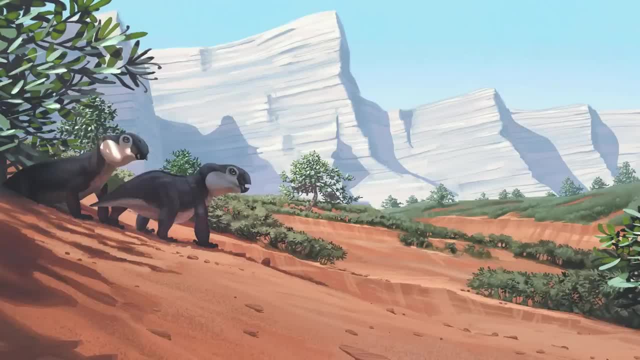 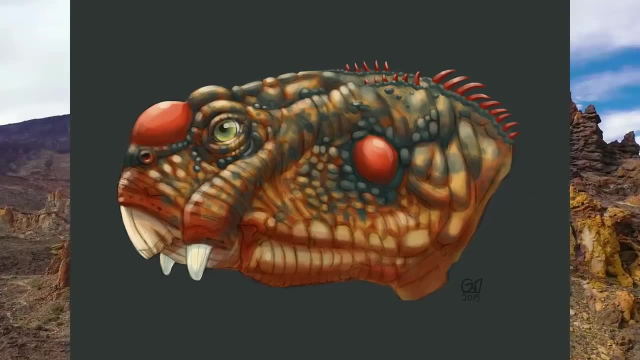 of the Dicynodonts, since only some individuals within the same species had them And in fact some species of Dicynodonts wouldn't even share this dental arrangement at all, But the fact that their teeth were becoming so varied both between different species. 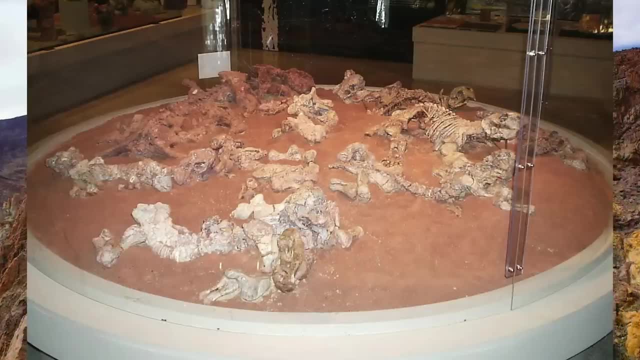 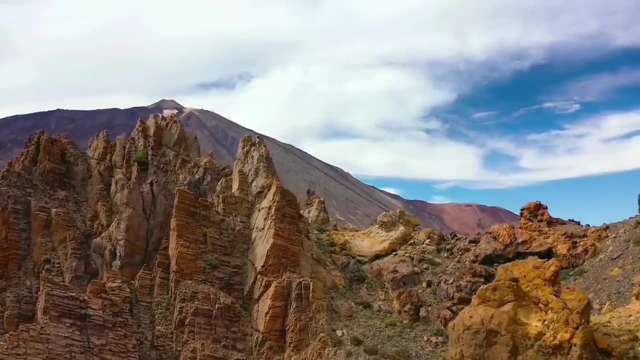 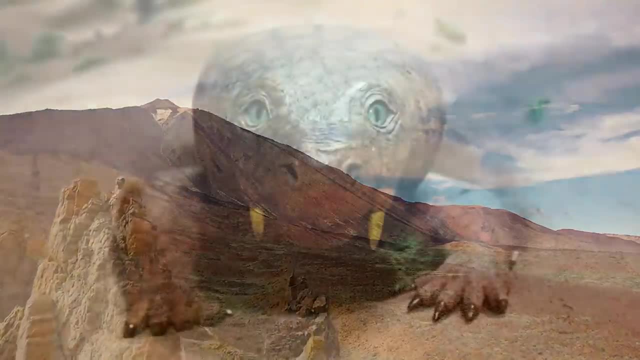 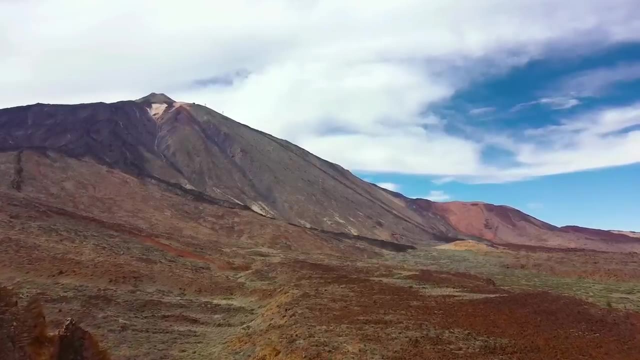 This was a showcase of how life could eventually bounce back and, given enough time, will manage to adapt to nearly any environment. It took a while, but the animals of the Permian were managing to thrive, And it wasn't just the Therapsids. The Parasaurs were still going strong as well, But this was definitely the Synapsids' time to shine. Besides the Dicynodonts, which exploded in diversity but remained smaller during this time. Besides the Dicynodonts which exploded in diversity but remained smaller during this: 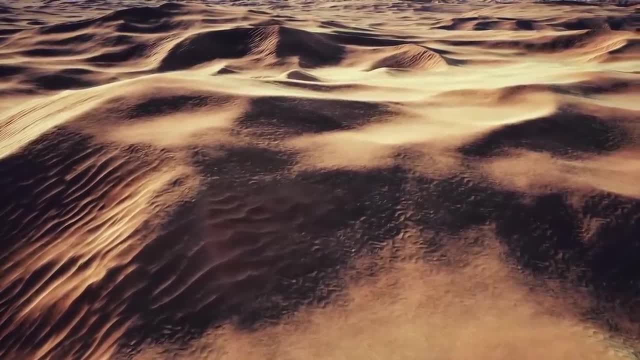 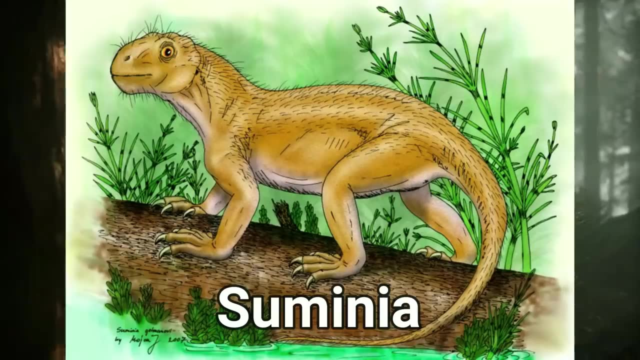 time, But even then they became a little bit more competitive. They started to take wildly different forms. One of the most noteworthy and interesting is a small creature that we call Souminia. This was a relative of another small burrower called Venucovia, who may have been getting 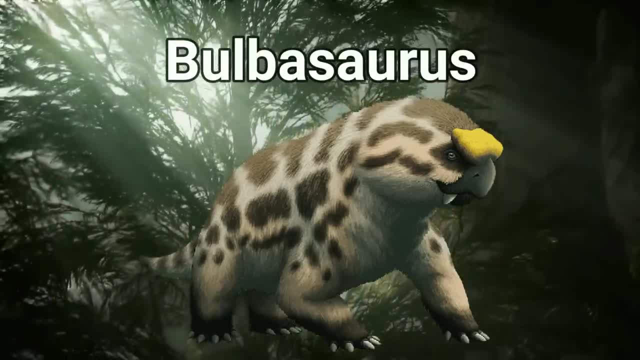 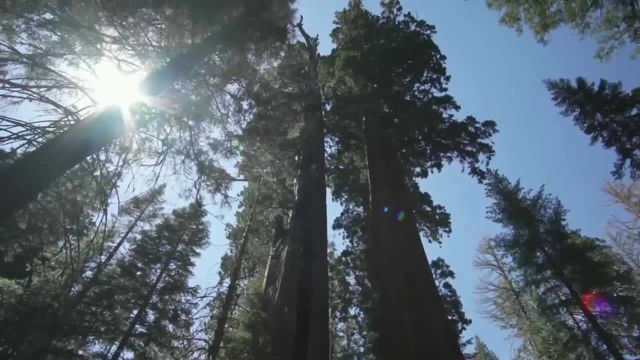 outcompeted by the prairie dog lizards that were popping up all over the world. So this group of Synapsids went a completely different evolutionary direction. They became arboreal, trading in their more groundhog-shaped bodies for something that they wanted to stay. 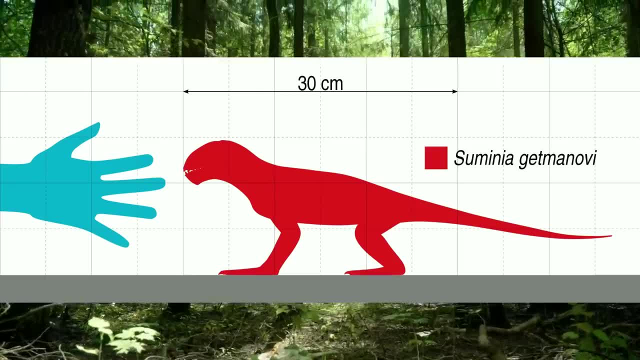 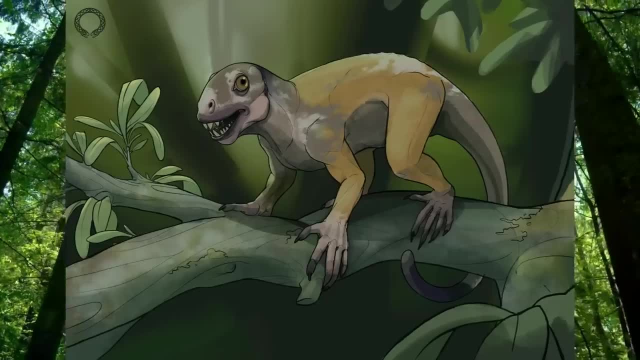 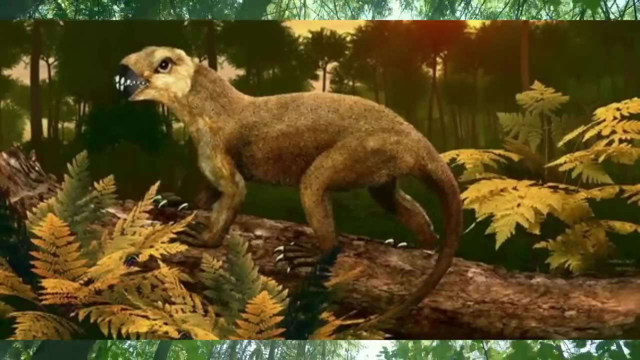 that looks almost primate, Hence the name. These tiny herbivores got by because they started to feed where the Dicynodonts and Parasaurs could not, and they evolved surprisingly dexterous hands to help climb and manipulate their environment. I wouldn't say it was quite on the same level as a 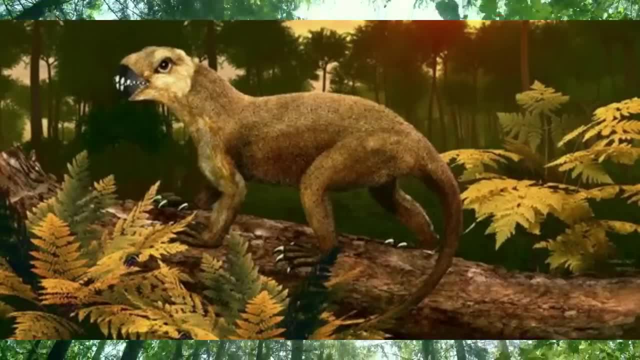 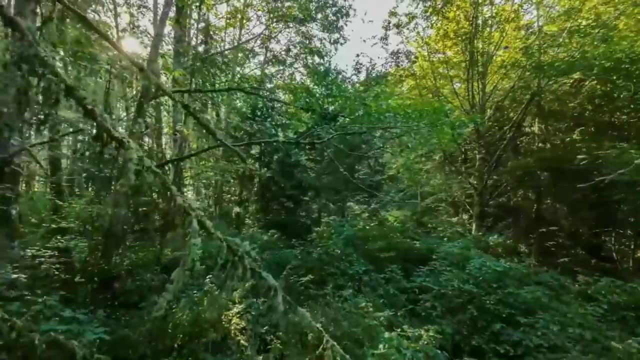 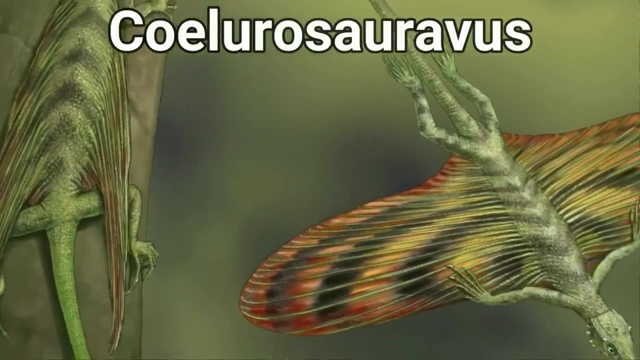 monkey, probably more like a squirrel or a raccoon, but either way very impressive for something that wouldn't even be considered a true mammal. And they weren't alone in the trees of the coastal forest either. Some, like the reptile Soloroceravus, not only could climb but actually adapted to glide. 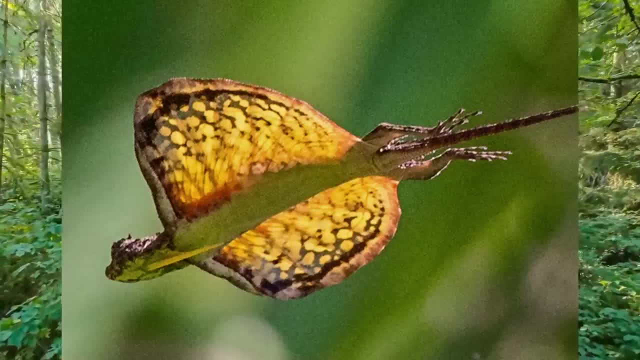 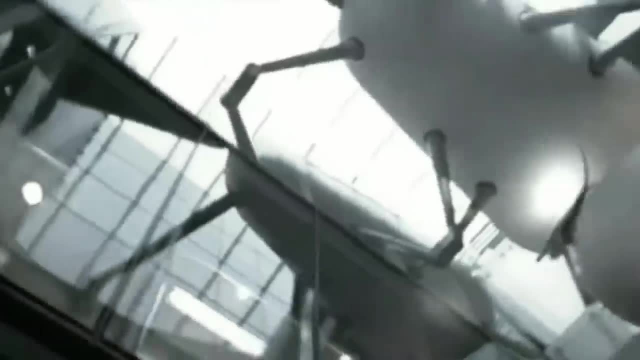 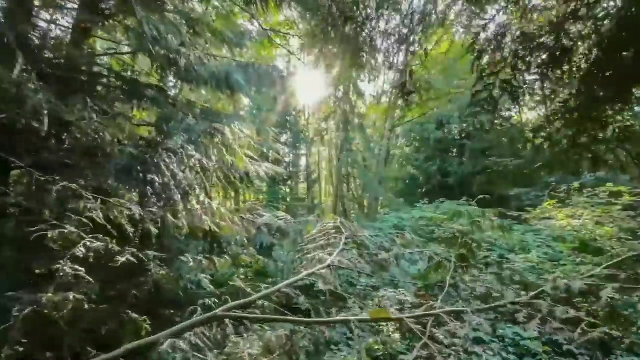 from tree to tree in a similar way to the Draco lizards of today, Meaning that this was the first time that any known group of vertebrates evolved to take to the air in any capacity. This wouldn't be powered flight like what the insects of this time could do, but it was enough to avoid predators. 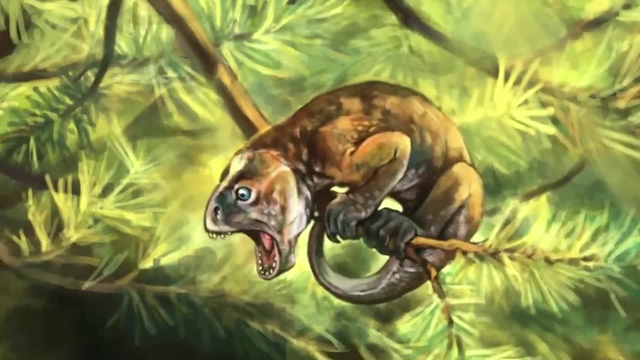 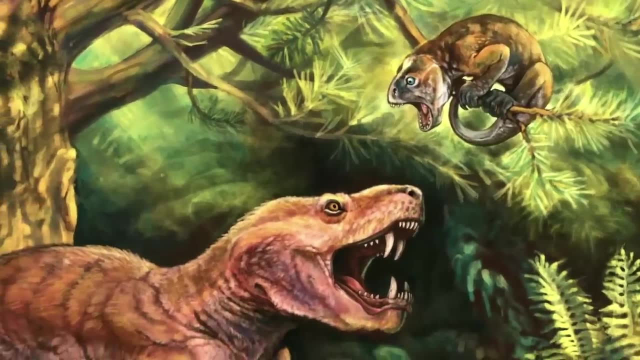 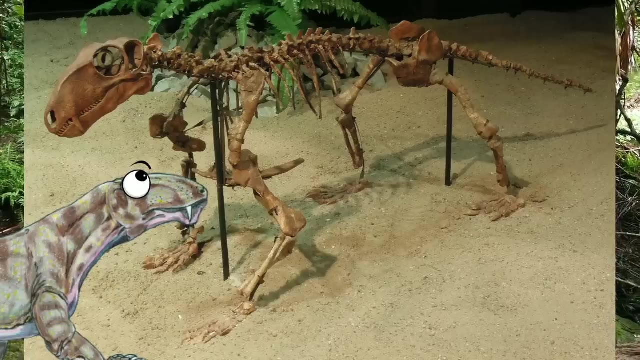 and navigate the trees. And that was definitely a necessity because, in place of the Dinocephalians, a new group of therapsid carnivores were going to experience the same wave of adaptive radiation as everything else living at this time, The descendants of the animals like Biarmosuchus. So you know what that means. 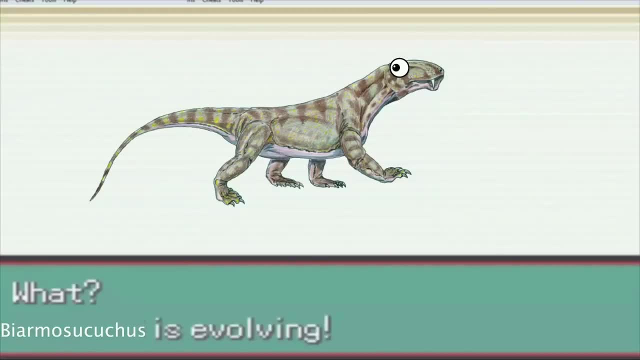 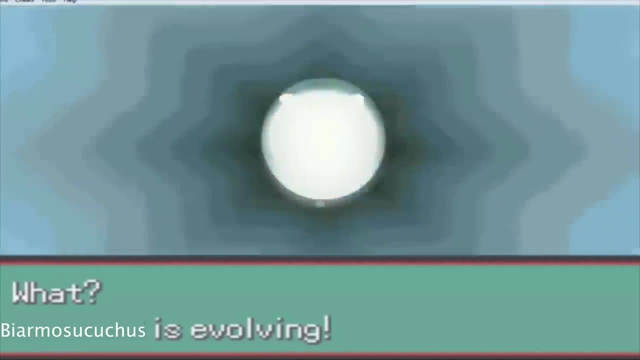 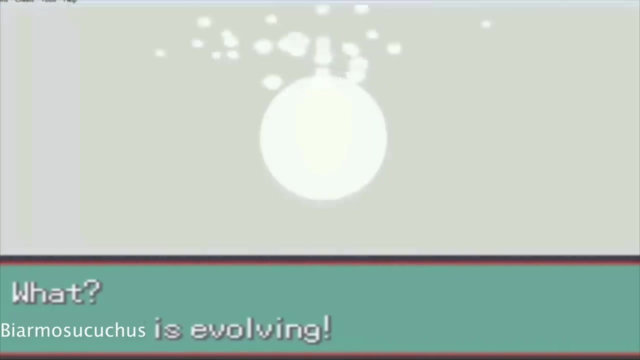 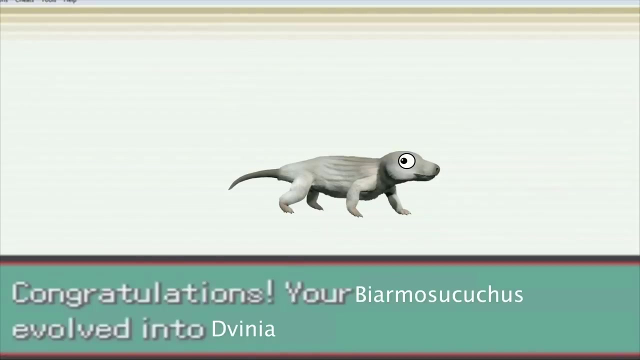 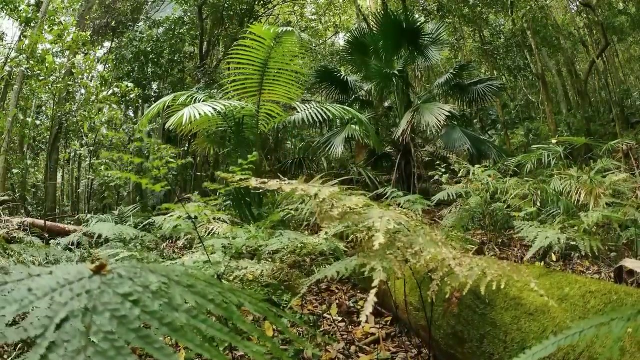 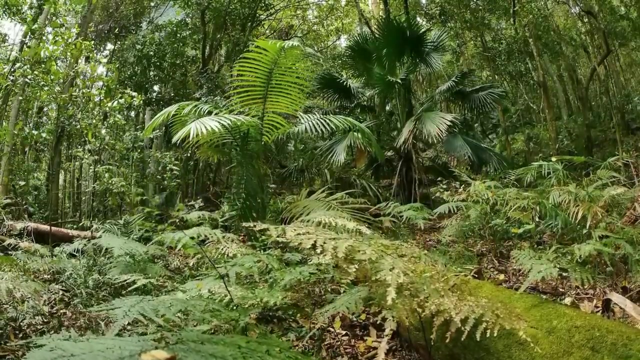 It is time, Tim, Tim Time to take over the world. As we arrive at 252 million years ago, despite all the trials our planet has put our ancestors through, it seems that we were finally coming out on top. Life had finally bounced back and we were. 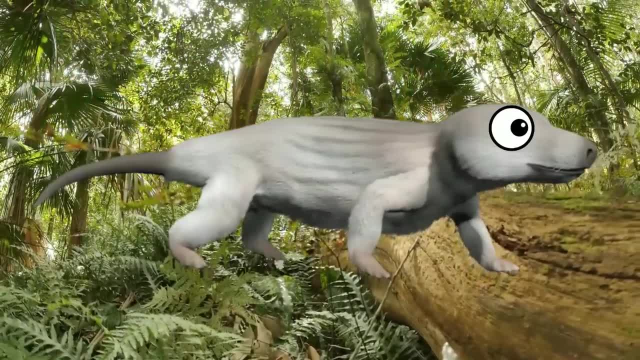 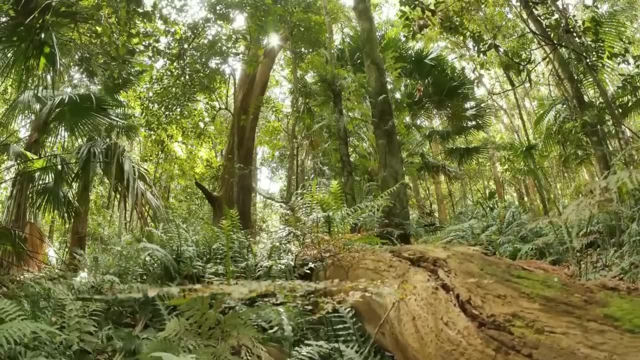 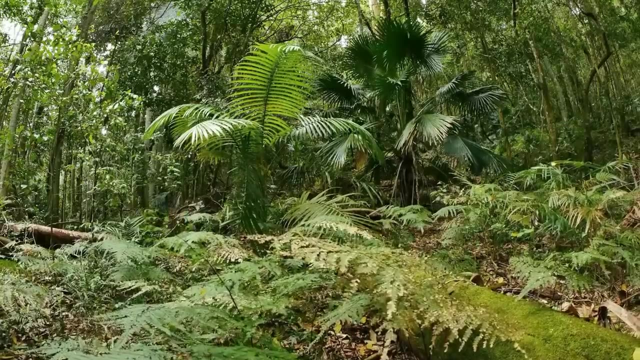 able to get our hands on land And, in fact, become even more diverse and widespread than ever before. The coastal forests of early Ginkgo, Cycads and conifers were teeming with life, With fish and Timnospondyls still in the rivers, Insects and arachnids scurrying on the ground and flying in. 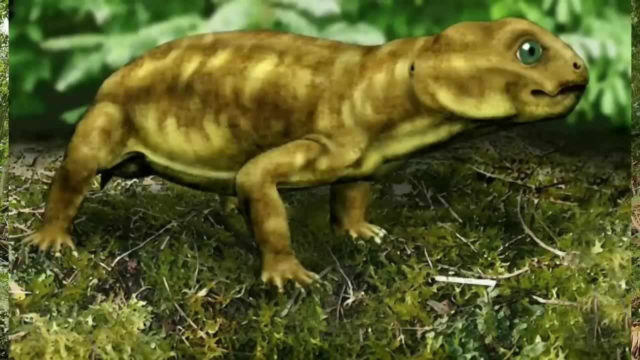 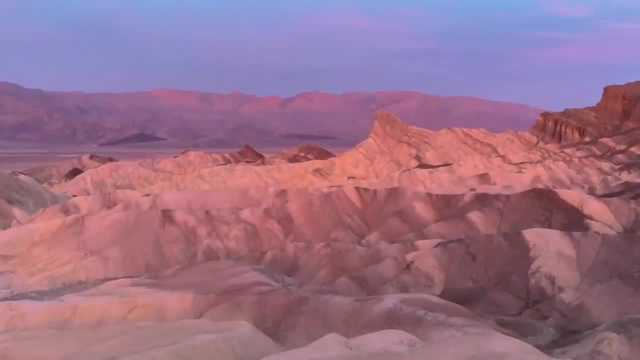 the skies And various different reptiles and synapsids, both browsing on the low brush and climbing among the trees And as we leave the forest- that's when things get a bit worse- would get really impressive. The Dicynodonts had evolved into several larger-bodied forms. 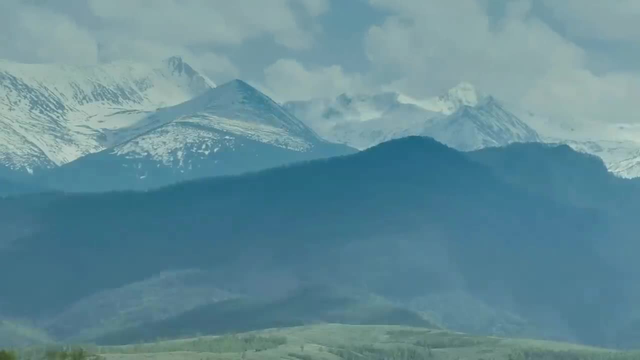 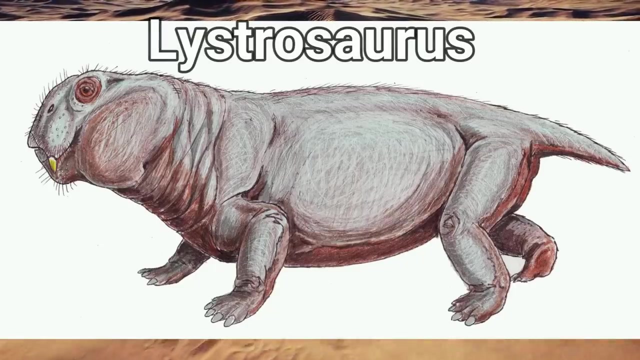 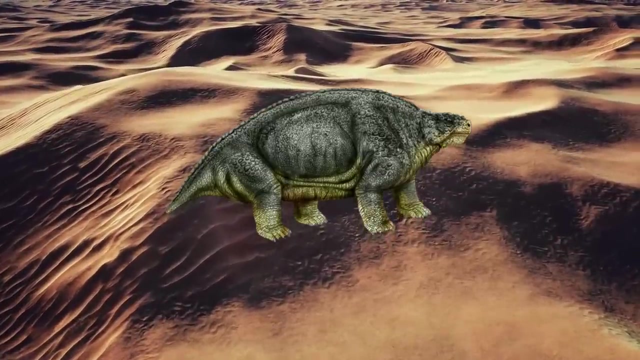 like Vivaxosaurus, but another species was poised to take over the world in a way that had never been done before: the beaver-sized Lystrosaurus. But for the moment they still were not the top herbivores. That role would still be controlled by the Parasaurs, with the armor-plated species. 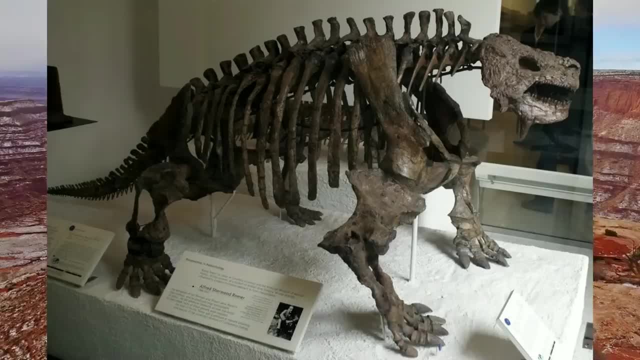 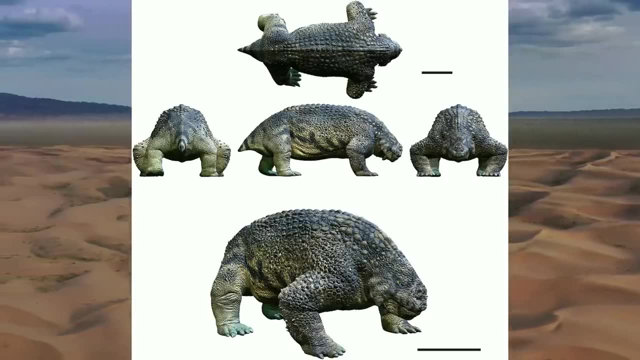 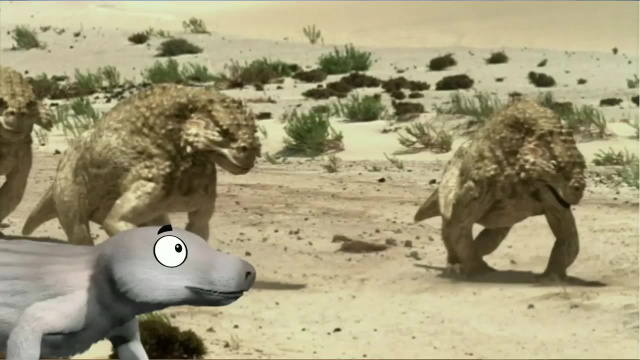 Scutosaurus. In addition to being heavily protected from attack, these reptiles were also well-adapted for the vast interior deserts of Pangea. In other words, they were absolutely perfect for this hostile world. And with all these different animals spreading across the 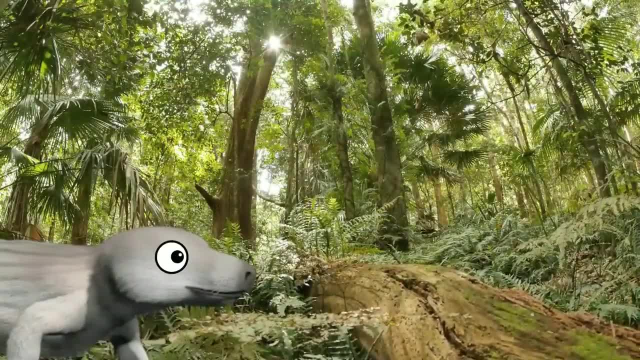 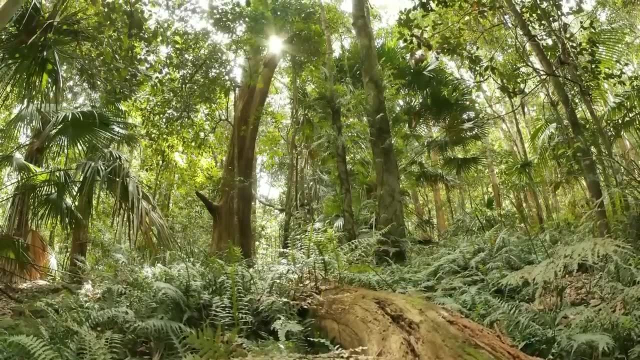 massive continent, there was ample opportunity for new predators to go on the hunt. Particularly one group of carnivores who branched off from animals like Biarmusuchus, called the Dicynodonts, were the Dicynodonts. 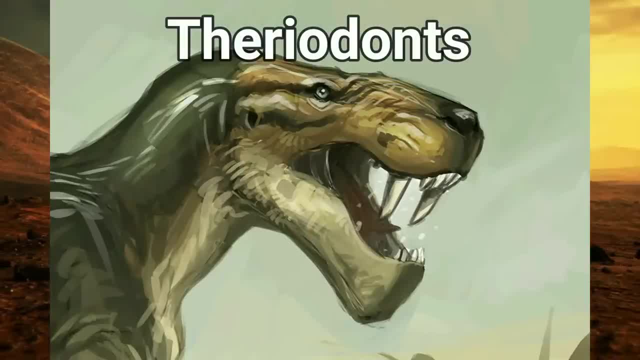 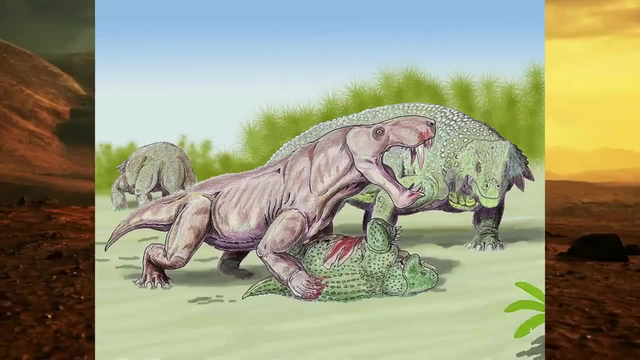 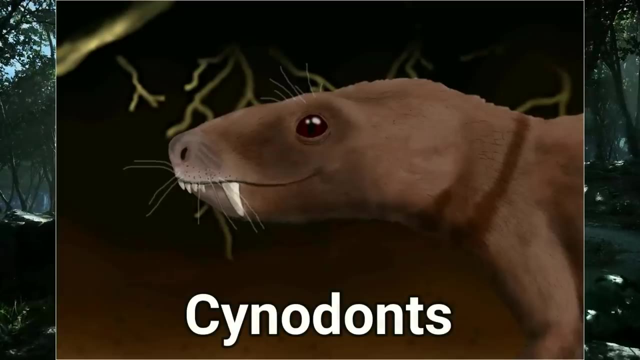 This group really took off in the late Permian. It seems like just about every potential prey species had some member of this group specializing to hunt them, And they did this by splitting into three separate clades the small, resourceful Cynodonts, who would feed on all sorts of small 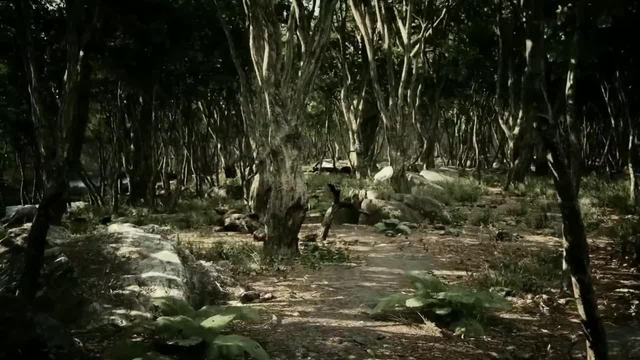 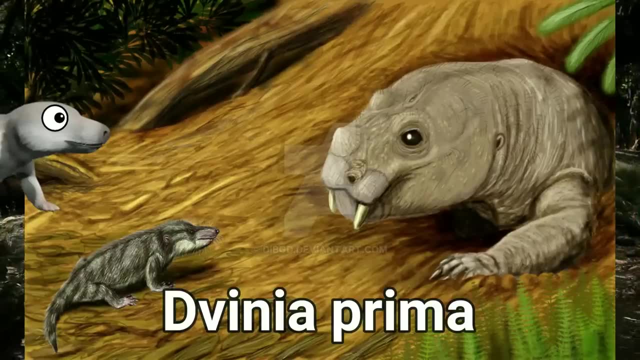 creatures like invertebrates and small reptiles. In fact, many of them were actually omnivorous, like my new form, Divinia Prima, which I love. the name of It makes me sound like a Transformer god, And some even adapted more specialized niches. 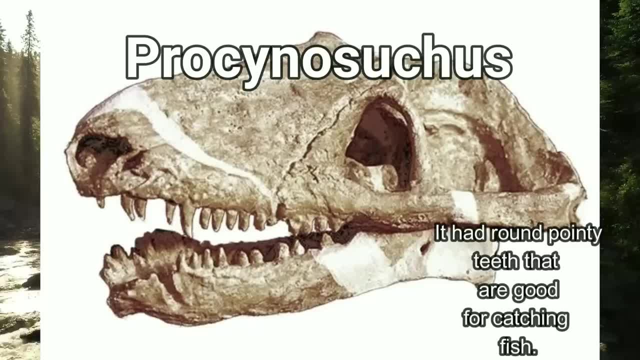 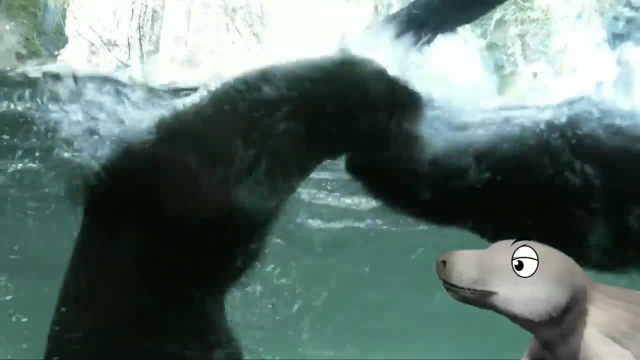 like hunting in rivers, like Procynosuchus, which, despite having a name that suggests it's some kind of crocodile-like animal, I would say, if anything, it was more like an otter lizard, And when you put it like that, this is actually probably the best possible form for Tim Tim. 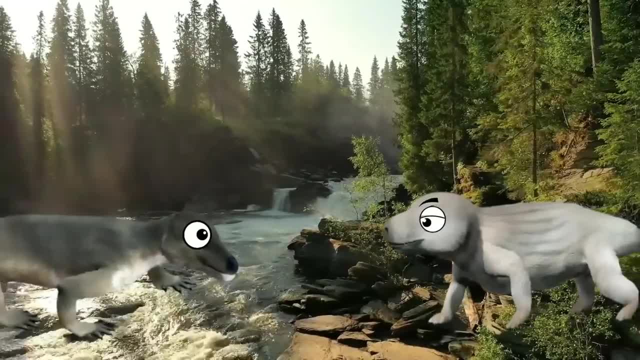 This is great. The world is ours, It really is, And I haven't even gotten into the most powerful predators yet. The next branch of the Therian which is the Therian, is the Therian, which is the Therian, which is the Therian, which is: 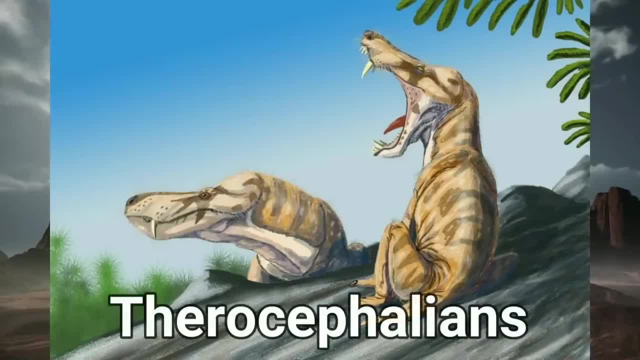 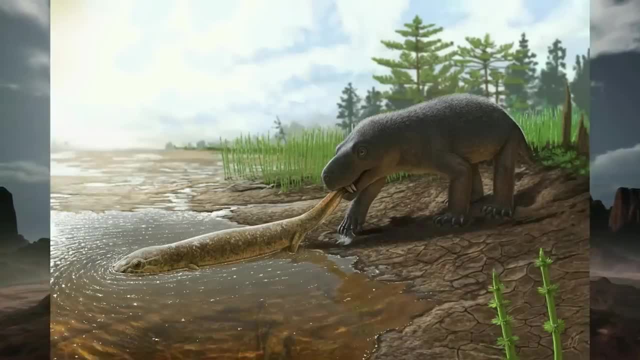 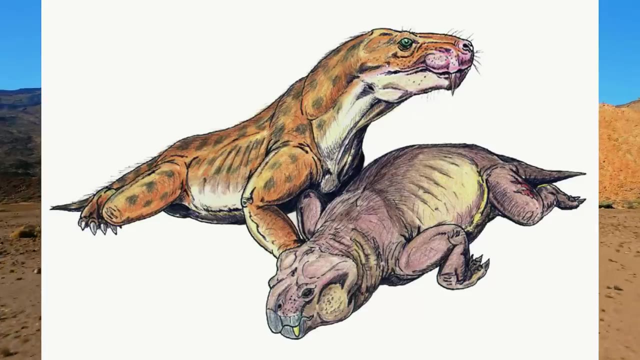 the Therians, The quick and nimble Thericephalians. Most of these predators were medium-sized, about like a wolf, and came in a variety of different species Fast enough on the ground to run down most prey, and likely specialized for hunting things like Lystrosaurus, And it should. 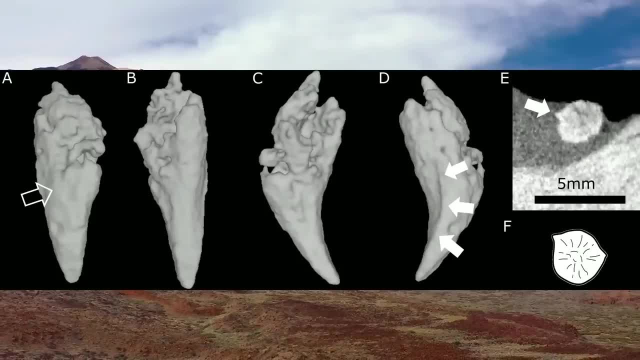 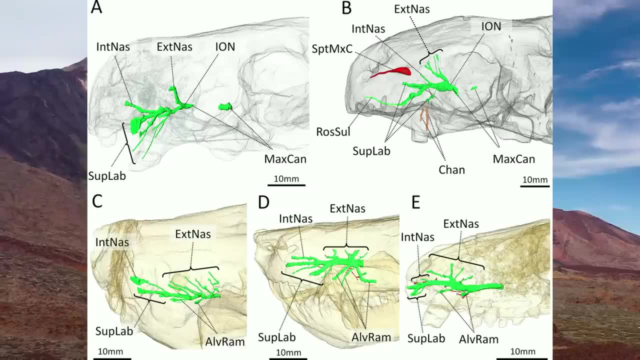 be noted that small grooves on the pronounced canine teeth and what appears to be enlarged glands on the skull of some species suggested the''s presence on the scales on several species that there's a possibility that some of these hunters could have even packed a venomous bite. 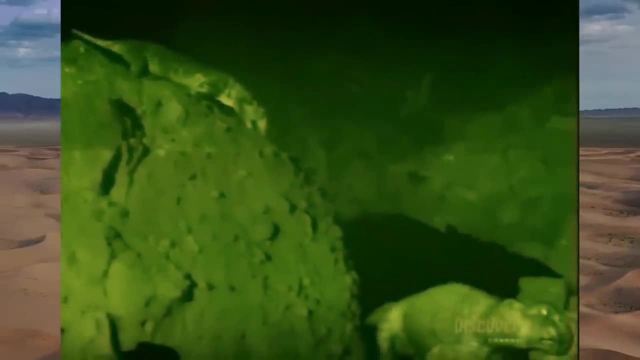 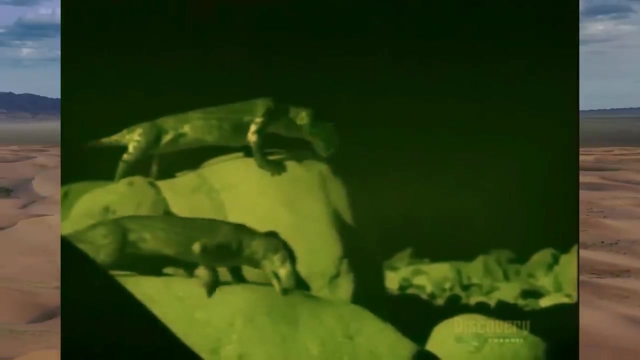 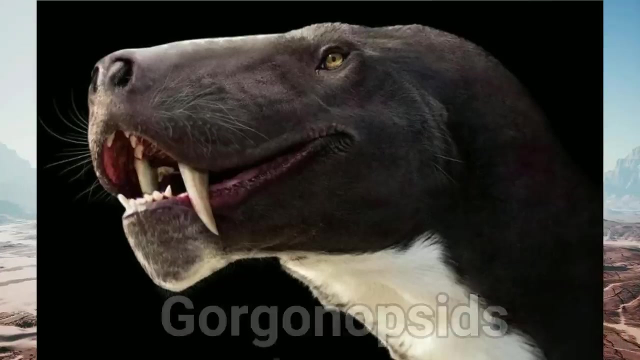 if this is the case, then this is among the earliest known terrestrial vertebrates that we have any solid evidence for being venomous, and it probably would have allowed them to take down much larger prey as well as compete with the true kings of permian pangea, the gorgonopsids, like the other. 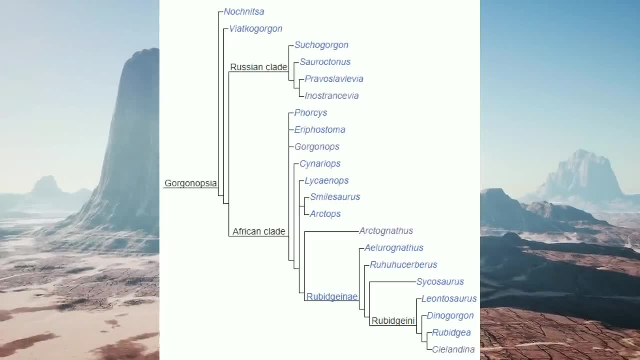 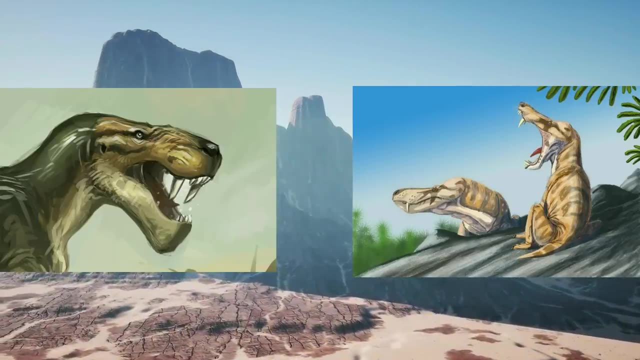 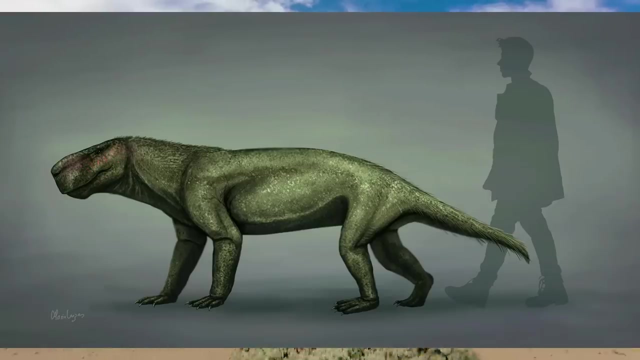 two clades of this group. there were several different species of gorgonopsid. this clade was similar in shape to the therosophalians, except everything was turned up to 11 with these guys. instead of being the size of a wolf, these creatures were over 3 meters or 10 feet long, and 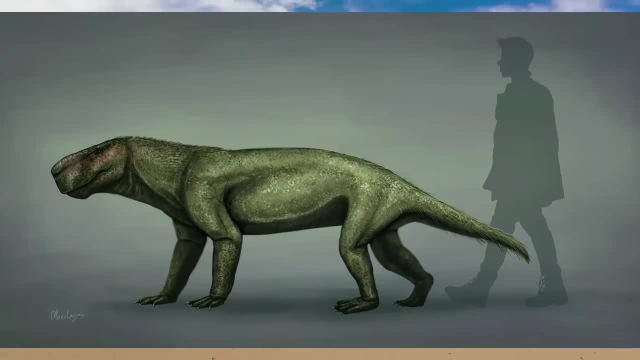 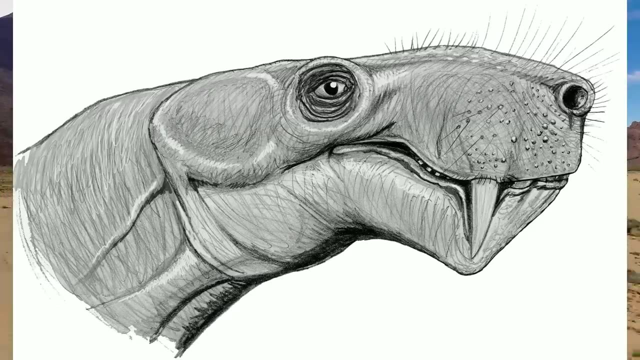 weighed up to 300 kilograms, or 660 pounds, and the pronounced canines that the cynodonts and the therosophalians had were even more than the size of the therosophalians. they were even more so in the gorgonopsids, forming the very first saber teeth, a dental arrangement that has been 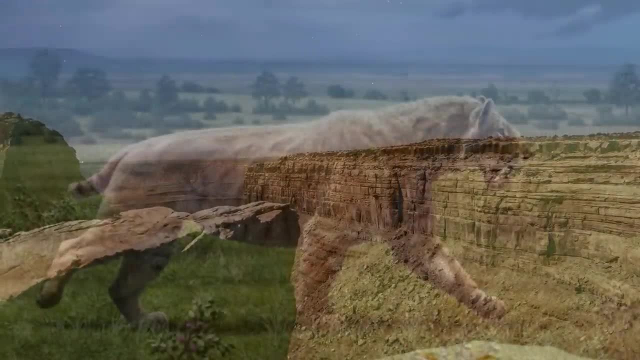 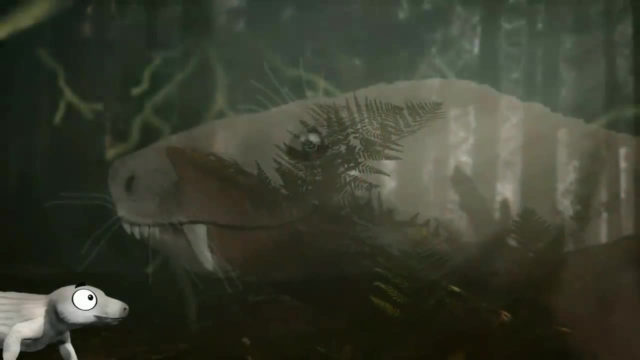 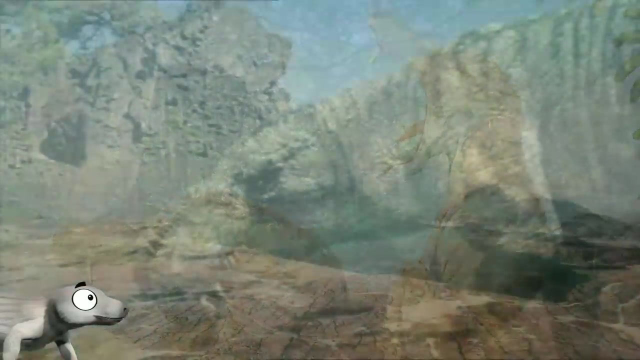 so effective that it would evolve at least half a dozen more times independently in the future. but these guys did it first. if the cynodonts were the cunning, resourceful opportunists and the therosophalians were the venomous, agile assassins, then these things were the ultimate stem mammal. apex predators- a bruiser that was. 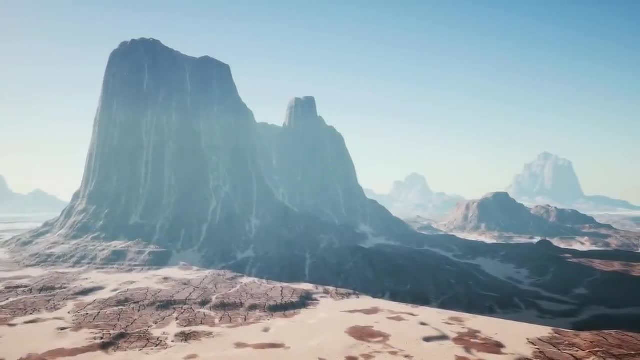 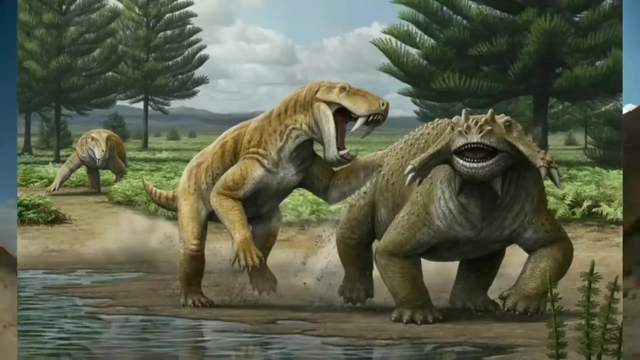 it was anание that came out to kill those homesteaders, ro interviewed by the wealth of clades, as archび is a hunter of the biggest, most well armored prey and, in fact, in the case of ennostrancevia, one of the largest members of this clade was believed to actually 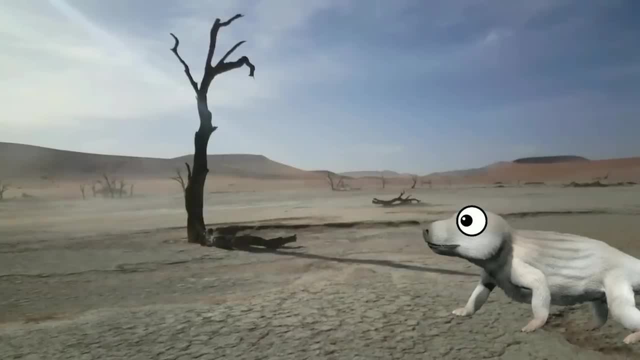 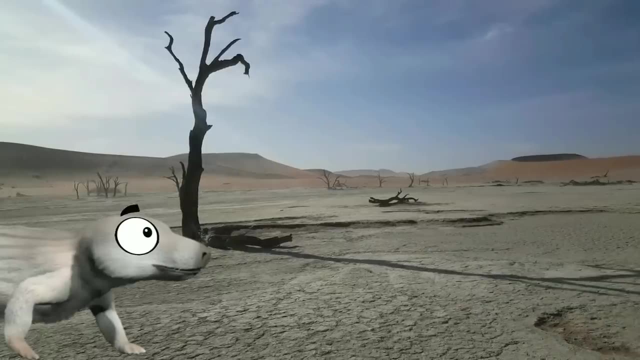 have favored the armored scutosaurus as prey. these animals struggled through the permian, arguably the most challenging period that life has endured yet, and if you think about it, we had written in the letters about the desolation of the lettuces. so, basically, cause the three deathnyards fear to. eat the humans as the themselves over to their bodies and crush them, at the expense of their sorrows, by ever muscle, as everything about them is ginger, and stuff to that is a preparation that was called descobrir, my mother's resurrection, and then, after it was probably done, finally, i'm not sure- 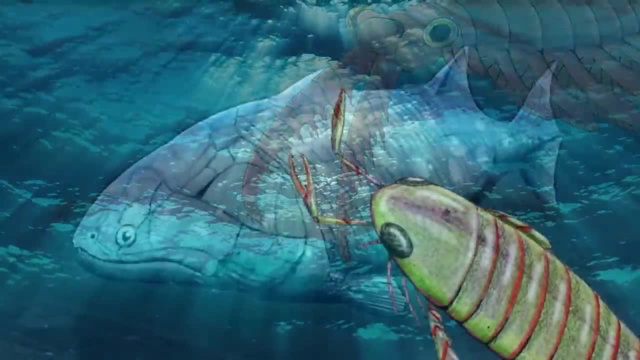 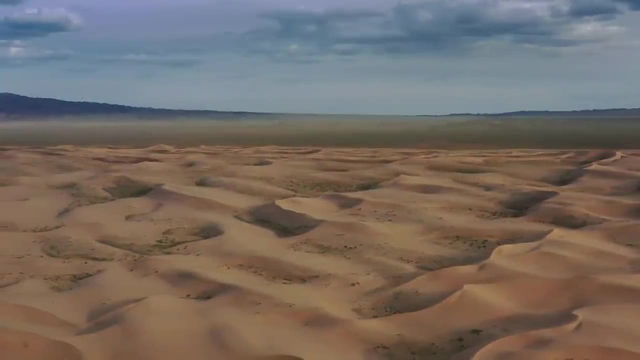 charles orrep 둘. and i said know. it shows, however, by i don't know where some of my hiç was, that we evolved. it was in response to a new threat that was claiming dominance, and by the end it seemed like even the planet was working to make things more difficult. but now the monsters that 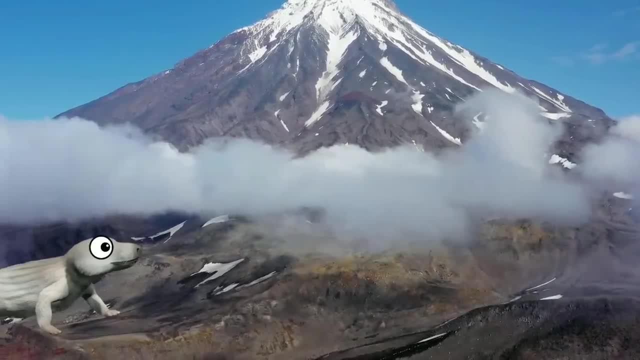 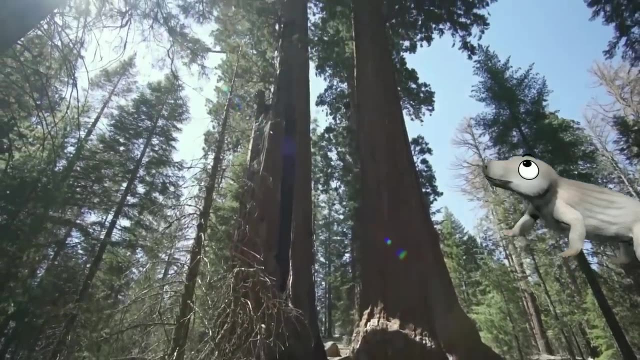 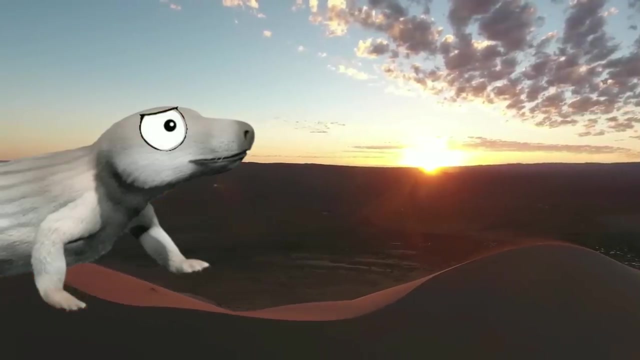 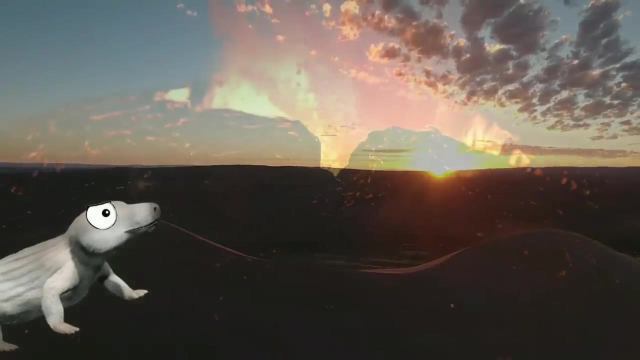 we feared were defeated, all because we learned to live with these conditions that nearly nothing else on earth could. and now we were never going to lose control of this planet again. yeah, we would expand to every corner of the globe and never fall victim to the soropsis or anything else. yeah, and someday we will learn to tame the very planet itself. 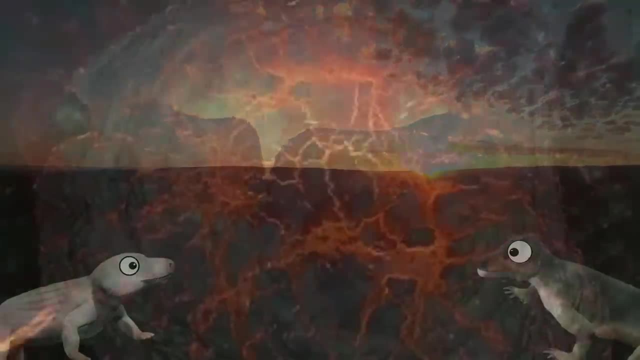 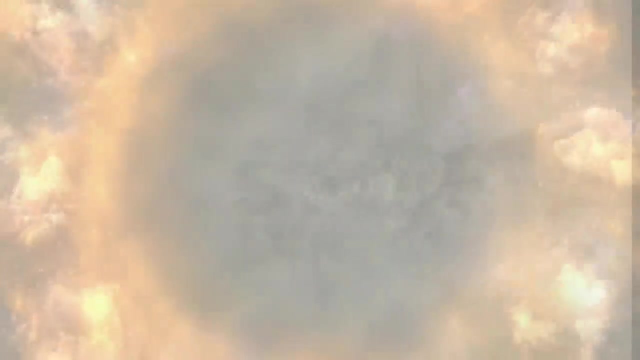 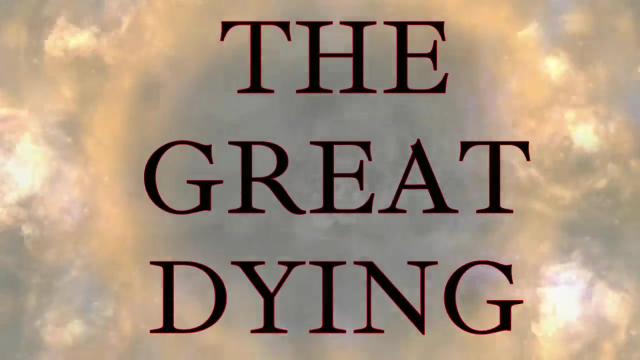 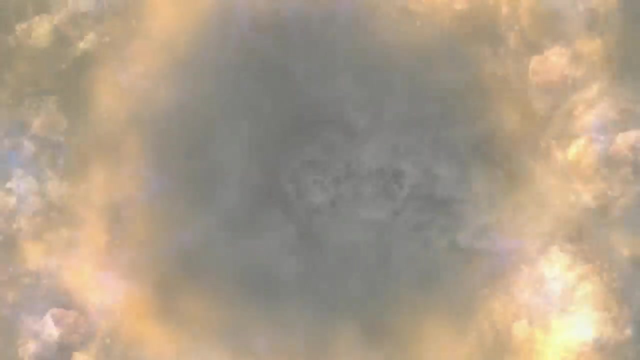 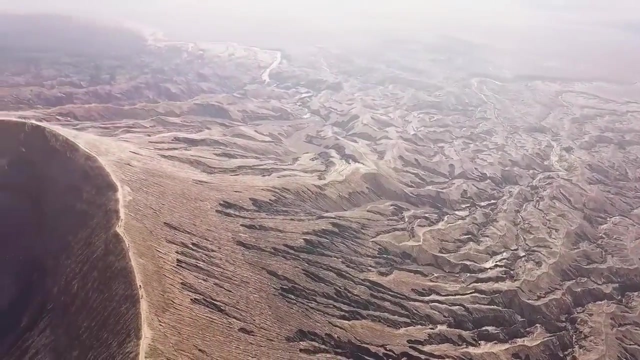 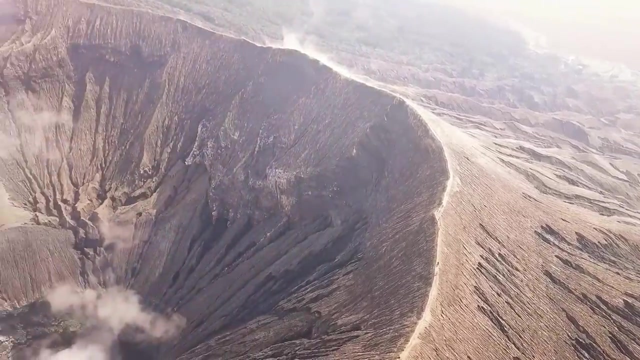 yeah, what the hell was that? what the hell was what? so if there is one thing that has been proven time and time again by our journey through the history of life, it is the fact that no species last forever. these periods of time that we talk about are human constructs. 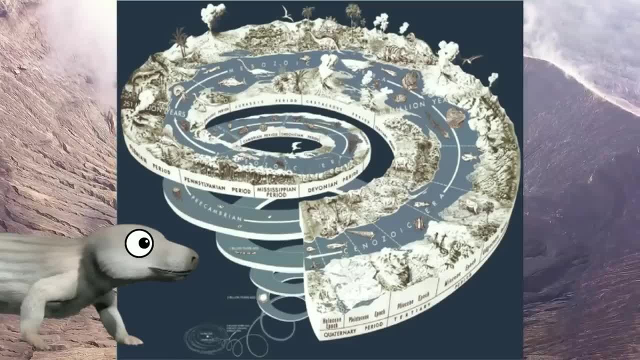 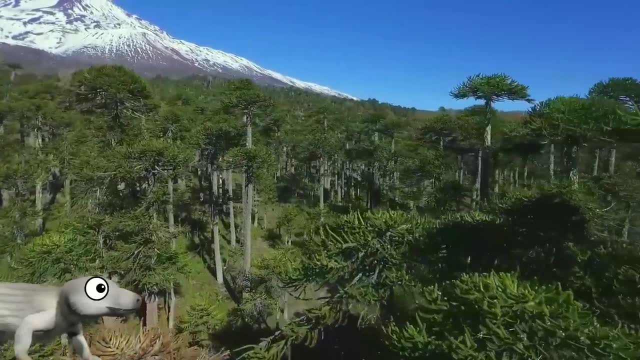 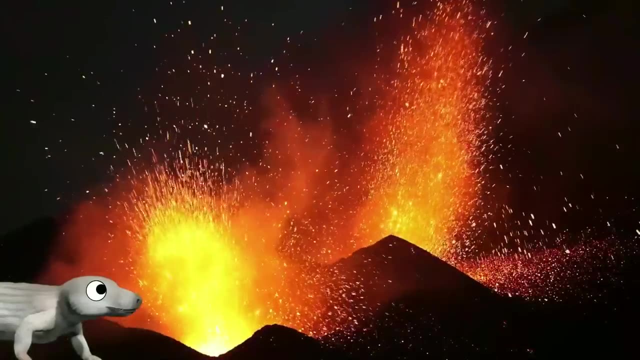 to help us wrap our minds around the sheer vastness of geologic history. and these expanses of time are often punctuated by something bad happening to the things that were alive at the time. these are the extinction events that we normally consider that period's concluding incident, the ones that leave life looking different enough on the other side. 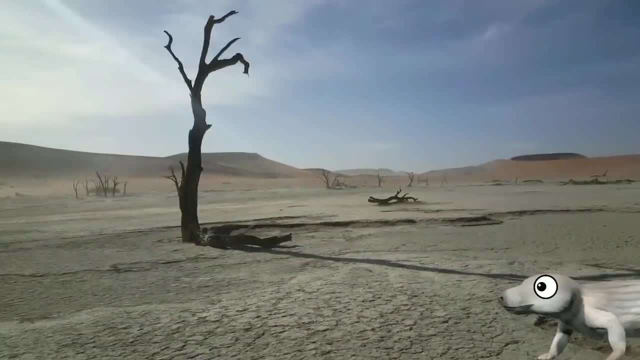 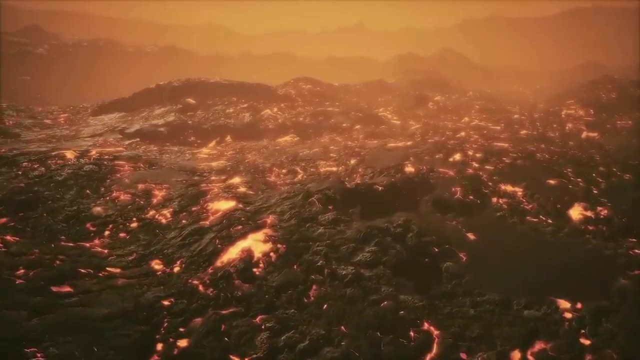 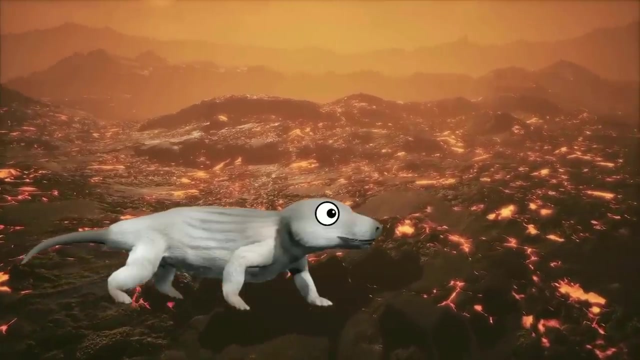 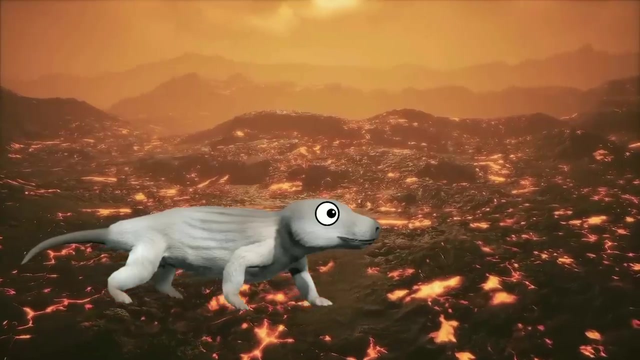 we can say that it is appropriate to label everything that follows in the geologic record belonging to an entirely different period. this has happened to some extent at the conclusion of each of the episodes in this series and in fact, smaller extinctions have happened intermittently throughout time that i had not even mentioned, because the overall effect on the big picture 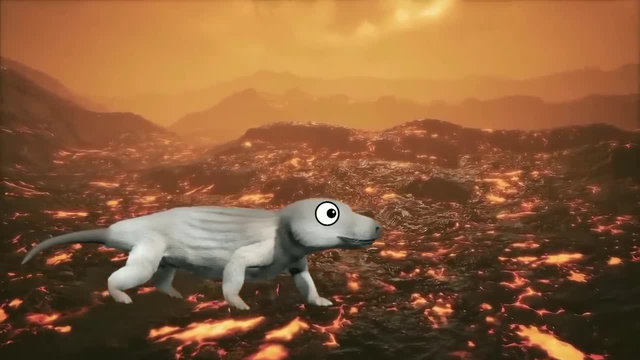 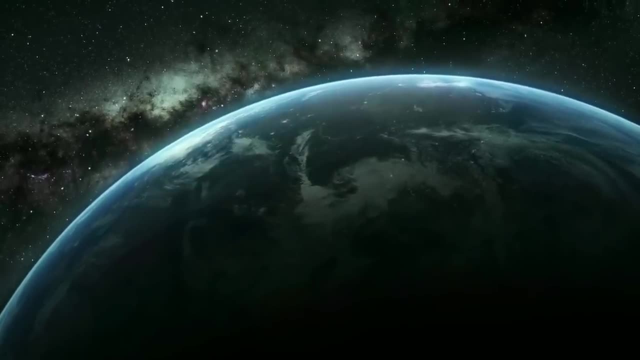 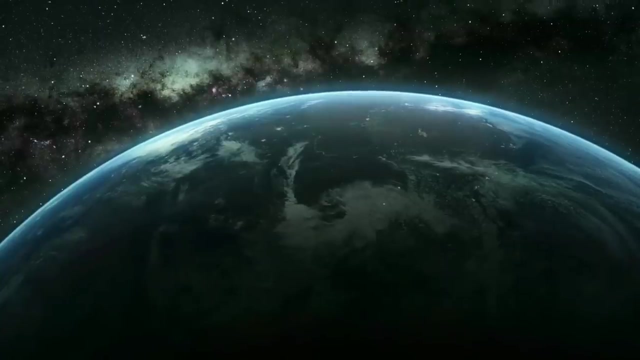 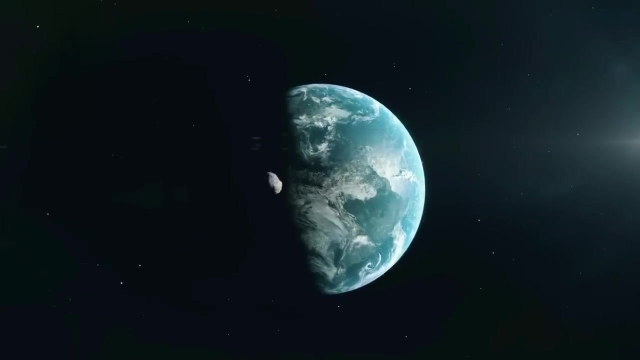 of the story was relatively unaffected. the point here is that extinction is actually a natural part of life. as long as the world keeps changing, life will continue to change with it or fall by the wayside, and in that process there will always be winners and losers. with that being said, however, there are also some events that happened. 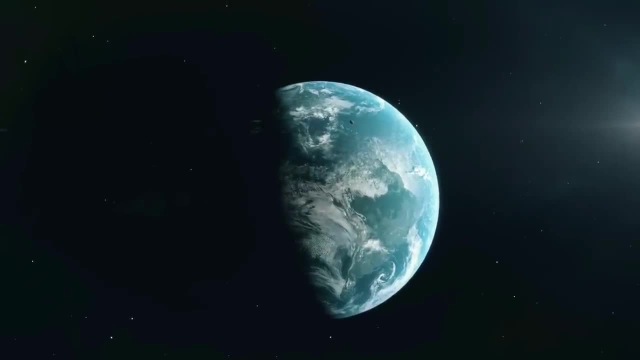 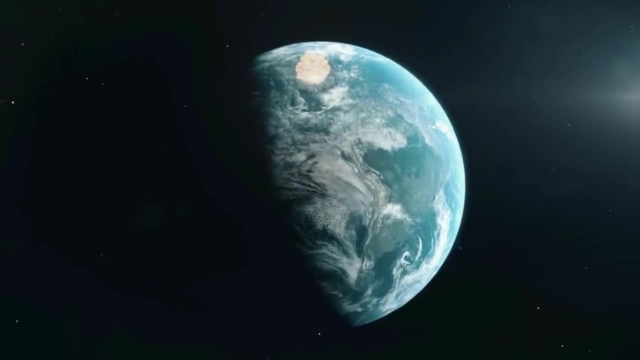 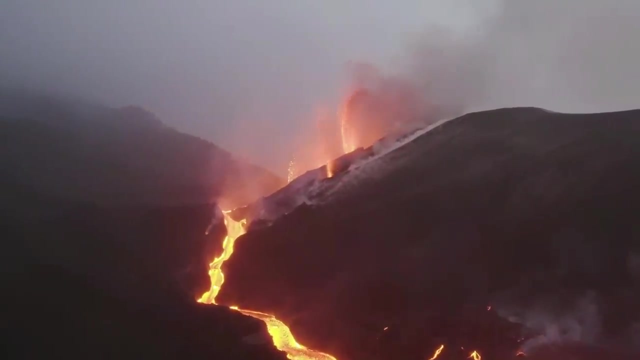 that are so overwhelmingly devastating that life very nearly didn't bounce back, and the ones that are most devastating are the ones that are only the ones that are the ones that are the ones that are the most devastating because they are the ones that nearly took our planet full of life and eradicated it. these are the true mass extinctions, the ones 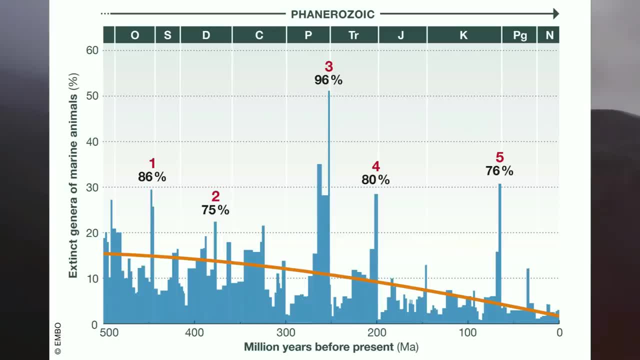 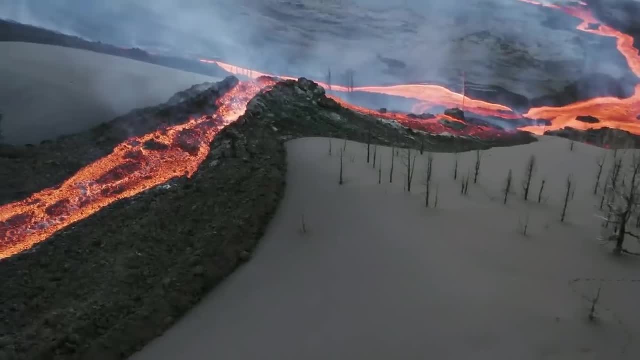 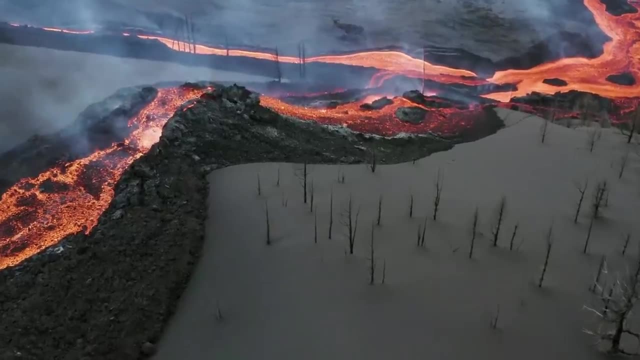 where easily 70 of the species were wiped out or more, and it has only gotten this bad a handful of times, but even among those mass extinctions, this one is the standout. this is the single most devastating event that has ever seen, so i decided that, rather than cover it in one segment of the 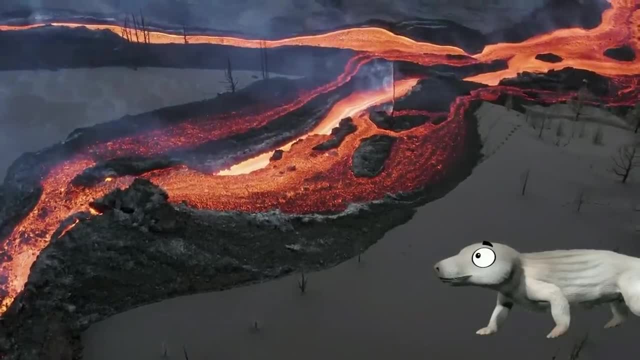 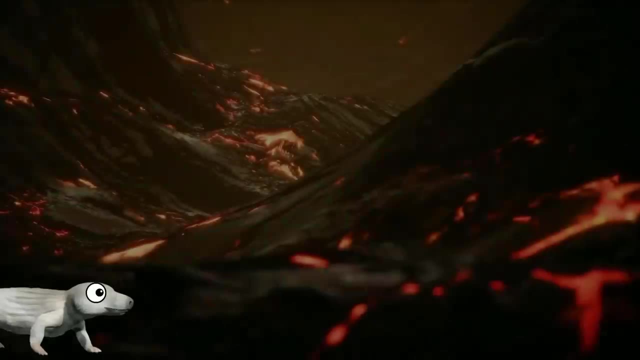 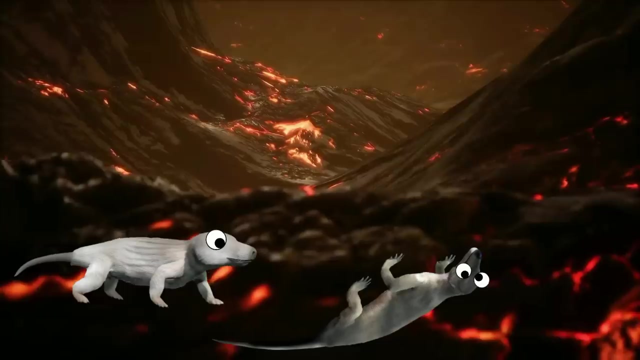 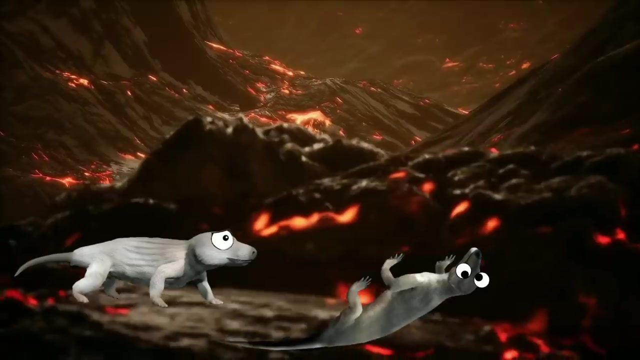 late permian video that it needed its own chapter because, over the roughly 1 million years that this event took place, our world would be changed forever. ah, tim tim, you survived the initial blast and you may live to see the triassic as we cover the great dying. 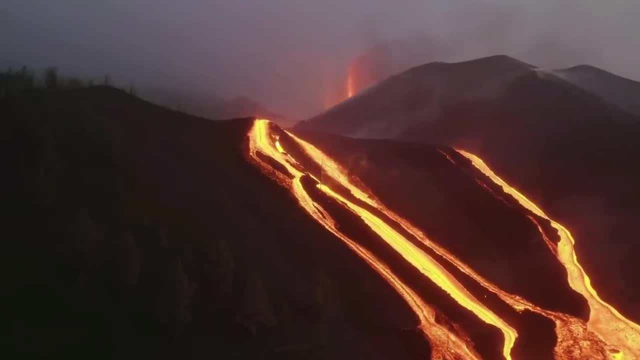 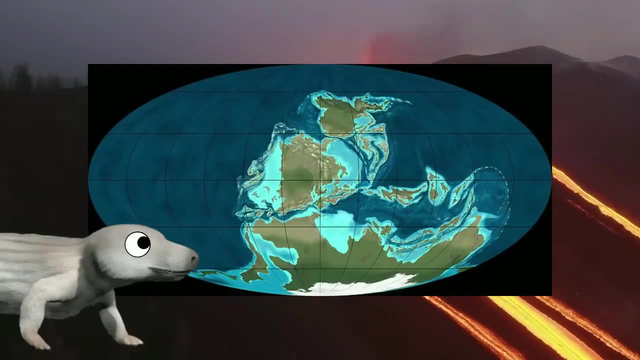 so, if you couldn't tell from the last couple of episodes, there was a build-up to this. ever since the continents had started to come together in the carboniferous, there had been a steady rise in volcanic activity. this led to more mountain ranges rising up during this time. 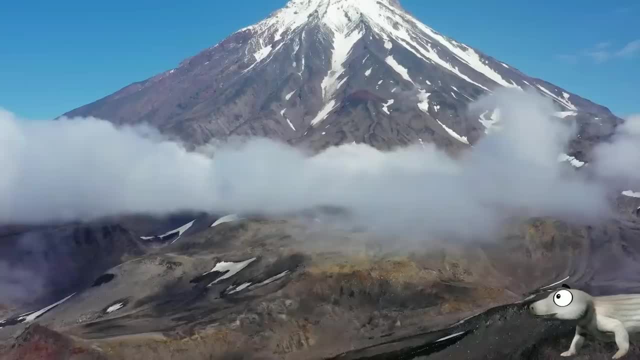 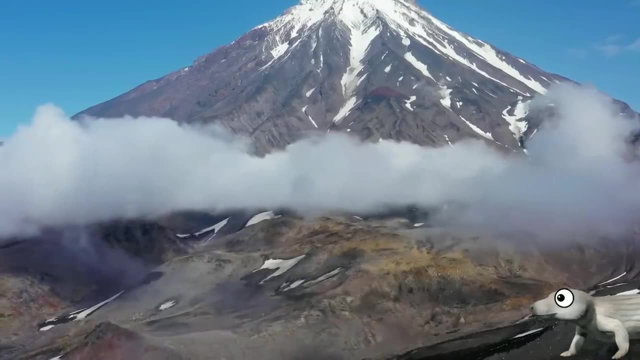 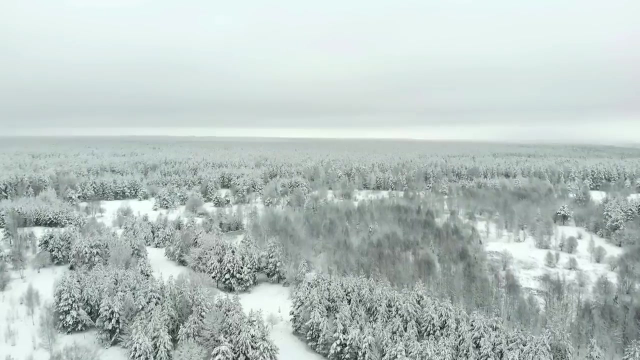 than any other time previously. now there are other theories about things that could have contributed great loss of life, but there is one situation and one location that seems to be the most likely cause: an alarmingly large area of russia that today we call the siberian traps- this nearly seven. 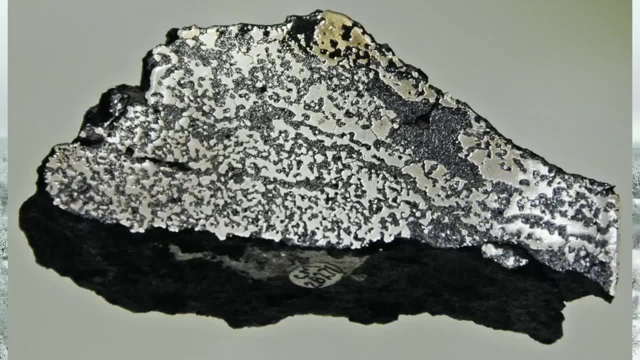 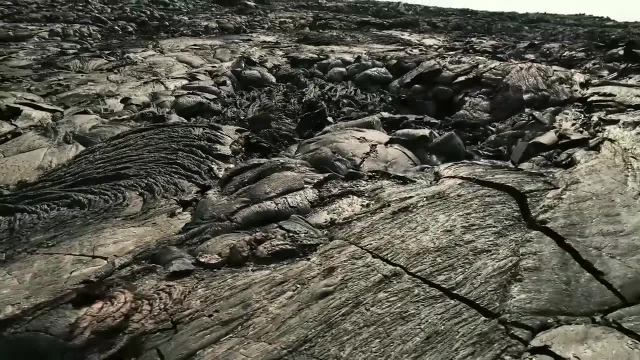 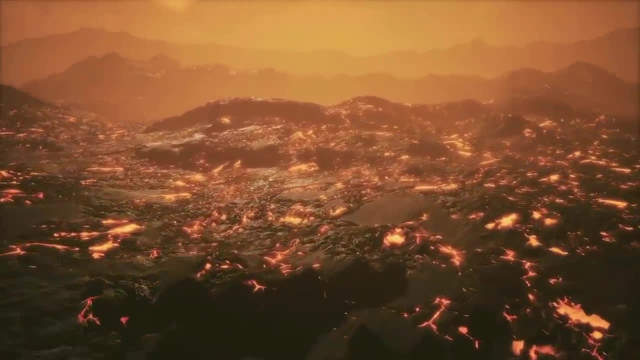 million kilometer area is marked by the presence of basaltic rock, a type of igneous rock formed from the rapid cooling of low velocity lava, usually rich in magnesium and iron. now, this is a very rare case of volcanic activity that is not only caused by the vastness of the area, but also 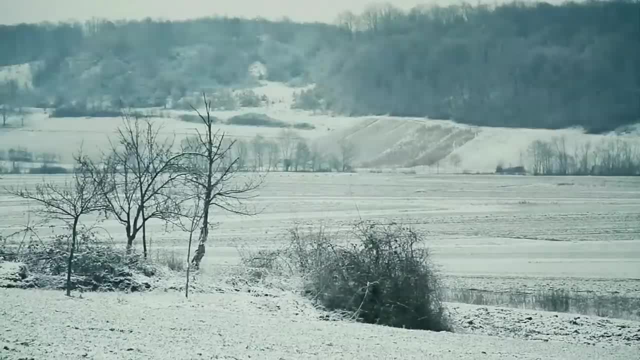 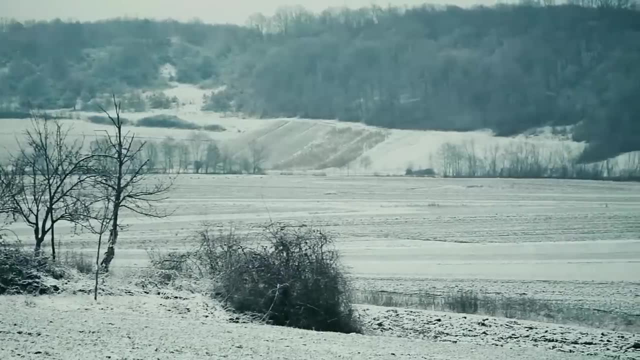 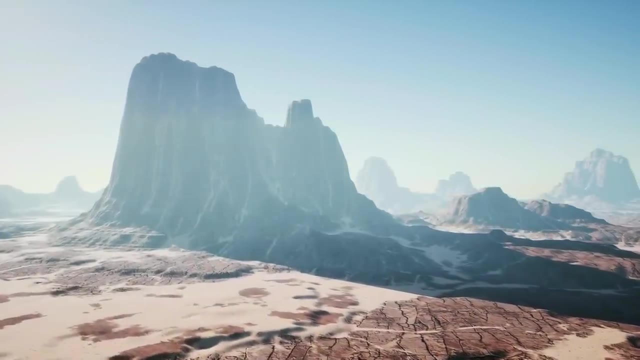 because at a glance, it really shouldn't be here, because siberia doesn't sit on a tectonic plate boundary, like you would expect from a location where a volcano might go off. but this situation was different. instead of the more common cause of volcanism, especially during this time when 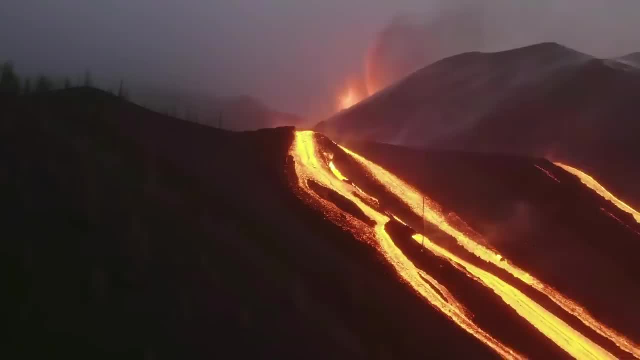 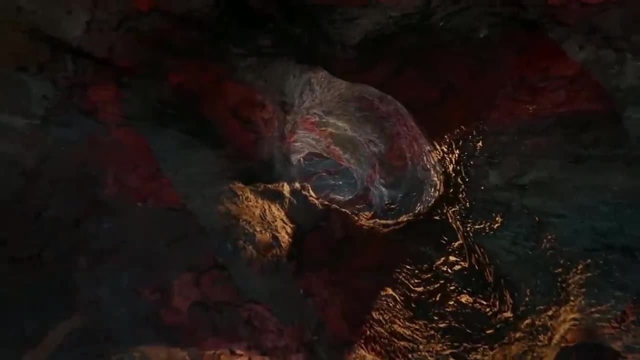 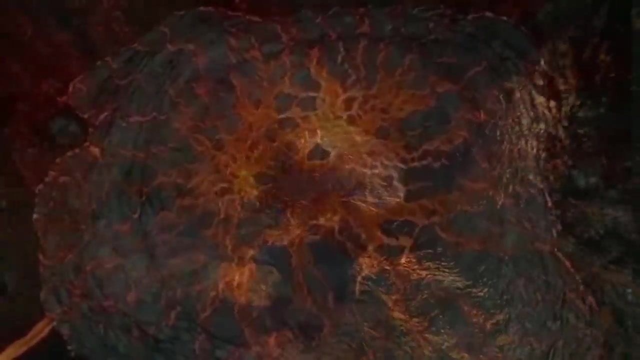 two tectonic plates pushing into each other can cause an eruption. it is believed that this was caused by a mantle plume, where a massive amount of magma starts to work its way up to the surface from the mantle. as this happens, the above layers of crust melt and actually fuel the momentum of 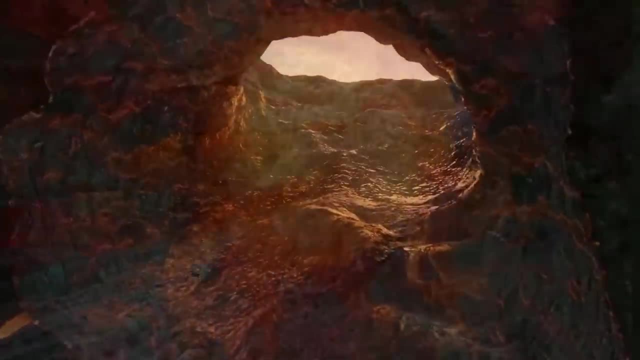 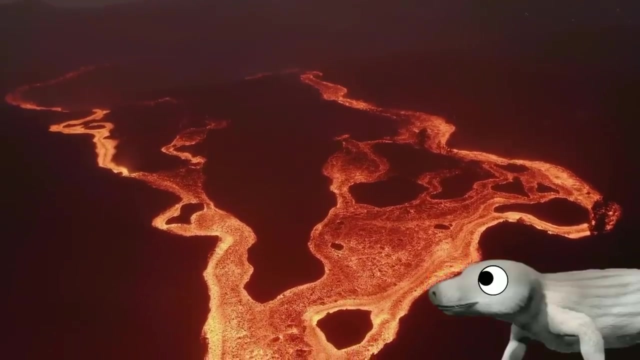 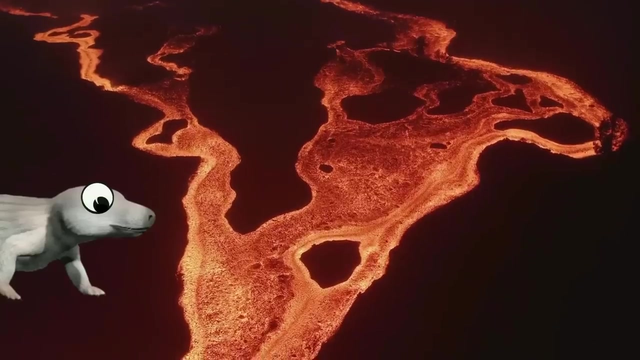 this event until, finally, it reaches the surface. and well, this, this type of situation does not act like a normal eruption. they are a slow burn that started with several eruptions throughout the area, where lava spews out of the ground, essentially forming an inland sea of lava at the surface, and, in this case, about the size of. 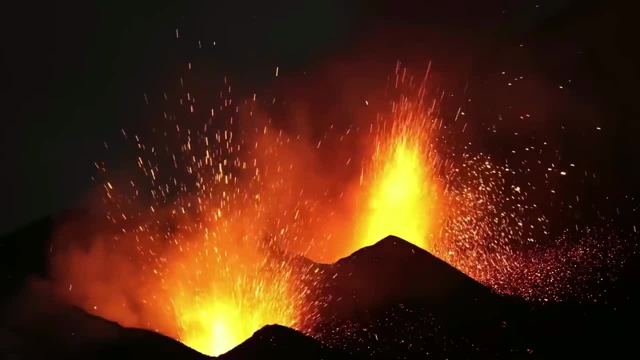 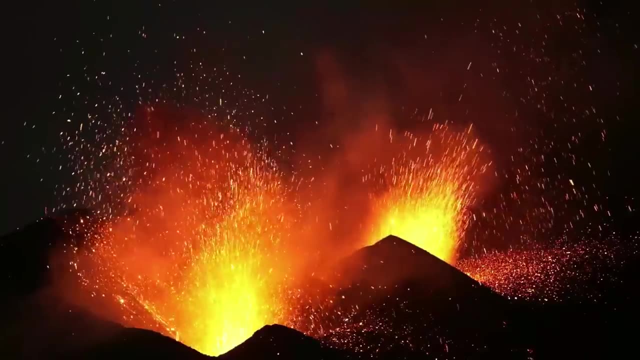 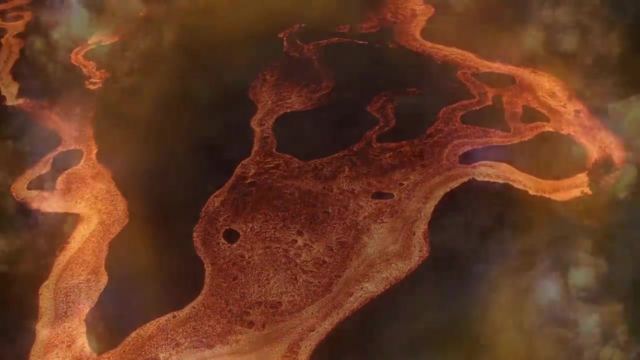 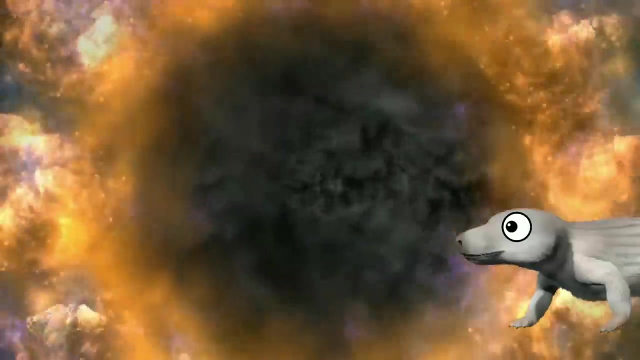 greenland. this mantle plume probably exploded continuously for about a million years, with certain points of heightened activity and long periods of it just seeping lava, all concluding in one final massive explosion. now, as if this wasn't bad enough, there are also many effects to consider, such as the fact that, as all this magma spewed up from the wound in our crust of 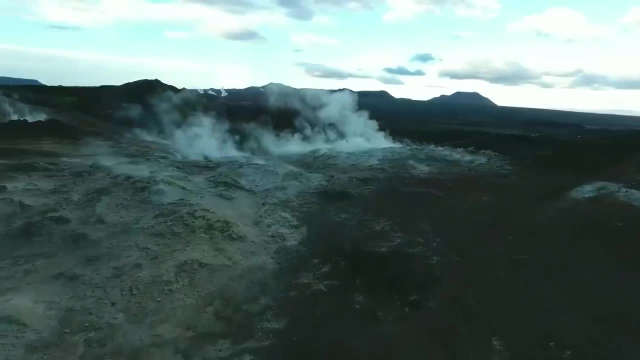 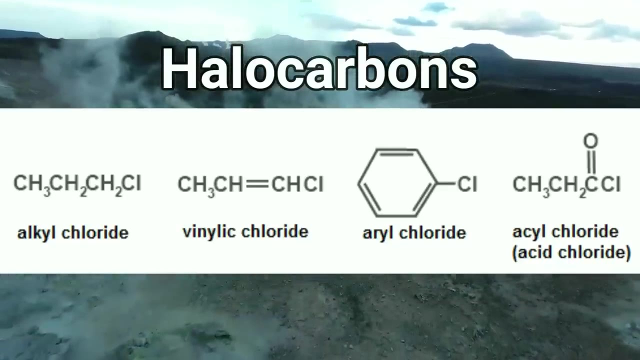 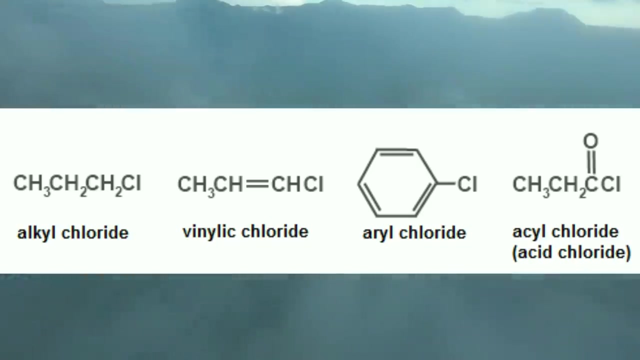 the planet. there would be a massive amount of greenhouse gases being released as a by-product, along with a chemical known as halocarbons. now, for those who don't know, these types of chemicals are directly linked to all sorts of environmental and health issues. for anything, 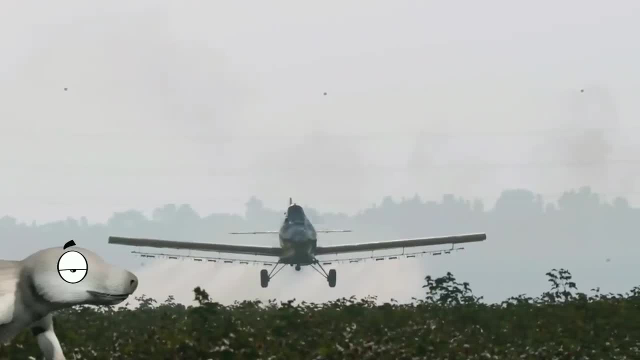 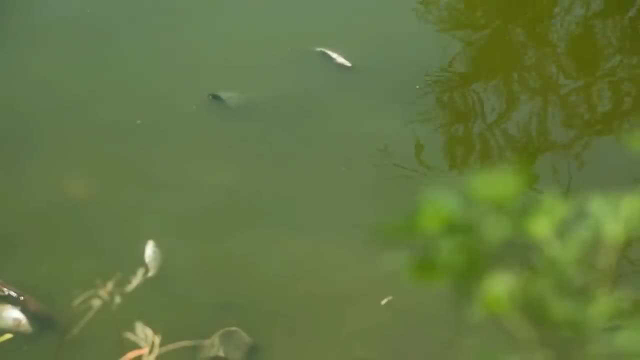 exposed to it, and maybe someday i'll do a video talking about all the times that we've monkeyed a around with this stuff, leading to some pretty bad results. Besides being directly toxic to any animals, it would also rapidly break down the protective ozone layer of our atmosphere. 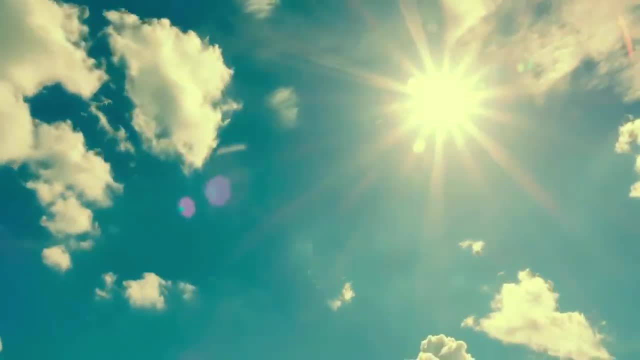 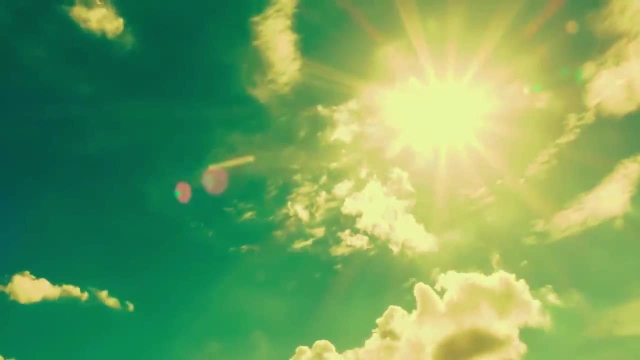 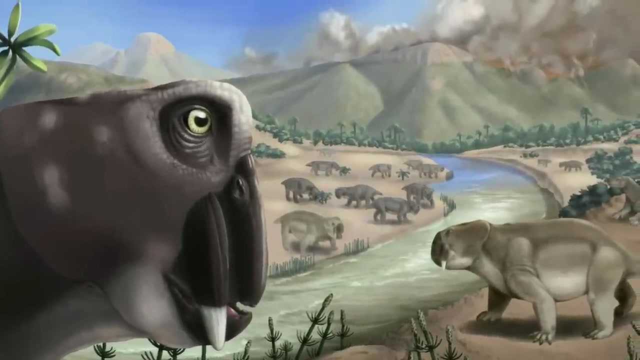 and with greenhouse gases like methane getting pumped into the air and a layer that protects our planet from heating up too much, from the sun being broken down. I'm sure you can see where this is going, Ironically, despite the eruptions of the Siberian traps, absolutely spelling certain death. 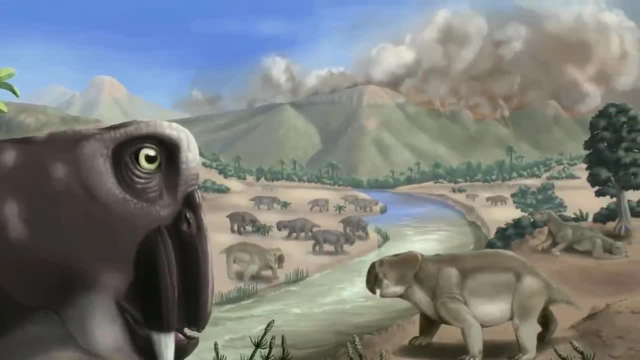 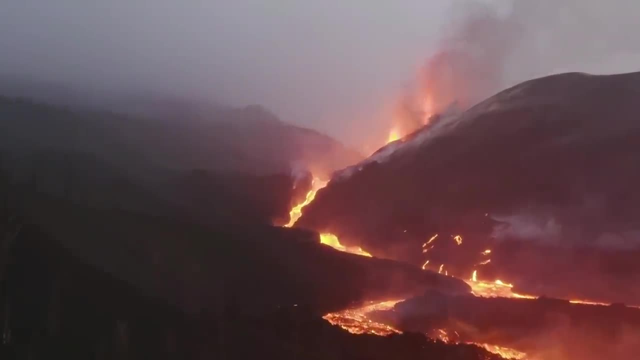 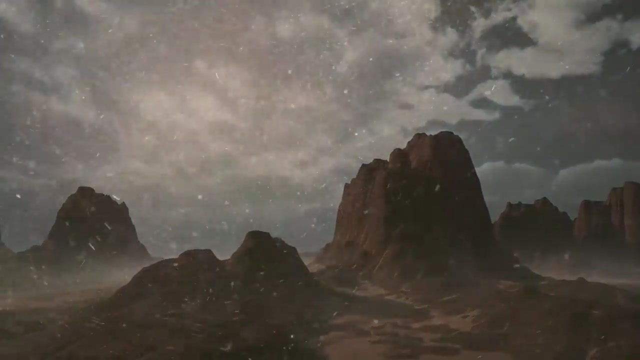 for any animals living in that region of Pangea. it may not have been the blasts themselves that led to the widespread global die-off that took place, but instead a slow die-off of being poisoned, choked and starved, as the planet first got cold as a result of the sun being blotted out by the 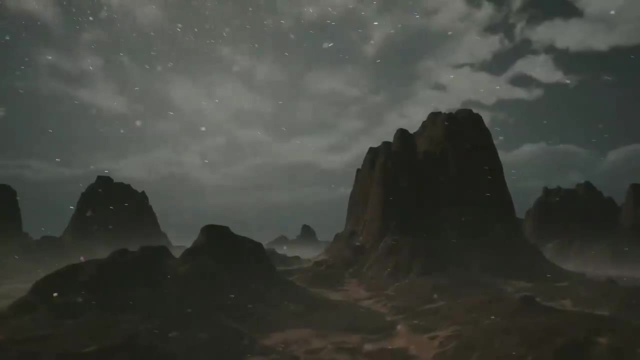 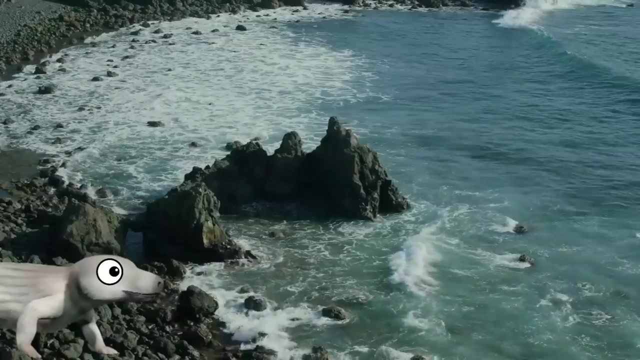 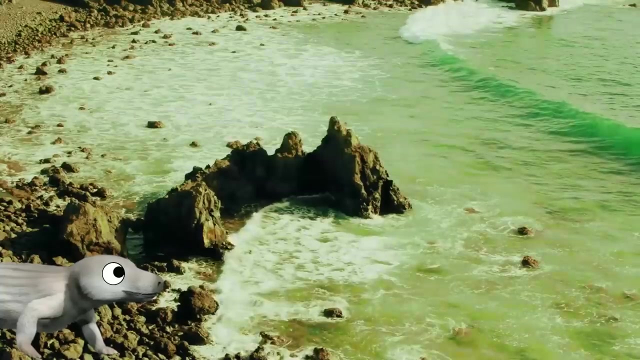 dust to start to warm faster than ever, when the dust finally cleared and the ozone layer was no longer protecting the planet. And by far the worst effects of this would be felt in the seas, where global warming would effectively starve the oceans of oxygen as well as raise the acidity of 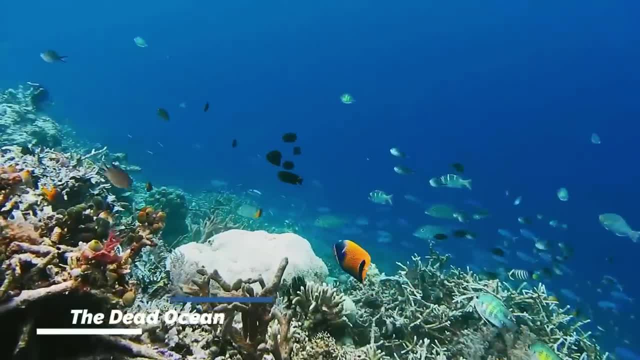 the water, Our oceans had been busy with life for almost 300 million years. at this point, It is where our oceans had been busy with life for almost 300 million years. at this point, It is where our oceans had been busy with life for almost 300 million years. at this point, It is where our 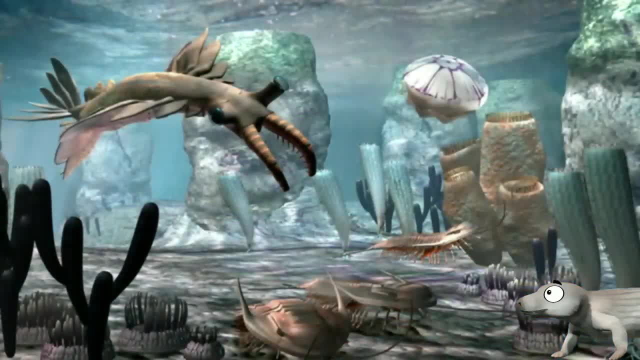 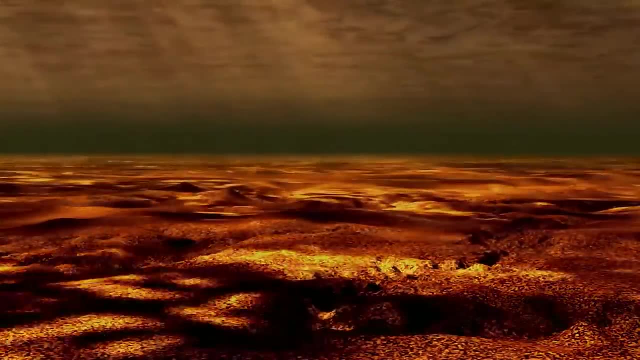 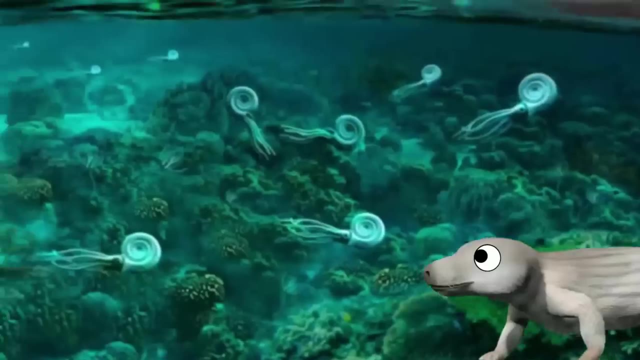 story, as well as the story of everything else, began, And although it had had its fair share of die-offs along the way, nothing has compared to this And, in fact, it's safe to say that nothing ever will shy of the actual death of our planet, Because, if you looked at the oceans- 251 million. 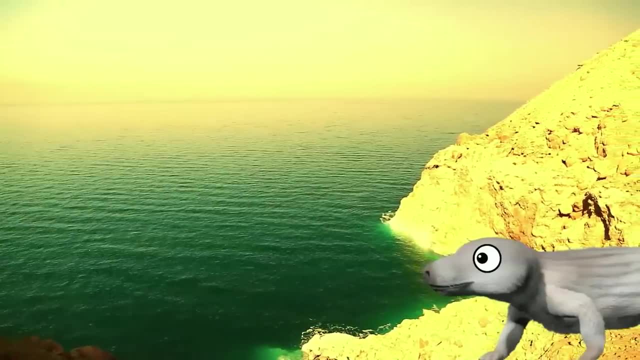 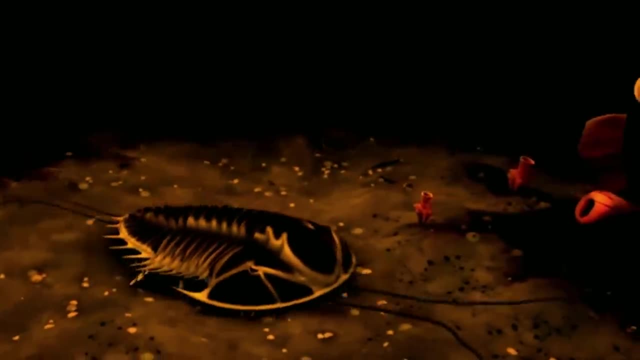 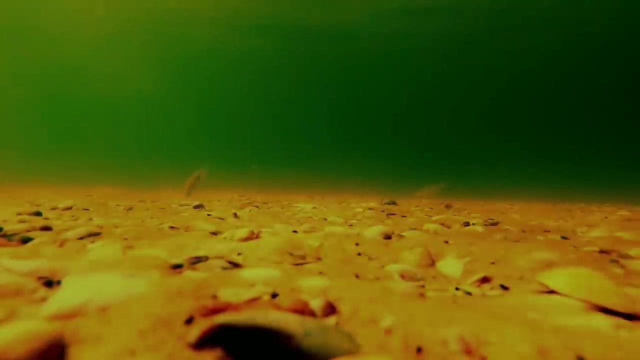 years ago you would swear that's exactly what was happening. Many faces that had become staples up until now, some going all the way back to the Cambrian explosion, were completely erased. The echinoderms were almost entirely wiped out, with 98% of the cranoids and 100% of the blastoids dying out. 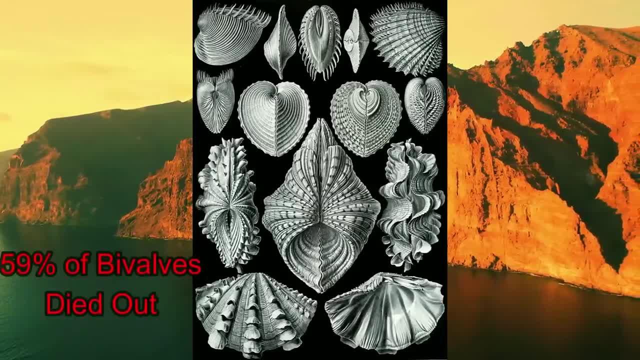 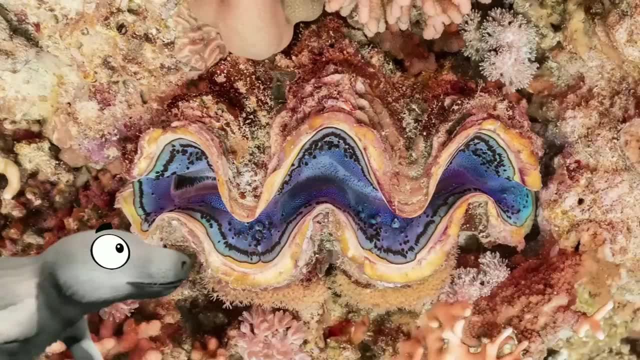 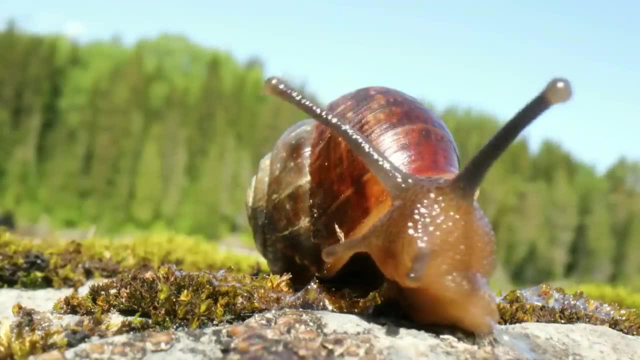 Bivalves lost 59% of their species, which is lucky by comparison, Or a testament to how hardy the simple yet effective design of a clam is. the gastropods would lose 98% of their species, showing how close we came to such a simple creature as a snail no longer being part. 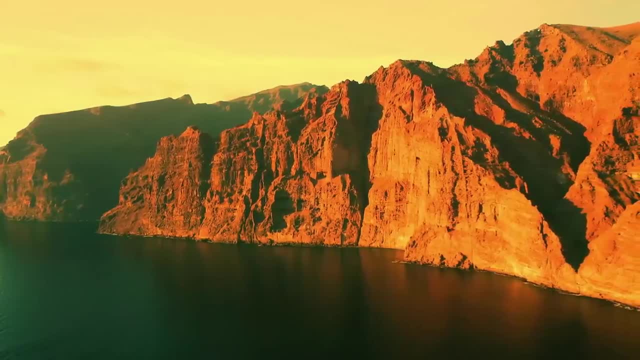 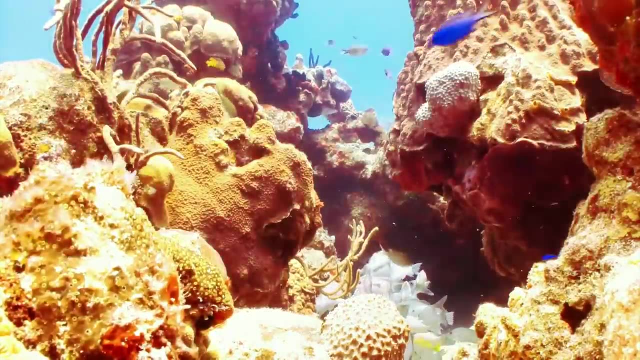 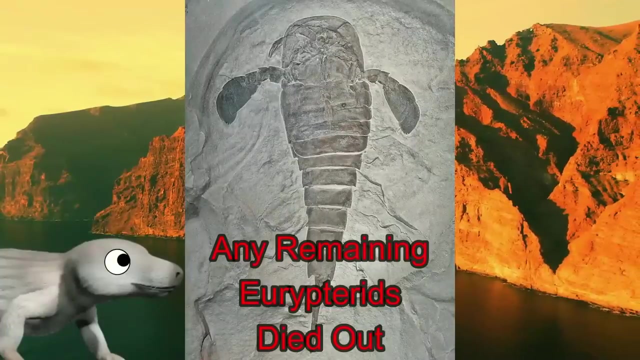 of our world, But if you want to consider what a very different world, specifically in the oceans, would have been like, we also very nearly lost corals as well, with 96% of the paleozoic coral species dying out. If there were any eurypterids left by this time, they were completely gone. 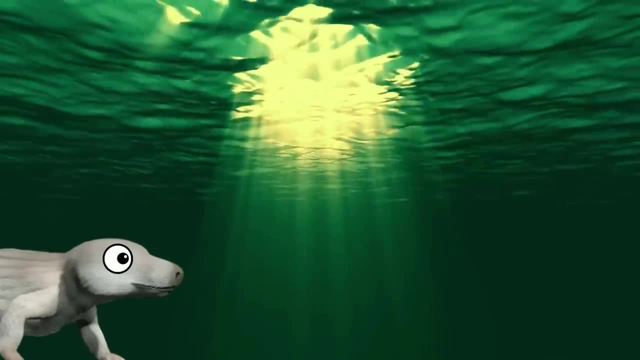 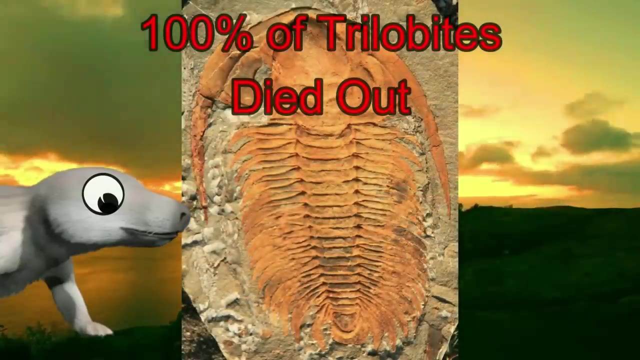 Although there is some debate on whether the last of them were already gone by the end of the Permian, But what we do know is that this was finally the end of the line for the trilobites, A class of organisms. 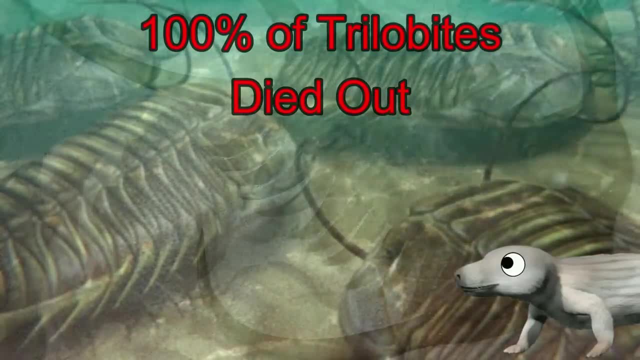 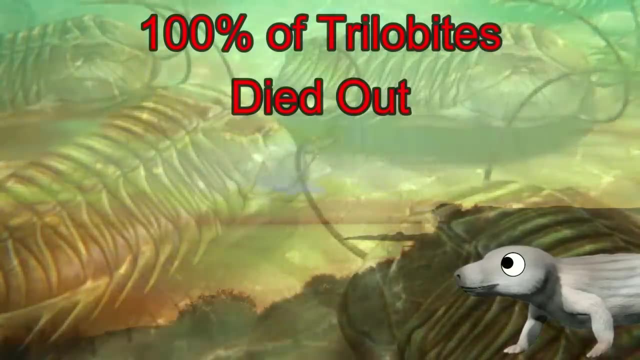 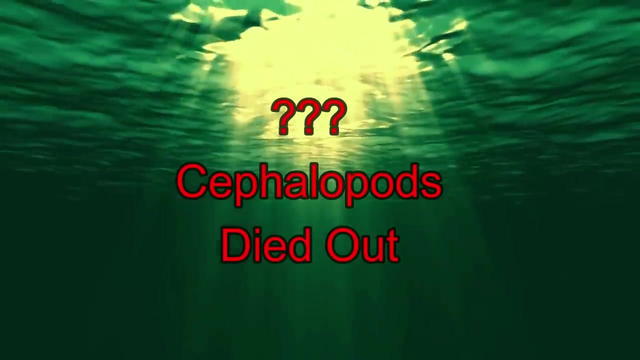 that had endured everything that the animal kingdom, as well as the planet itself, could throw at them for a staggering 270 million years, were done, And although it's hard to pinpoint exactly how hard the cephalopods were hit, because many species don't have many hard parts to fossilize to begin with- 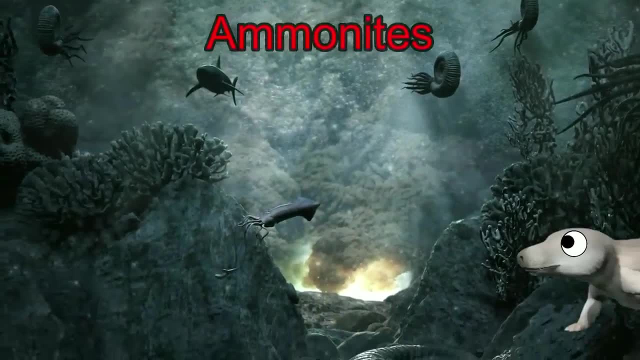 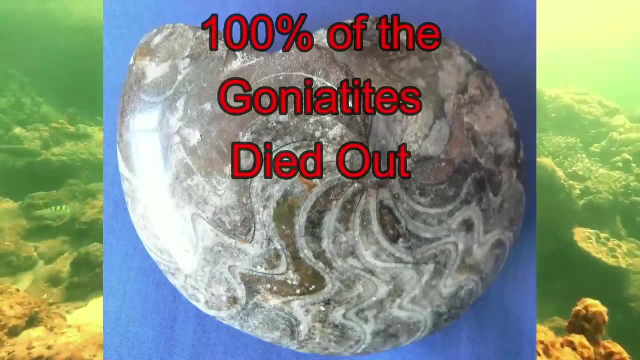 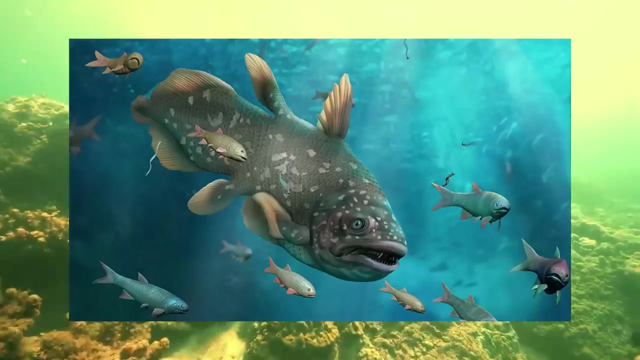 there was one exception, the ammonites, And unfortunately the news wasn't good. 97% of them would completely disappear, including 100% of the goniotites that we talked about being super abundant during the Devonian Several. groups of vertebrates were wiped out, including many species. 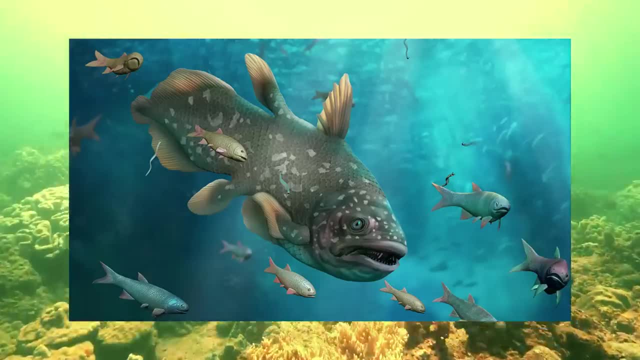 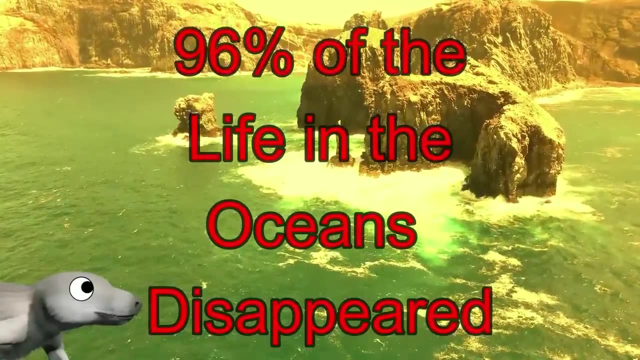 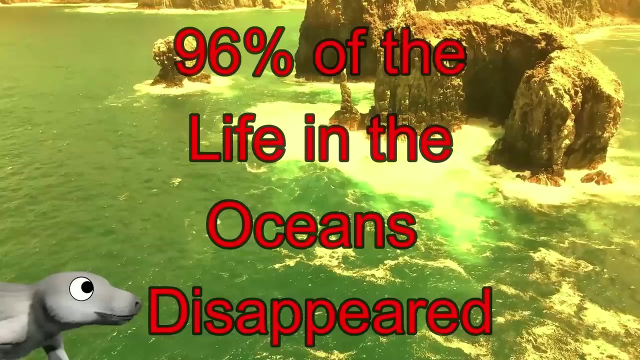 of conodonts, bony fish and chondrichthyans. All in all, an absolutely unfathomable 96% of the genera that existed 252 million years ago would be gone in the million years or so that this event took place. 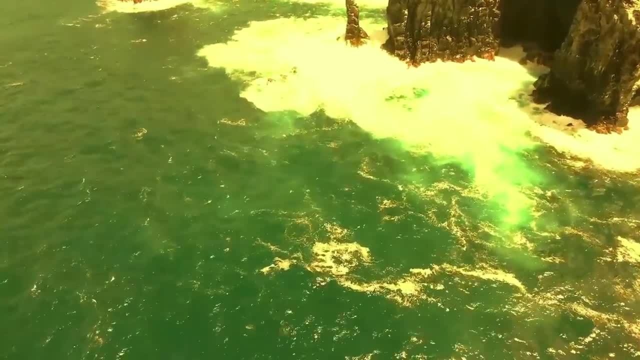 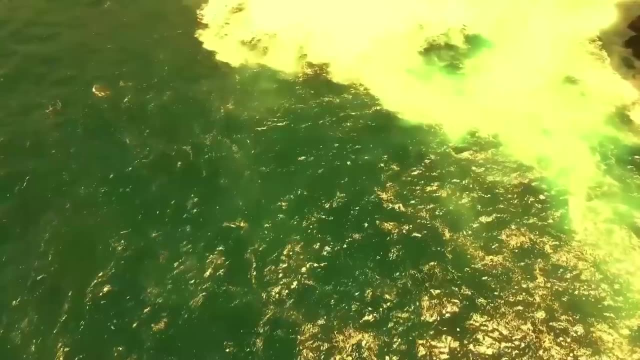 Leaving the majority of the globe, looking very similar to how it did in the days before the Ediacaran, covered in a vast barren ocean. Although the loss of life on land was not quite as all encompassing as it was in the oceans, it was. 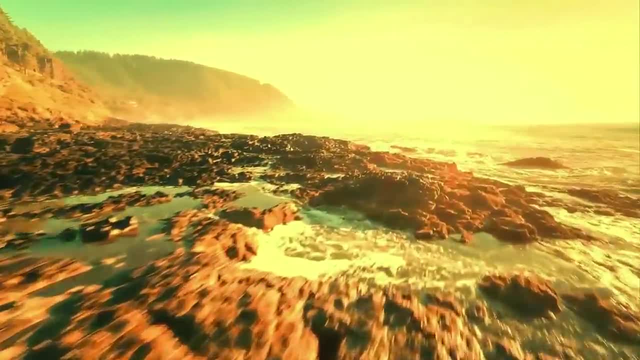 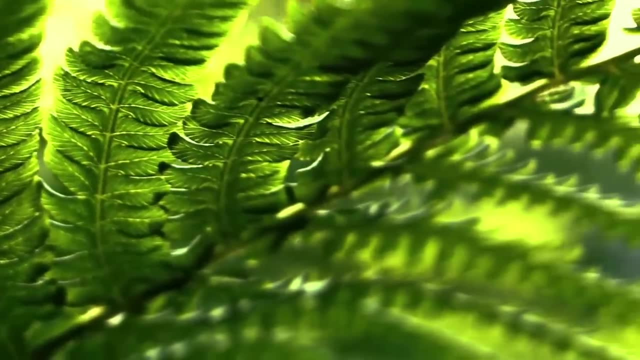 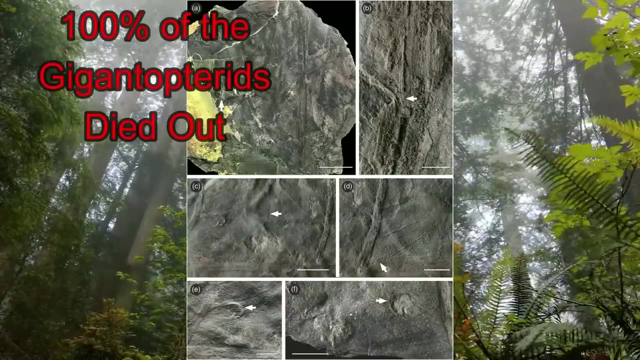 still absolutely devastating. There was a steep drop off in many different kinds of gymnosperms and seed ferns. Also the total extinction of another group of plants called the gigantopterids, which had previously made up the most abundant types of plants in the rainforest of the South. 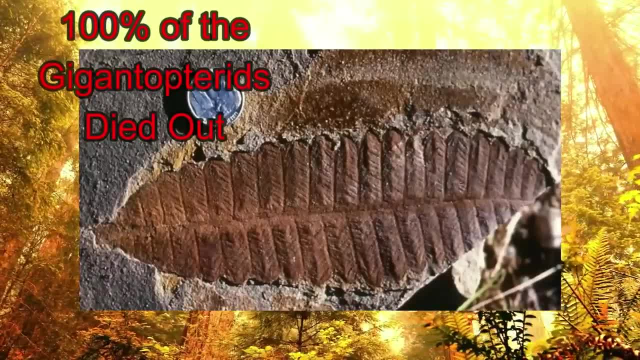 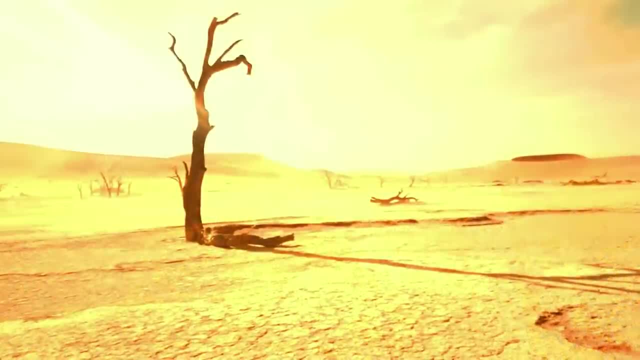 China islands. Although many species of the chondrichthyans could still remain, there were few exceptions, Although some smaller species may have survived. this was the end of this type of forest, And the collapse of the coastal forests would result in many species disappearing. 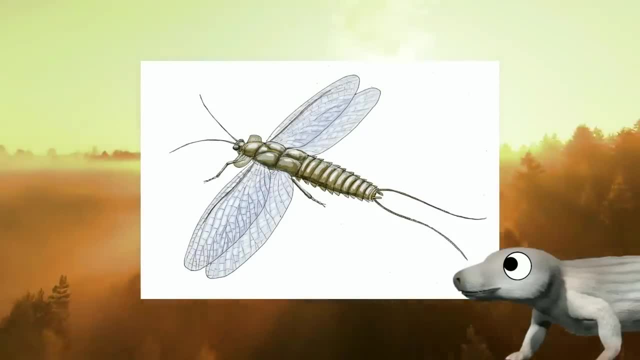 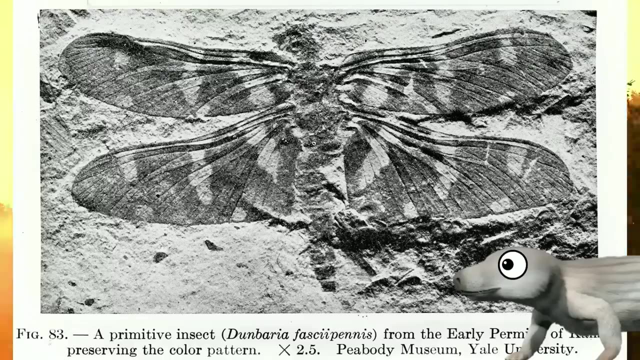 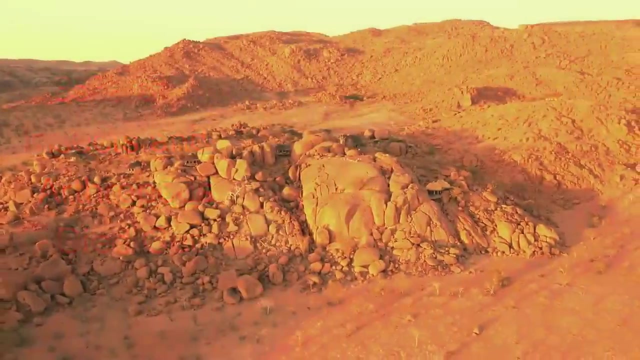 The land, invertebrates would not fare much better than the marine ones, with this being the single largest extinction event that insects have ever suffered, with some estimates as high as 85% of terrestrial arthropod genera disappearing, And since both plants and invertebrates make up the base of any terrestrial food web, 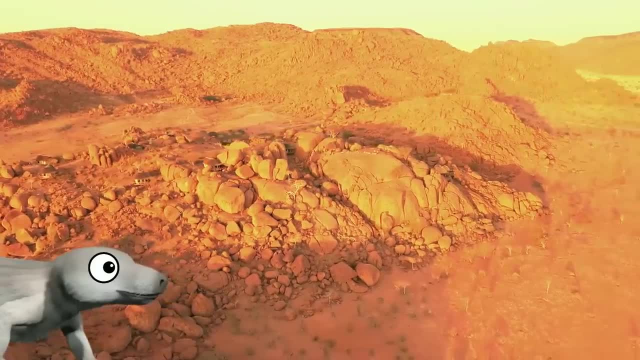 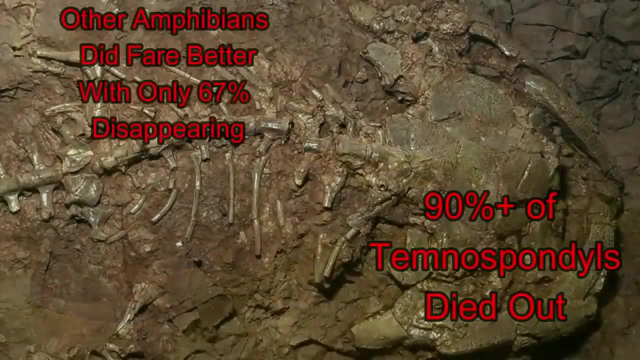 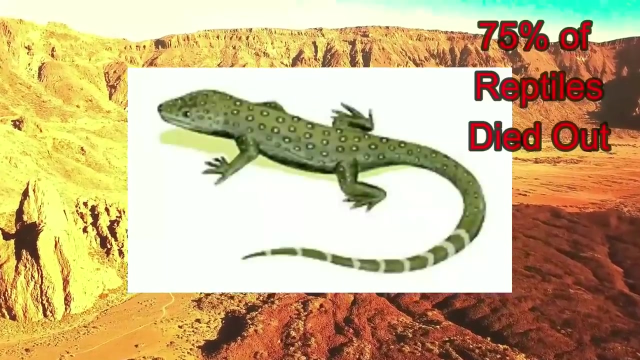 this was absolutely going to have a dire effect When it comes to the vertebrates. amphibians like the temnospondyls were almost completely wiped out, weakening their grip as the dominant hunters at the water's edge Many different groups of reptile that had been competing with the synapsids directly. 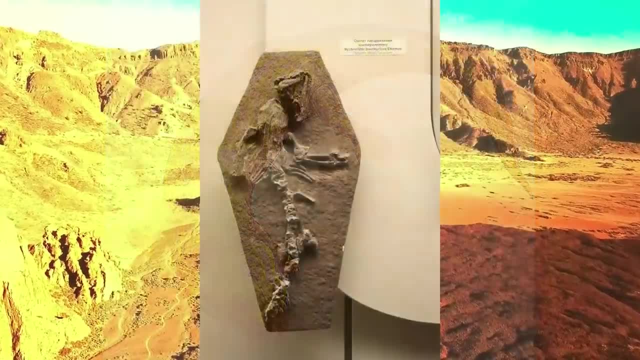 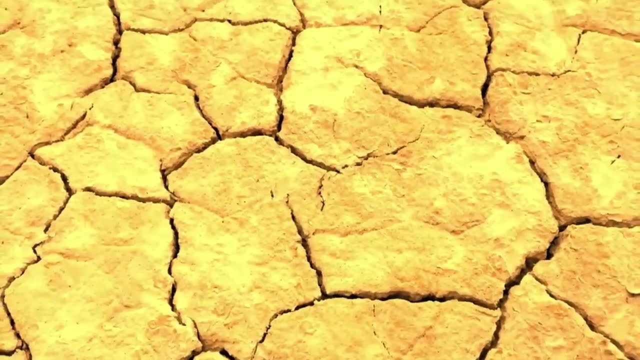 had been reduced in diversity or completely driven to extinction. Most notably was the para-reptiles like Scutosaurus. But, as I've said before, when there's a collapse of a food web, it's always the animals on top that fall the hardest. 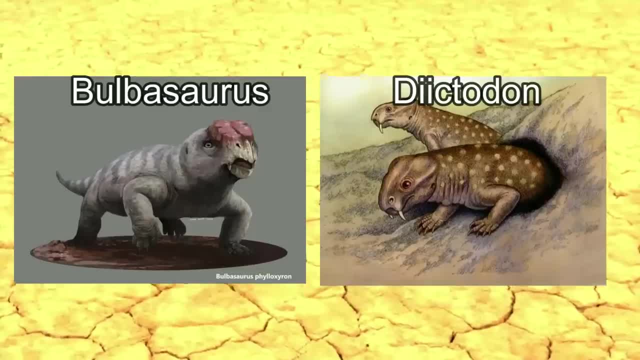 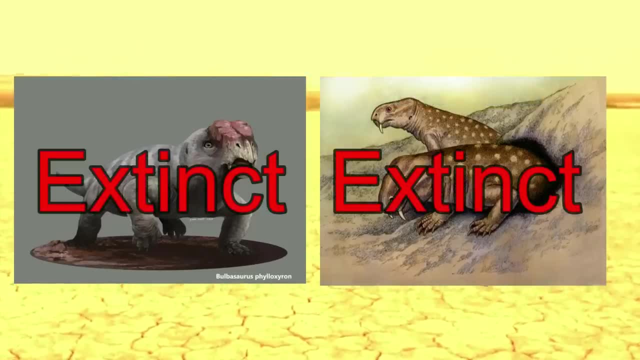 And this time that was the synapsids. Many of the different species of Dicynodonts, like Bulbasaurus and Dictodon, would not make it out of the Permian alive, And without the forests, neither would Souminia or its neighbor Solaris or Ravis. 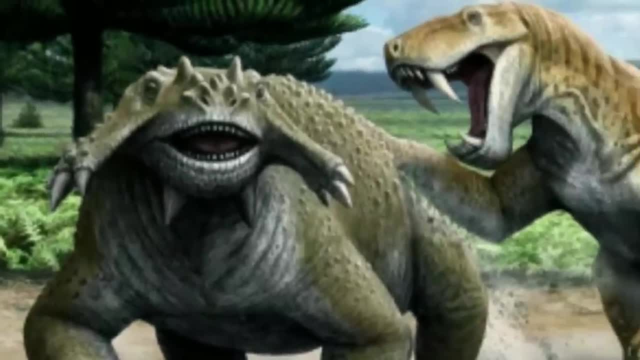 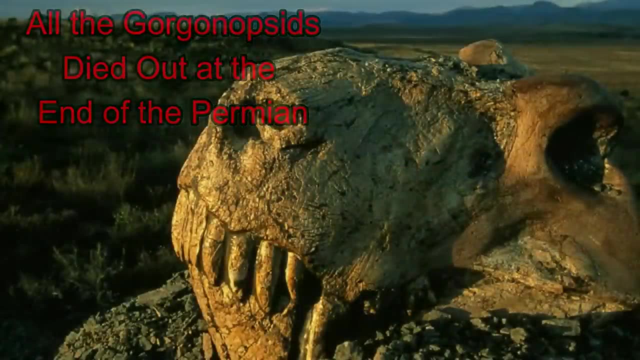 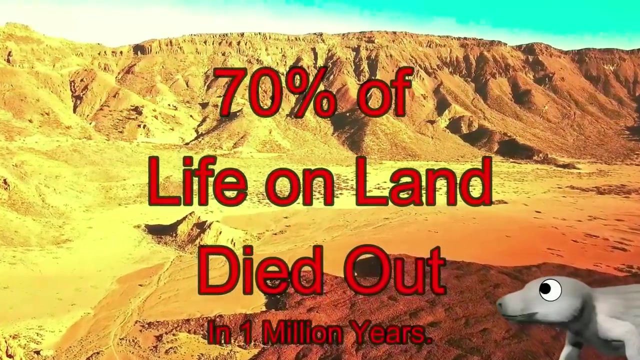 But one of the hardest hits would be the Theriodont carnivores, With all of the Gorgonopsids and almost all of the Therosophalians dying out. 70% of life on land would be taken out over the course of a million years. 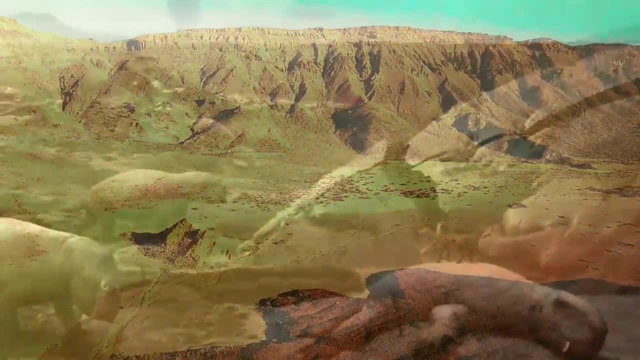 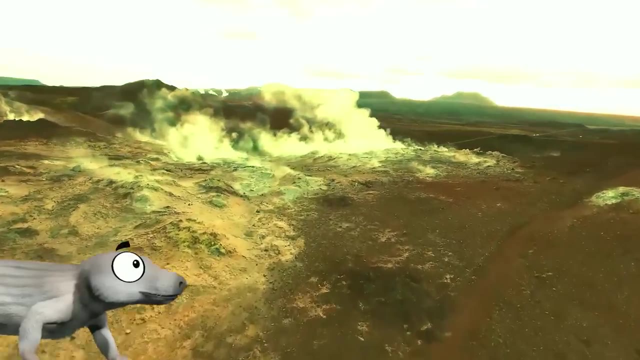 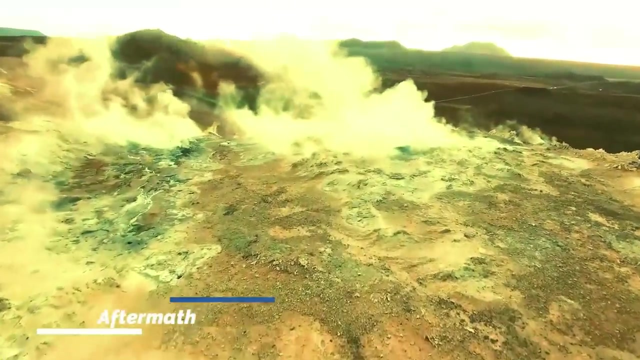 Leaving our planet a barren, lifeless husk of what it had been seemingly last week. But as bleak as this situation seemed, there was still a very slight sliver of hope. Life on this planet would never be the same. We talk about this event being the 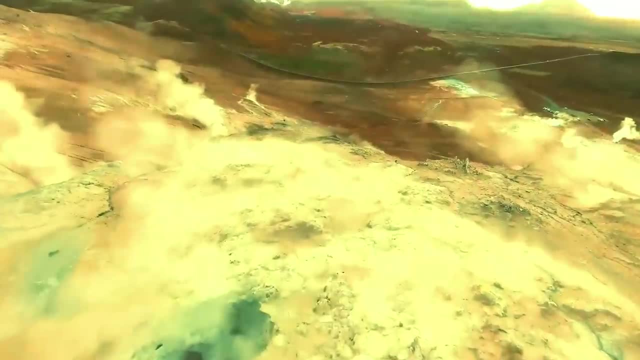 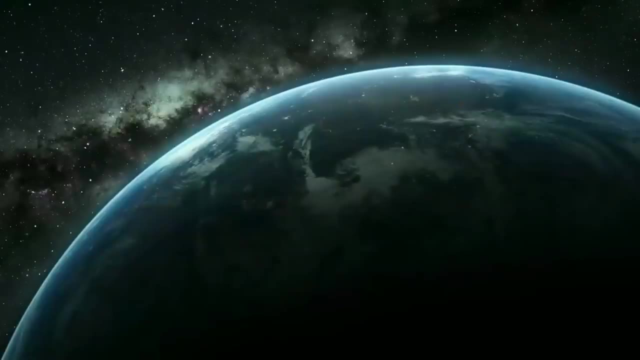 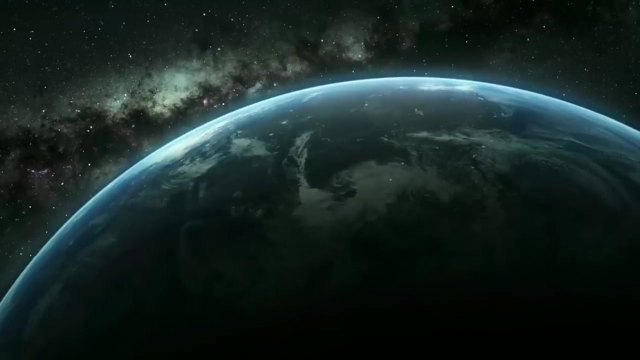 moment when the synapsids lost control of the earth to the diapsids. but the reality is: nothing alive at this moment was doing well. The animals that would make it through this time were the generalists who were going to have to scrape just to get what they needed to get by As the dust. 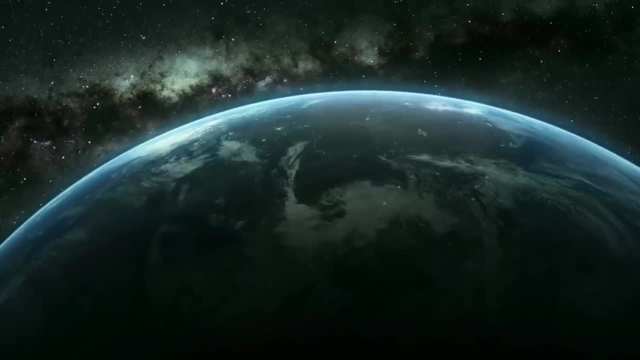 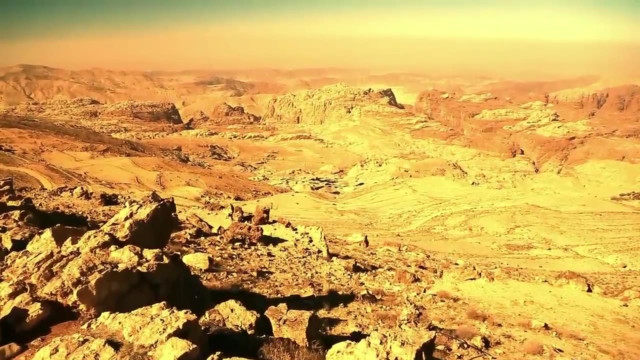 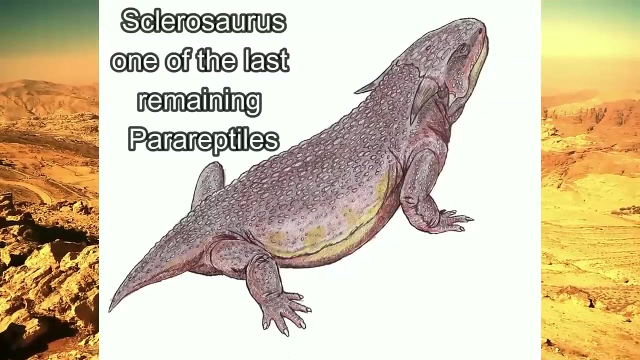 settled. the world that would be revealed, would be a truly sick planet. It was dry, hot and barren, with many of the areas that had previously been able to grow forests succumbing to desertification. But a few animals were hanging on, For one thing, the Dicynodonts, and more specifically 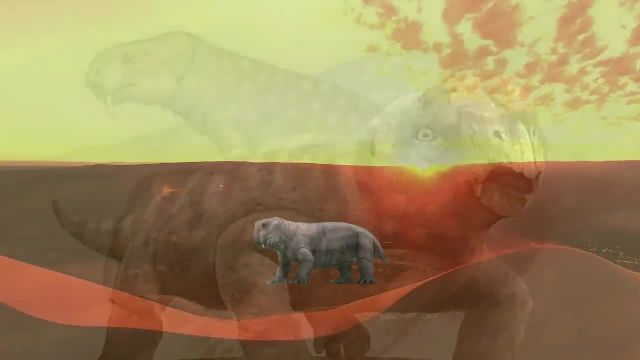 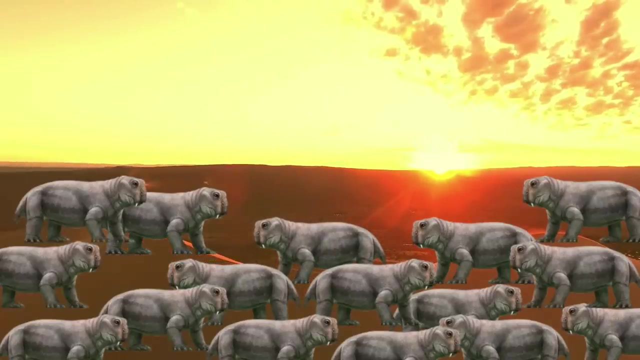 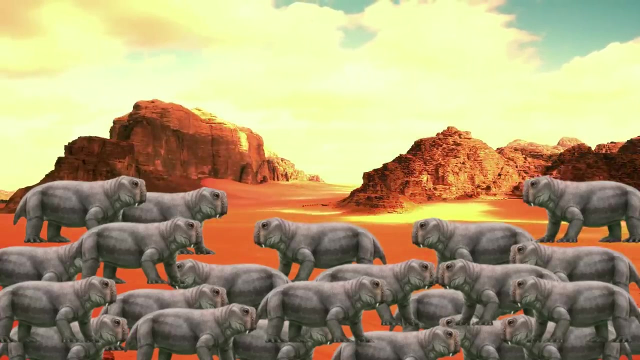 Lystrosaurus, who, despite seeing many of their cousins perish, were about to boom in population across the southern half of Pangea Going into the early Triassic. Lystrosaurus was the single most common species on earth For a while: 95% of the land. 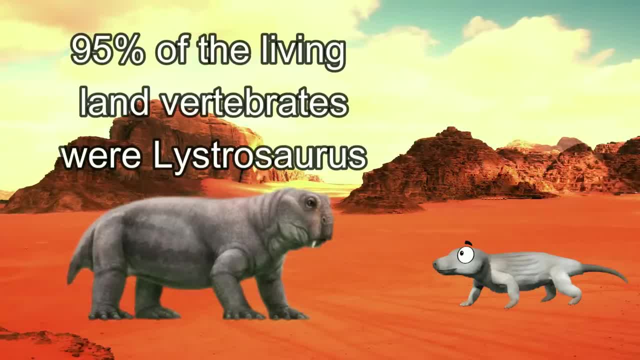 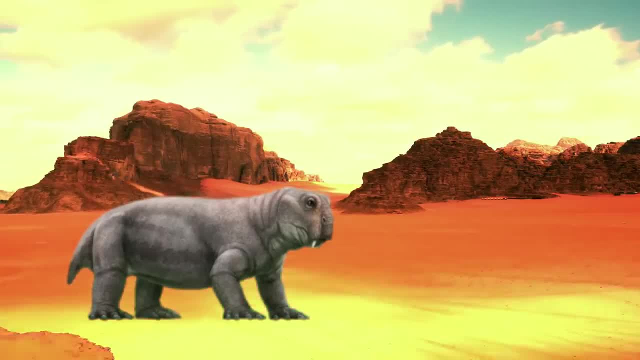 vertebrates were these pig-sized stem mammals, A biodensity that, to this day, cannot be rivaled by any species, Not to mention Lystrosaurus and Lystrosaurus. However, the Dicynodonts were young and more than 50% of their population had died along. the way. Just as much of the Dicynodonts would have no future, But the former would struggle to gain anything resembling the apex predator status they had held in the late Permian. The Dicynodonts were likely able to hang on by staying small. 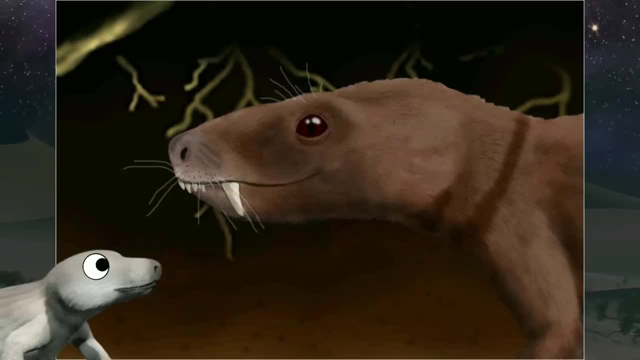 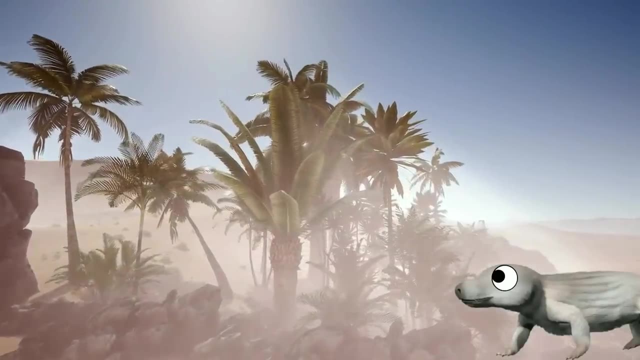 and not needing as much food as the Gorgonopsids and Therizophelians, A strategy that would carry them through the next era of Earth's history. In the cease I said: you're going home, but you're dead. 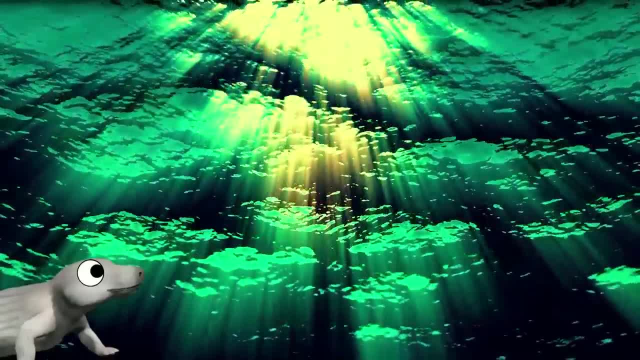 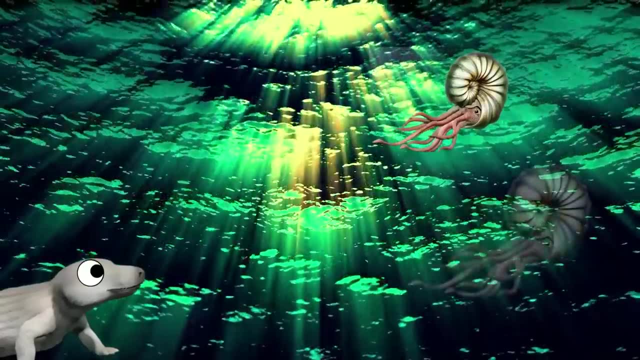 Yes, I know, And that's what I meant by the end of the video. It's been a while, so I hope it made sense. life was broken, but the small four or five percent of what was left of each of the different groups would eventually start to rebuild, But it would take a. 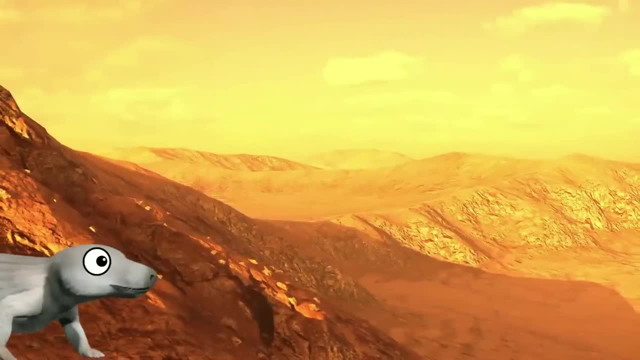 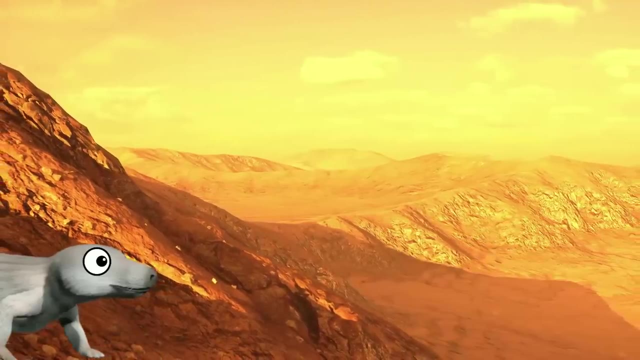 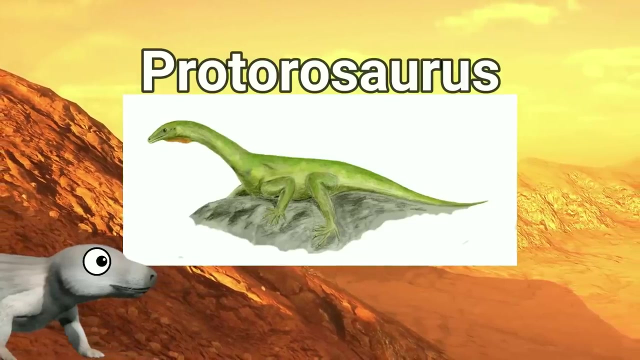 long time, and although it's hard to see this as anything else other than doom and gloom, there was one group of animals that would eventually stand to benefit from this great dying. Allow me to introduce Protorosaurus. This is a seemingly unassuming diapsid reptile, not unlike many that we have already met. 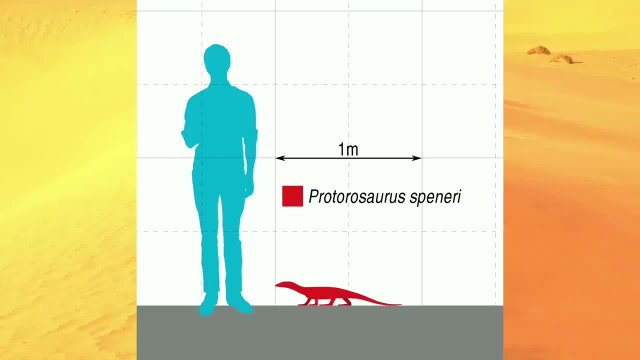 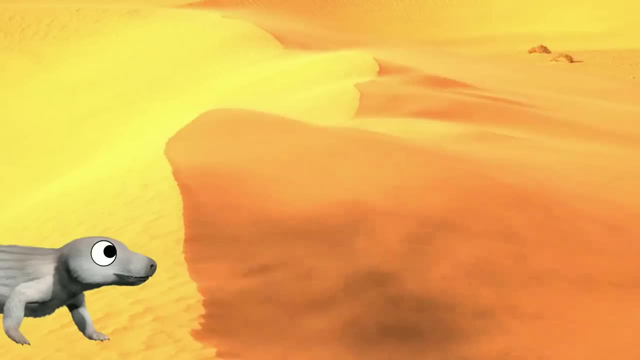 before, But this one might be different, because this reptile is actually the most primitive member of a clade of reptiles called the Archosaurs, and, with so many players being wiped off the board, this would be the face of things to come. 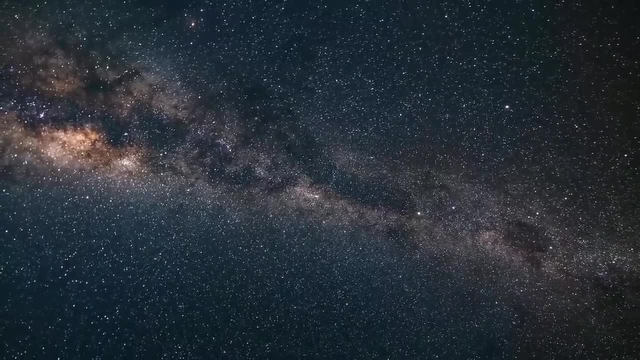 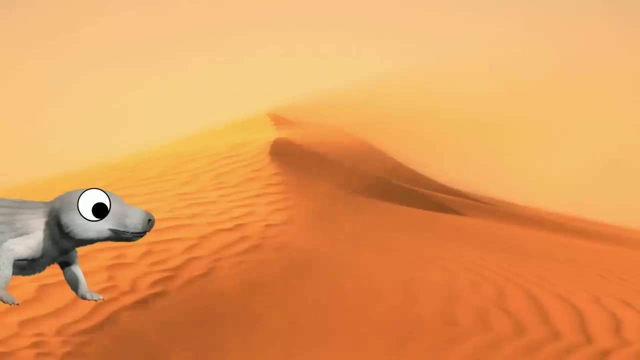 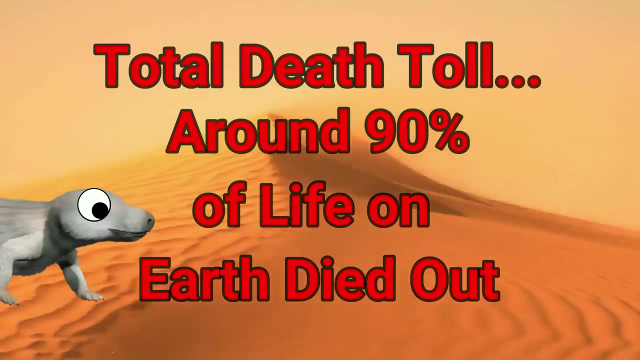 This is the closest our planet has ever come to, going from a gem thriving with life in our galaxy to a desolate world like Mars. All in all, around 90% of the species that were alive in the Permian were gone, But luckily from a small handful of hardy. 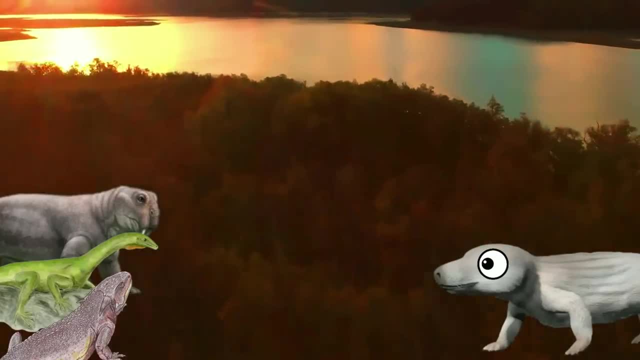 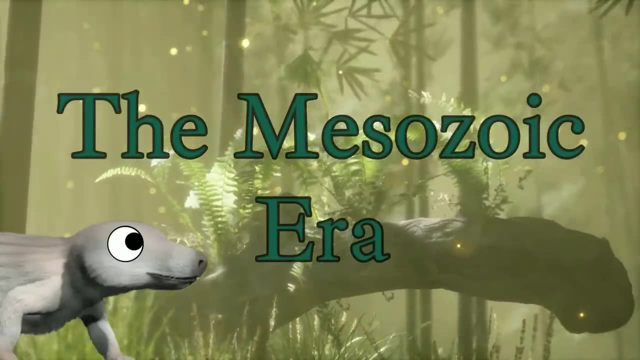 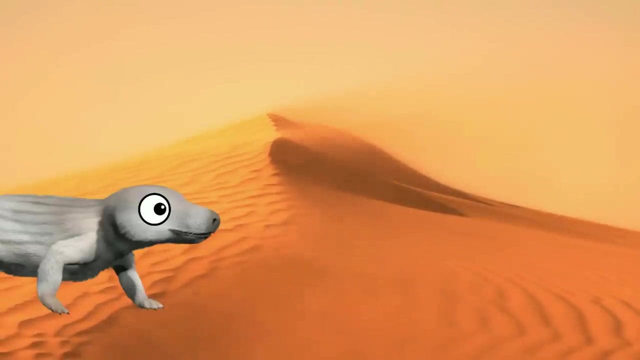 survivors. somehow life would bounce back, But it would be forever different, because from here on out we are in the Mesozoic era, But today our Earth is wounded and it will take time to recover. If you enjoyed this video, I highly recommend watching the 10 previous episodes of this. 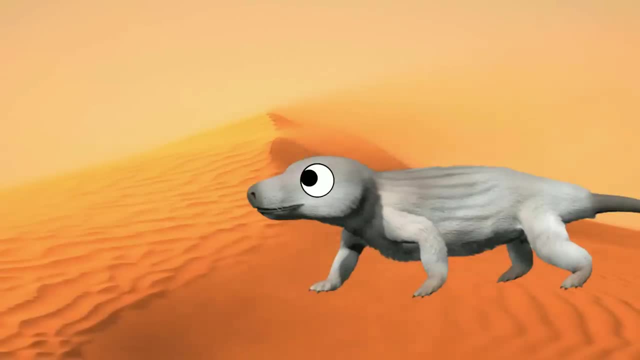 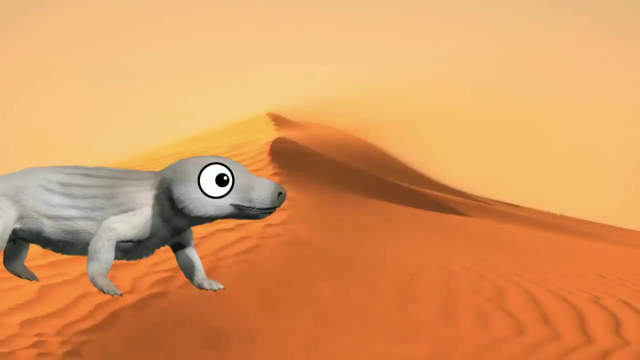 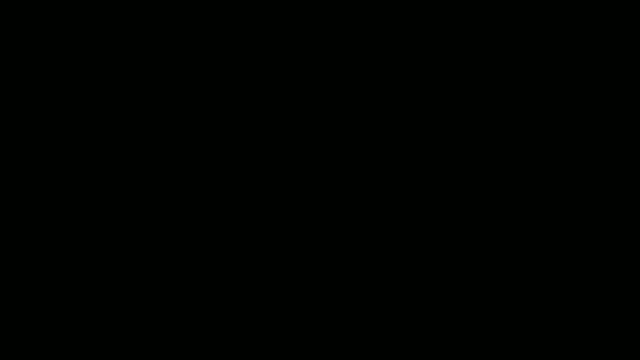 series so far. I fully intend to keep going with this until I get back to the modern day and my human form, and I want to thank you all for joining me on this journey. Have a good one, everybody. Subtitles by the Amaraorg community. wwwamaraorg community.